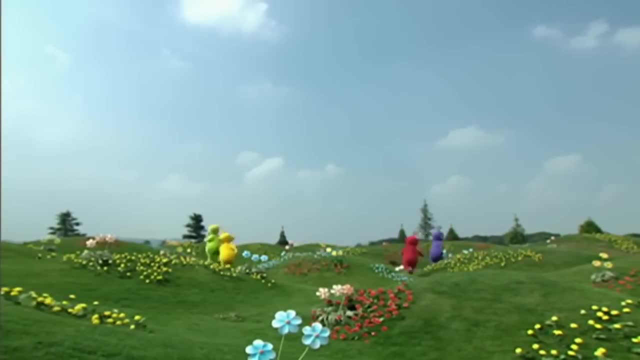 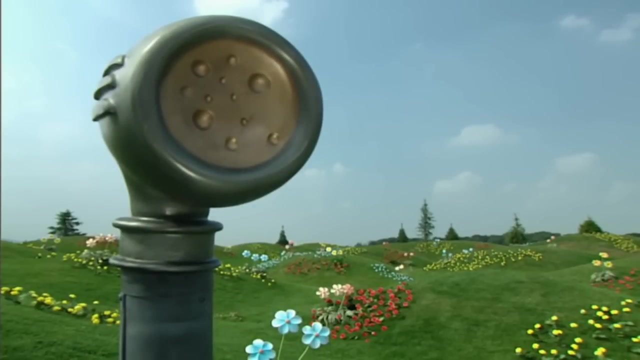 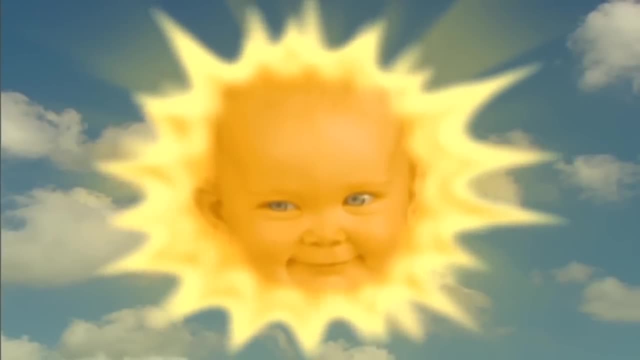 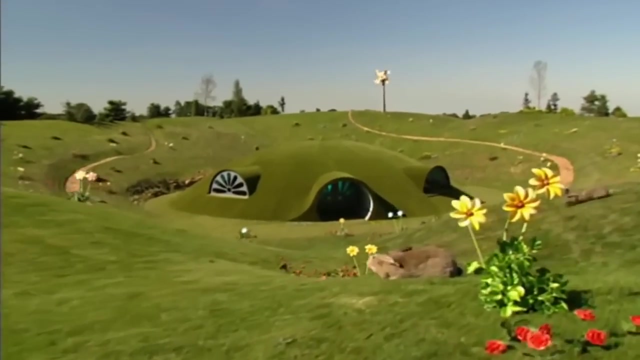 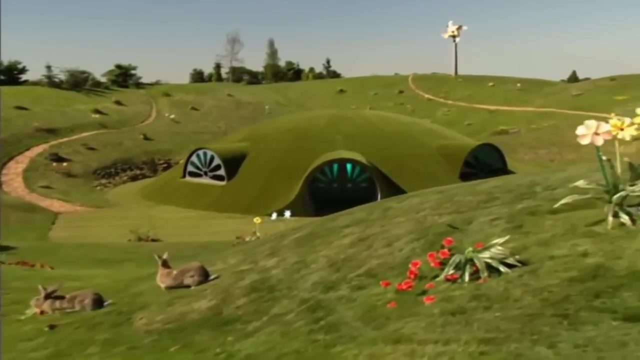 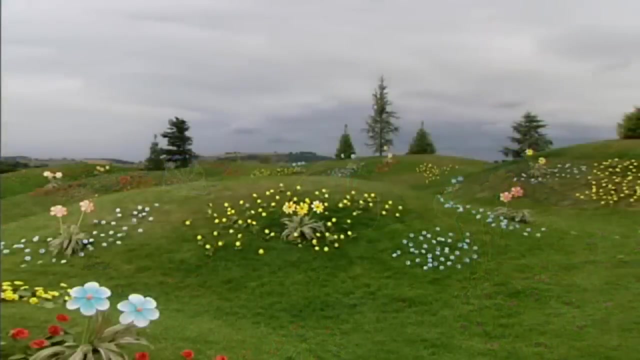 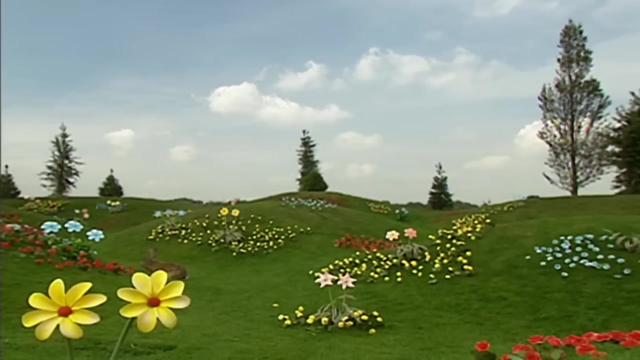 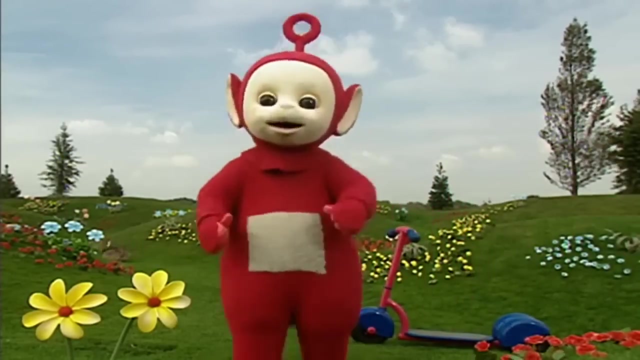 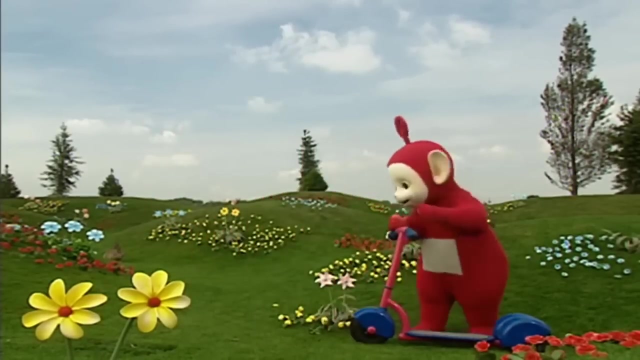 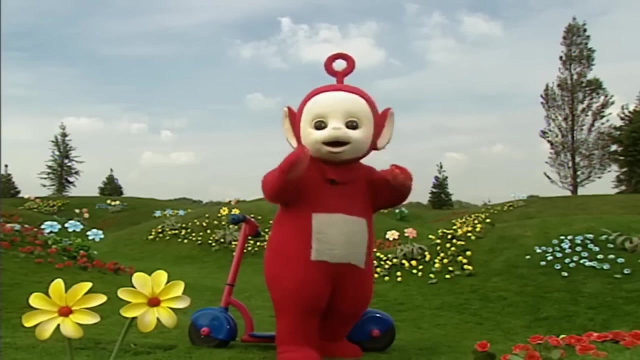 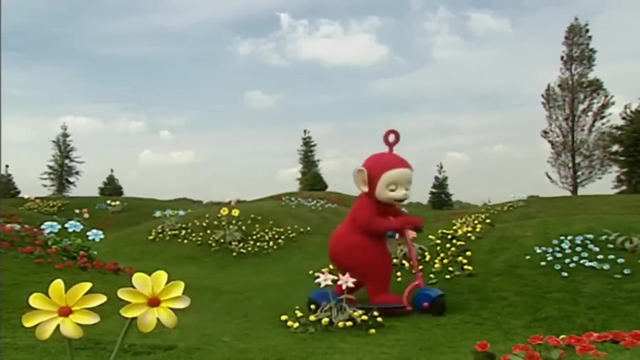 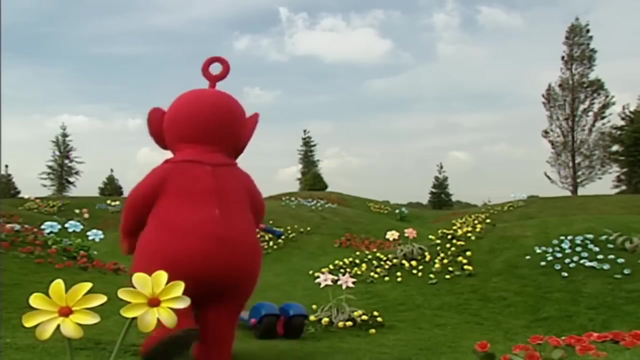 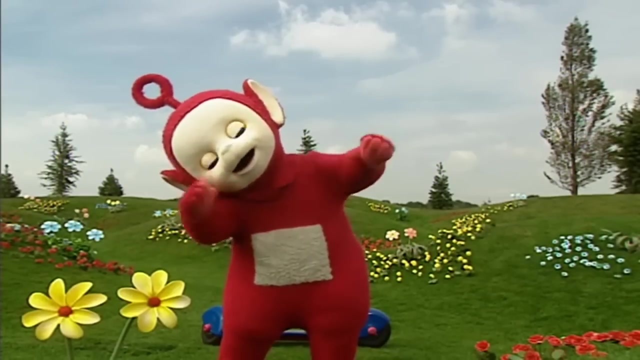 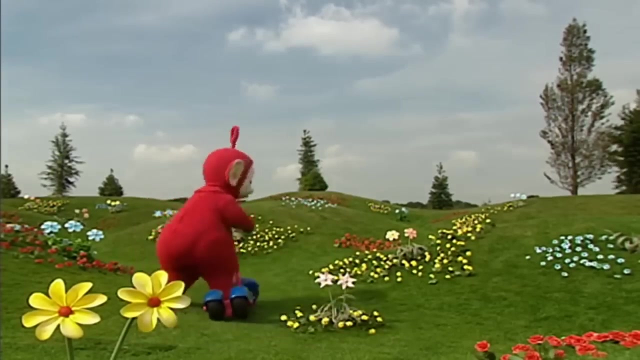 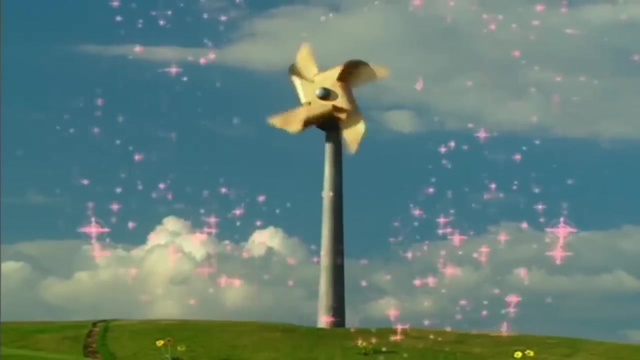 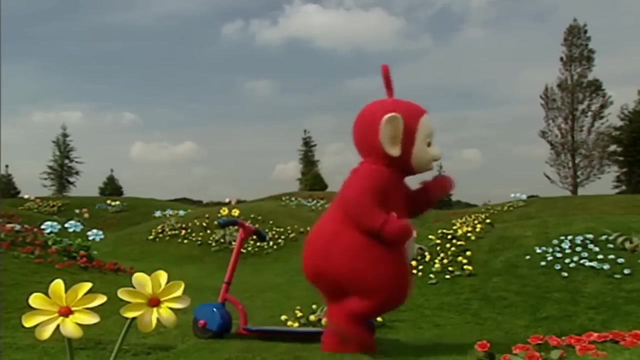 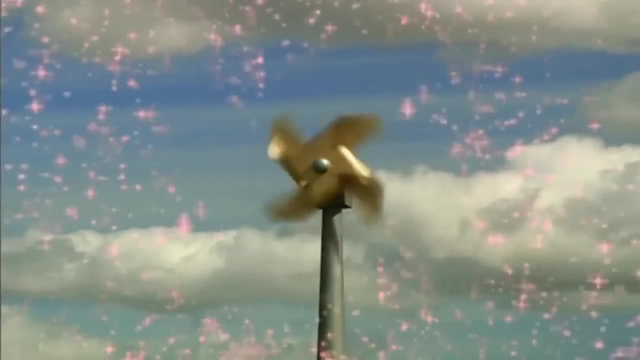 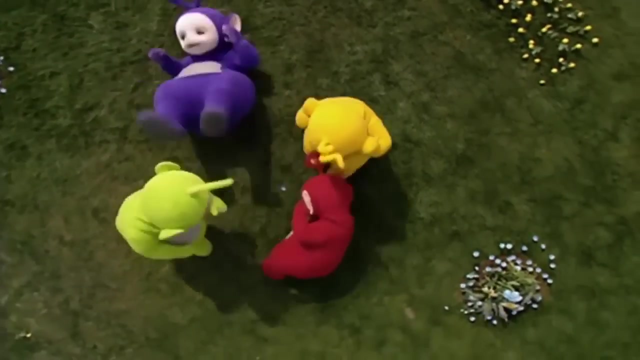 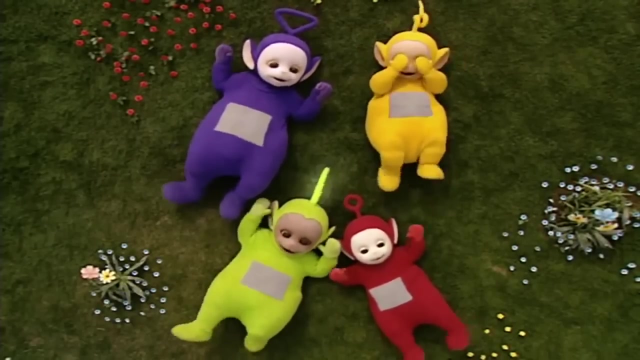 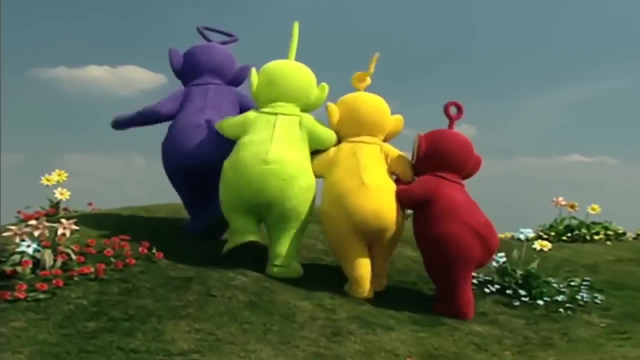 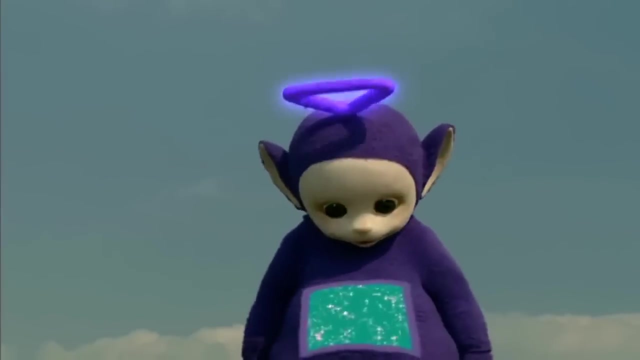 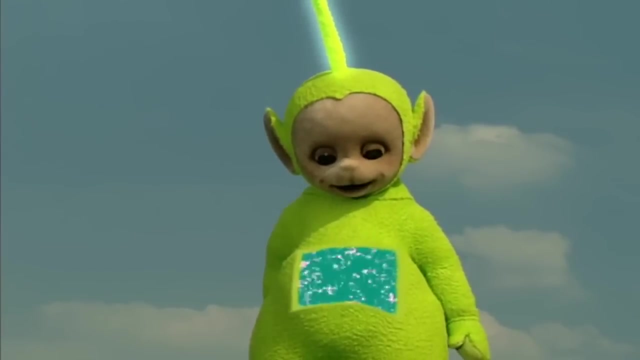 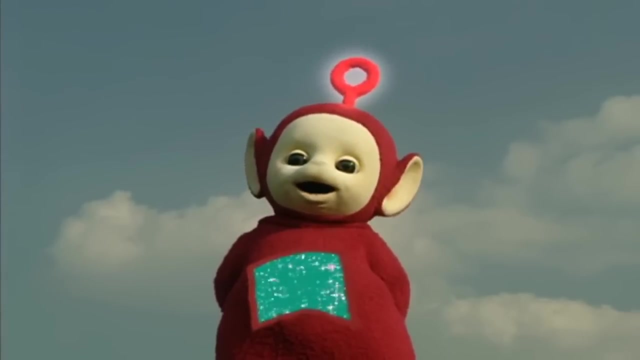 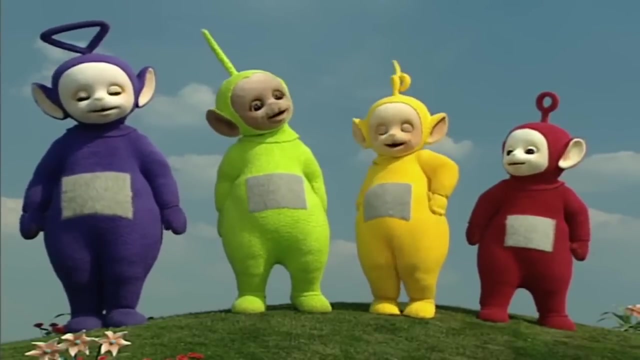 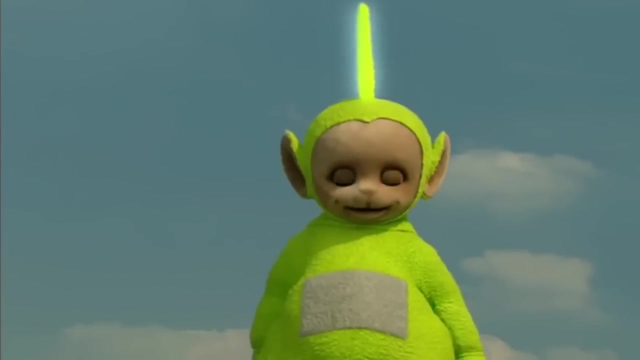 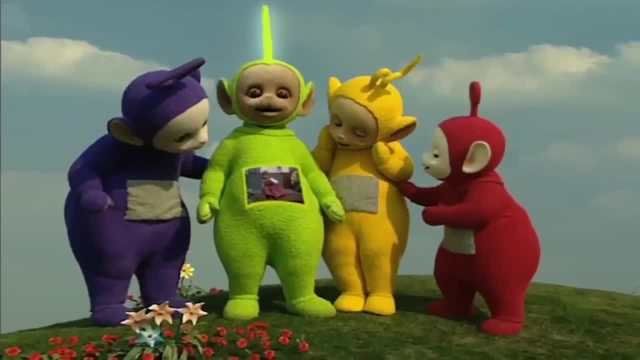 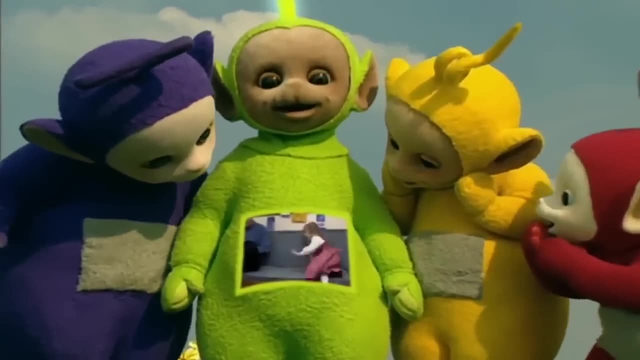 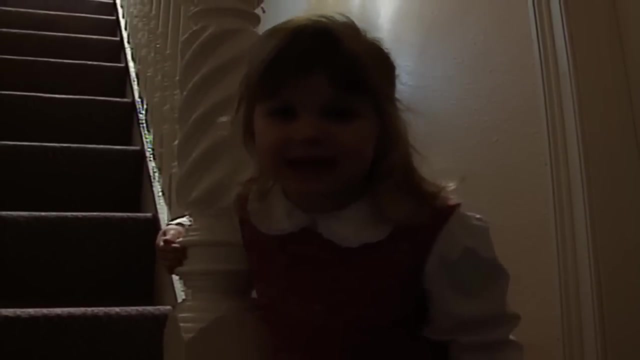 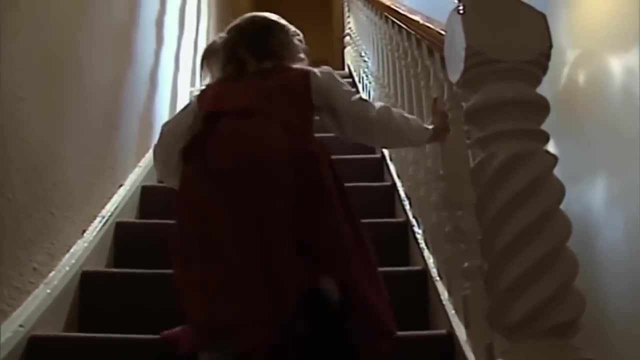 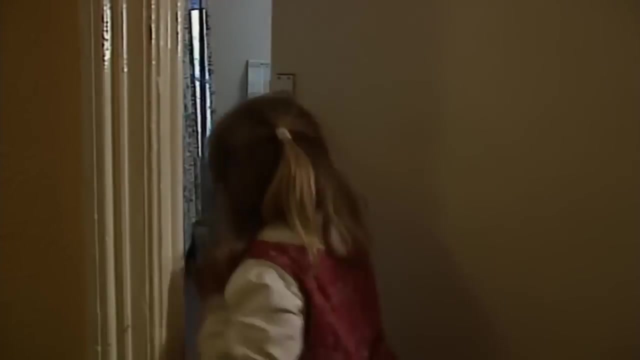 Hello, Hello, Hello, Hello, Hello, Hello. my name Jenny. Come and meet my mummy. My mum is a doctor, And if you're poorly, she makes you better. Have you finished that, mummy? Not yet. Why don't you come and sit down while I just finish what I'm doing? 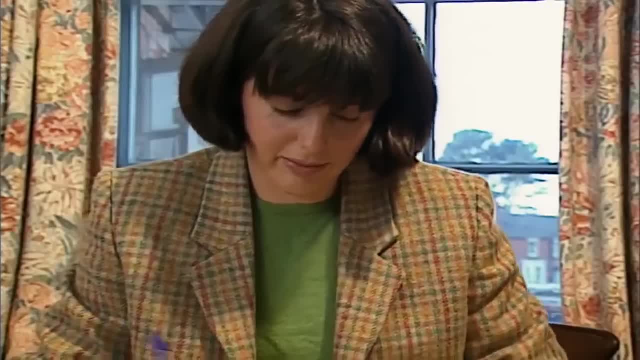 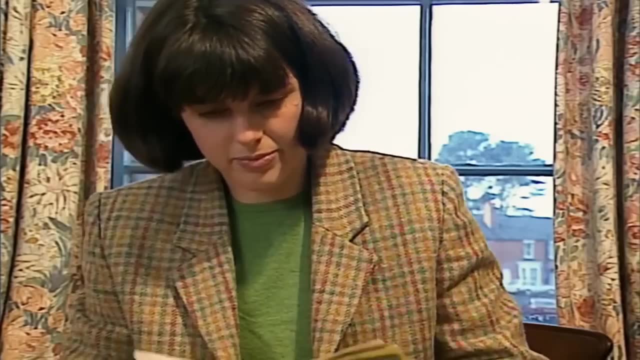 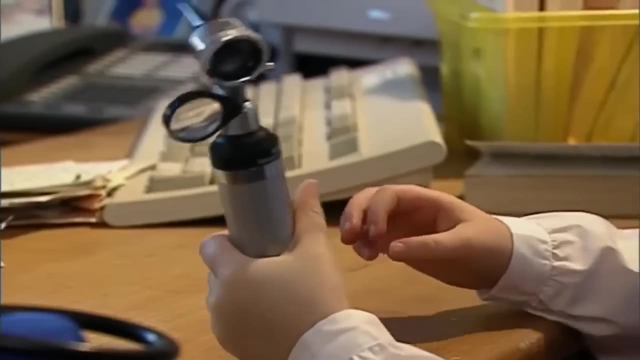 My mum is a doctor. When you're not feeling very well, first of all you're going to see my mummy. My mum is very special. She can make people feel better. My mummy uses a torch to look in your ears and mouth. 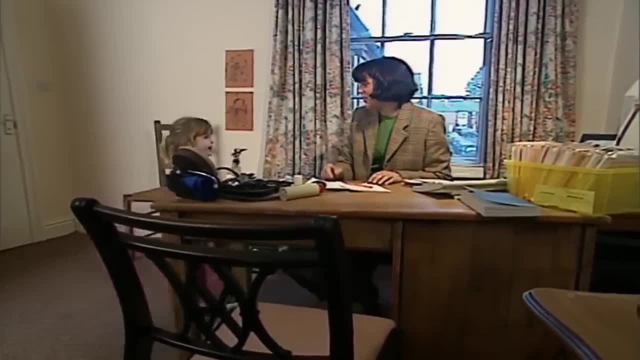 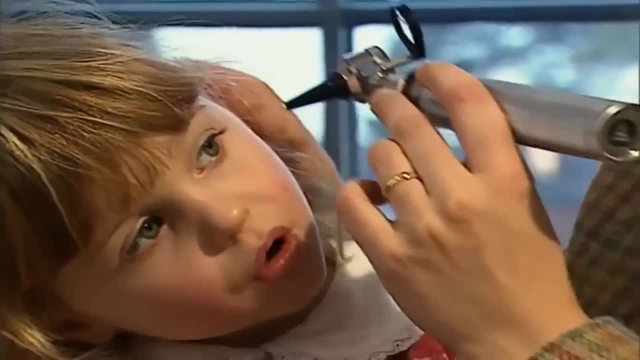 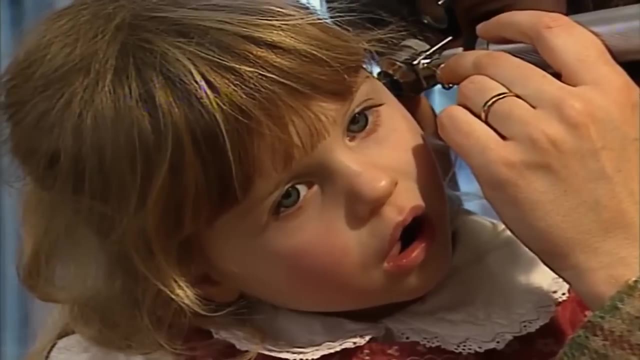 Do you want me to check yours for you? Yeah Shall, we Let's have a look. Tilt your head like that, Shine this torch in your ear And we look to see if it's red, Because sometimes, if ears are poorly, they go very red. 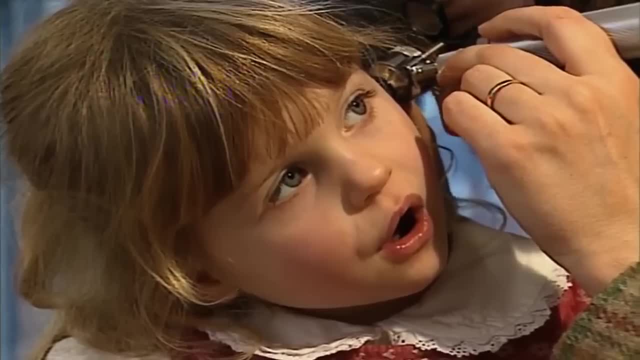 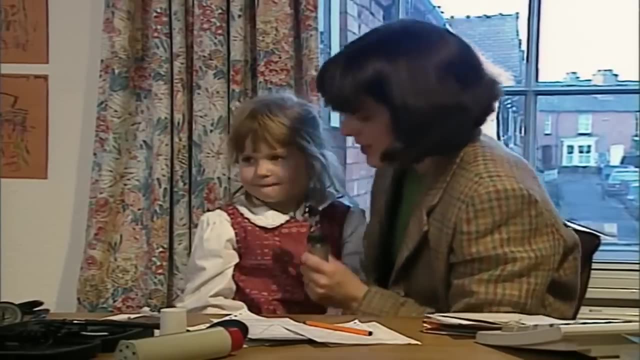 And then we can give people some medicine to make them better. That one's fine, though When children come and they're poorly, do you know what else we have to look at? Well, we look at their throats to see if they've got poorly throats. 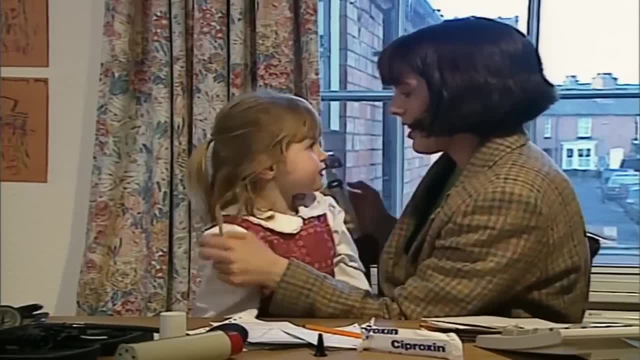 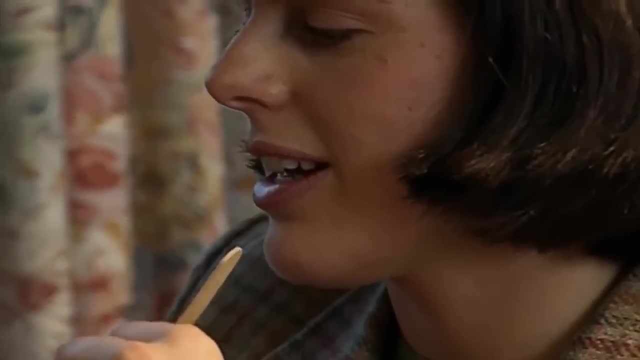 Shall, I show you what I do. Can you turn around and look at me? That's it. And you say Ah. And you tilt your head up so I can see right down and you say, Ah, That's a good girl. 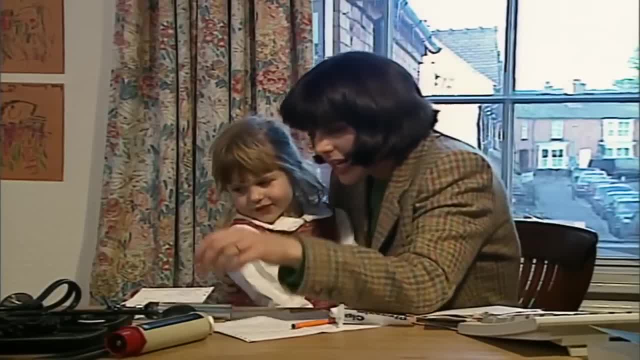 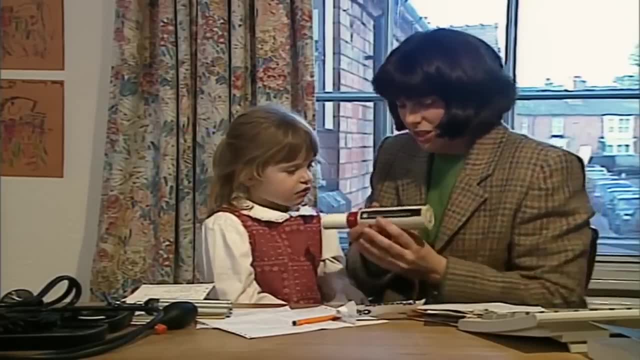 Oh, that looks very healthy. And the other thing that we do is we get them to blow into this special machine. I can do that, Do you? Yeah, Right, So what you need to do is you need to go big blow. 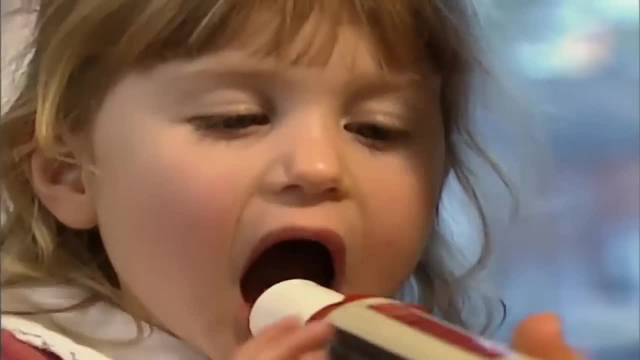 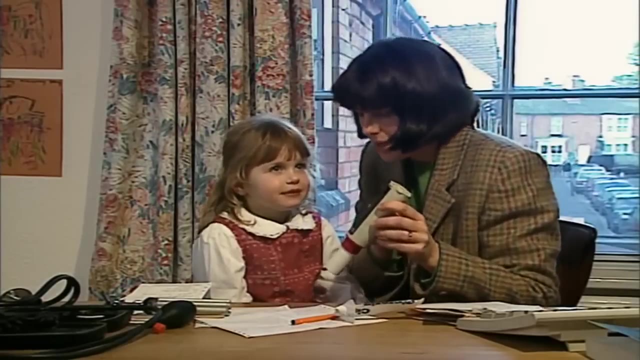 Look, that's good, Right up there, Have another go. That means that your lungs are very healthy. Your chest is very healthy, because you can blow that all the way up there. That's very good. Well, I know, Mummy, Do me a tum-tum check. 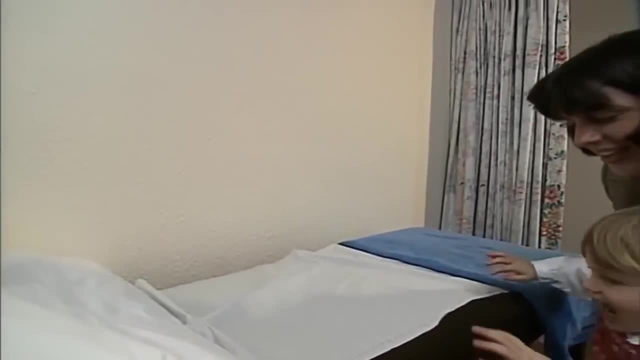 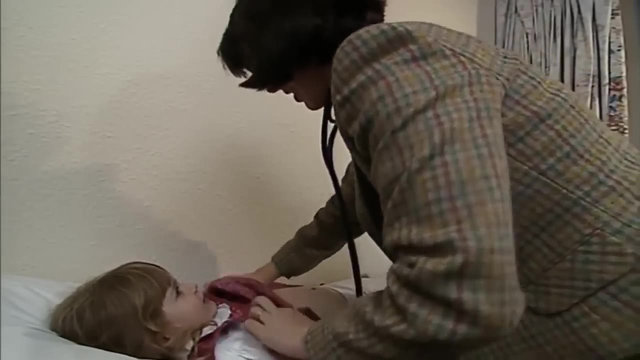 OK, Let's go and check your tummy. That always makes me giggle Up. you go Right, Lie down. Shall I listen to your chest first. Listen to your breathing. That's it There. Have a listen with this. 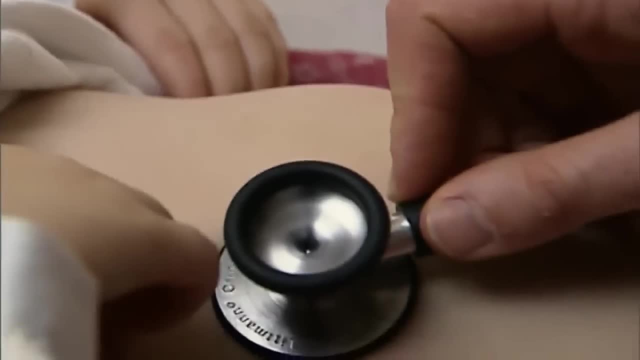 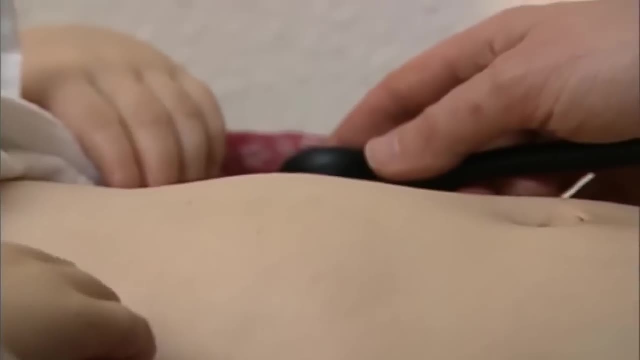 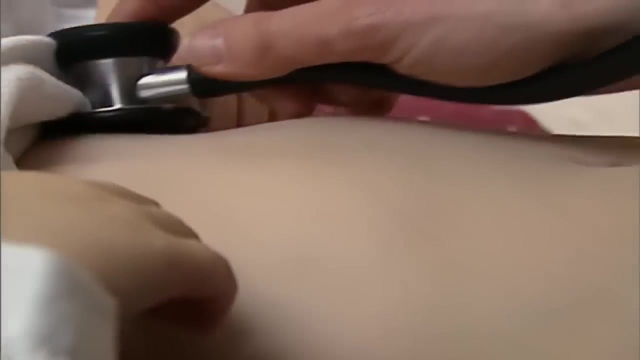 Big breaths in and out. That's it. Nice and slowly, Good girl, And again, And again And again. When Mummy does a tum-tum check, she listens to a noise with a stethoscope. She can listen to noises in your tummy. 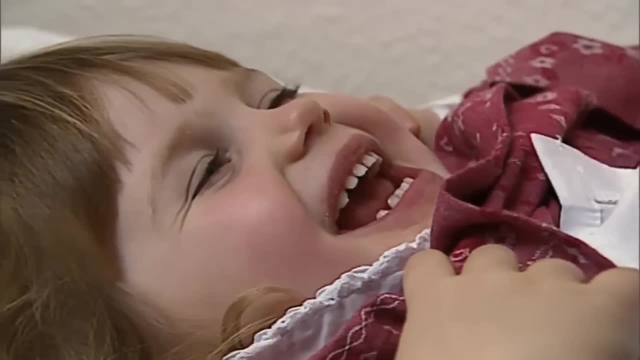 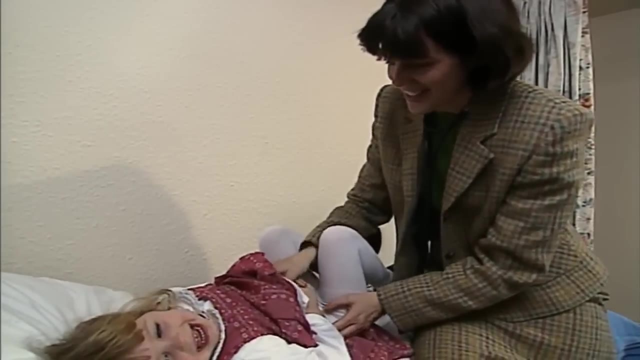 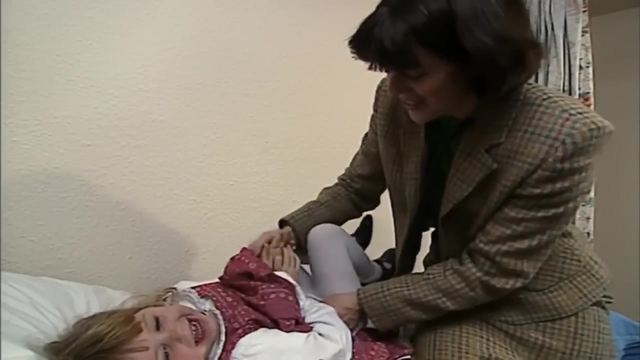 And again: OK Shall, we feel your tummy. What can we feel here? Can't feel your breakfast, Can't feel your lunch. You've got a very tickling tummy, haven't you, And it tickles me. I think you're missing, you're lacking your tea. I think you need your tea. 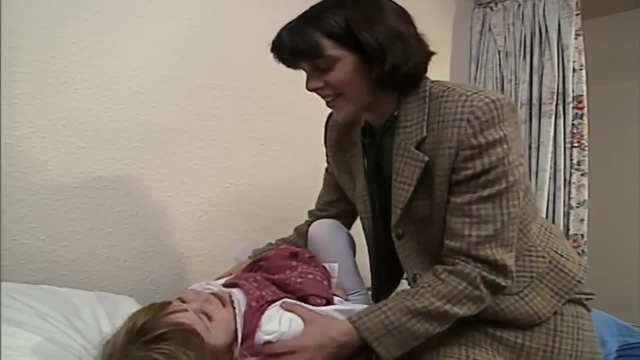 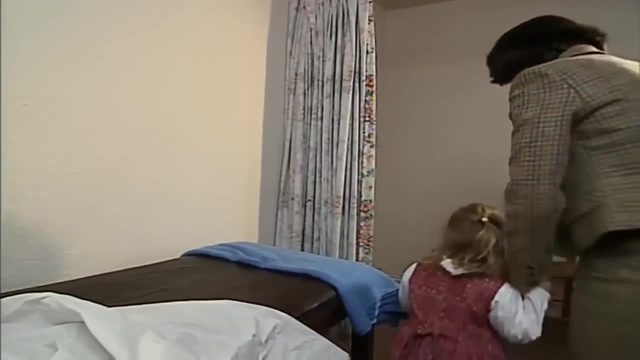 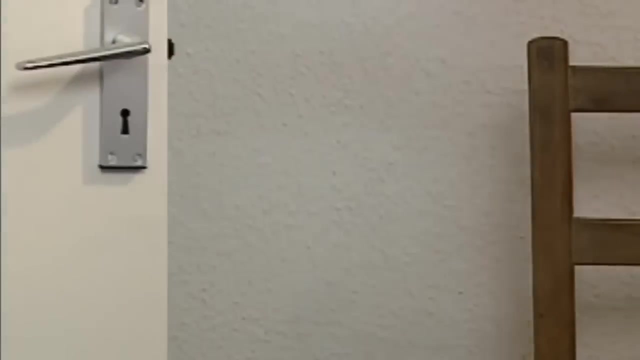 It feels fine. otherwise, Right Shall we take you home for your tea now. Yeah, Come on, then Let's get you down. Yeah, I love my Mum and I love seeing my Mummy when she's a doctor. Bye-bye, Bye-bye. 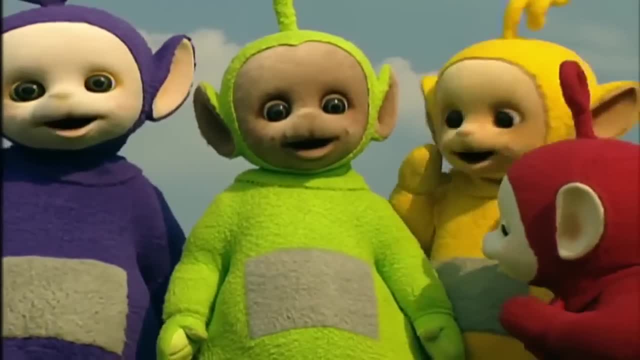 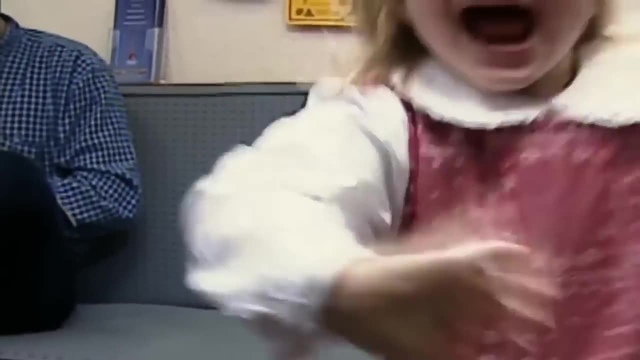 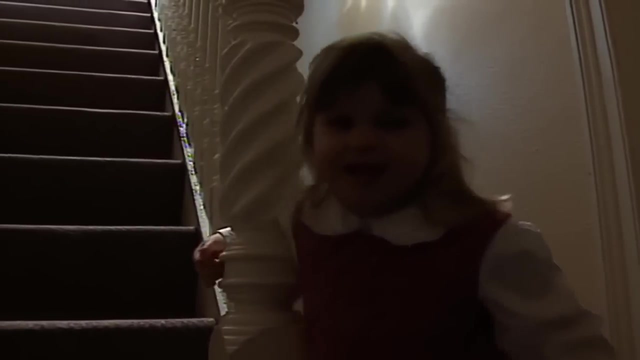 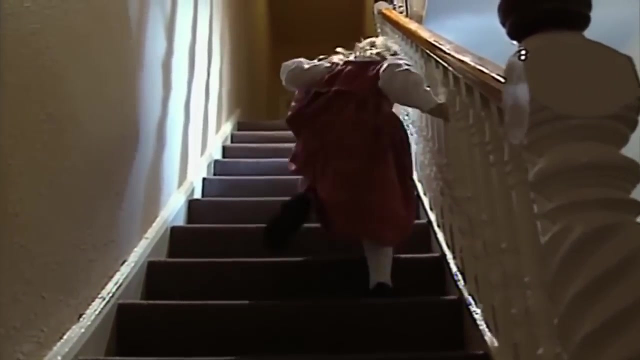 Bye-bye, Aw, Again, Again, Again, Again, Again, Again, Hello, Hello, Hello, My name Jenny. Come and meet my Mummy. Hello, My mum is a doctor and if you're poorly she makes you better. 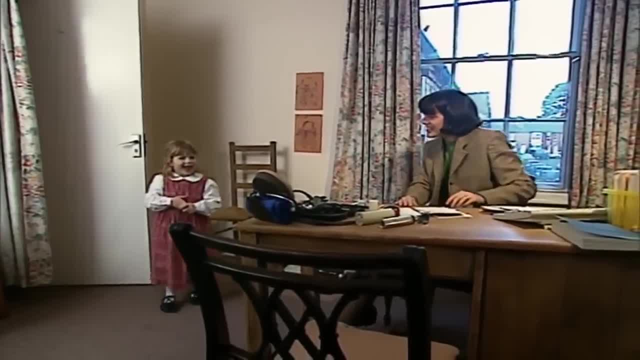 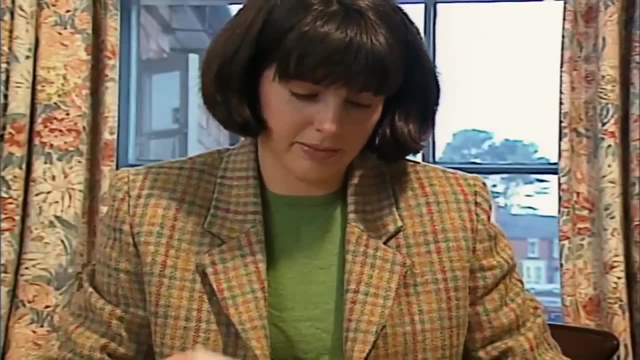 How do you finish that, Mummy? Not yet. Why don't you come and sit down while I just finish what I'm doing? My mum is a doctor. When you're not feeling very well, first of all you're going to see my mummy. 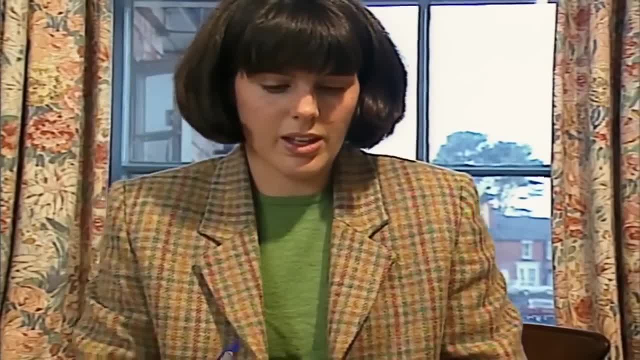 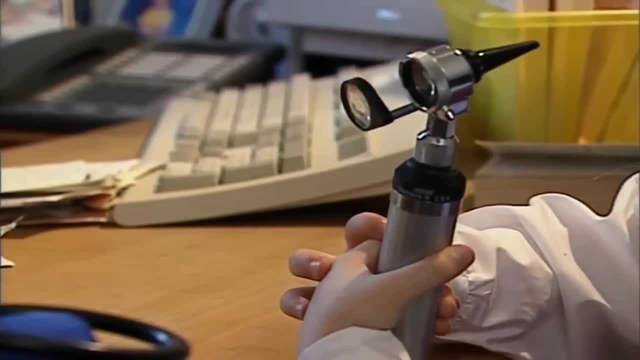 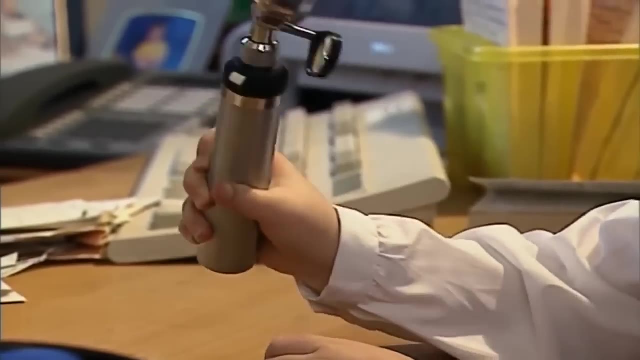 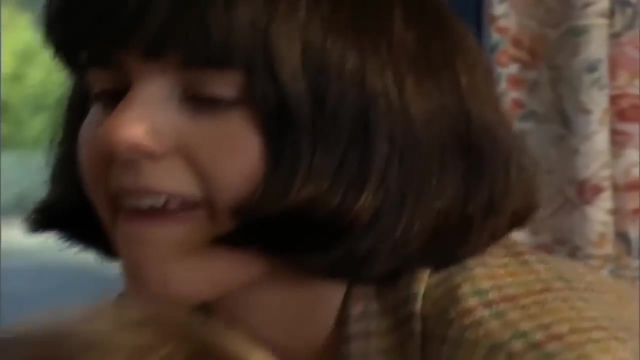 My mummy's very special. She can make people feel better. My mummy uses a torch to look in your ears and mouth. Do you want me to check yours for you? Yeah, Yeah, Shall, we Let's have a look. 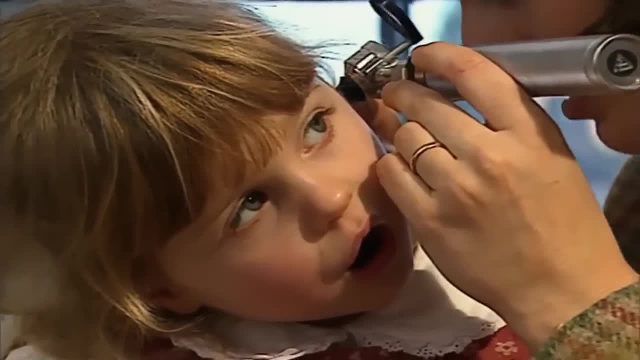 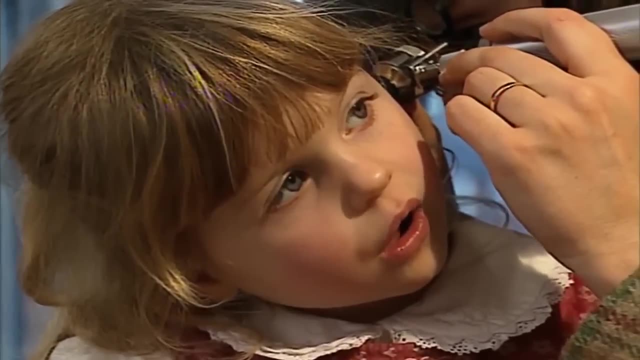 Tilt your head like that, Shine this torch in your ear and we look to see if it's red, because sometimes if ears are poorly they go very red, And then we can give people some medicine to make them better. That one's fine though. 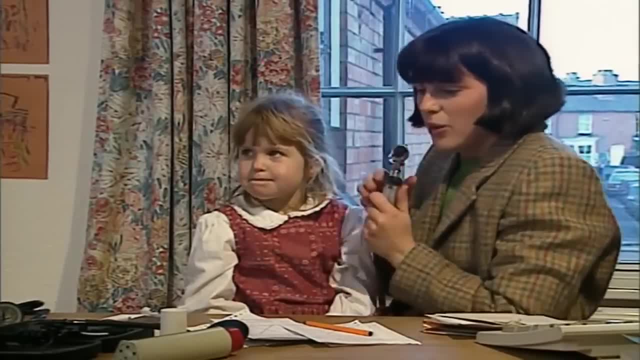 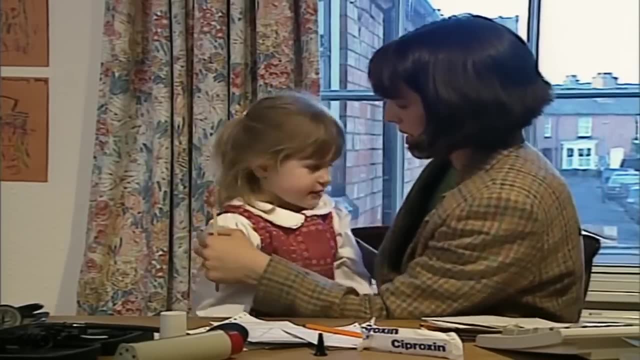 When children come and they're poorly, do you know what else we have to look at? Well, we look at their throats to see if they've got poorly throats. Shall I show you what I do. Can you turn around and look at me? 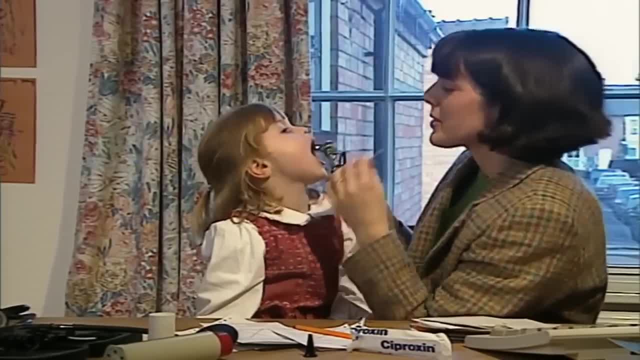 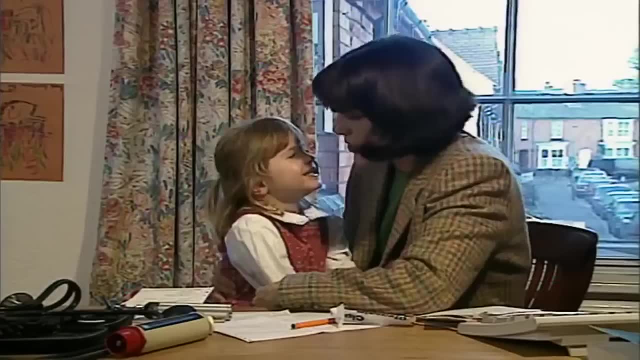 That's it. And you say ah. And you tilt your head Up so I can see right down and you say, ah, That's a good girl, Oh, that looks very healthy. And the other thing that we do is we get them to blow into this special machine. 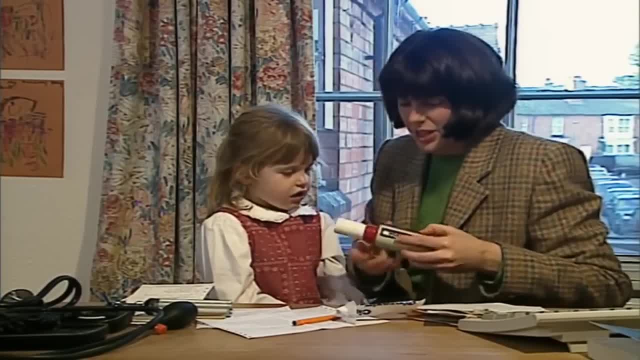 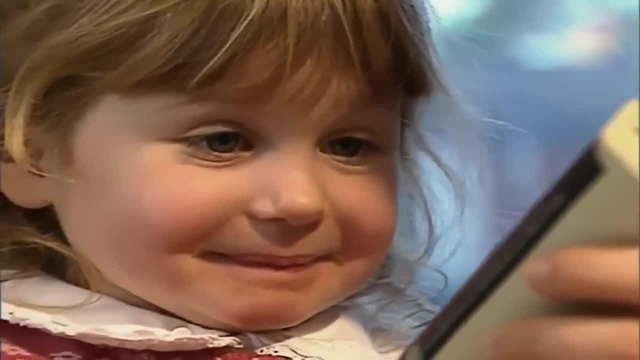 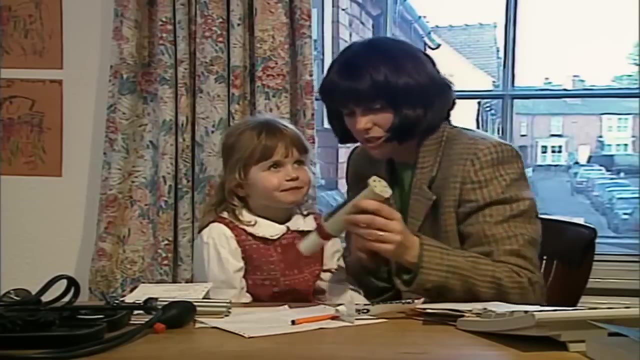 I can do that, Do you? Yeah, Right. So what you need to do is you need to go big blow. Look that's good, Right up there, Have another go. That means that your lungs are very healthy, your chest is very healthy. 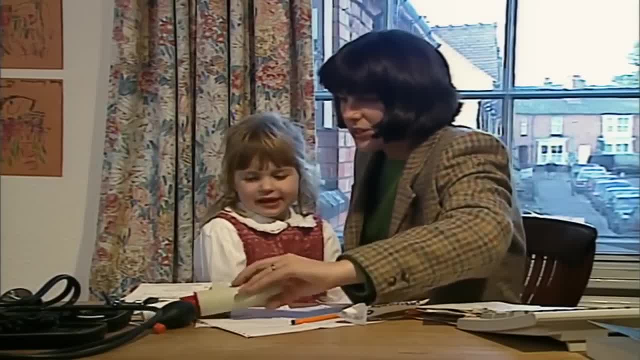 because your lungs are very healthy, Because you can blow that all the way up there, That's very good. Well, I know, Mummy, Do me tum-tum check. Okay, let's go and check your tummy. That always makes me giggle. 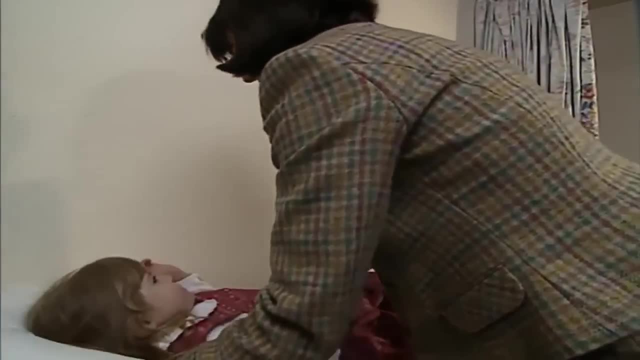 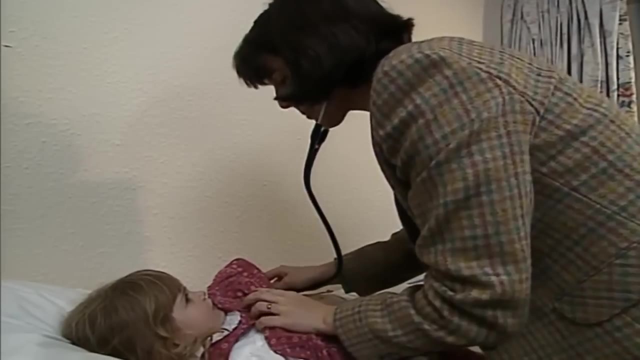 Up. you go Right, lie down. Shall, I listen to your chest first. Listen to your breathing, That's it There. have a listen with this Big breaths in and out. That's it nice and slowly, Good girl. 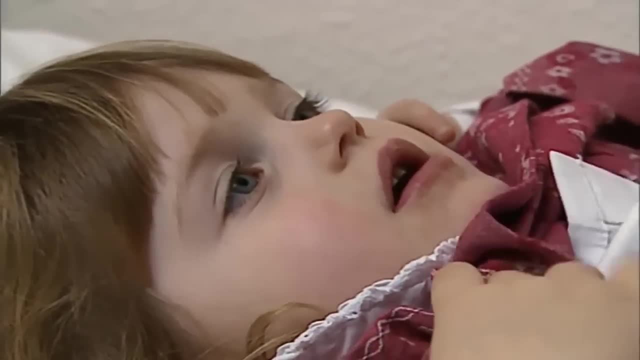 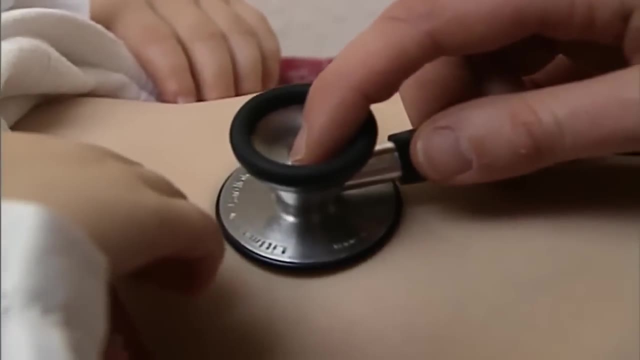 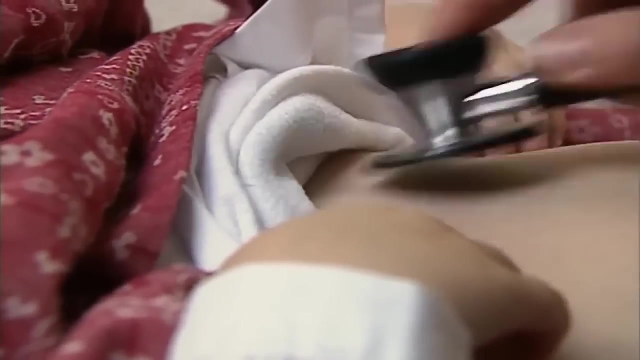 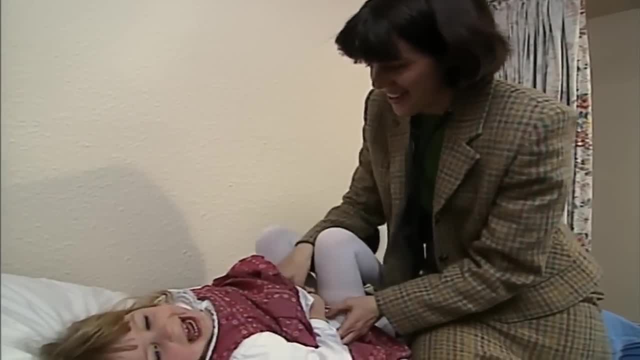 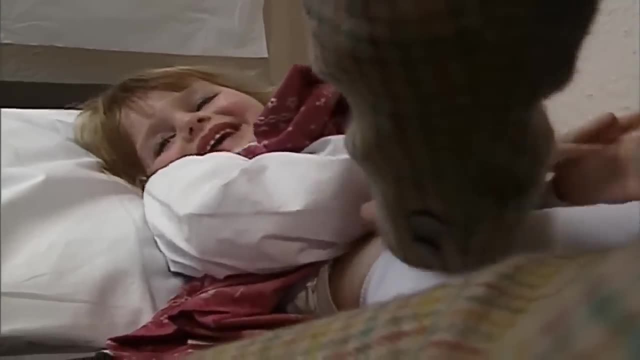 What can we feel here? Can't feel your breakfast, Can't feel your lunch. You've got a very tickling tummy, haven't you? And it tickles me? I think you're missing, you're lacking your tea. I think you need your tea. 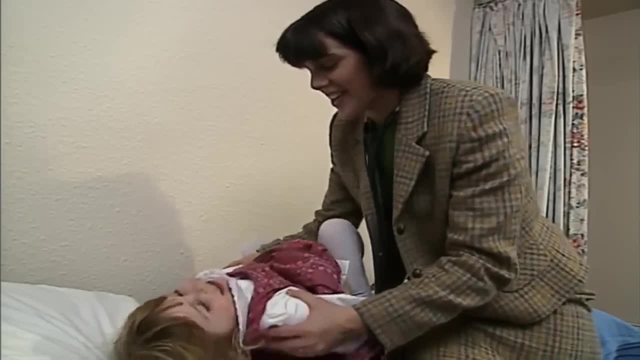 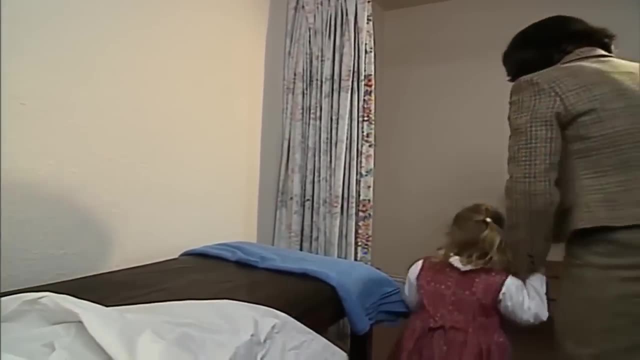 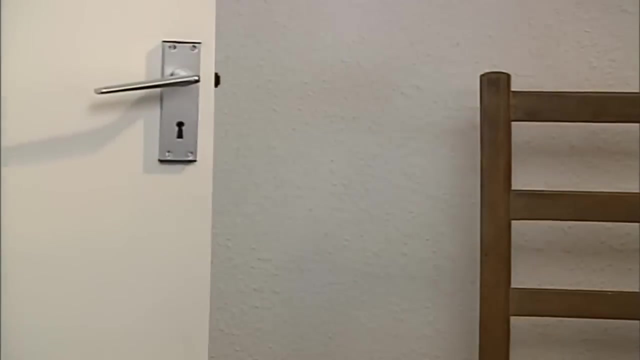 It feels fine, otherwise, Right, shall we take you home for your tea now? Yeah, Come on, then let's get you down. I love my mum and I love seeing my mummy when she's a doctor. Bye-bye, bye-bye, bye-bye, bye-bye. 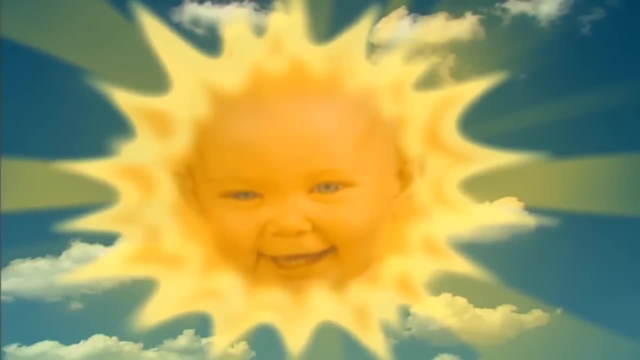 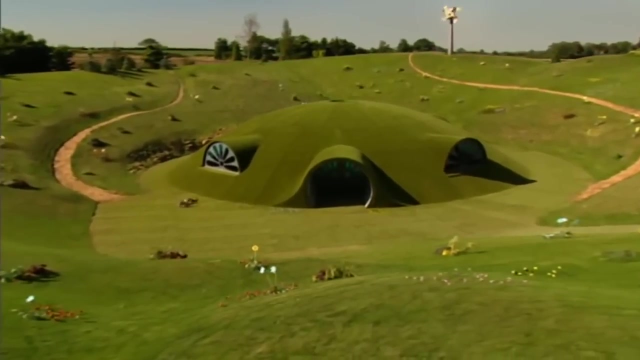 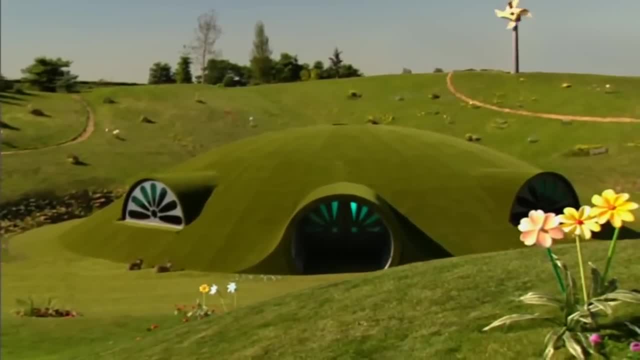 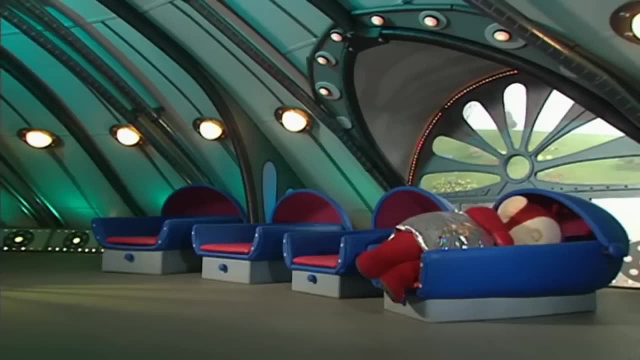 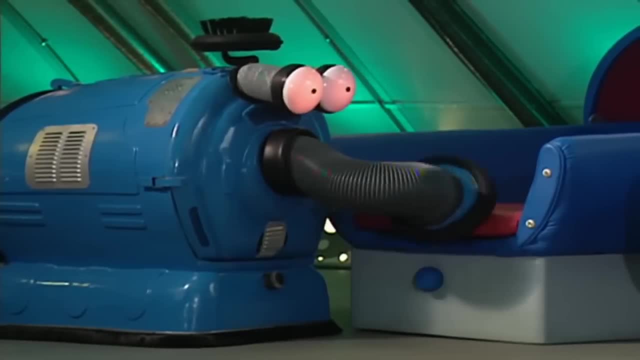 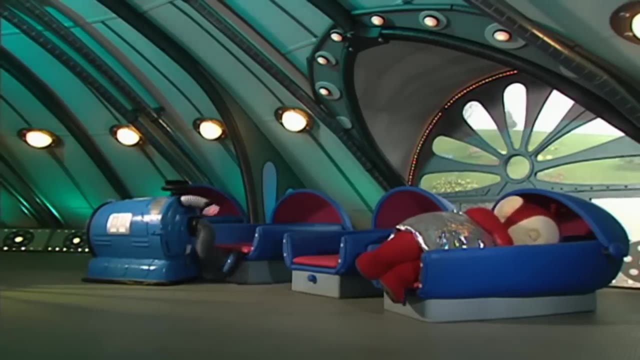 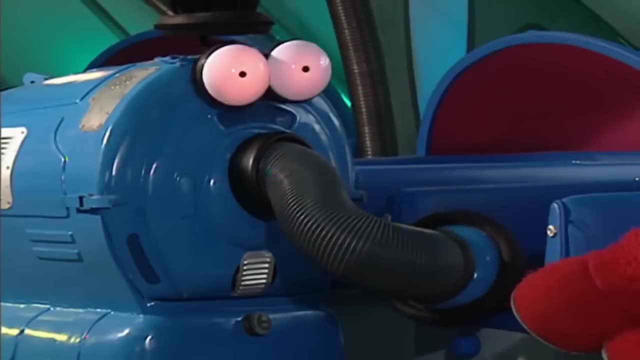 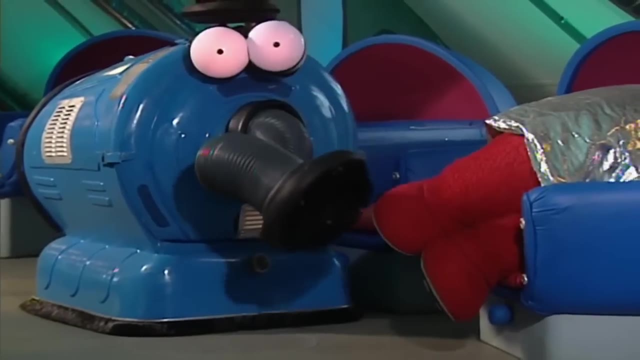 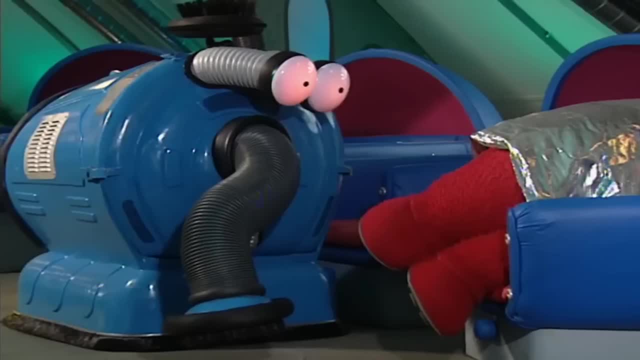 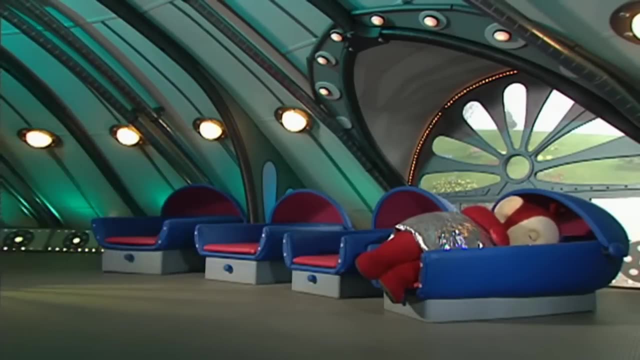 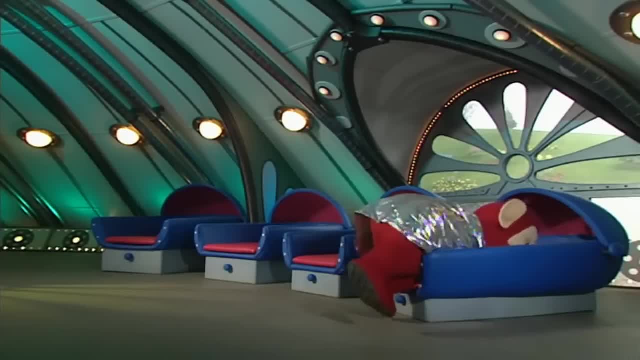 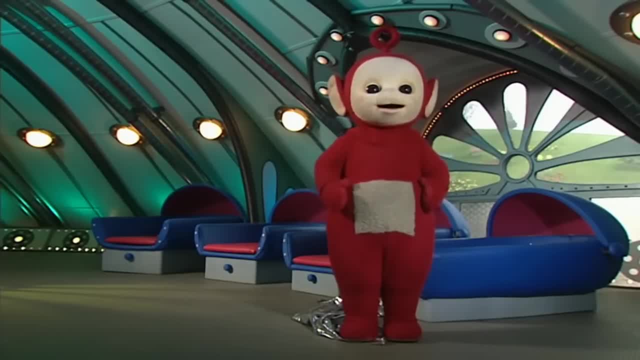 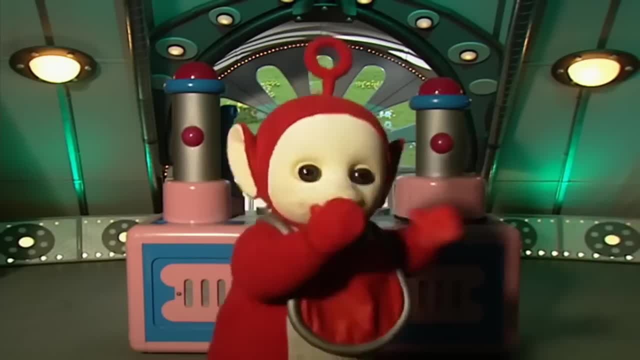 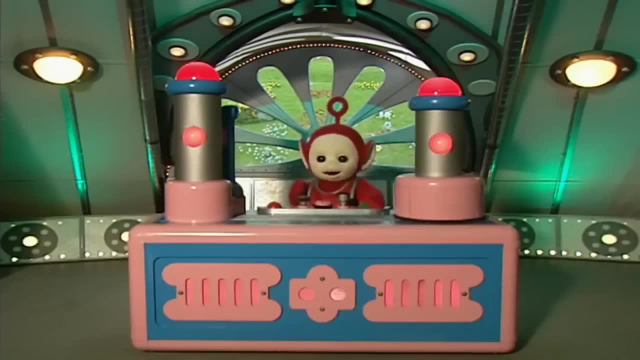 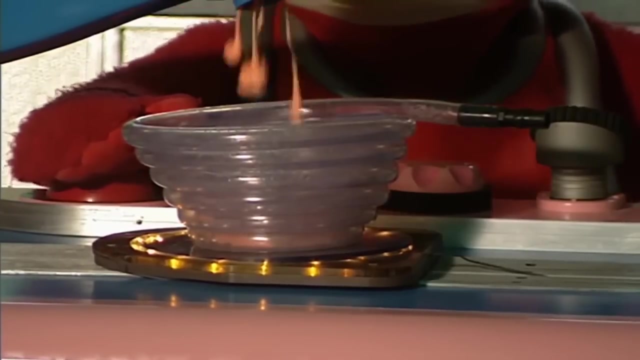 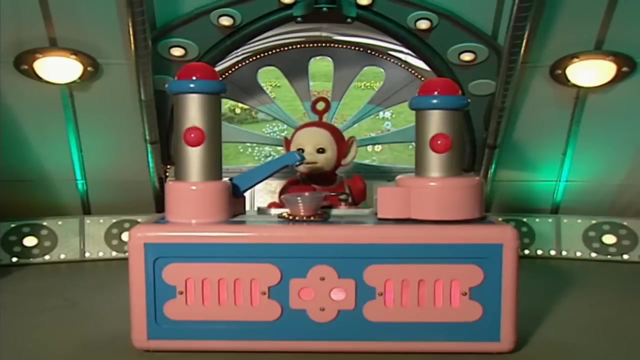 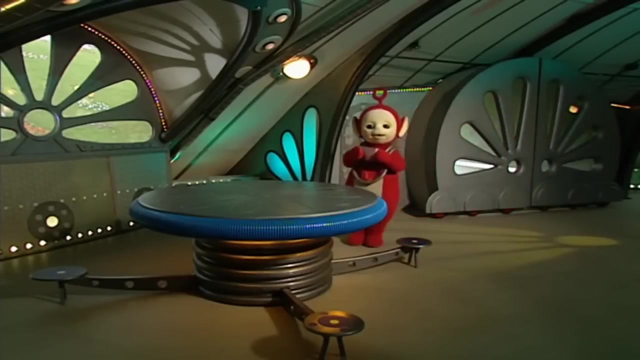 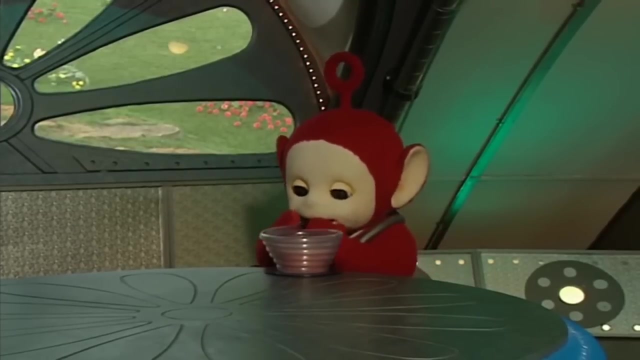 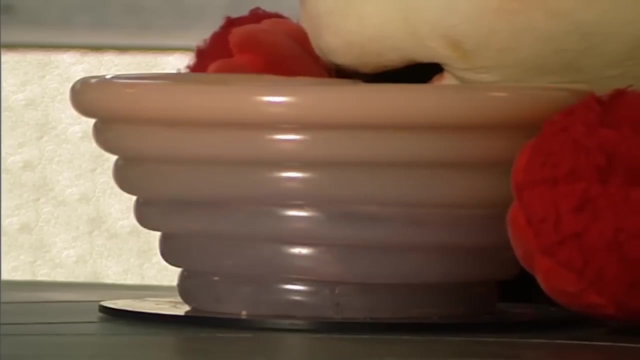 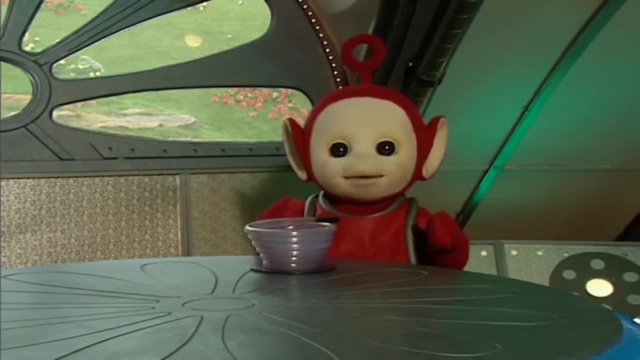 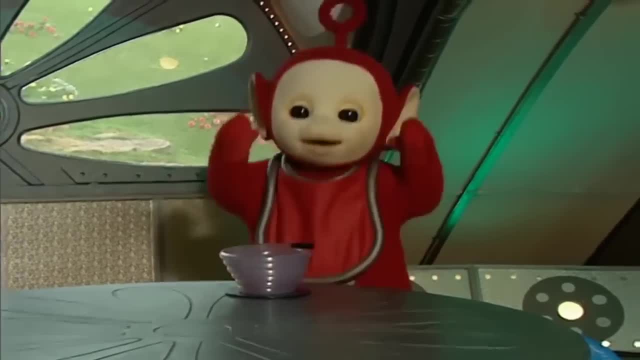 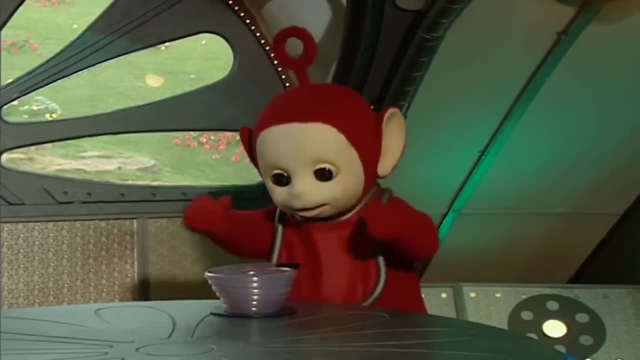 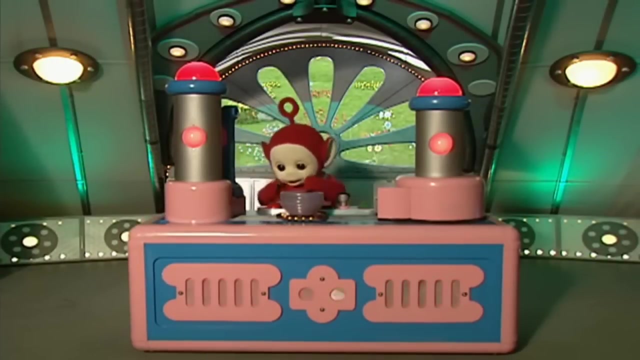 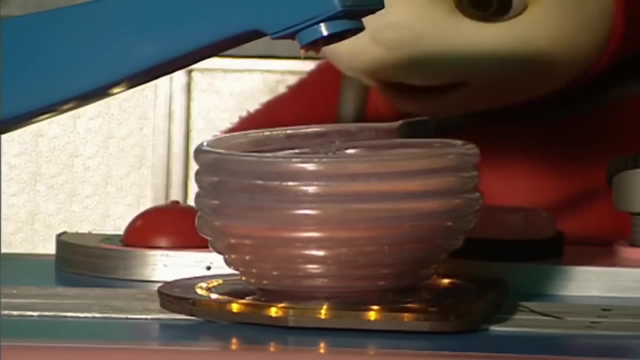 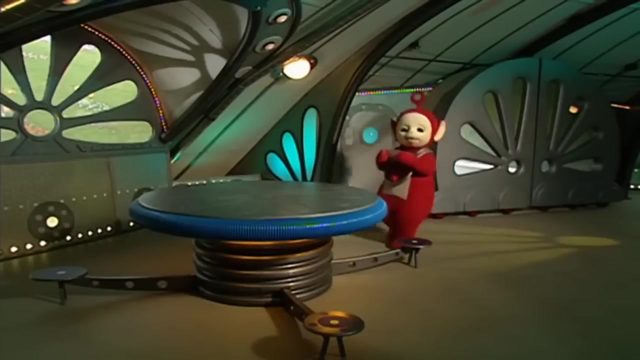 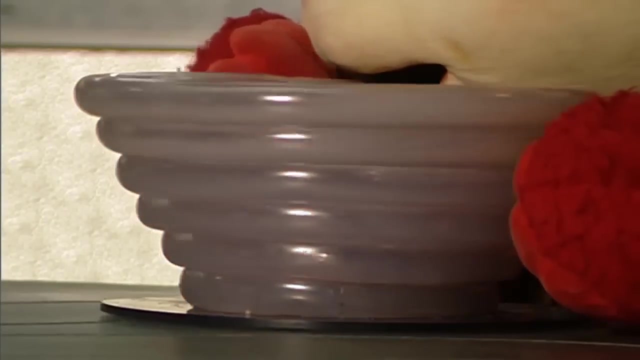 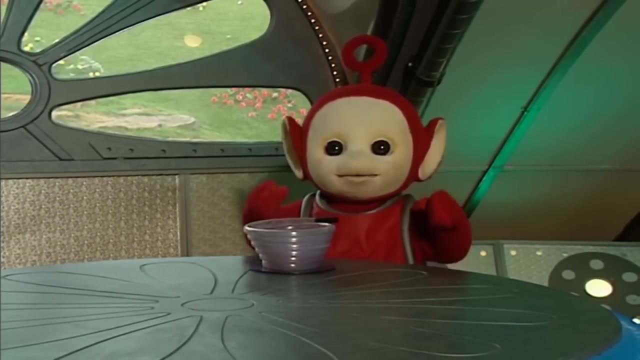 Po like toppy custard. Again, Again, Again, Again, Again, Again, Again. Toppy custard, Toppy custard, Toppy custard. Ah, Toppy custard, Toppy custard. Po likes toppy custard, very, very much. 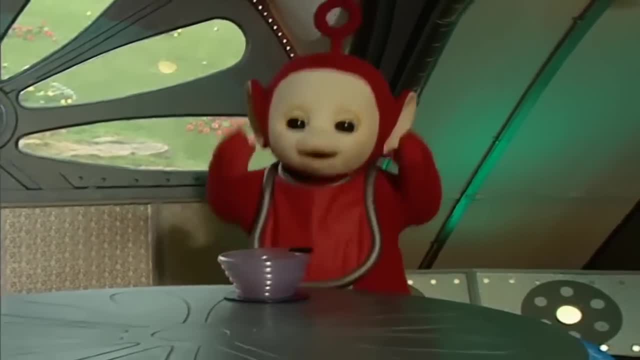 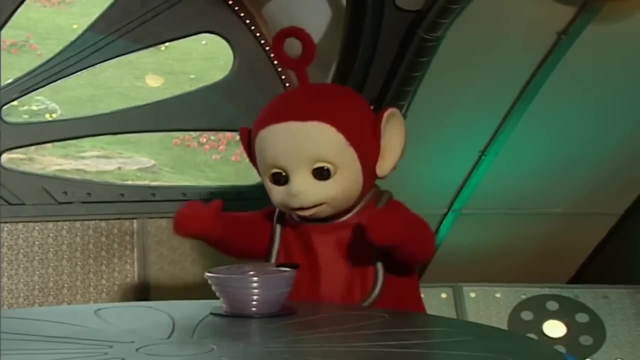 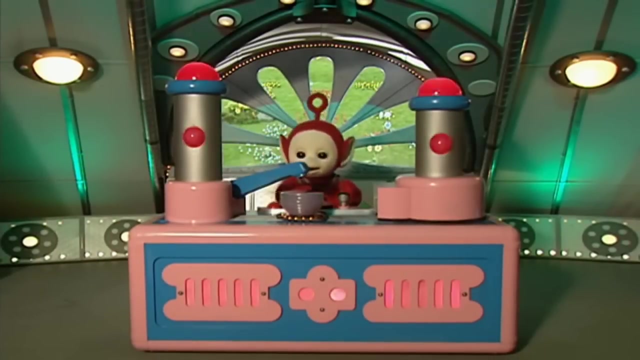 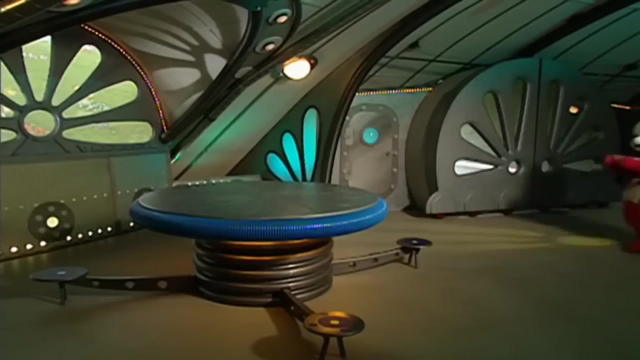 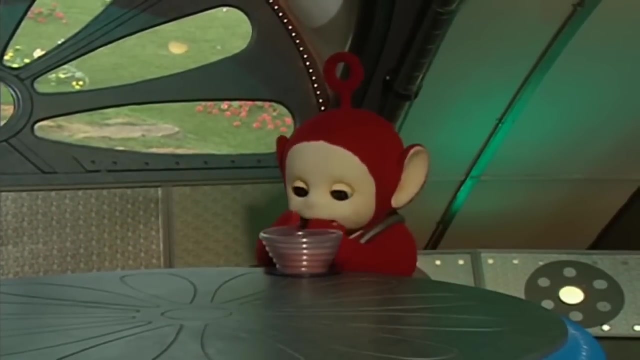 Po like toppy custard. Again, Again, Again, Po went to get some more Tubby custard. Tubby custard, Ooh, tubby custard. Po likes tubby custard, very, very, very much. 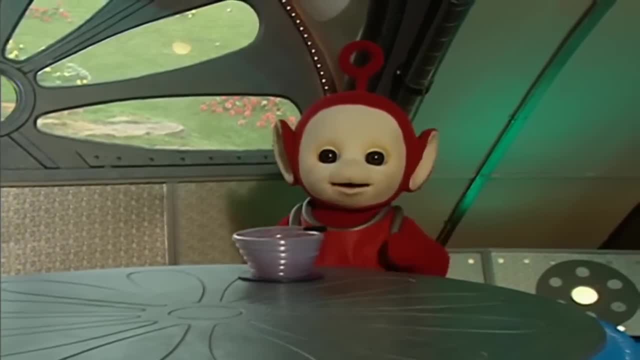 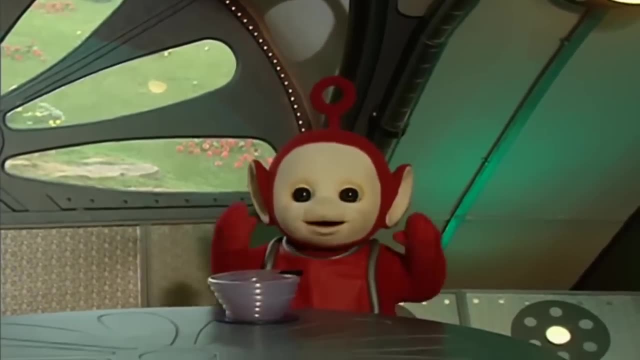 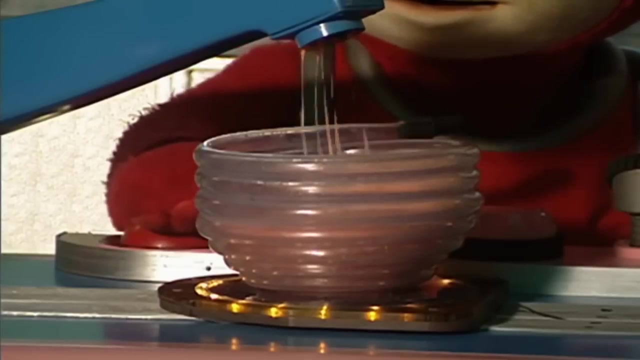 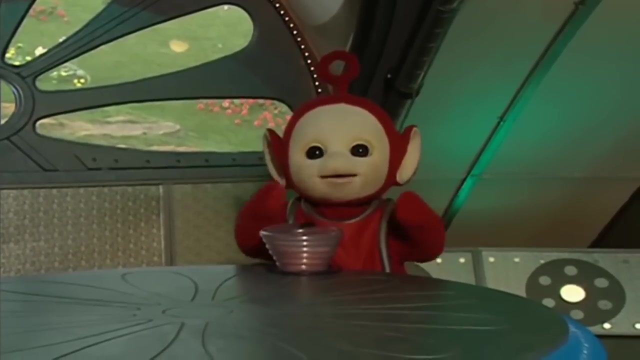 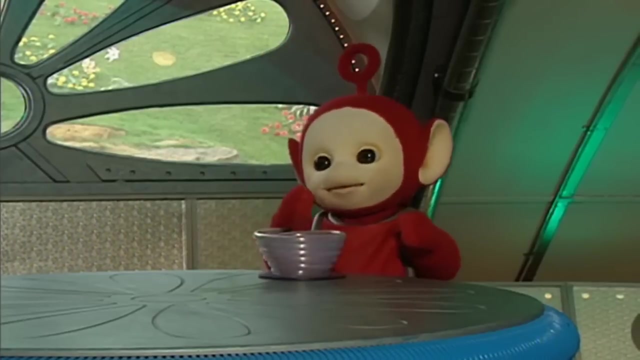 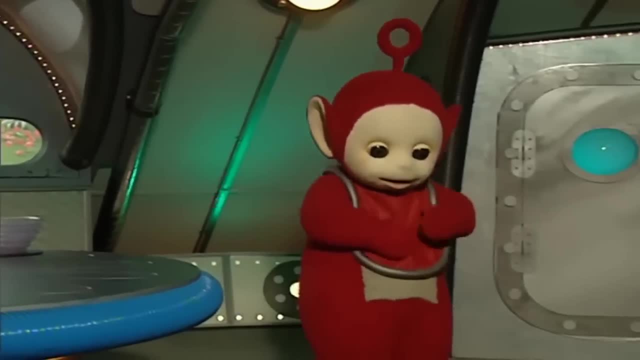 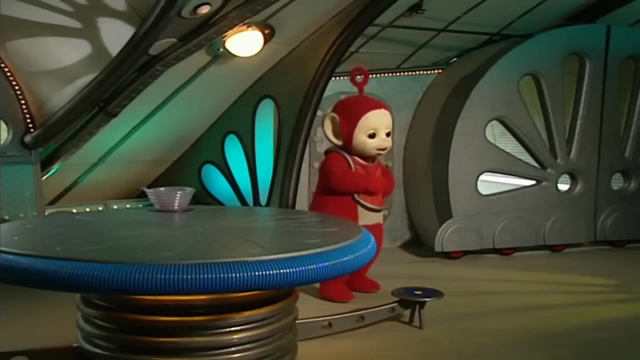 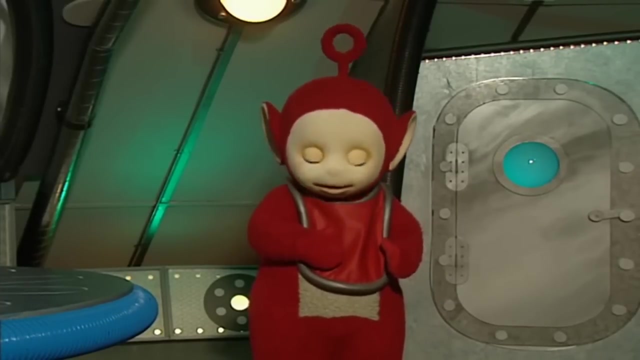 Ooh, Ooh, Ooh, Oh dear, Oh dear Po. Tubby custard tummy. Sometimes, if the Teletubbies eat too much tubby custard and they eat their tubby custard too fast, they get tubby custard tummy. 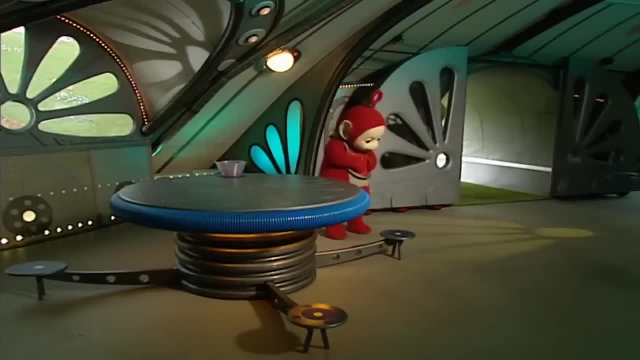 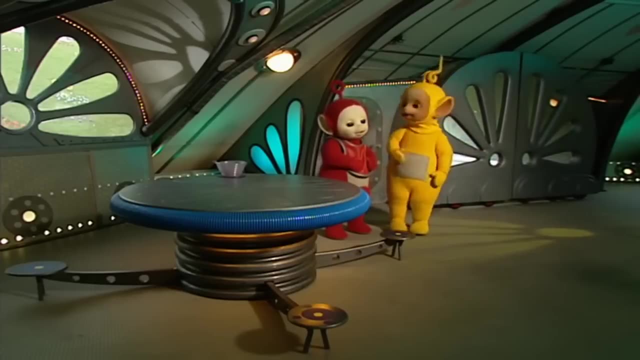 Tubby, custard tubby. Oh dear La-di-la-di-la-di-la-di-la-di-la, La-di-la-di-la-di-la-di-la-di-la-di-la-di-la, Eh-oh, Eh-oh Po, Eh-oh La-la. 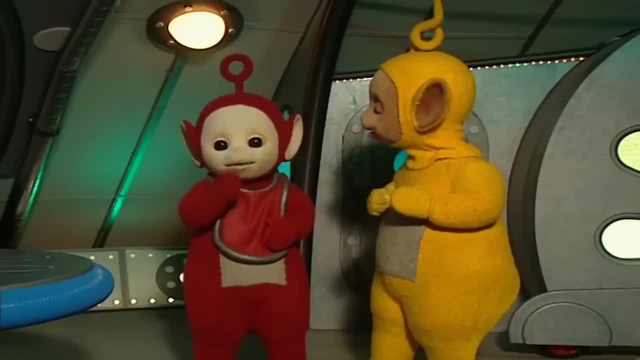 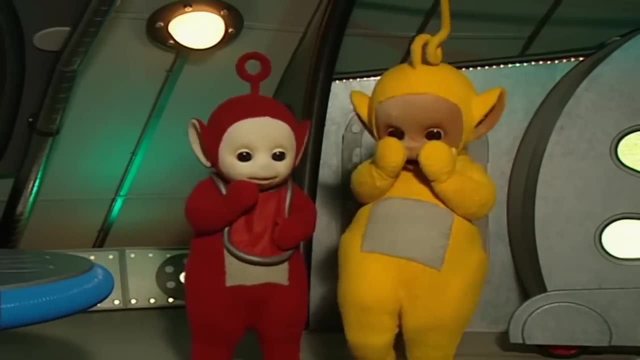 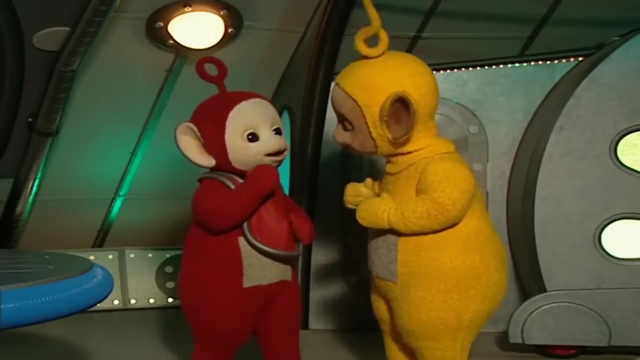 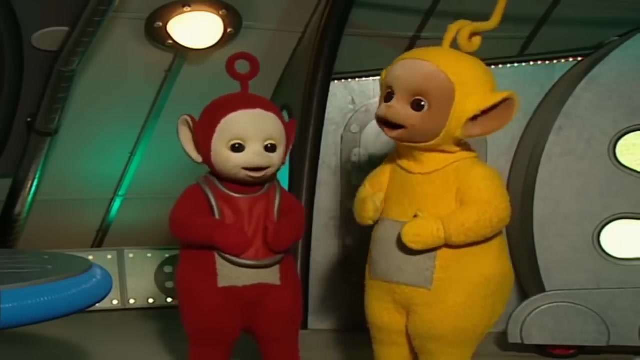 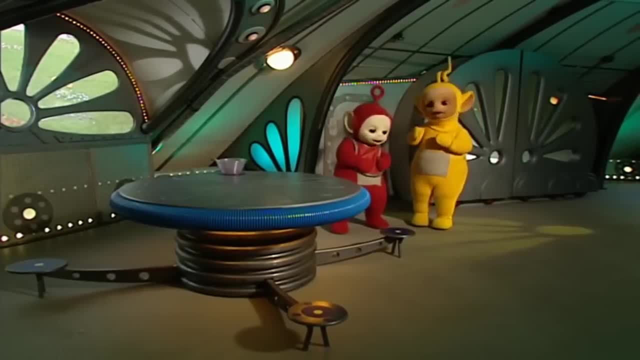 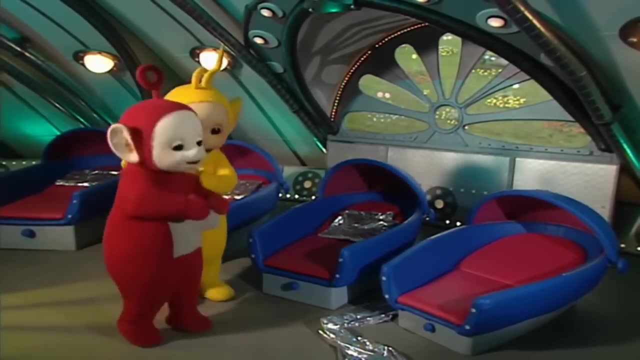 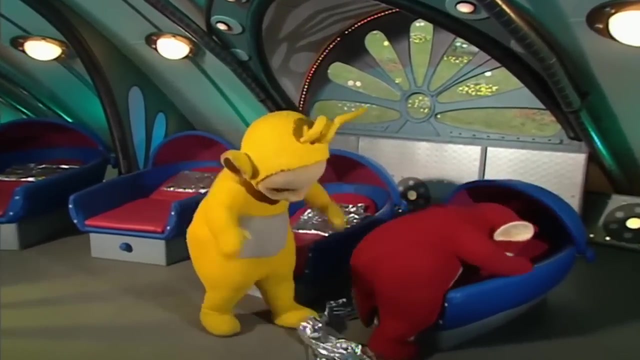 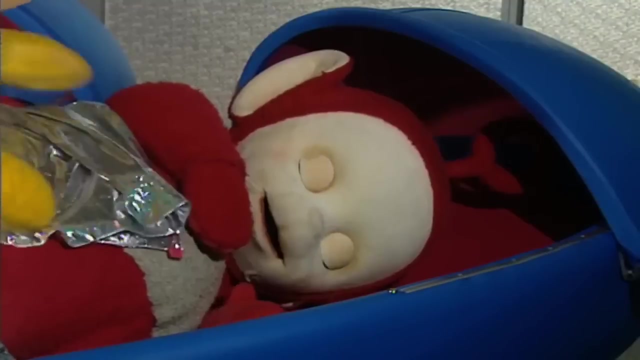 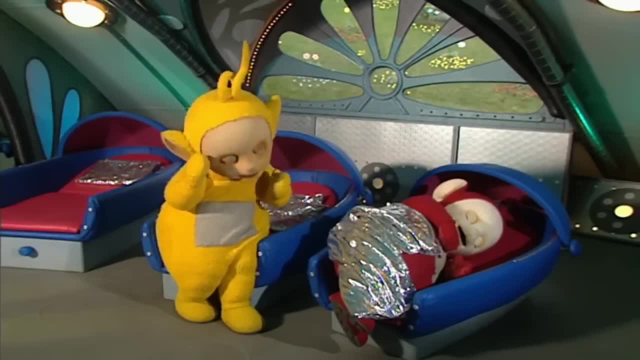 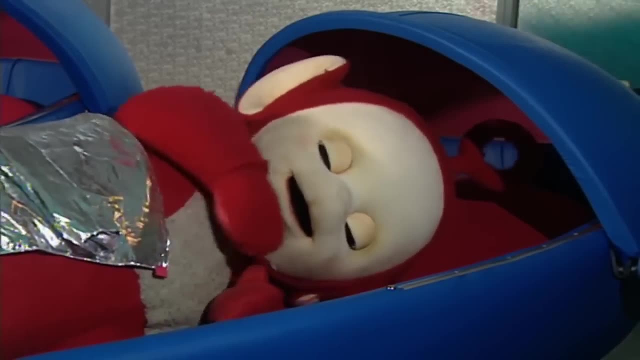 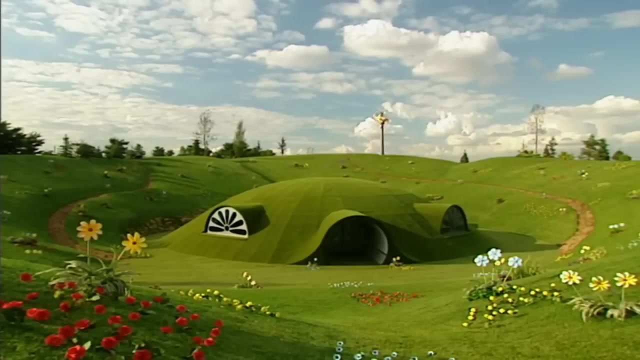 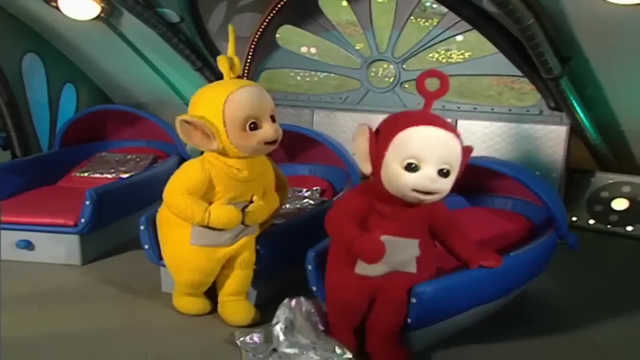 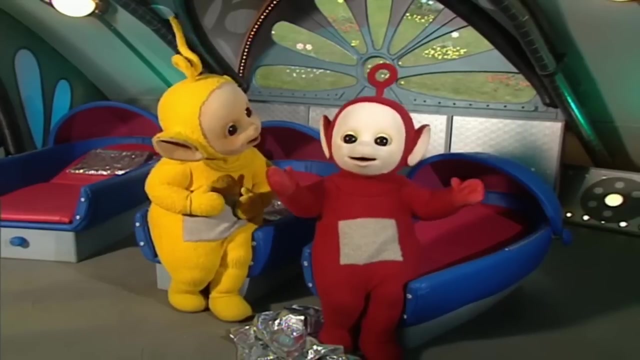 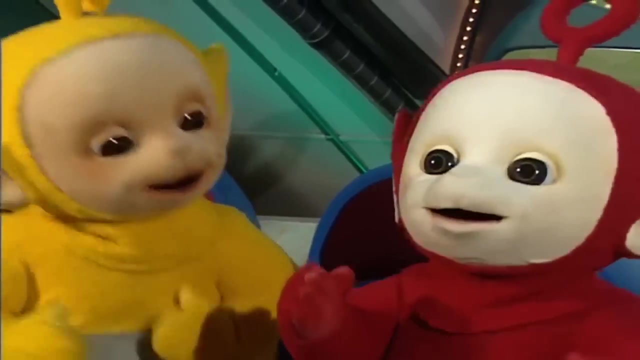 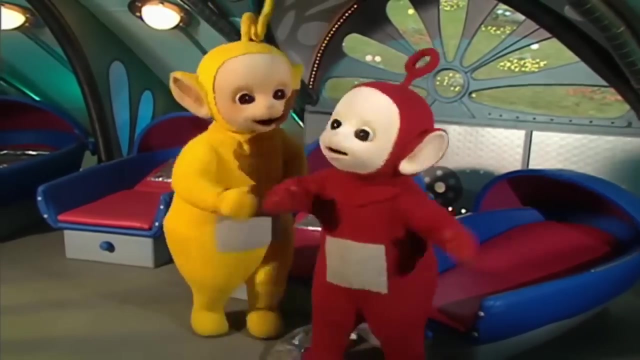 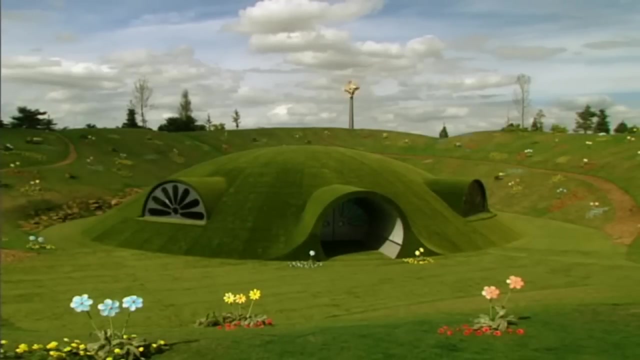 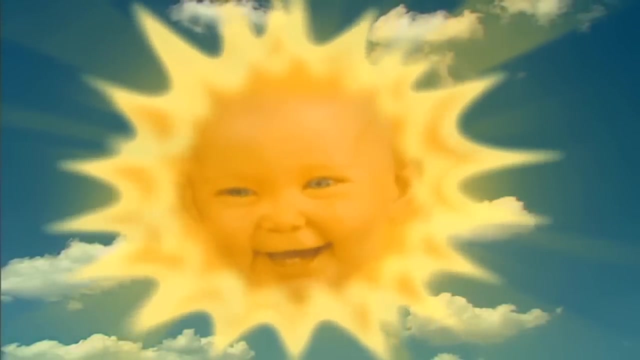 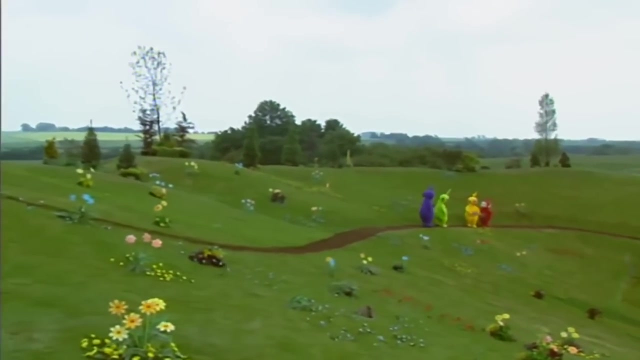 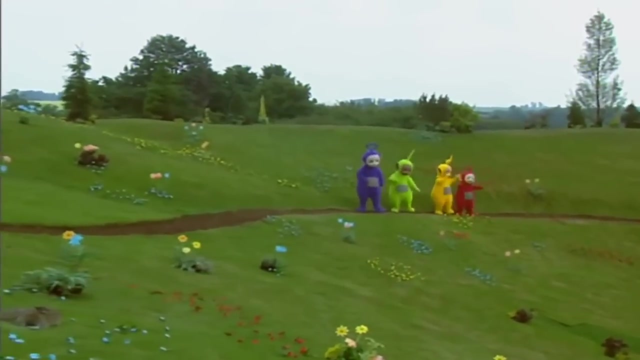 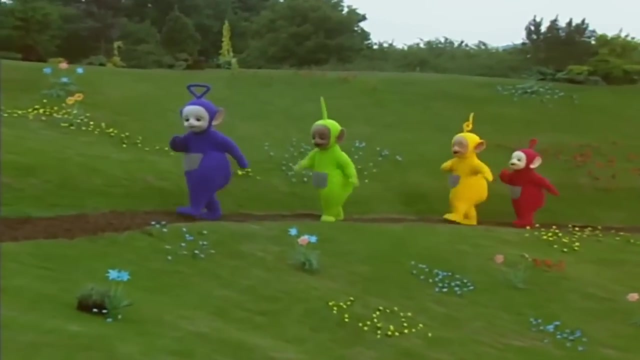 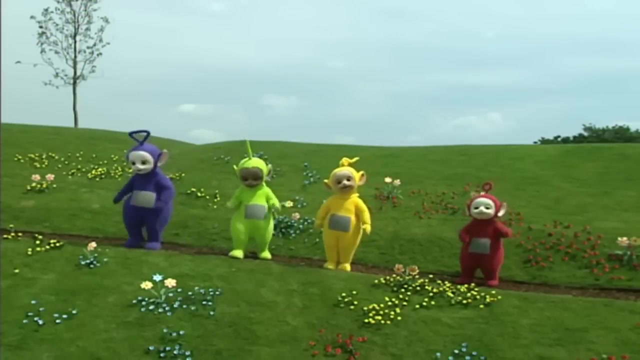 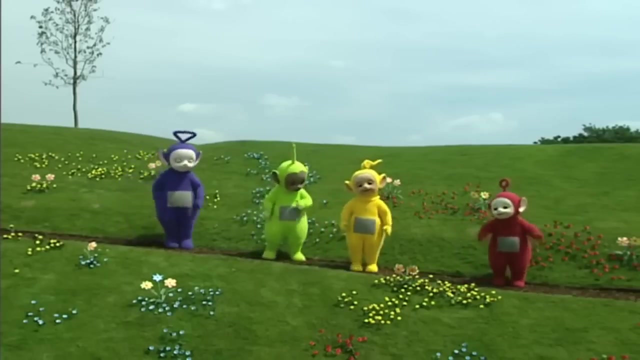 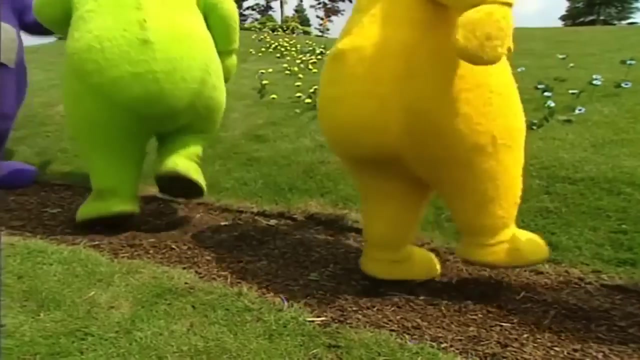 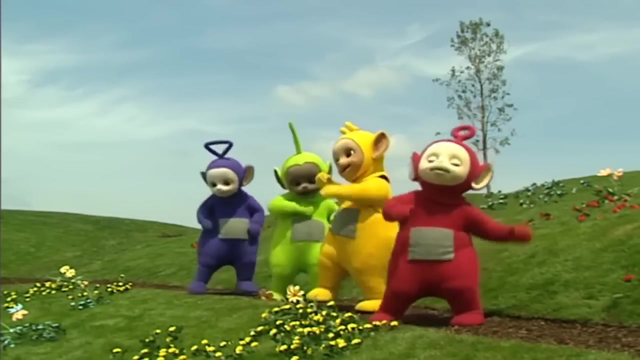 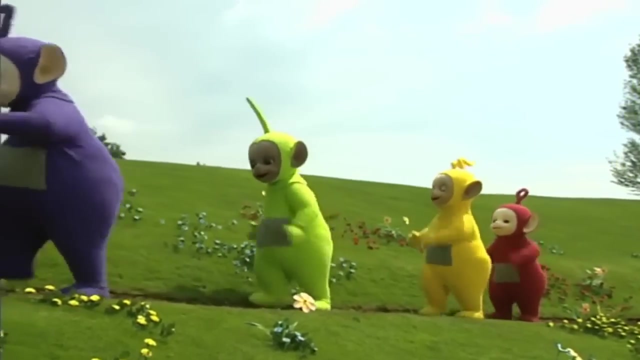 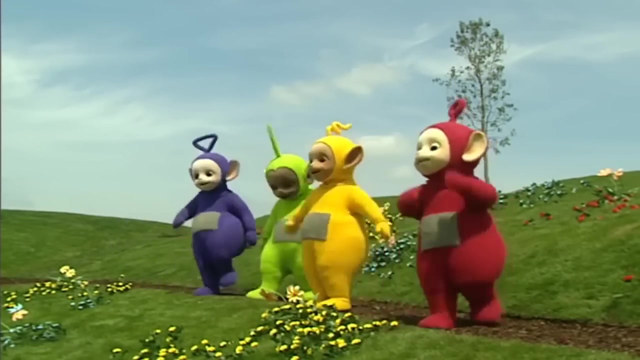 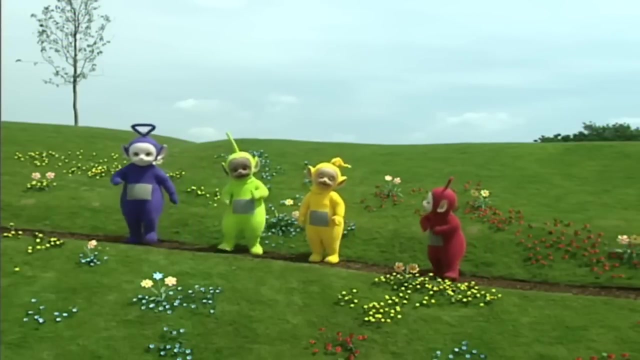 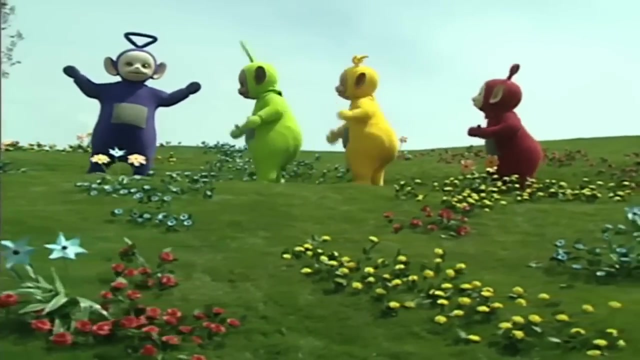 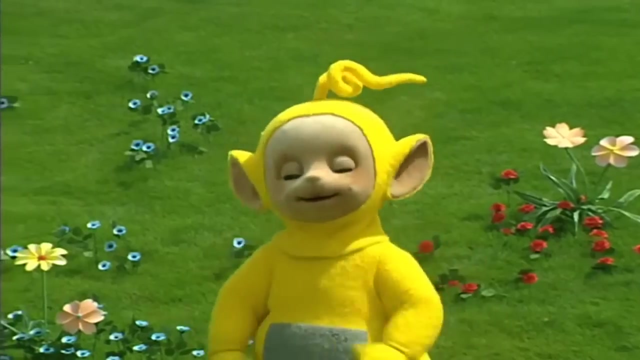 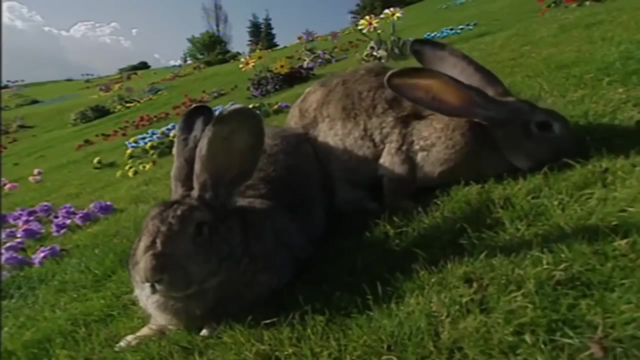 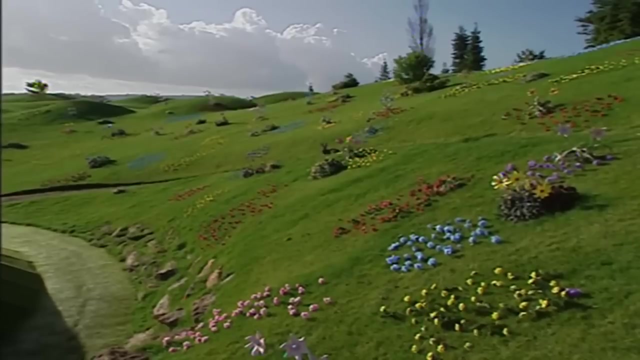 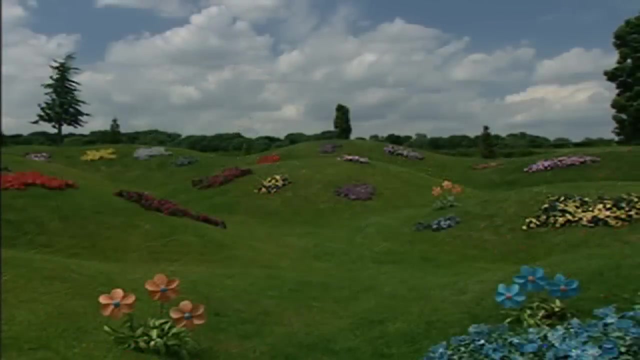 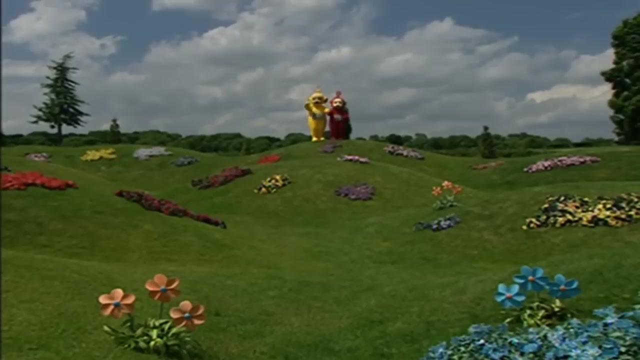 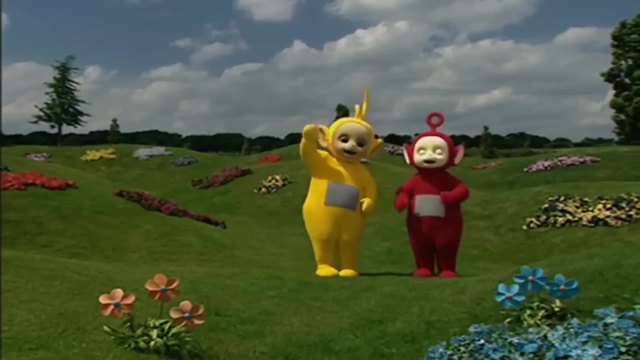 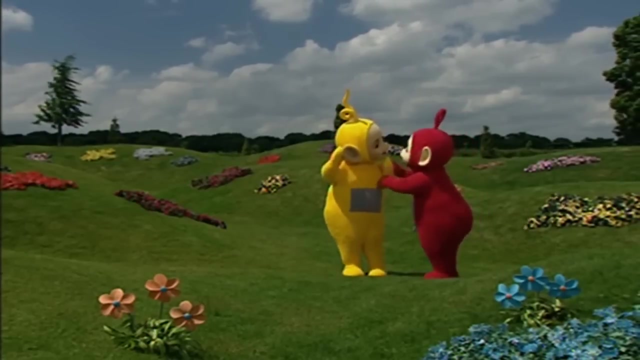 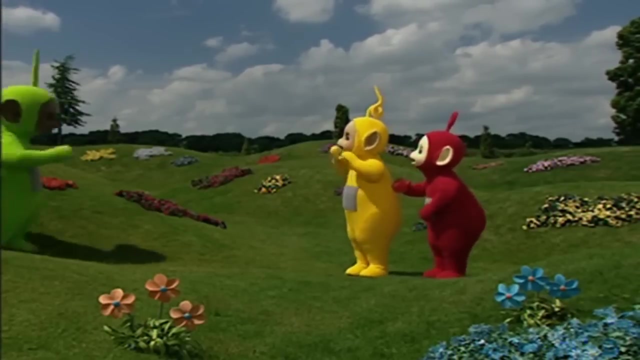 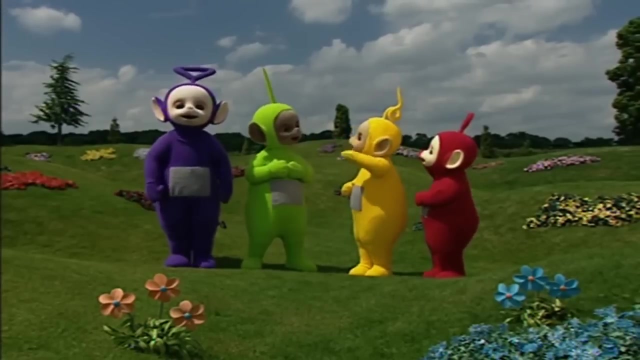 Oh, dear, Yeah, Oh, Oh, Oh, Oh, Oh, Oh, Uh, oh. La-di-la-di-la-di-la-di-la-di-la-di-la-di-la-di-la-di-la-di-la-di-la-di-la-di-la-di-la-di-la-di-la-di-la-di-la-di-la-di-la-di-la-di-la-di-la-di-la-di-la-di-la-di-la-di-la-di-la-di-la-di-la-di-la-di-la-di-la-di-la-di-la-di-la-di-la-di-la-di-la-di-la-di-la-di-la-di-la-di-la-di-la-di-la-di-la-di-la-di-la-di-la-di-la-di-la-di-la-di-la-di. 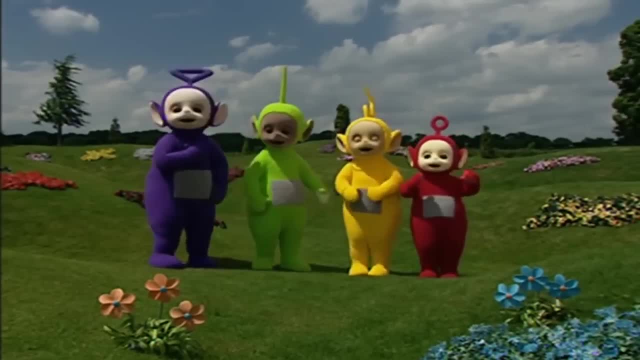 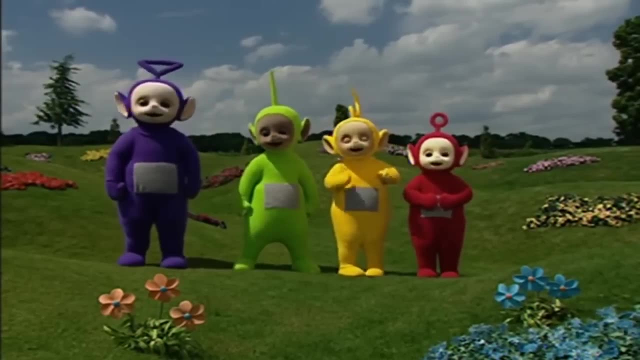 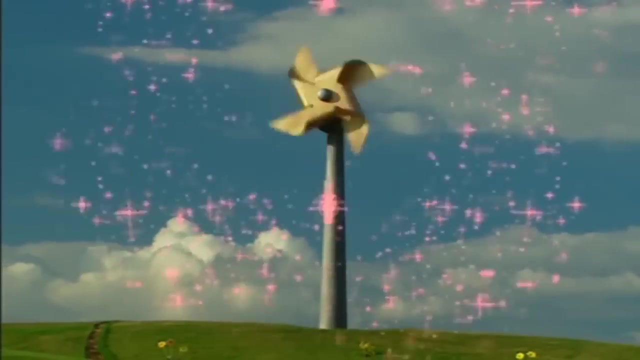 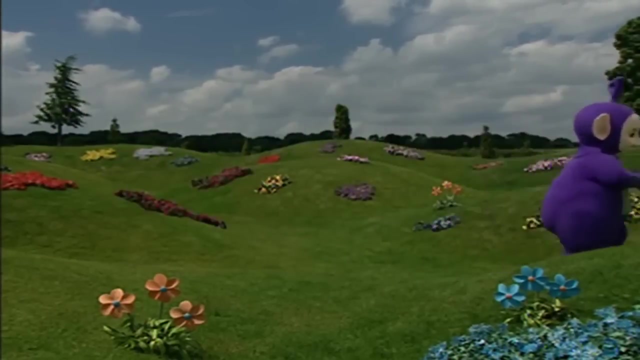 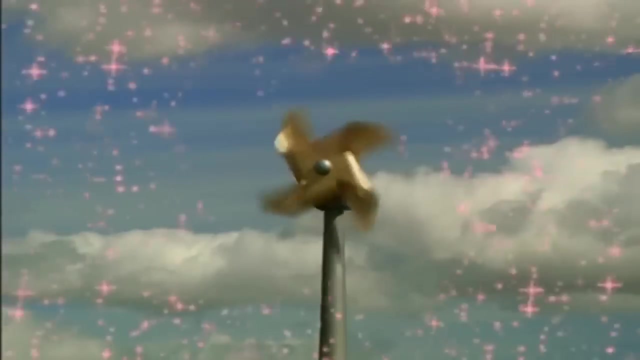 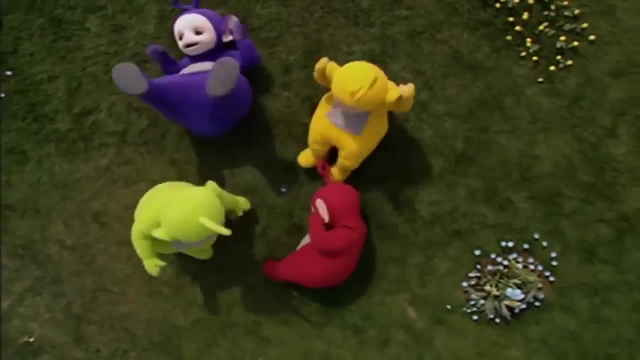 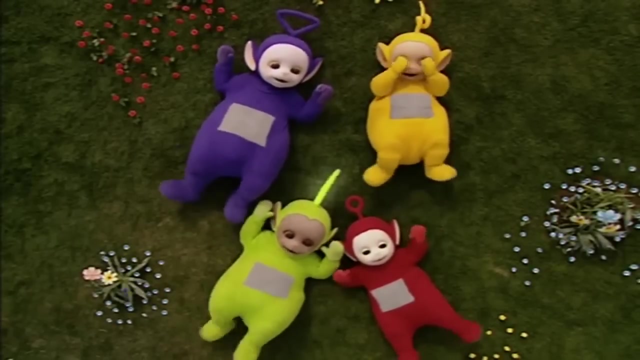 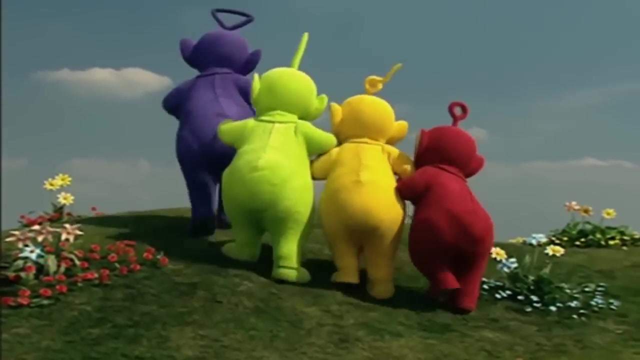 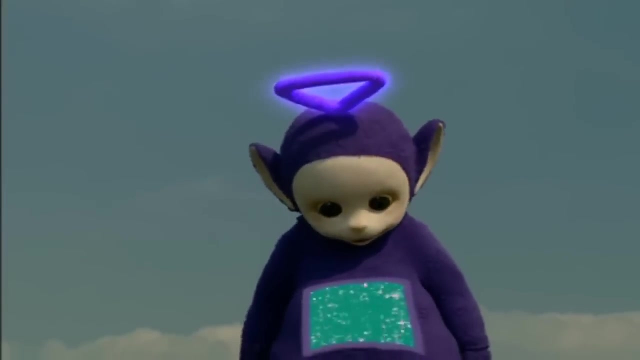 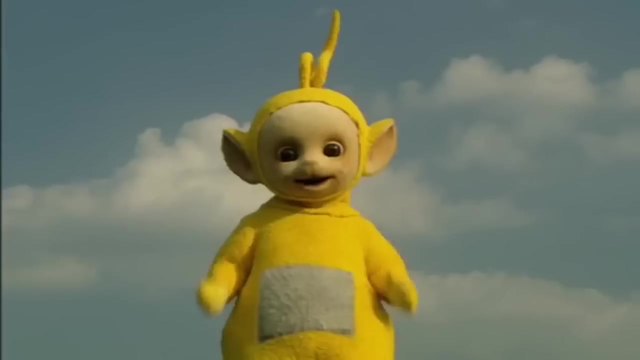 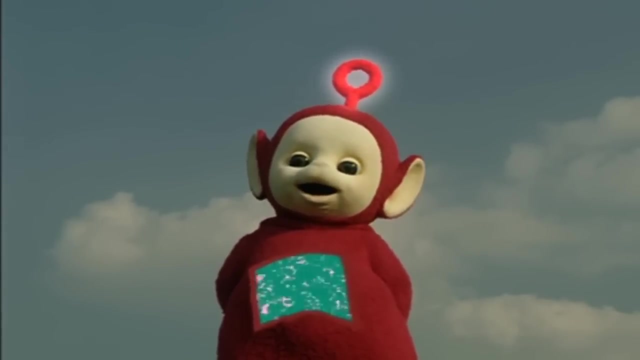 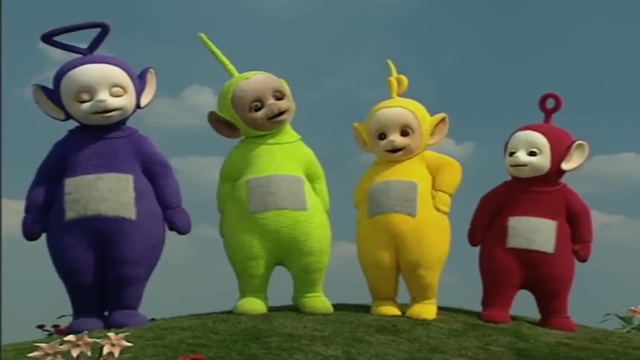 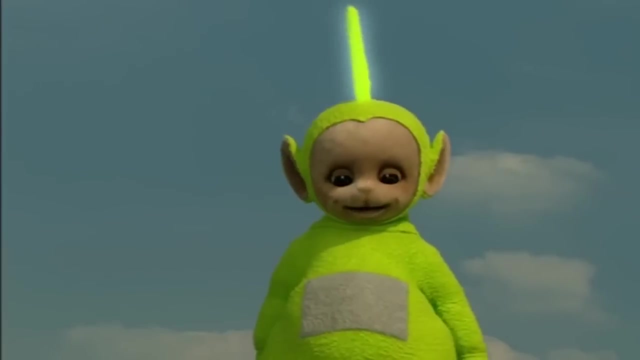 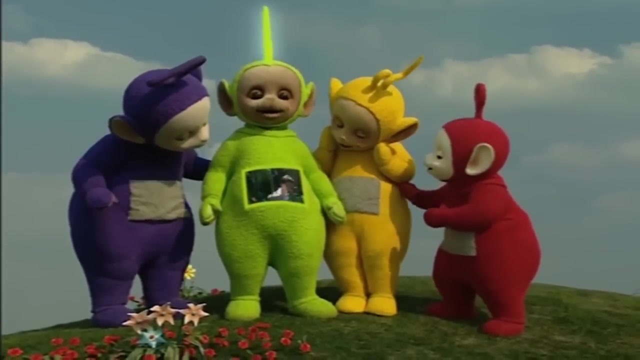 Uh, oh, Uh, oh, Uh oh. أو ICU. Untranslated Subtitles by Abbey Tiki-wiki: Gipsy Yalla, Oh, look, Oh, Gipsy Gipsy. Hello, hello, hello, Hello, hello, hello. 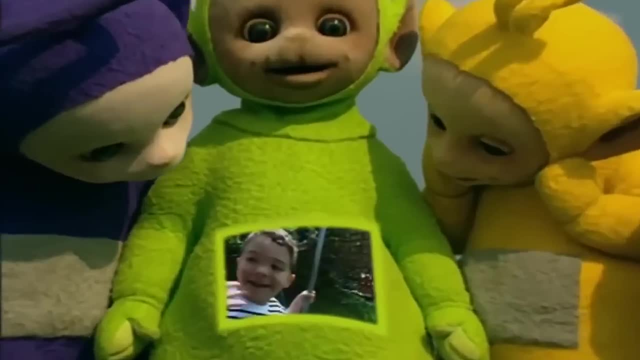 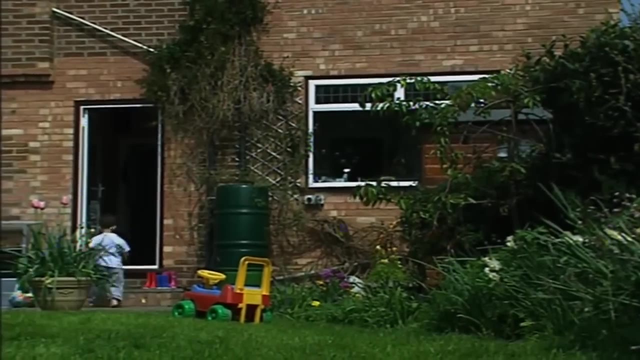 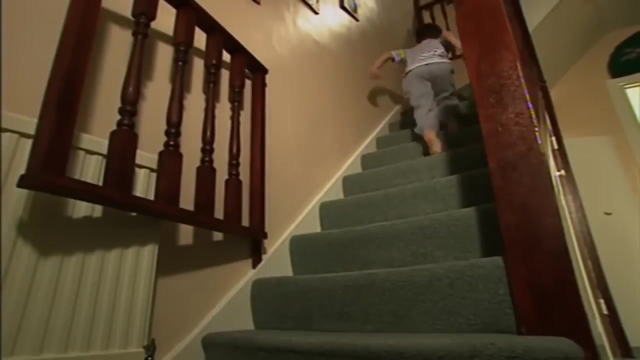 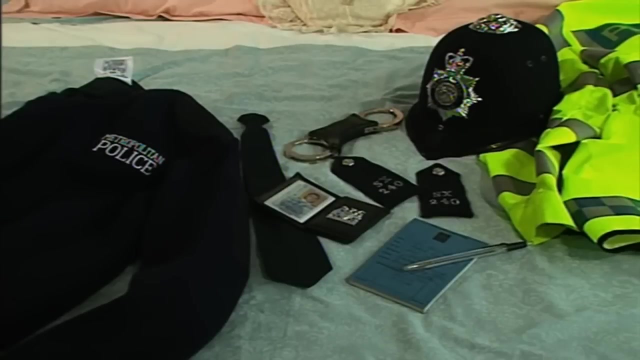 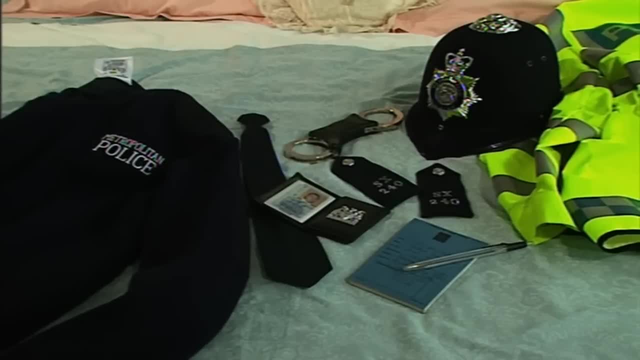 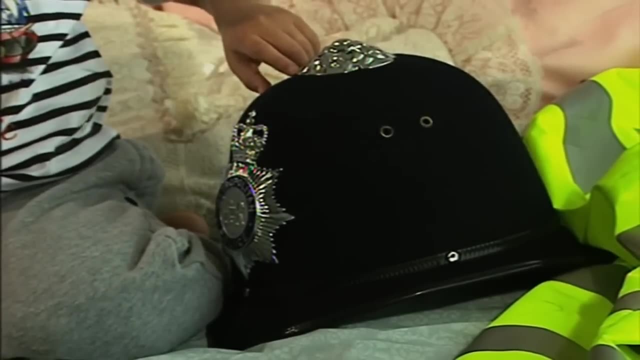 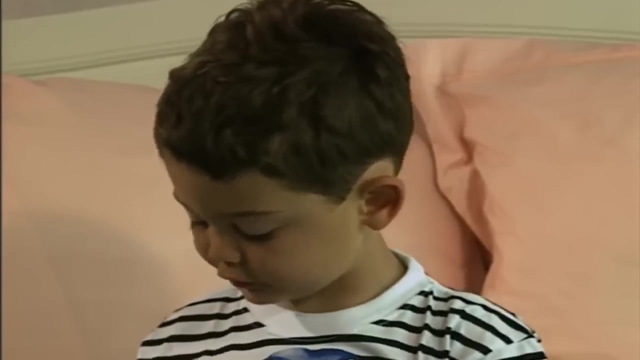 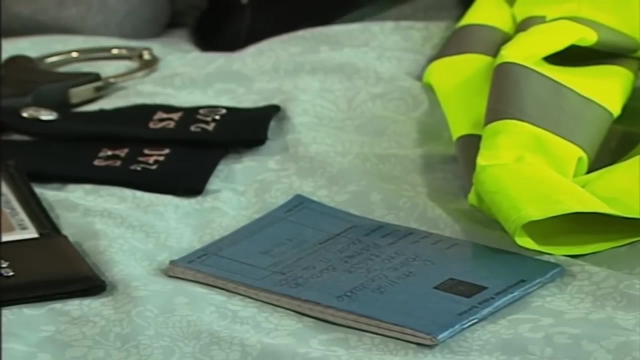 his jumper and his badges. This is daddy's helmet and he wears it on his head. These are his numbers for his arms And he wears a tight bit of length in his neck. This is my daddy's notebook. The writing inside: 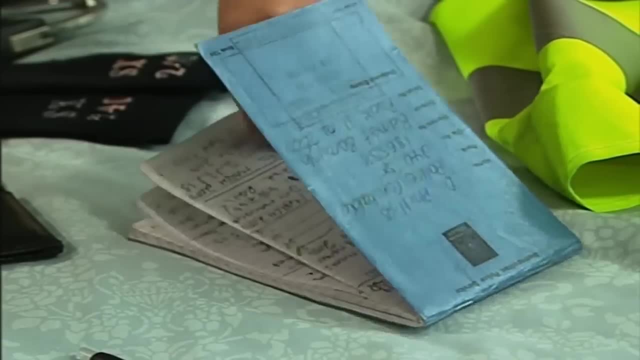 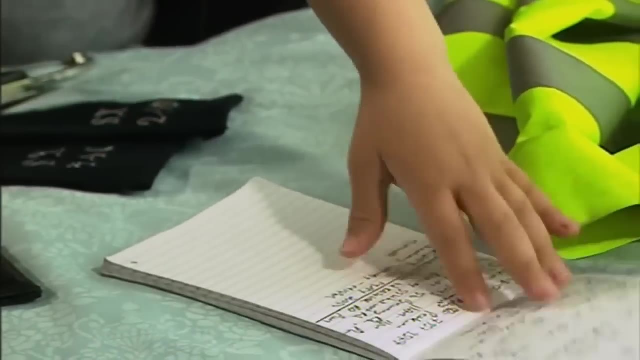 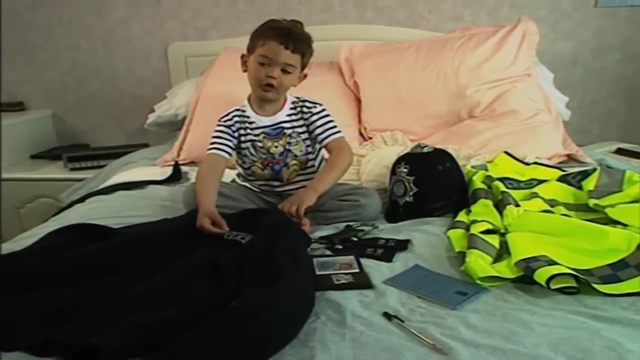 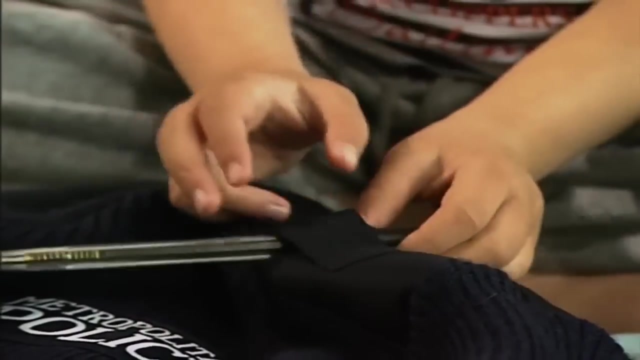 The two, one writing, two writing this one I need and another writing That pencil goes in here and it makes it really tight so it doesn't fall out the bottom end. Look, you put it there and you put it inside here. 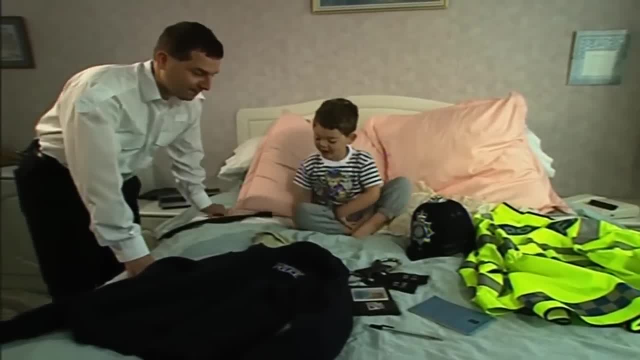 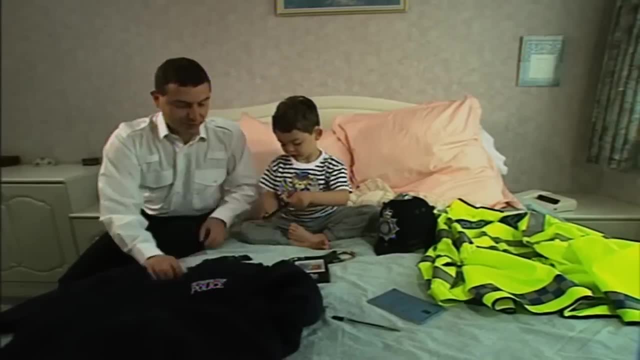 Look there, you've been getting all my things ready for work. Yes, I paused it and I did that. And what did you do with my numbers? I paused them. look Good, shall we put them on my jumper? Pull that off. 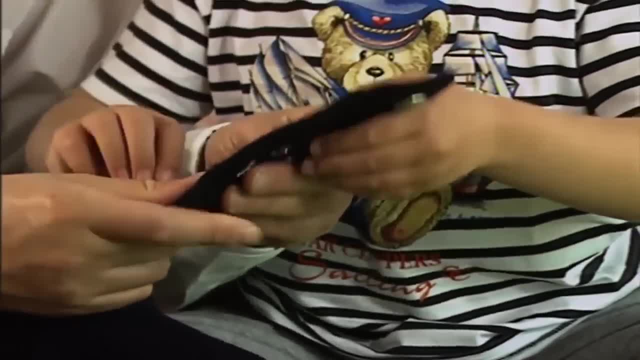 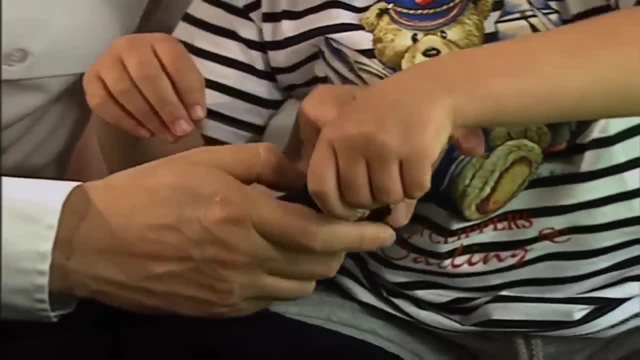 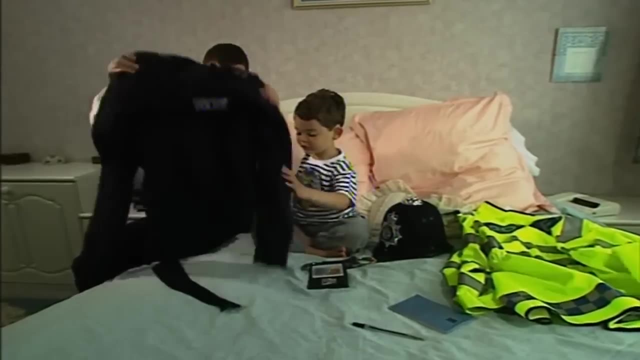 That's a good noise. OK, It's hard to pull it through, isn't it? I'll do this. I'll do this bit. OK, hold that and stick it on. That's it. OK. Now put your jumper on. 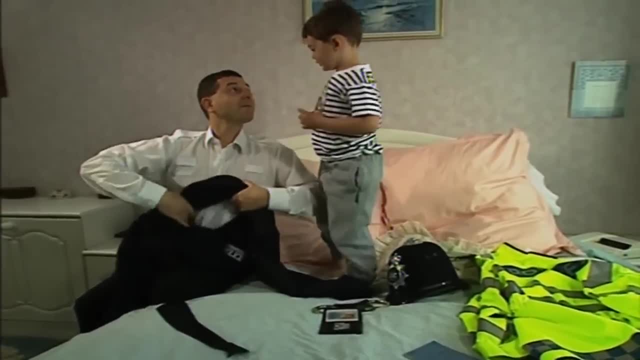 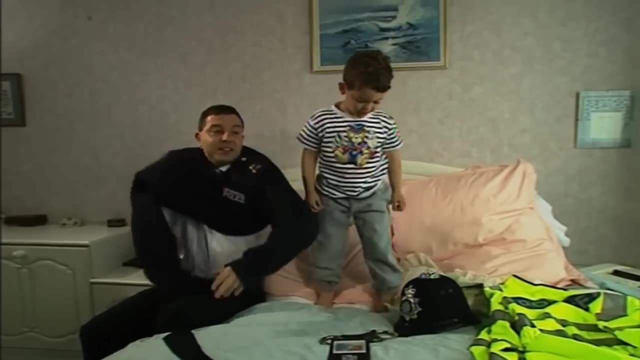 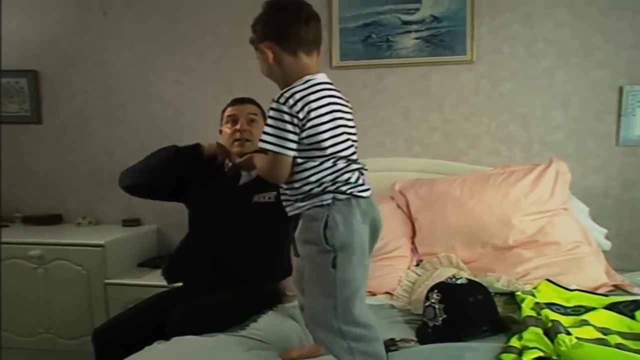 OK, Help me, I'm going to stand up and put it on your head, OK, That's good. Now I'm going to put it on, now, OK, And then We've got my tie to put on Tie. It's a special tie, isn't it? 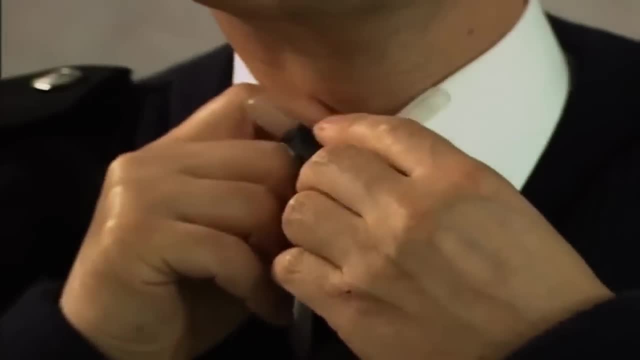 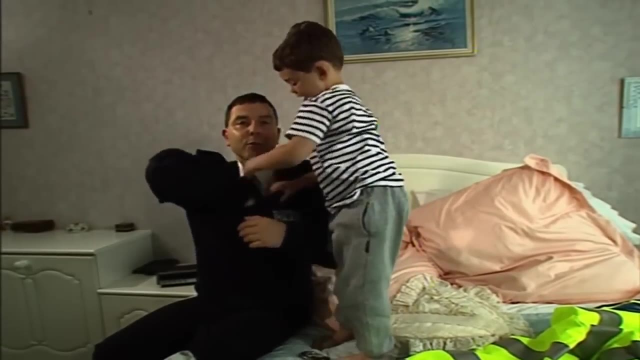 I can put it on. Tuck it in for me, Tuck it in Super And my pen. I need my pen, Super-duper, Super-duper, Super-duper, And my helmet. please, I'll put it on your head. 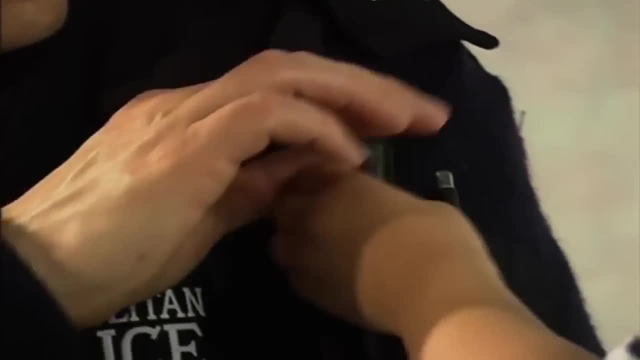 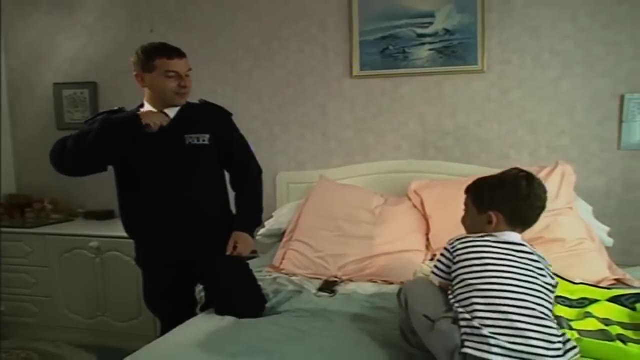 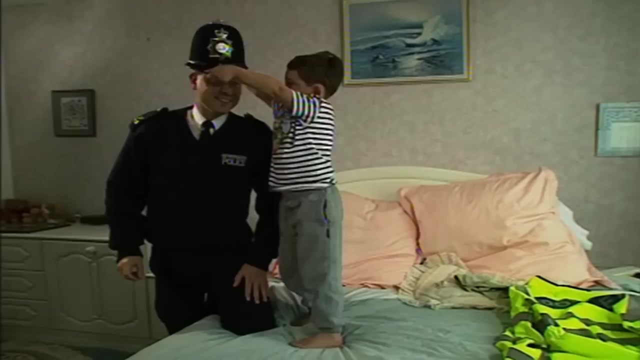 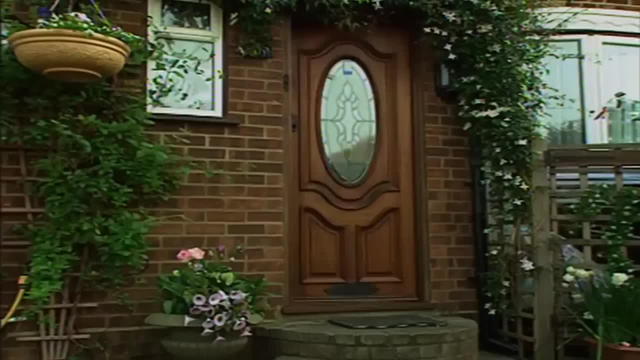 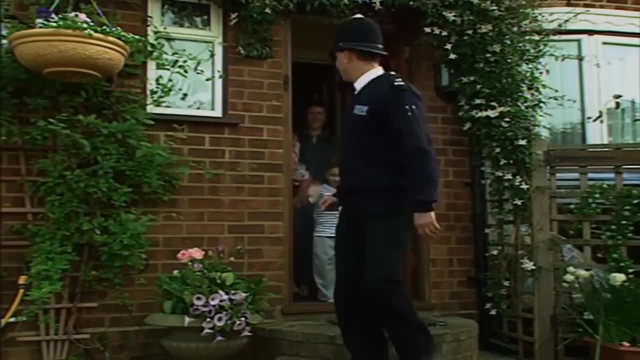 Yeah, Thanks very much. Get on then. Thank you pretty much. OK, I'm off to work now. Bye, Bye, Bye-bye, See you later. Have a good day, Bye, bye, See you later, Bye-bye. 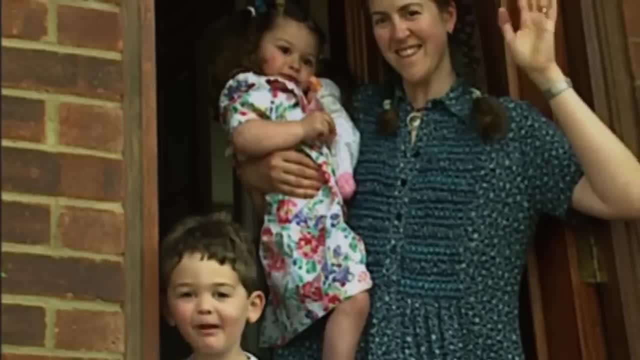 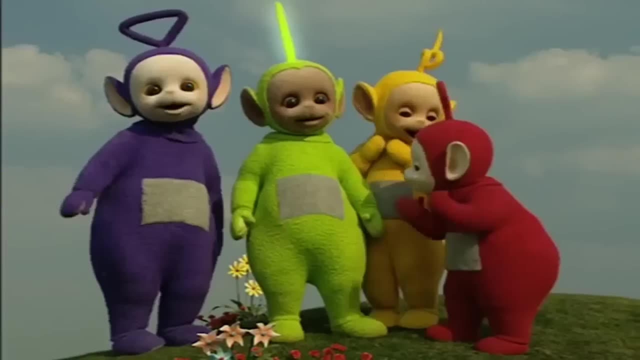 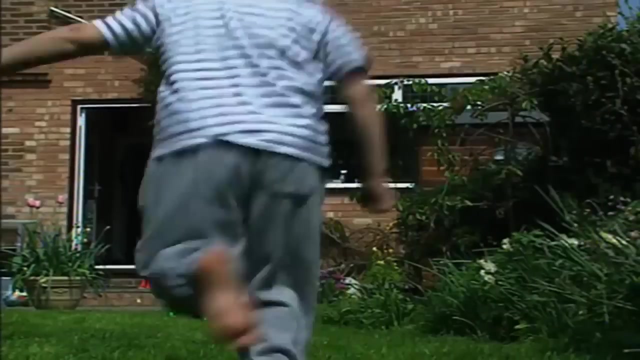 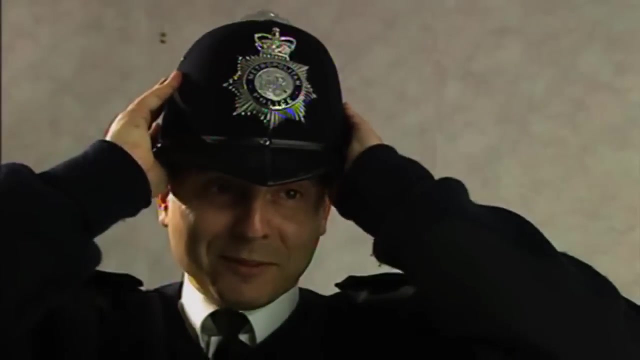 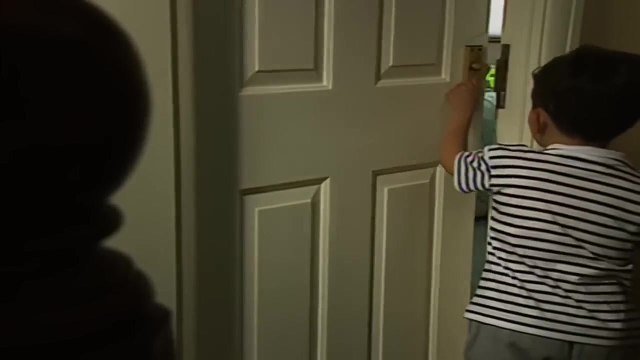 Bye-bye, Bye, Bye-bye, Bye-bye, Bye-bye, Bye, Bye-bye, Mm. Oh, Again, again, Again, again, God, Okay, again. Hello, My name's David. My dad is a policeman. Come and see his uniform Here's. 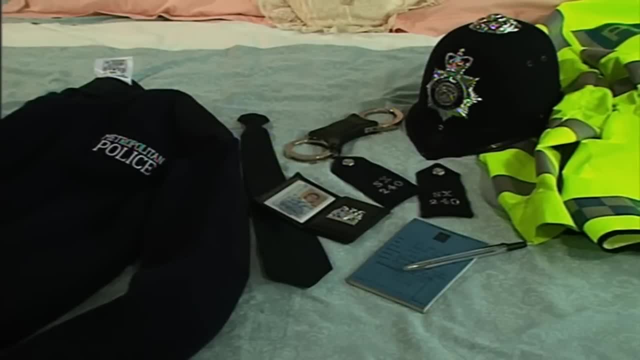 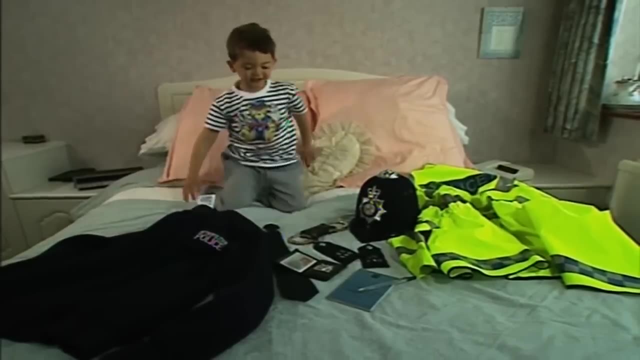 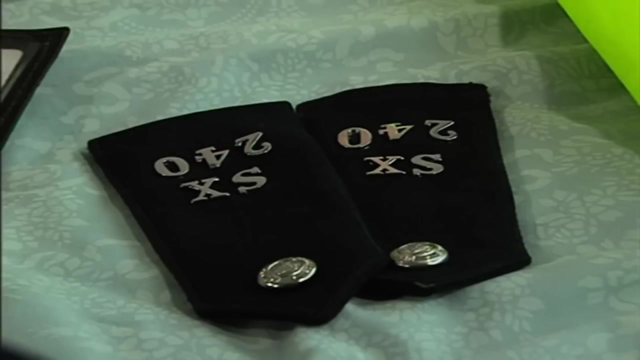 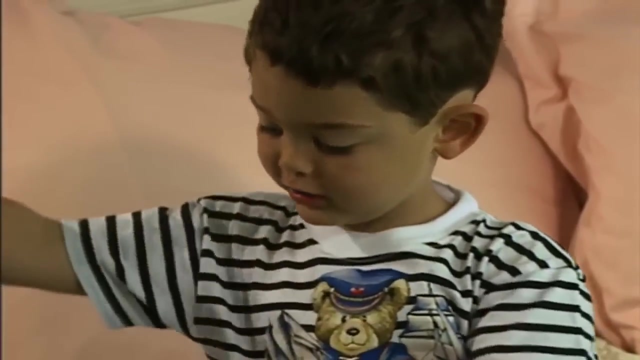 his uniform on the bed: His hat, his jumper and his badges. This is daddy's helmet And he wears it on his head. These are his numbers for his arms And he wears a tight bit of length in his neck. It's my daddy's night book. 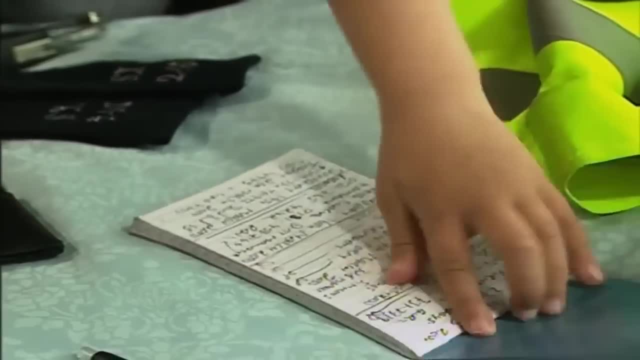 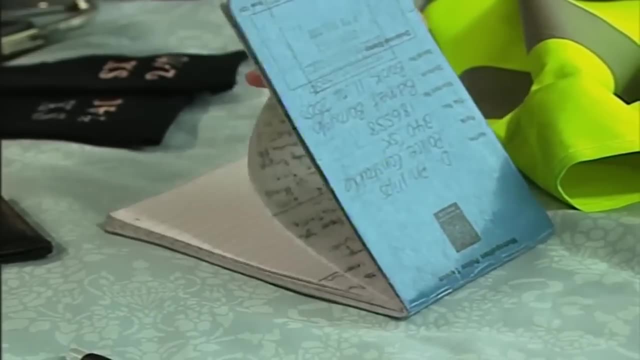 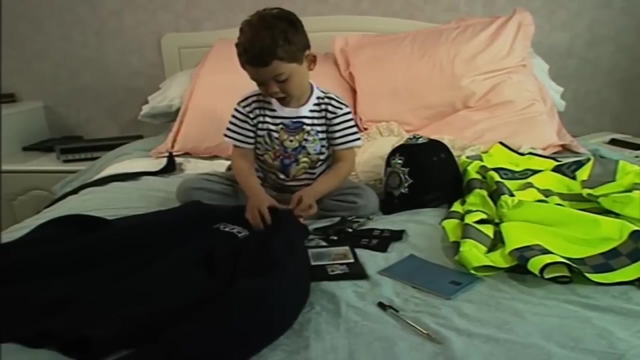 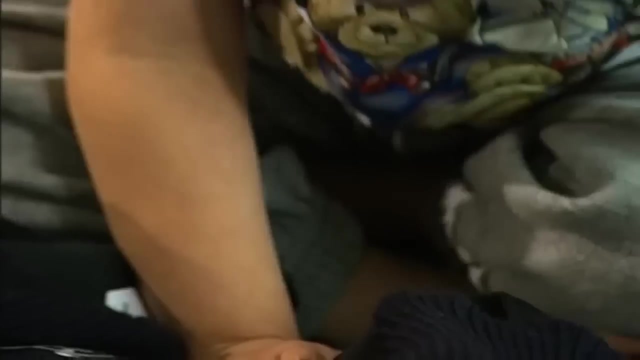 They're writing inside The two: One writing, Two writing And another writing. That pencil goes in here And it makes it really tight so it doesn't fall out the bottom end. Look, you put it there and you put it inside here. 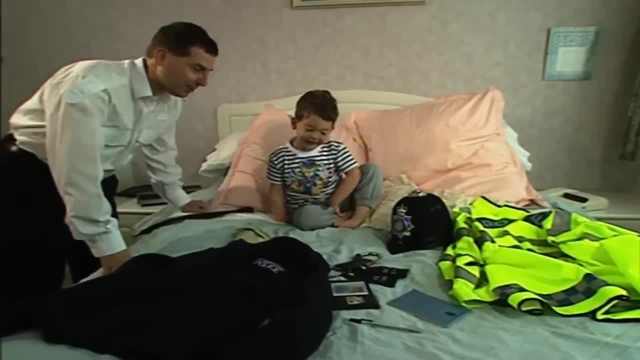 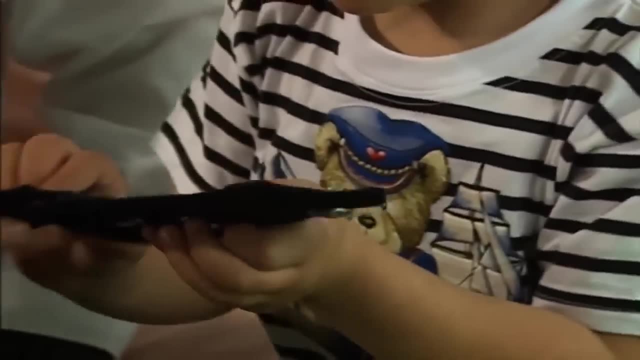 Hello David, You've been getting a lot of letters from your dad. I've been getting all my things ready for work. Yeah, I saw, I published it. I did that. And what did you do with my numbers? I posted them up. 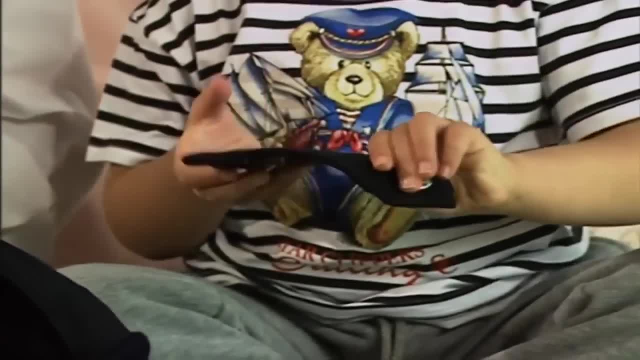 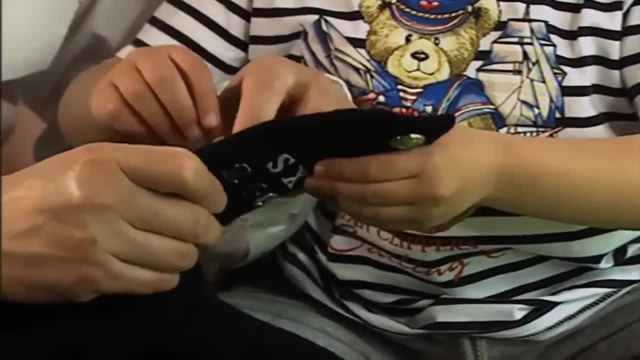 Good Shall, we put them on my jumper. Pull that off. That's a good noise. Okay, It's hard to put it through, isn't it? I'll do this, I'll do this bit. Okay, Hold that and stick it on. 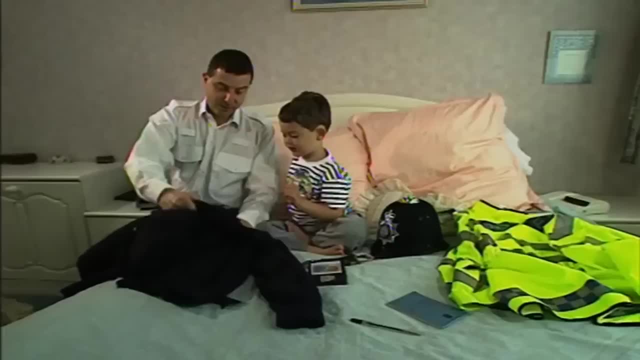 And stick. That's it. Okay. Now put your jumper on. Okay, Help me, I'm going to stand up and put it on your head. Okay, That's good. Now I'm going to put it on now, Okay. 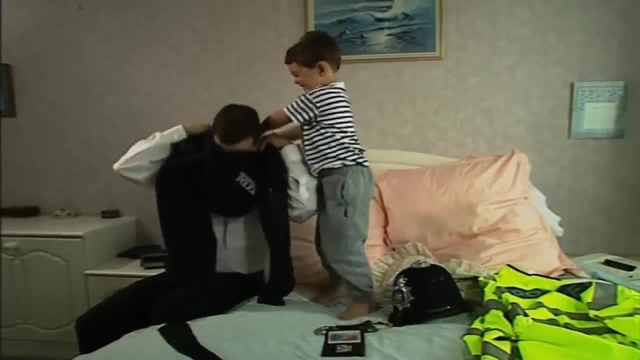 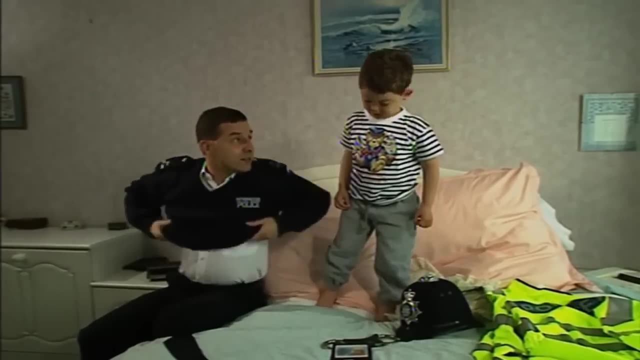 And then We've got my tie to put on. Tie, It's a special tie, isn't it? I can put it on. Tuck it in for me. Tuck it in, Okay, Okay, Okay, Okay Okay. 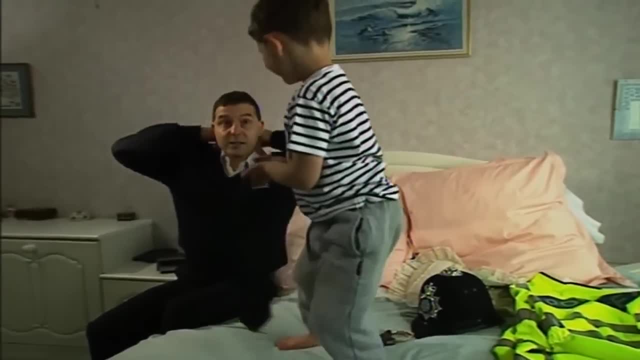 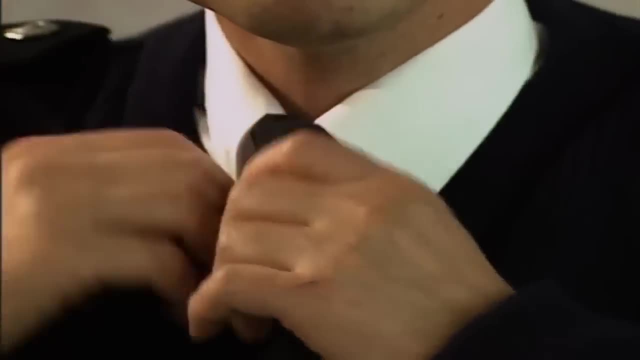 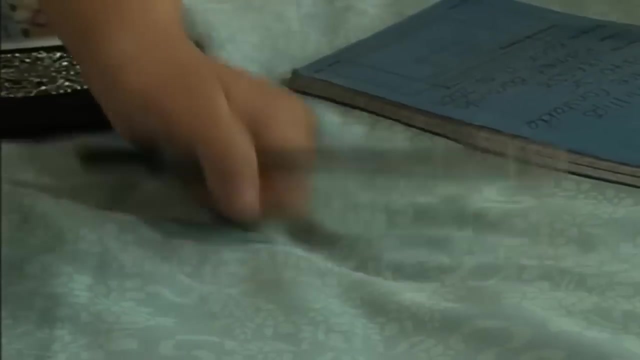 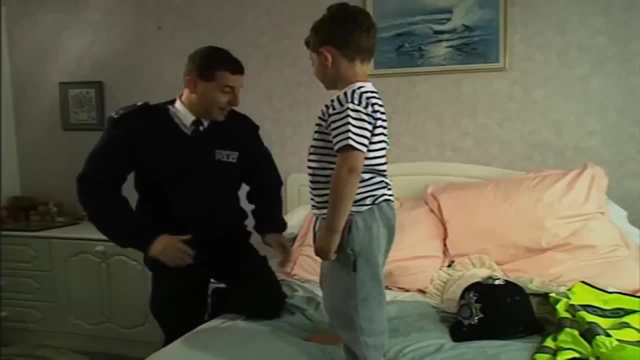 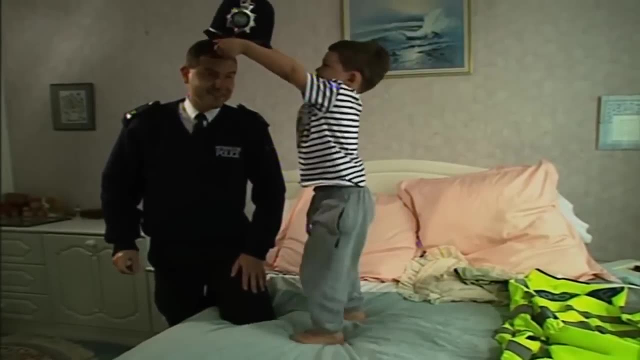 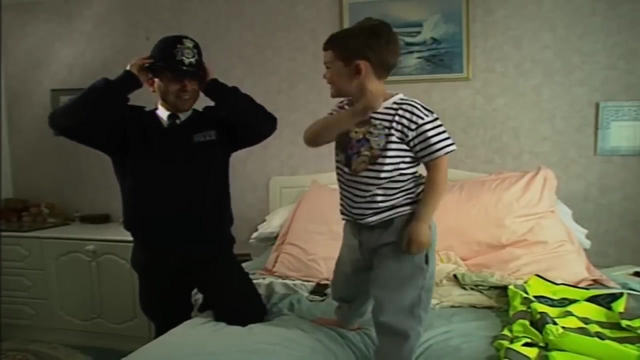 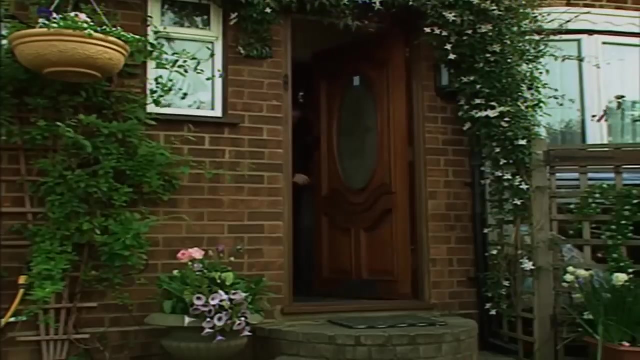 Super duper, Super duper And my helmet. please Open it for your head, Okay, All right, Perfect, I have to straighten it a little bit. Thanks very much. Come on then. Wow, Okay, I'm off to work now. 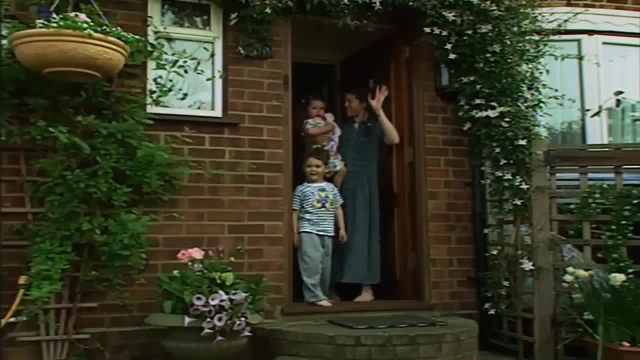 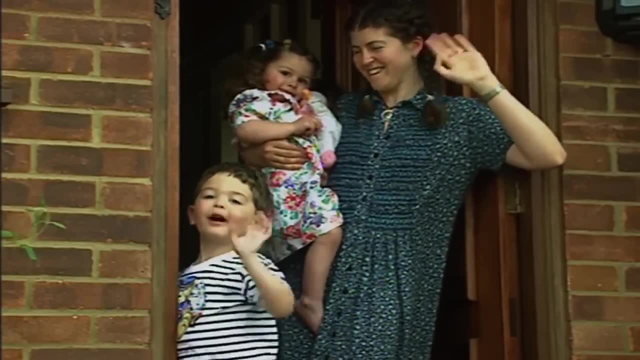 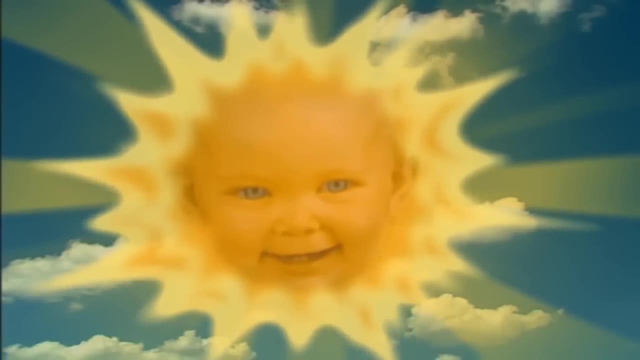 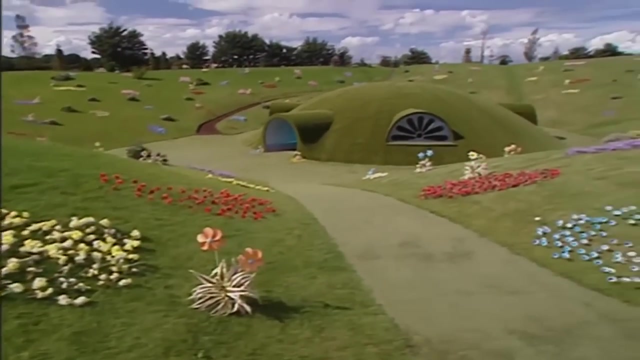 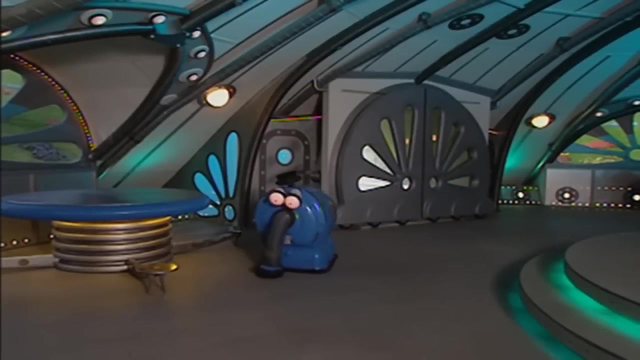 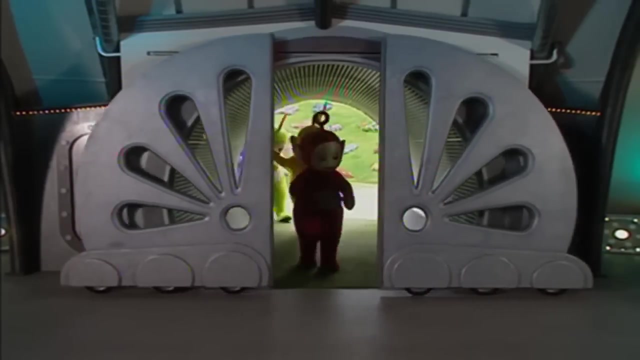 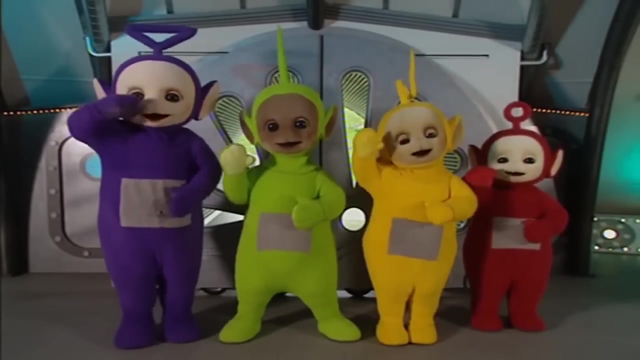 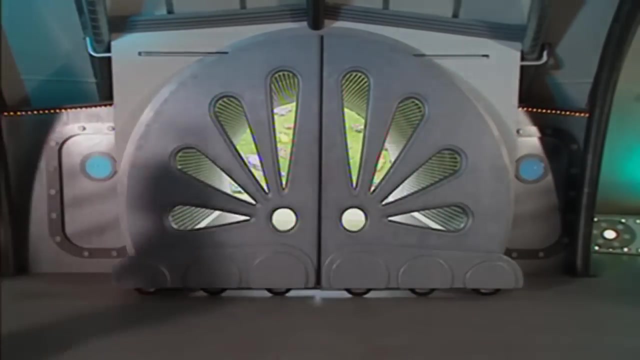 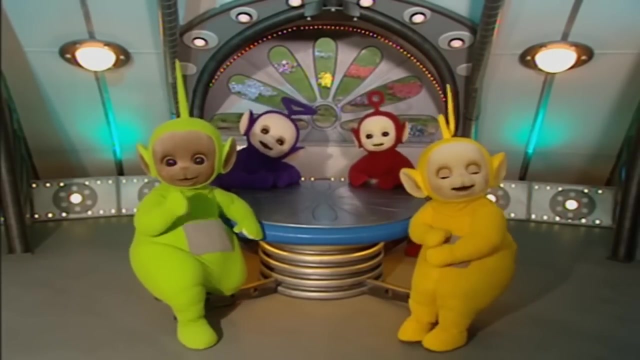 Bye, Bye-bye, See you later. Have a good day. Bye-bye, Sissy, See you later, Bye-bye, Bye-bye. One day in Teletubbyland, the Teletubbies heard a funny noise. 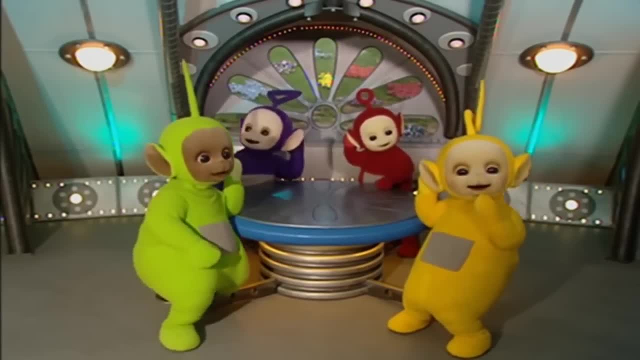 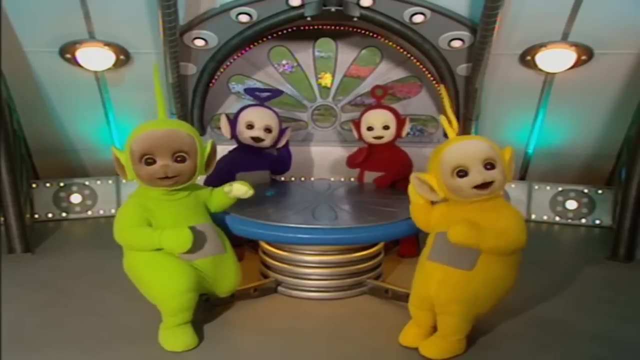 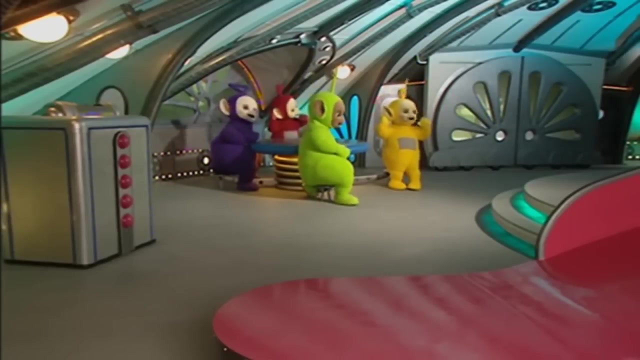 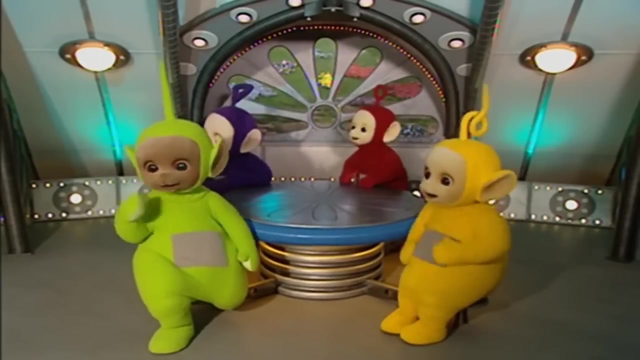 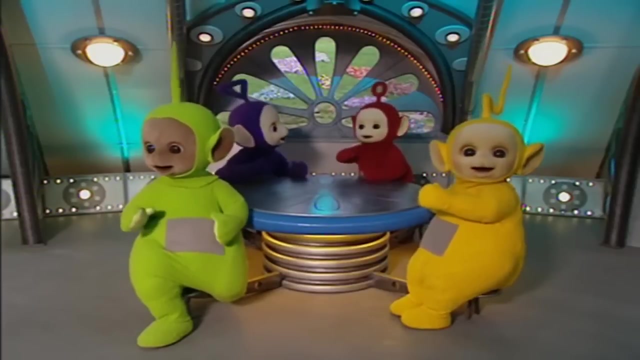 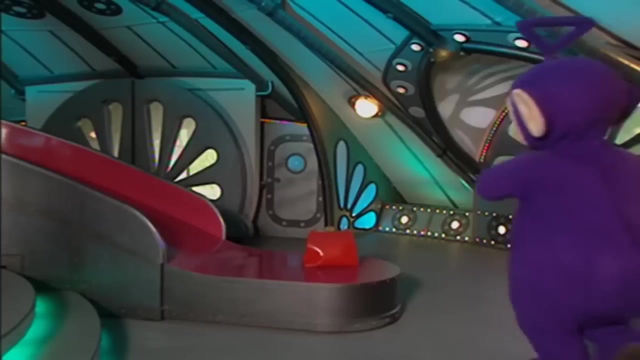 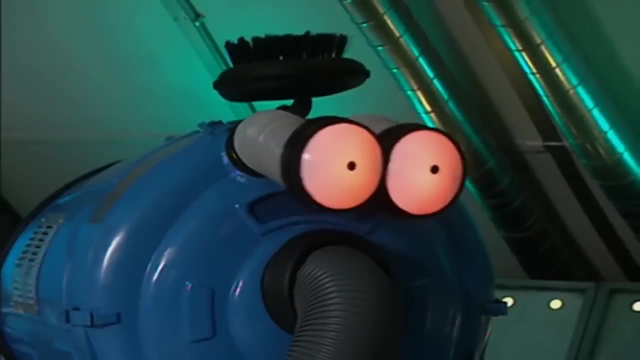 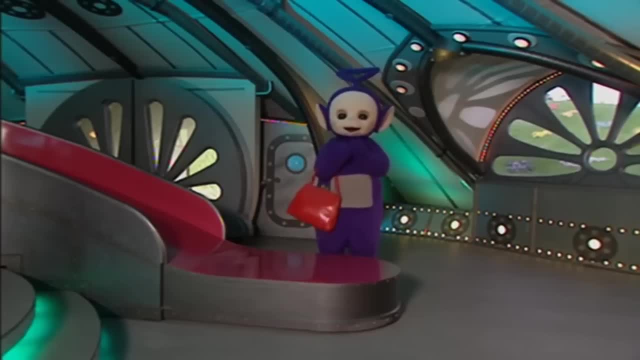 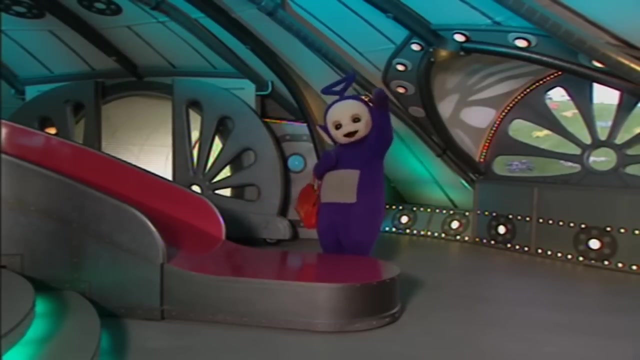 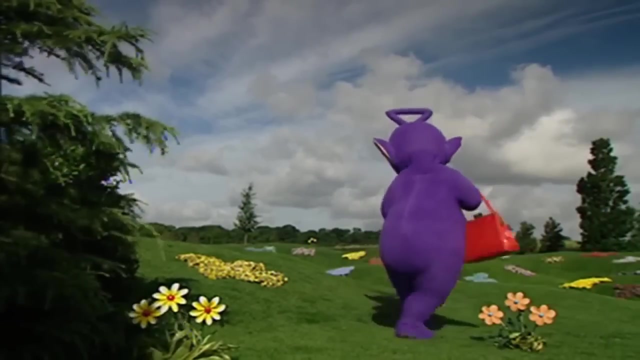 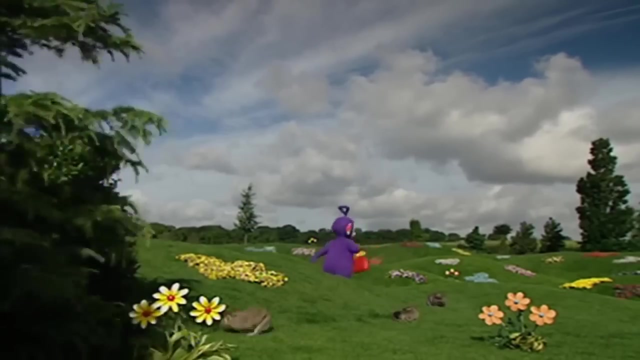 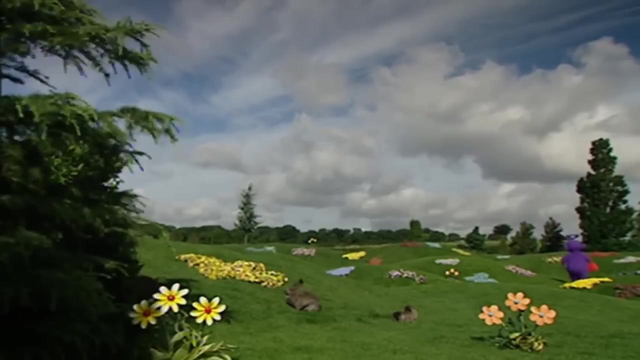 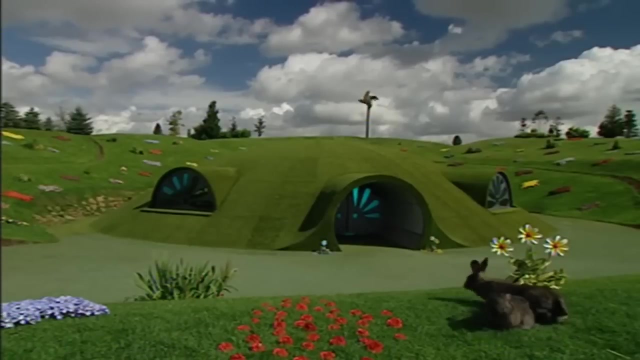 With his bag. With his bag, Tinky Winky walked back. Bye-bye Dipsy, Bye-bye Lala, Bye-bye Poe, Bye-bye Tinky Winky. Oh Then Dipsy, Lala and Poe heard another funny noise. 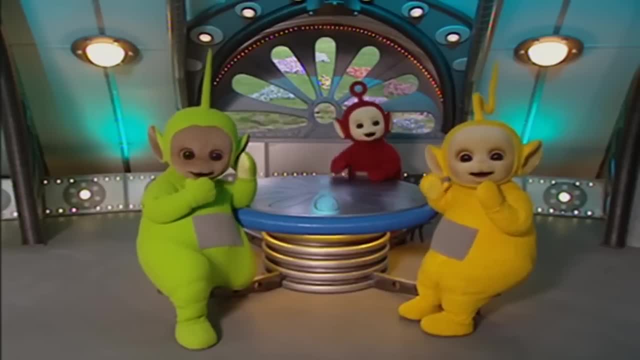 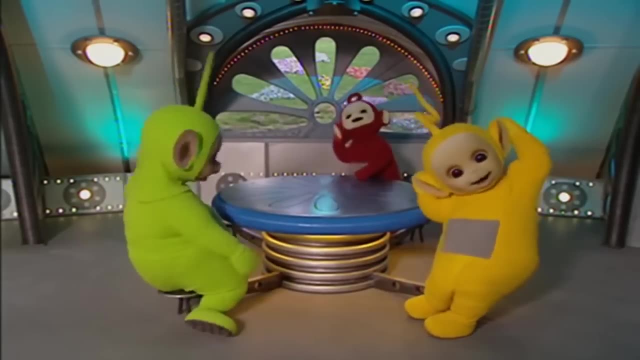 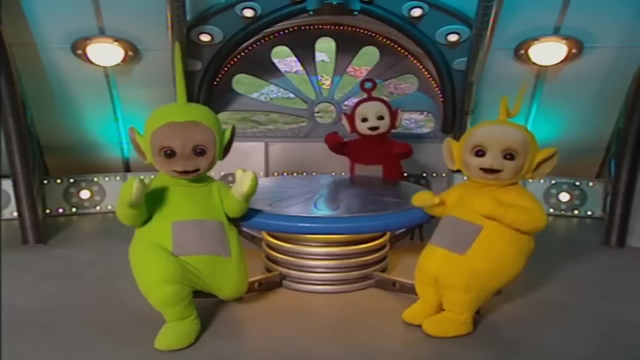 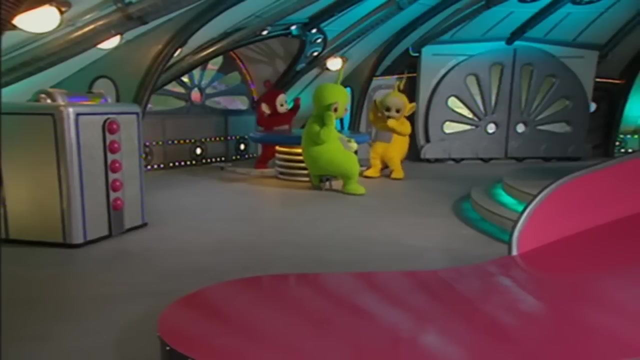 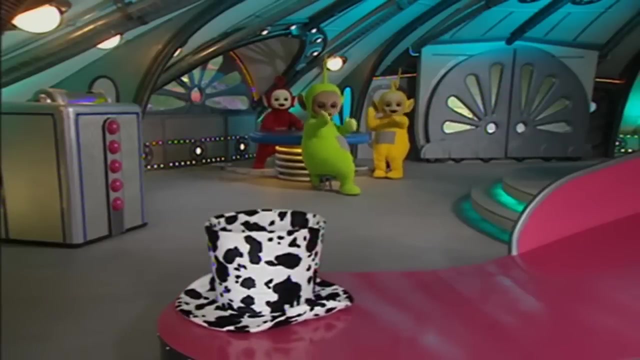 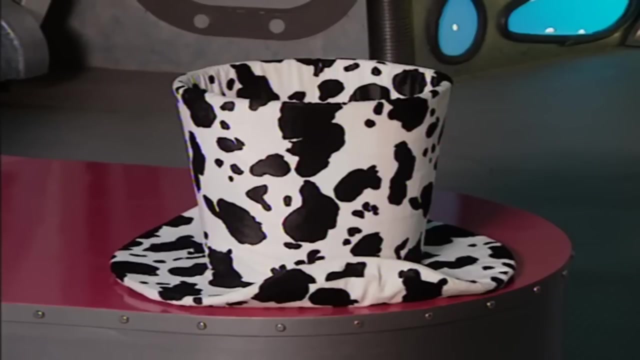 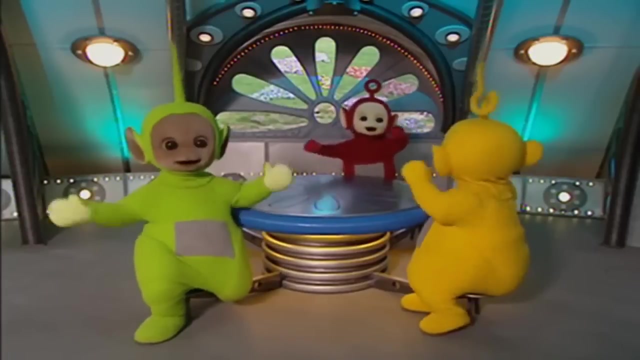 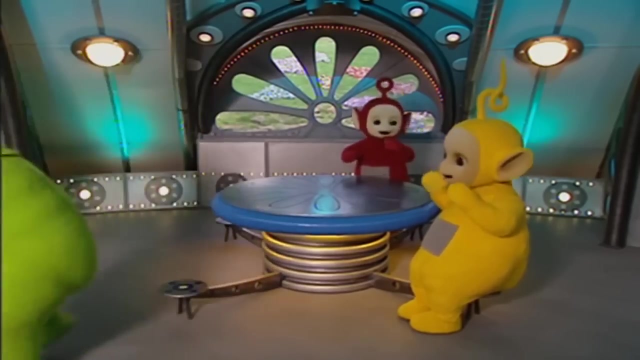 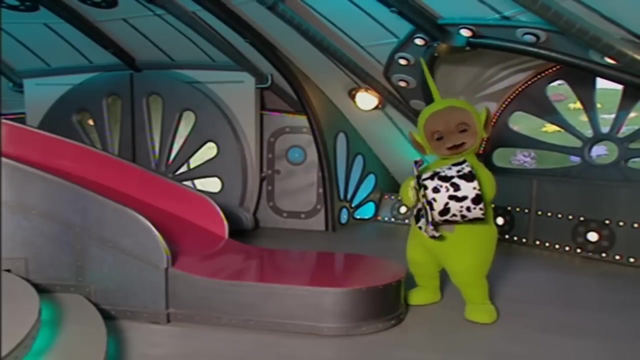 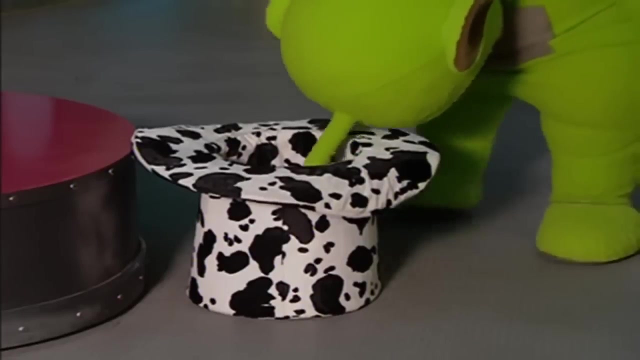 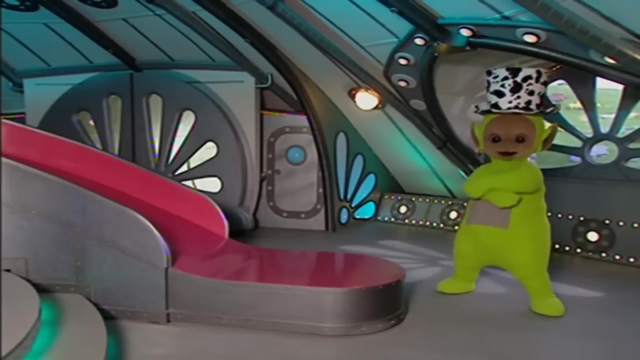 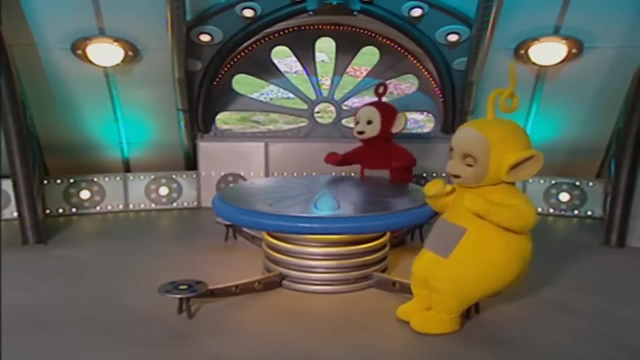 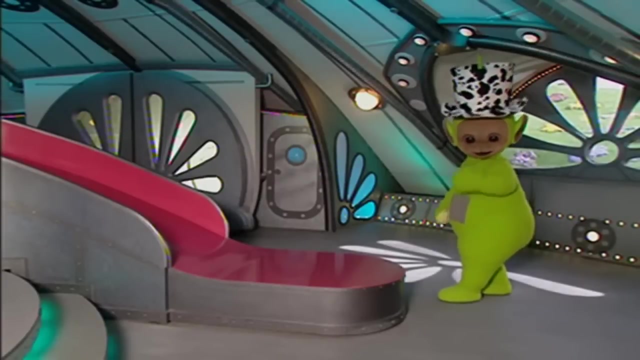 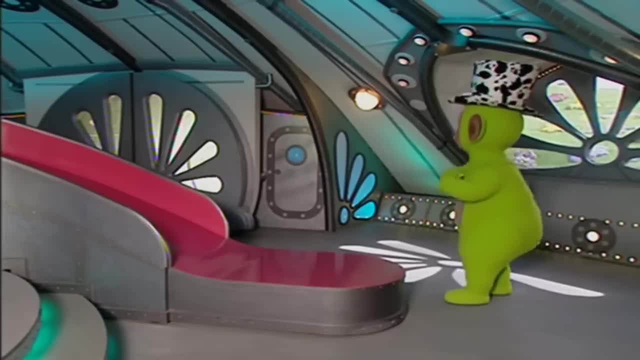 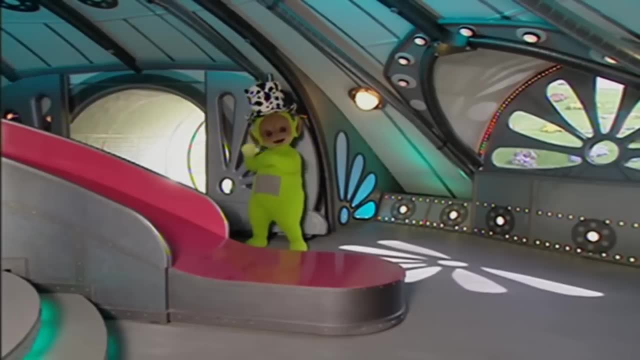 Dipsy walk hat. Bye-bye Lala, Bye-bye Poe, Bye-bye Dipsy, Bye-bye Dipsy. Dipsy walk hat, Dipsy, walk hat, Dipsy walk hat. 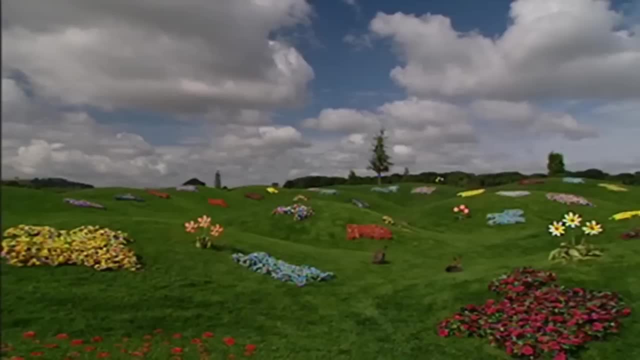 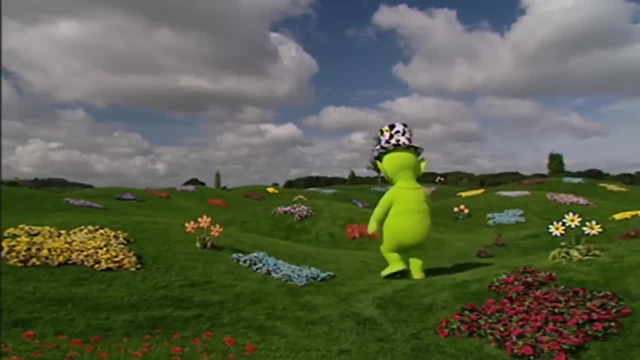 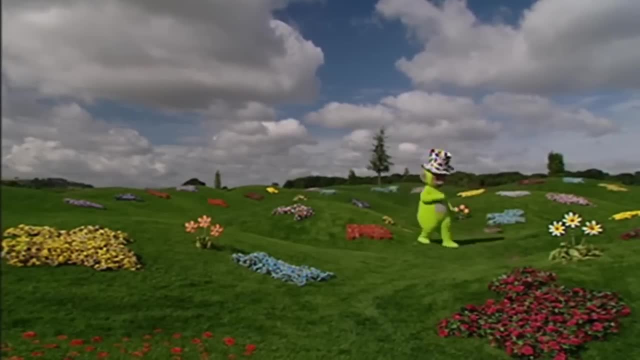 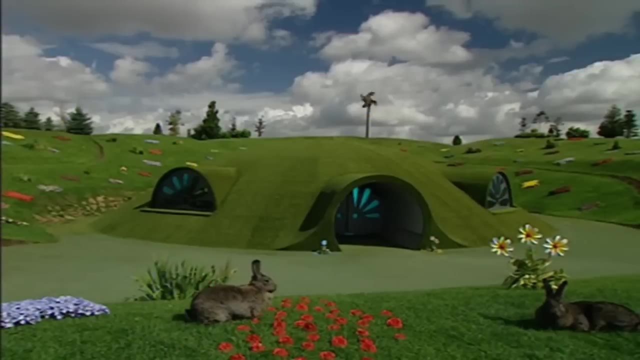 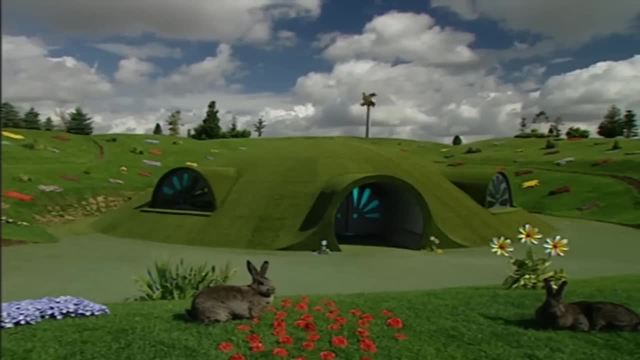 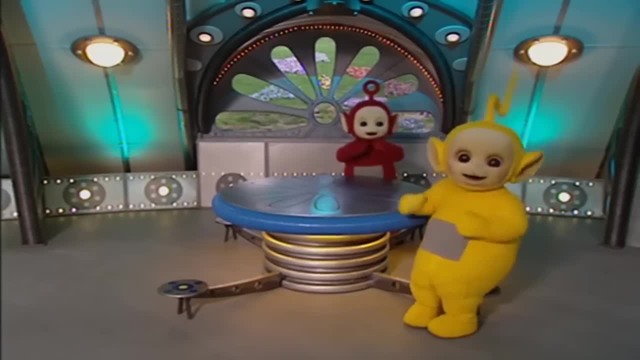 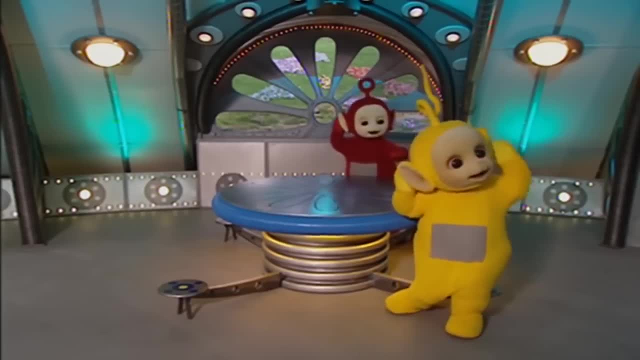 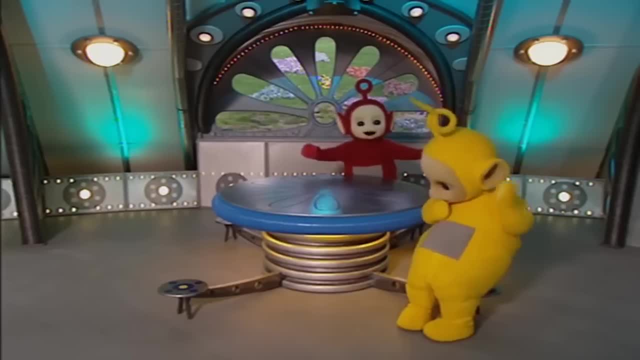 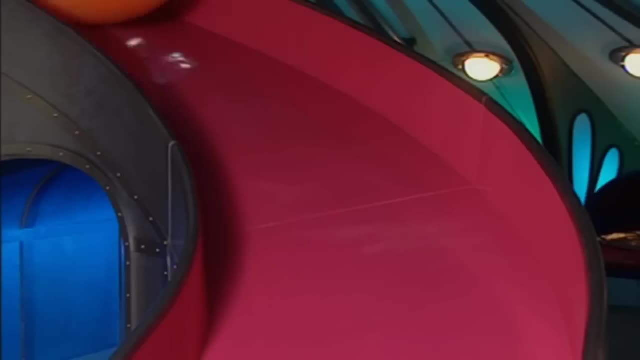 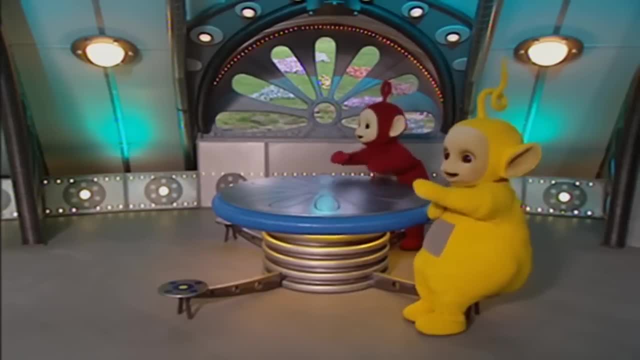 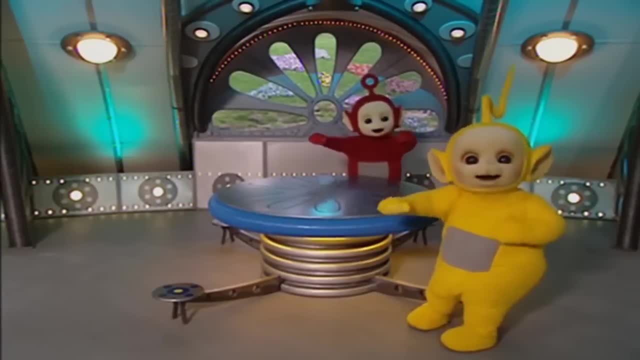 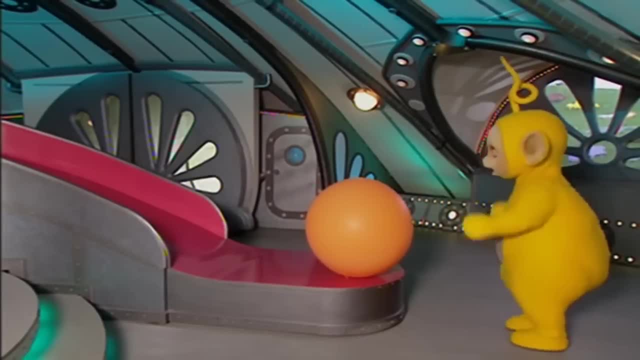 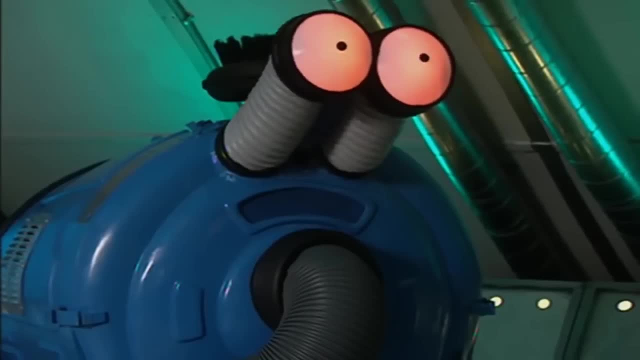 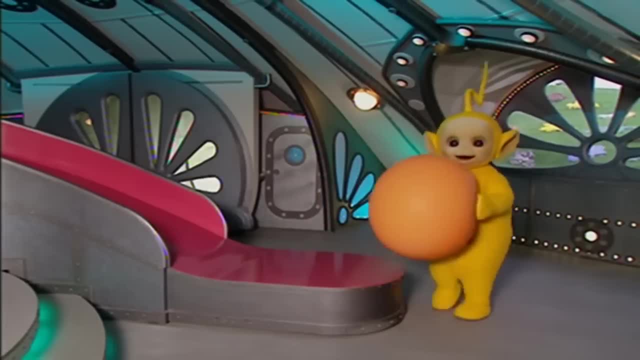 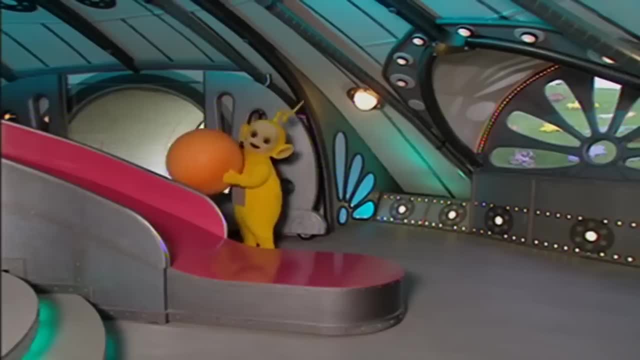 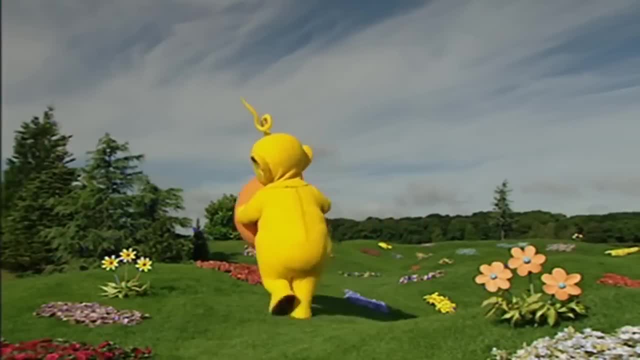 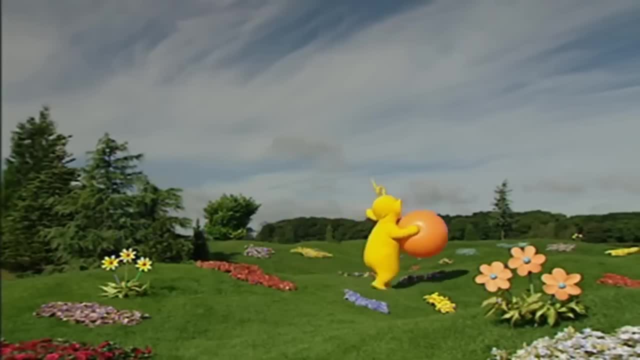 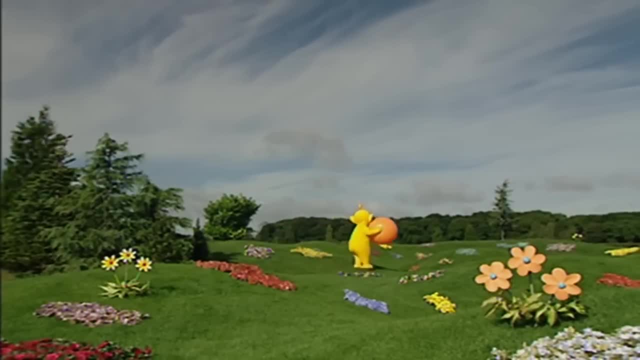 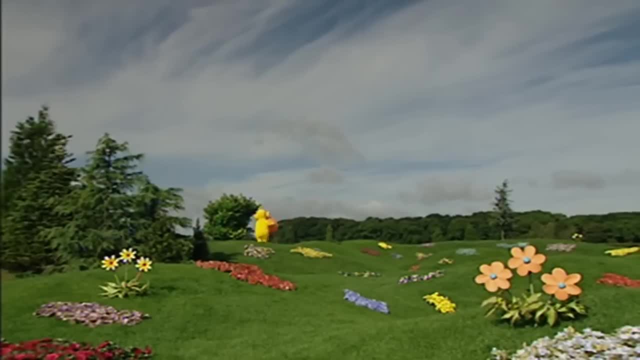 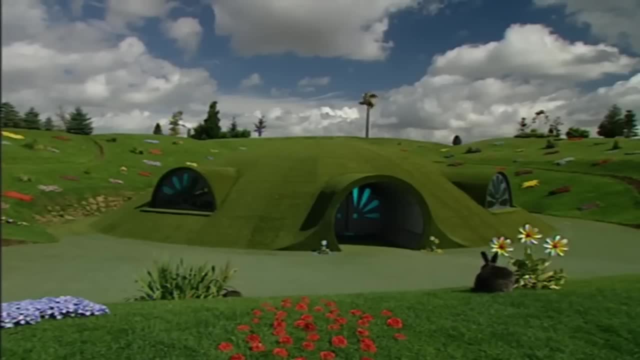 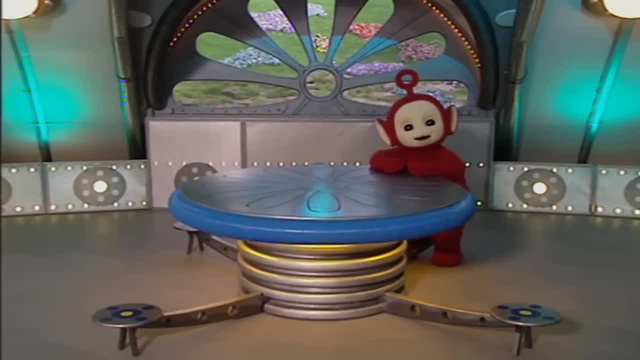 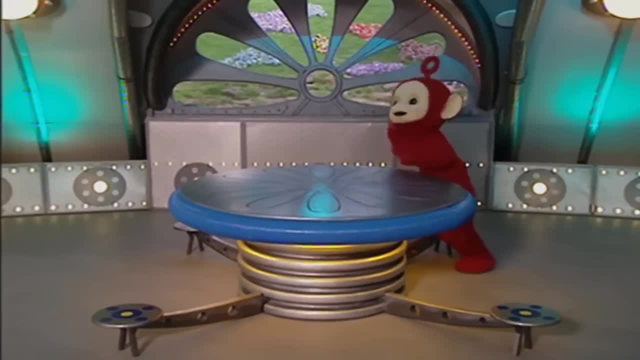 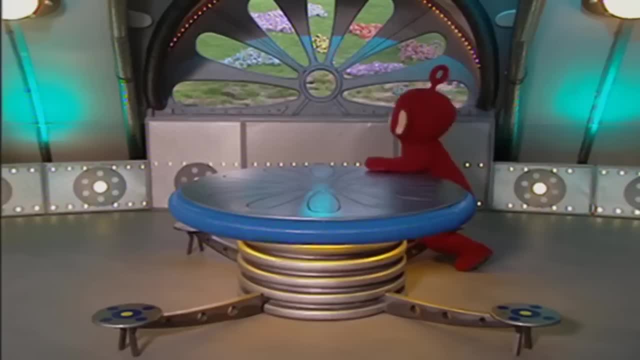 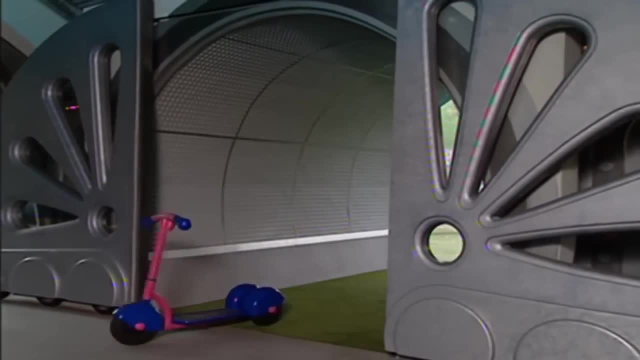 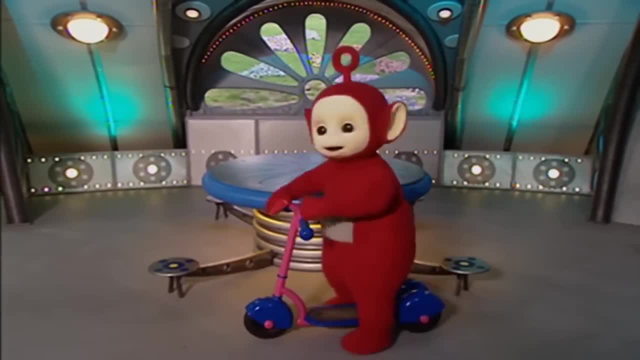 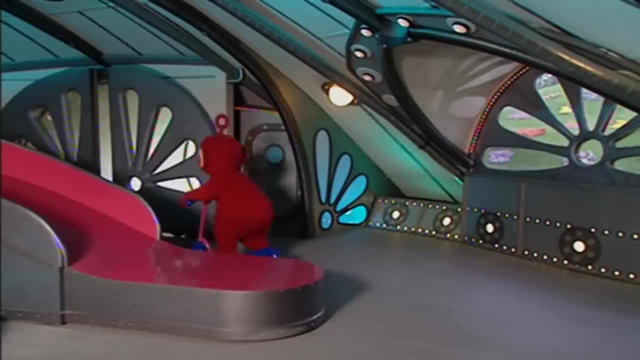 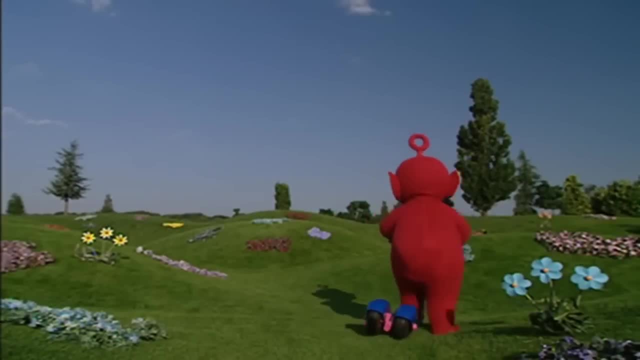 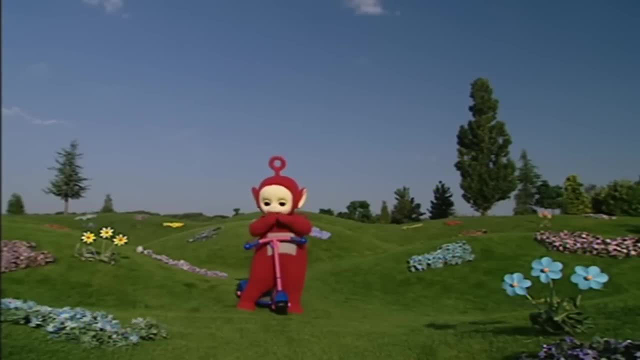 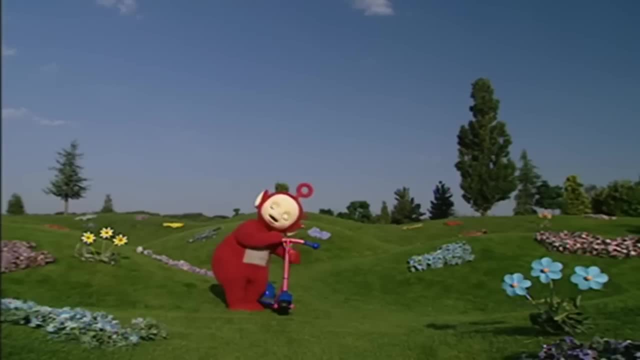 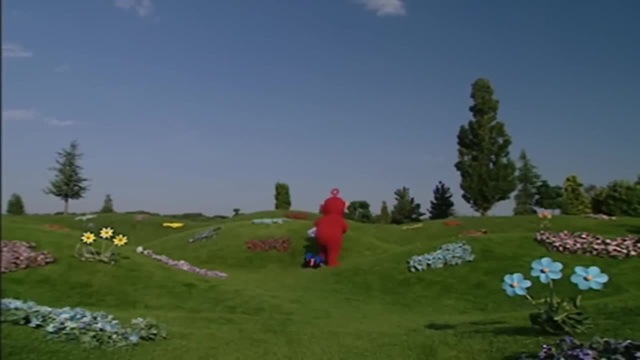 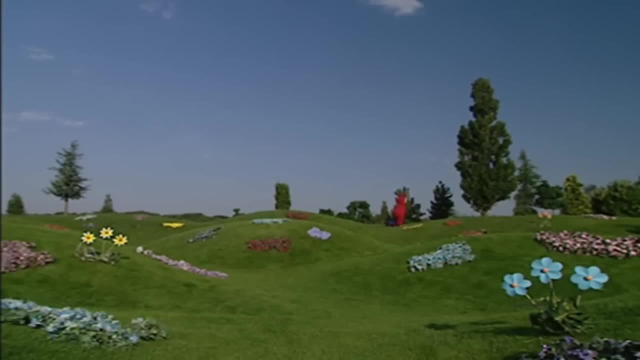 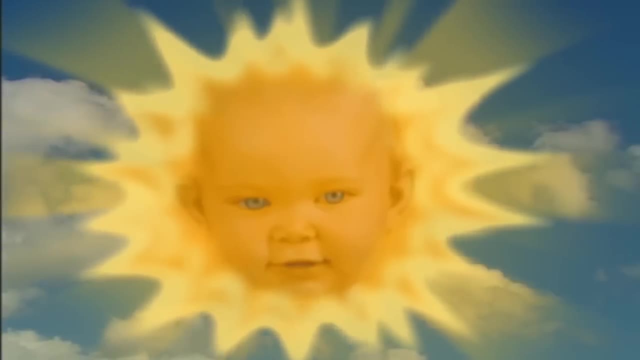 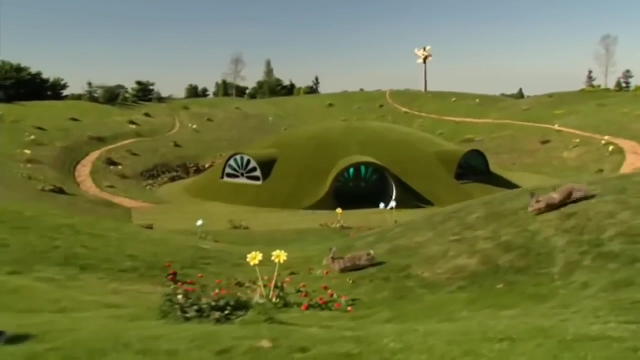 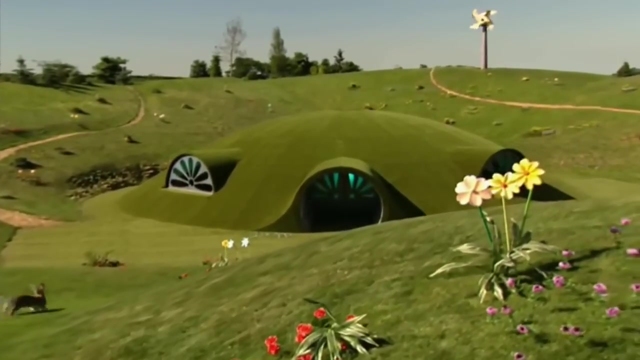 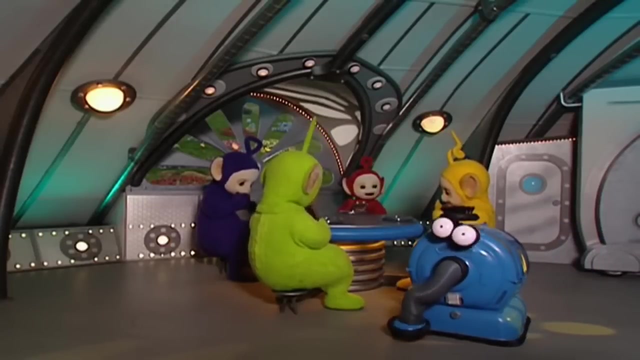 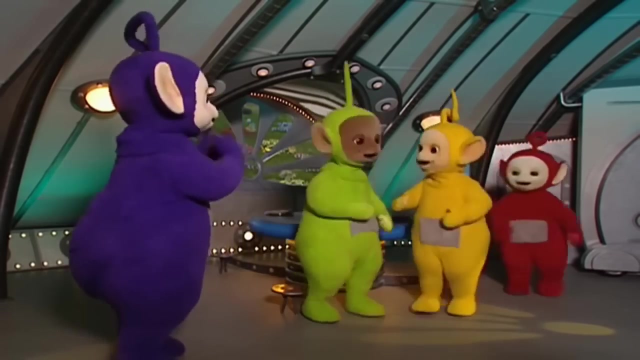 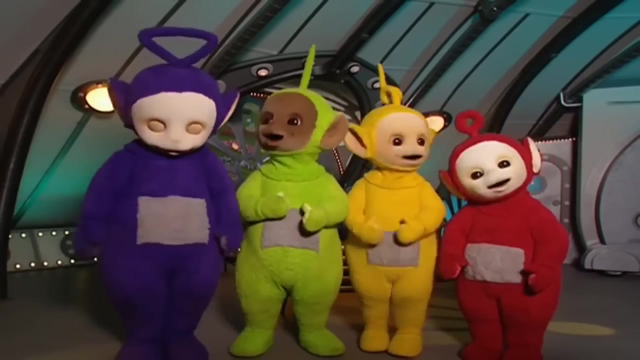 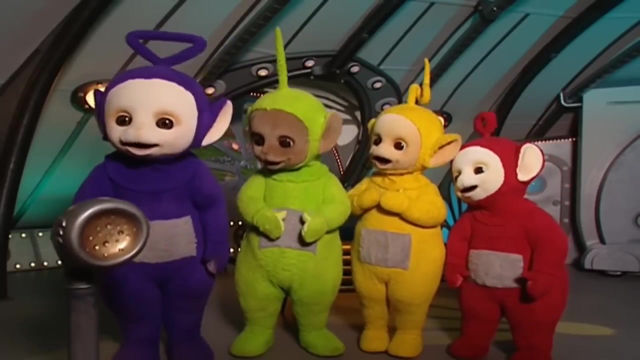 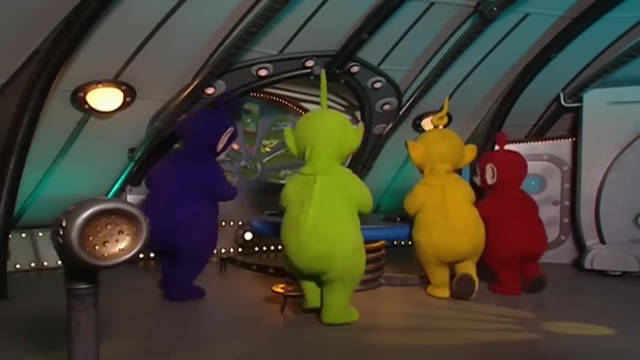 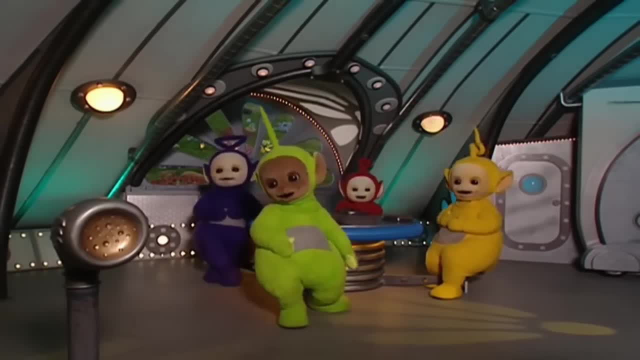 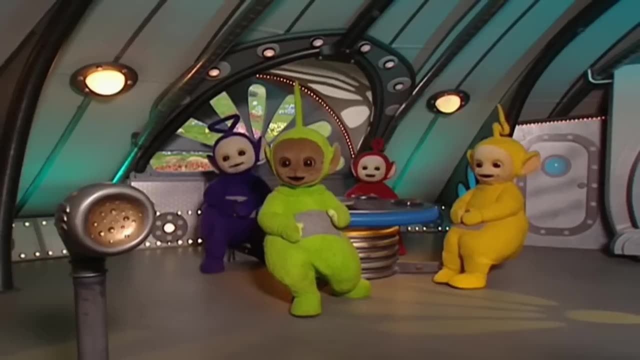 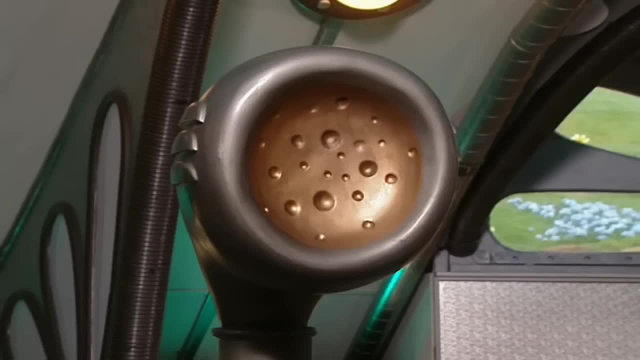 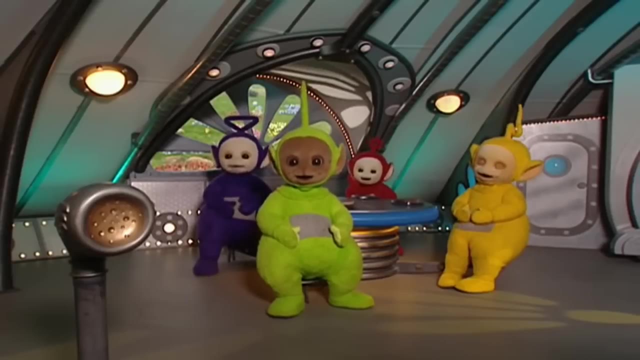 What's that? Again, again, Again, again, Again. Hark Hark. The dogs do bark. Hark Hark. The beggars are coming to town. The beggars are coming to town, Some in rags. 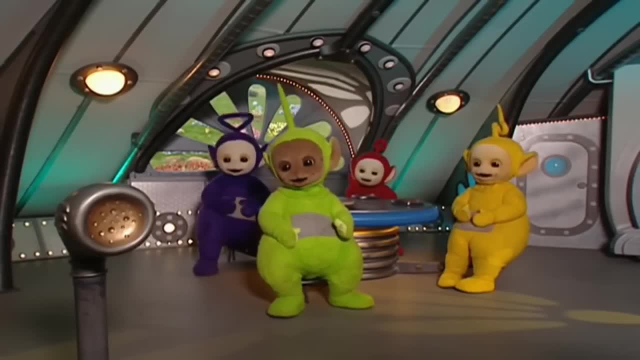 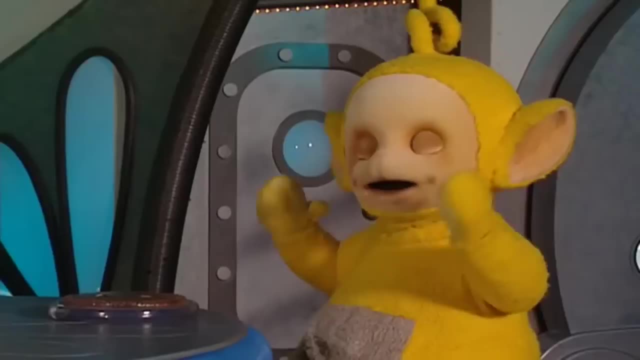 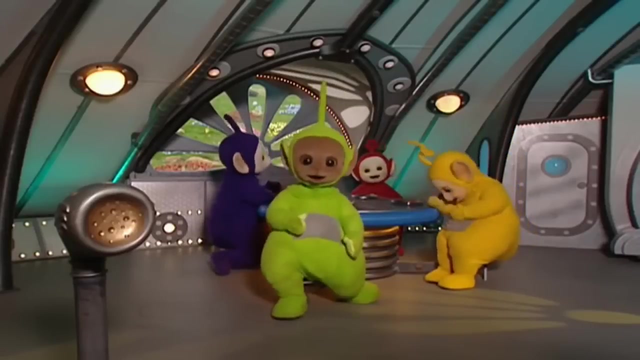 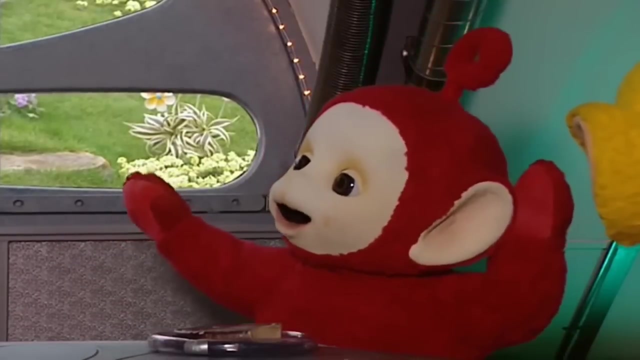 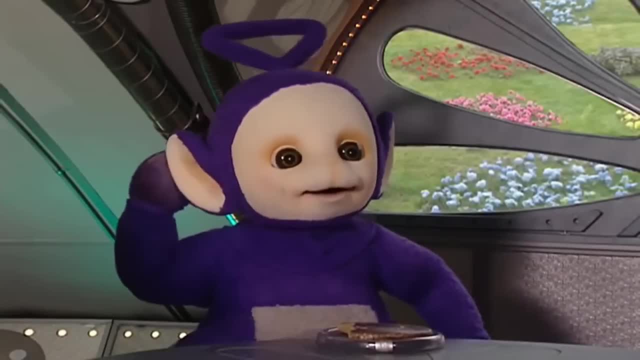 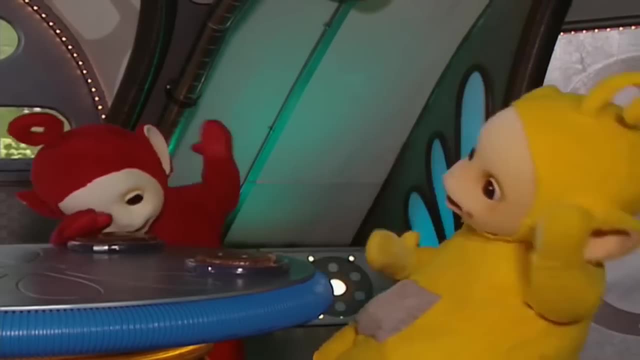 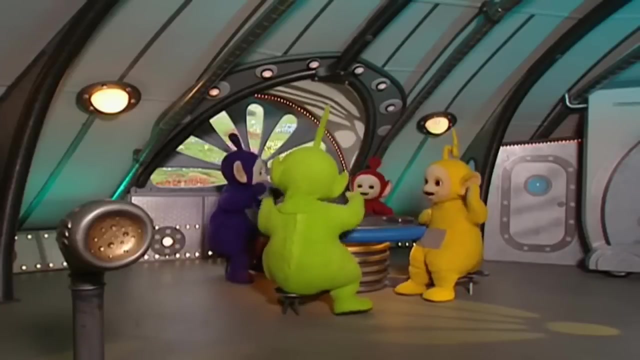 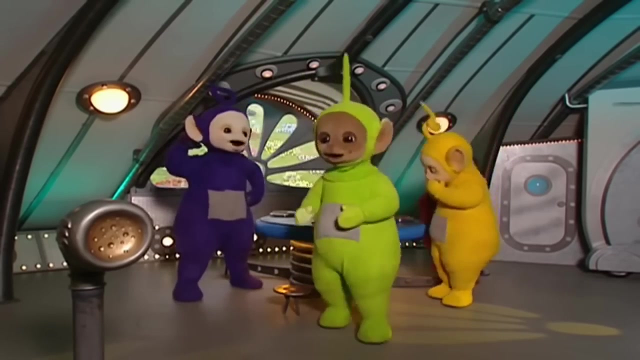 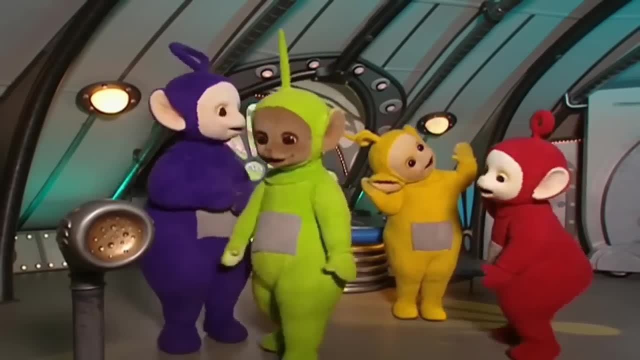 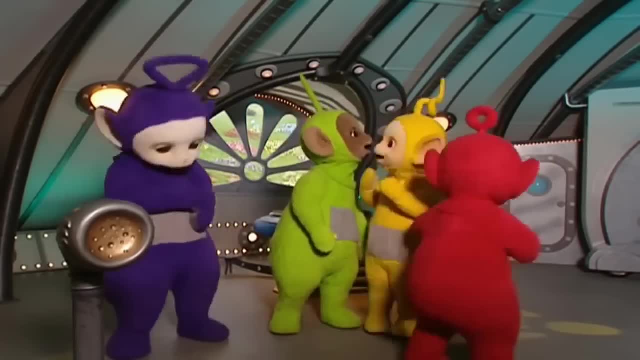 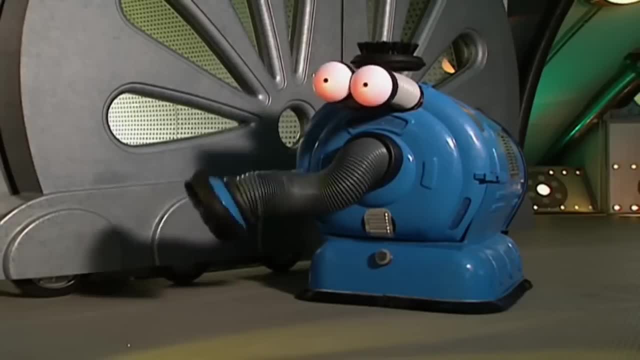 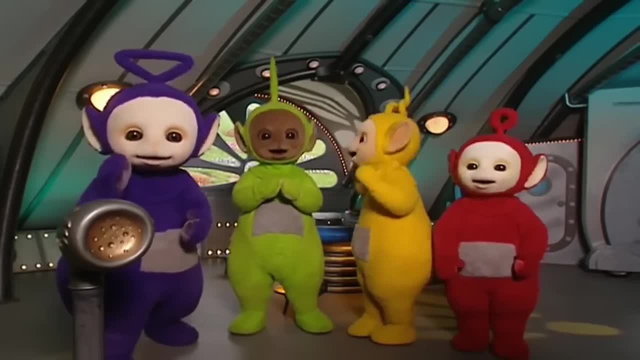 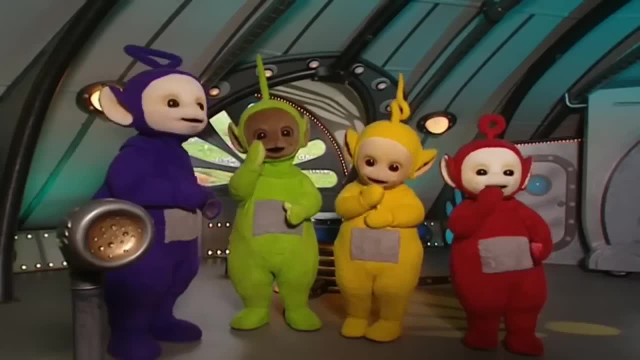 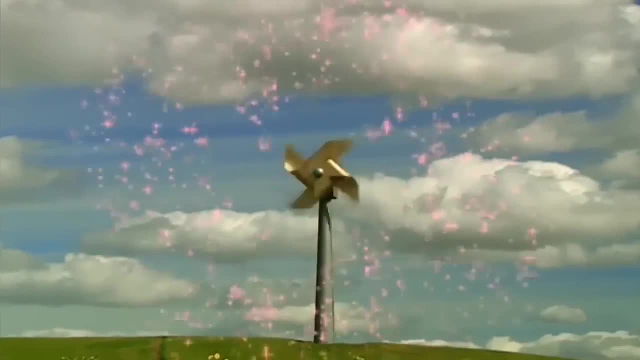 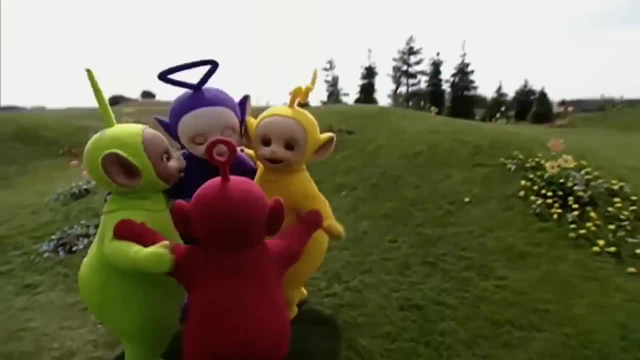 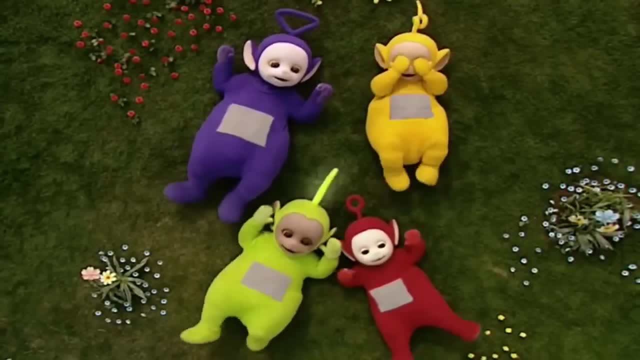 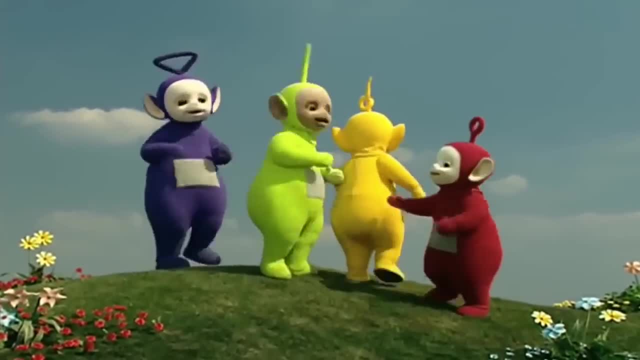 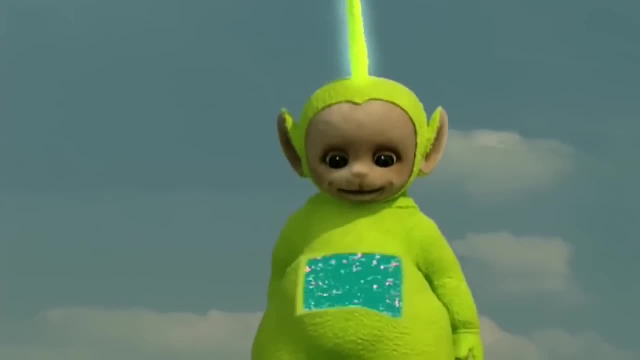 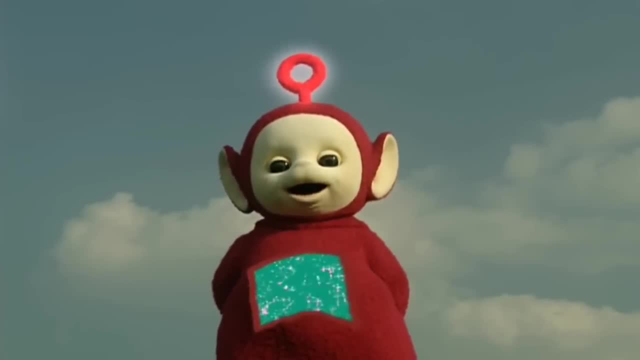 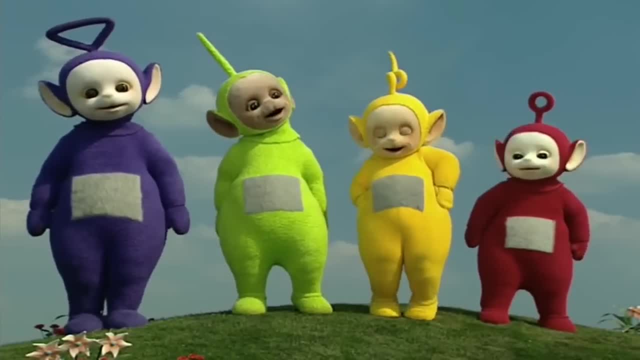 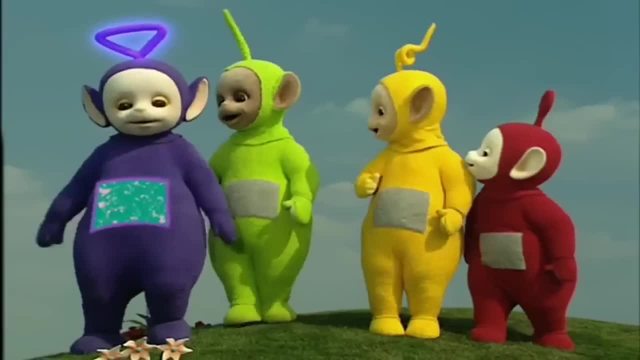 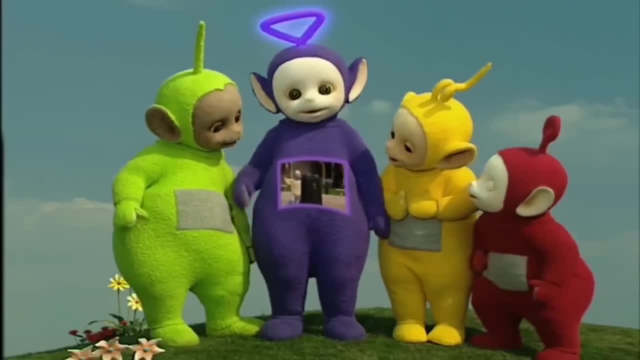 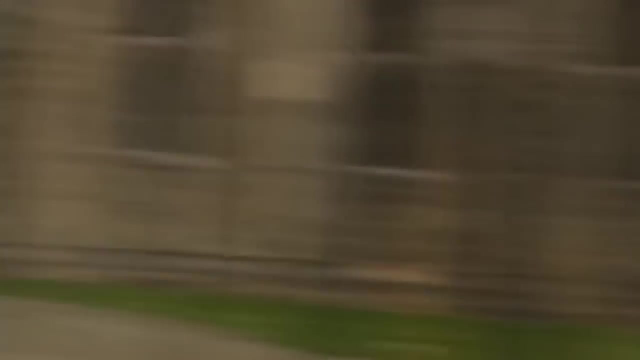 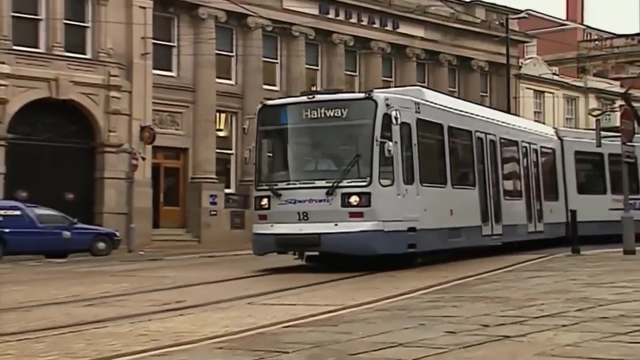 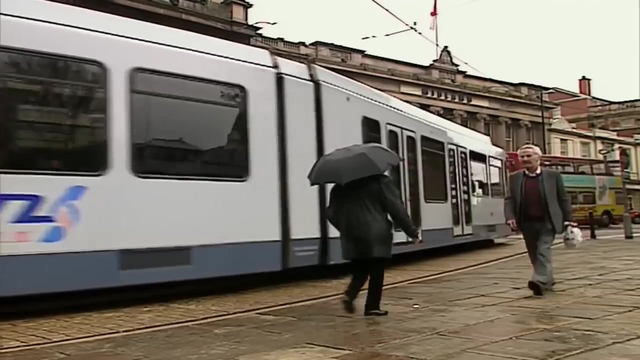 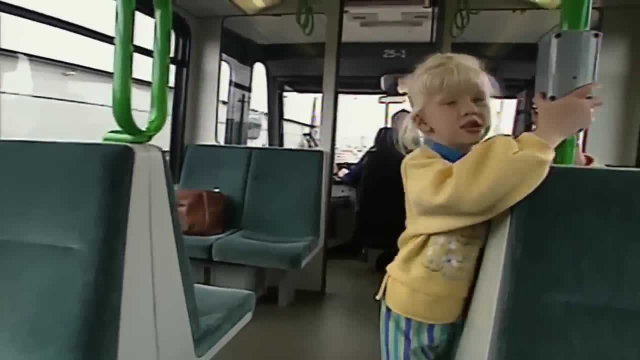 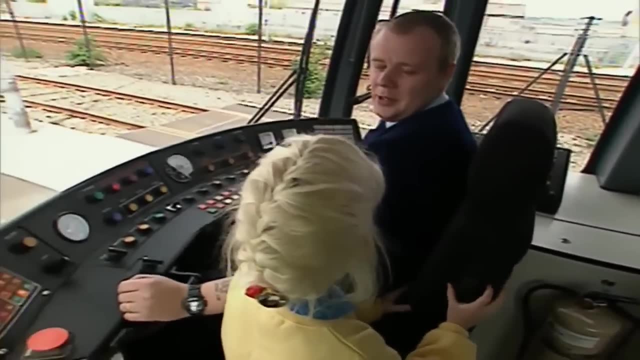 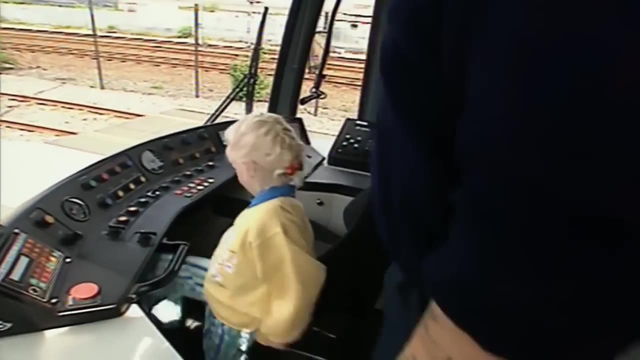 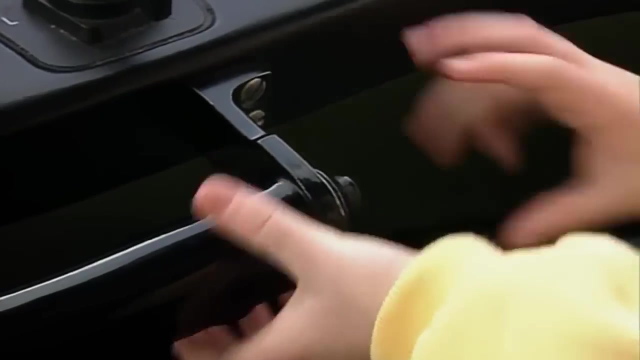 My Daddy's driving. This is where Daddy sits. Here's Daddy, Hello, Hello, Becky. Hello, Do you want to come and sit in my seat? Do you want to show me where the bell is? This is the bell. This is the horn. 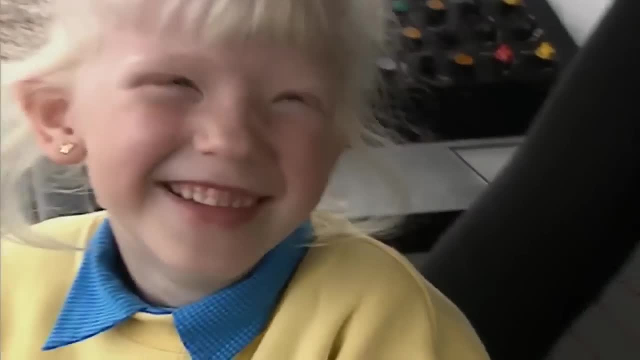 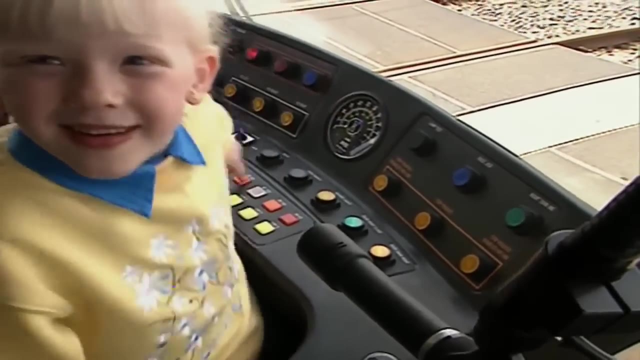 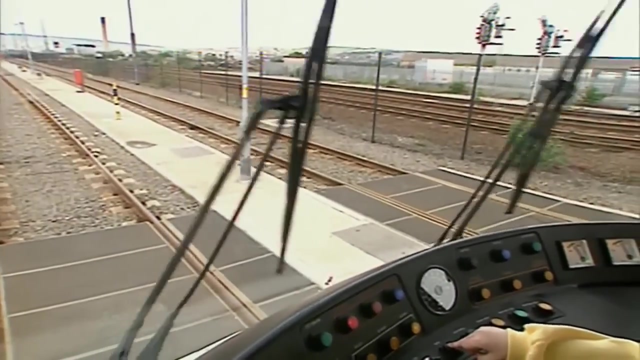 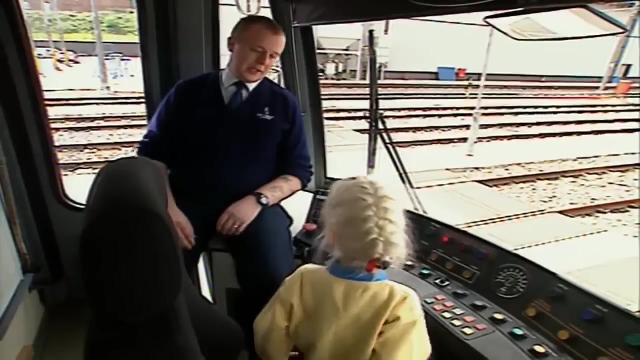 BELL RINGS Next stop the next way. There's the window washer. The window washers are my favourite Right. come on, Bex, it's time to go. You don't sit with Mummy. This is Mummy. 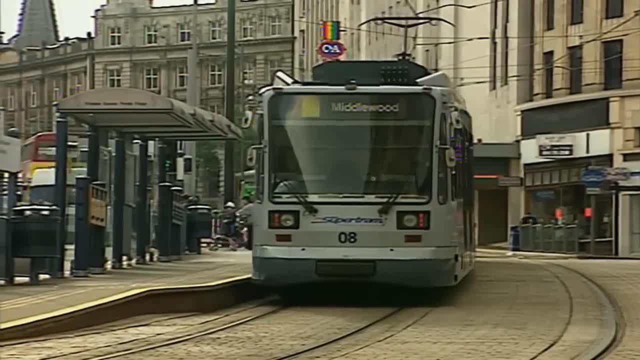 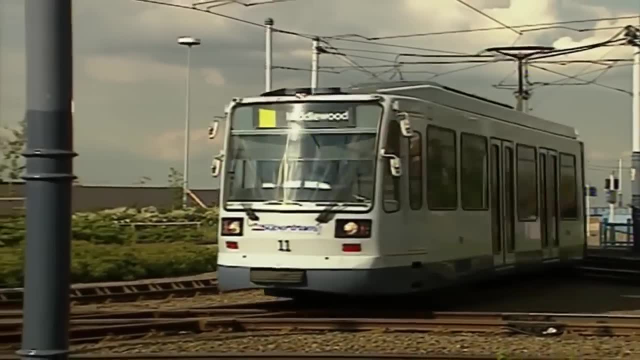 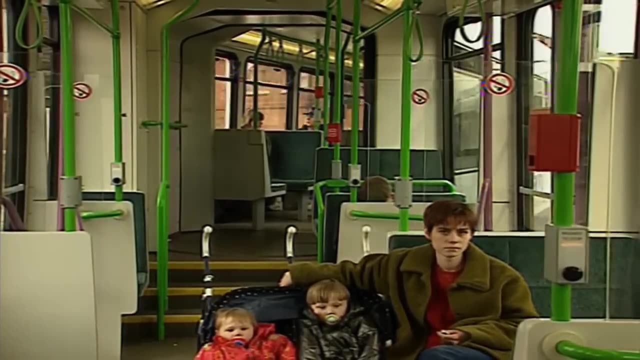 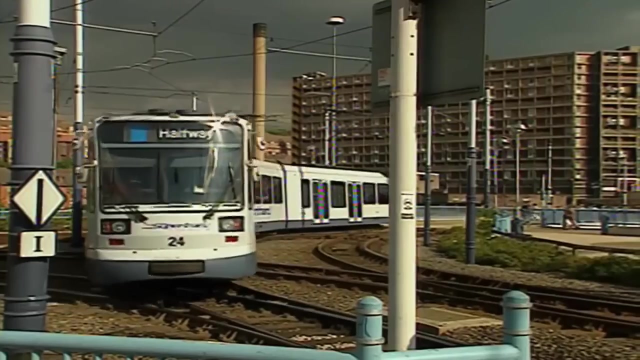 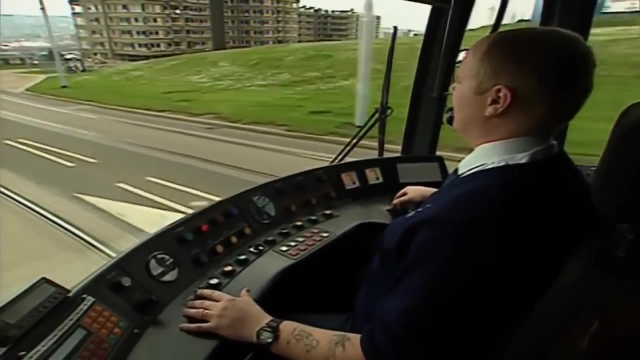 Hello, Where are we going round the corner? Trams are all bendy. The tram's like a big snake. See how the tram goes round the corner. MUSIC PLAYS MUSIC FADES. Look, there's Daddy driving MUSIC FADES. We're going up the hill. 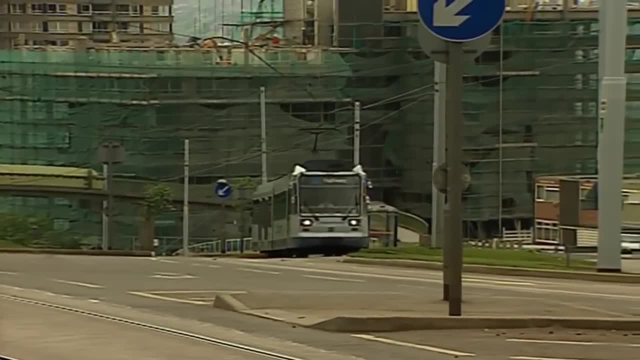 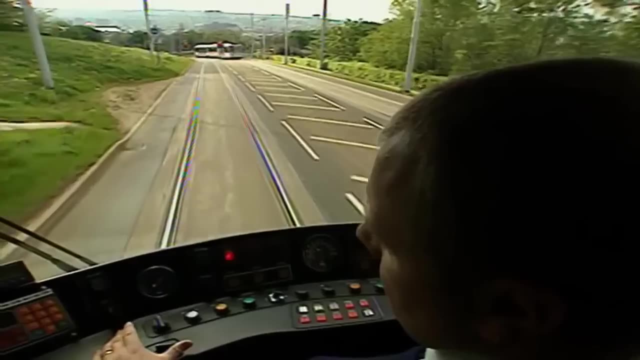 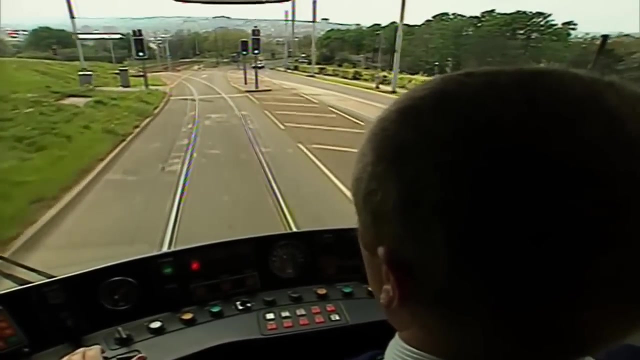 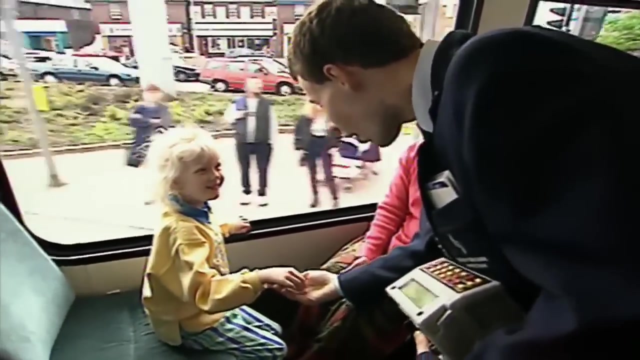 MUSIC FADES. Daddy's got a good view. MUSIC FADES- BELL RINGS. There's another tram. MUSIC FADES- Look, here's the conductor. MUSIC FADES- MUSIC FADES- Hello, MUSIC FADES- One and a half, please. BELL RINGS. 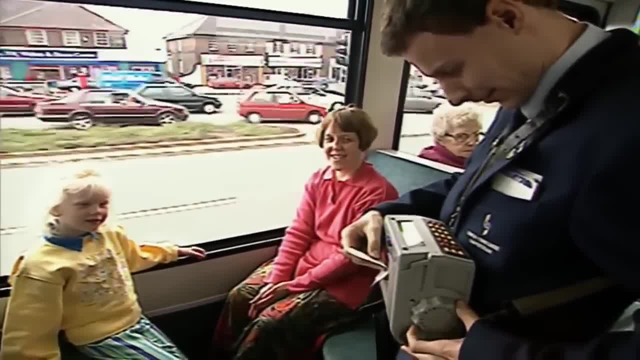 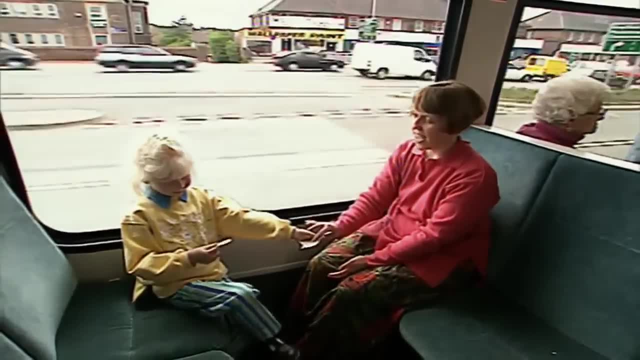 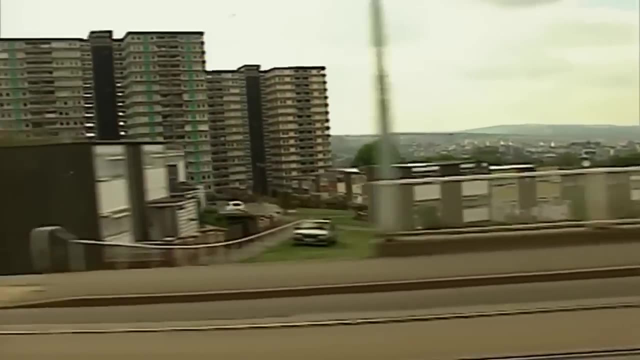 BELL RINGS, BELL RINGS, Next stop. I'll make a tent. Thank you, MUSIC CONTINUES. Thank you, MUSIC CONTINUES. That's my ticket. BELL RINGS, BELL RINGS, Ding ding ding. MUSIC FADES. 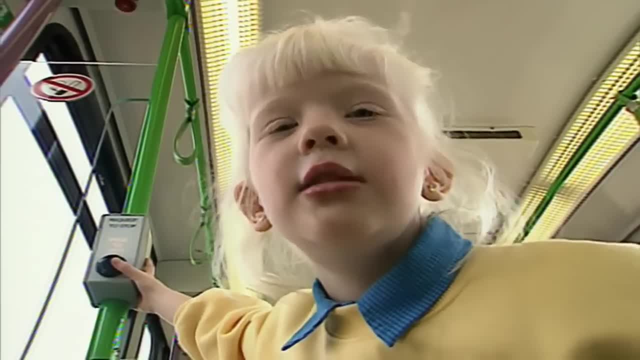 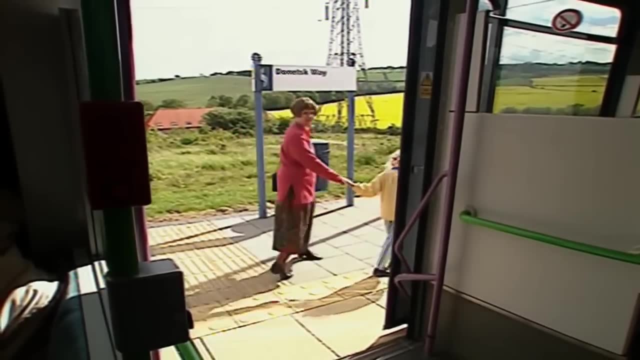 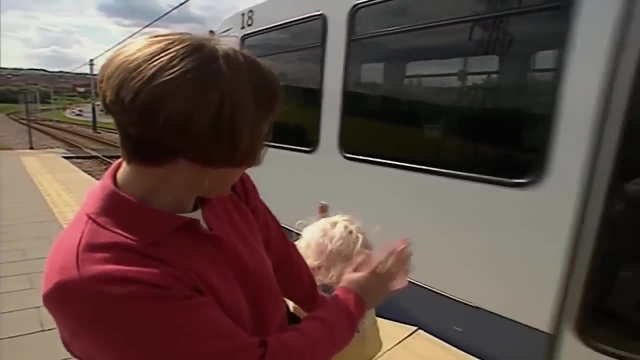 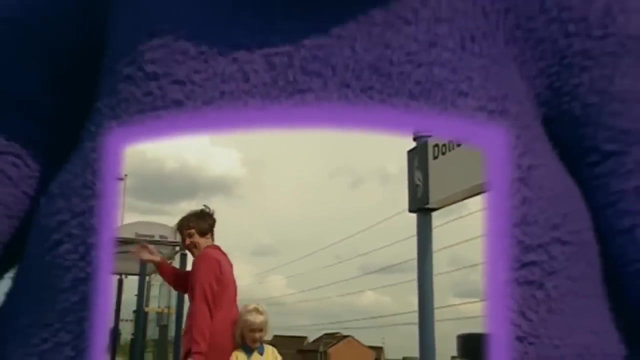 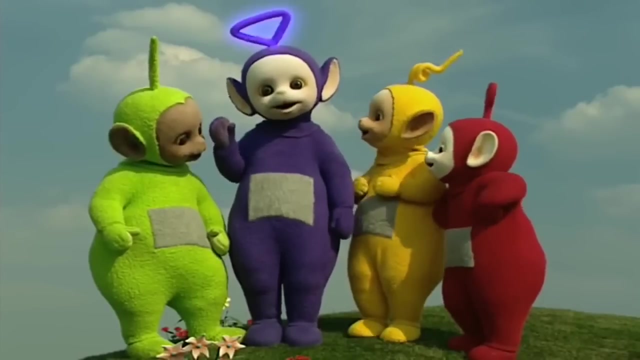 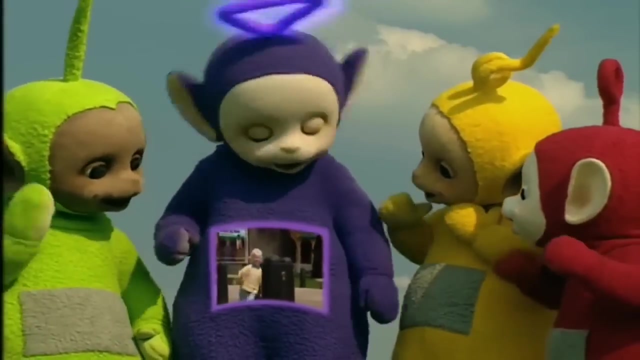 MUSIC FADES. Here's the biller to get off. I'm going to get off. Bye, Daddy, Bye, Bye, Bye-bye Daddy, Bye, Bye, Bye, Bye, Aw, Again, Again, Again, Uh-oh. 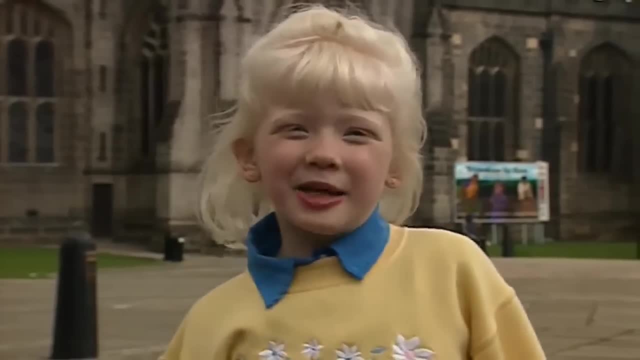 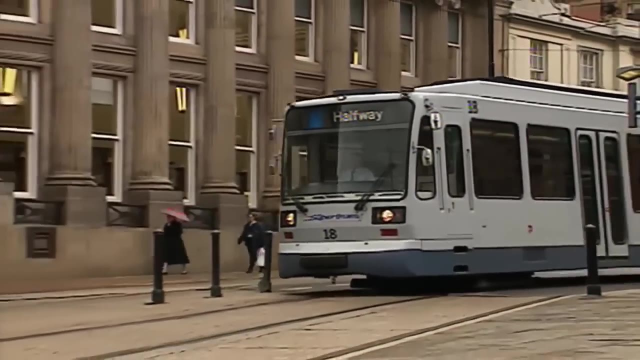 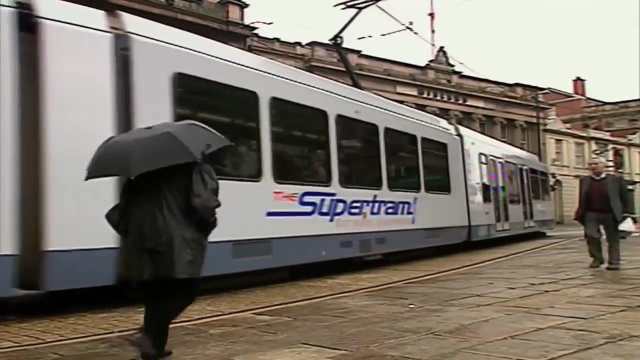 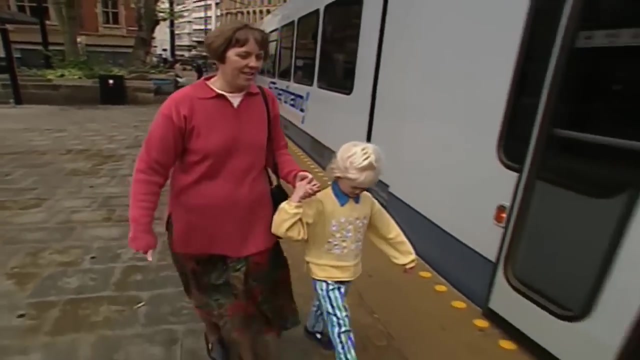 Hello. Hi, my name is Becky. Come and see the trams. We're going on the tram. I'm getting on the tram with Mummy. I'm getting on the tram with Mummy. I'm getting on the tram with Mummy. 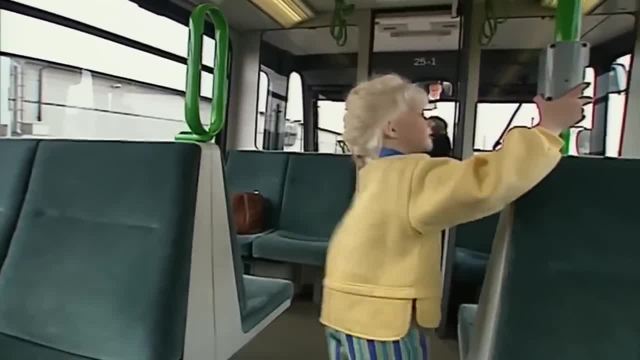 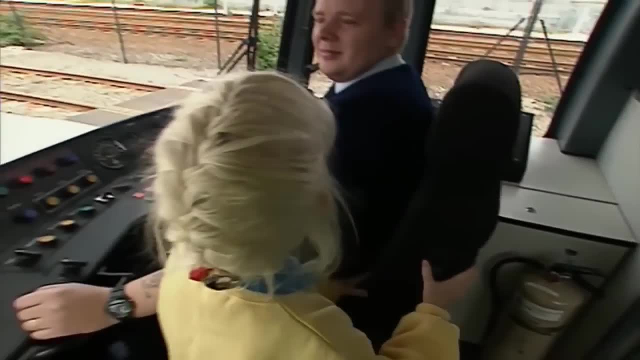 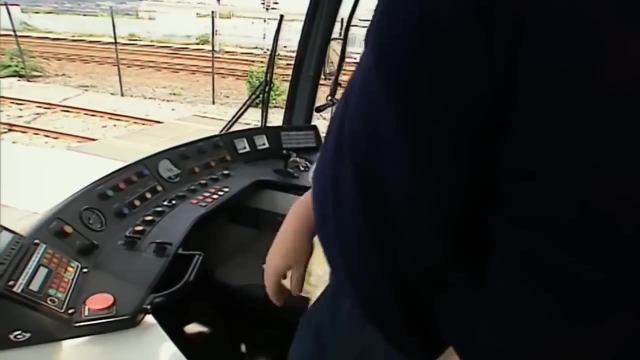 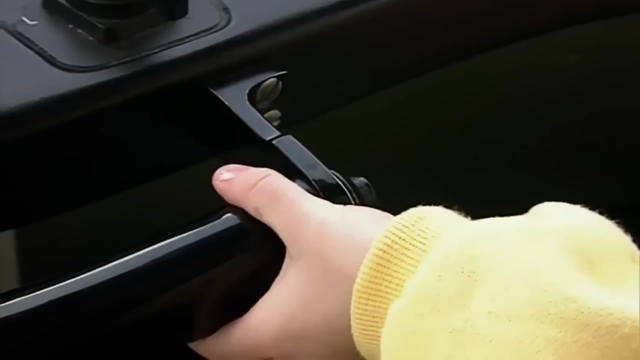 My Daddy's driving. This is where Daddy sits. This is where Daddy sits. Here's Daddy, Hello. Hello, Becky. Hello, Do you want to come and sit in my seat? Yes, Do you want to show me where the bell is? 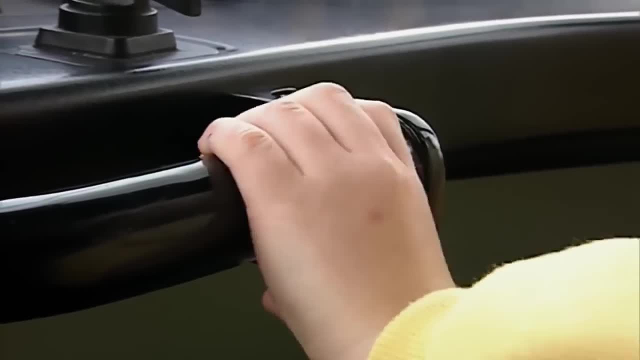 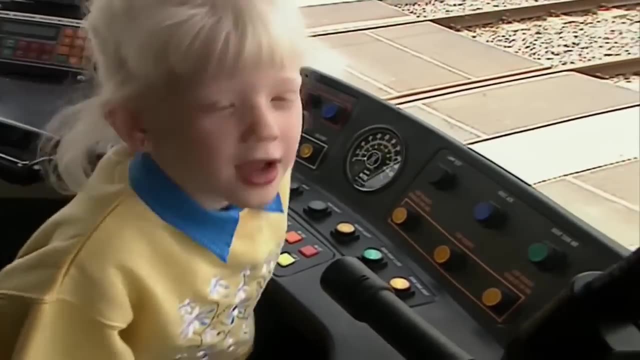 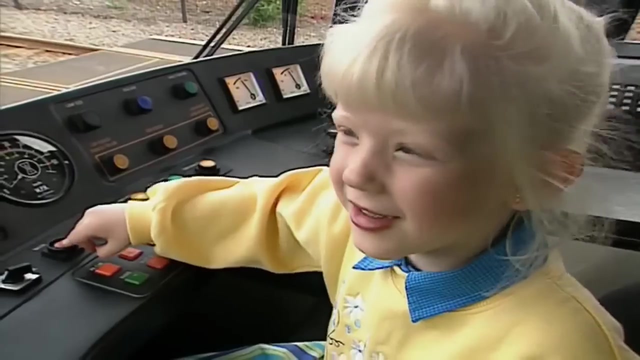 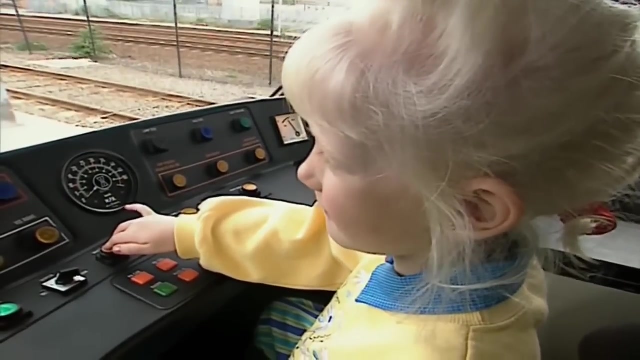 This is the bell, This is the horn. Next stop, the next way. There's the window washer. There's the window washer. The window washers are my favourite. The window washers are my favourite. The window washers are my favourite. 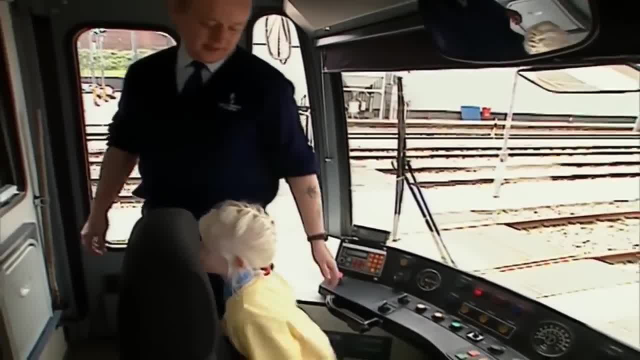 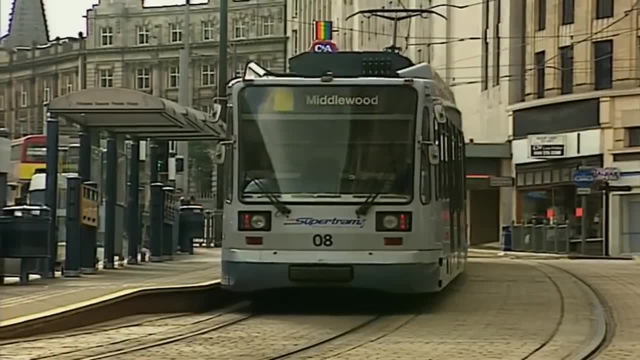 Right, come on, Bex, It's time to go. You don't sit with Mummy. You don't sit with Mummy. This is Mummy. Hello, We're off. We're off, We're going round the corner. 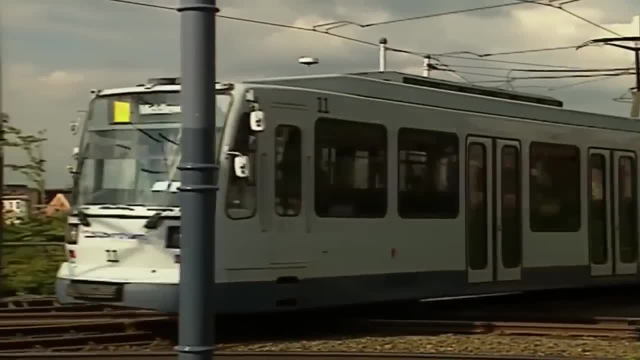 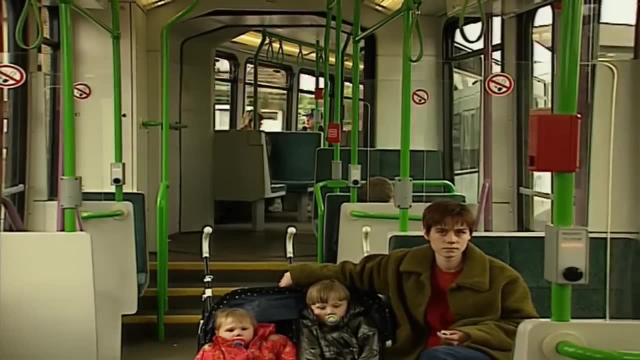 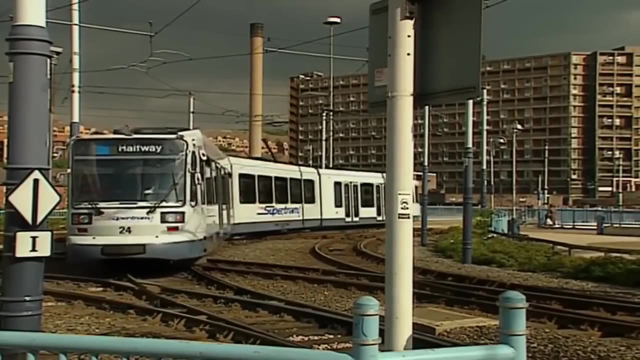 We're going round the corner. We're going round the corner. Trams are all bendy. Trams are all bendy. The tram's like a big snake. The tram's like a big snake. See how the tram goes round the corner. 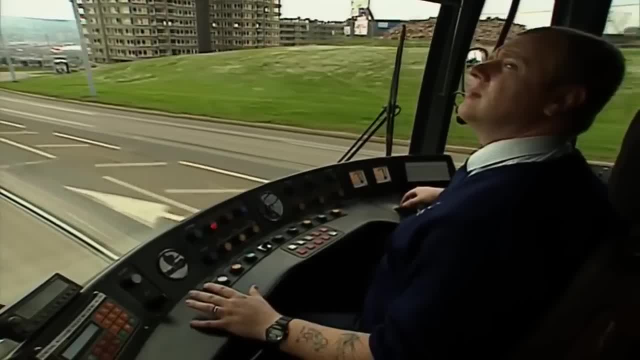 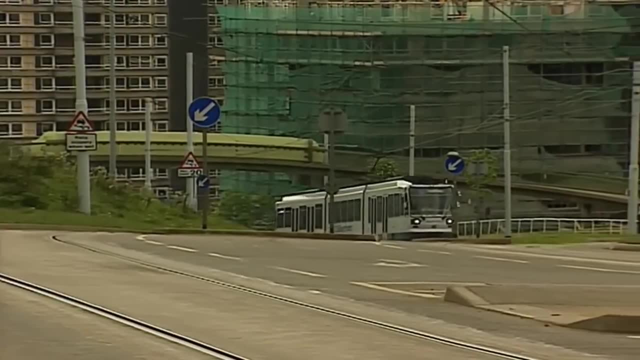 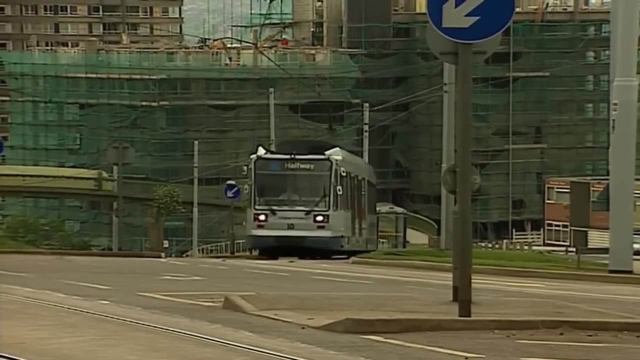 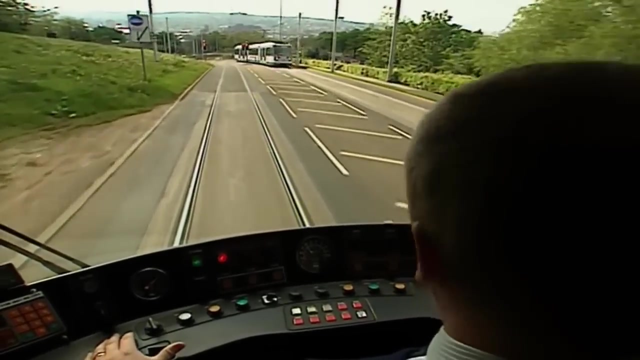 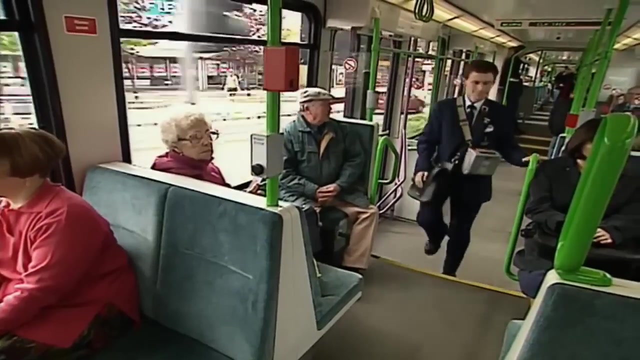 See how the tram goes round the corner. There's daddy driving. There's daddy driving. We're going up the hill. We're going up the hill. Daddy's got a good view. There's another tram. Look, here's the conductor. 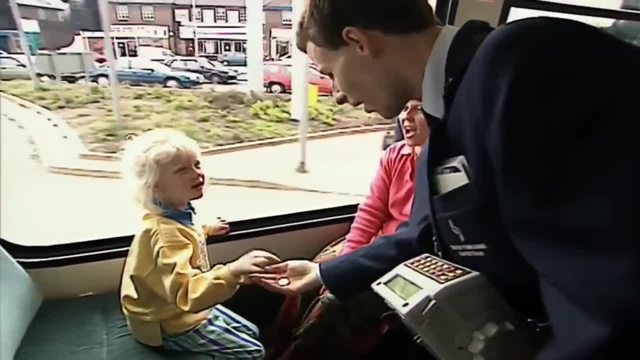 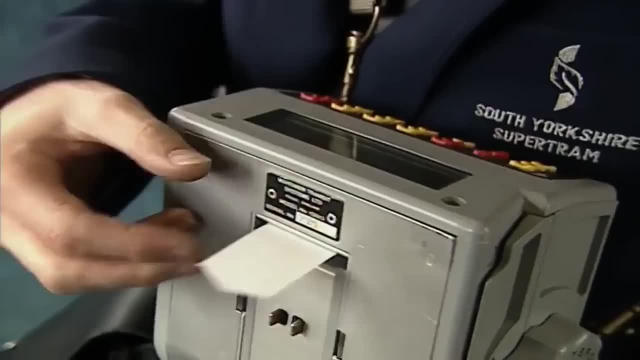 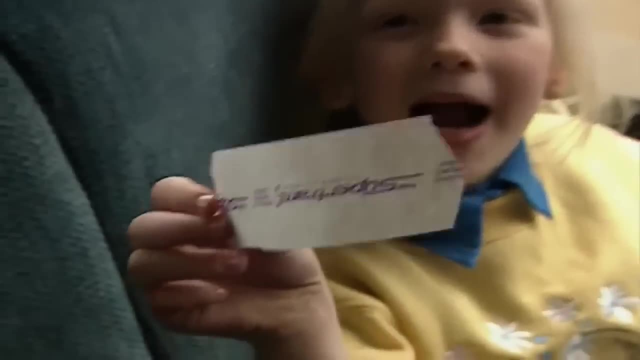 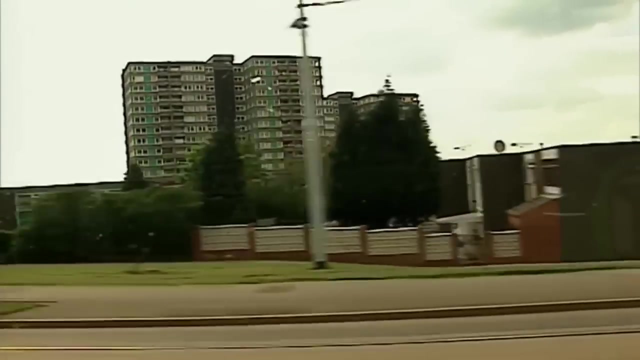 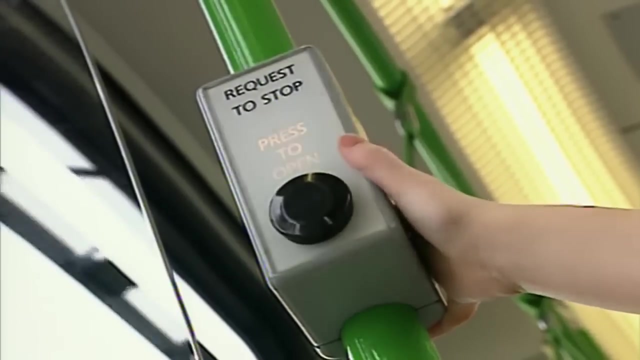 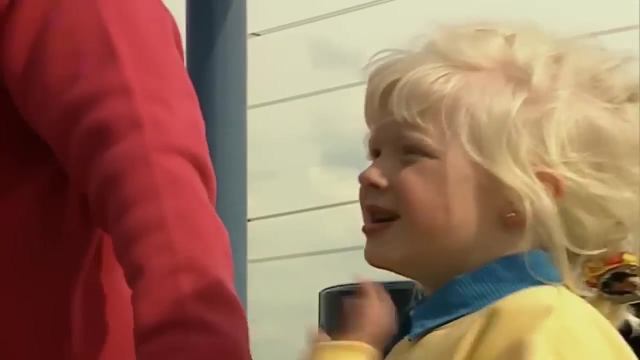 Hello, One and a half, please. Thanks, sir, I'll make a ticket, Thank you. Thank you, That's my ticket. Ding Ding Ding. Here's the billet to get off. Bye, Daddy, Bye. 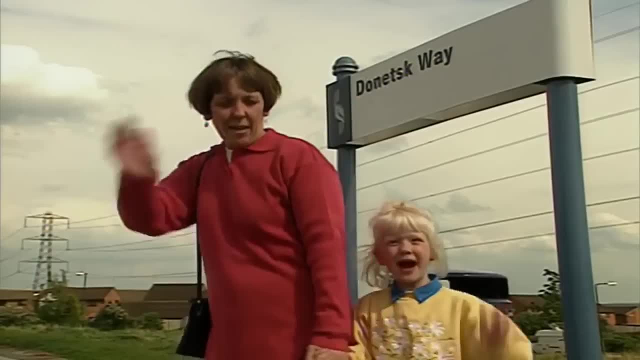 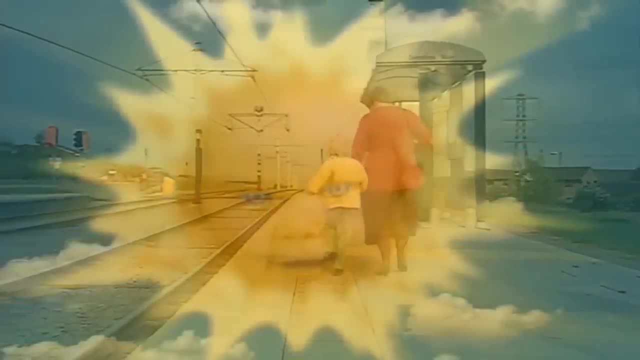 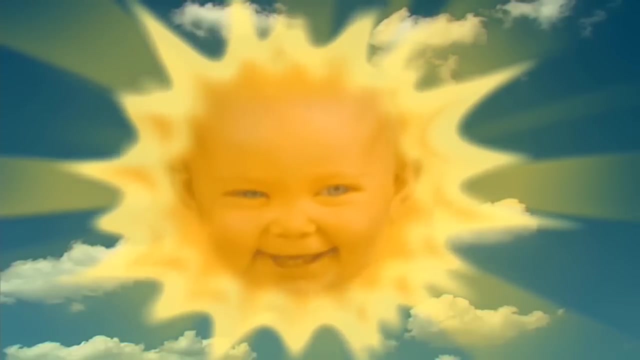 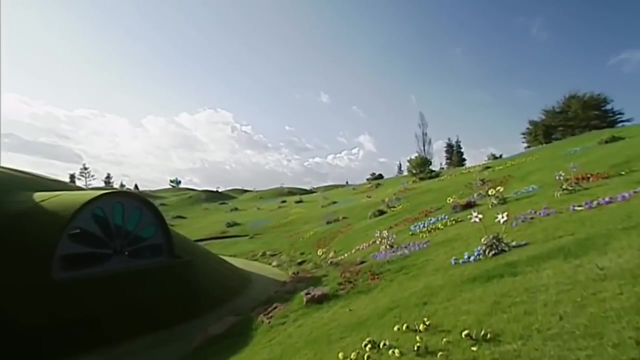 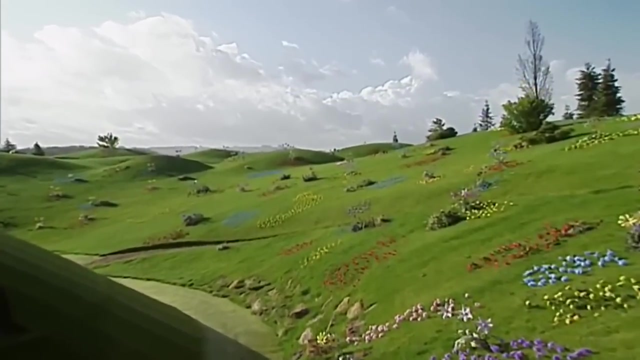 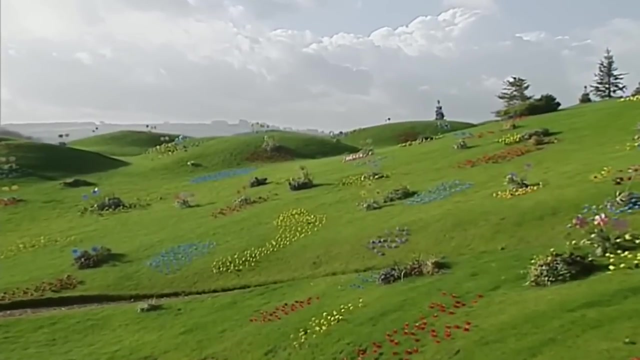 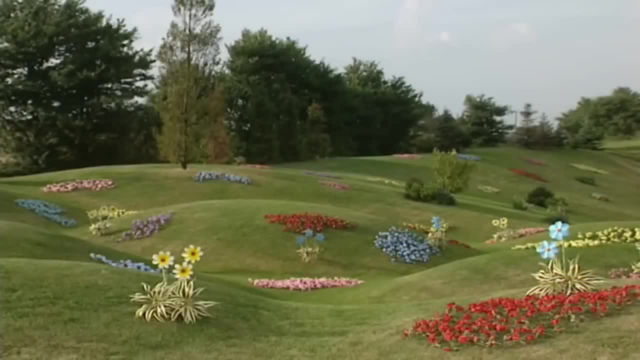 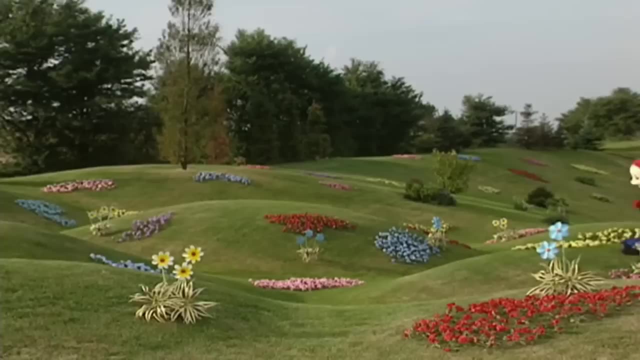 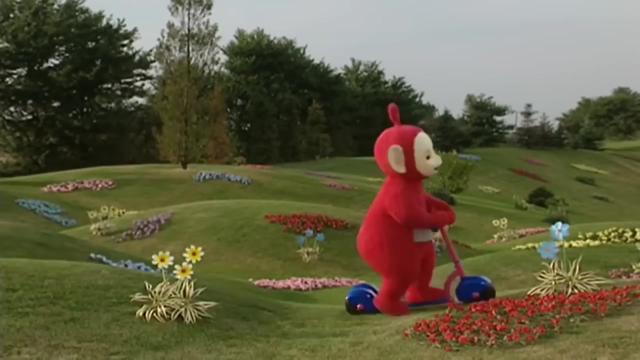 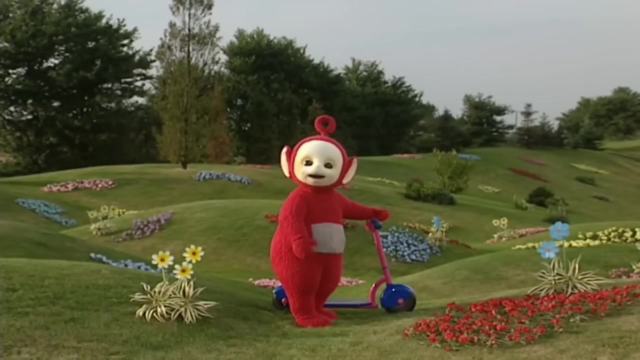 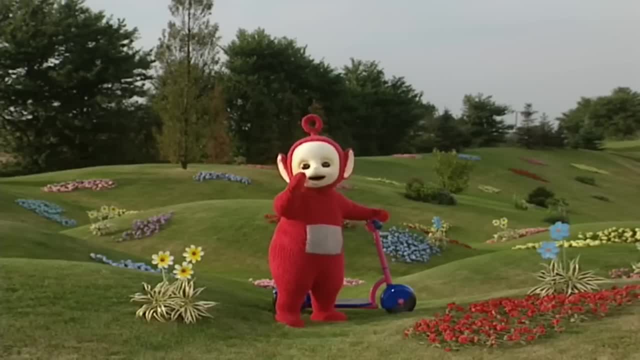 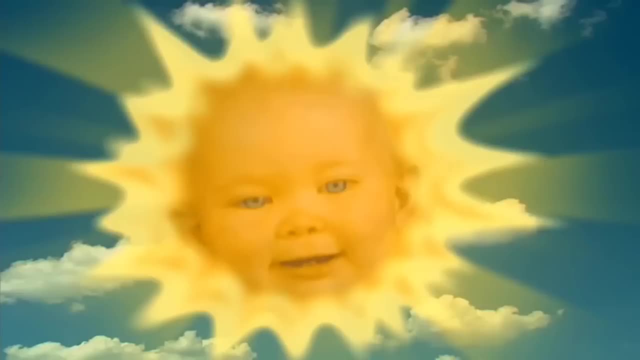 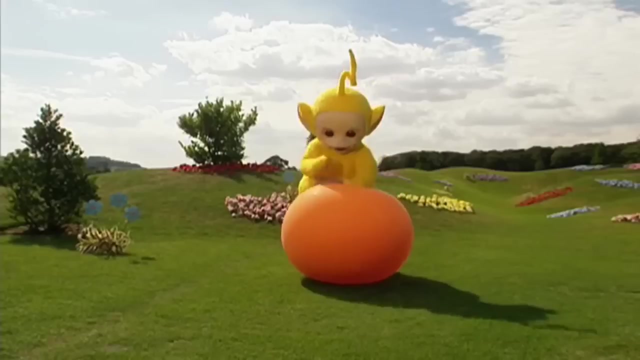 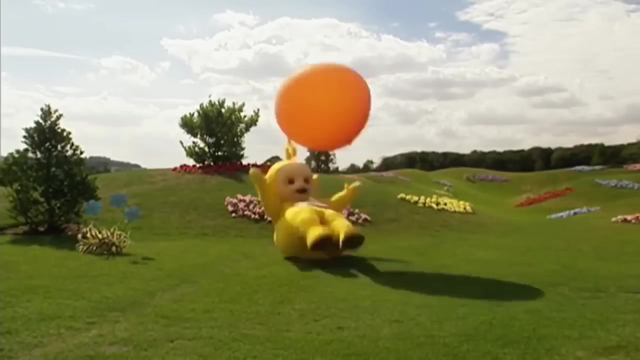 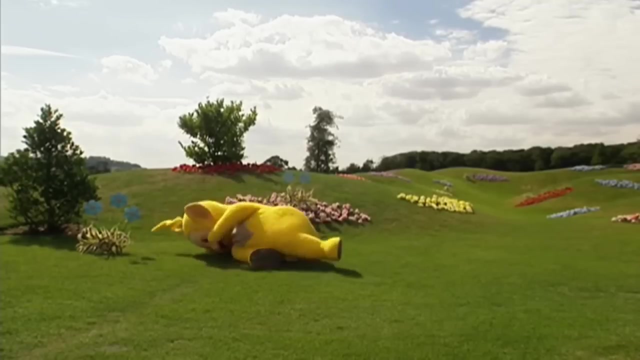 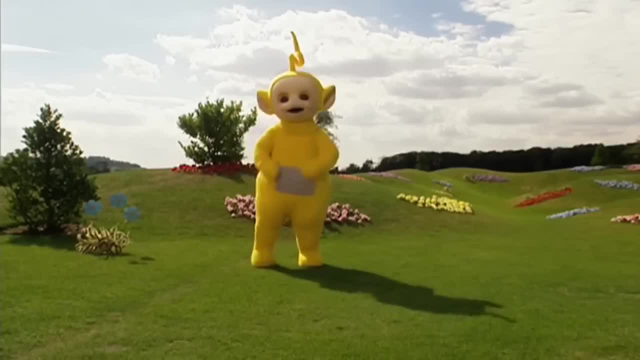 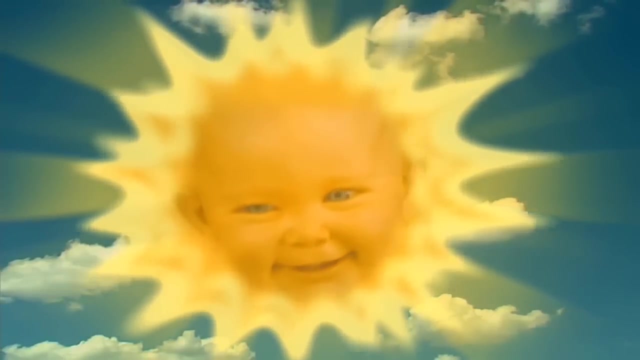 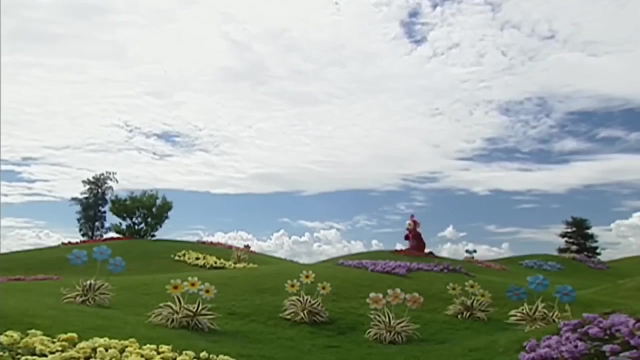 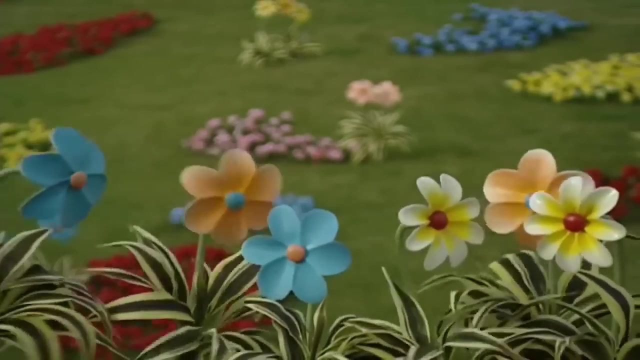 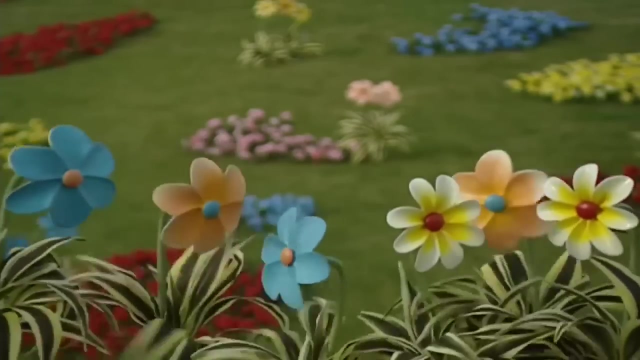 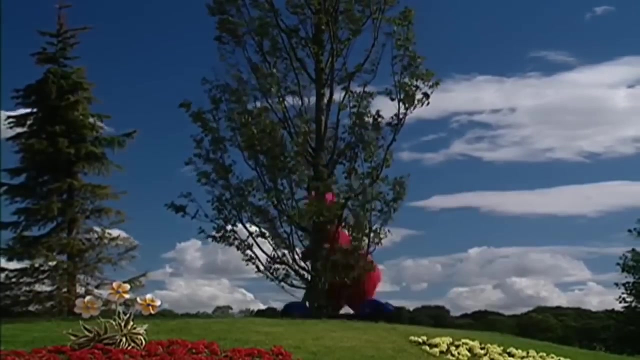 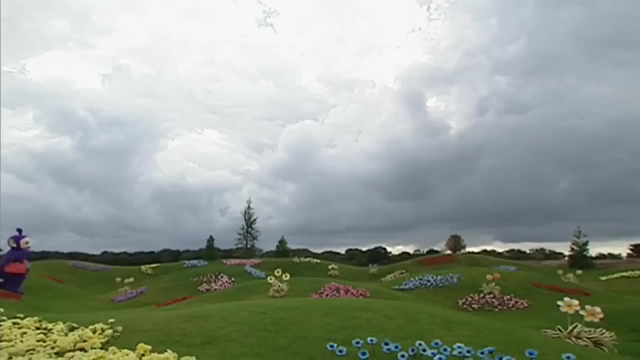 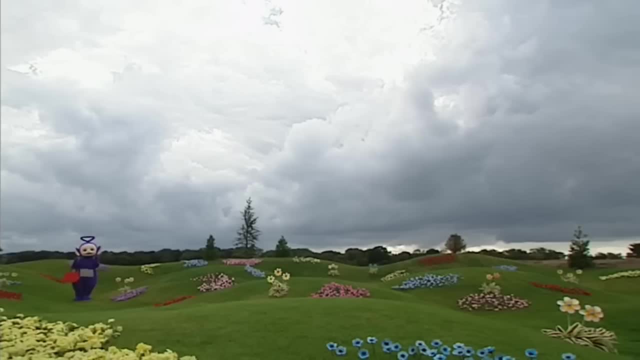 We're going to bed. Come on Poe, Come on Poe, Come on, Come on Poe, Poe, Poe, Come on, Come on Poe, You can go to bed. Puddle, puddle, puddle, puddle. 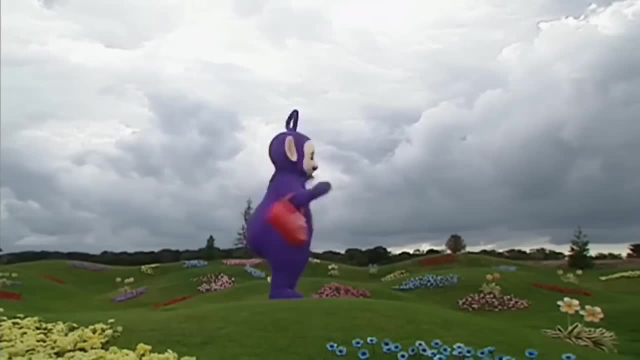 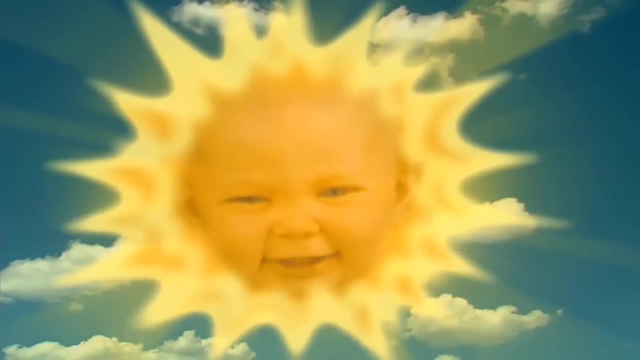 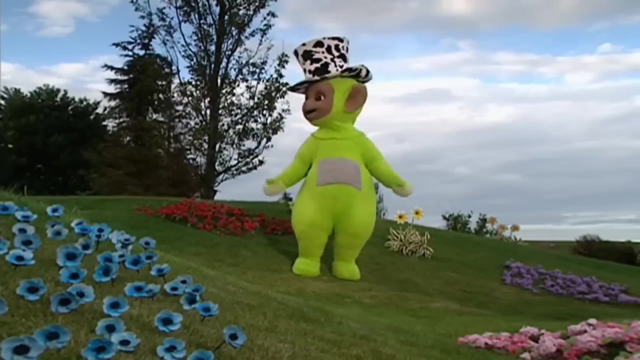 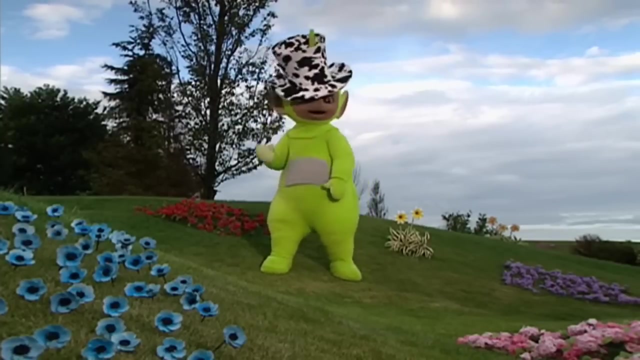 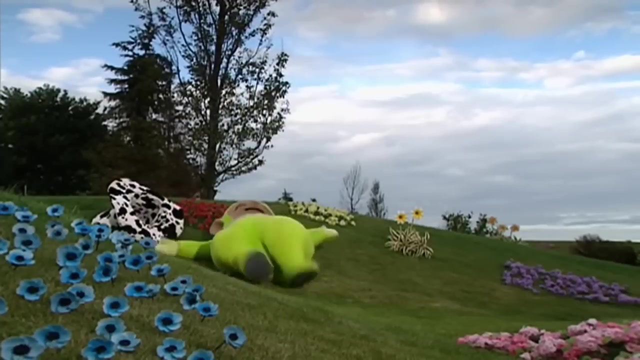 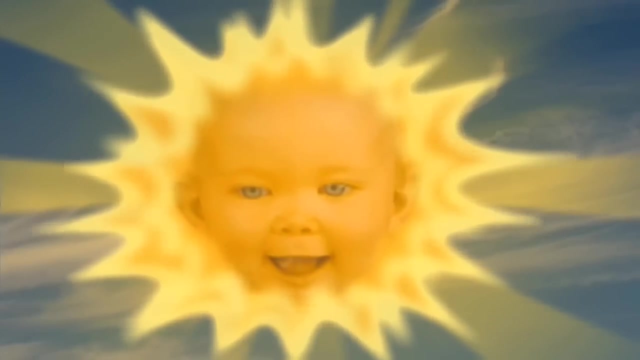 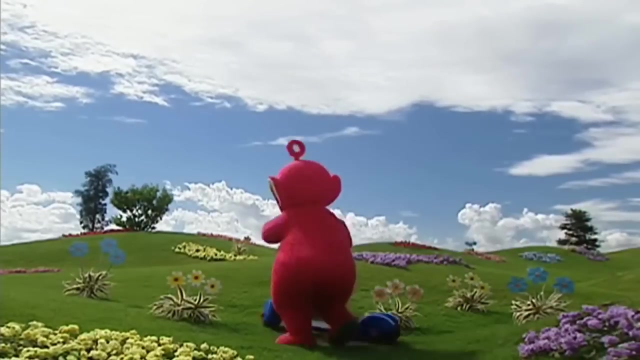 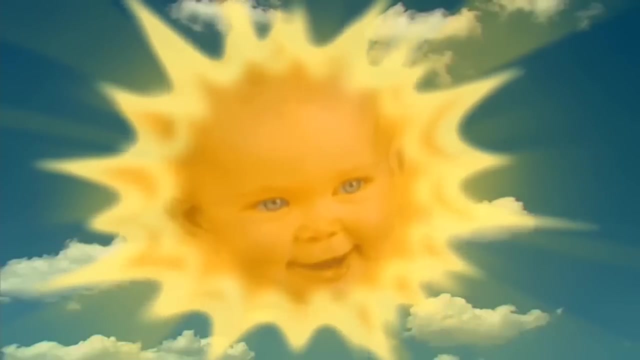 Too fast Po. And Gipsy was dancing in his hat. Too fast, Po, Too fast, Po, Too fast, Po. But it's much too fast, So dangerous, Awful. But then Po fell off her scooter. 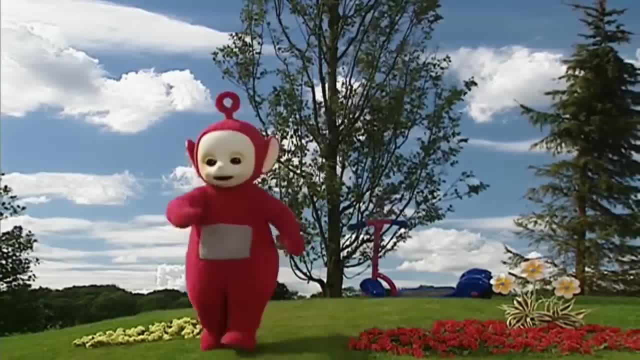 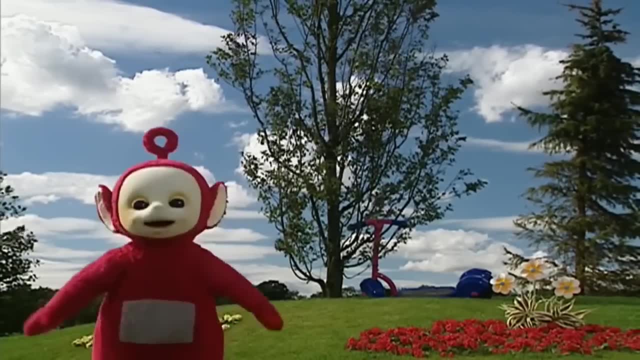 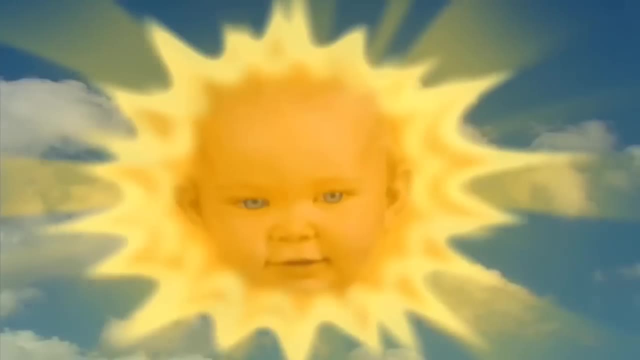 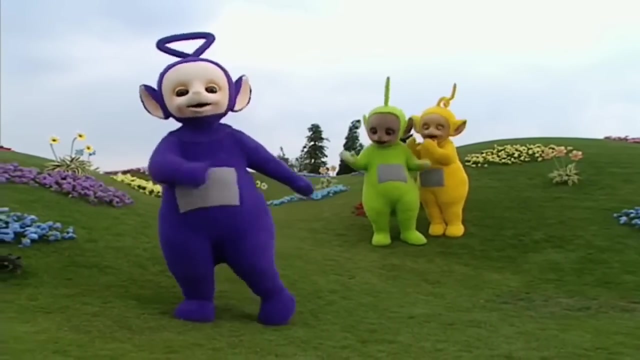 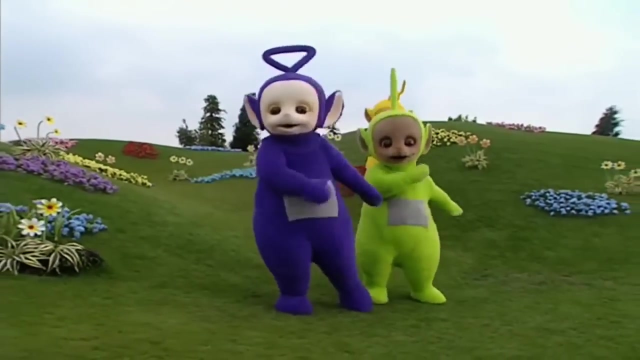 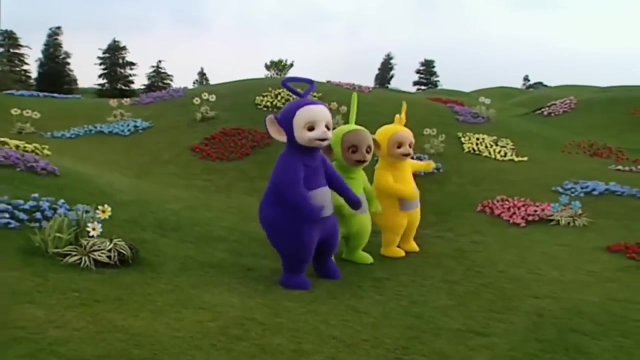 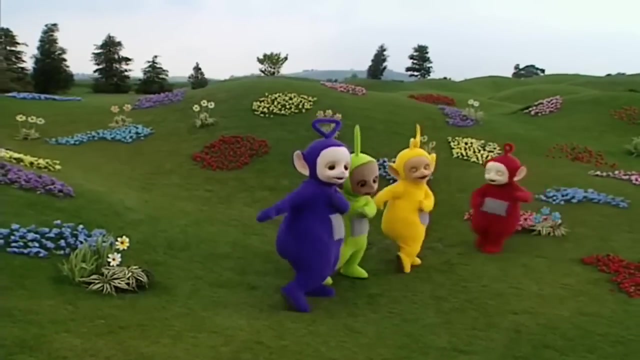 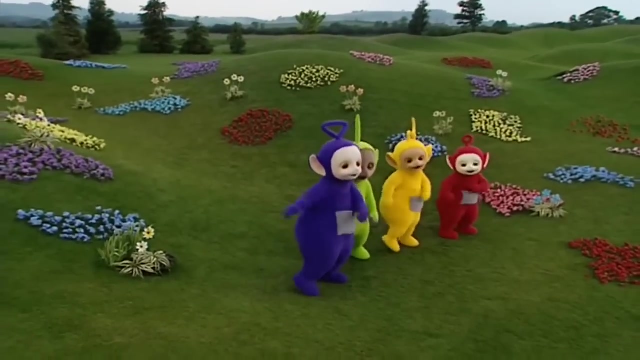 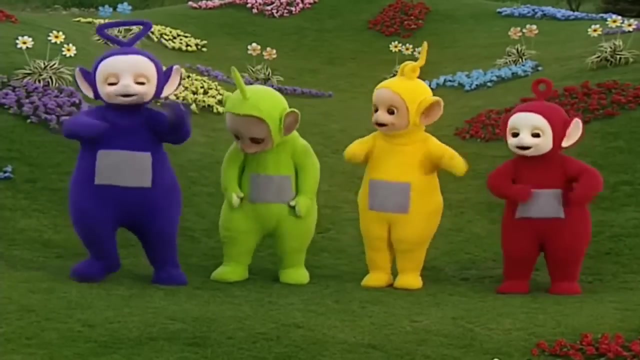 Too fast Po Too fast Po Too fast Po Sossaaden. too fast Too fast Po Too fast. Po Too fast Po Too slow. Too slow Po Too stop Poonaarios. 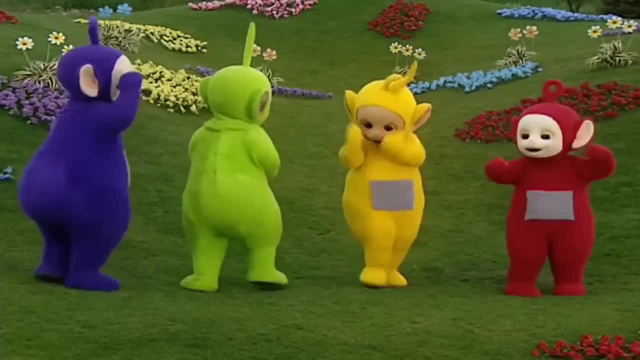 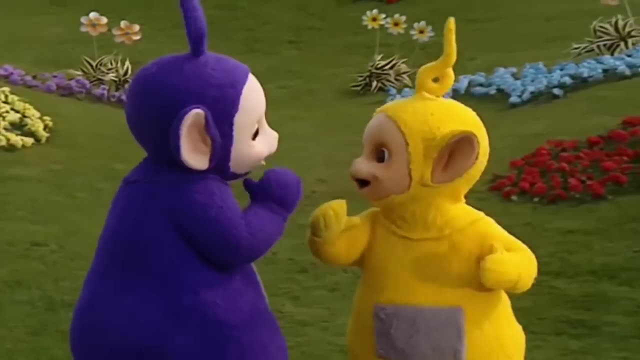 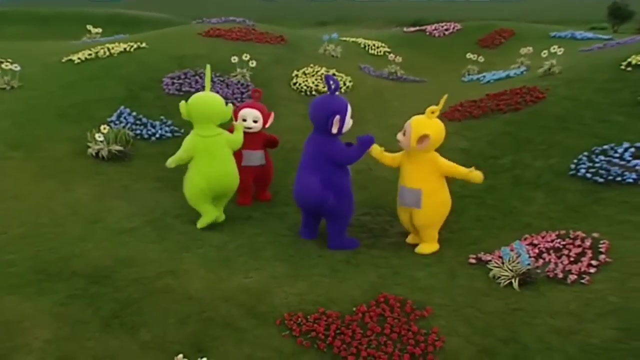 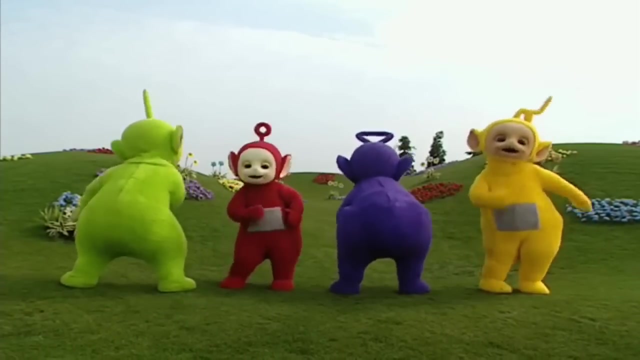 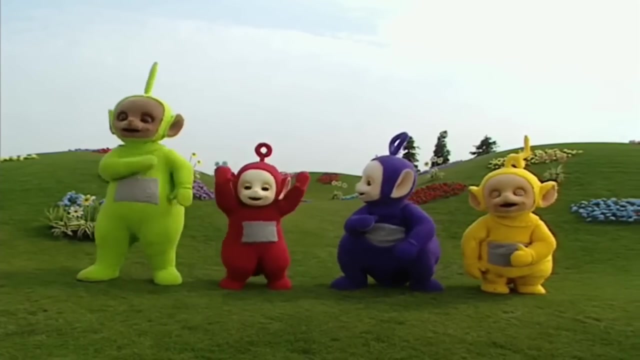 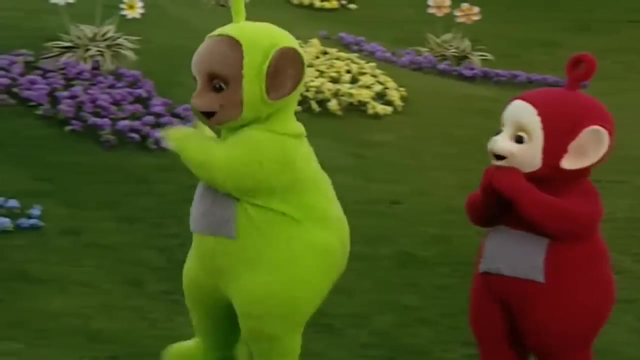 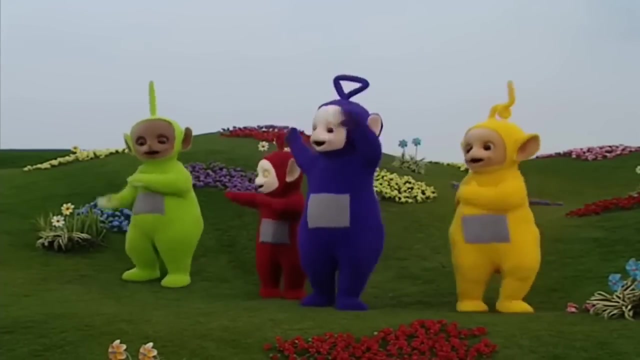 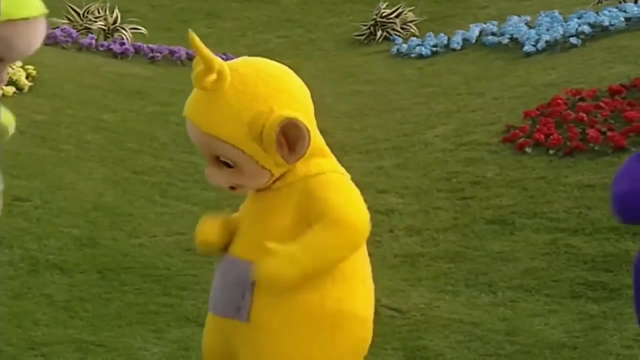 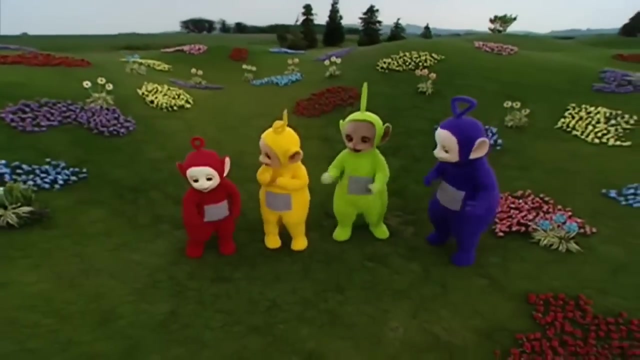 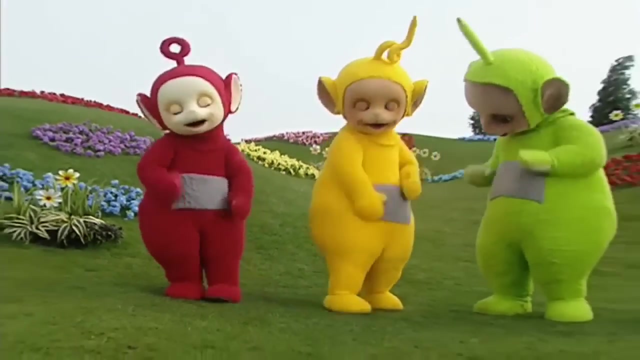 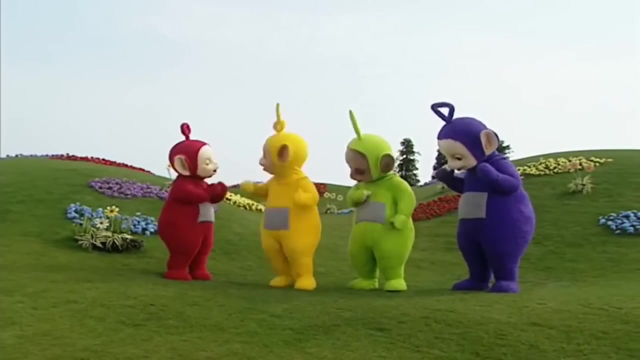 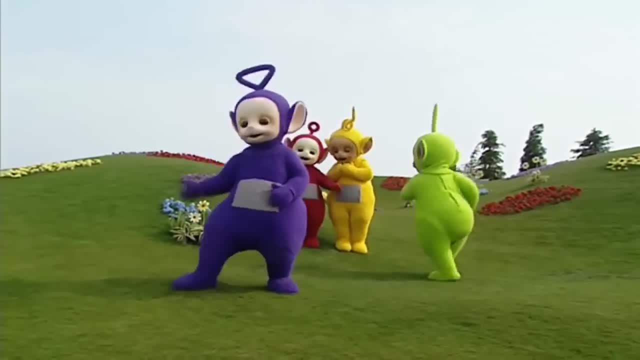 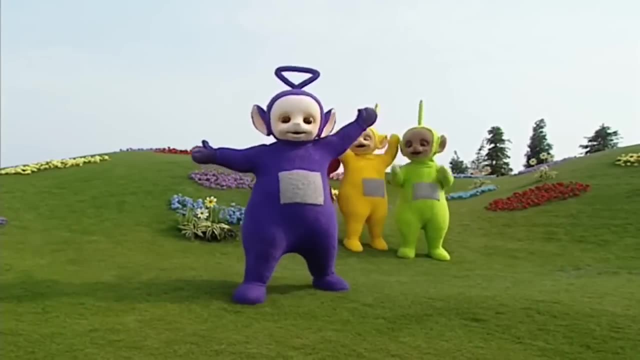 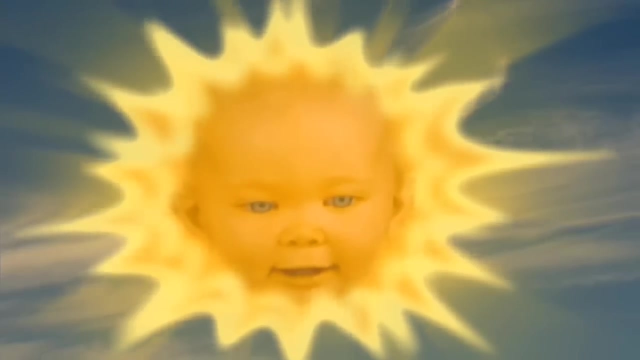 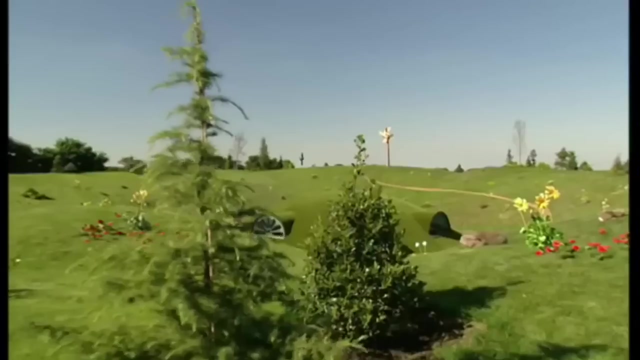 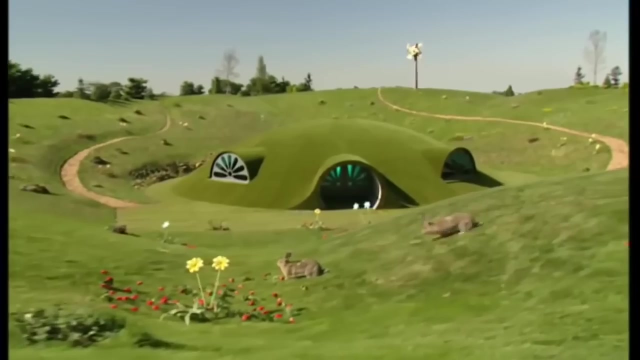 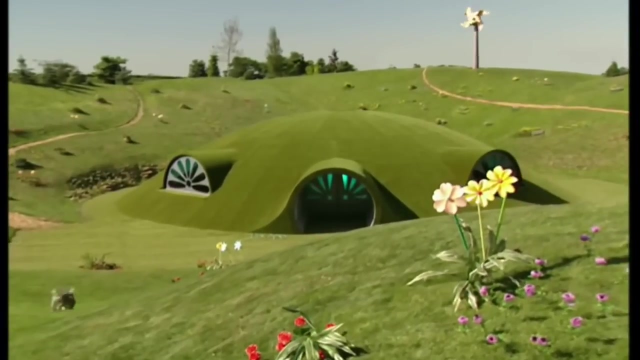 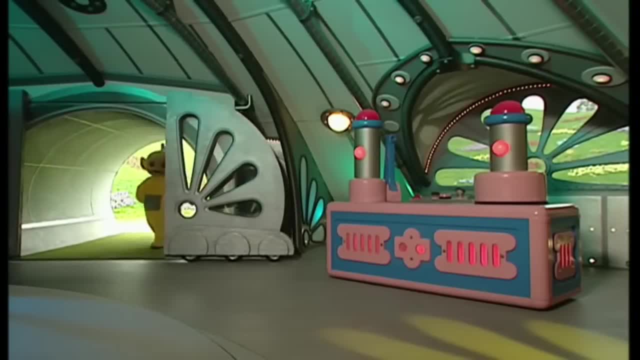 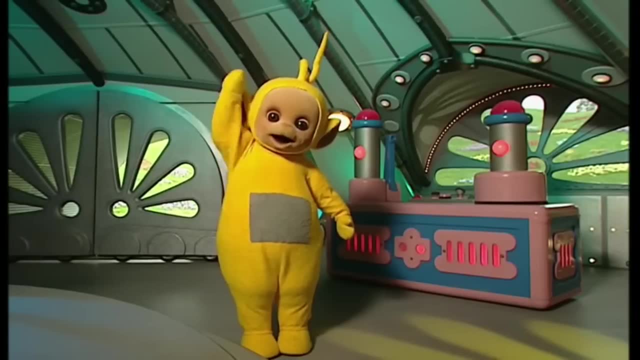 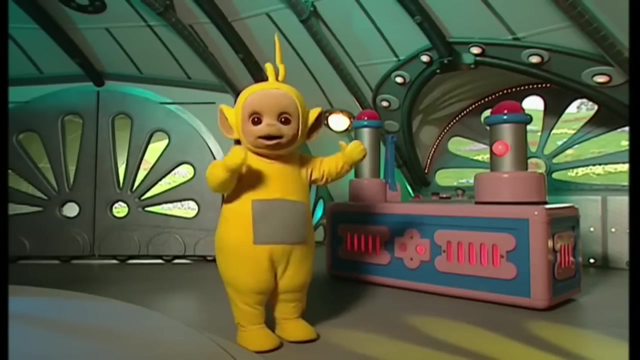 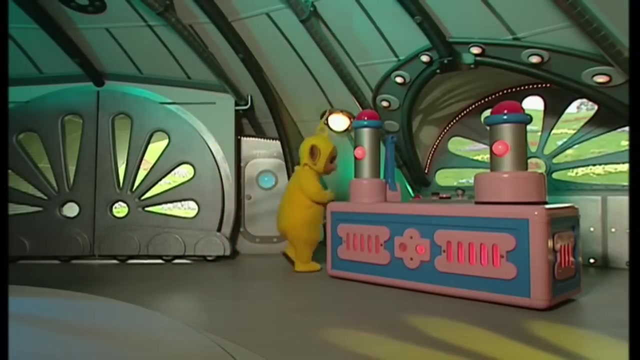 La-la-la-la-la-la-la-la-la-la-la-la-la-la-la-la-la-la-la-la-la-la-la-la-la-la-la-la-la-la-la-la-la-la-la-la-la-la-la-la-la-la-la-la-la-la-la-la-la-la-la-la-la-la-la-la-la-la-la-la-la-la-la-la-la-la-la-la-la-la-la-la-la-la-la-la-la-la-la-la-la-la-la-la-la-la-la-la-la-la-la-la-la-la-la-la-la-la-la-la-la-la-la-la-la-la-la-la-la-la-la-la. 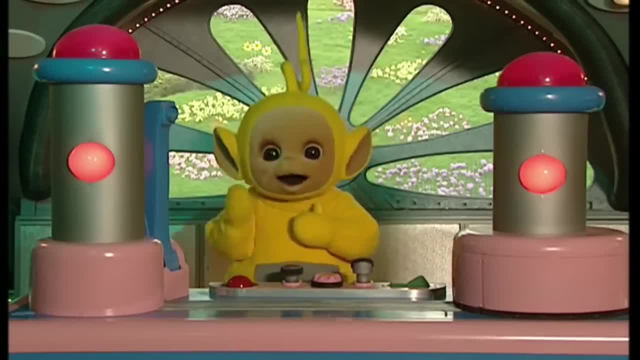 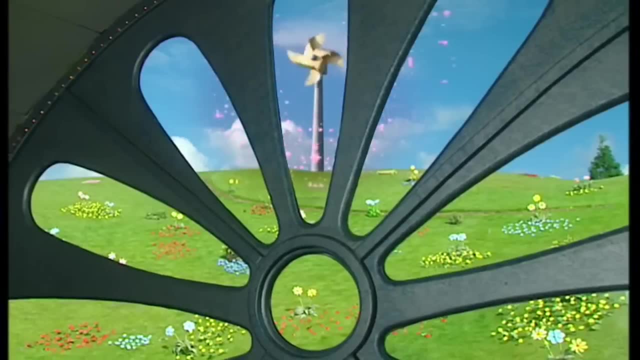 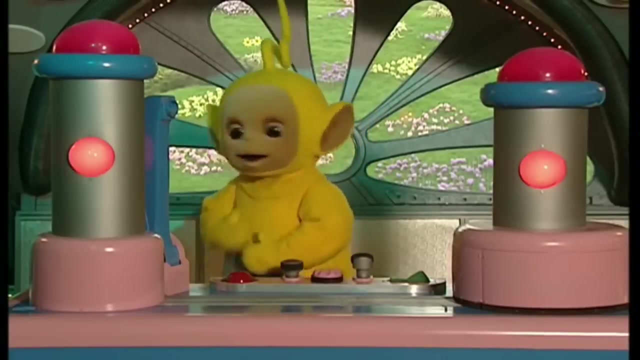 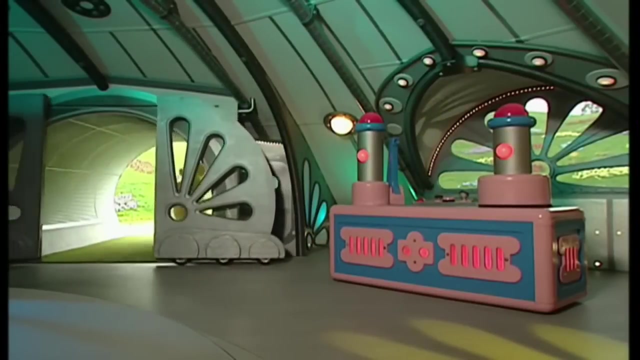 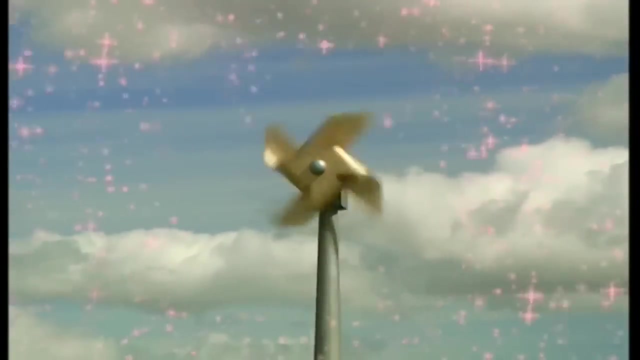 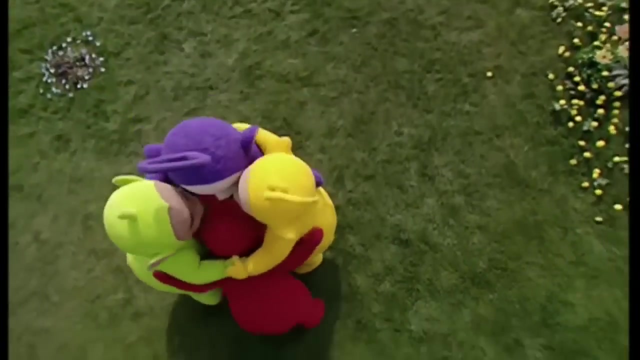 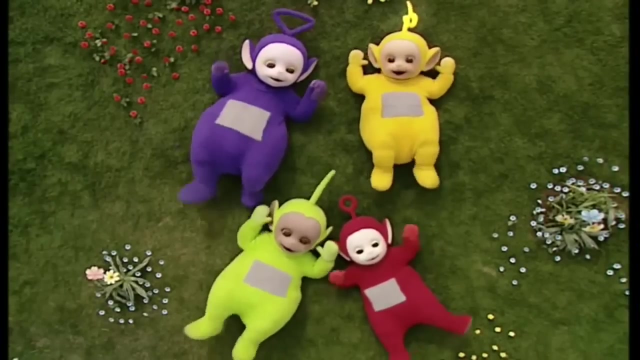 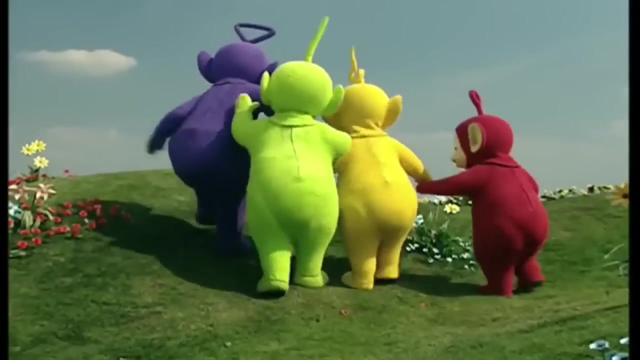 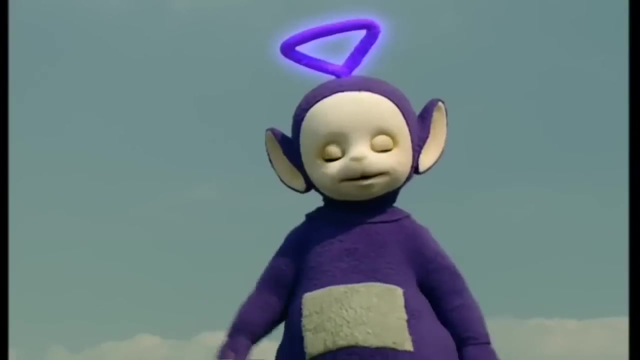 Ha ha ha ha. Pfft Test that test that Ha ha ha ha-ha-ha-ha-ha-ha-ha-ha-ha-ha-ha-ha-ha-ha-ha-ha-ha-ha-ha-ha-ha-ha-ha-ha-ha-ha-ha-ha-ha-ha-ha-ha-ha-ha-ha-ha-ha-ha-ha-ha-ha-ha-ha-ha-ha-ha-ha-ha-ha-ha-ha-ha-ha-ha-ha-ha-ha-ha-ha-ha-ha-ha-ha-ha-ha-ha-ha-ha-ha-ha-ha-ha-ha-ha-ha-ha-ha-ha-ha-ha-ha-ha-ha-ha-ha-ha-ha-ha-ha-ha-ha-ha-ha-ha-ha-ha-ha-ha-ha-ha-ha-ha-ha-ha-ha-ha-ha-ha. 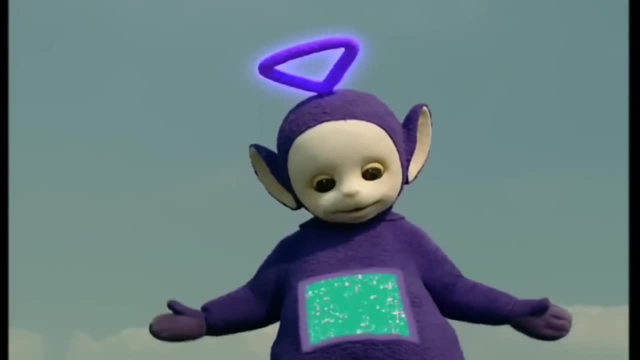 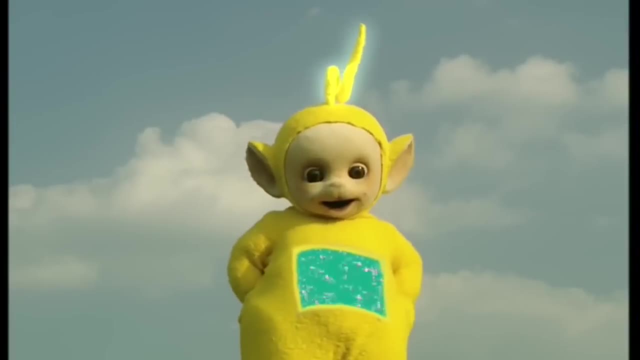 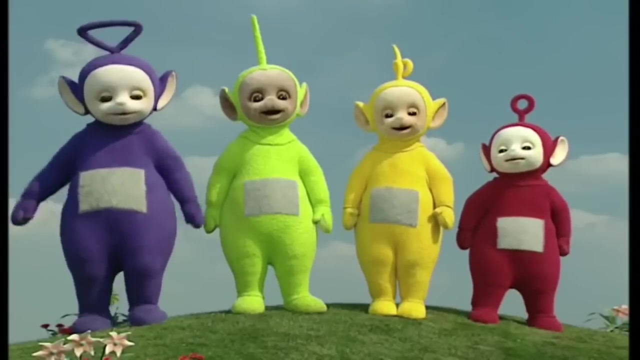 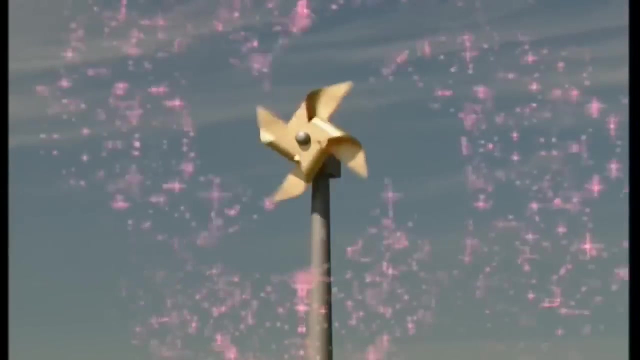 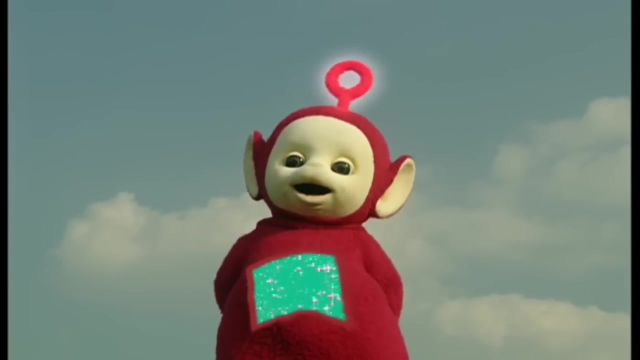 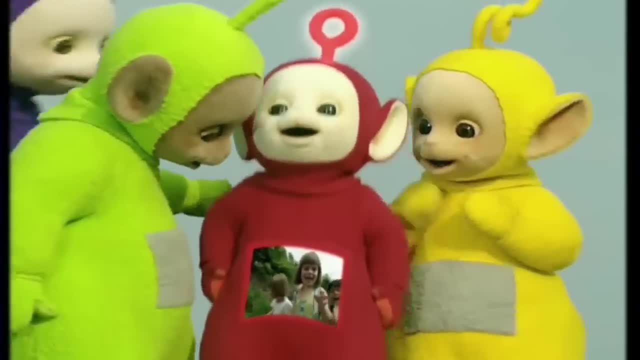 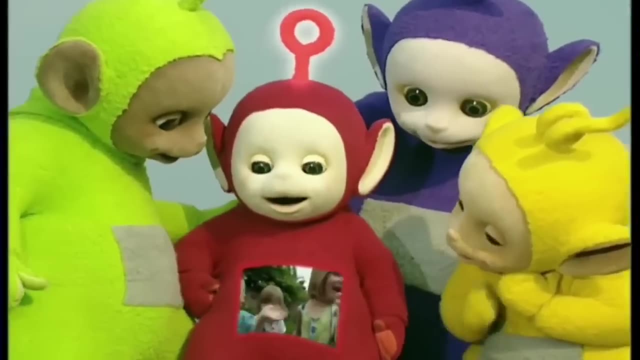 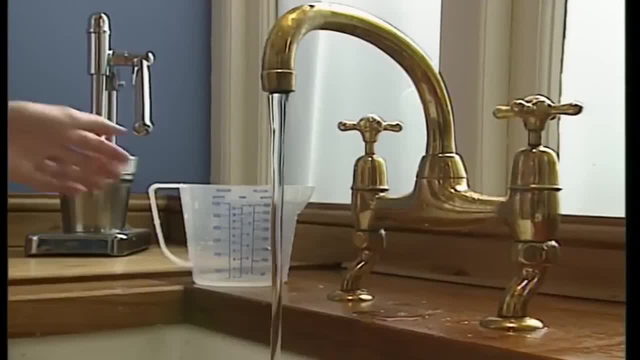 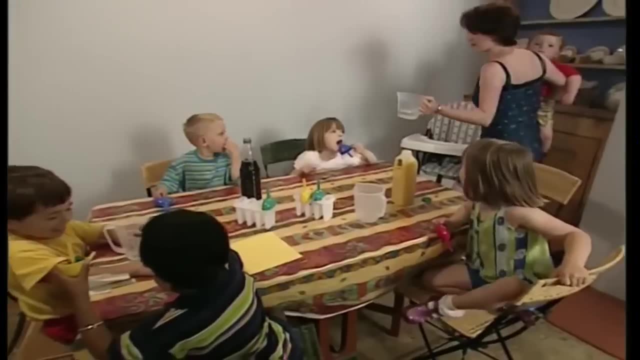 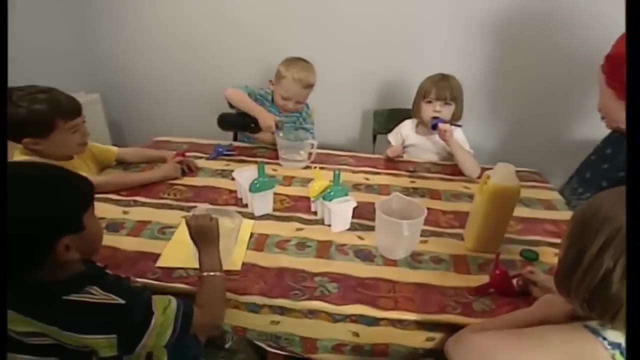 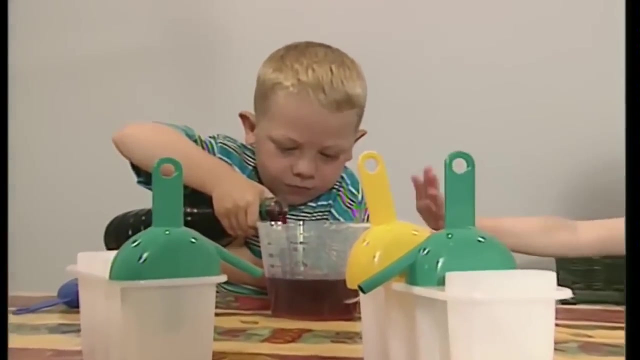 oh, oh, oh, oh, oh, oh oh, We're going to make ice lollies. Come and see You're doing Very carefully, Kyle, Is that okay? Then we put in some blackcurrants. 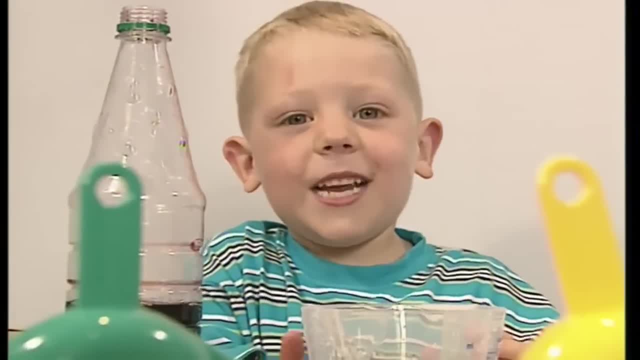 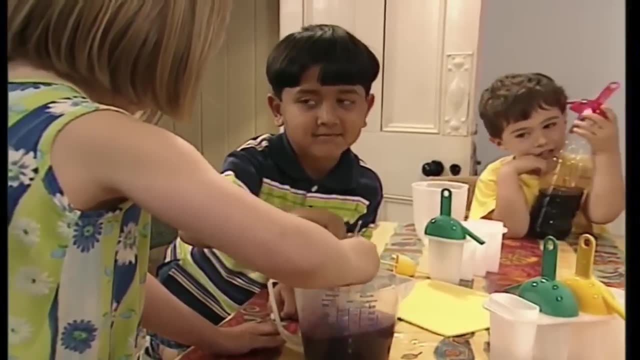 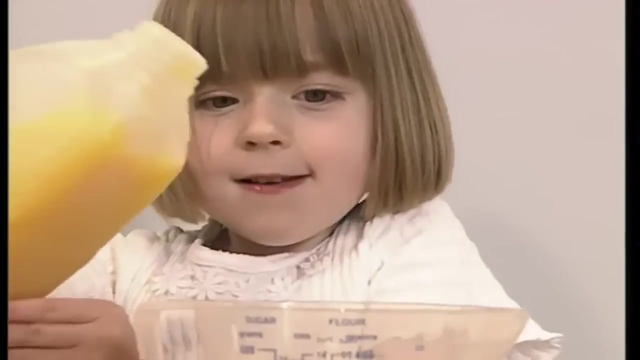 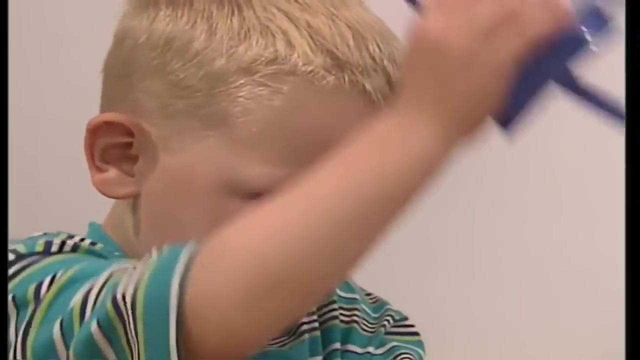 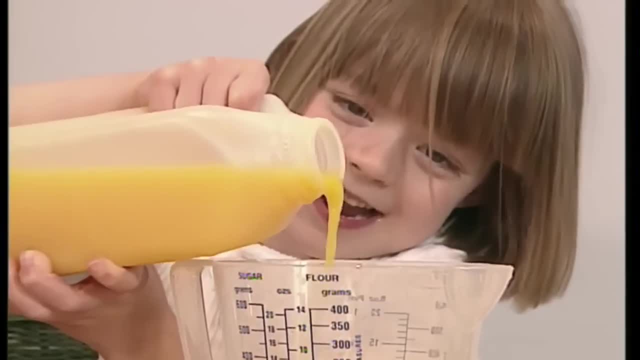 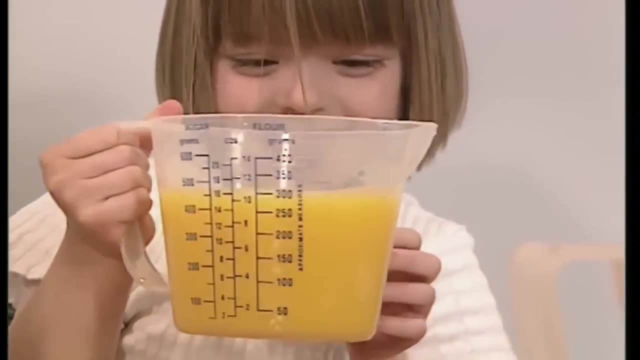 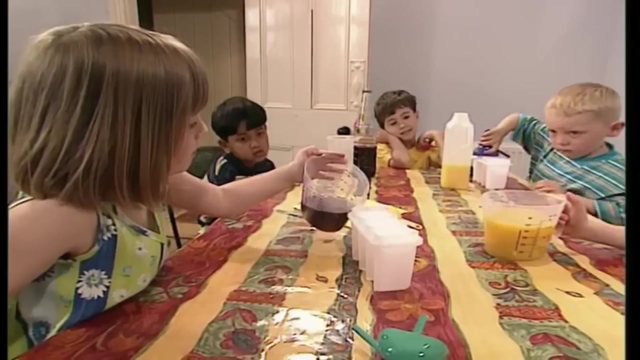 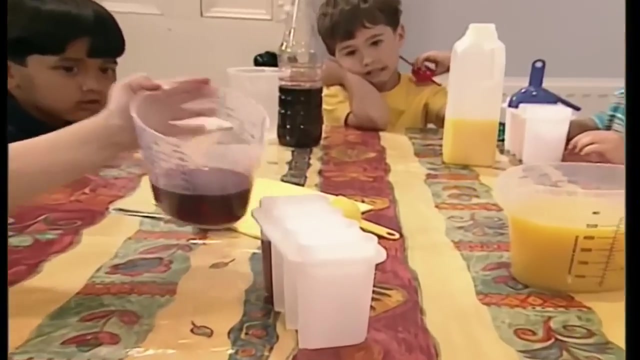 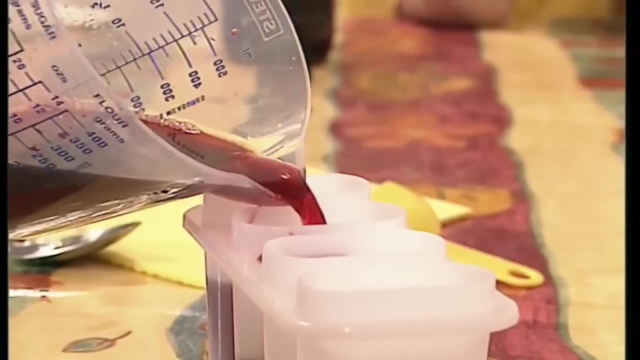 Enough, That's enough, That's enough. Then it's ready to pour into the little pots. Stop, Stop, Stop, Stop. What What's that? Is that enough? Yes, Oops, Ah, Stop, Stop, Stop. 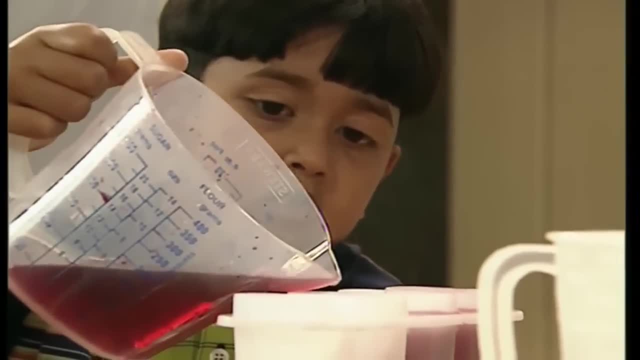 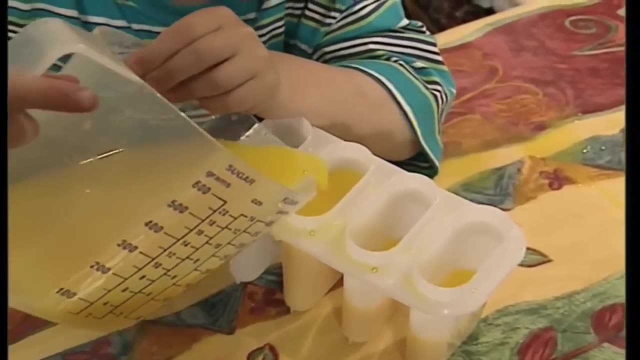 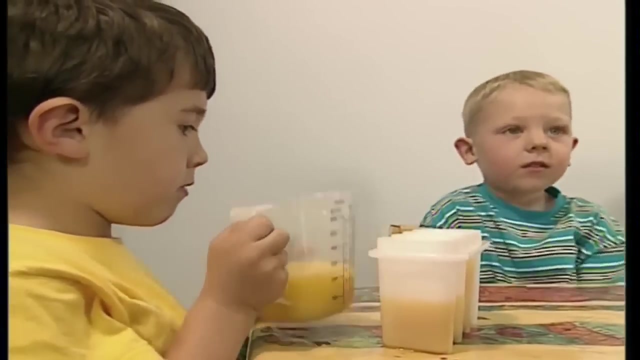 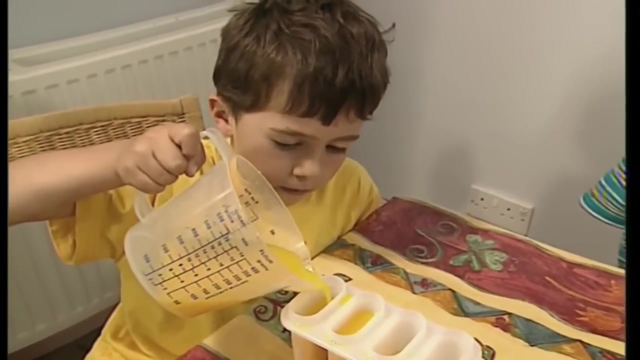 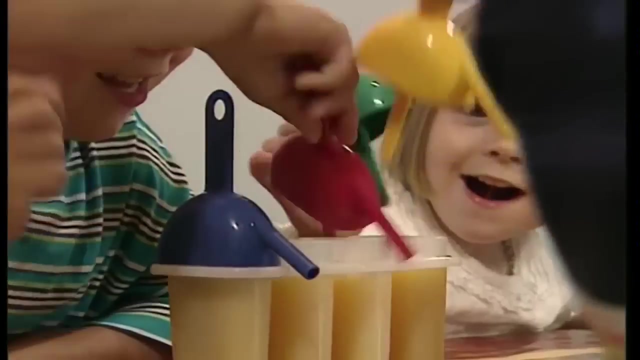 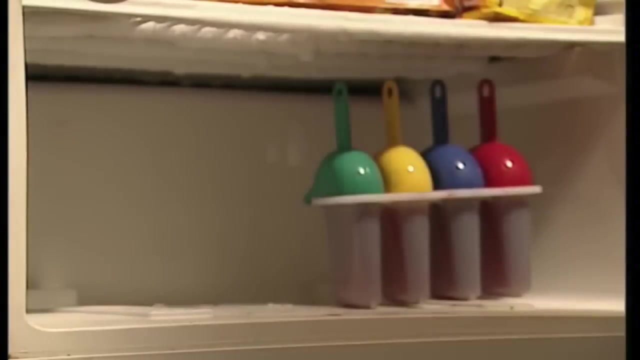 Stop, Stop, Stop, Stop. It's sharing And that's enough. That's enough. We're taking this in turns. You have to leave a space for it to grow. Stop. Let's put the sticks in Mummy's putting them in the freezer. 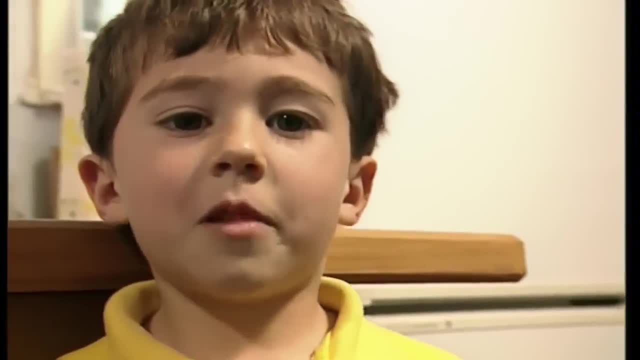 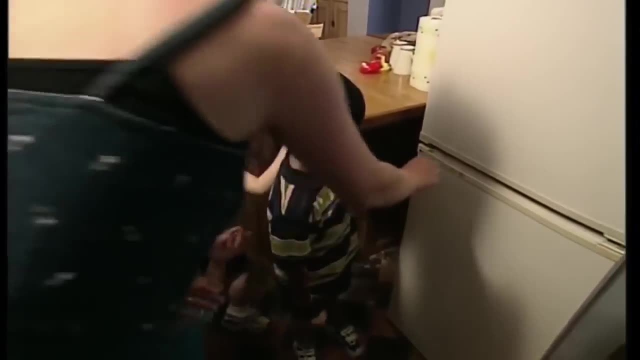 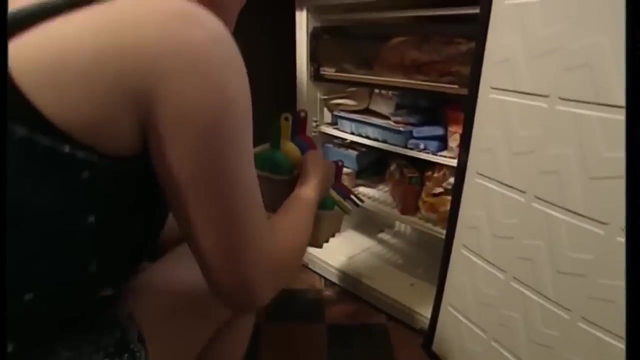 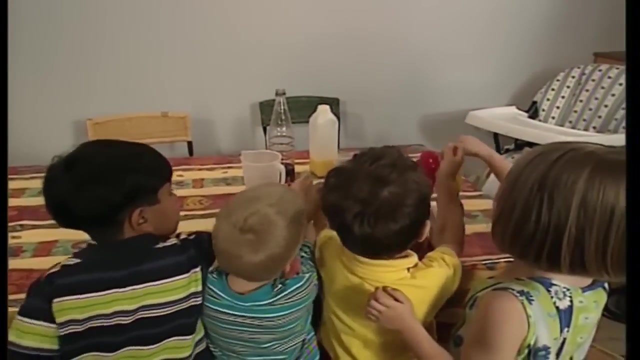 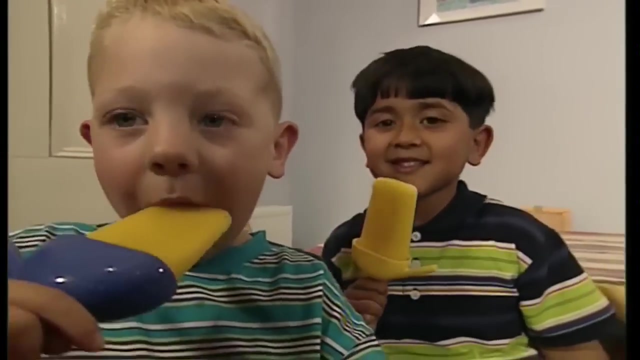 I hope they're not going to take too long to freeze. Hurry up ice lollies. They must be ready now They're ready, Come and see the ice lollies. Ice lollies at last. Come on. 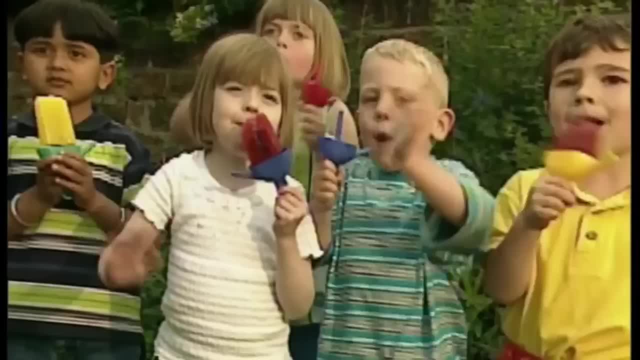 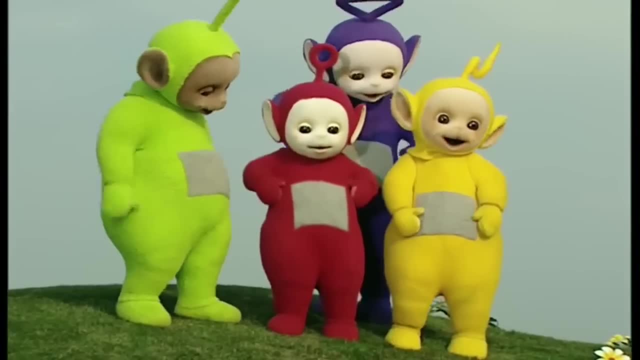 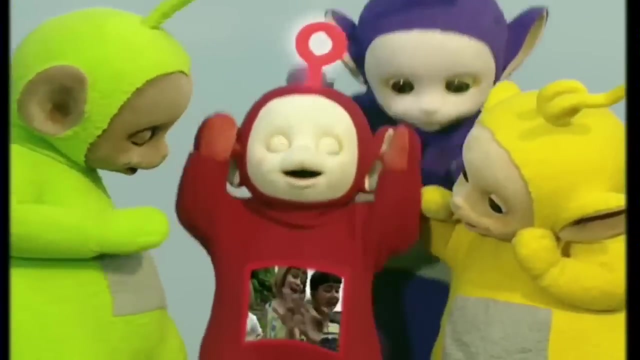 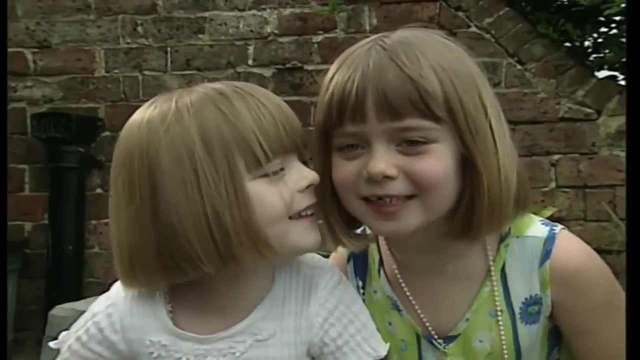 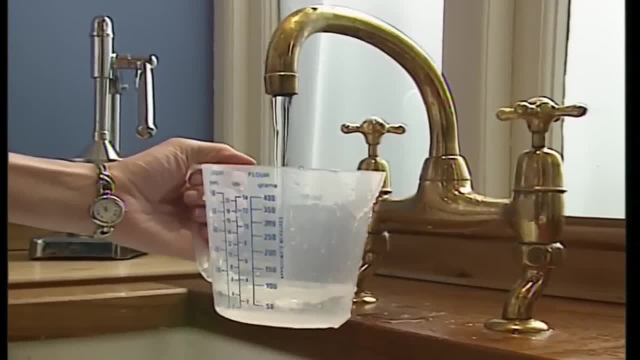 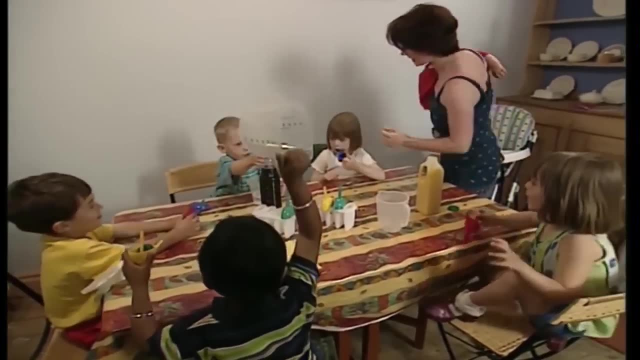 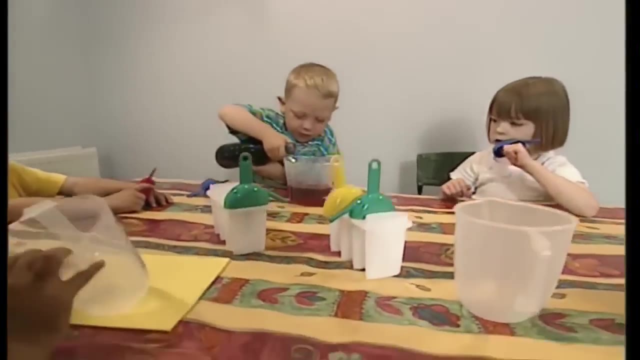 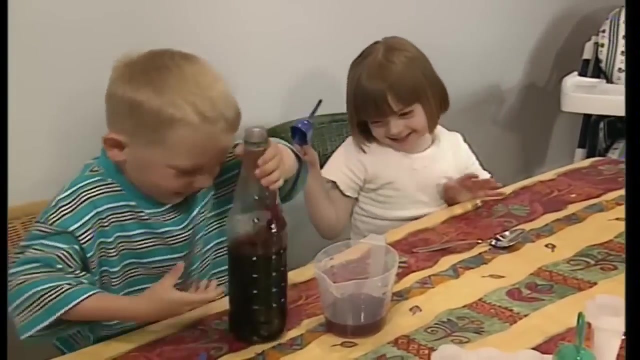 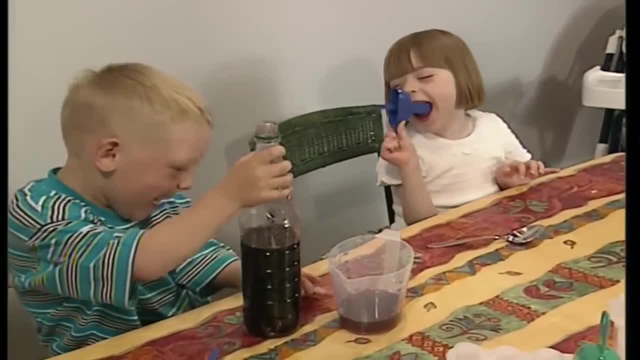 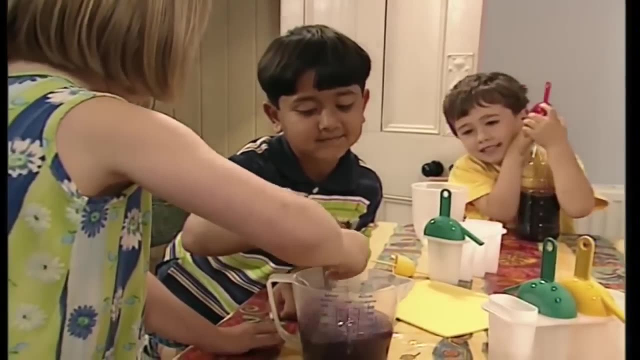 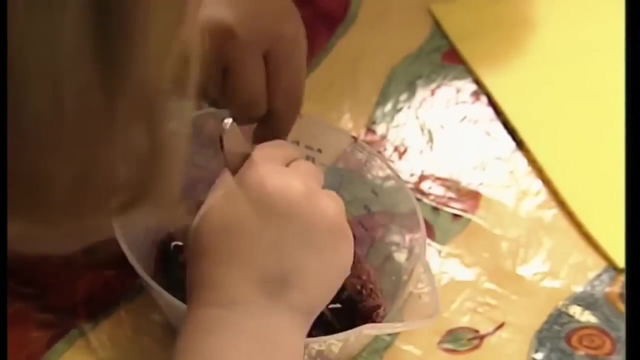 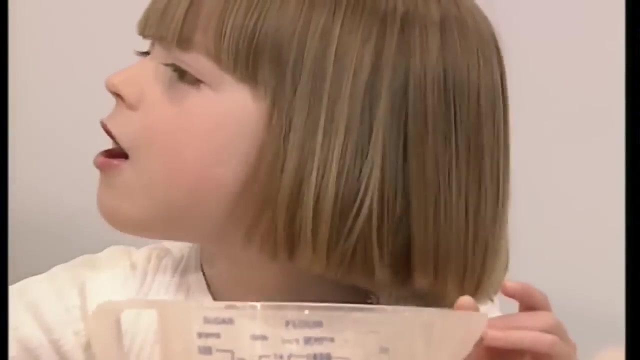 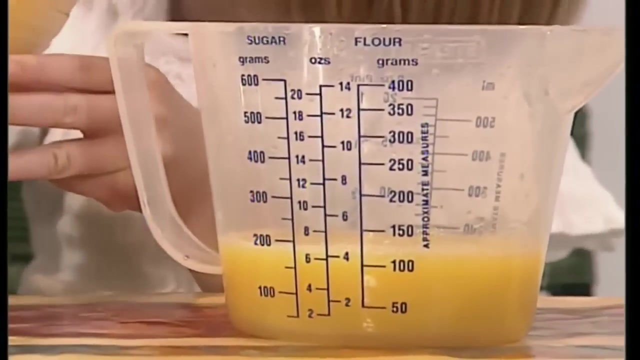 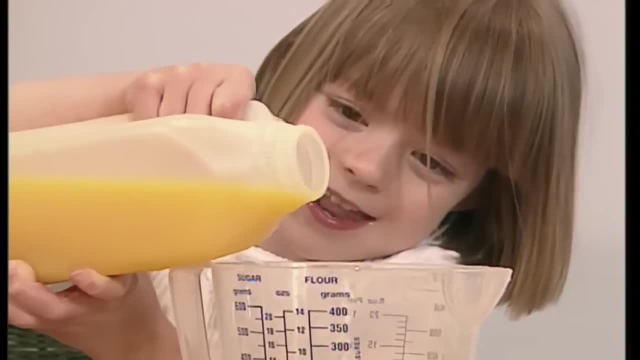 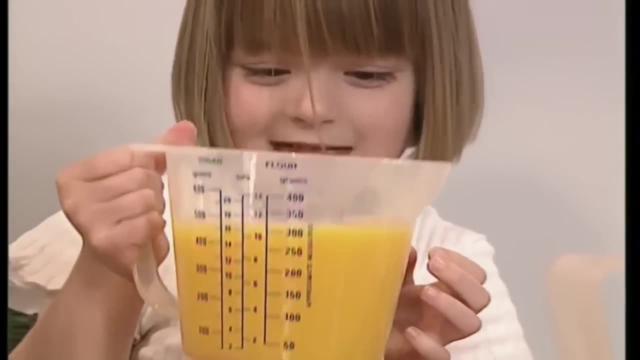 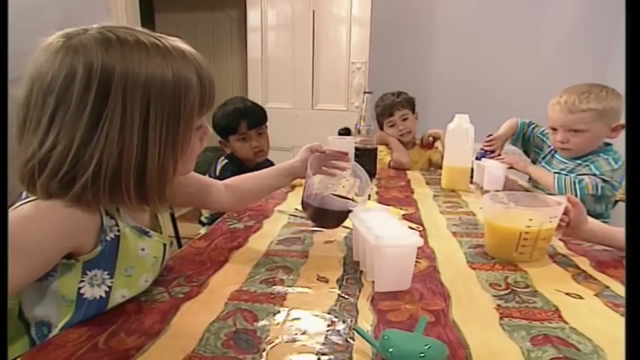 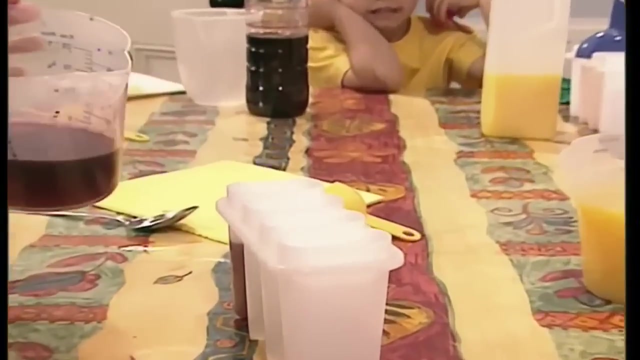 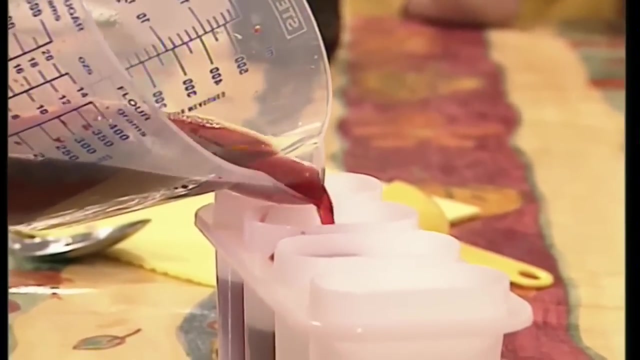 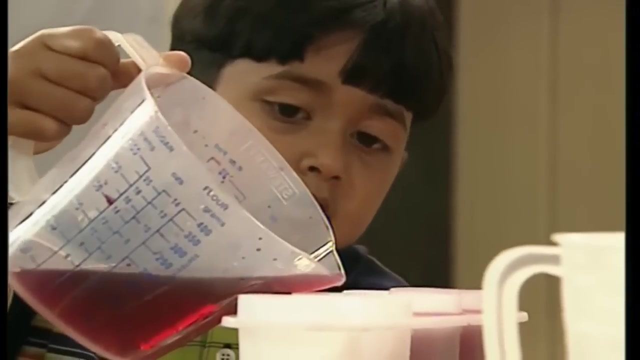 Enough, That's enough, That's enough. No, no, no, Then it's ready to pour into the little pots. Stop, Is that enough? Stop, stop, stop, stop, stop. We're stirring. Can I have some honey now? 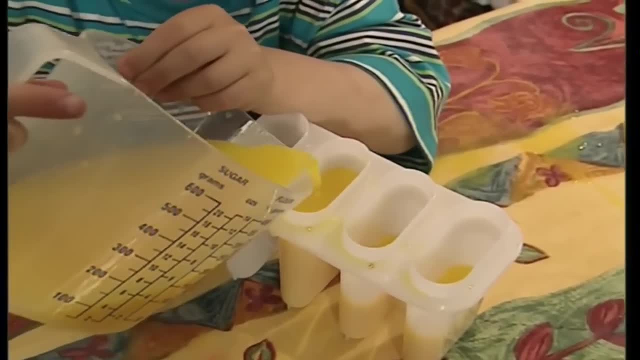 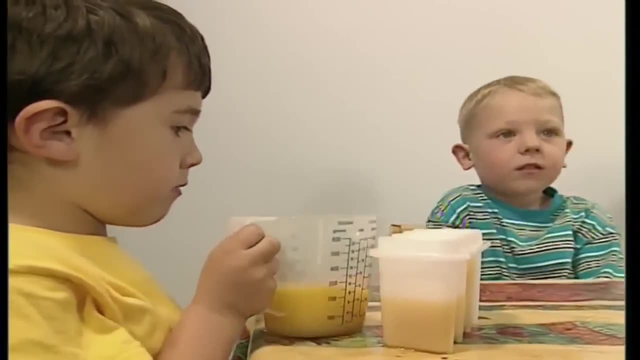 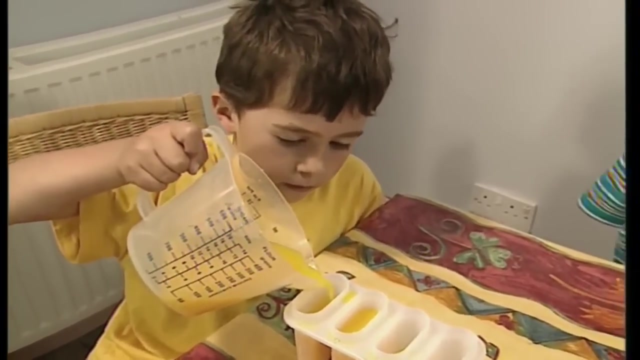 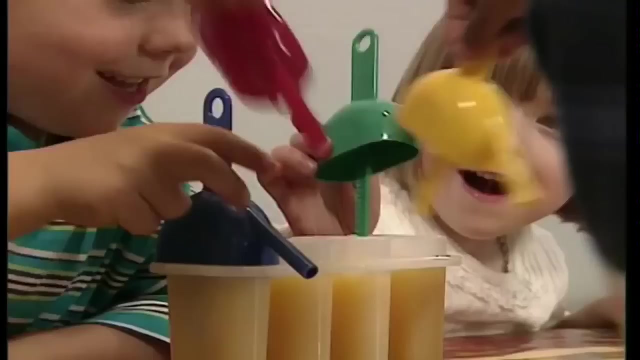 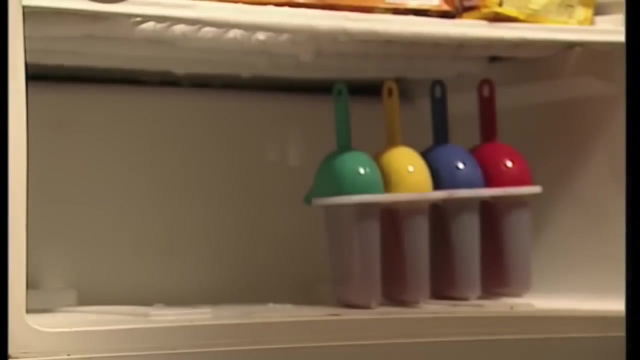 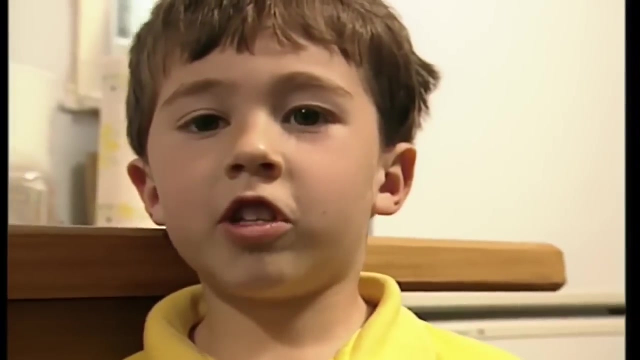 Yeah, Don't want to put too much in. We're taking it in turns. You have to leave a space for it to grow. Stop, Let's put the sticks in. Mum is putting them in the freezer. I hope they're not going to take too long to freeze. 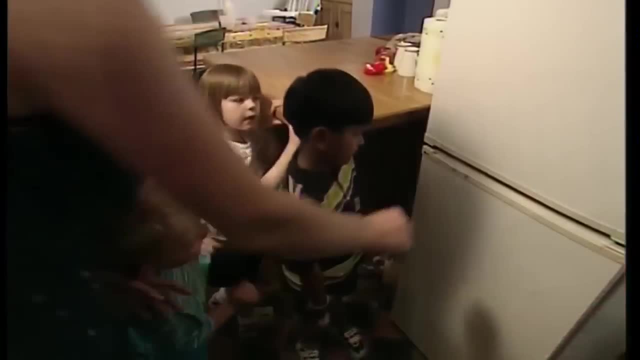 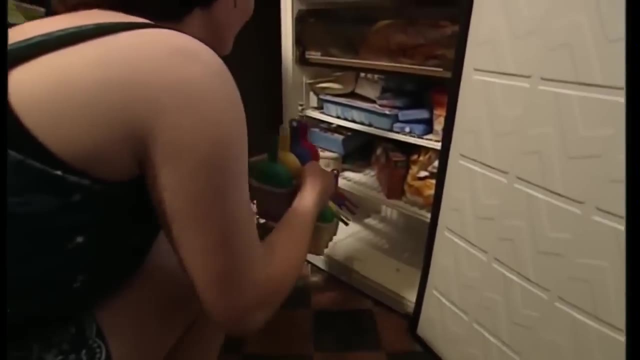 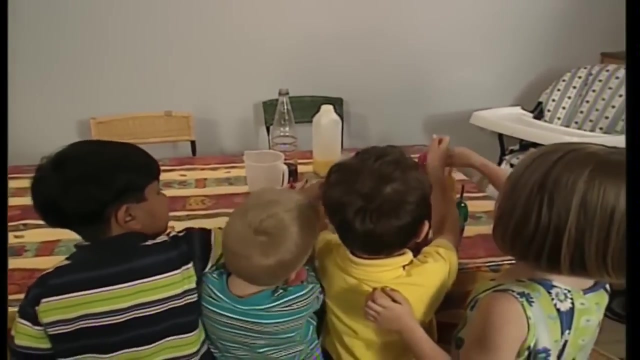 Hurry up ice lollies. They must be ready now. They're ready. Come and see the ice lollies. Come and see the ice lollies. Come and see the ice lollies. Ice lollies at last. 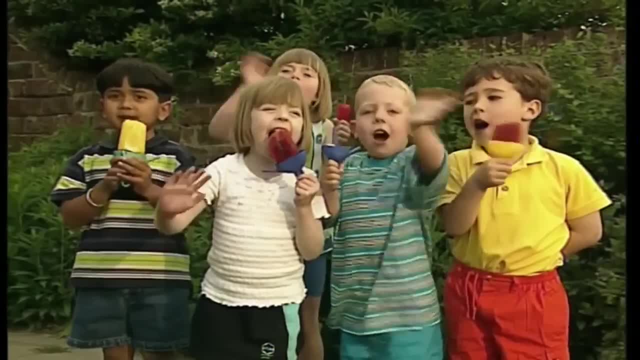 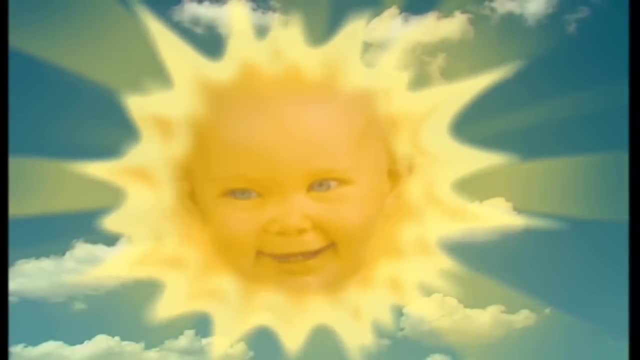 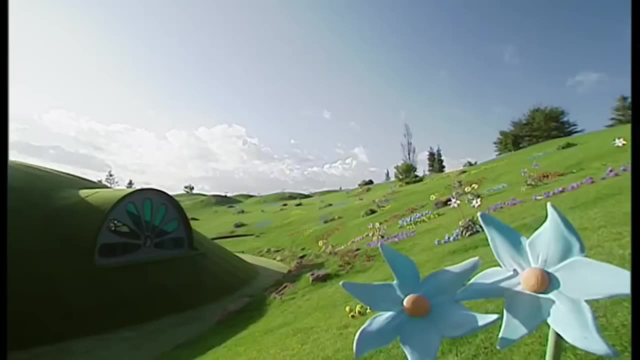 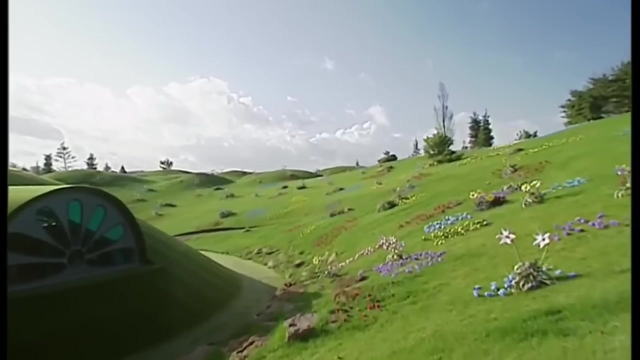 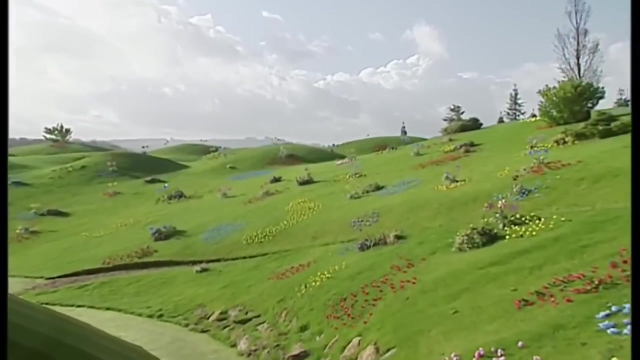 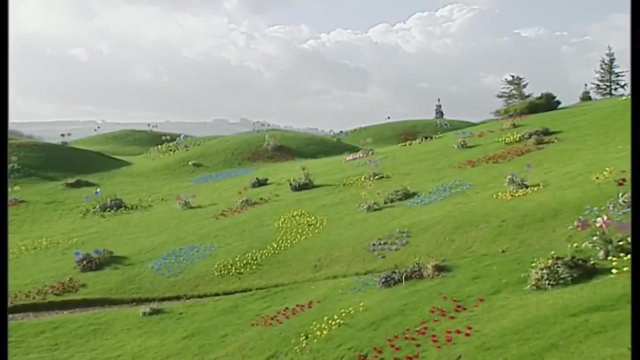 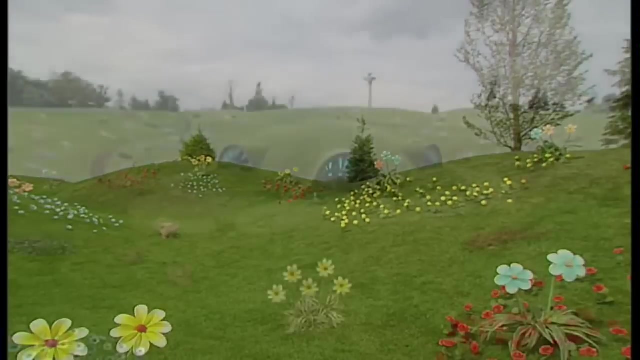 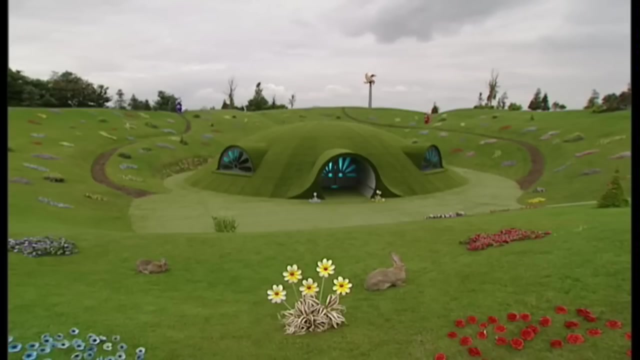 It's lovely. Bye-bye, Bye, Bye, Bye, Bye, Bye, Bye. I love you, baby. Bye Bye, My dear. I love you. I love you. Thank you for watching. Thank you for watching. 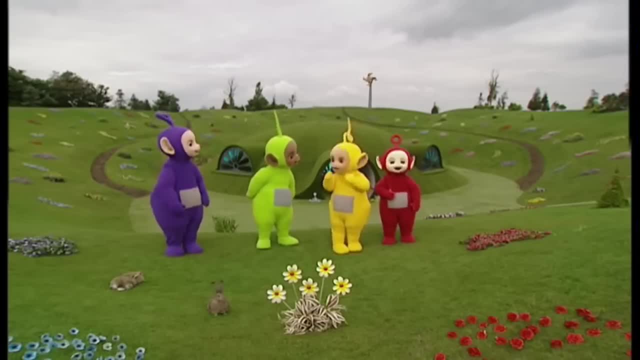 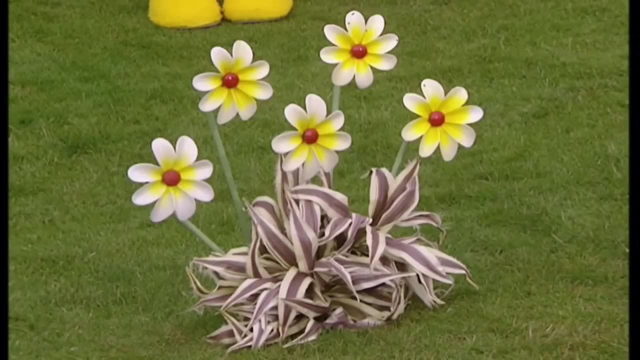 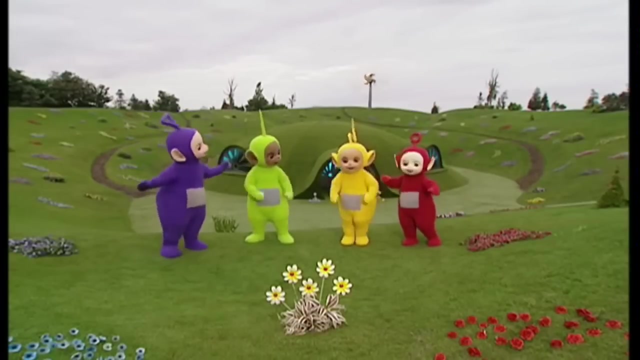 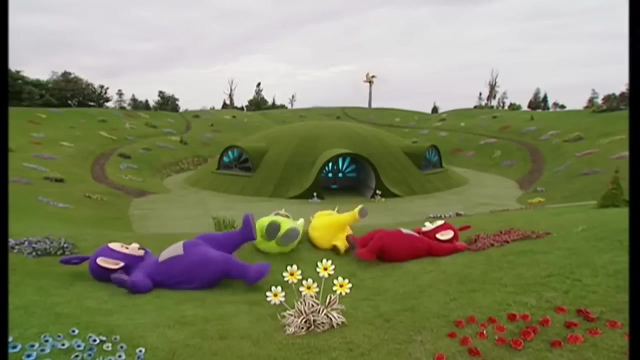 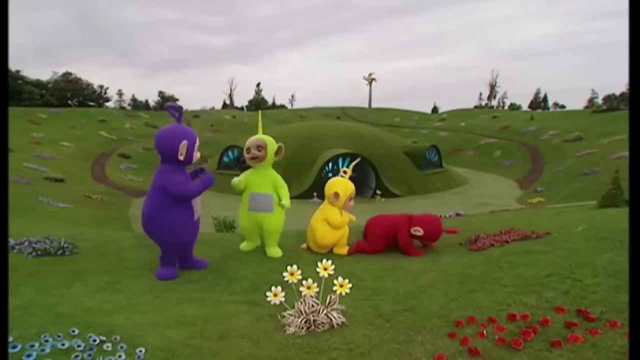 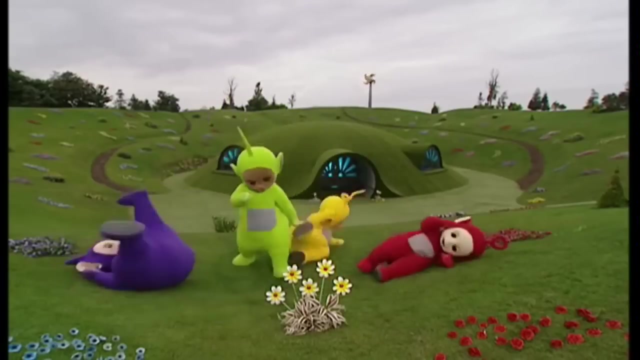 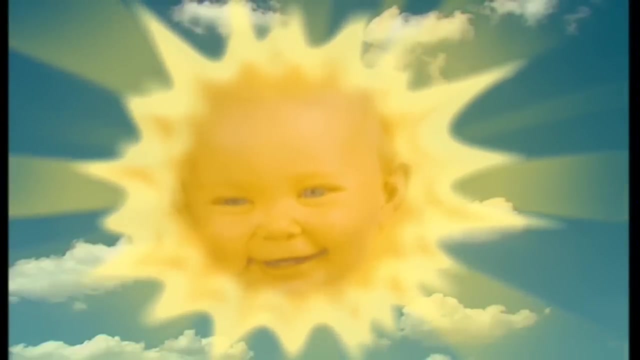 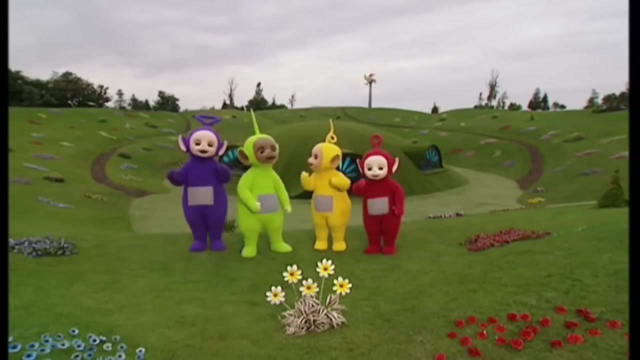 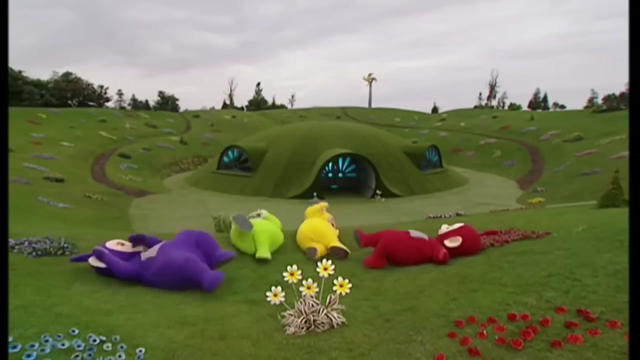 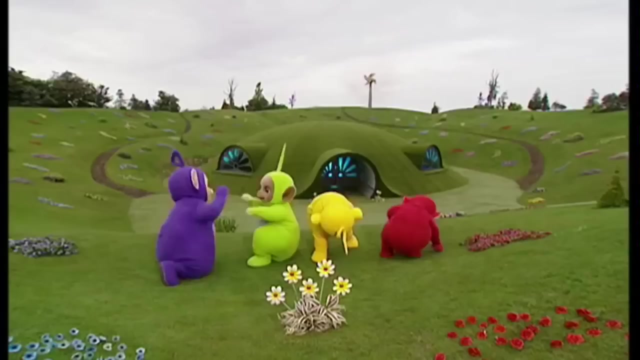 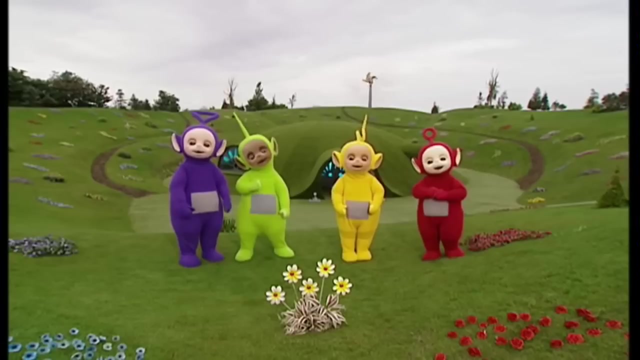 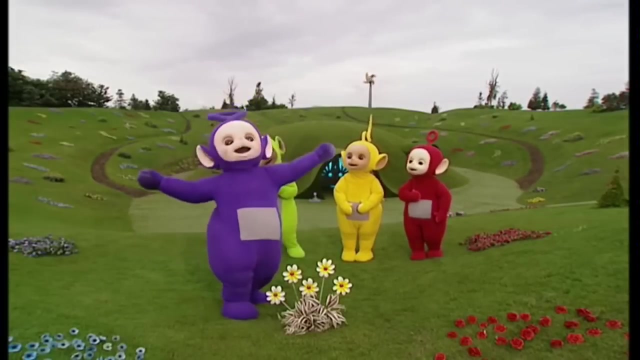 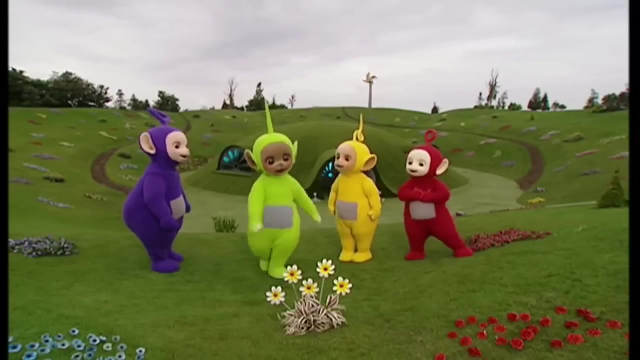 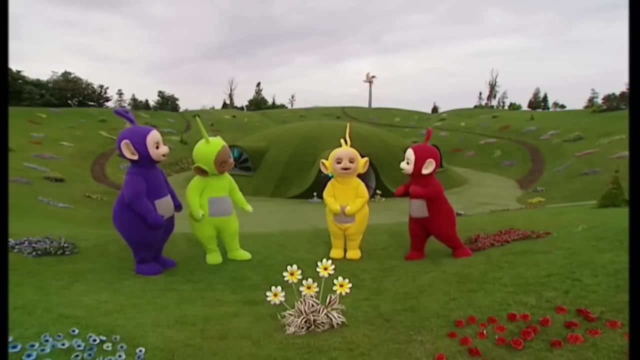 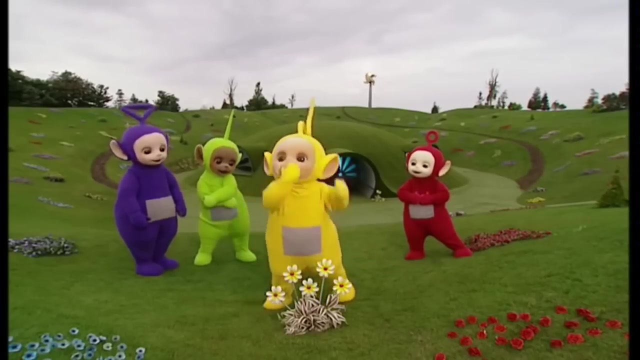 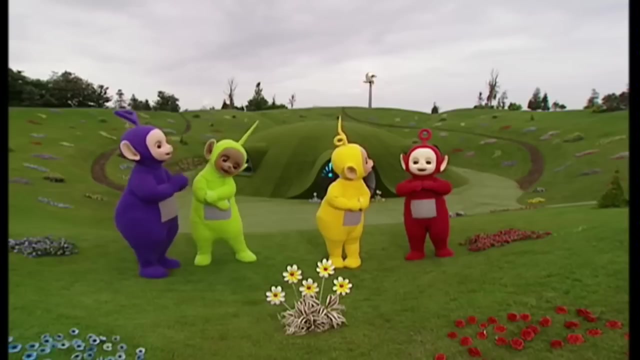 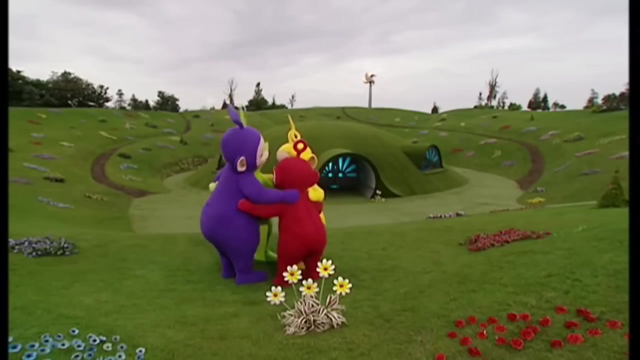 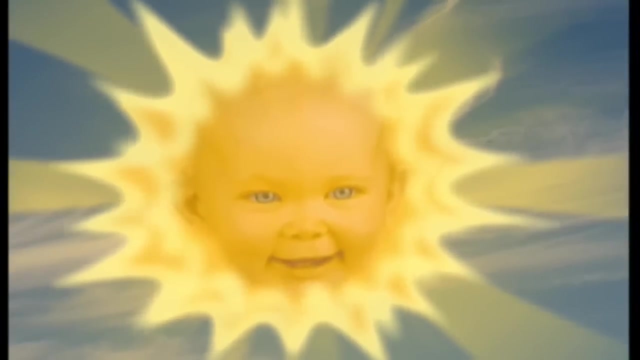 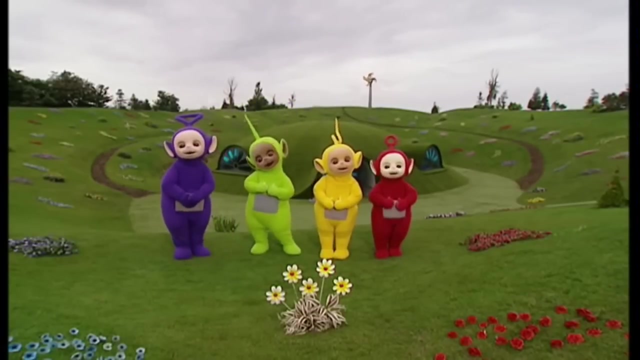 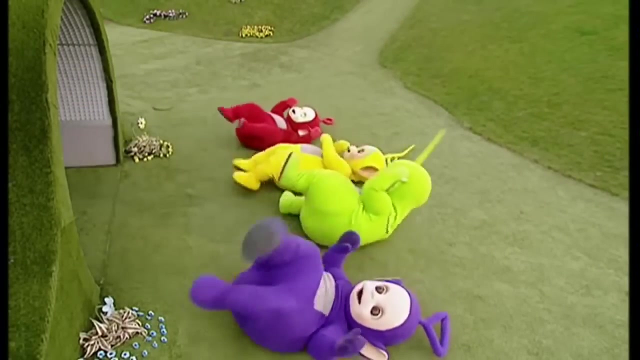 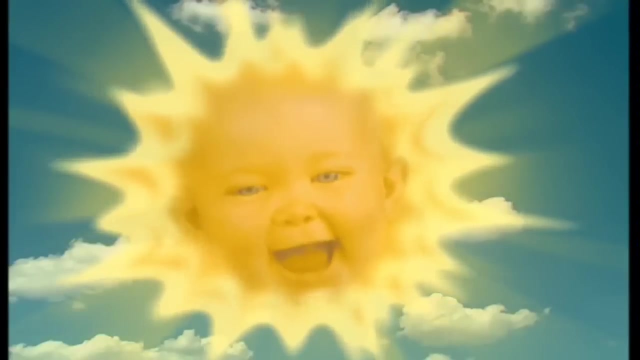 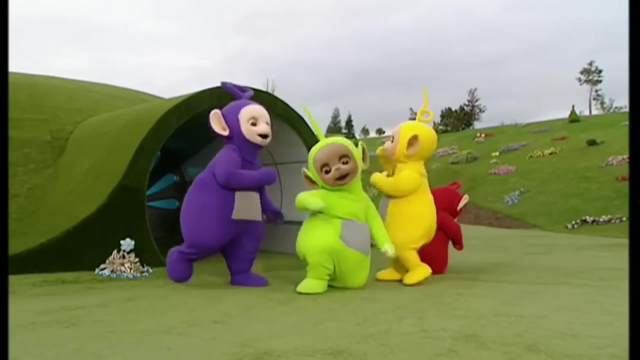 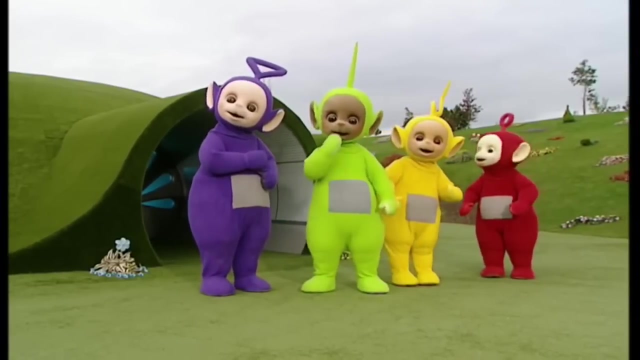 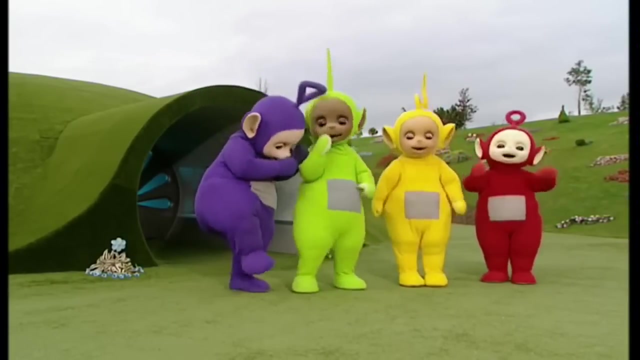 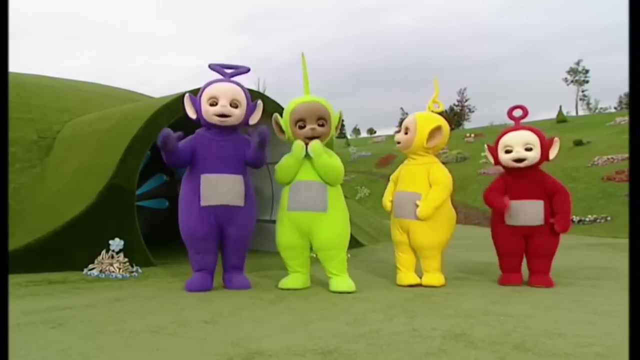 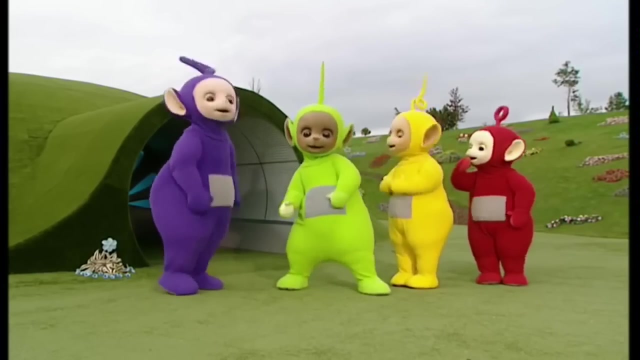 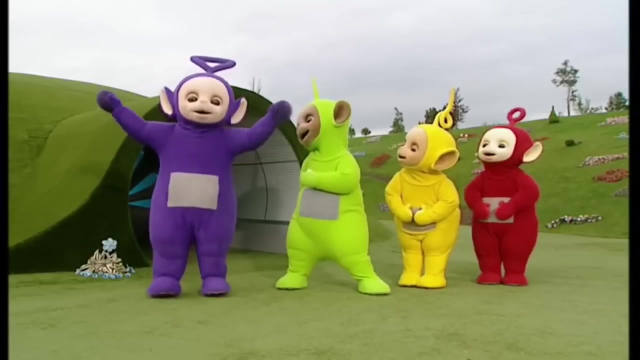 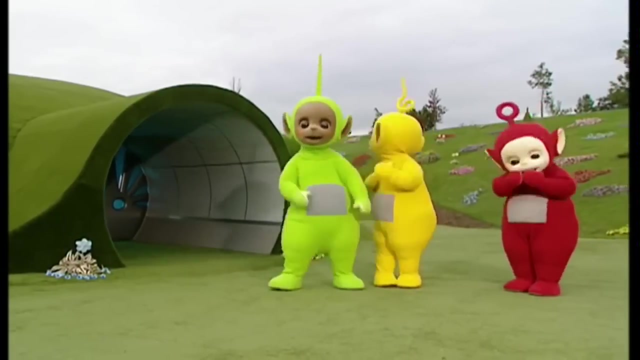 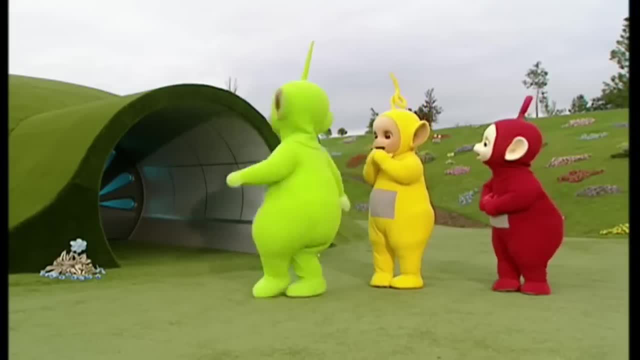 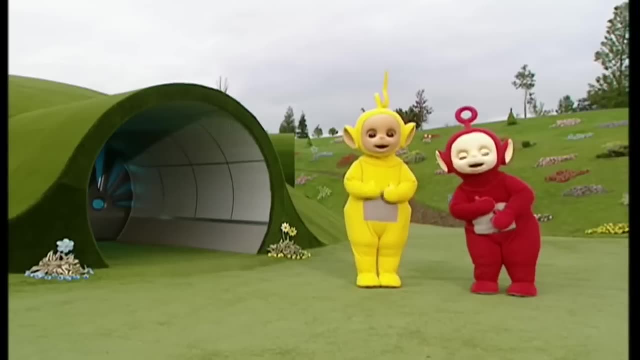 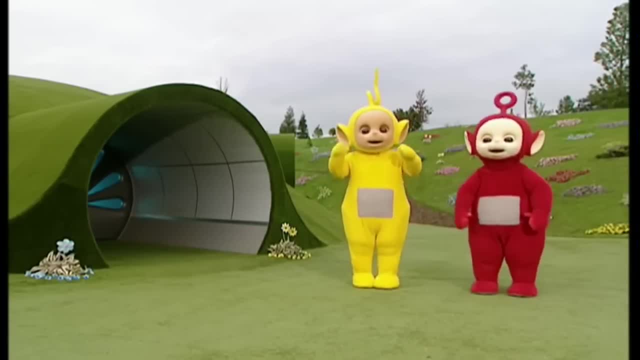 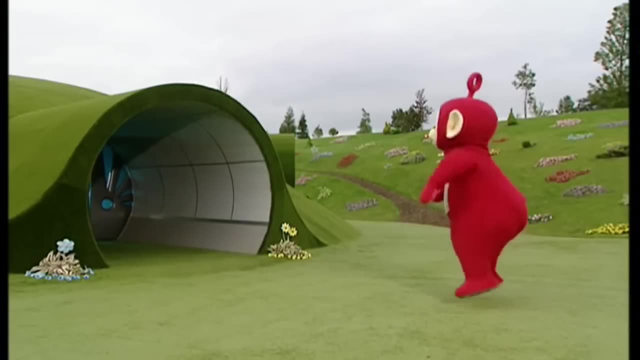 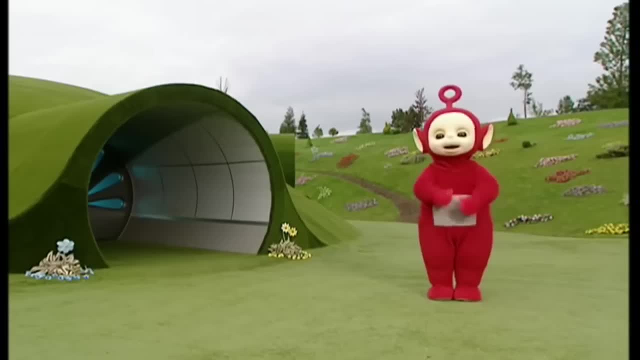 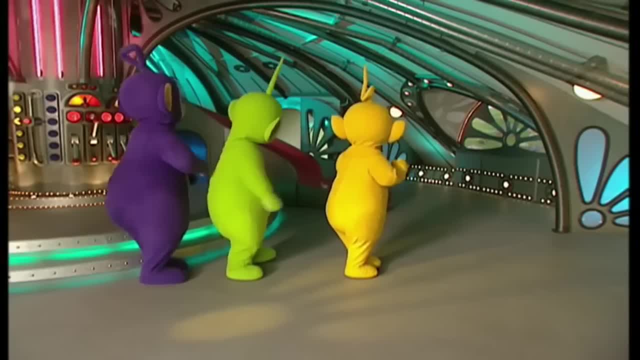 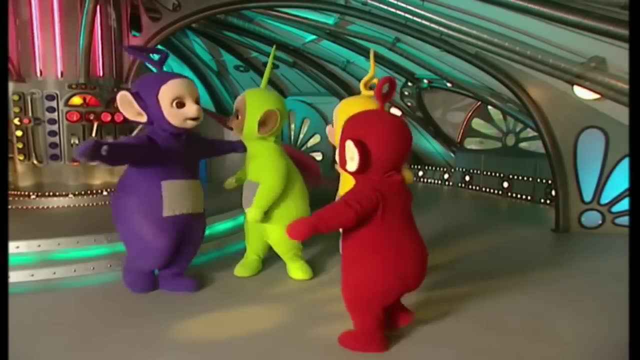 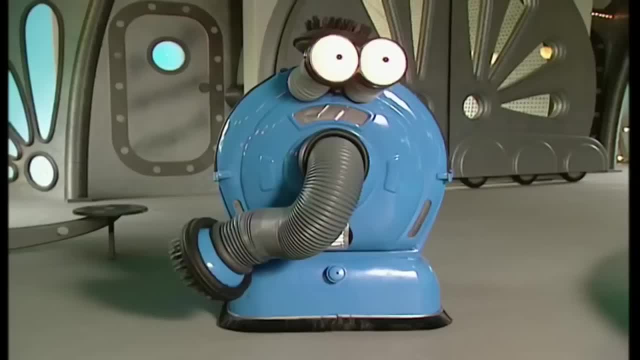 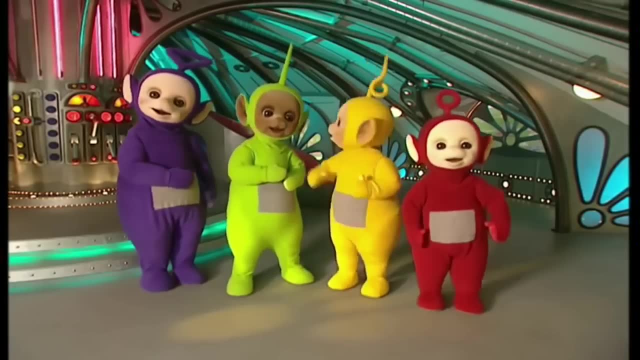 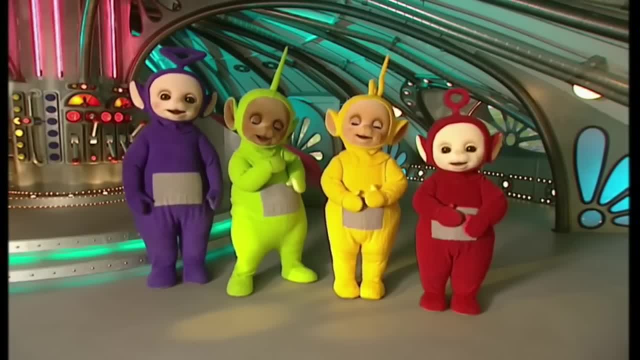 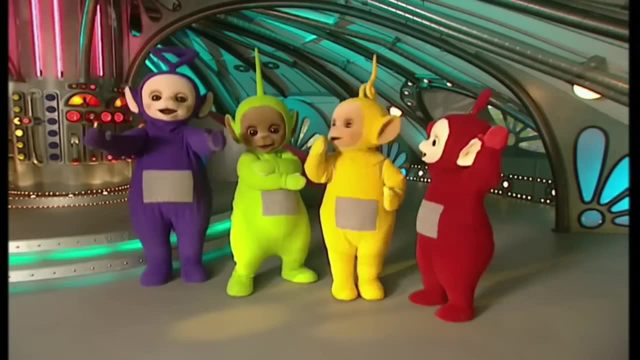 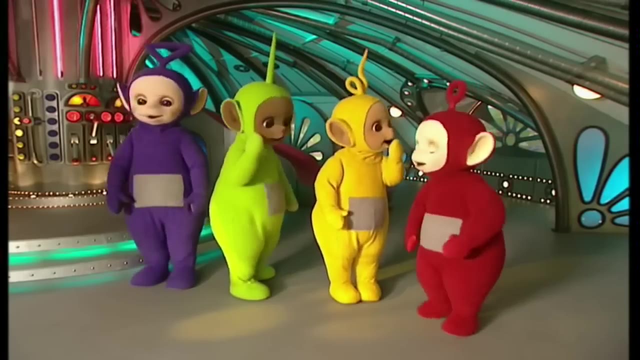 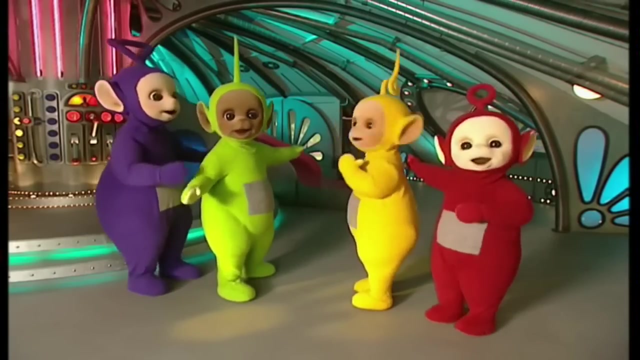 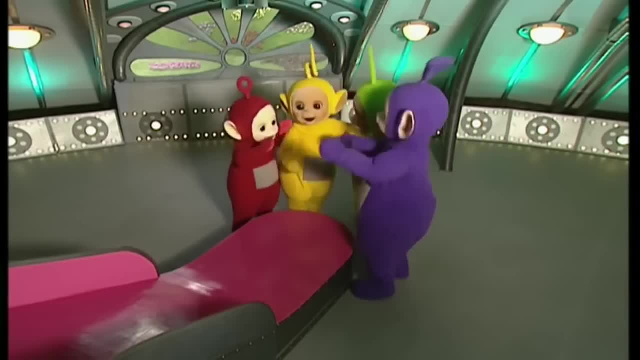 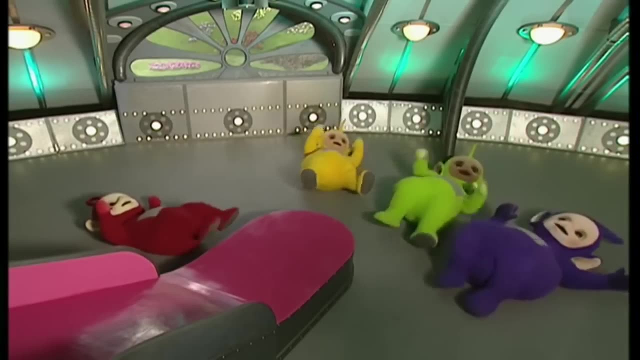 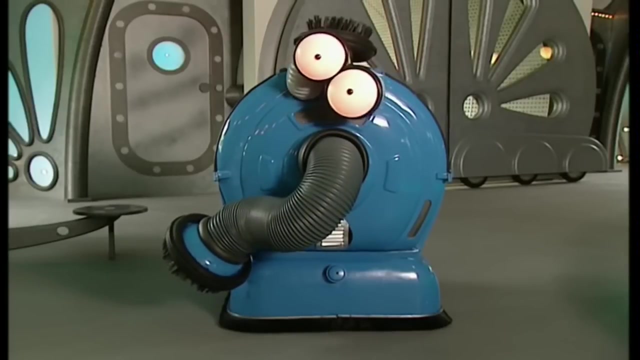 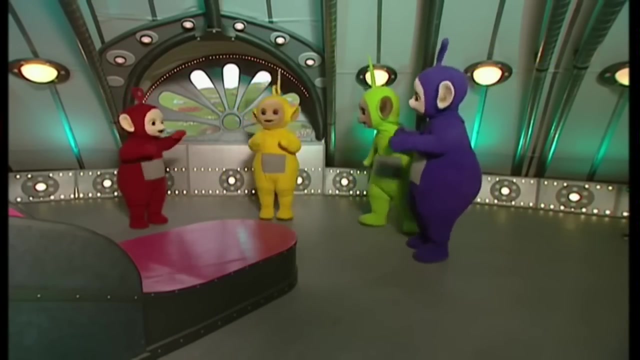 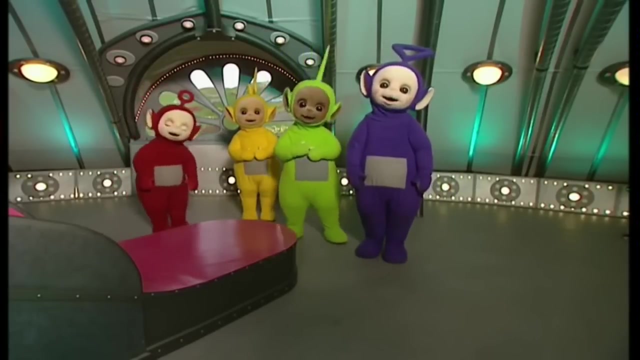 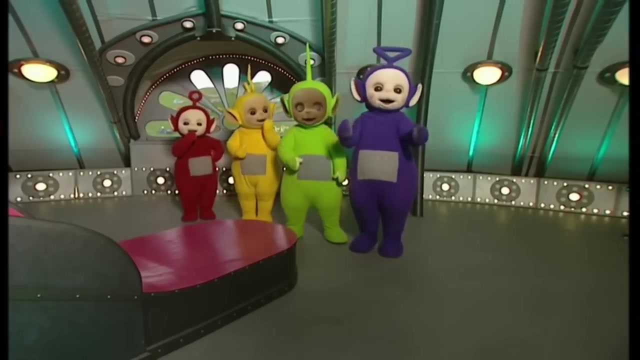 Up a slide. Oh dear, Oh dear Teletubbies, you can't all go up the slide at once. Oh dear Teletubbies, Oh dear, Oh dear, Uh-oh, You have to go up the slide one at a time. 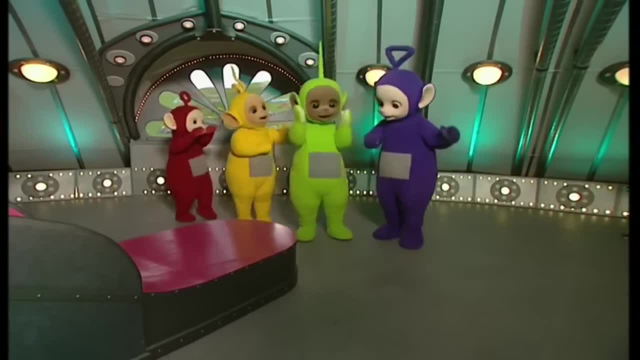 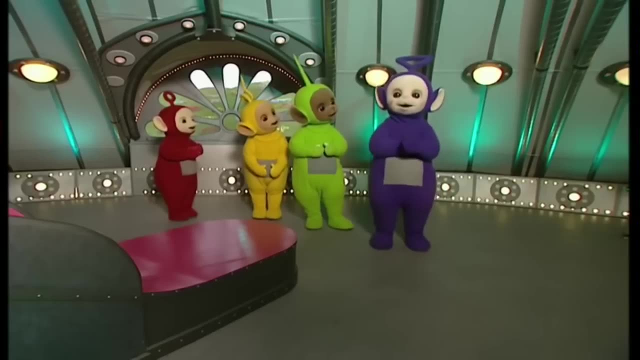 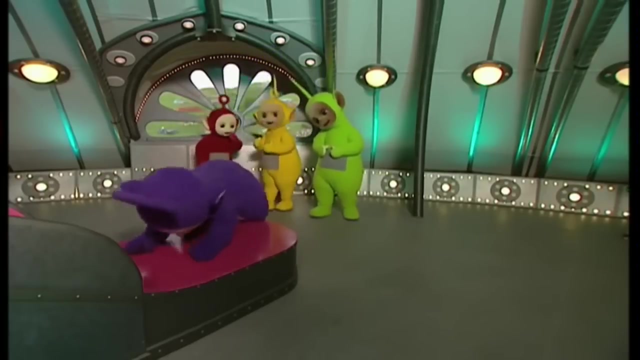 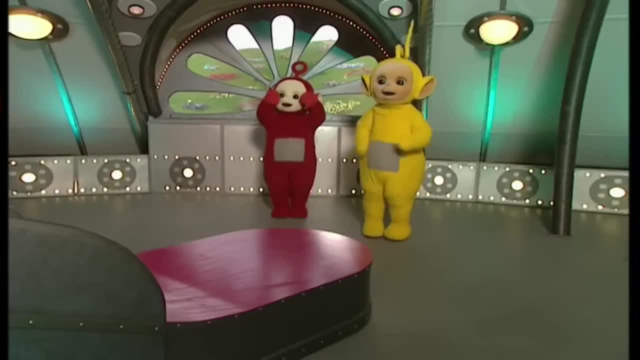 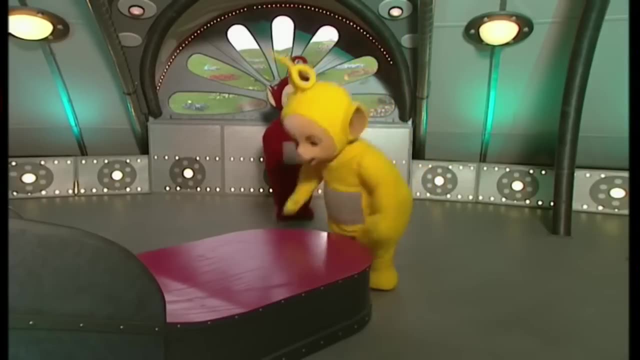 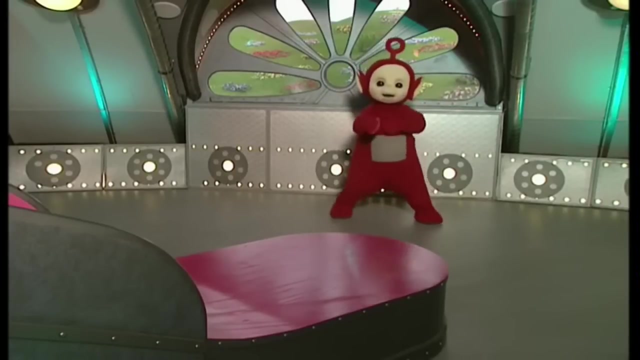 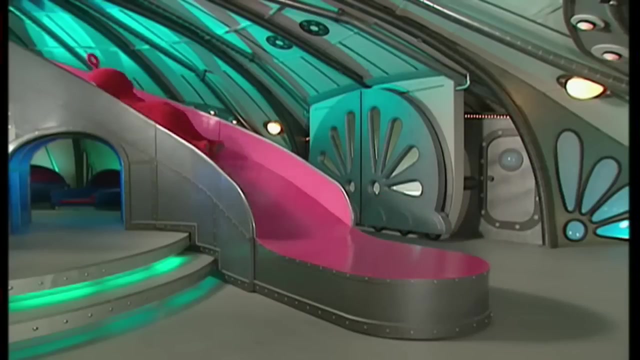 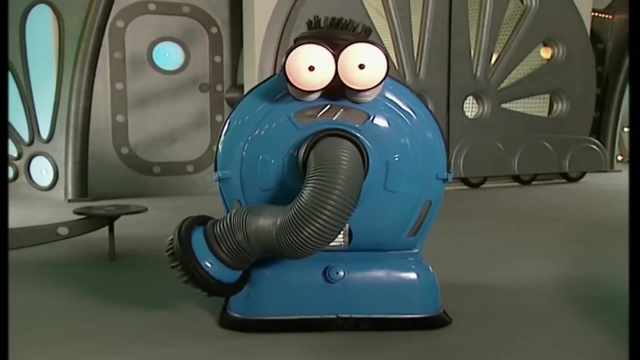 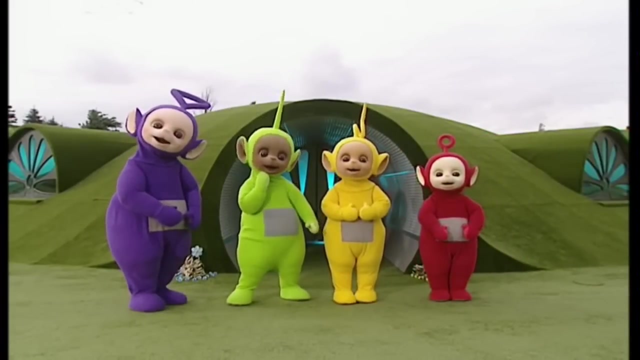 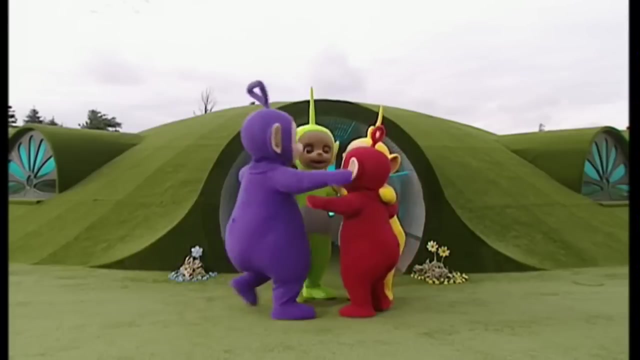 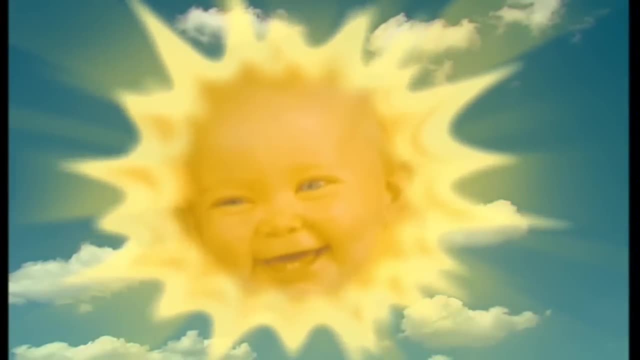 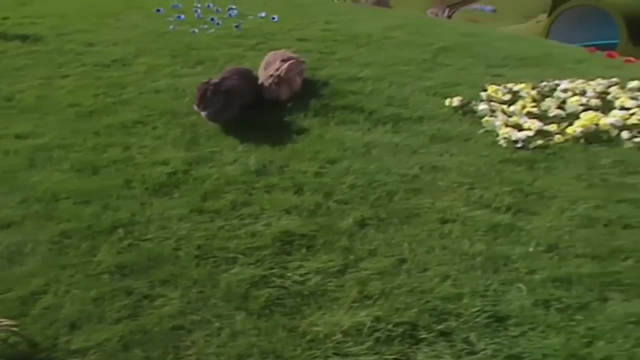 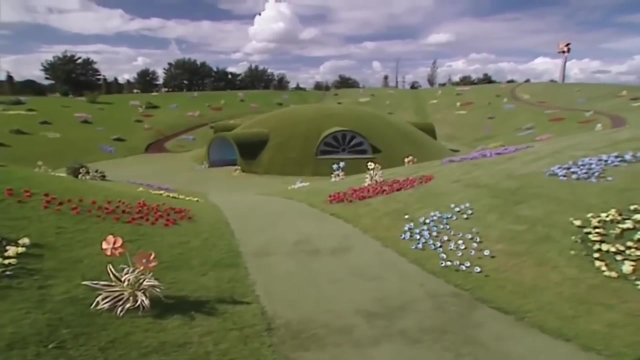 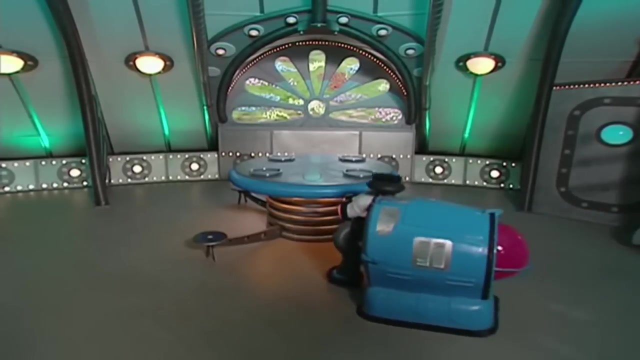 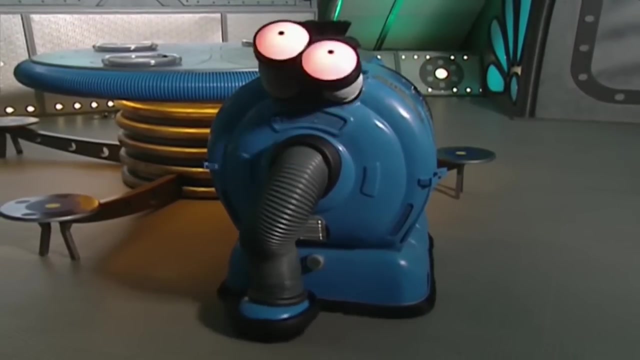 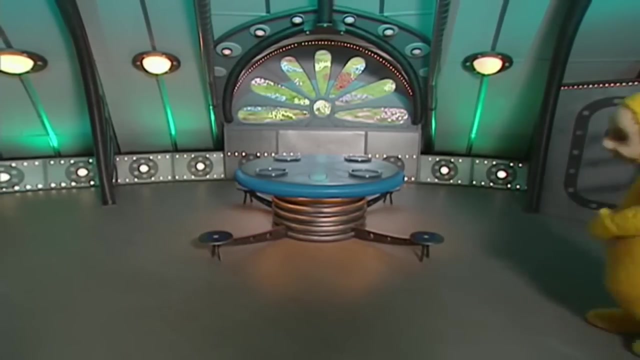 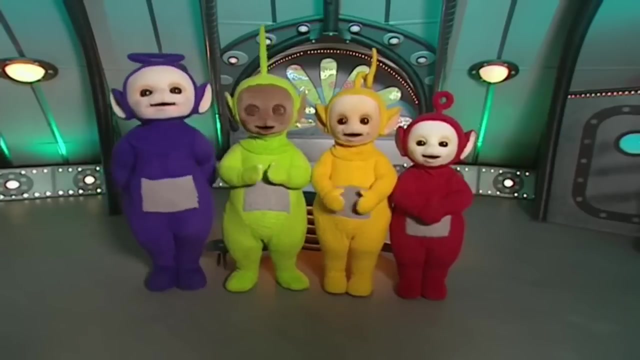 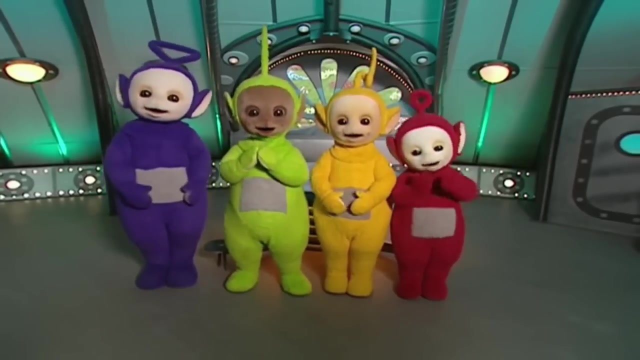 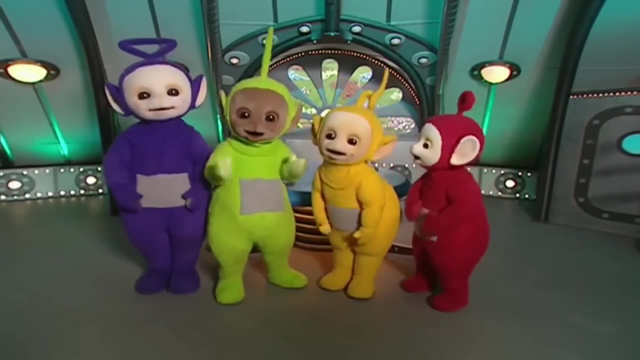 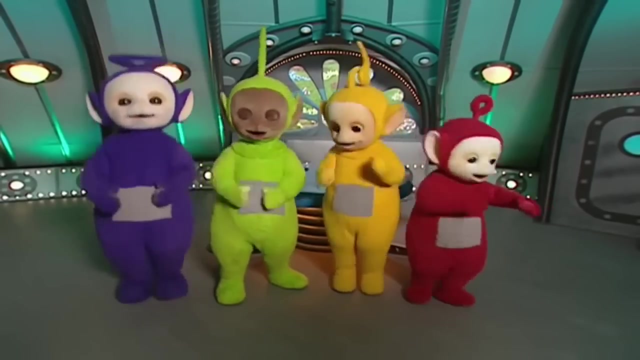 Big hug carbon baby. One day in Teletubbyland, the Teletubbies were feeling hungry, Ooh, hungry. But then it was time for Tubby Toast. Ooh, Tubby Toast, Tubby Toast, Hey, Tubby Toast. 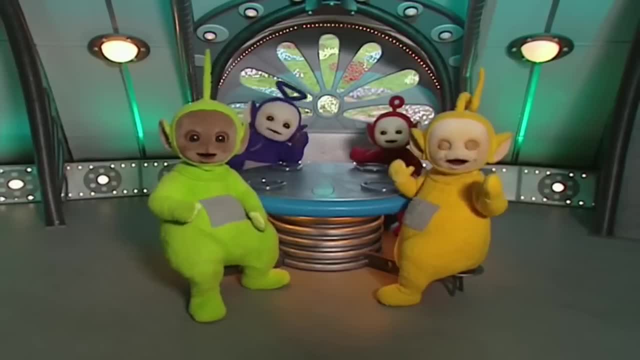 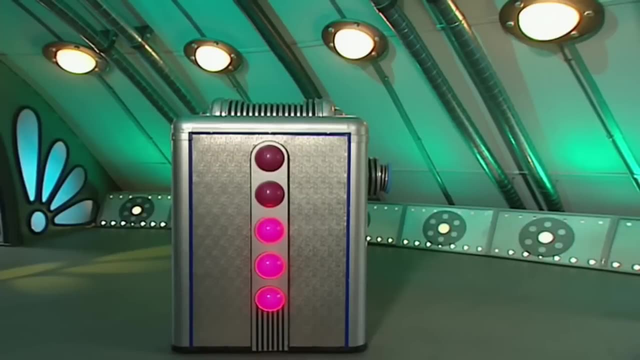 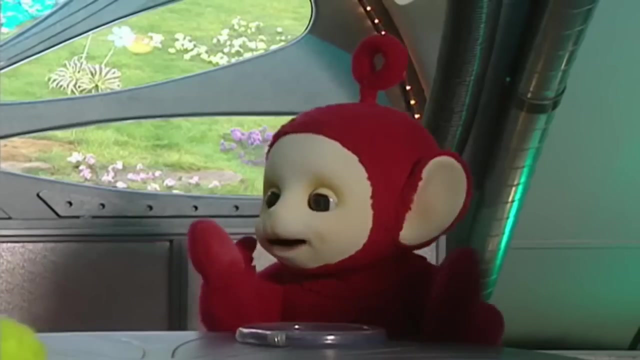 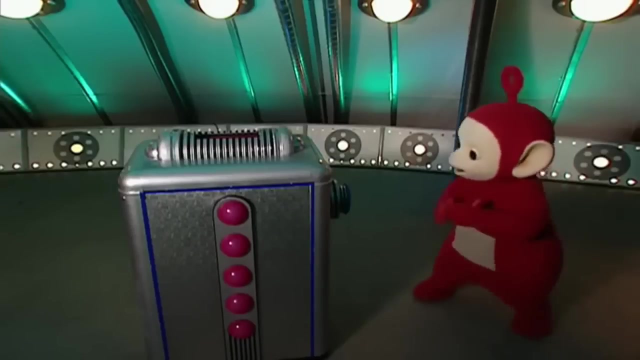 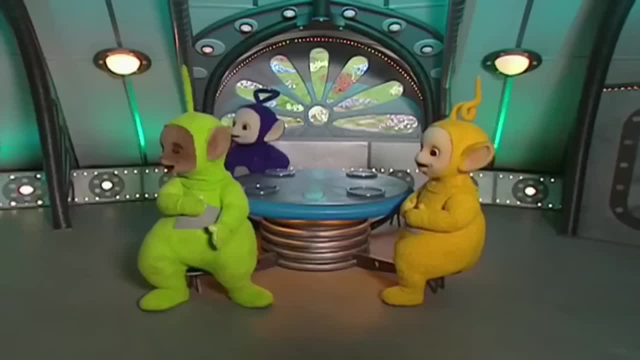 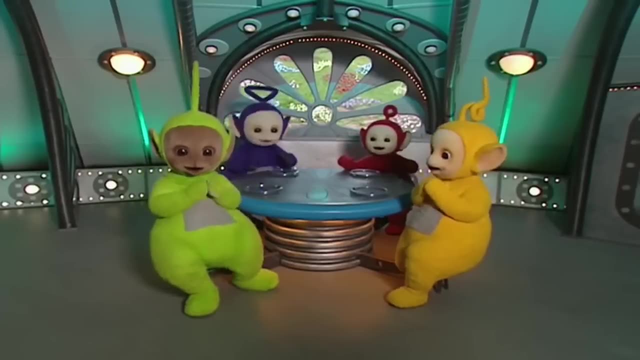 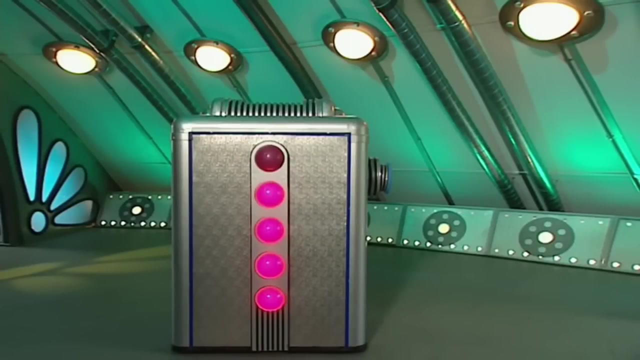 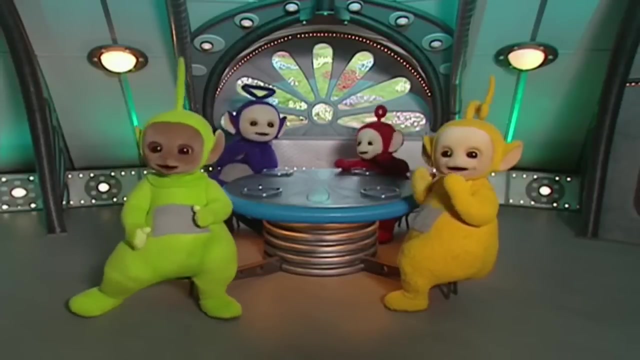 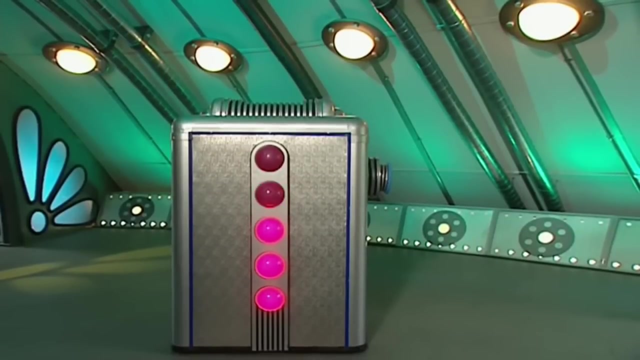 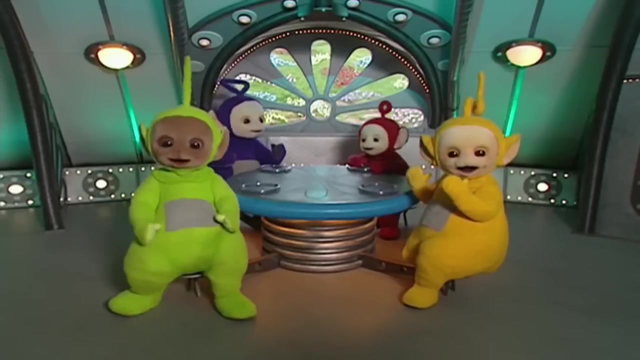 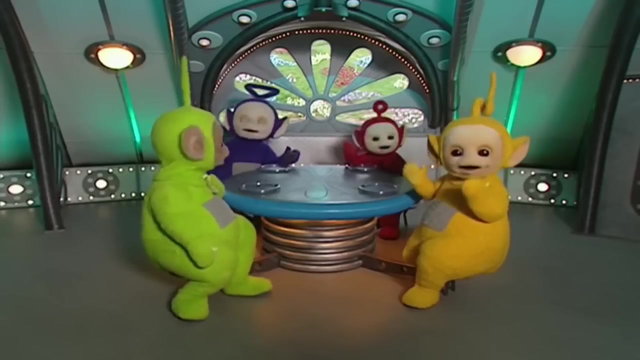 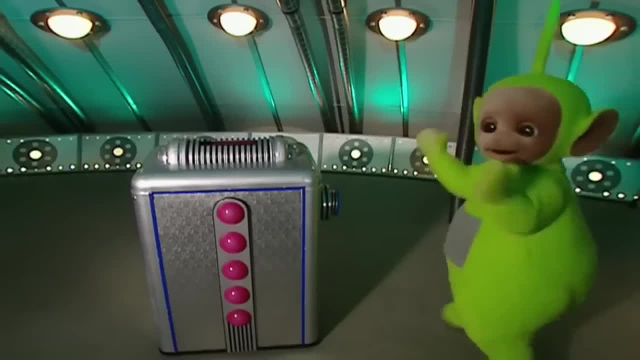 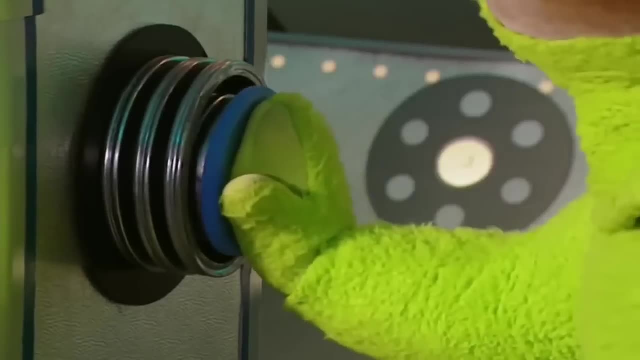 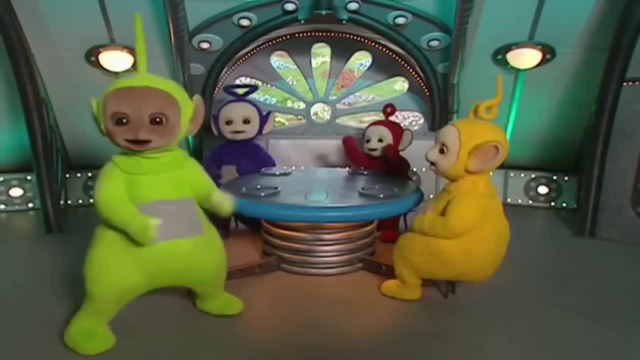 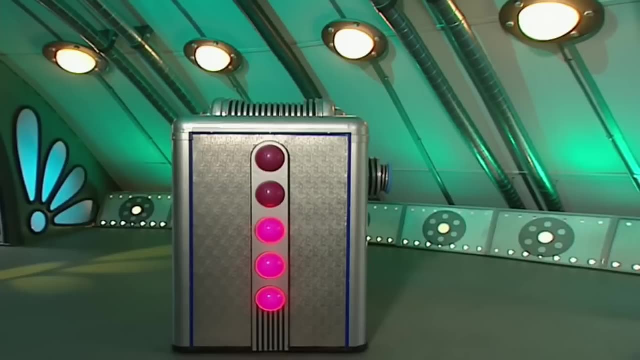 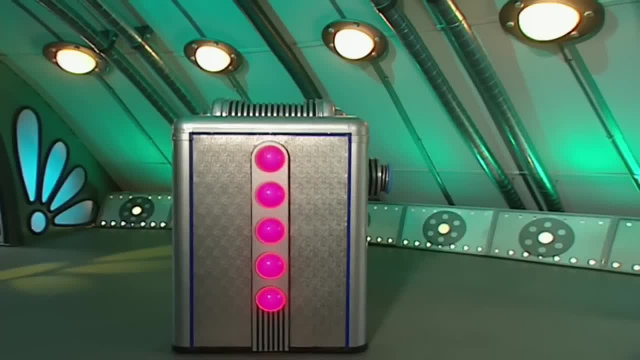 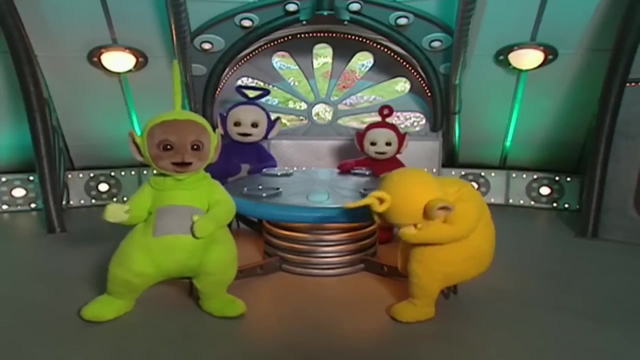 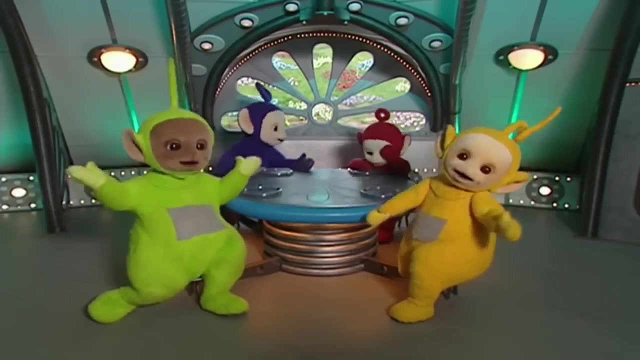 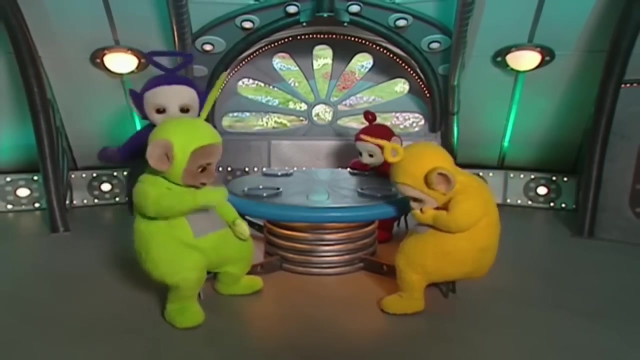 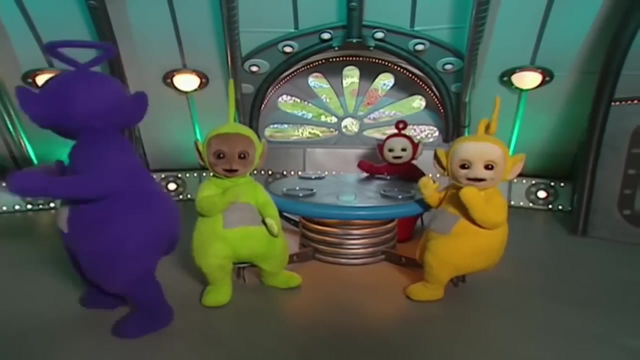 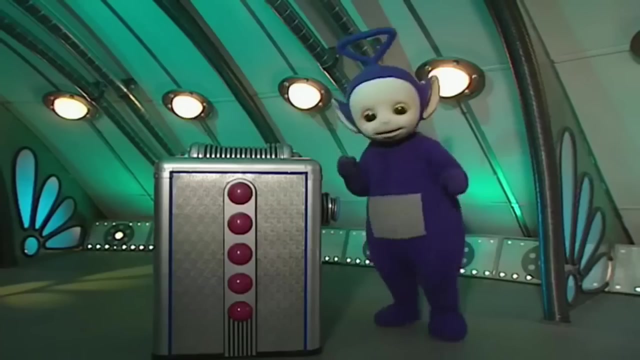 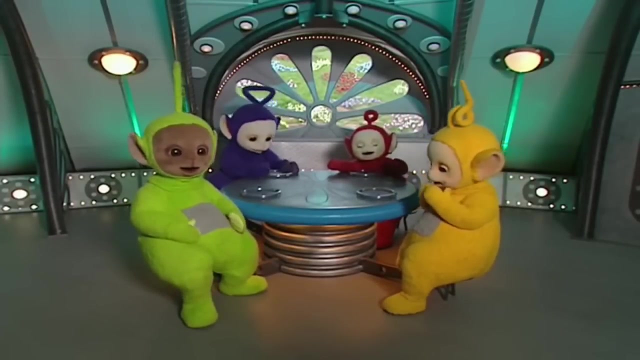 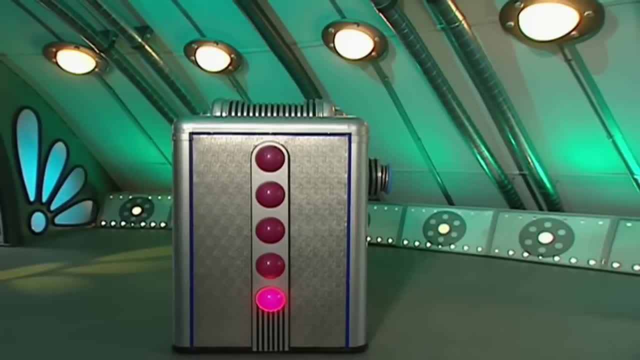 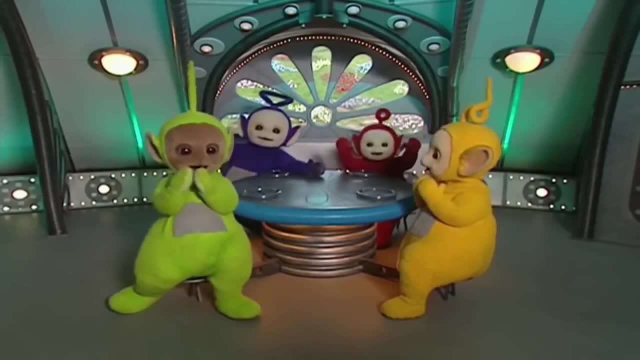 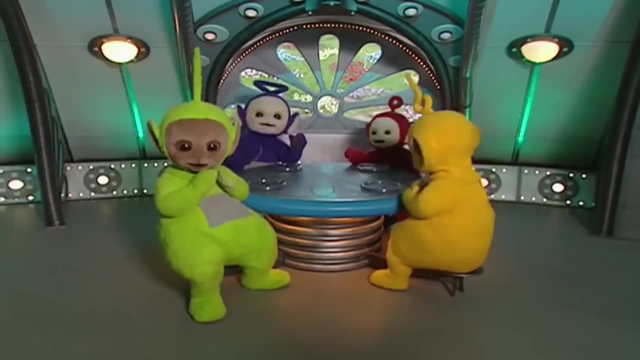 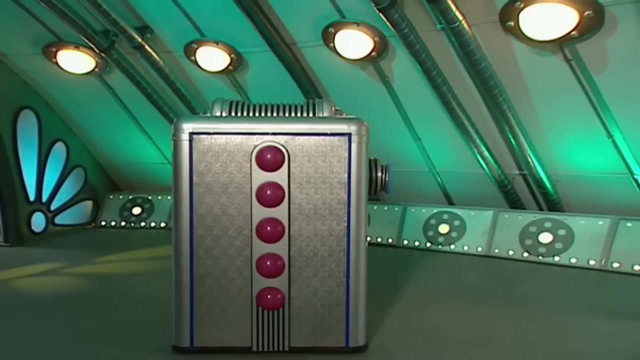 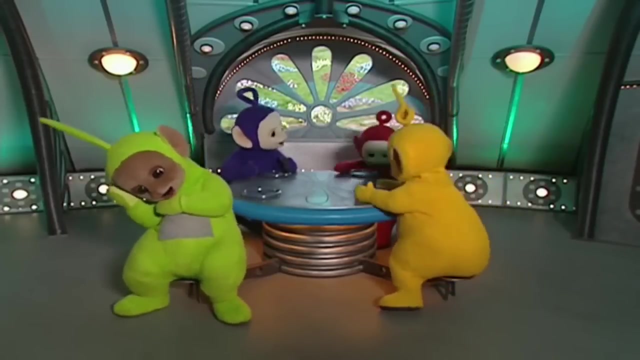 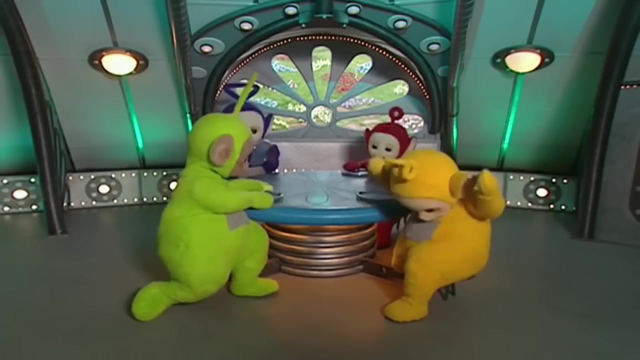 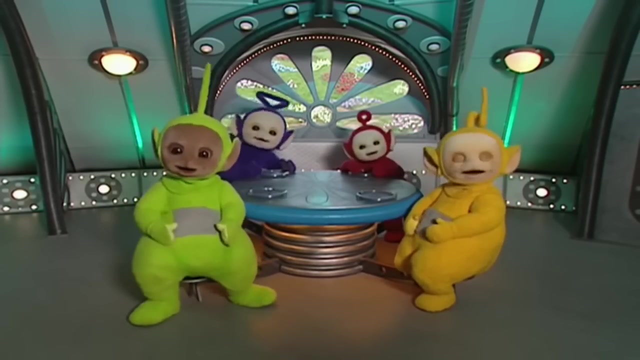 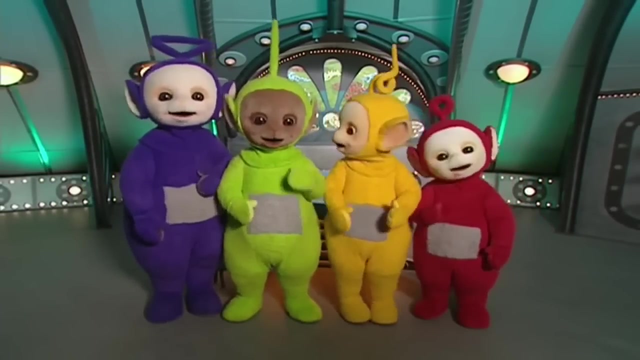 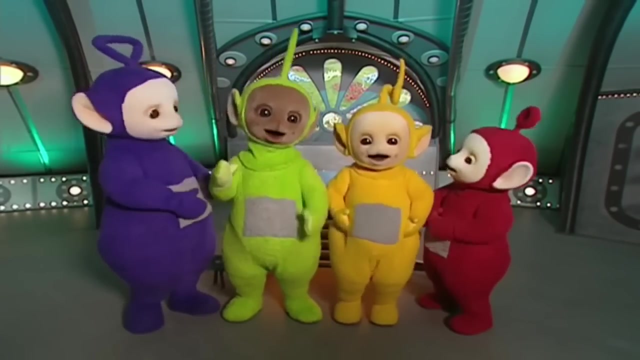 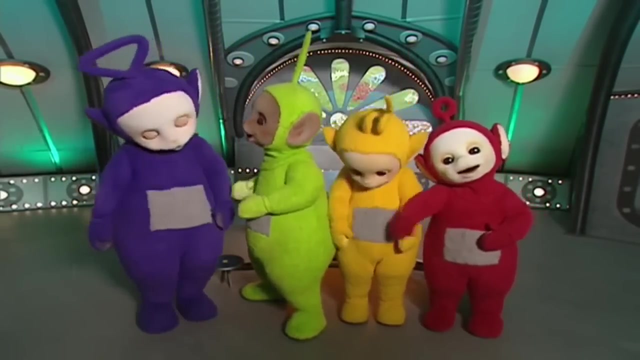 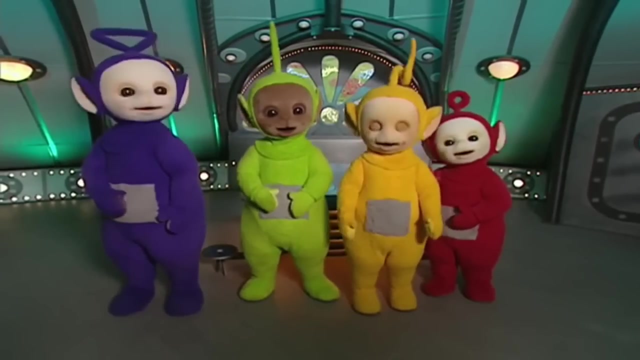 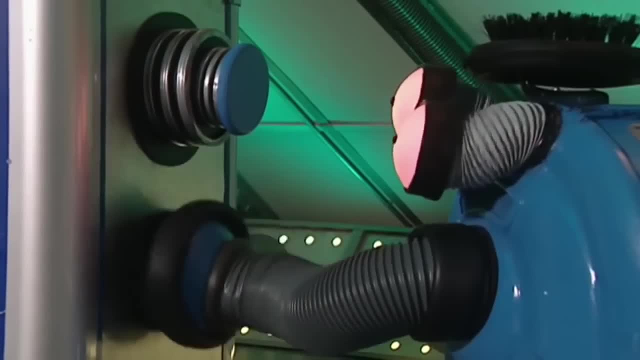 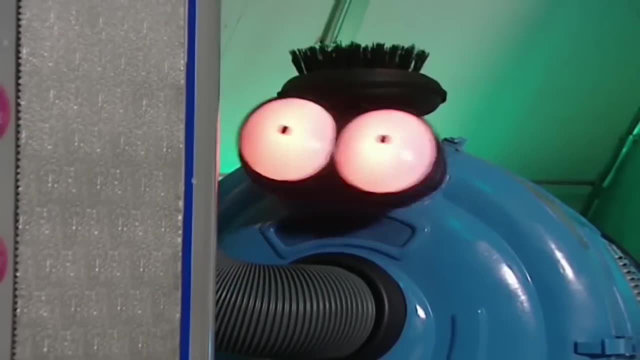 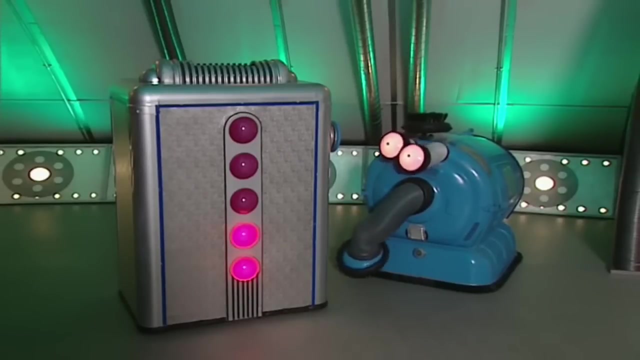 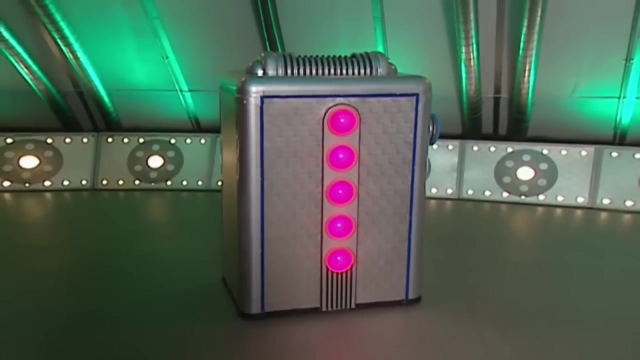 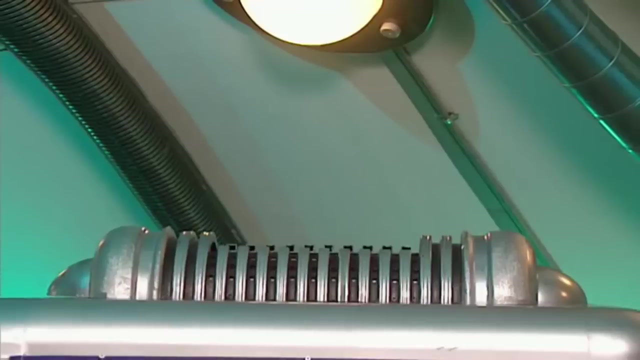 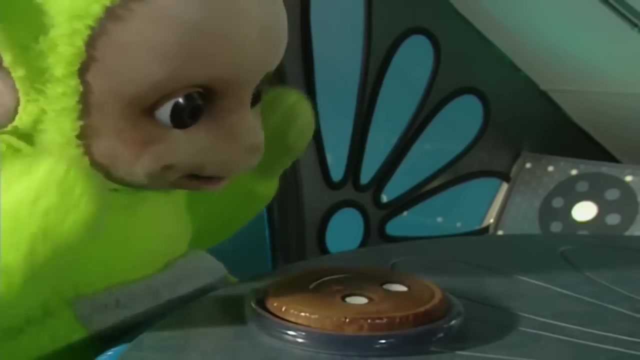 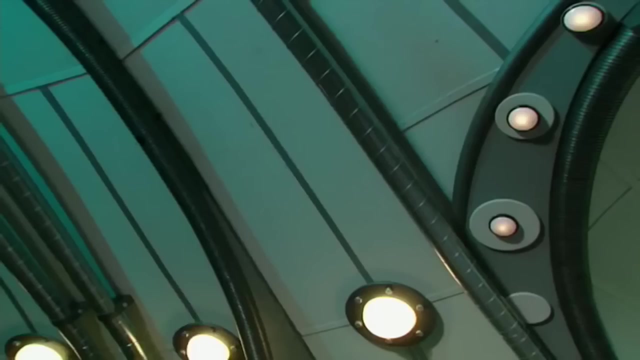 Ooh, they're getting hung up. Hey, Tommy Tunes. Tommy Tunes, Whatcha doing? Yay, Dipsy Toast, Dipsy Toast. Ooh, Tommy Toast, Yay, Ticky Wicky Toast. 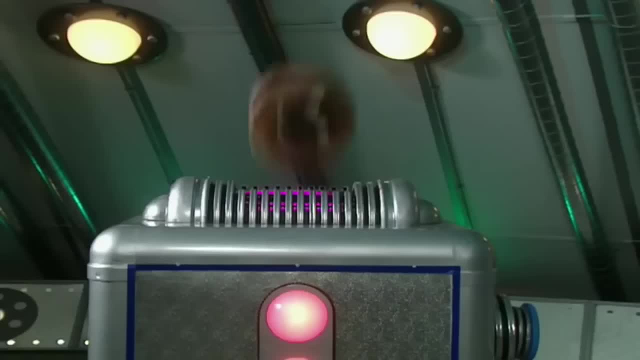 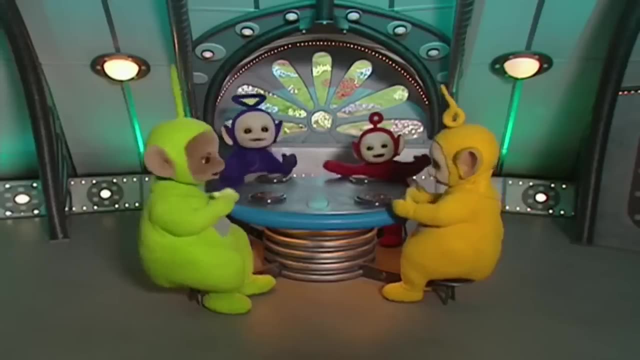 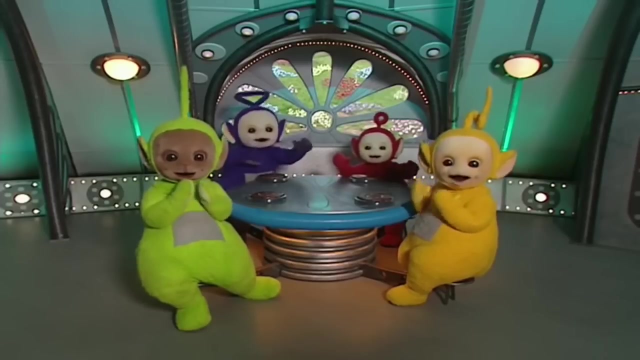 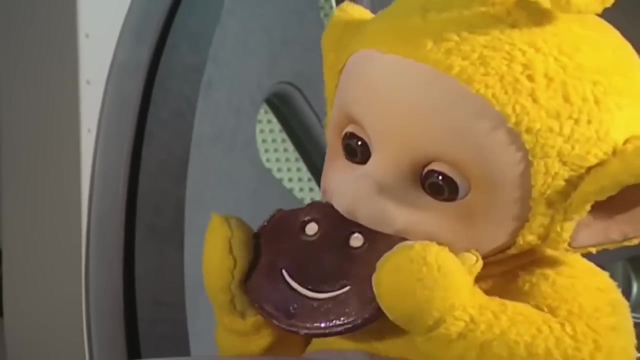 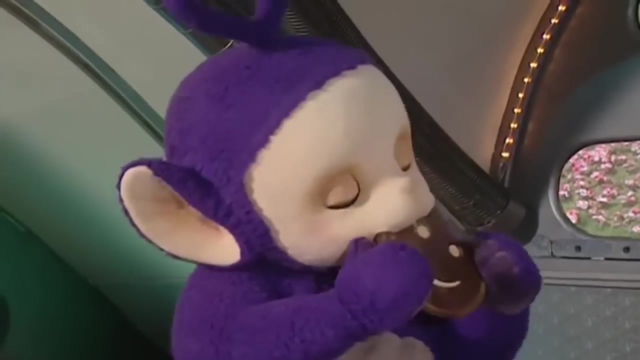 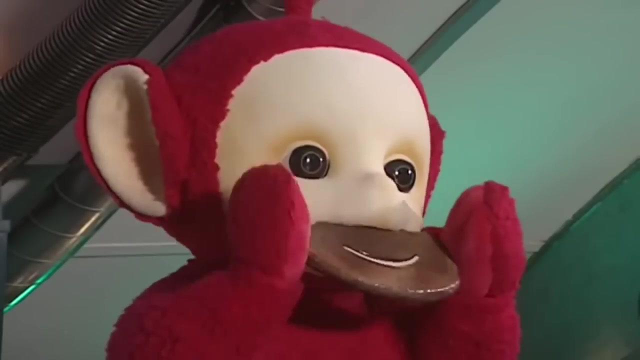 Tommy Toast, Tommy Toast Toast, Tommy Toast, Ticky Wicky Toast, Tommy Toast, Ticky Wicky Toast, Ticky Toast. The Teletubbies ate their tubby toast, Tubby toast, Tubby toast. And the Teletubbies weren't hungry anymore. 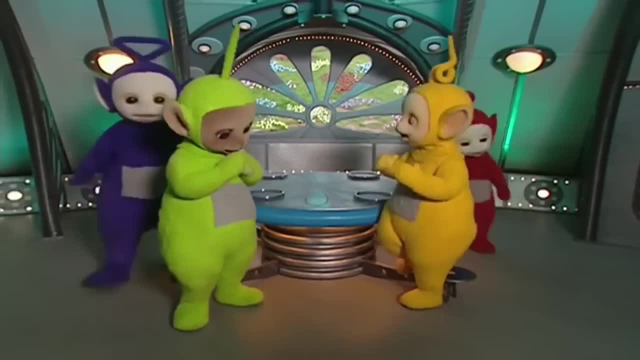 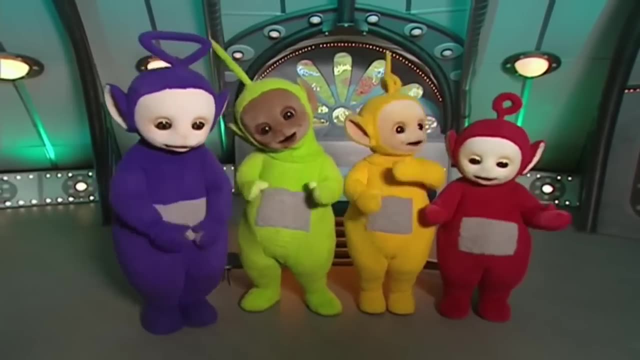 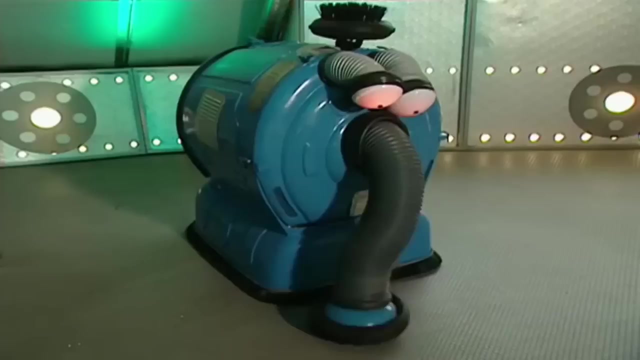 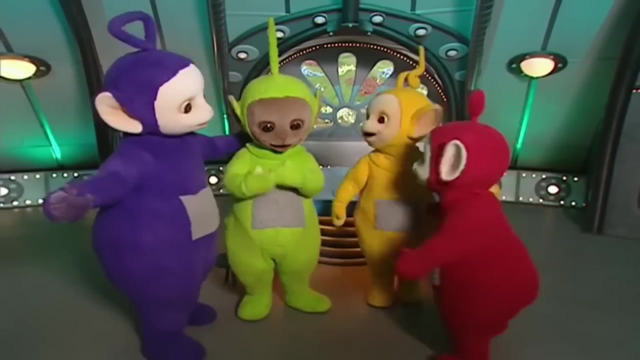 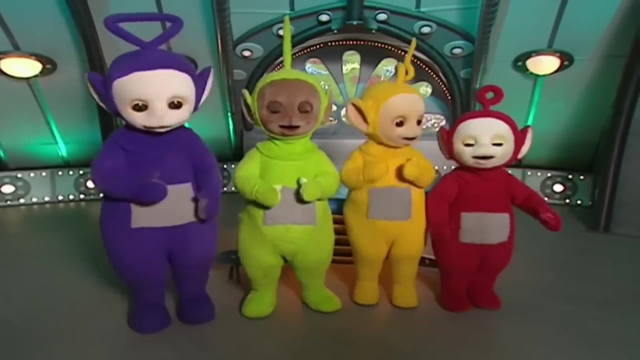 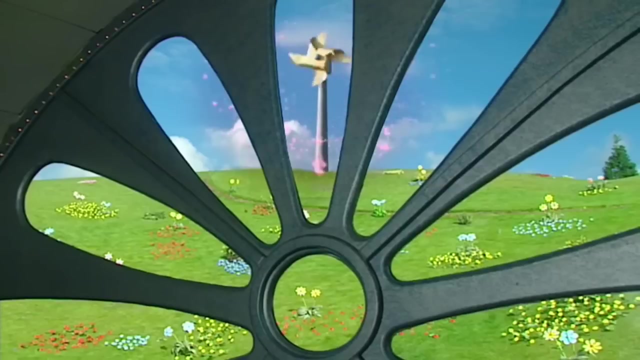 Not hungry anymore, Hungry anymore, Hungry anymore, Not hungry anymore, Not hungry anymore. How can you move? I'm hungry, I'm hungry, I'm hungry. I can't move. Big hug, Aww, Uh-oh. 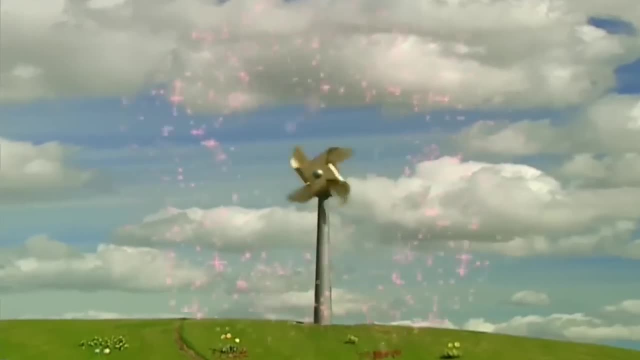 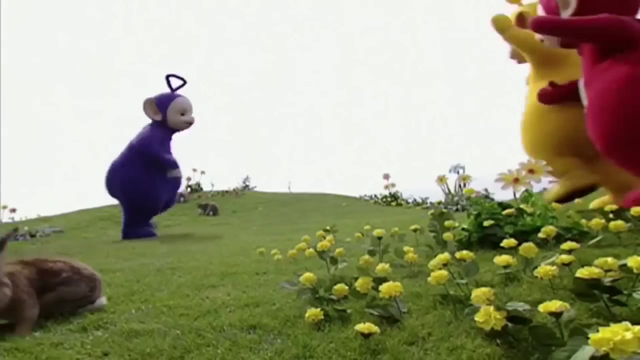 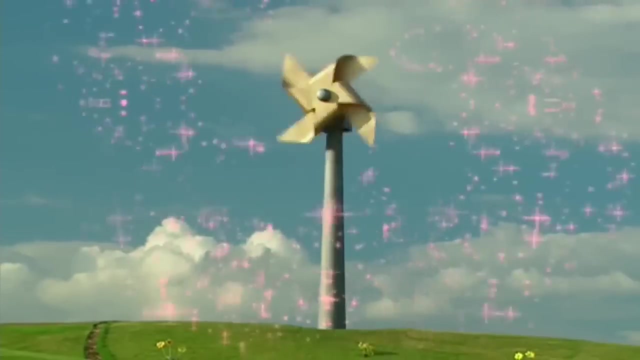 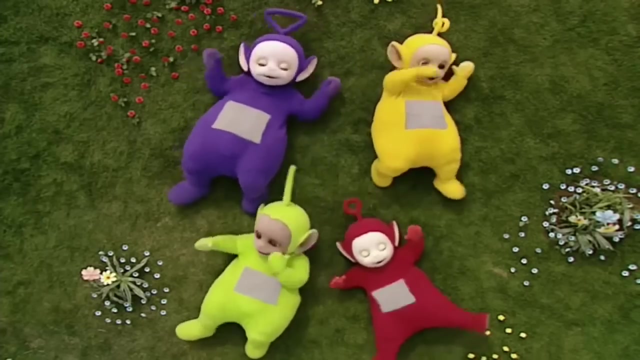 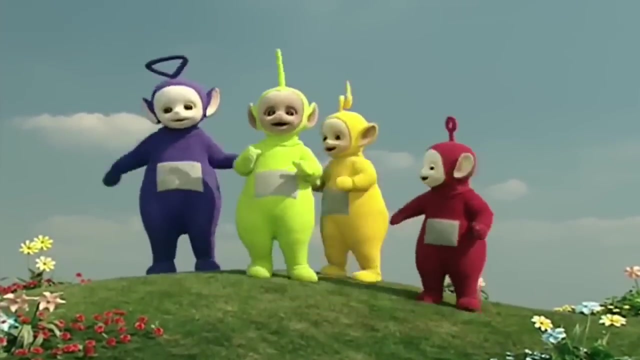 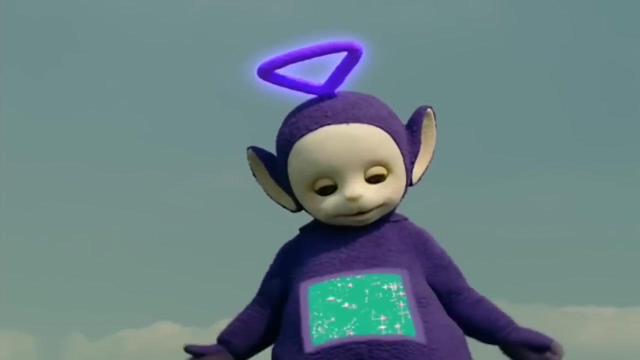 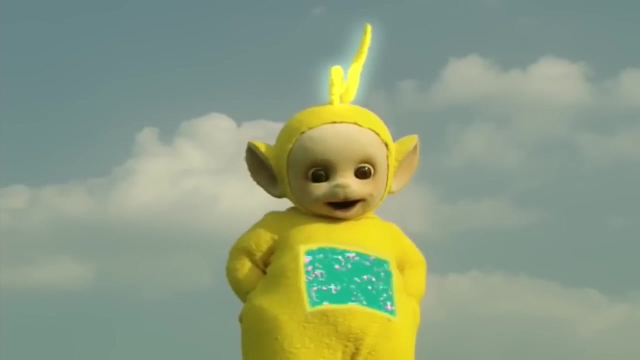 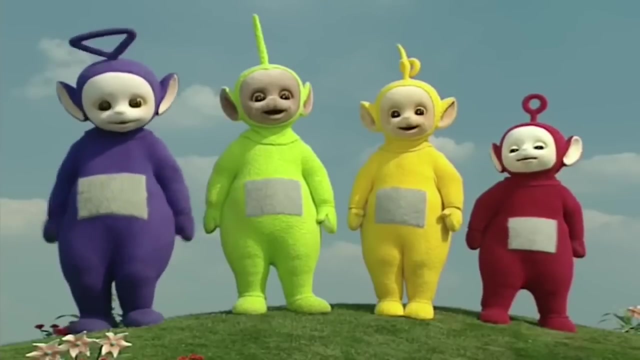 WOW, Wow. What is that? Oh, Oh, selecting, Wow, Oh, practiced Celebrating. Yeah, That's what it's all about. This is it? Tiki-wiki? Dipsy Yalla Hi. 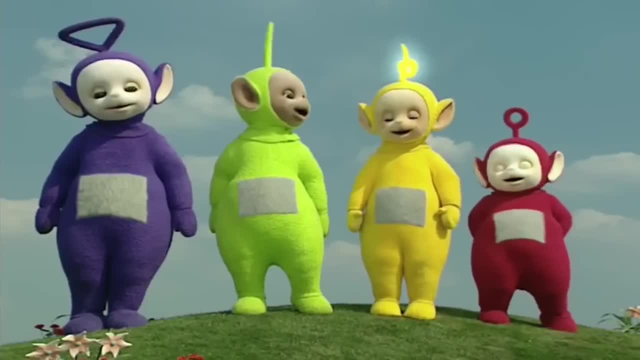 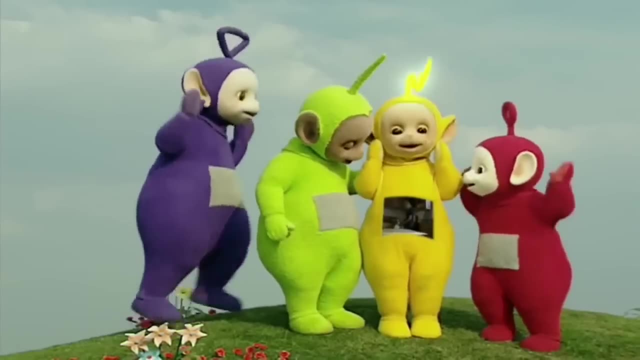 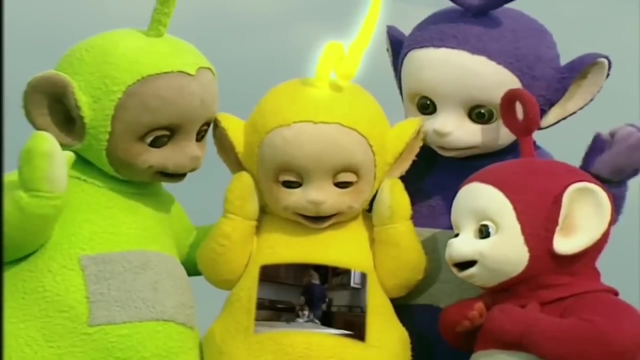 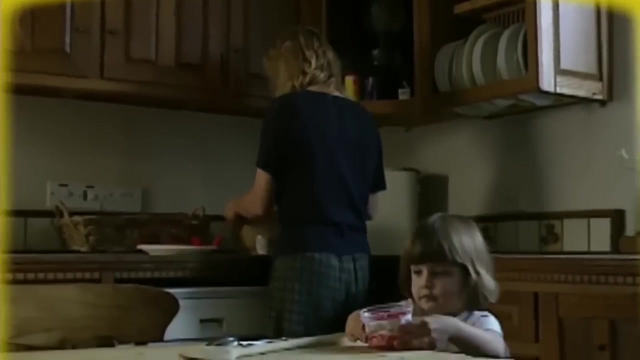 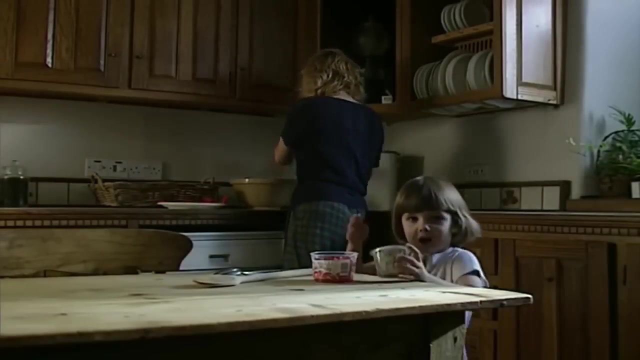 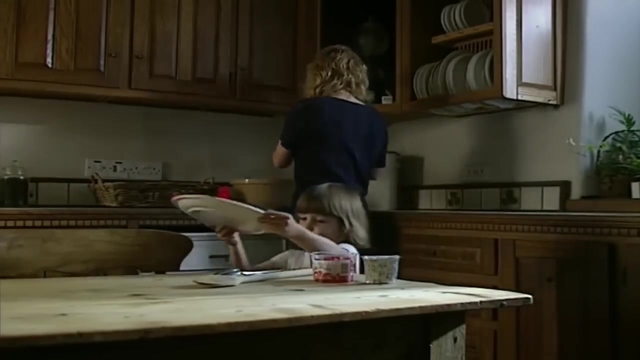 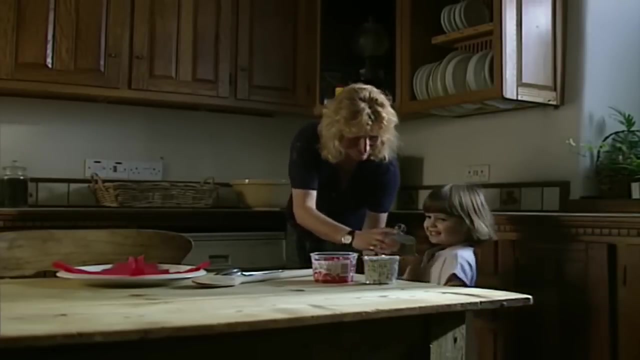 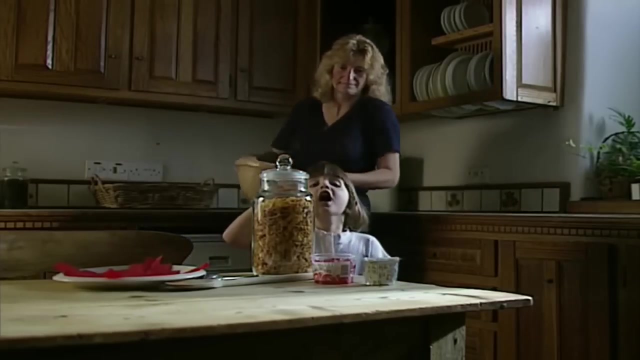 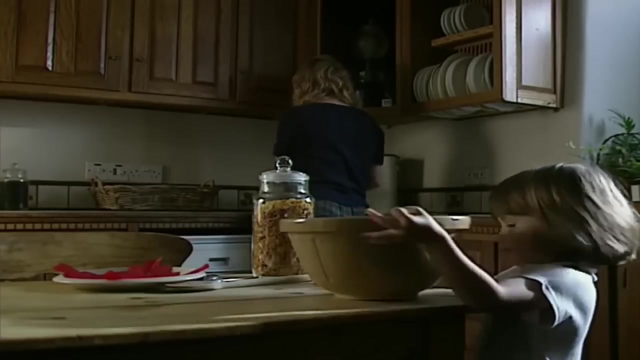 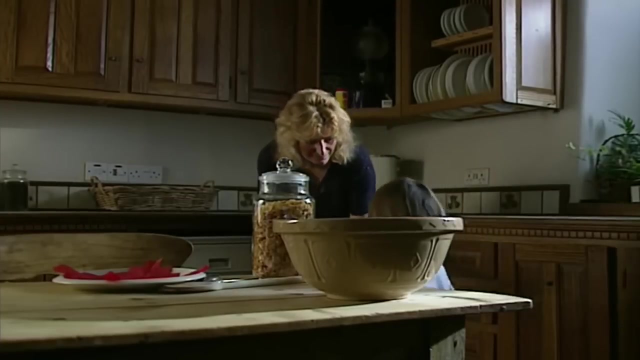 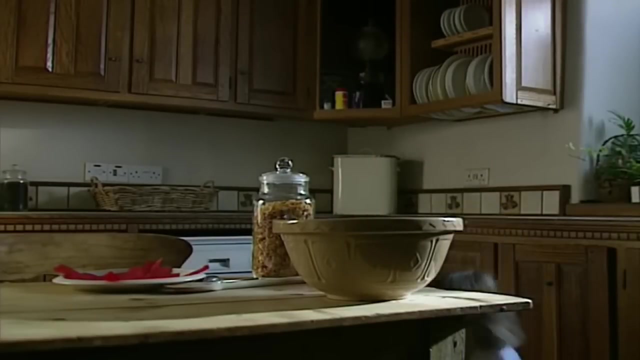 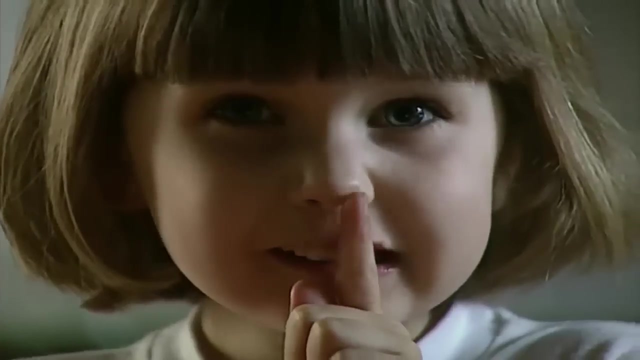 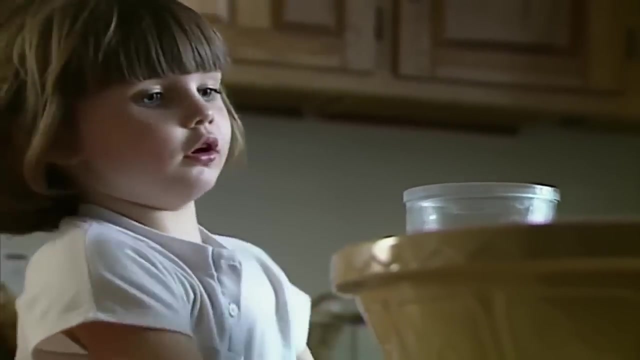 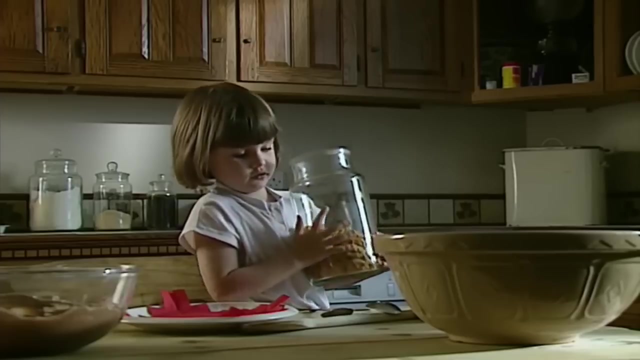 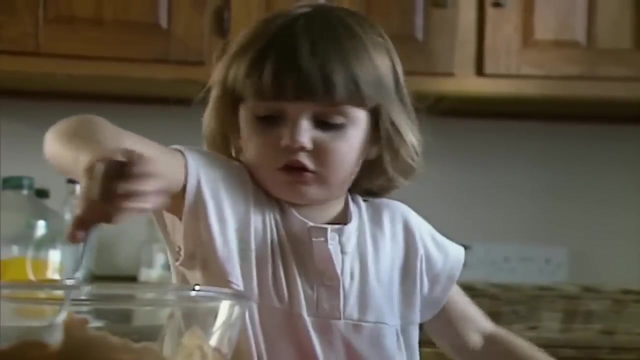 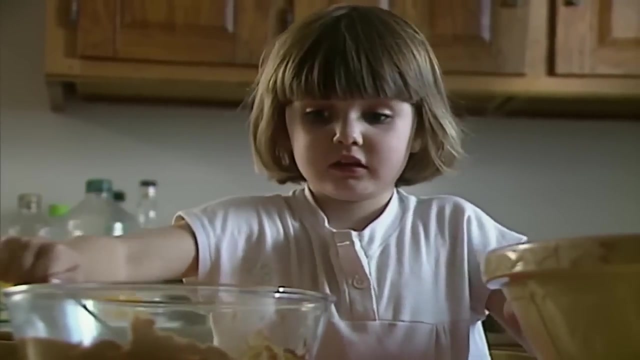 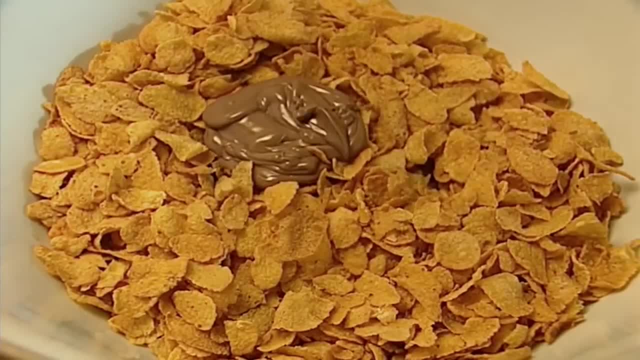 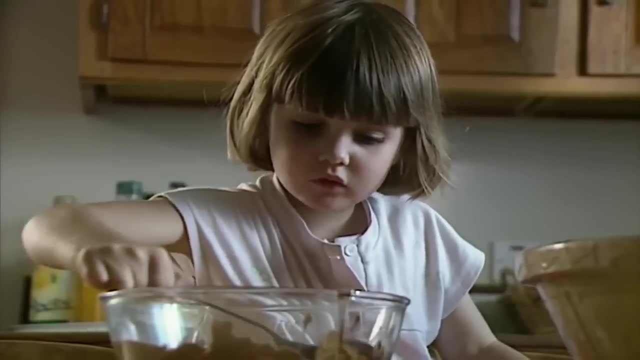 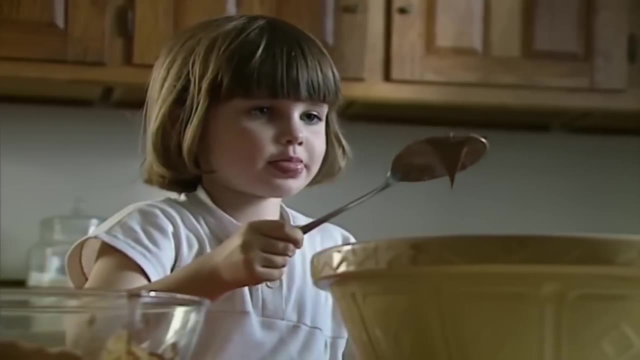 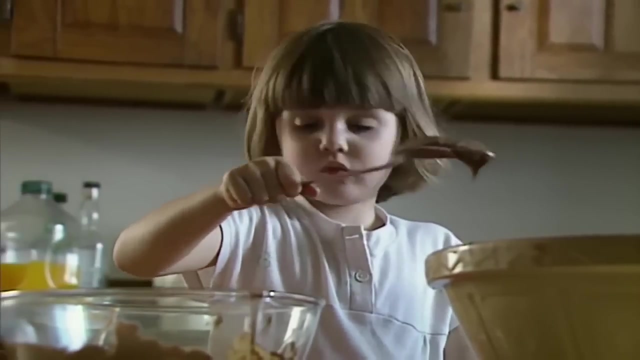 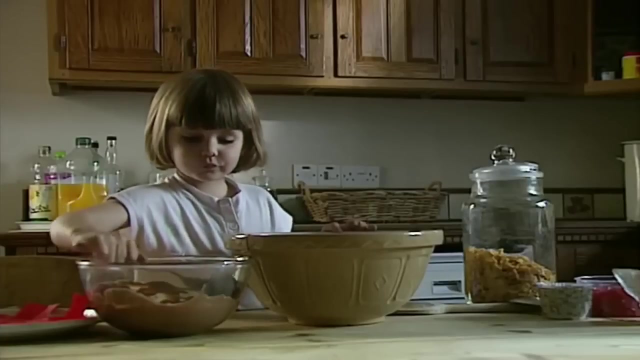 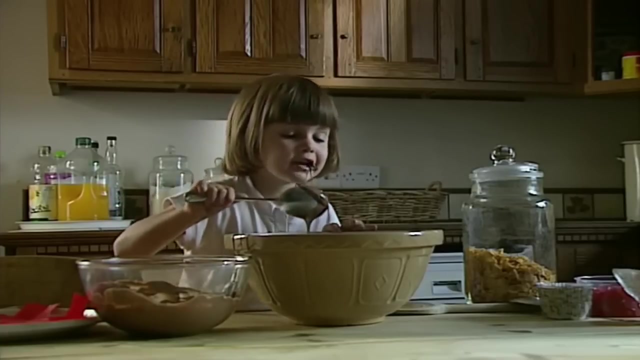 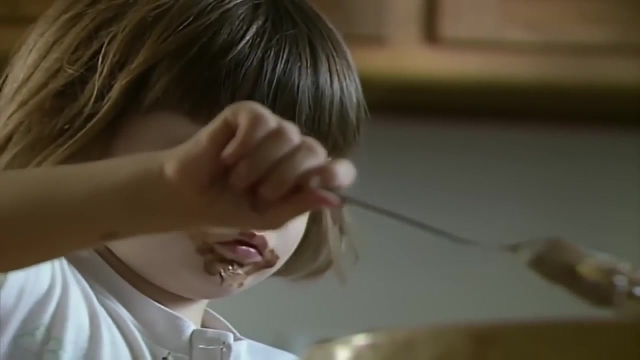 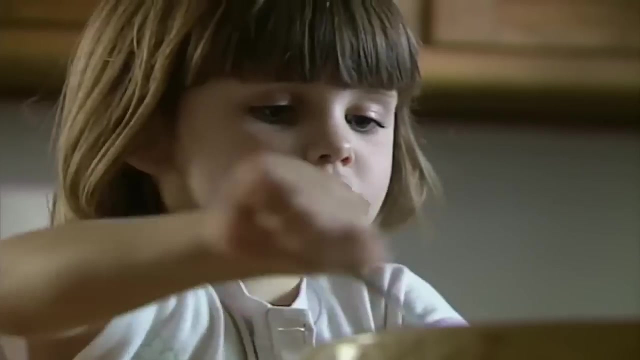 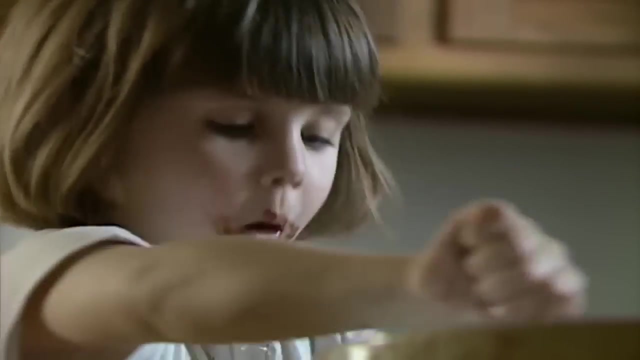 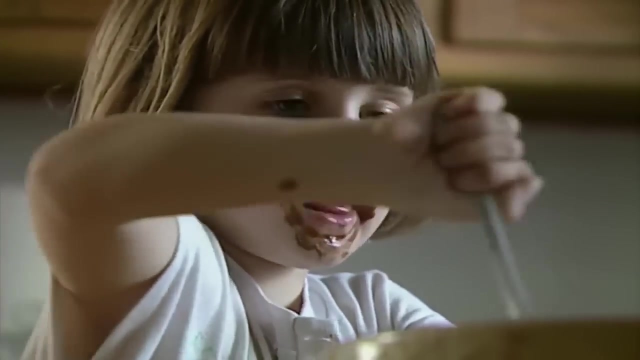 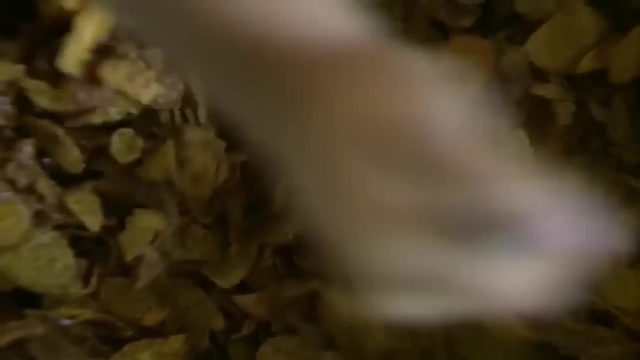 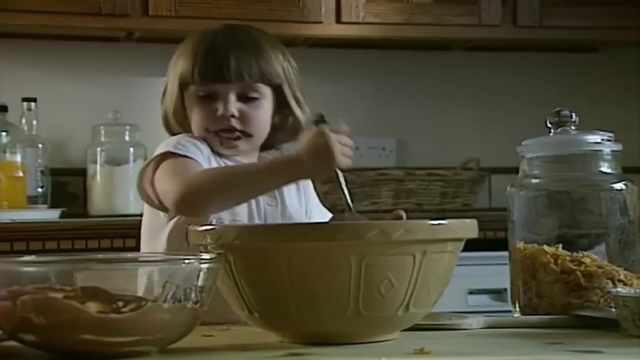 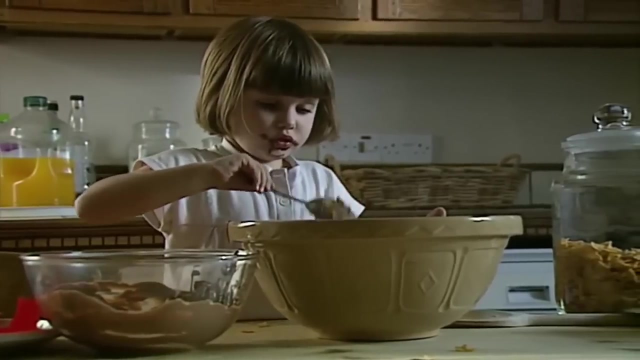 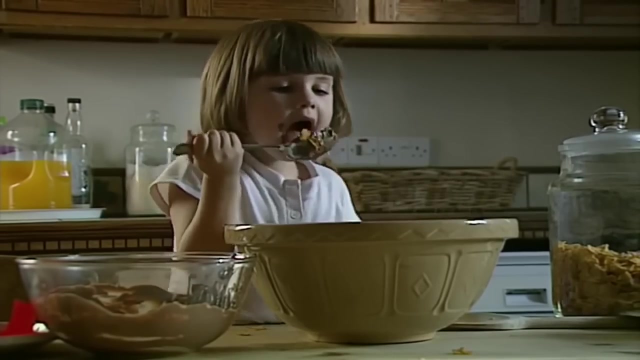 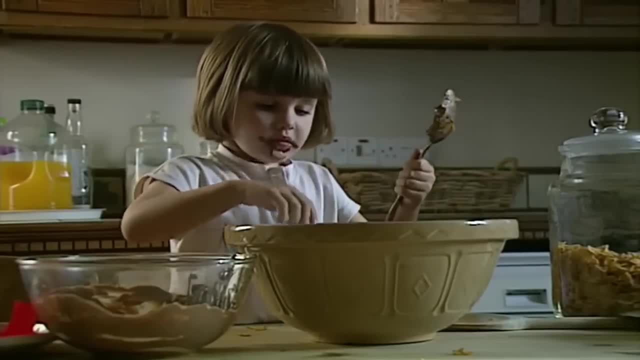 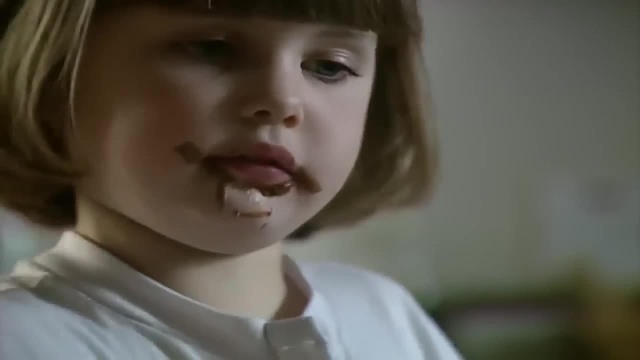 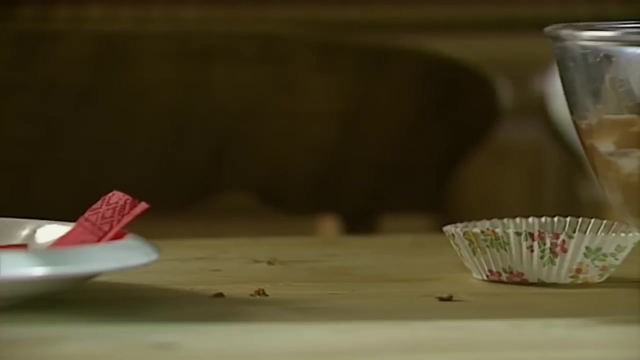 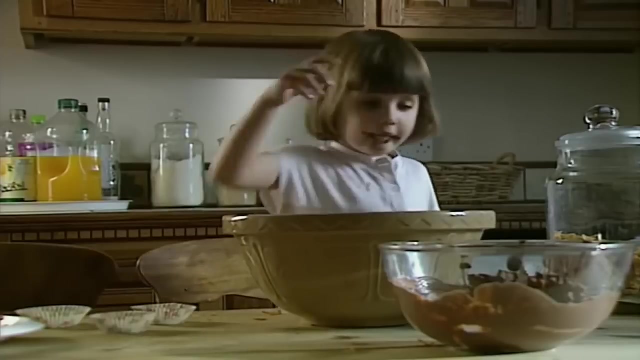 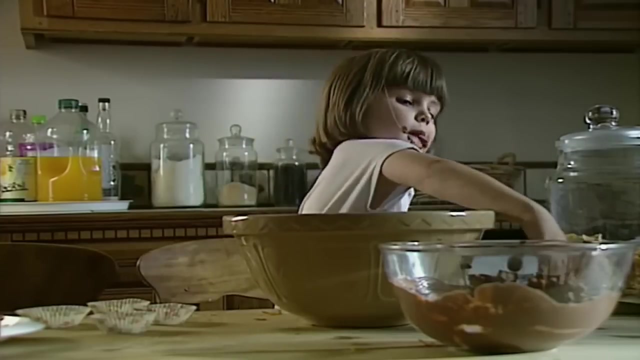 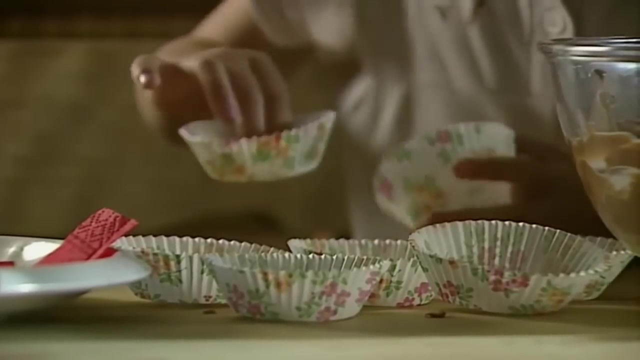 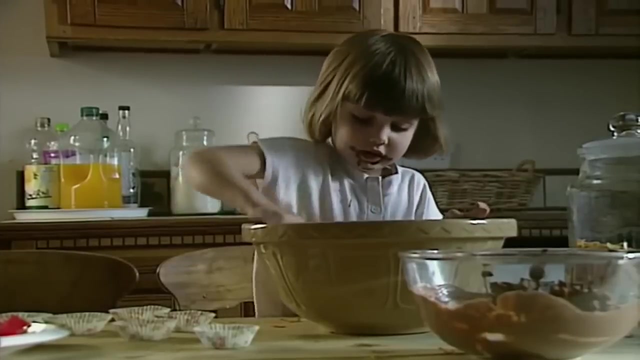 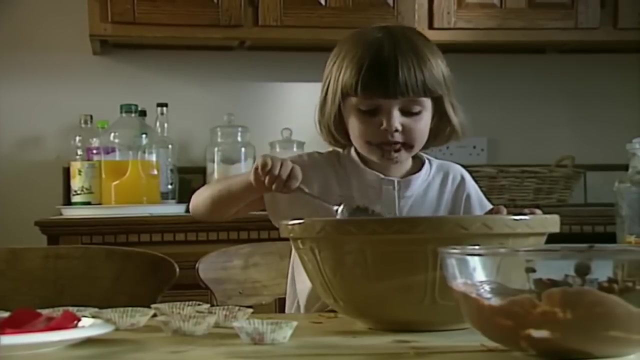 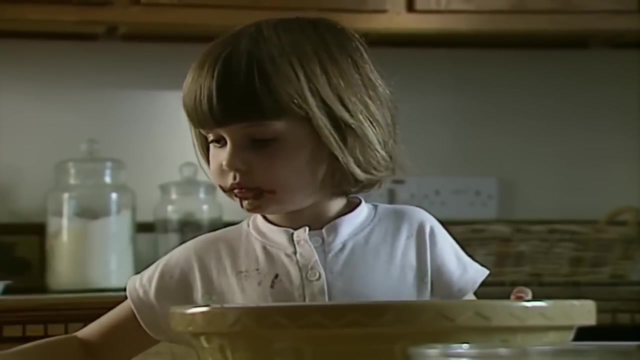 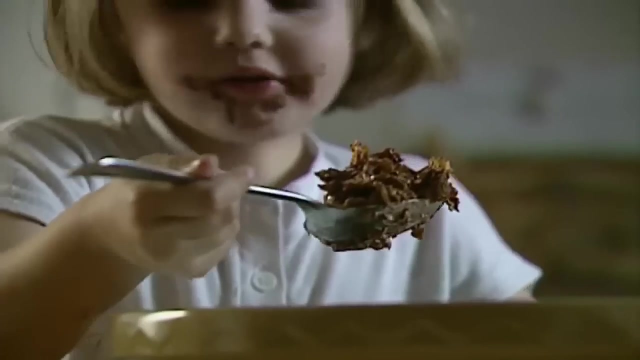 All of it's covered, Or What? Two, Three, Five, Three, four, Five, Six, Seven, Seven I티м clutch. That looks good. Yay, Yeah, I wanted to do it like a cake. 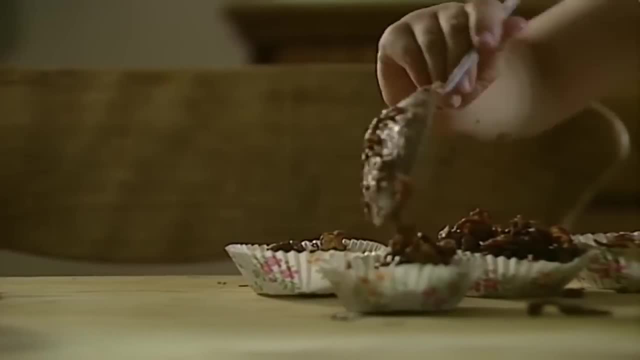 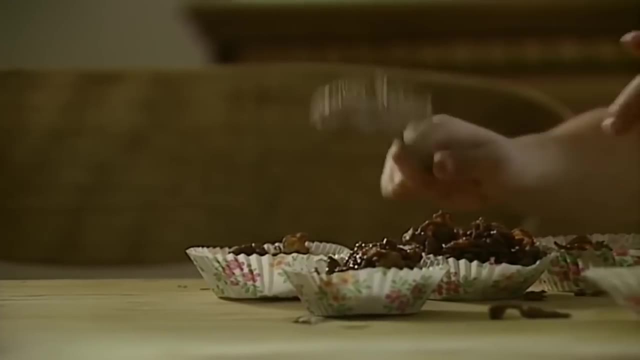 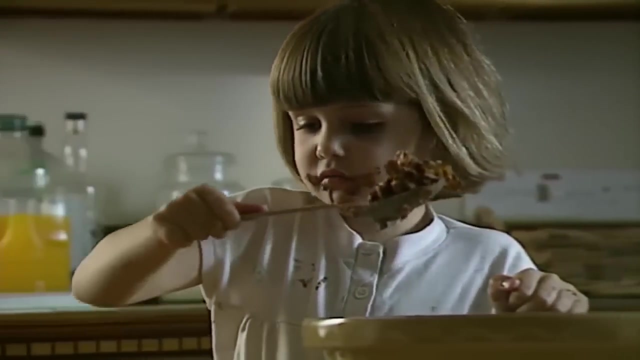 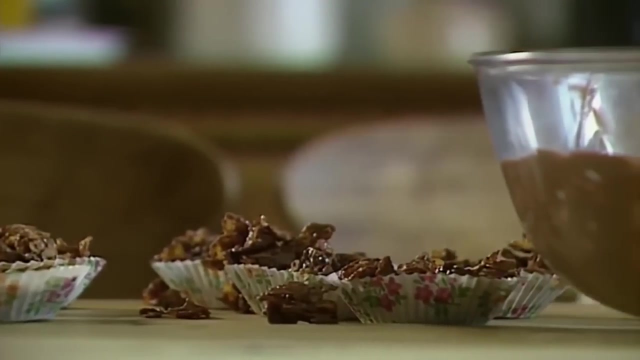 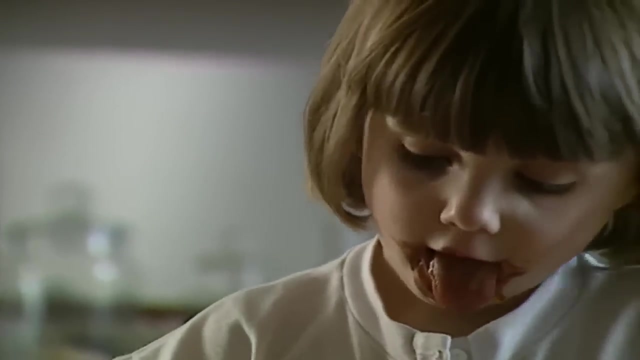 It's all good, This is all the cake. Eww, What's that? Eww, Mark's going to be very pleased. It's a good surprise. Now, this is the last one There. Now I'm going to do Timmy's. 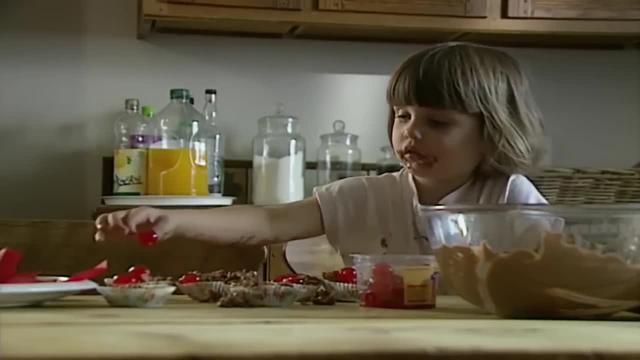 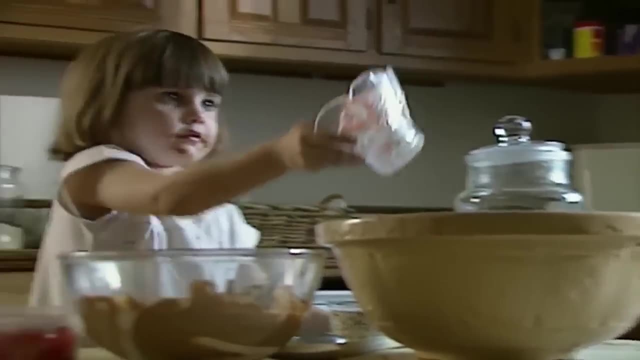 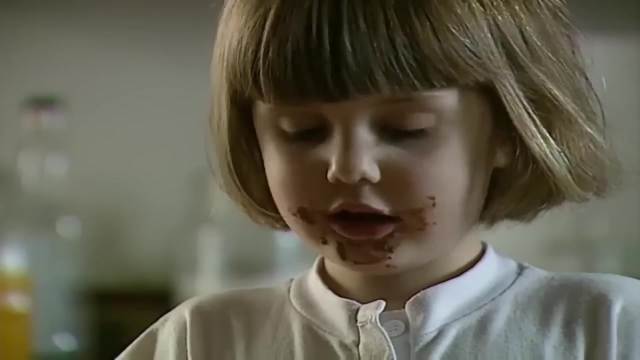 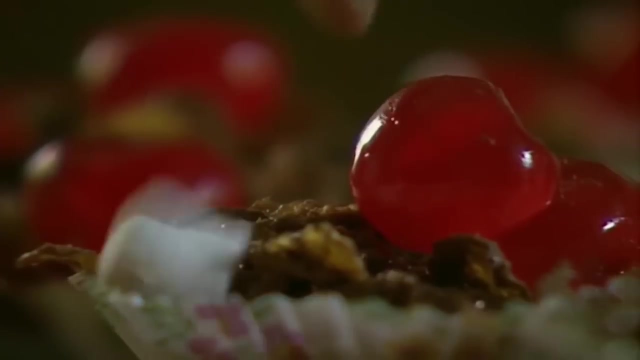 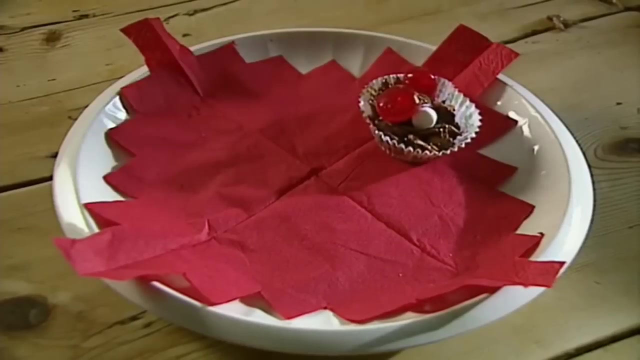 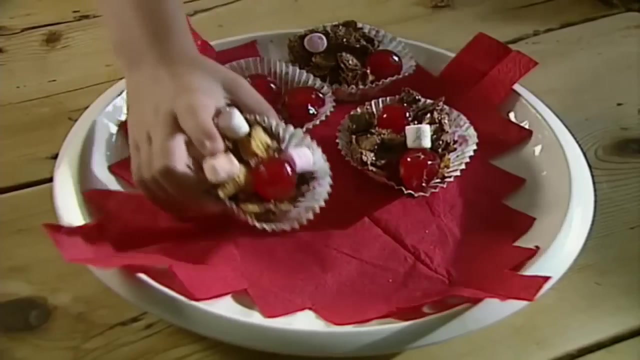 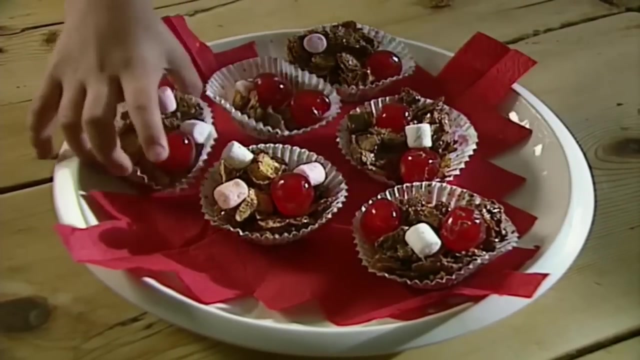 I love marshmallows and they look pretty on my cakes. I know Mark's going to like these. He likes marshmallows. I think I give him another one There. One, two, three, four, five, six and seven. 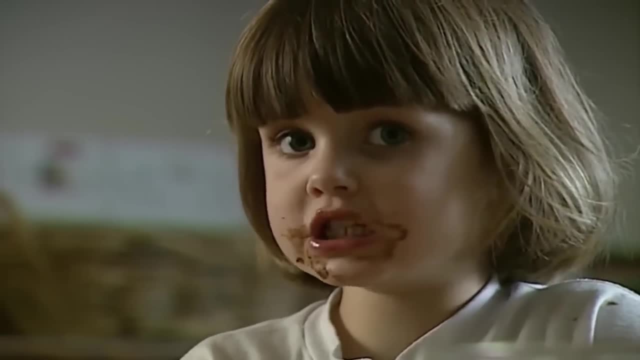 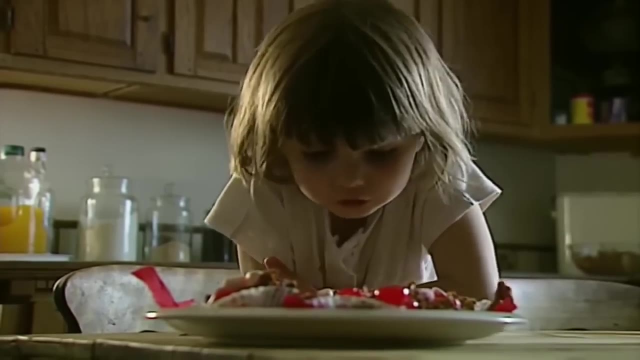 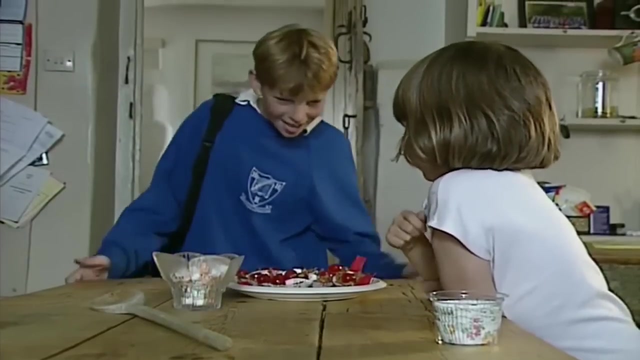 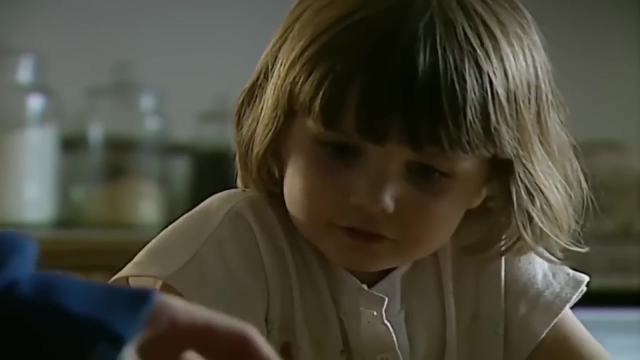 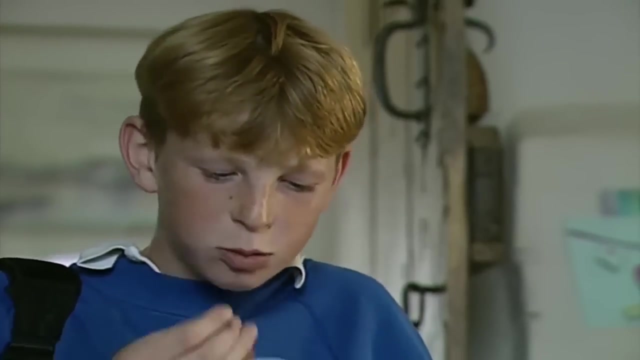 Mark will be very pleased with those. I wonder which one he picks. Hi Cool, Who made those Me? Am I allowed one? Of course you can. I made them for you, Cool Thanks, Becky. I'm going to have one too. 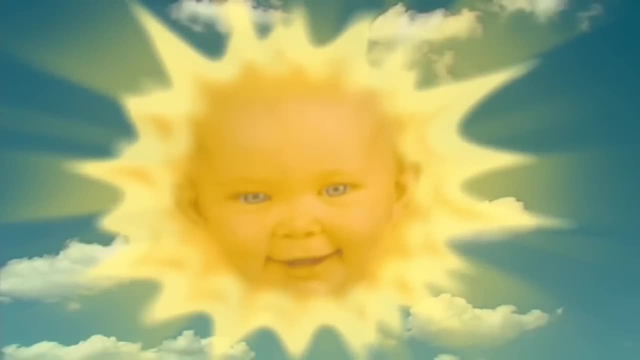 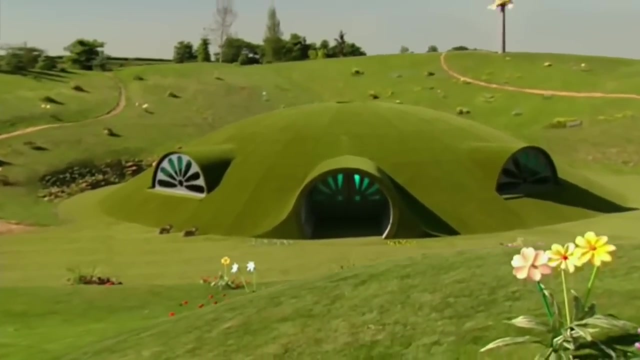 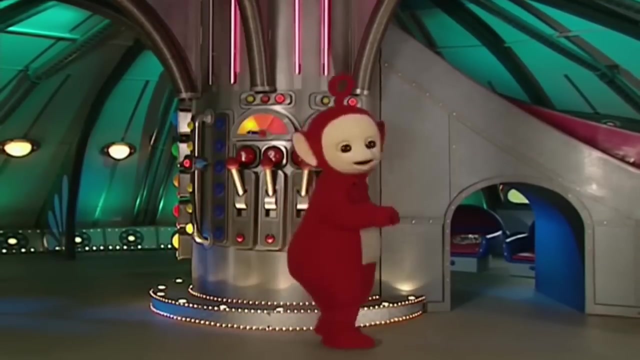 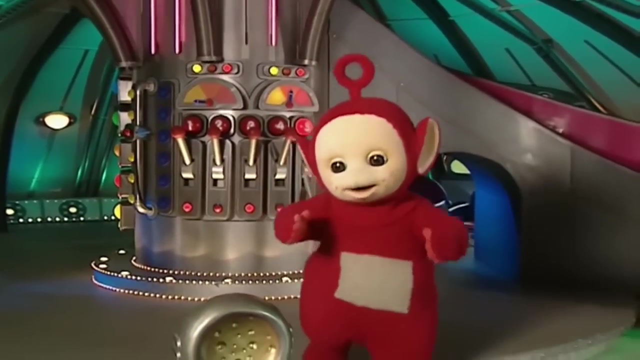 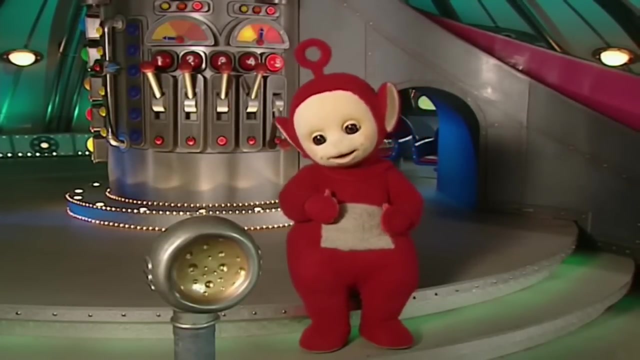 Bye-bye, bye-bye, Pat-a-cake, pat-a-cake baker's man, bake me a cake as fast as you can. Pat it and prick it and mark it with B, Put it in the oven for baby and me. 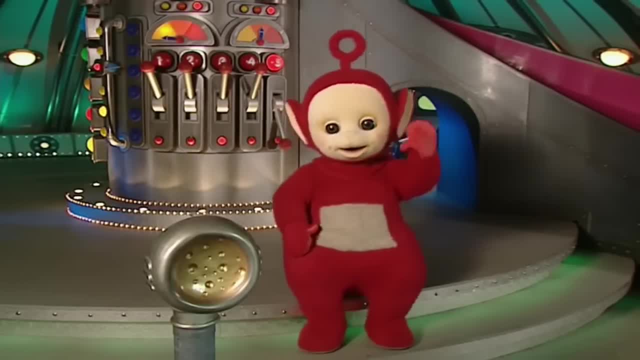 Again, again, again, Pat-a-cake. pat-a-cake baker's man, bake me a cake as fast as you can. Pat it and prick it and mark it with B, Put it in the oven for baby and me. 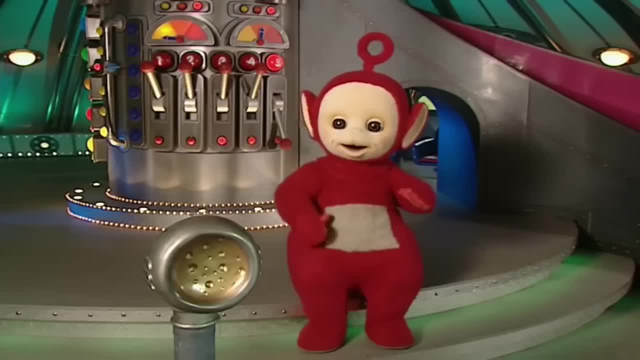 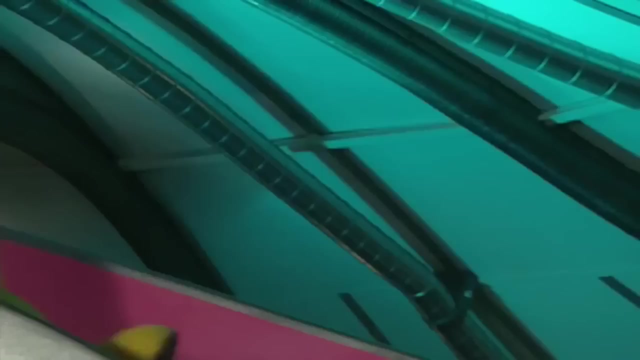 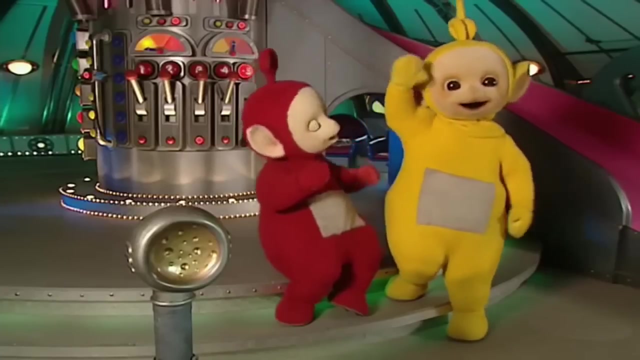 Pat-a-cake. pat-a-cake baker's man, bake me a cake as fast as you can. Pat it and prick it and mark it with B. Put it in the oven for baby and me. Eh-oh, Eh-oh Po, Eh-oh La-La. 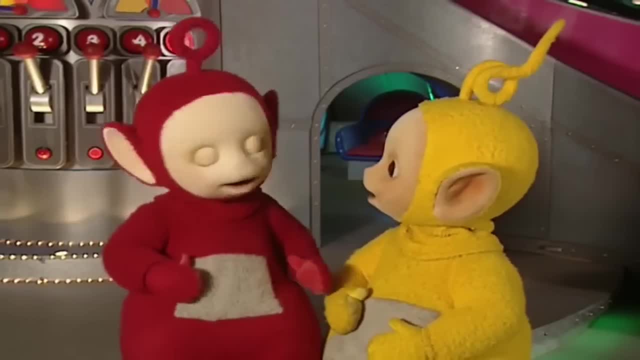 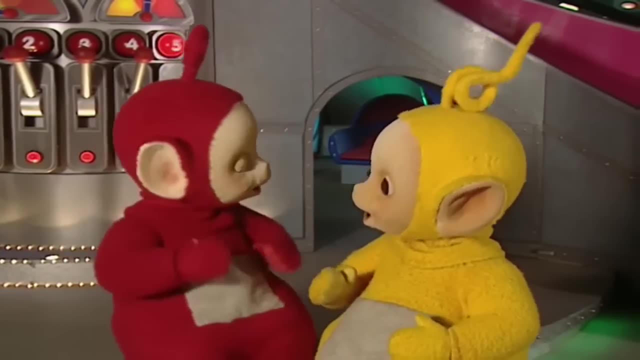 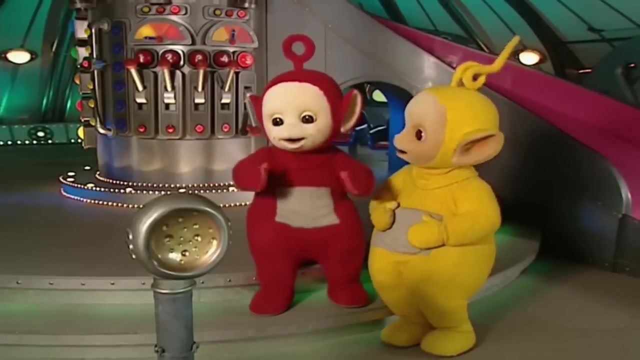 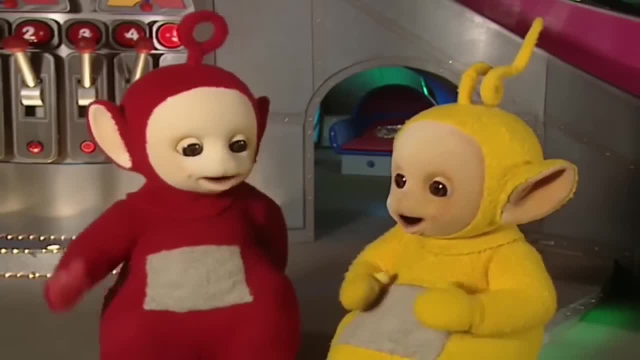 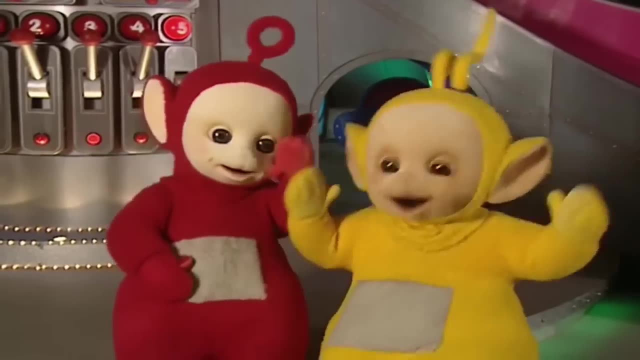 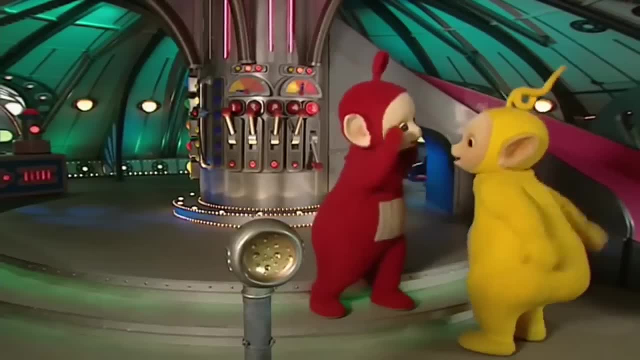 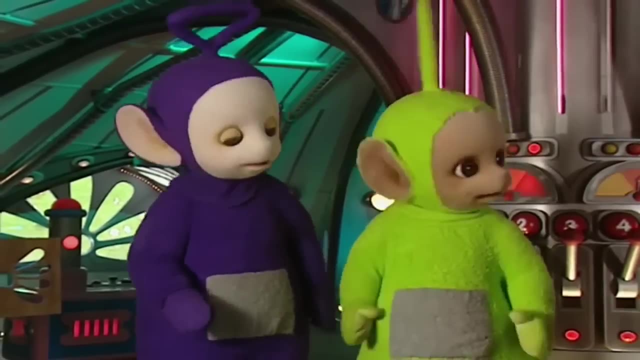 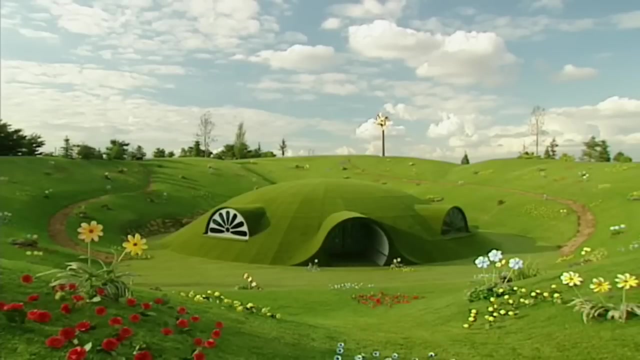 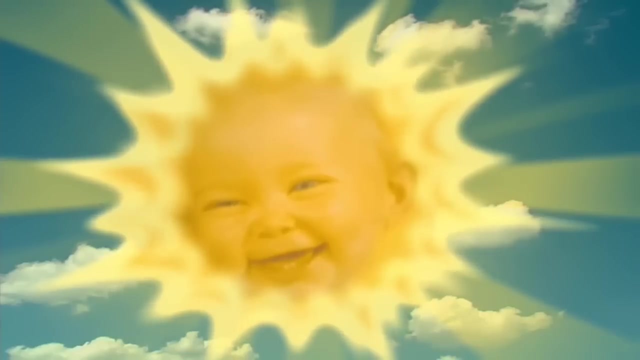 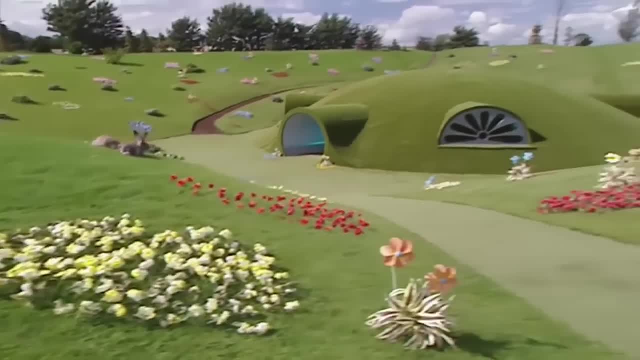 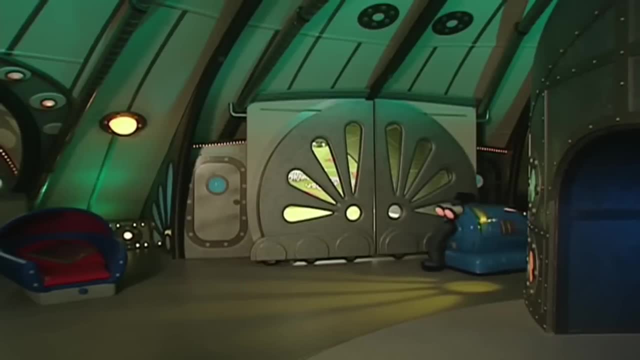 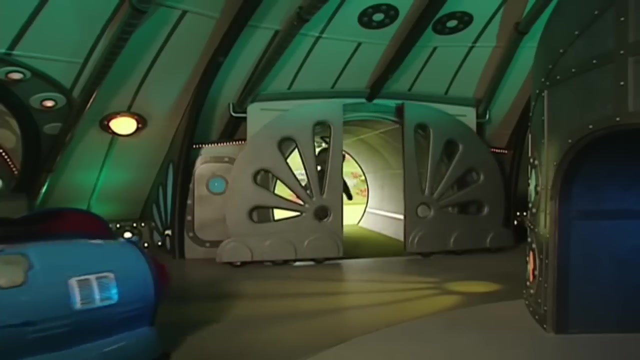 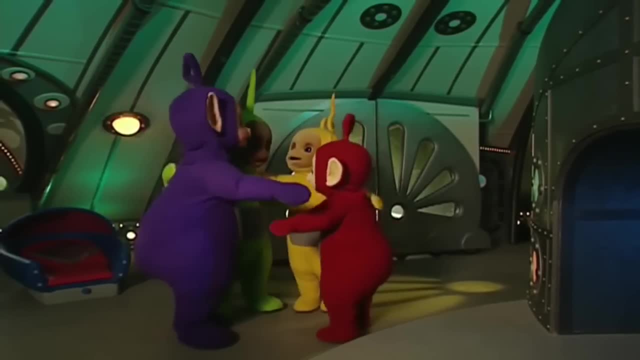 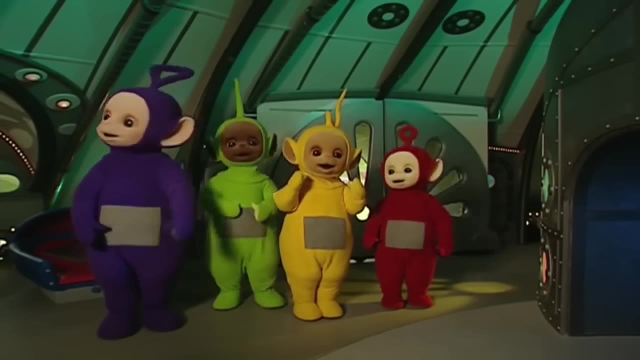 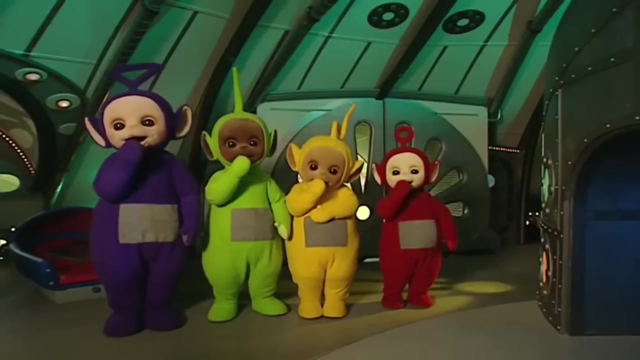 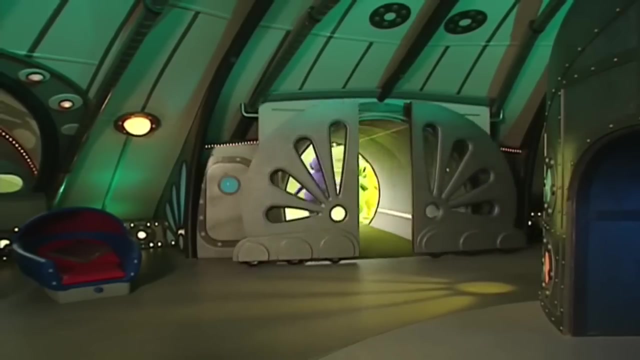 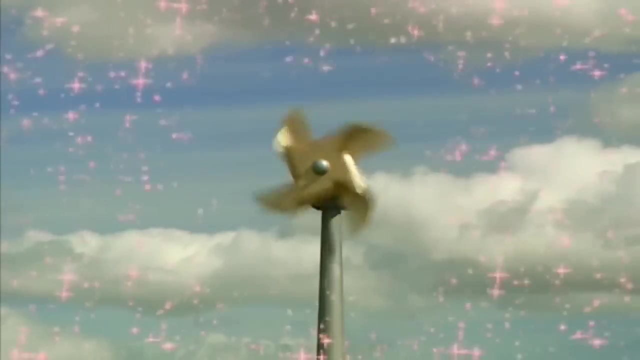 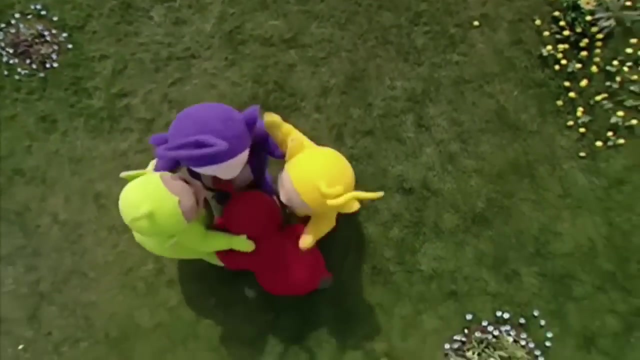 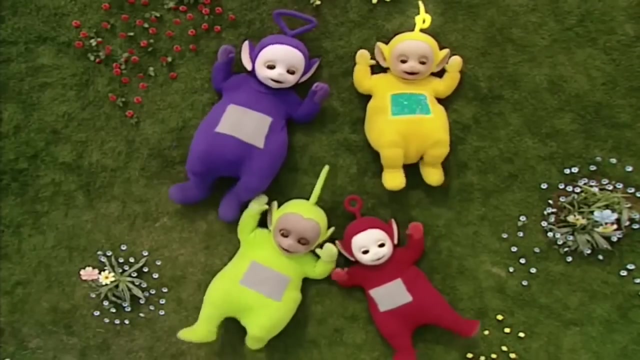 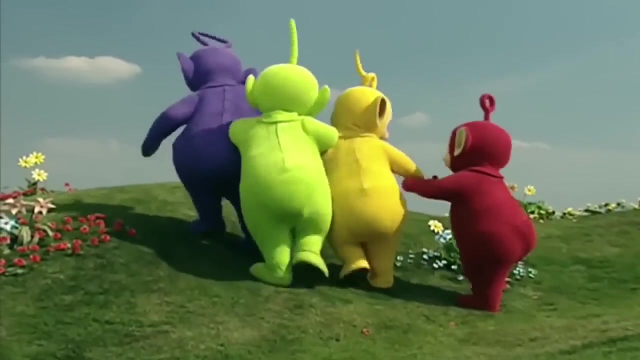 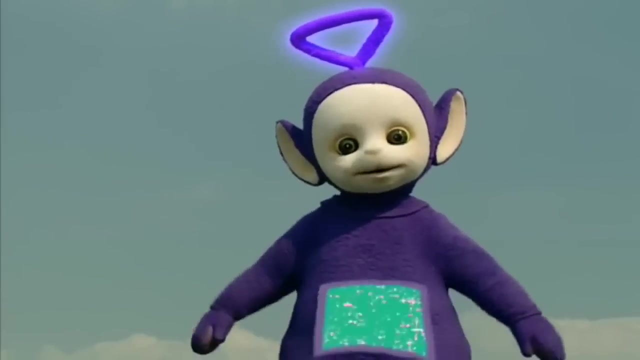 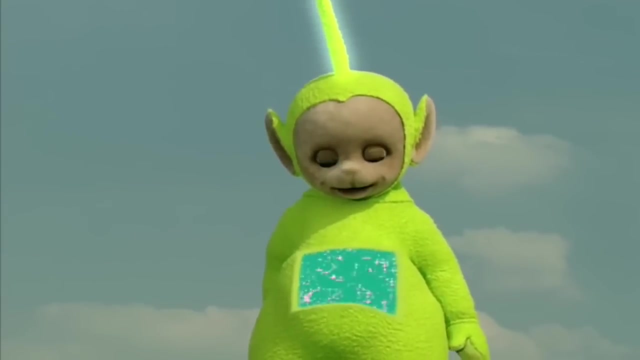 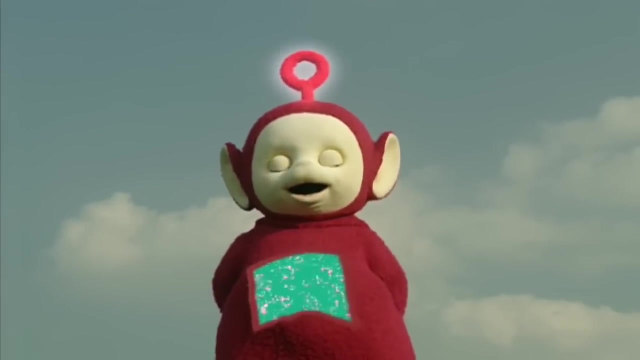 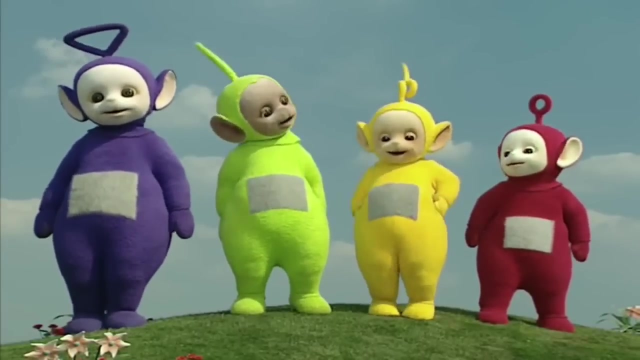 Uh-oh, Oh my God, what's going on. Oh my God, what's going on. Oh my God, Oh my God, what's going on? Tiki-wiki- Tipsy Yalla, Oh. 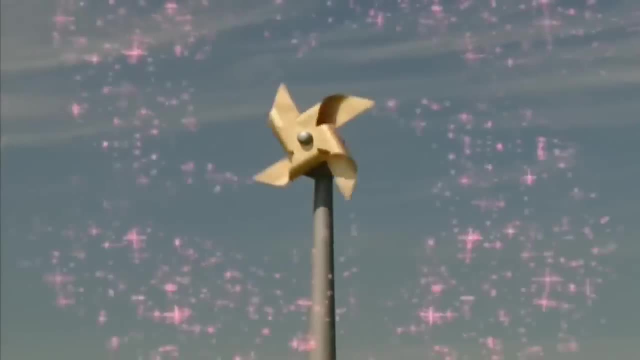 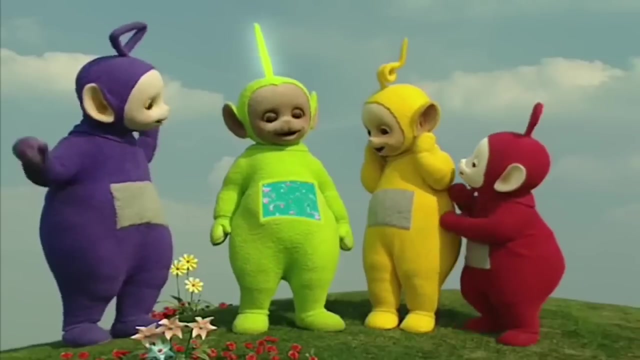 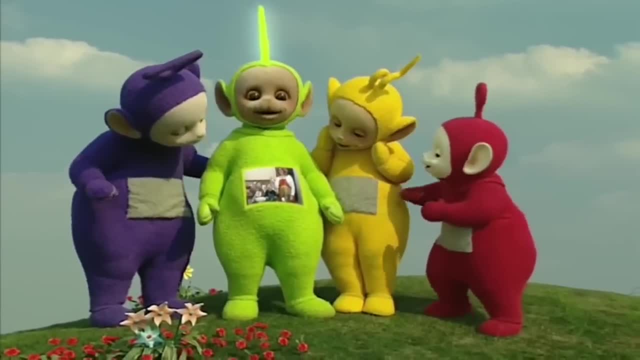 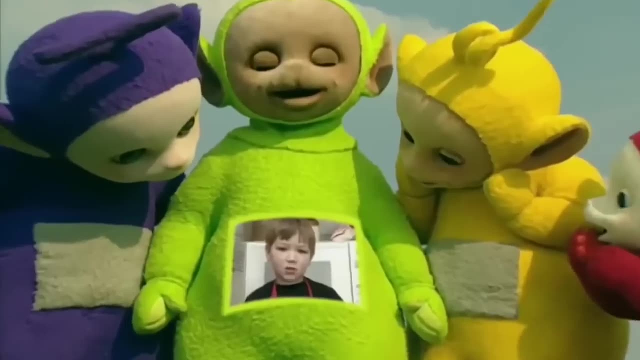 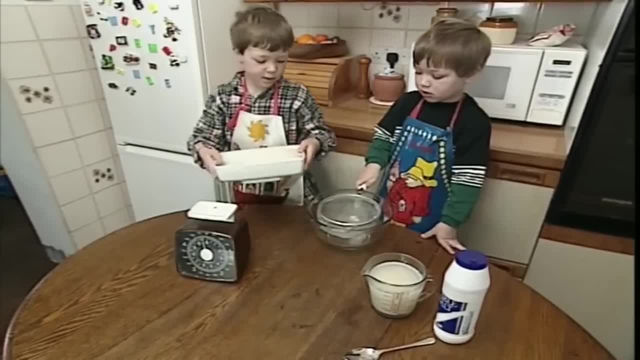 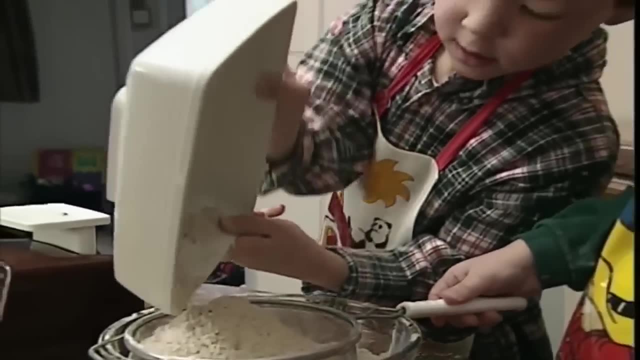 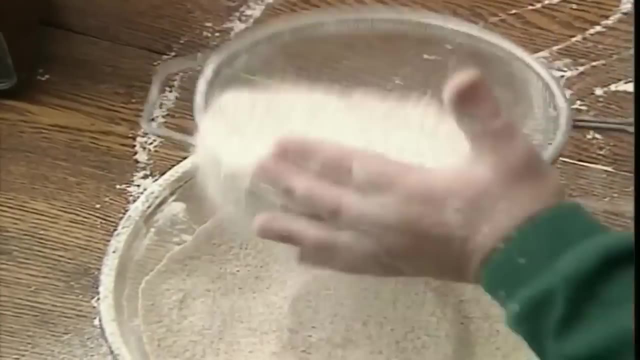 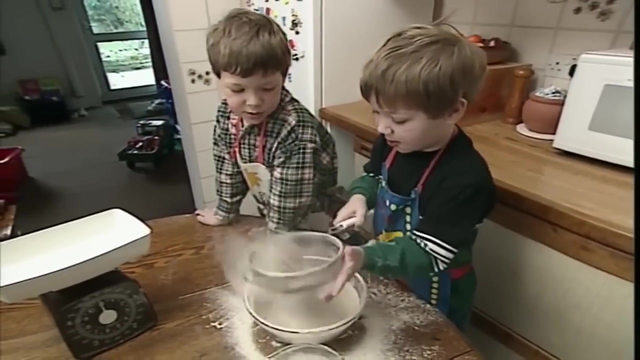 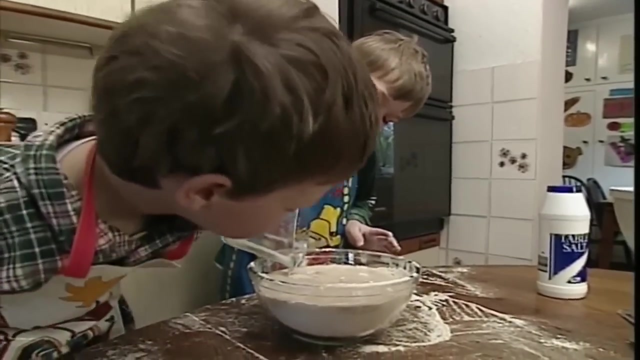 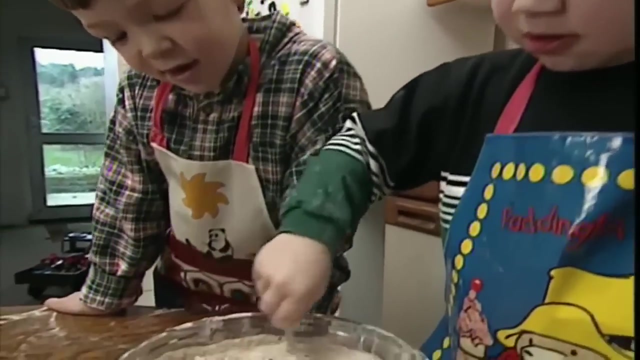 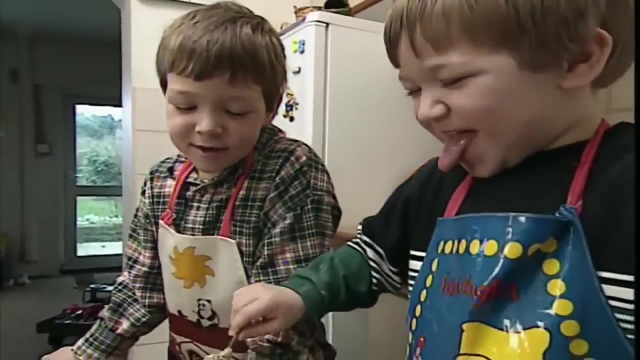 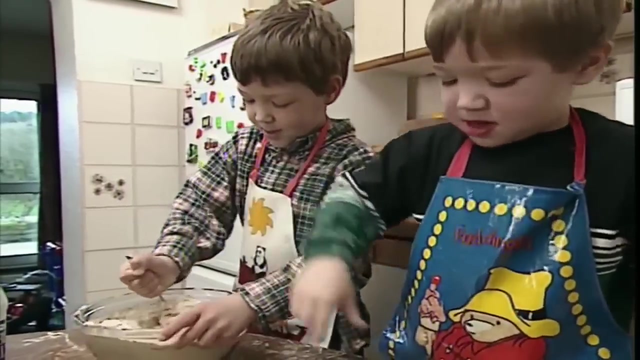 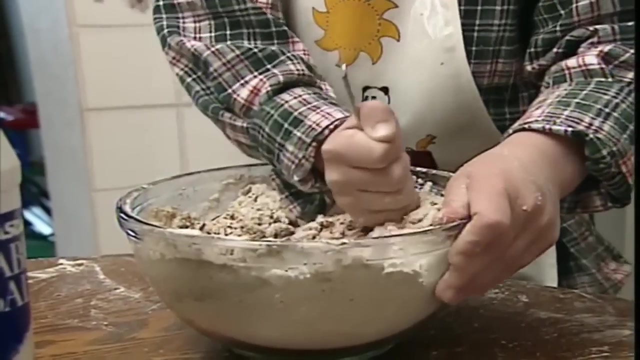 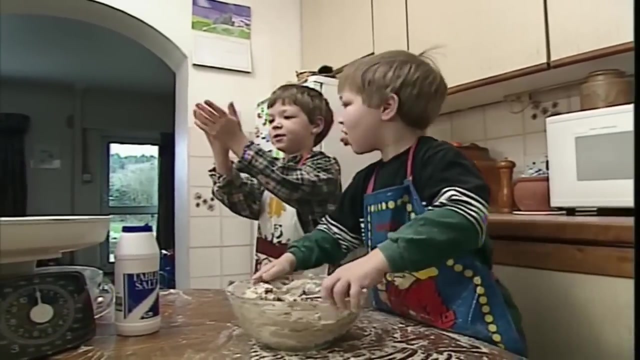 We're making bread. We're making bread. We are adding the flour into the sieve. We added the eastern water. We stir it. Don't Let me have a stir. It's really sticky And very gooey. It's really good. 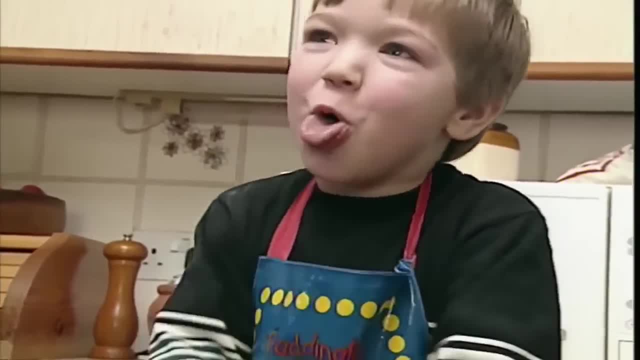 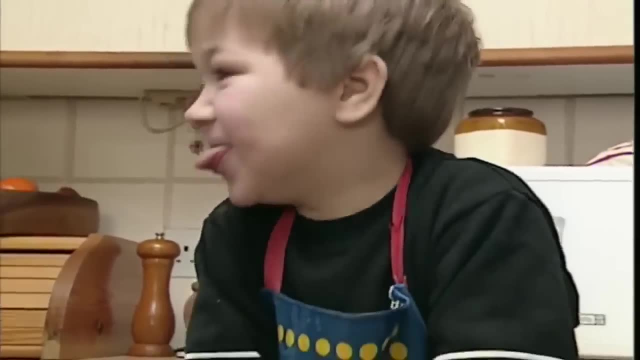 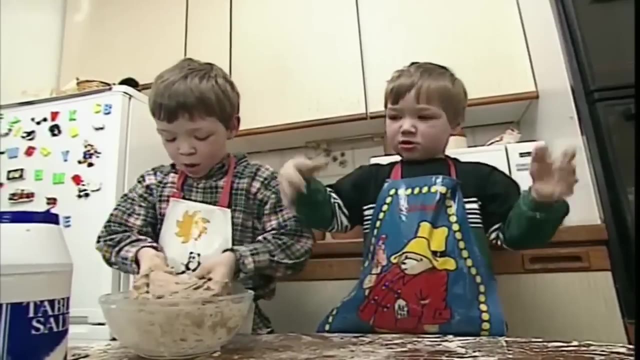 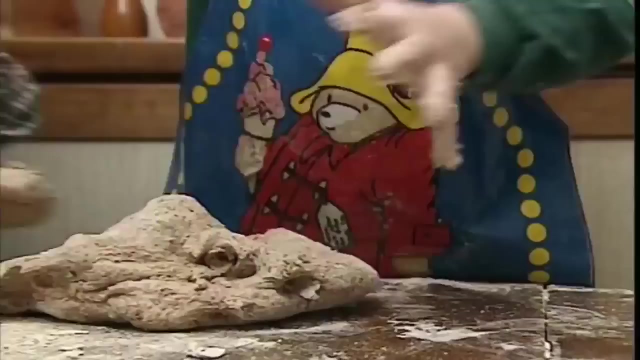 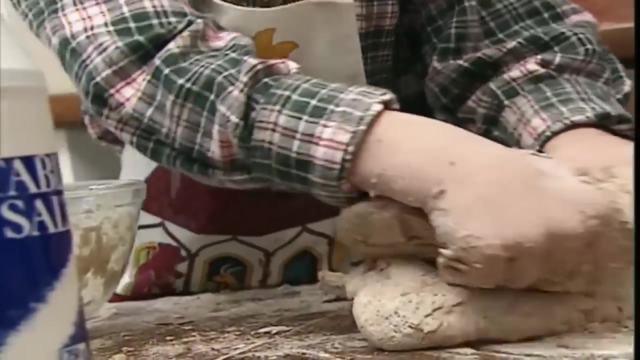 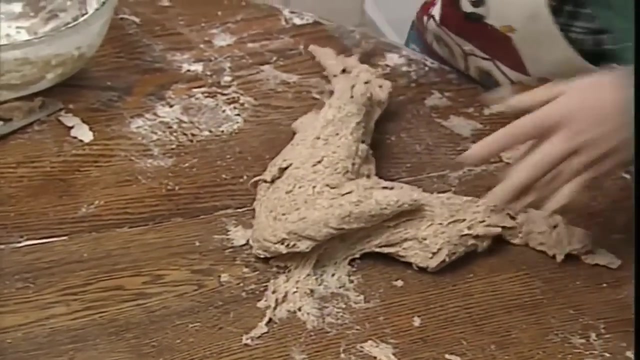 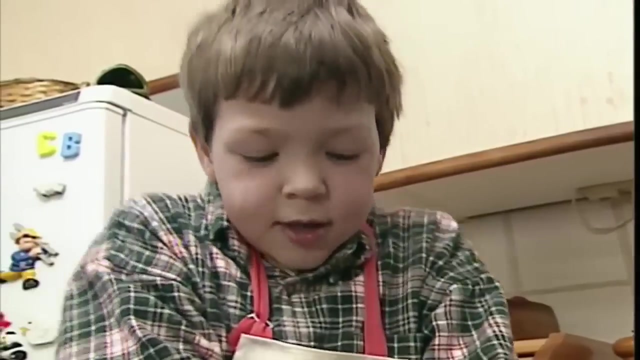 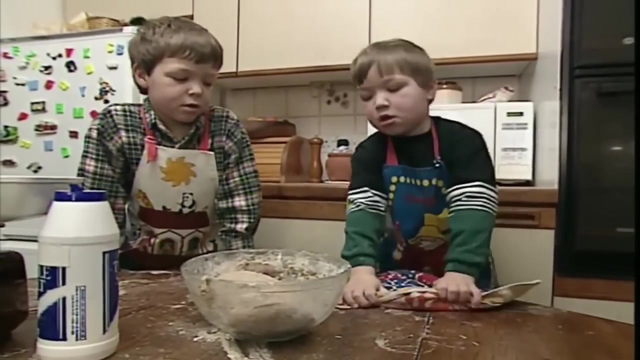 Poozy, squeezy, eww, Eww. Now we have to knead it. We need to knead it. Good day, Eww. It's so sticky, That's long. Now we knead it with a settle. 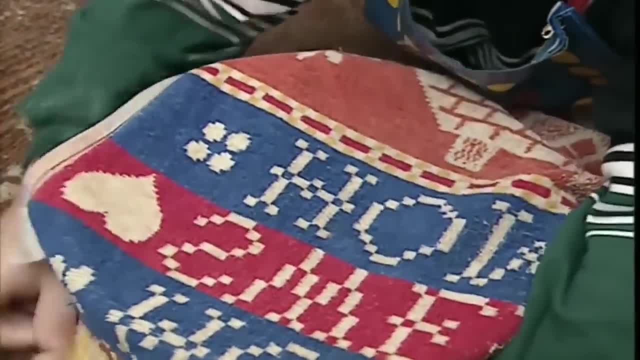 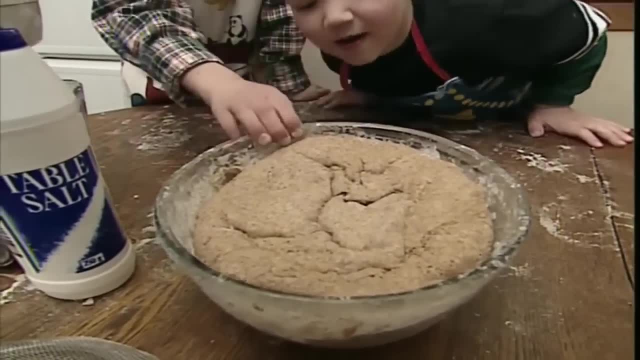 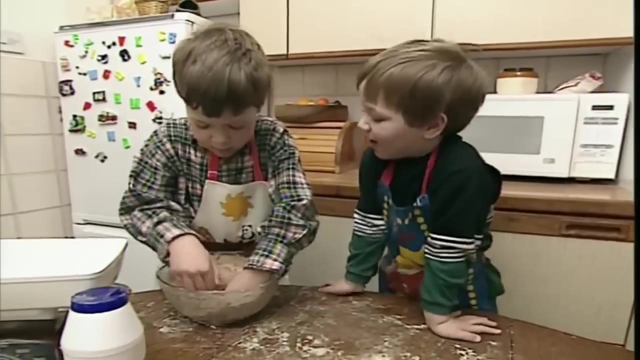 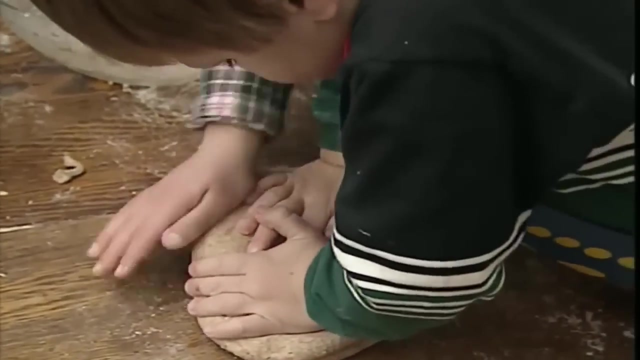 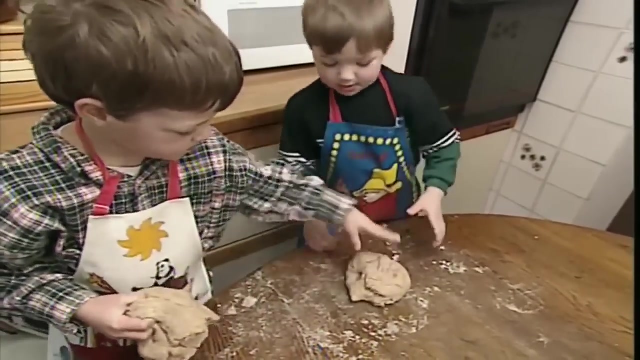 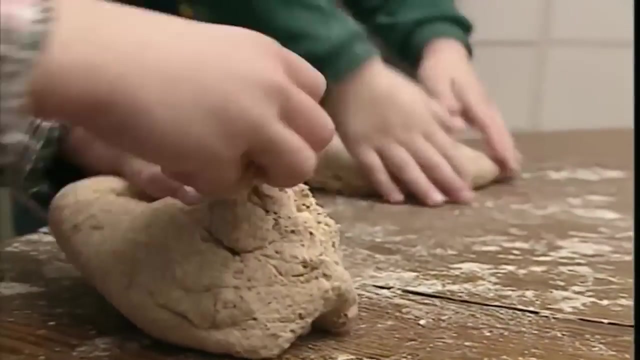 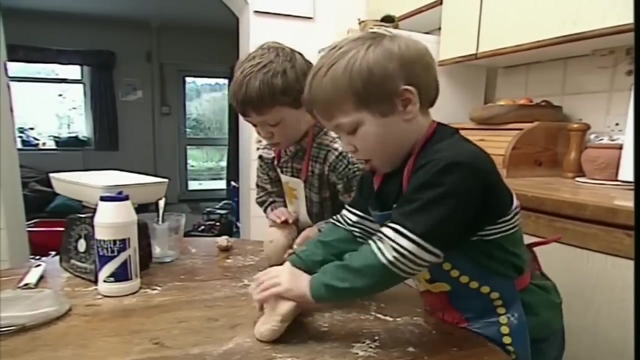 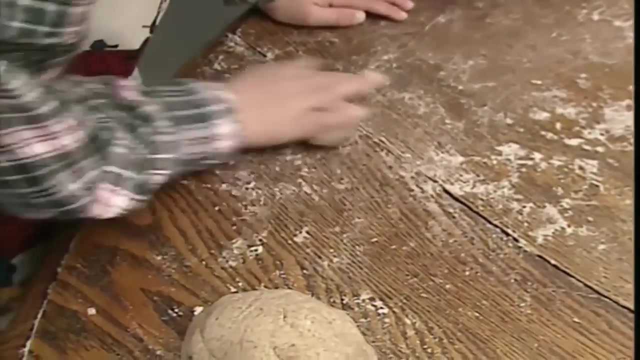 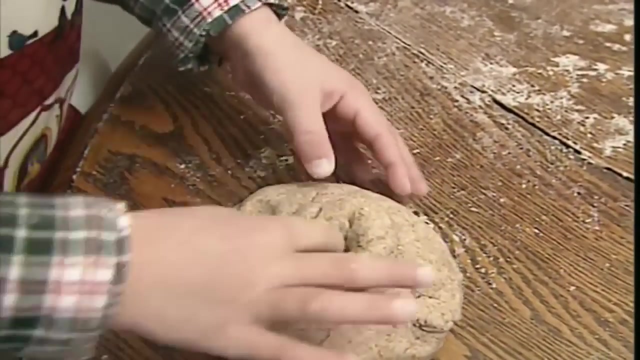 Sorry about that. That's it Now. let's look at the bread. Thomas gets it out the bowl And we have to knead it again, And we have to knead it again. We're making bread rolls There, Finished. 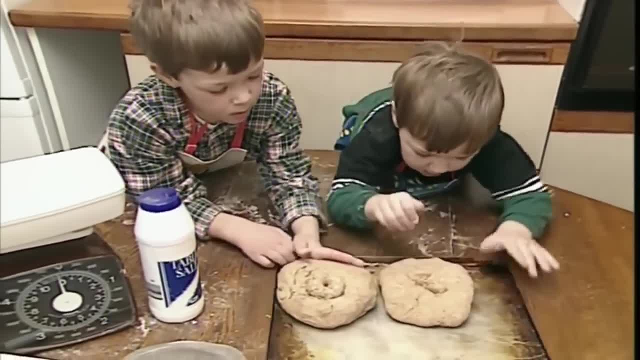 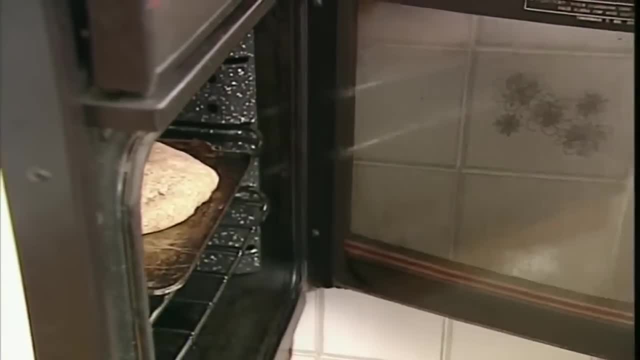 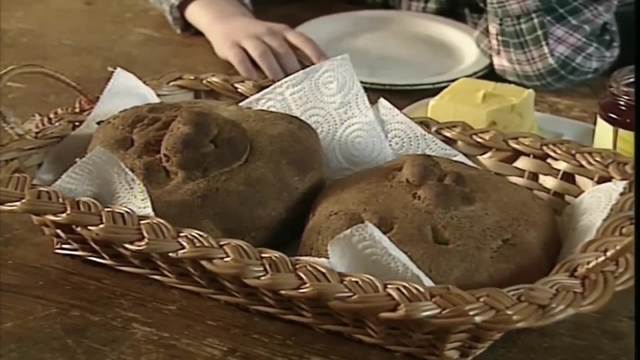 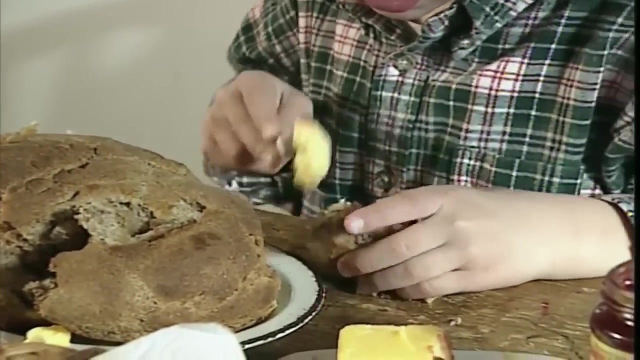 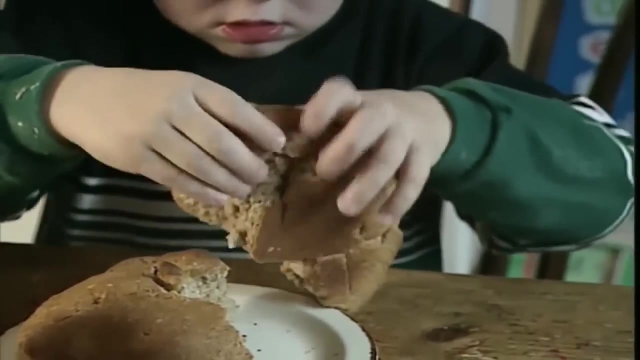 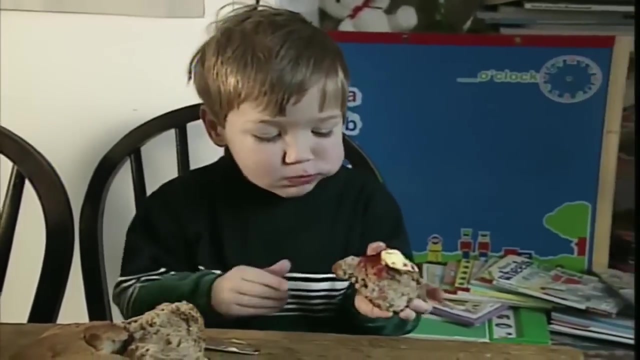 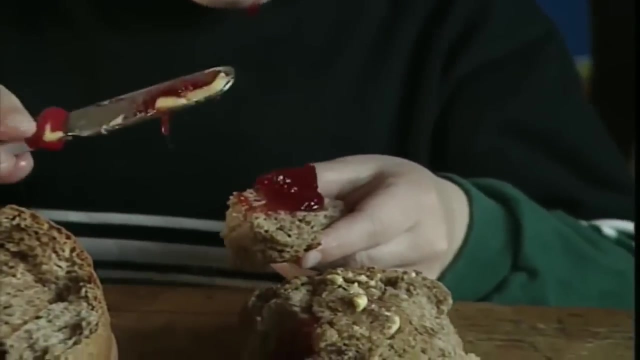 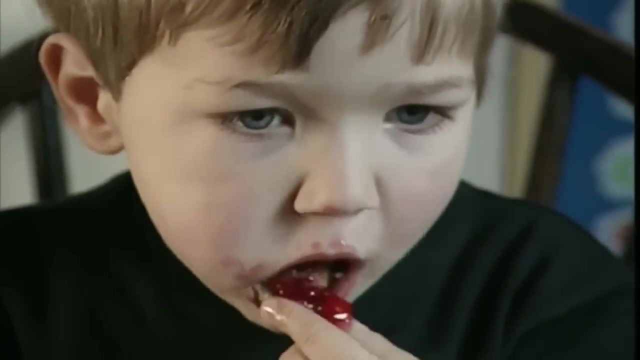 Sharon puts it in the oven to cook. Now they're all ready. I like putting lots of butter on mine. I like putting lots of butter on mine, Yum yum, And I like lots of jam. It's delicious, It's nice. 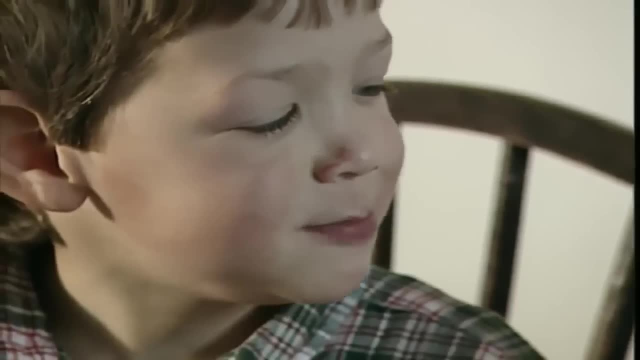 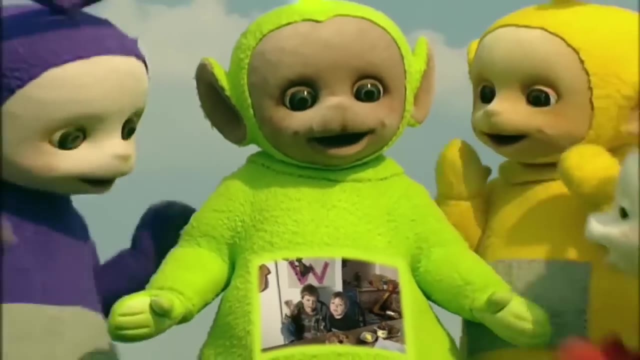 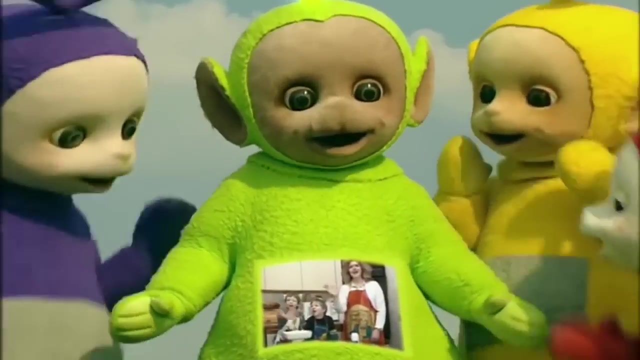 It's yummy, It's really good, And it's good again, but I'm going to eat it again. It's not a good idea. He's going to eat it again. He's going to eat it again. Bye-bye. 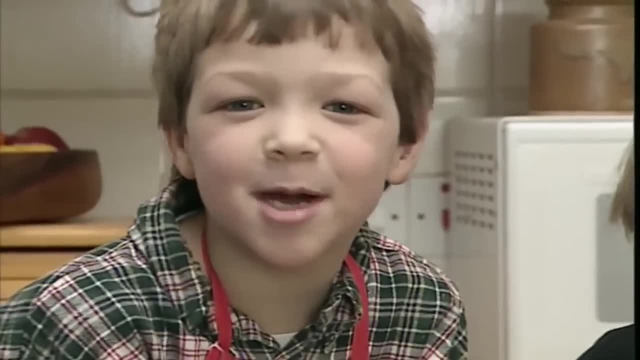 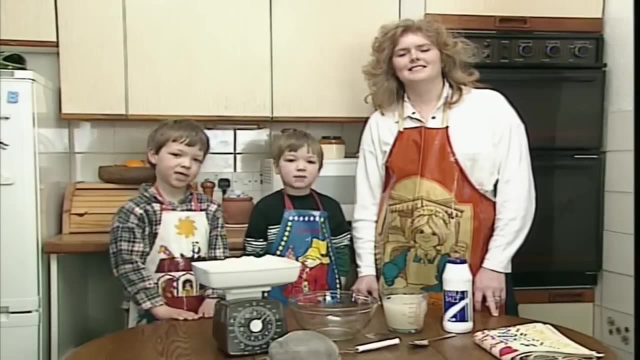 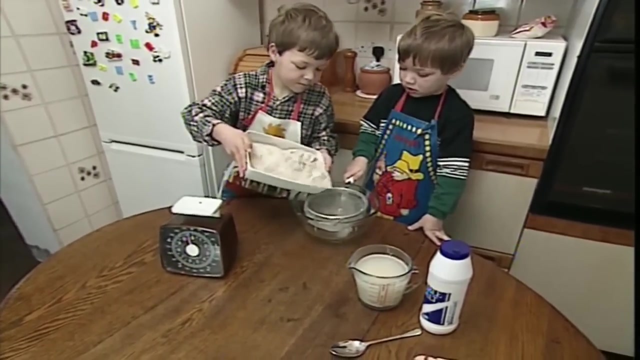 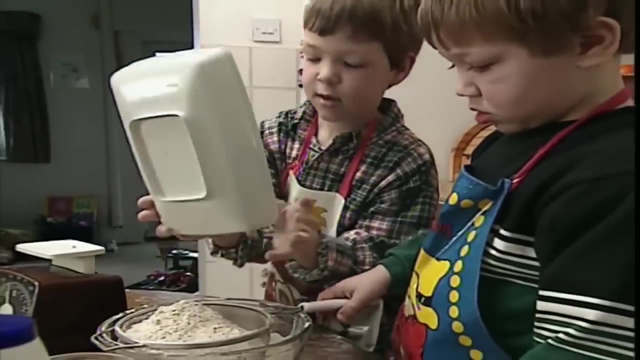 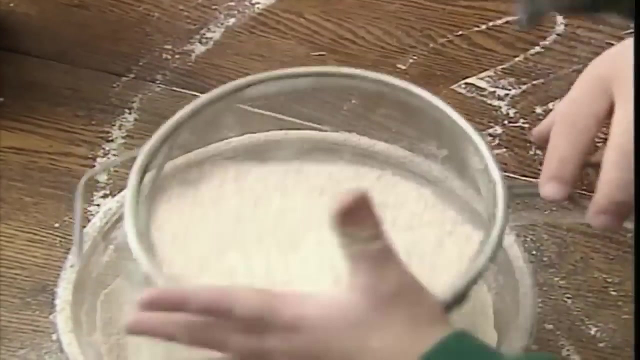 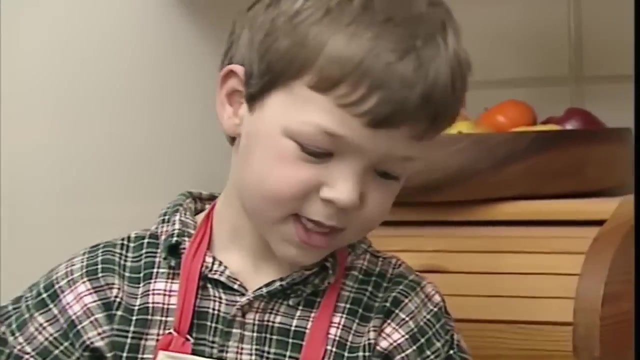 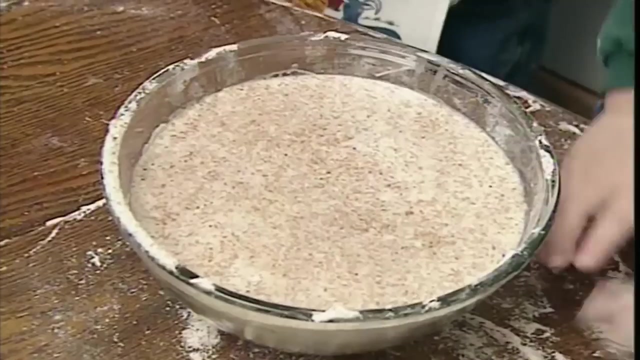 Bye-bye, Bye-bye, Bye-bye, Bye-bye, Bye-bye, Goodbye, Bye-bye, bye-bye, Bye-bye, Bye-bye. We are adding the flour into the sieve. We add the yeast and water. 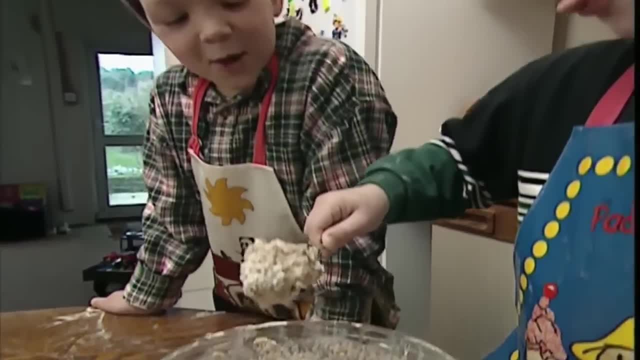 We stir it. Don't Let me have a stir. You don't have to stir it. It's not that hard to stir. You can use a bit of water if you want. You don't have to stir it, You just need to stir it. 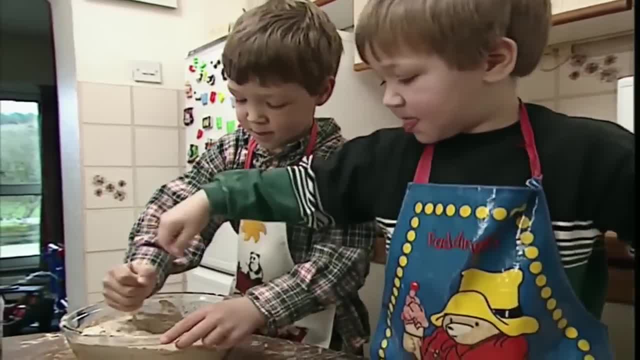 You can stir it. You just need to stir it. You can stir it, You can stir it, You can stir it. You don't have to stir it, You don't have to stir it, You don't have to stir it. 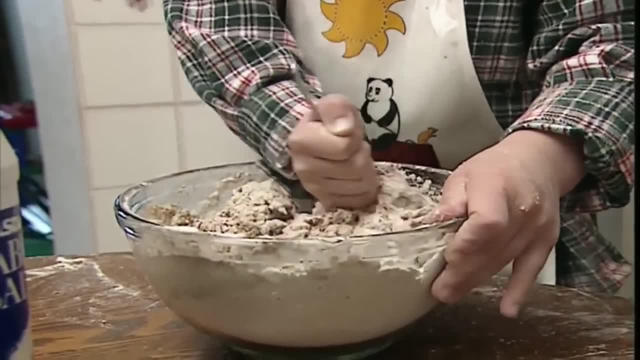 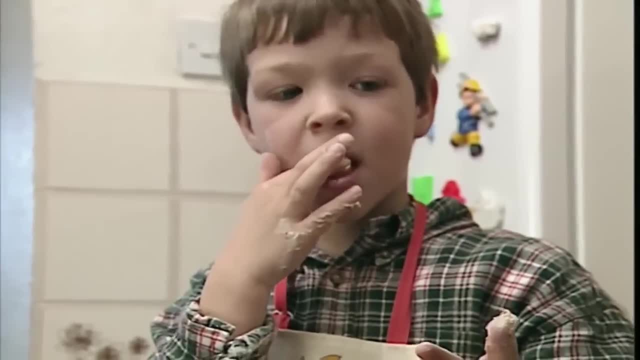 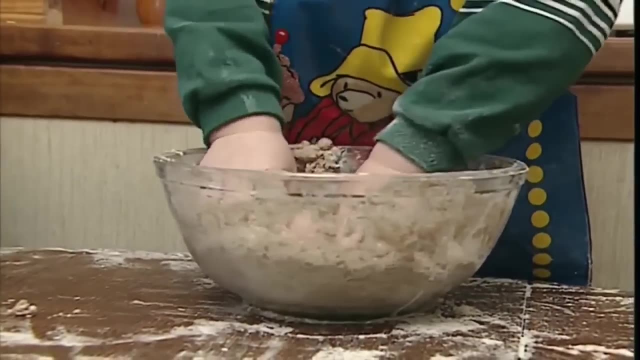 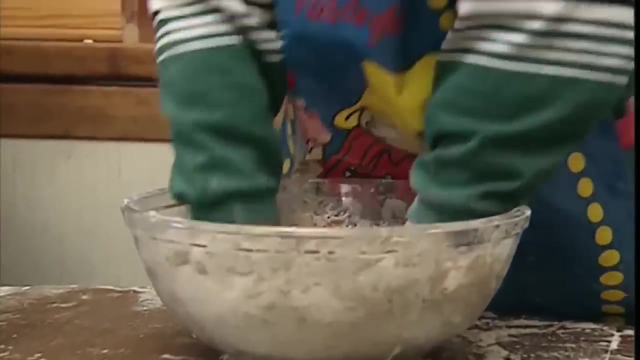 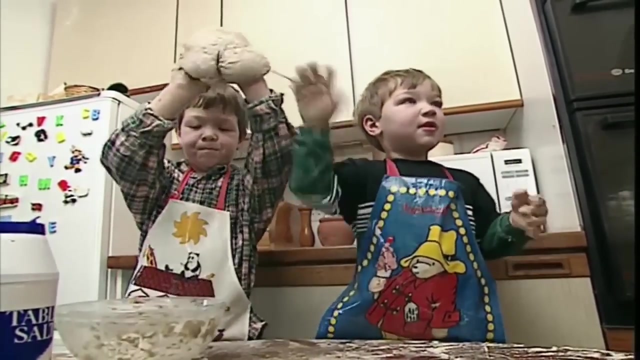 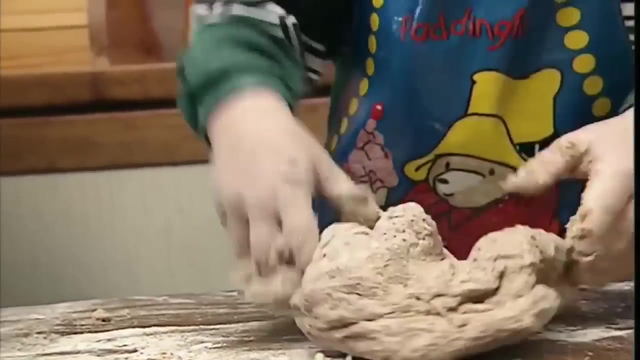 Put a little bit of chocolate, Just pour it, Just pour it into the pot. Add the sugar, Add a bit of salt, Add a bit of saltil Maison, Add the yeast. Now we have to knead it. We need to dough. 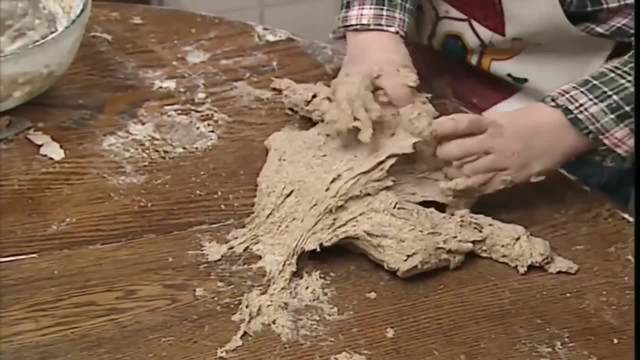 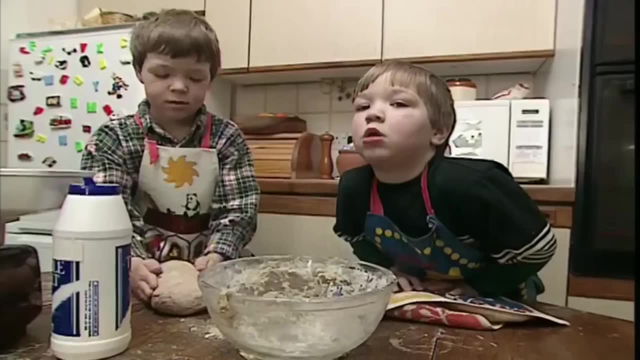 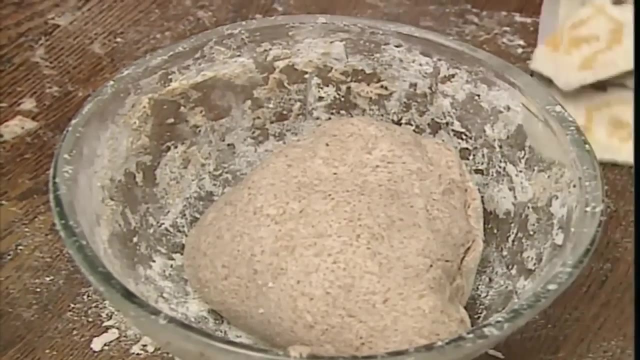 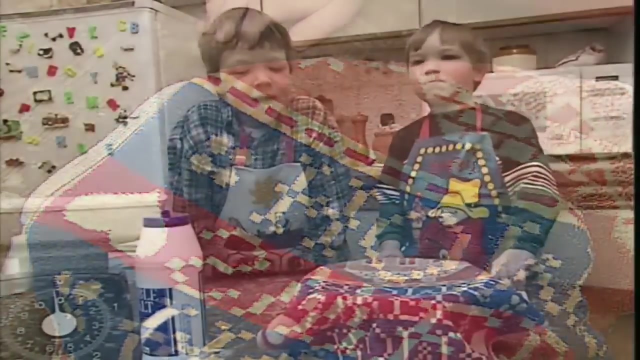 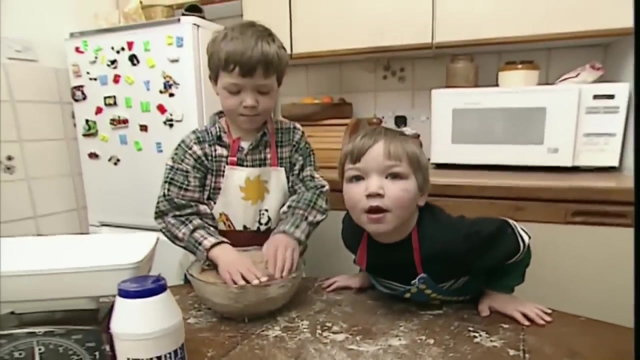 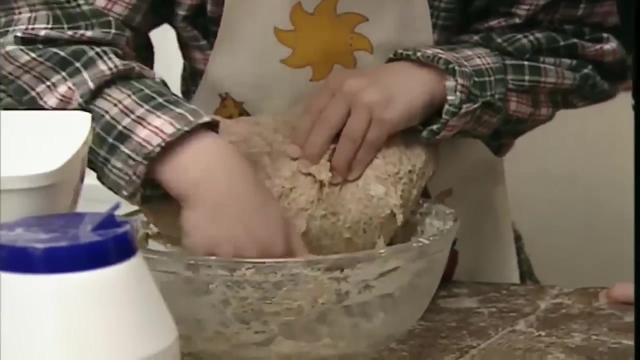 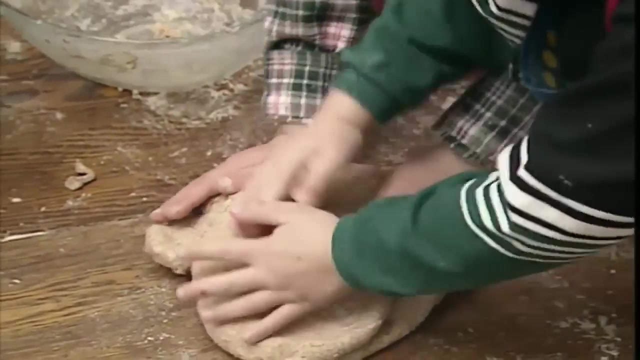 Yeah, It's so sticky, It's long. Now we need it to settle. Now let's look at the bread. Thomas can't see out the bowl, Can he? We have to knead it again. We have to knead it again. 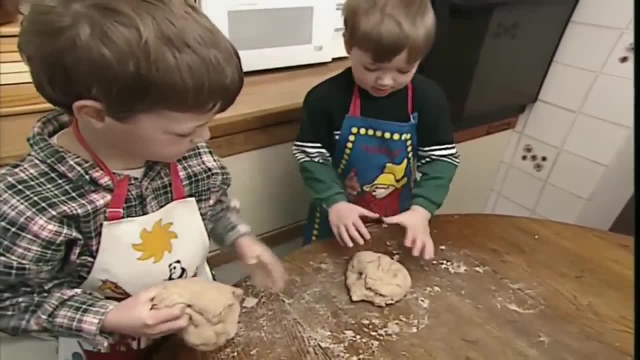 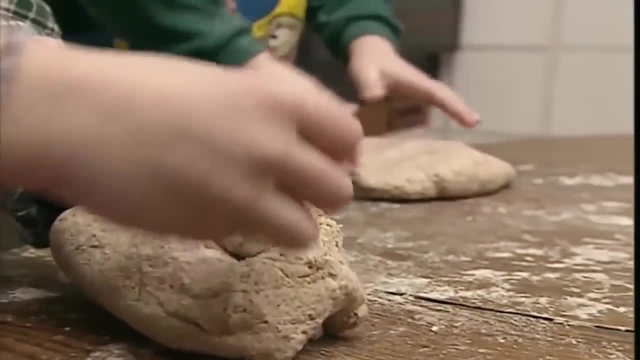 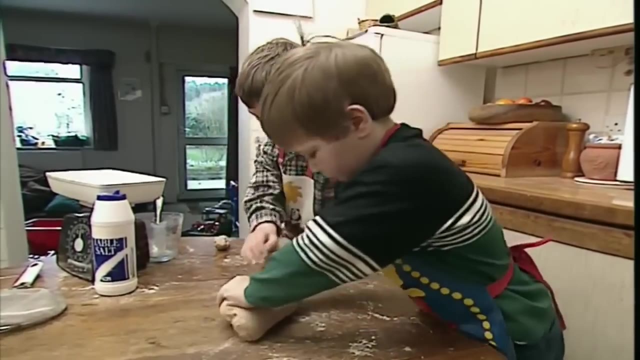 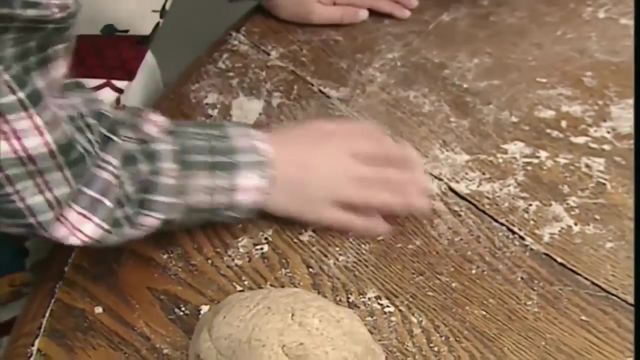 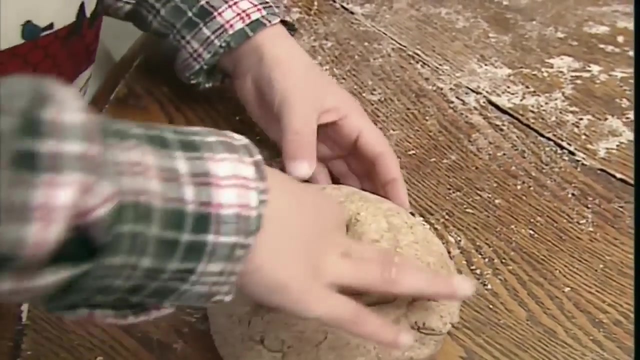 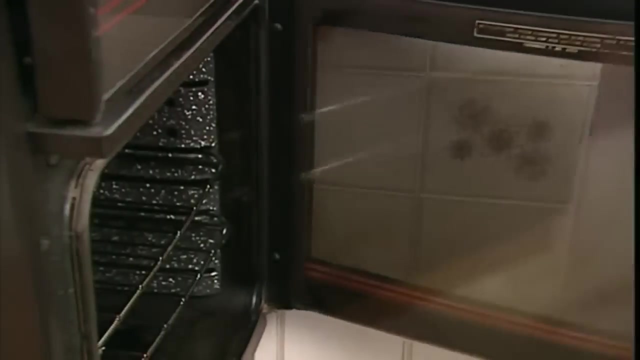 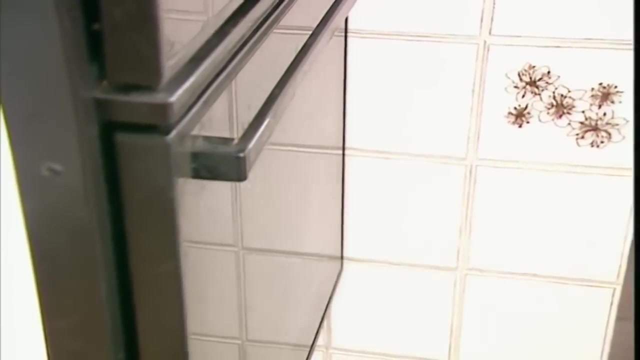 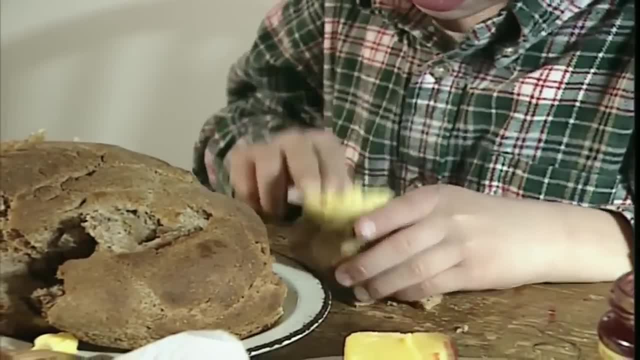 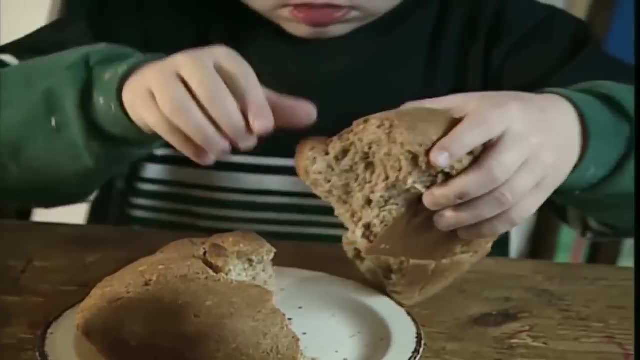 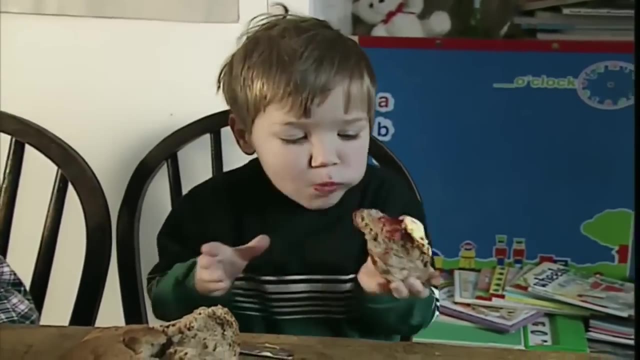 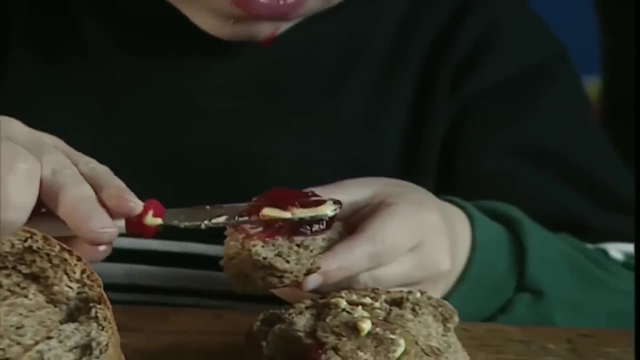 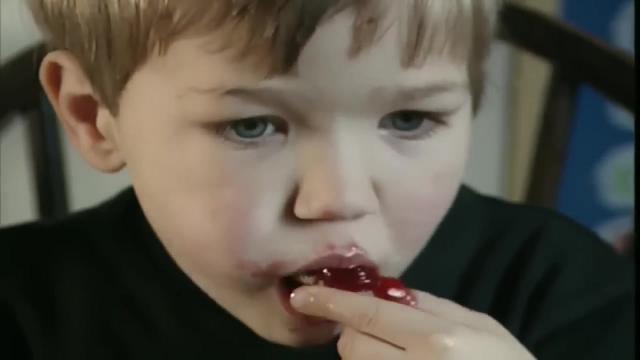 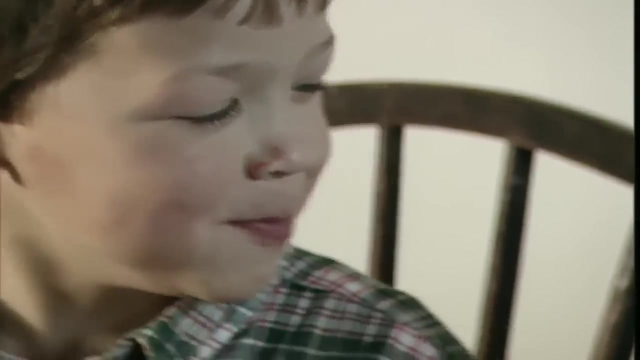 I like putting lots of butter on mine, Yum, yum, And I like lots of jam, Yum, It's. It's delicious. Bye-bye, bye-bye, Bye-bye, bye-bye, Bye-bye. 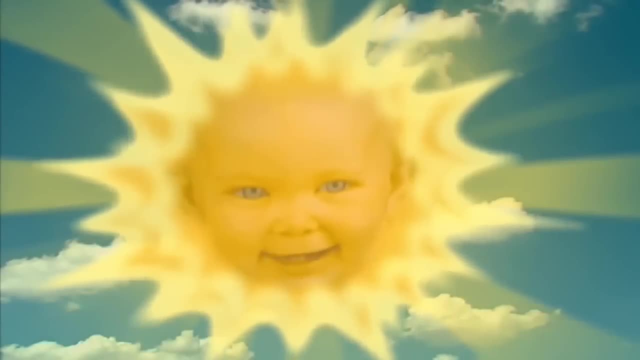 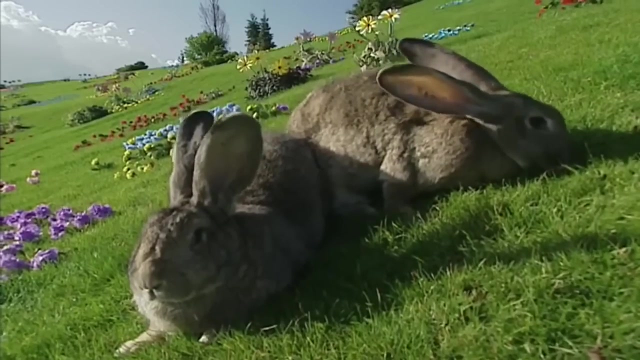 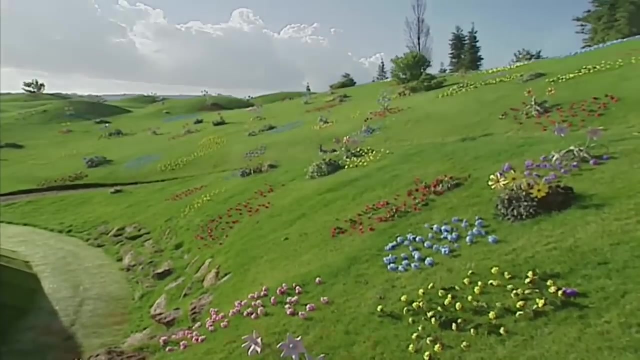 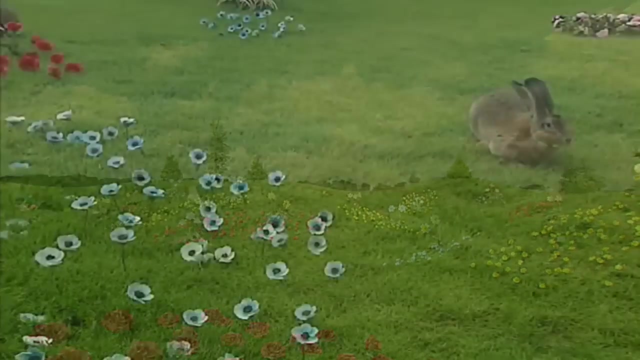 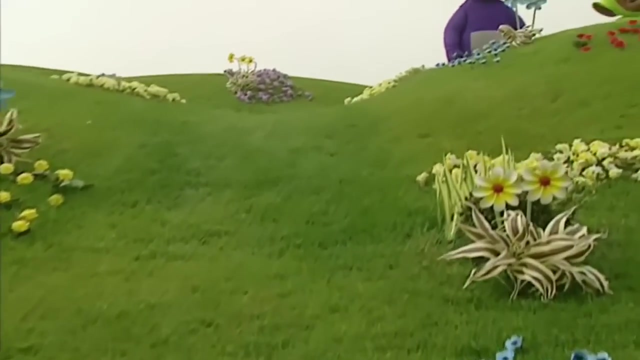 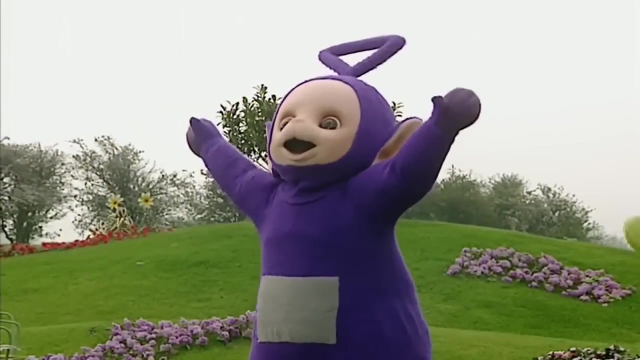 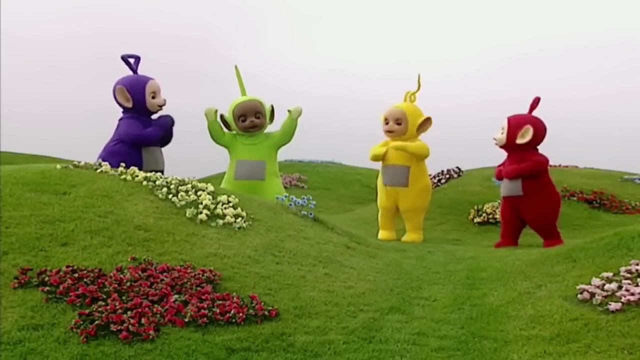 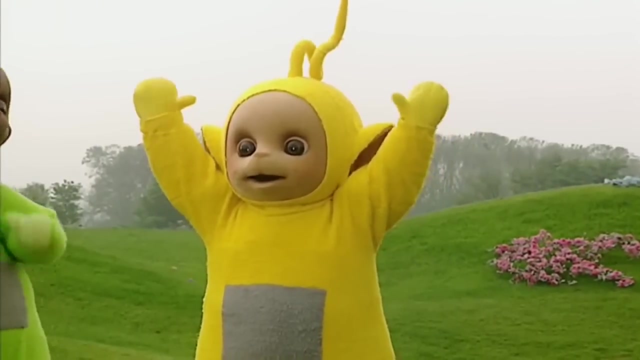 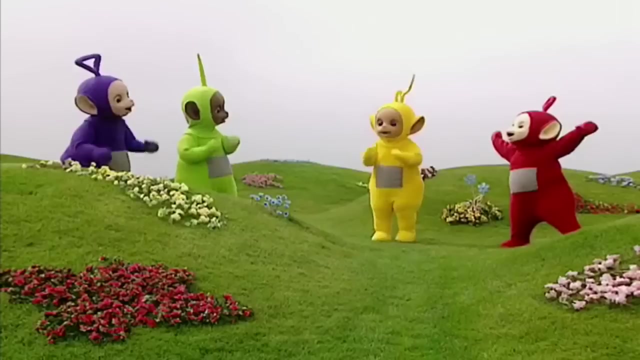 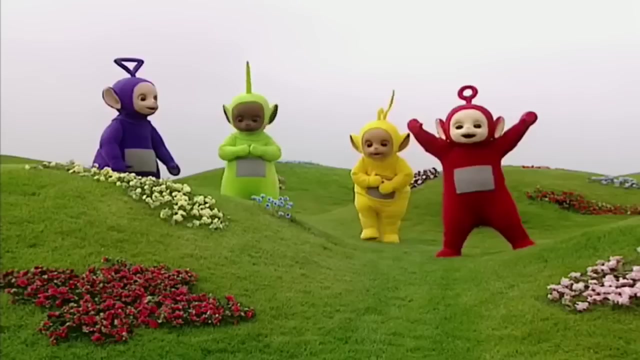 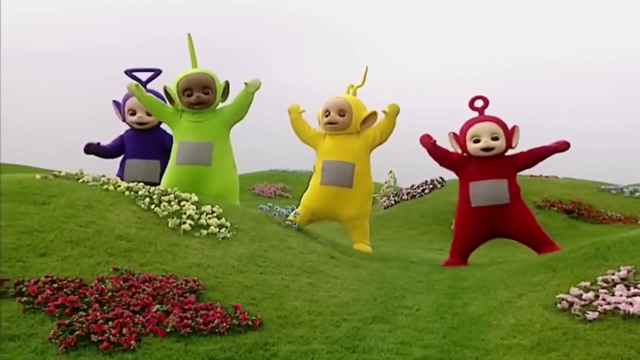 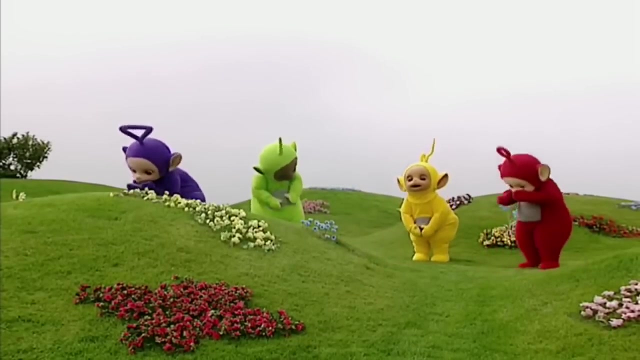 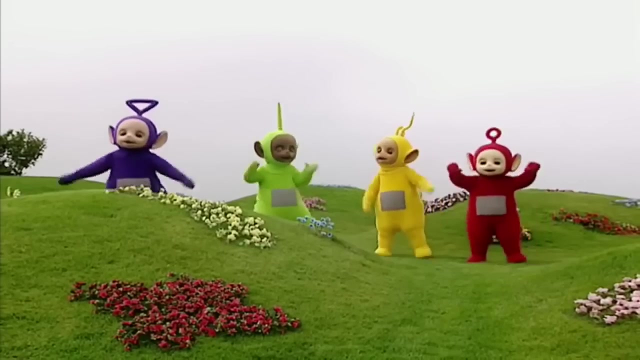 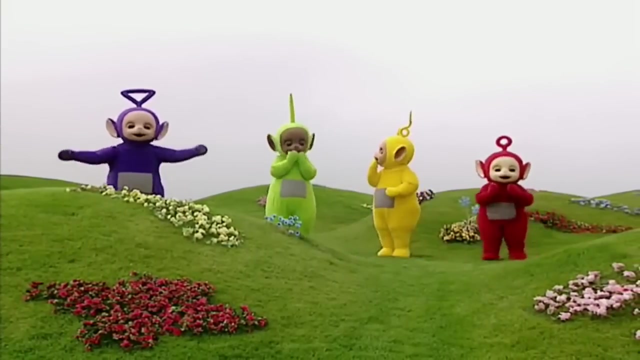 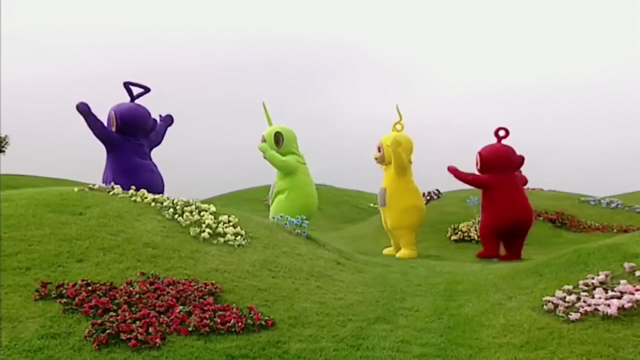 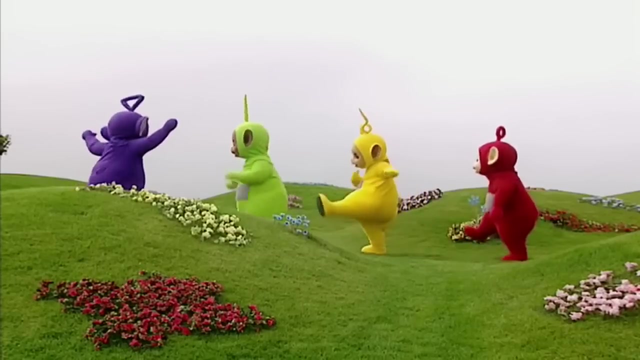 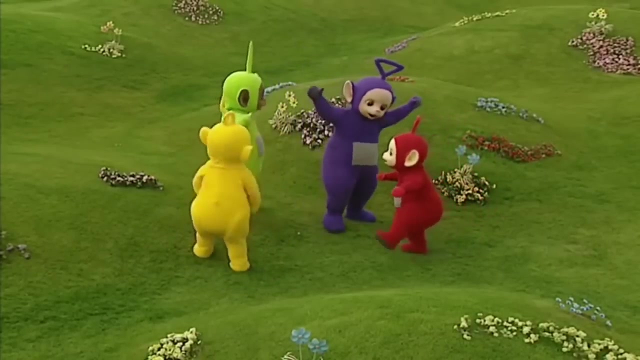 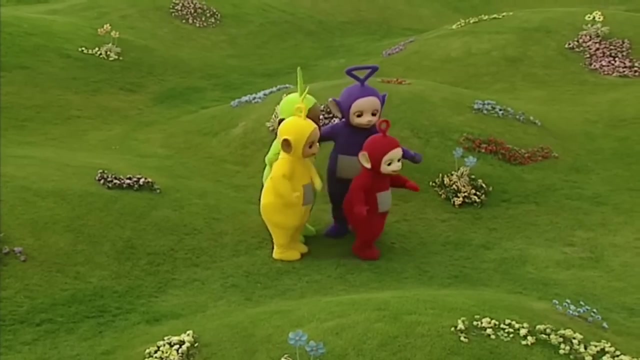 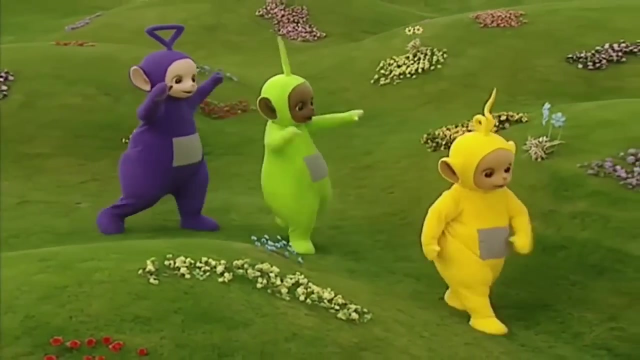 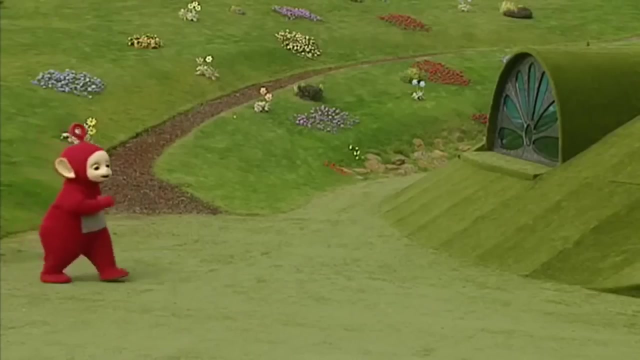 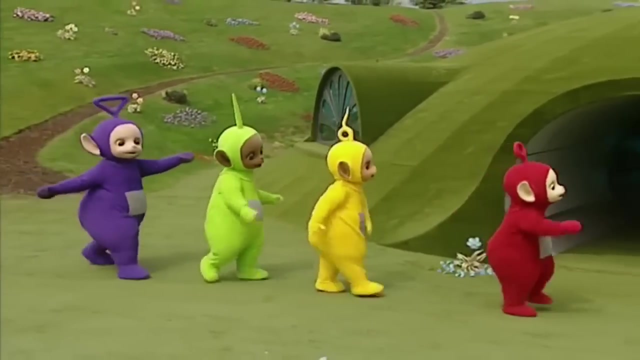 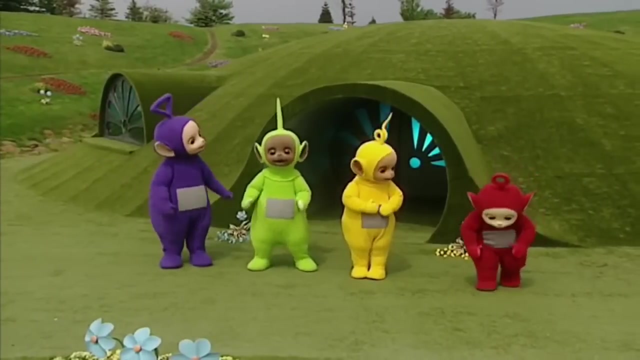 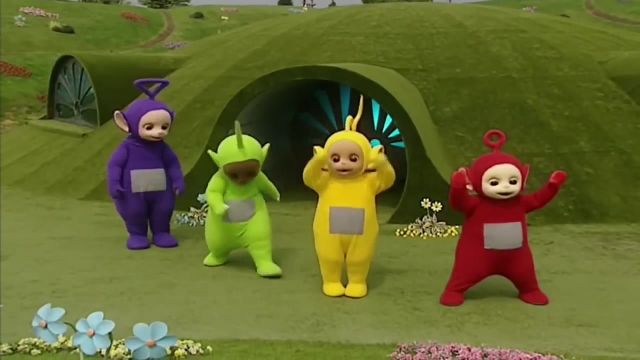 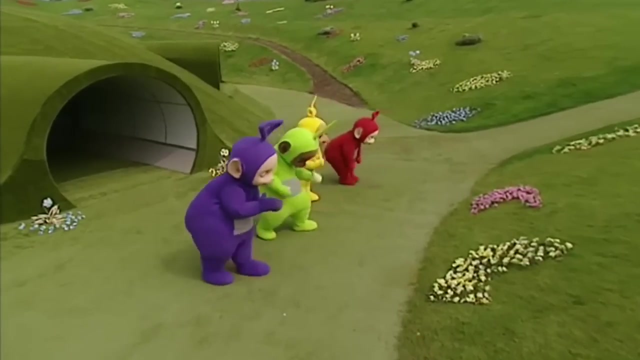 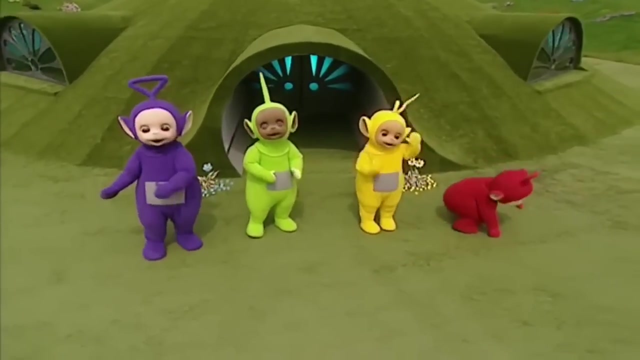 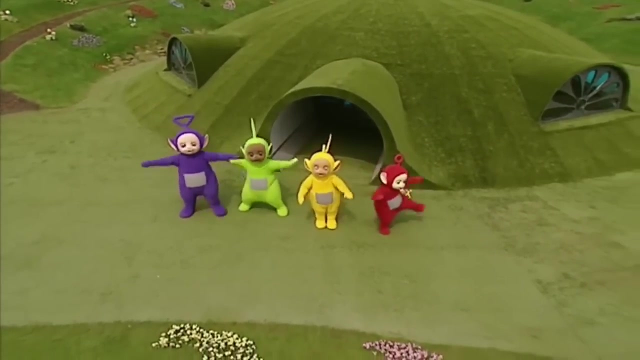 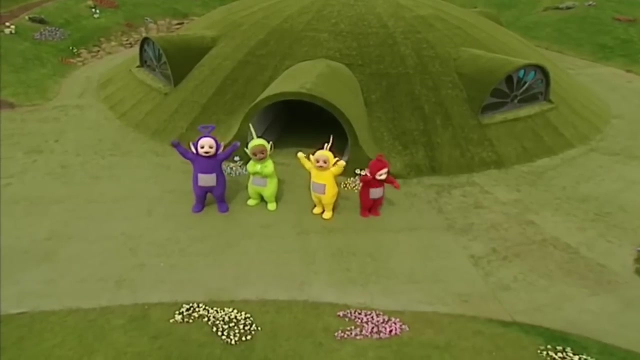 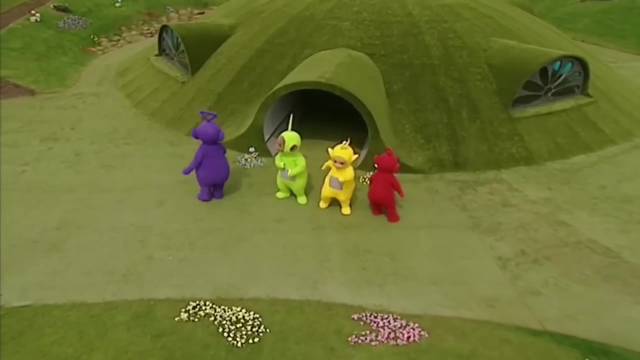 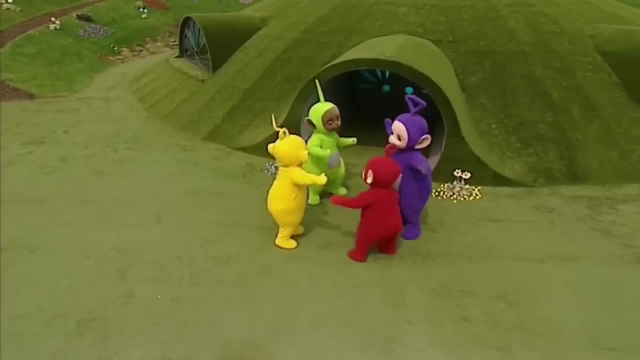 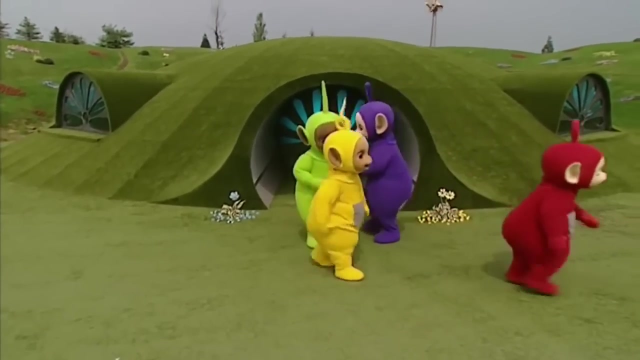 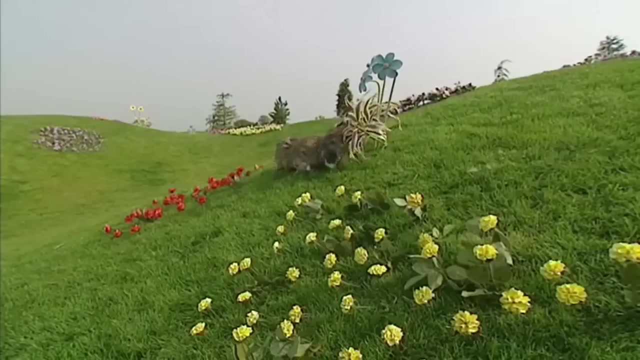 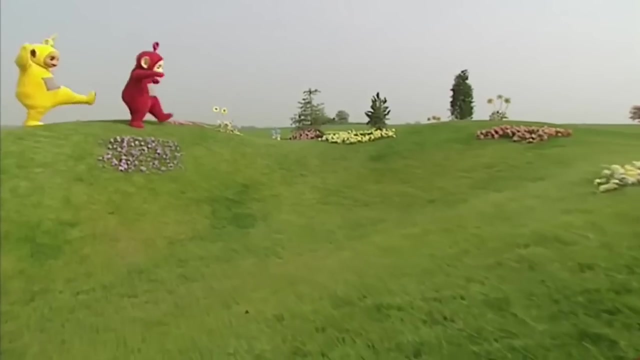 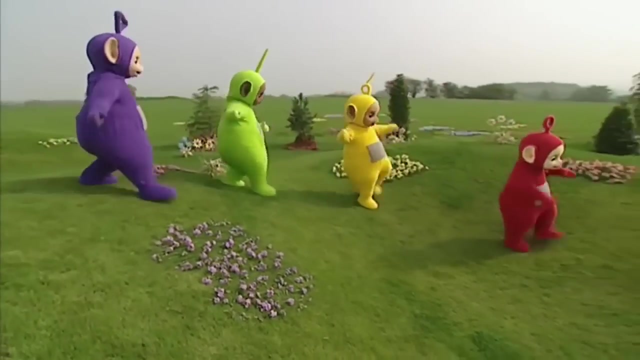 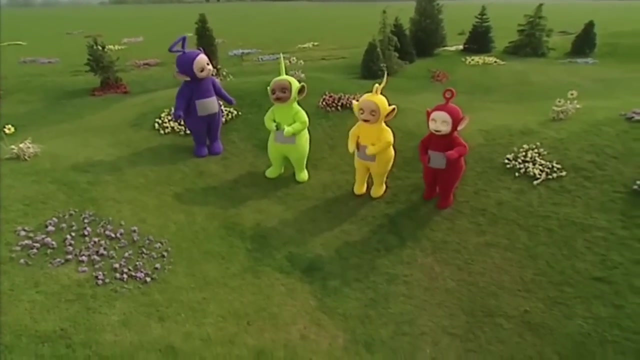 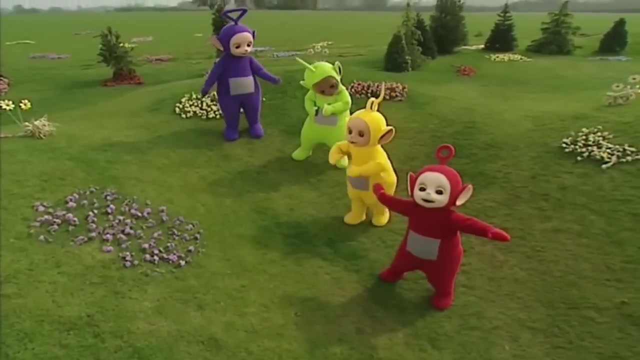 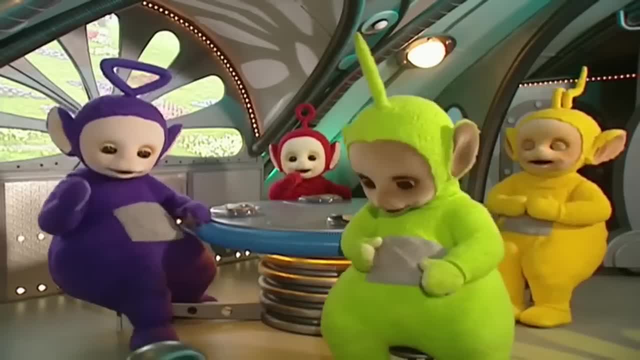 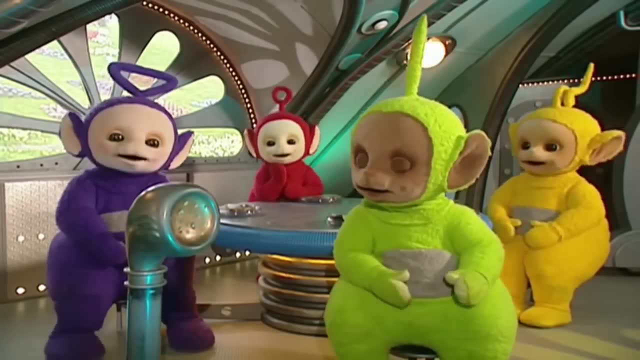 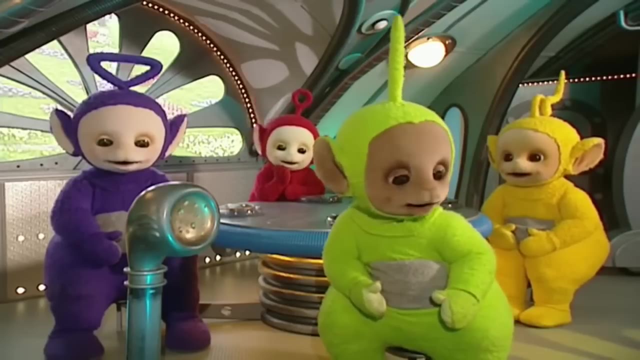 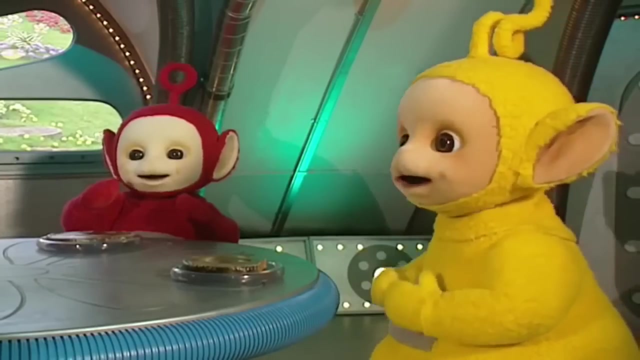 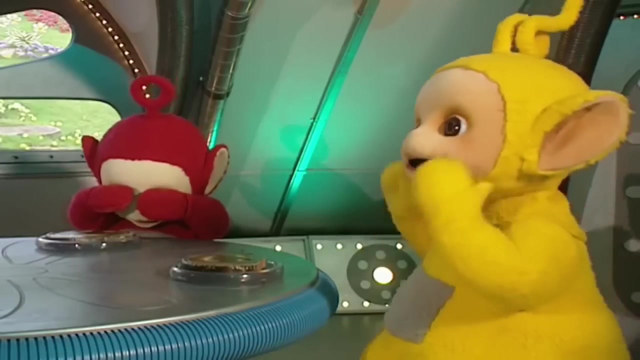 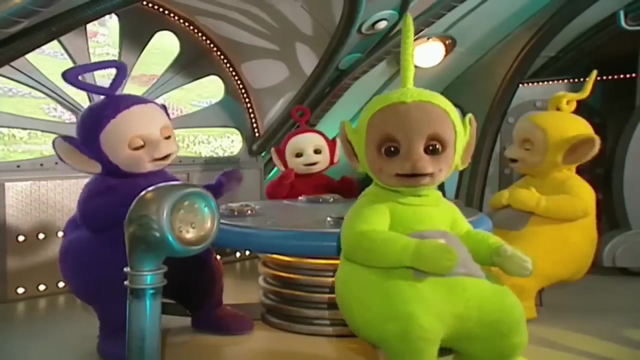 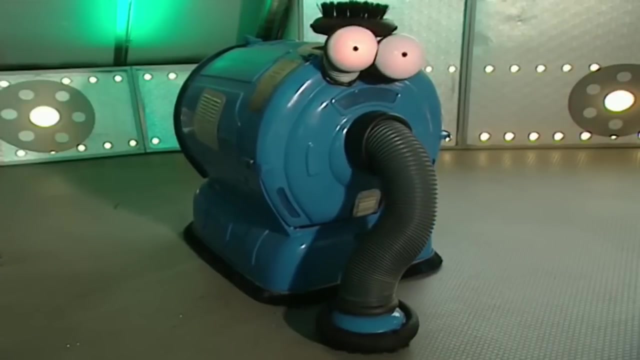 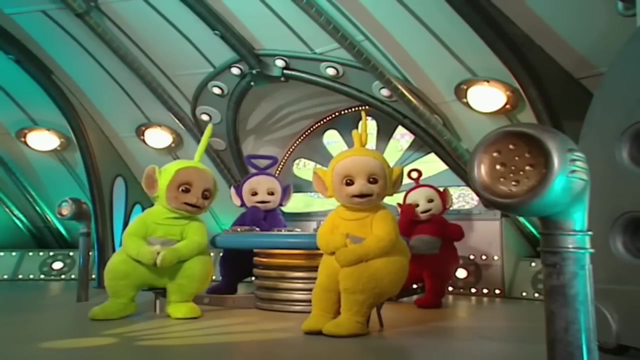 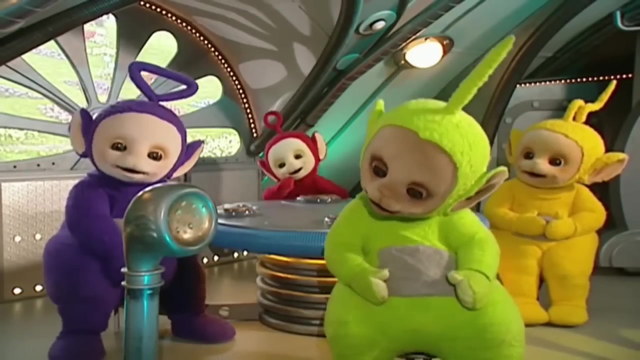 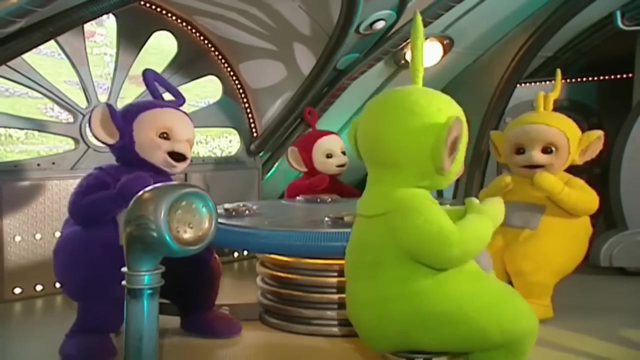 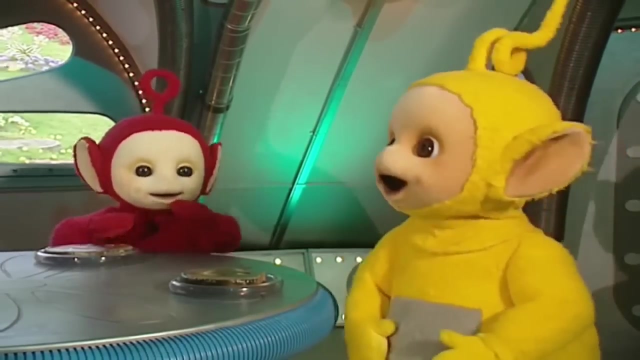 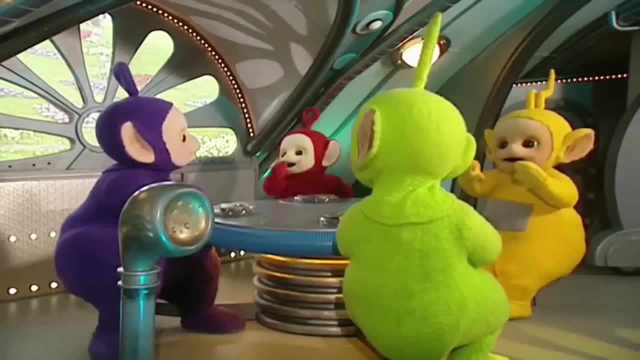 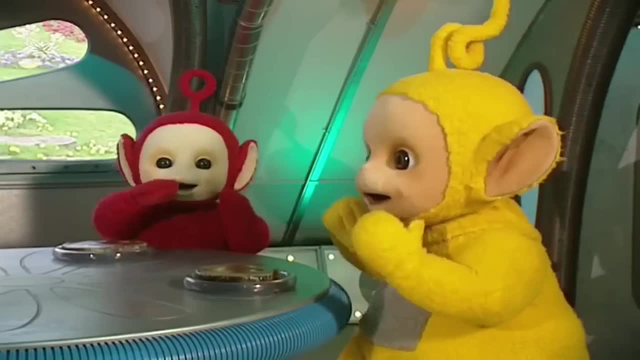 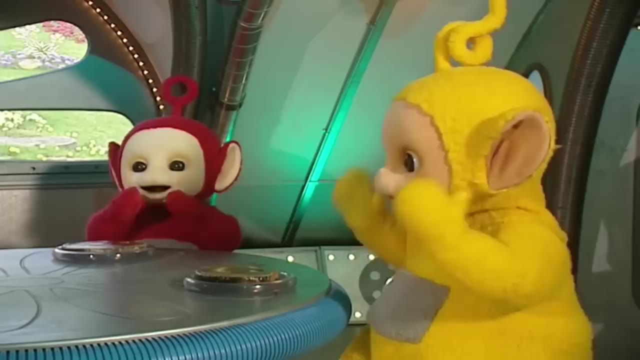 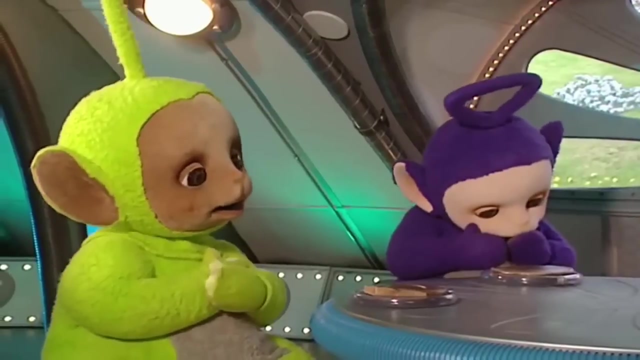 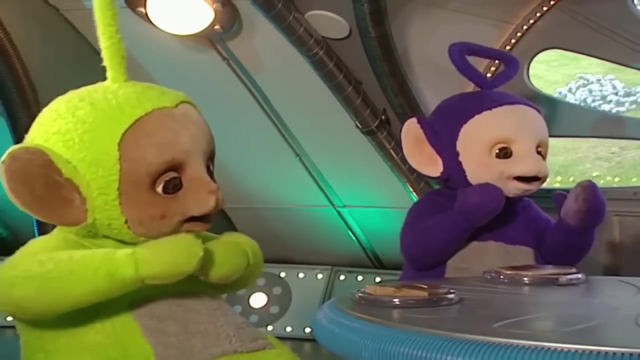 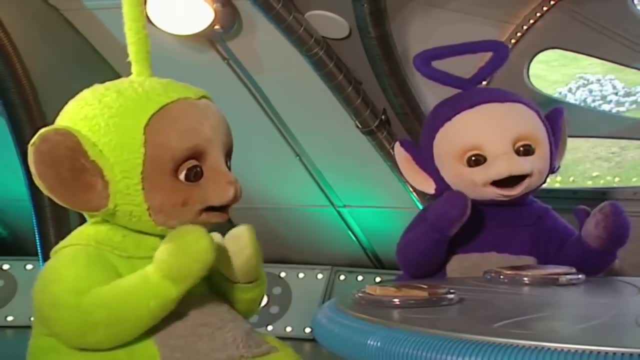 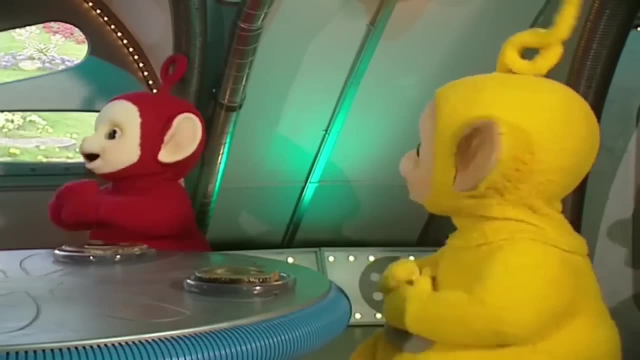 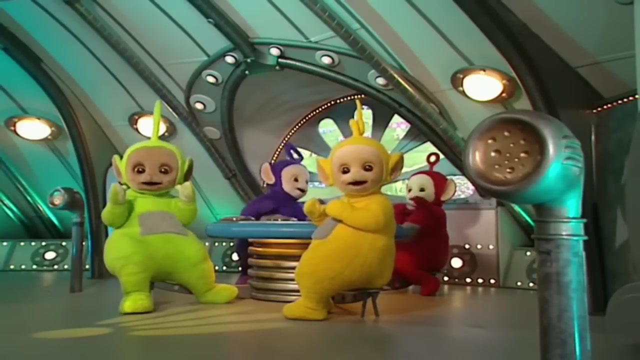 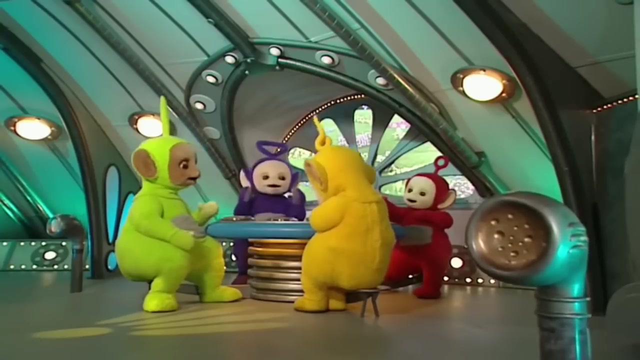 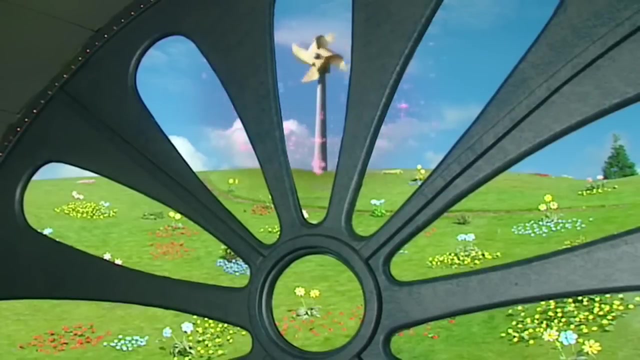 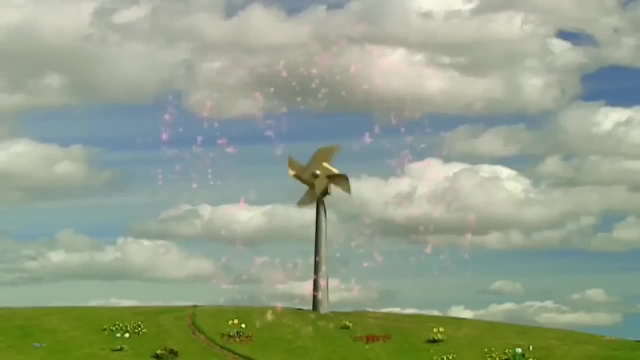 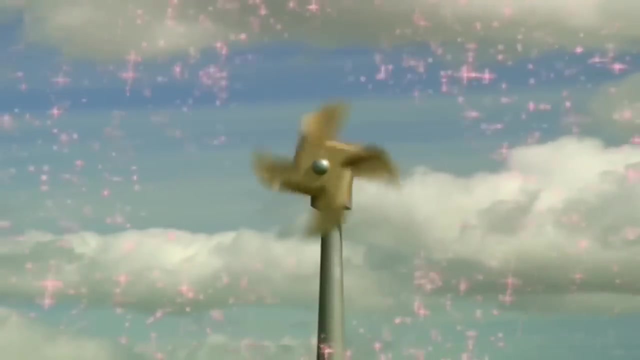 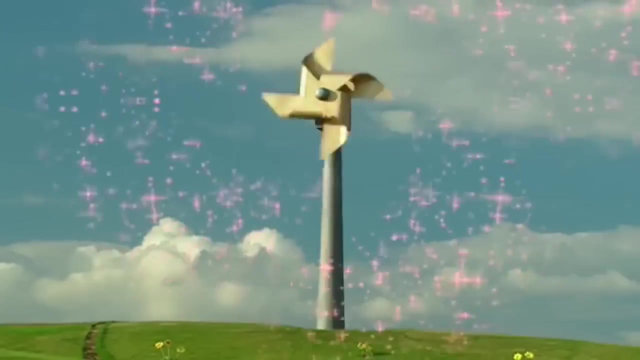 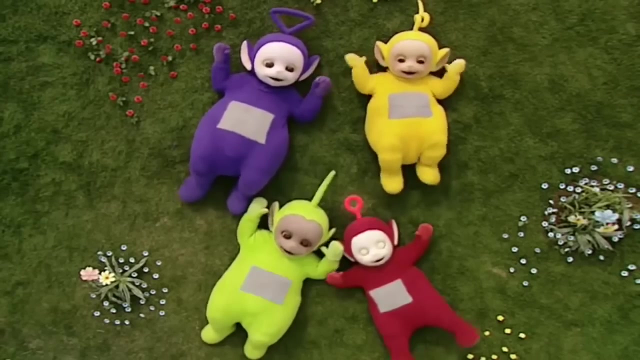 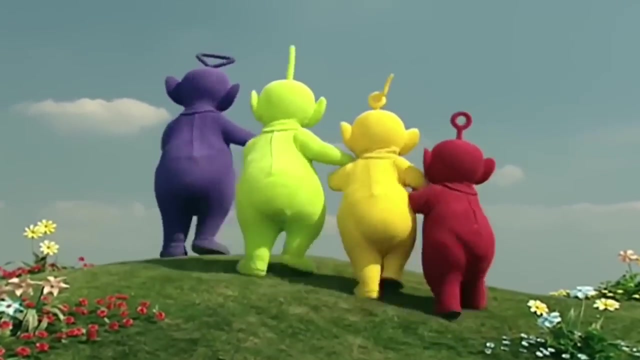 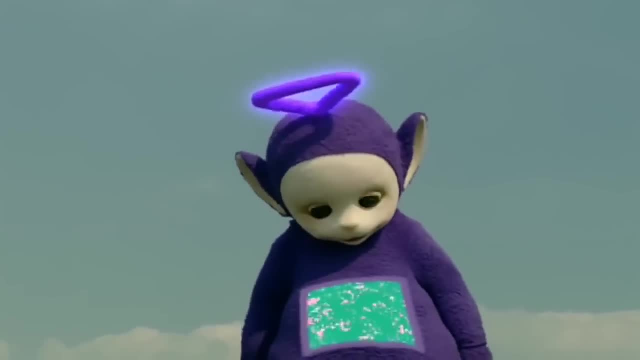 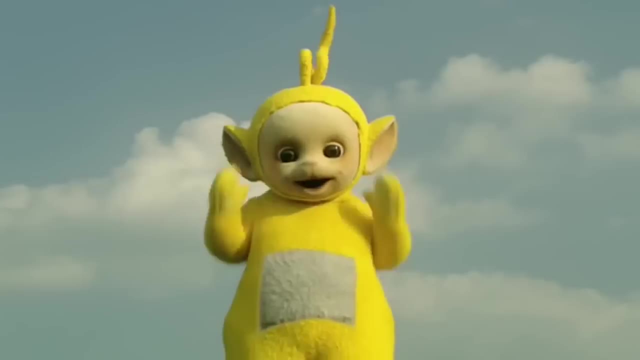 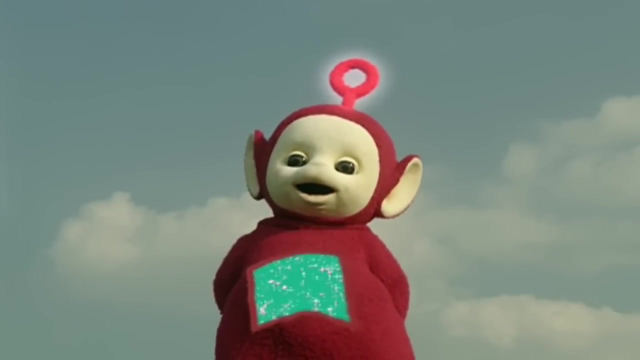 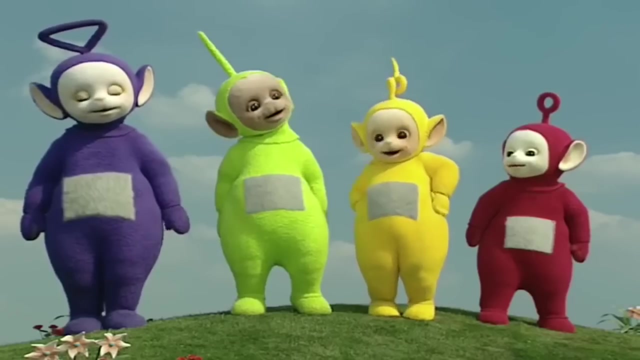 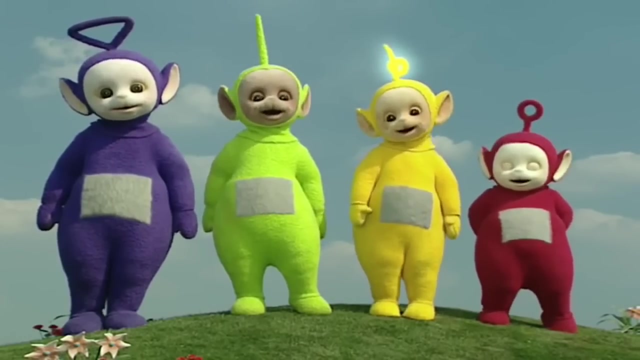 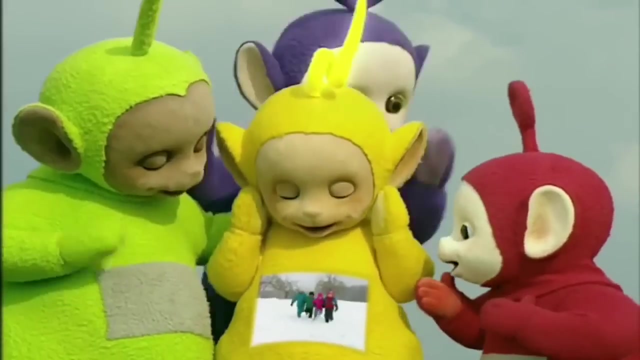 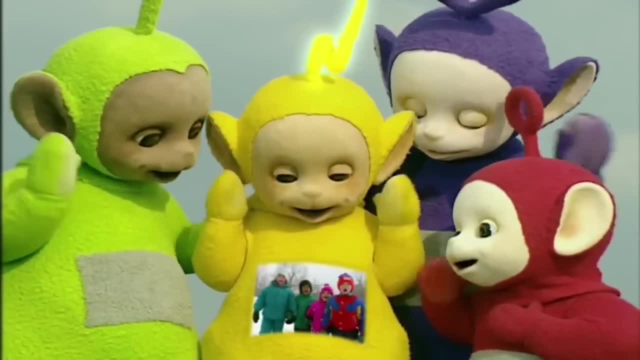 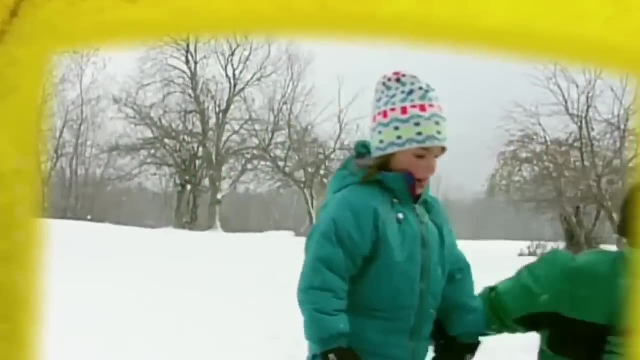 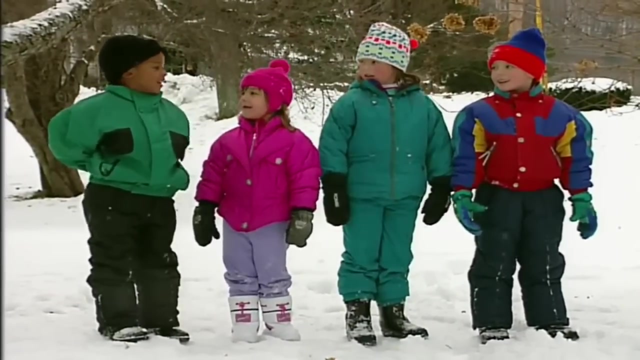 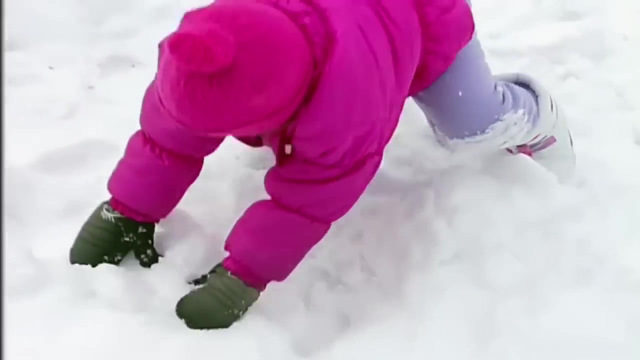 Hello, Hello, Hello, Hello, Hello, Hello. Hi, my name is Joseph, Hi, my name is Katie, Hi, my name is Dominique And this is Pauline. Come with us, Come with us, The snowman. 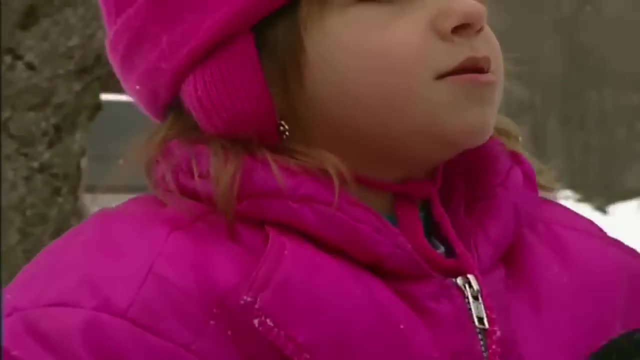 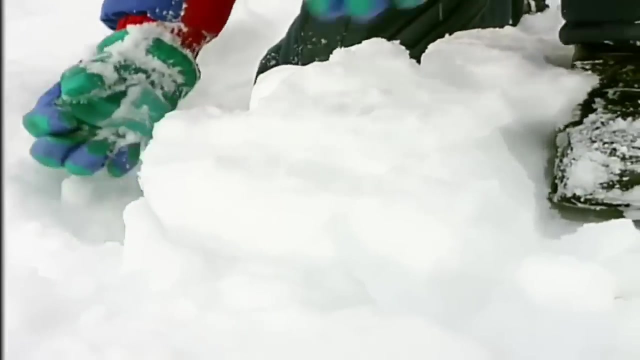 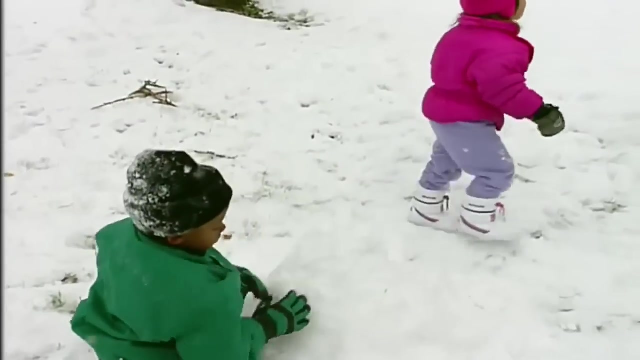 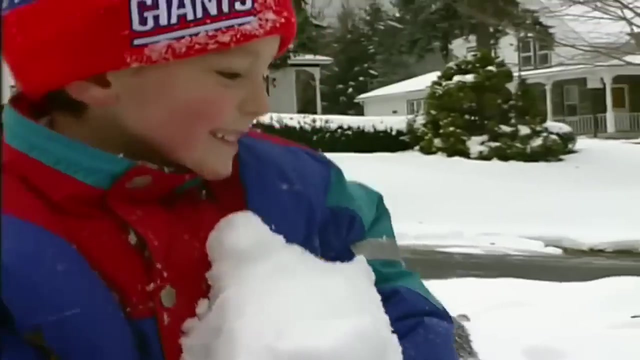 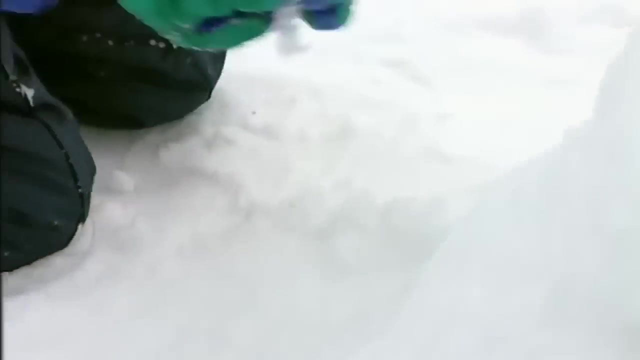 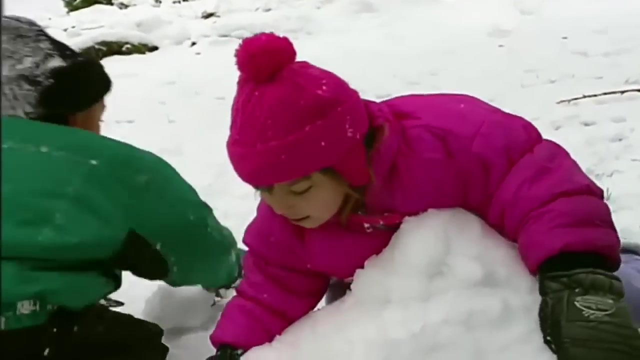 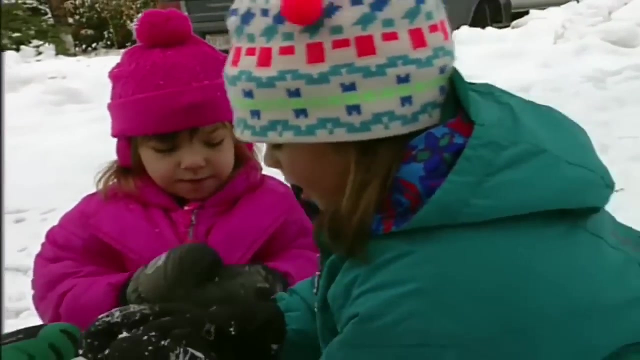 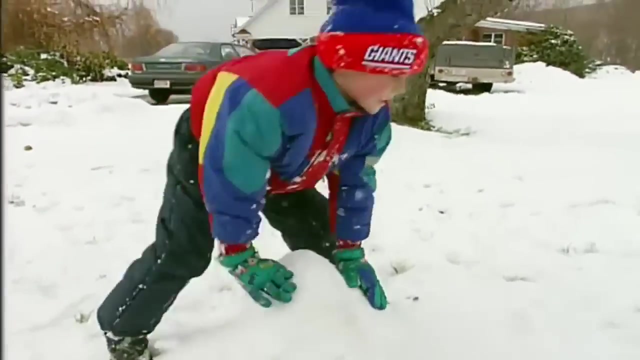 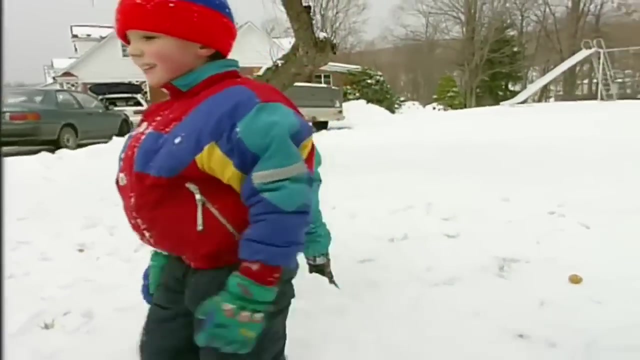 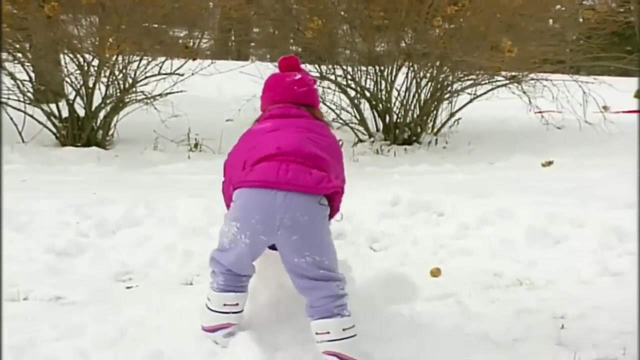 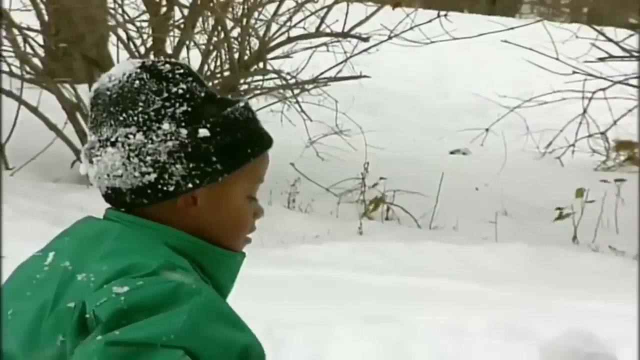 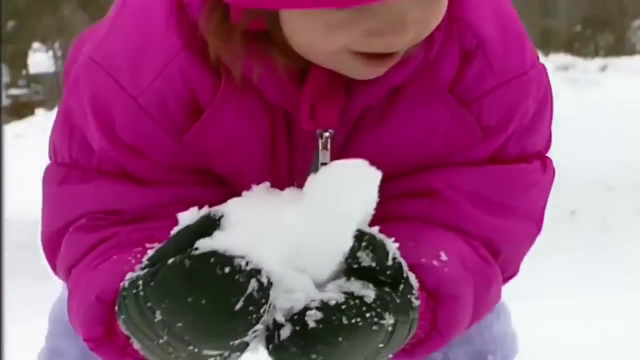 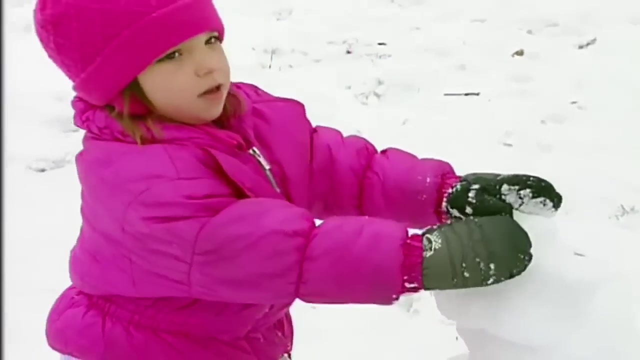 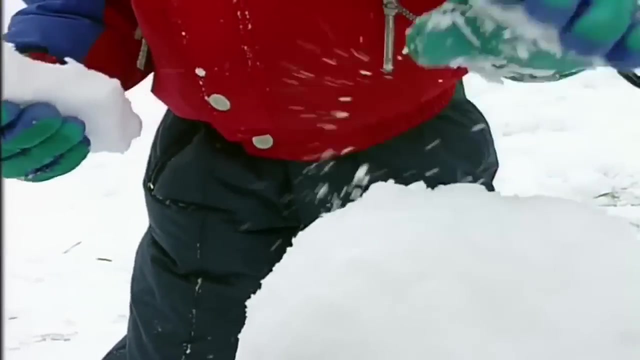 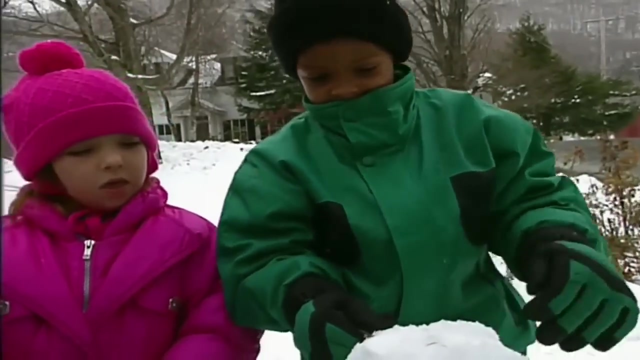 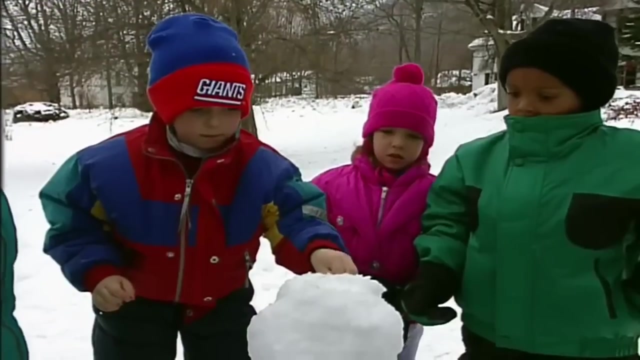 Last night it started snowing and it didn't stop. Now there's snow everywhere. Music- We collected lots of snow Music. The snow is cold and soft Music I like in the snow. Hi Hi, Joseph, put the eyes on the snowman. 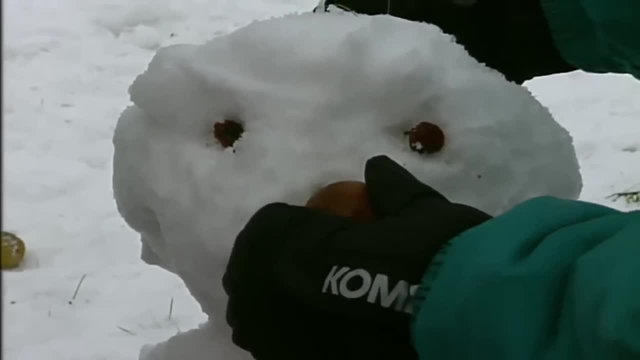 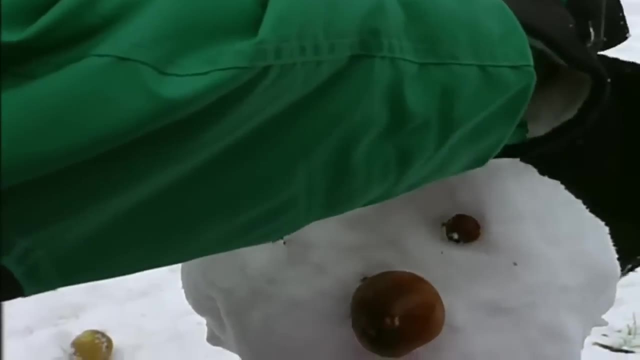 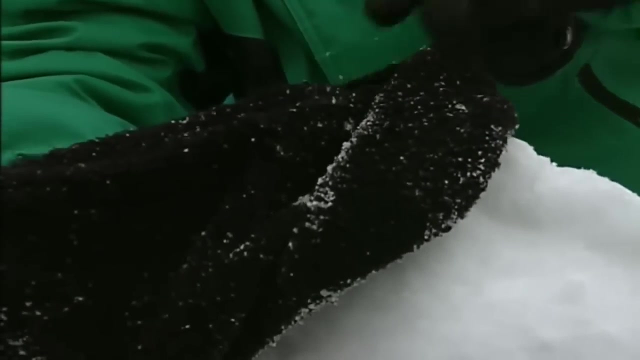 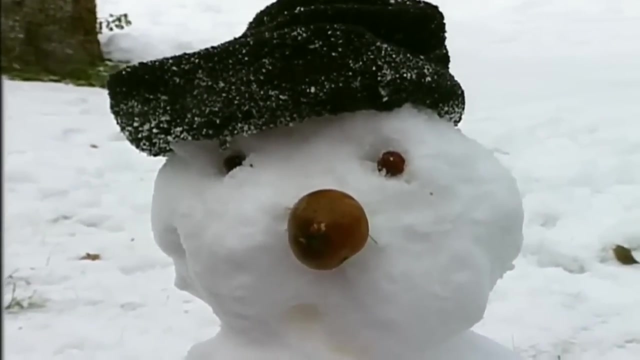 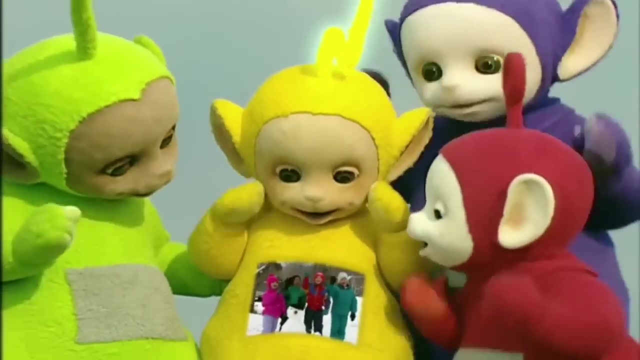 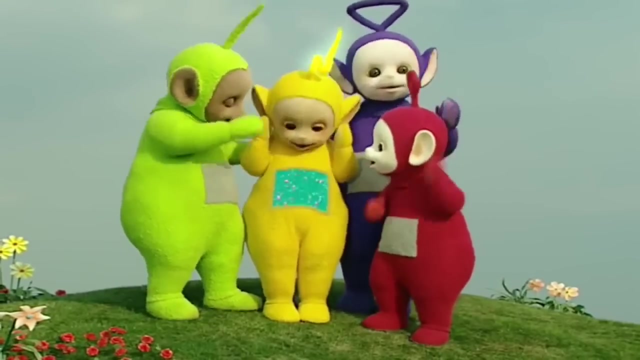 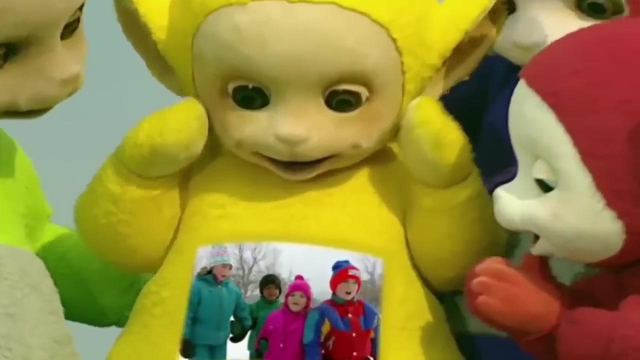 Katie put his nose on Dominique, put the hat on the snowman. Our snowman is really cool. Bye, Bye, Again, Again, Hi, Hello, Hello, Hi. My name is Joseph, Hi, My name is Katie. 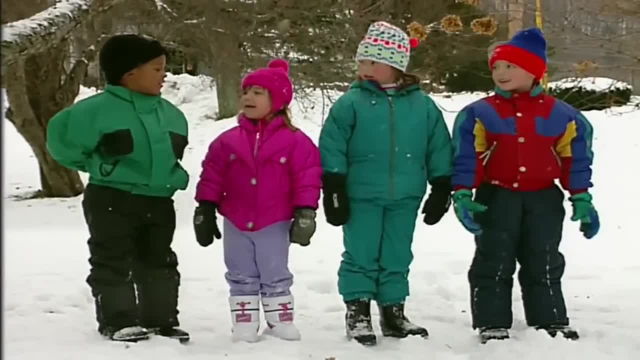 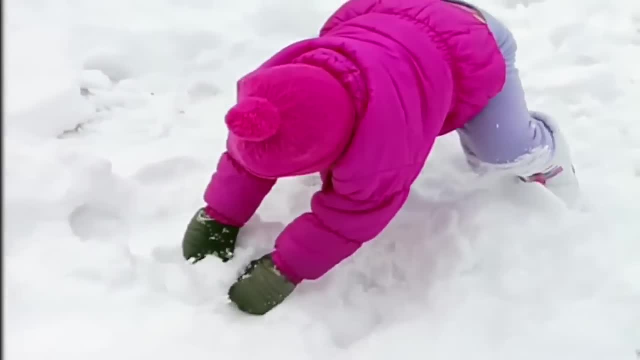 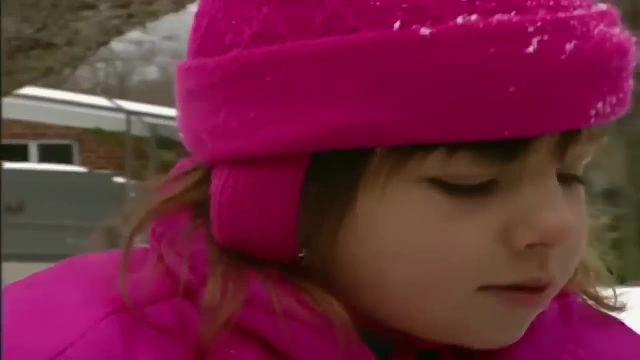 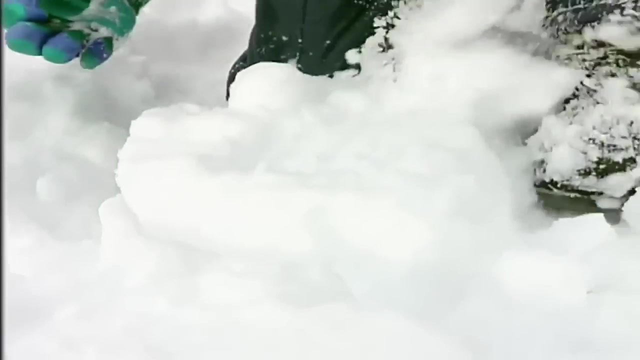 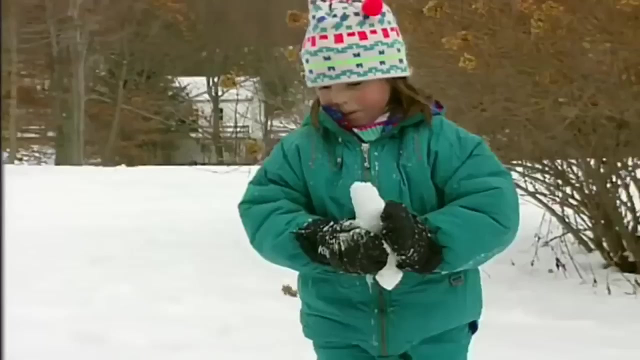 Hi, My name is Dominique And this is Pauline. Come with us. Come with us, The snowman. Last night it started snowing and it didn't stop. Now there's snow, There's snow everywhere. We collected lots of snow. 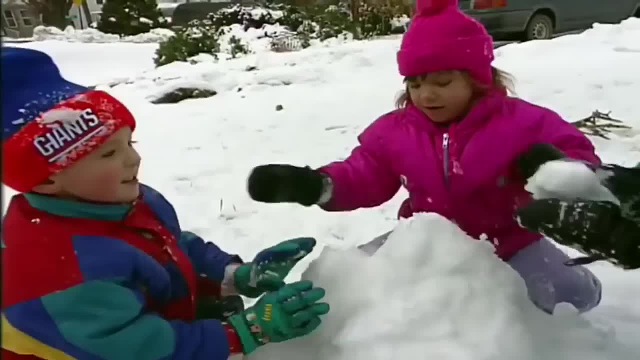 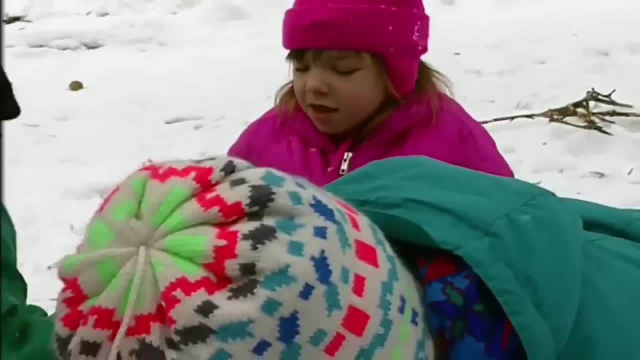 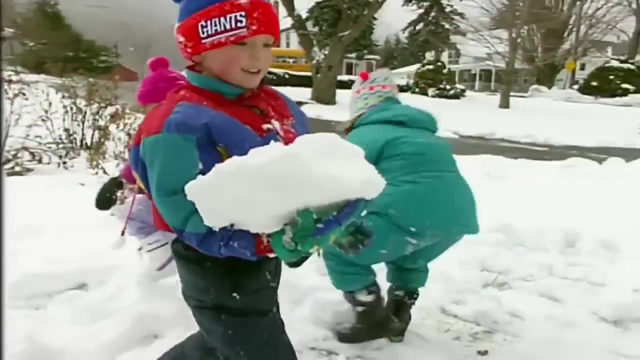 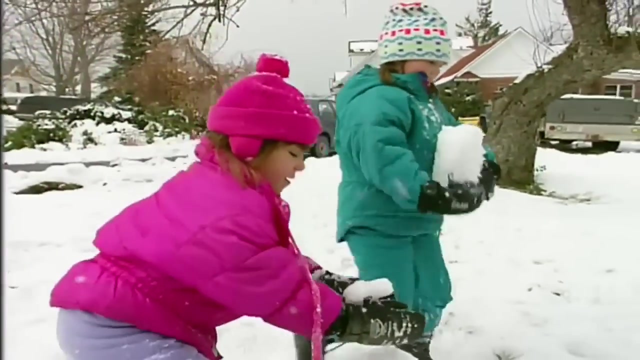 The snow was cold and soft. I like playing in the snow. I like playing in the snow. Yes, Yes, Yes. Look up in this way. Look up in this way. Yes, Yes, Yes, Yes, Yes, Yes. 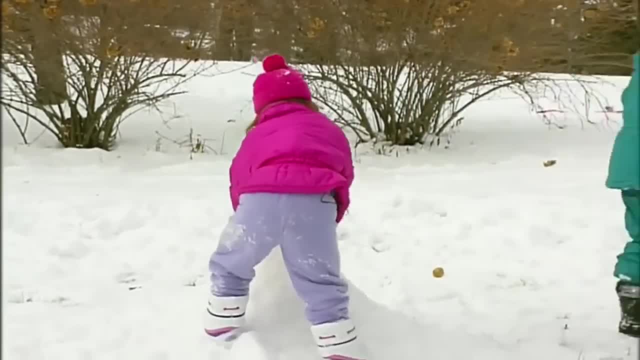 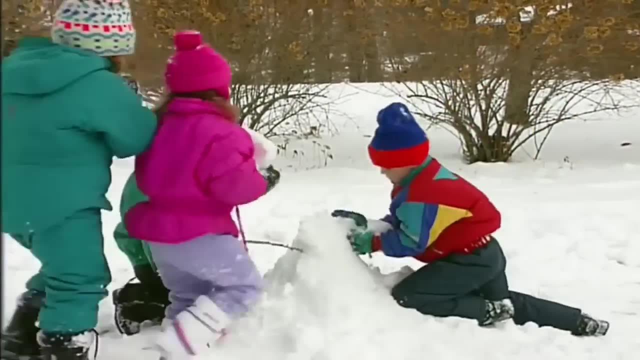 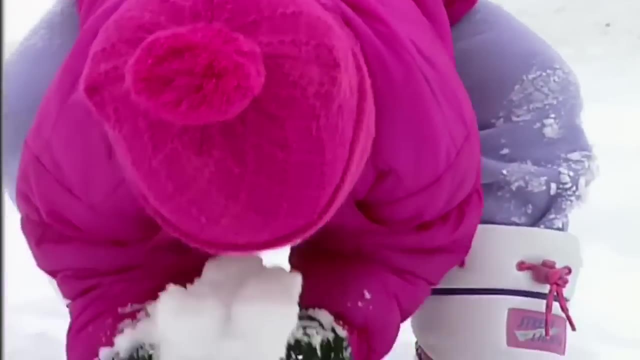 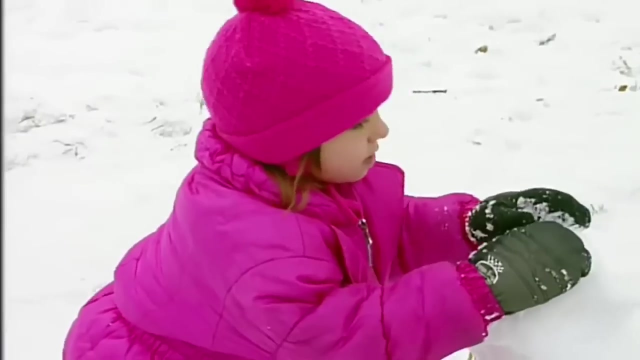 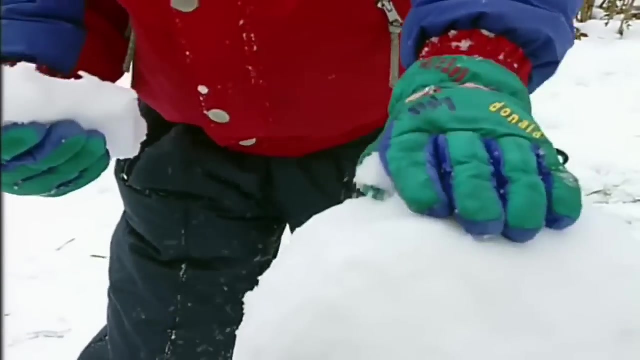 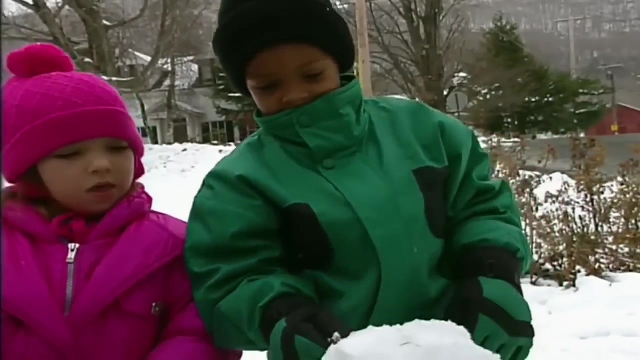 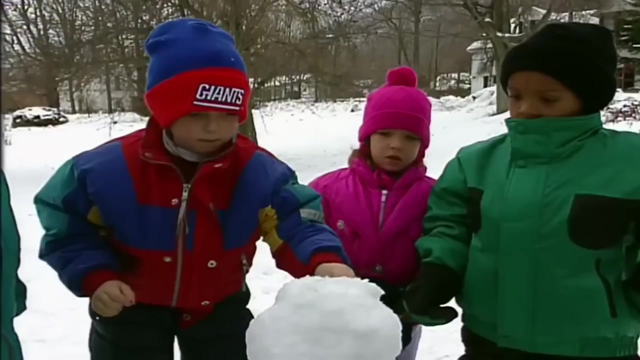 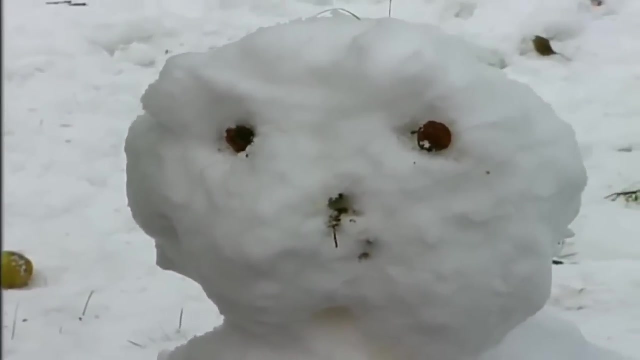 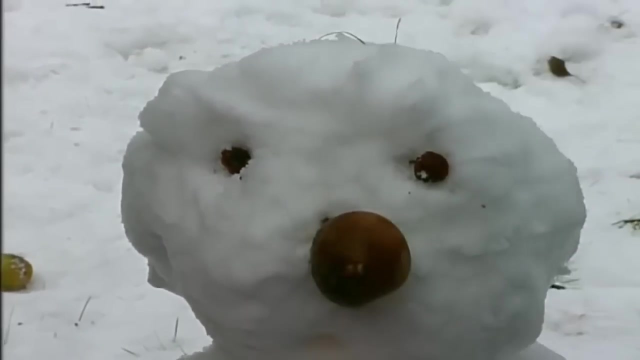 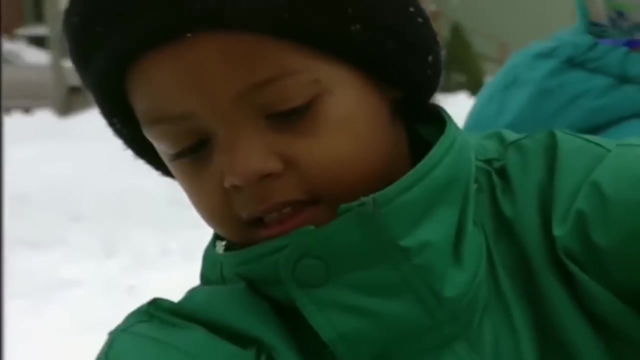 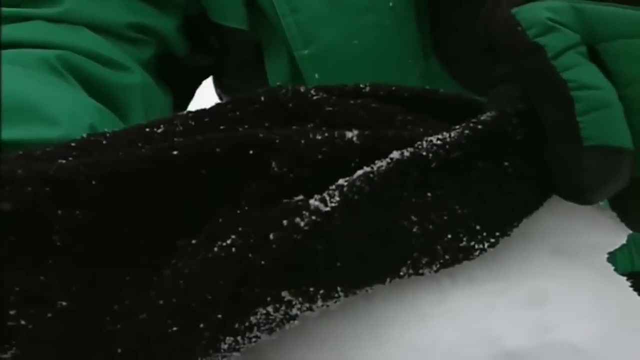 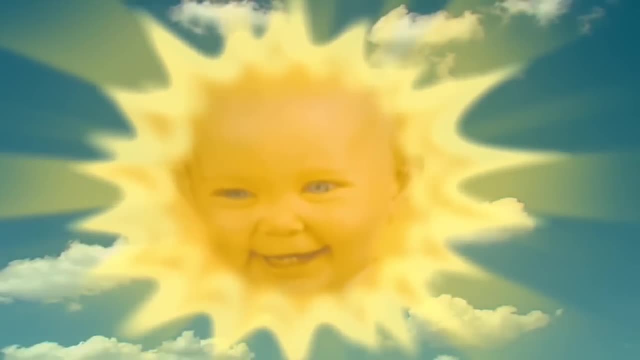 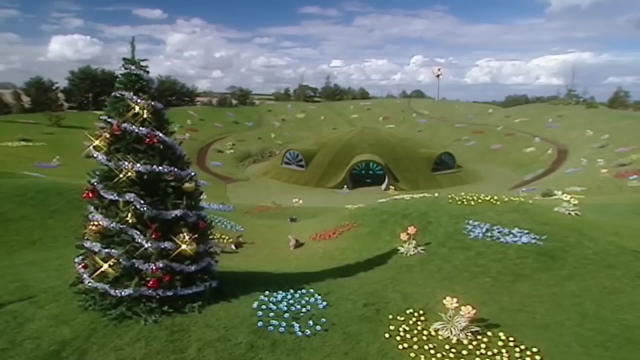 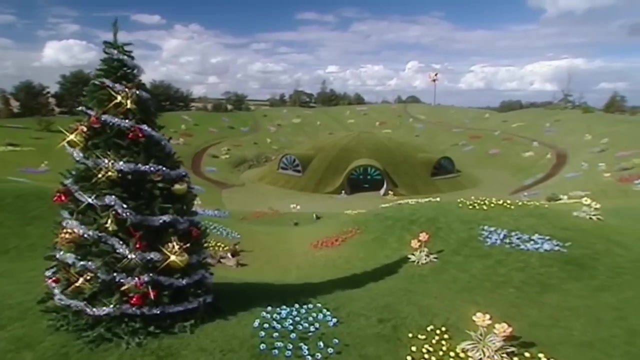 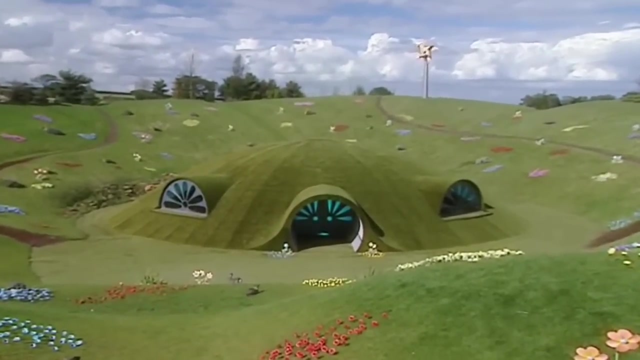 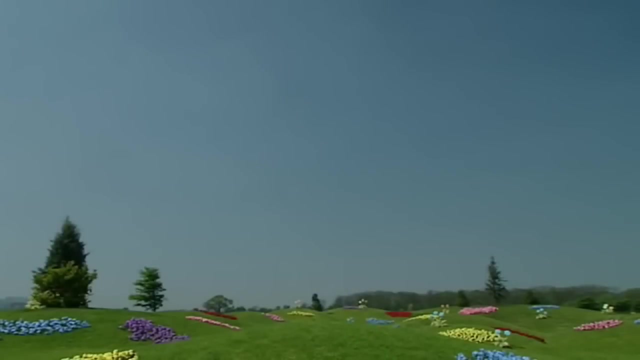 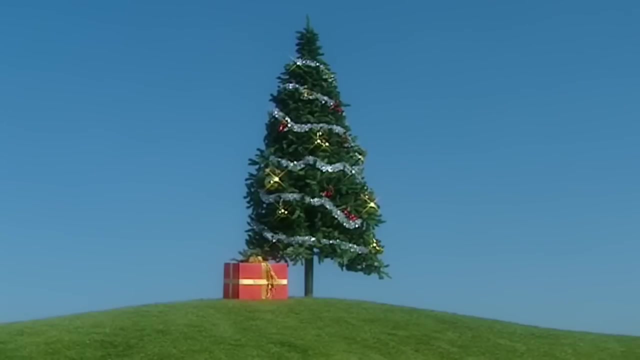 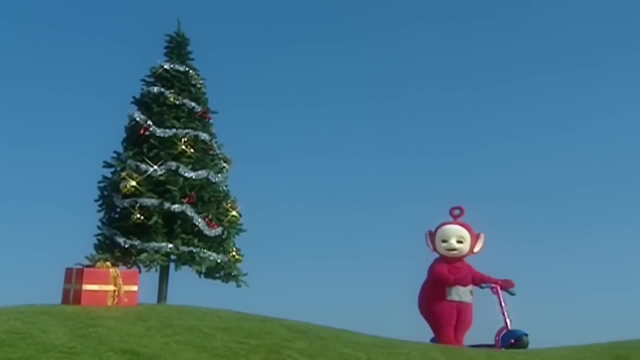 Cough, cough, cough, cough, cough, cough. One day in Teletubbyland Poe had a present. Oh, Oh, Oh, Oh, Oh, Oh Oh. Poe's present, Oh, Oh, Look Oh. 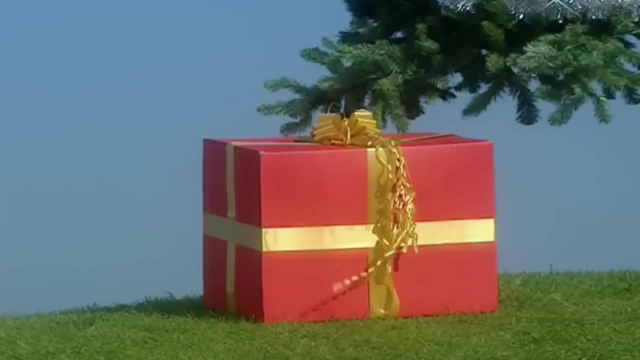 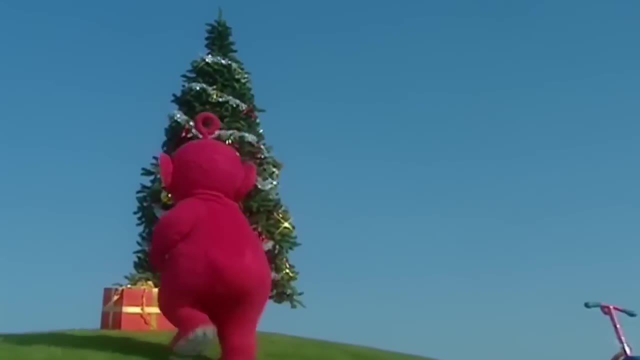 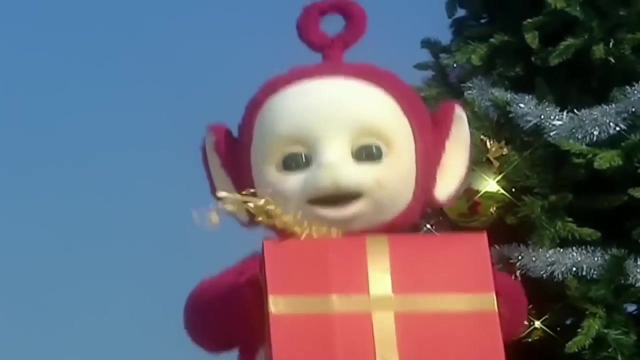 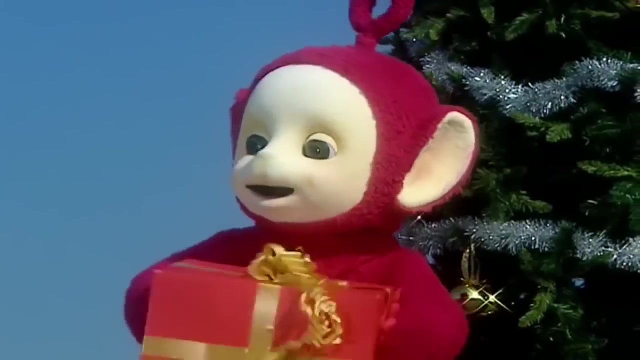 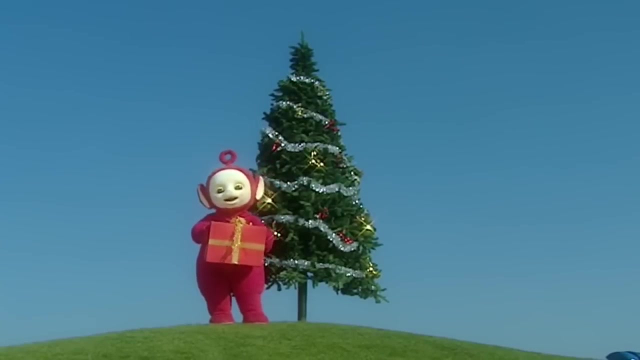 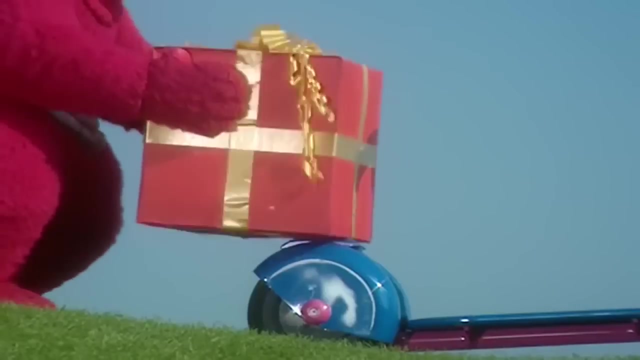 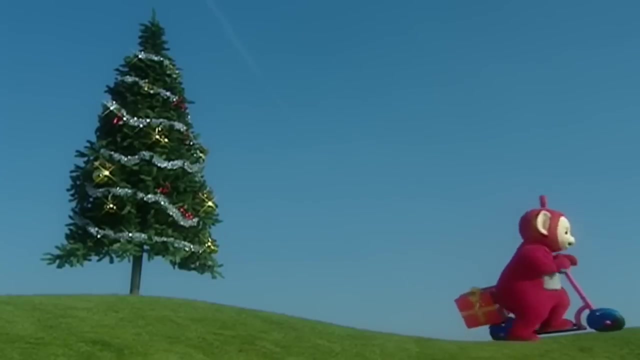 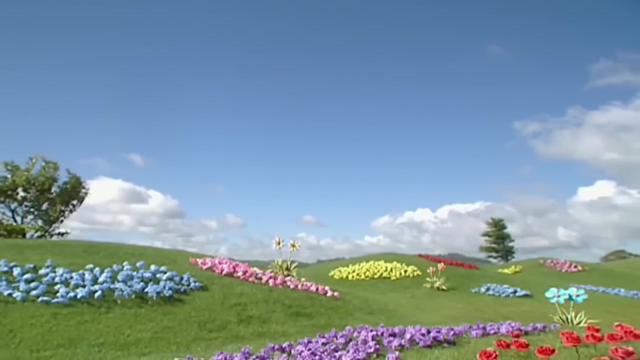 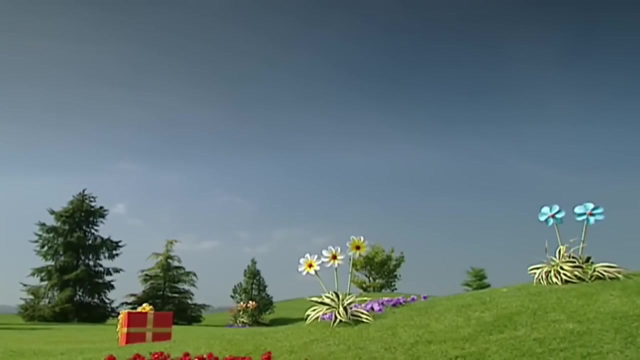 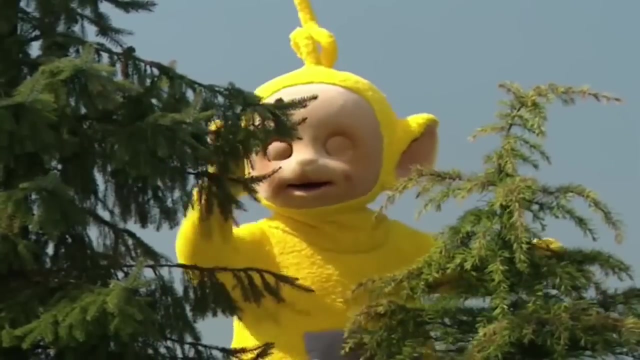 Oh, Poe's present. Oh, Oh, Oh, Poe's present. Poe's present. Wow, La-li-la-li-la, la-li-la-li-la, la-la-li-la, Uh-oh, La-la saw that Po had left her present behind. 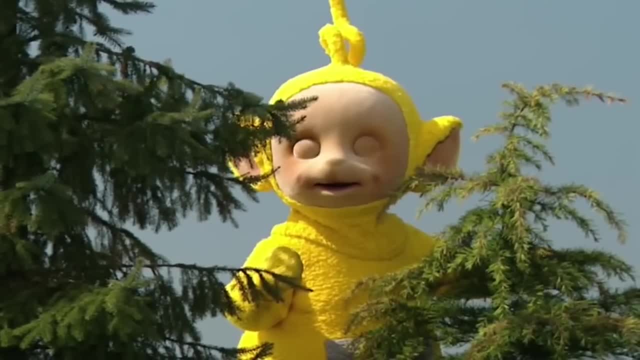 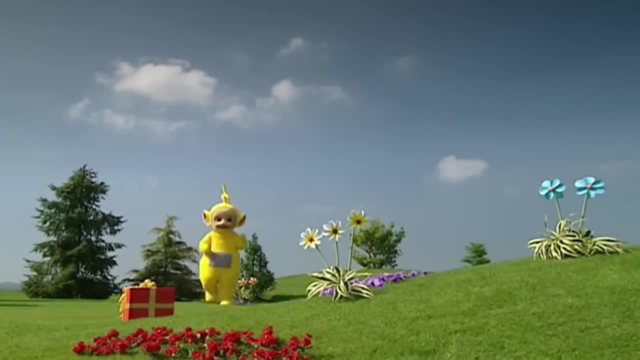 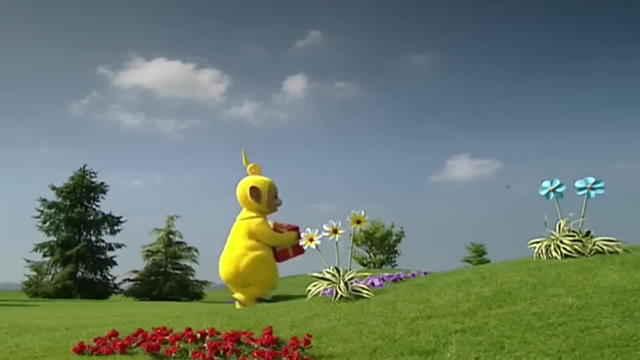 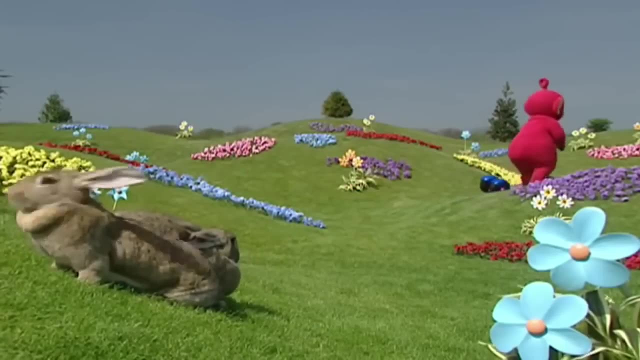 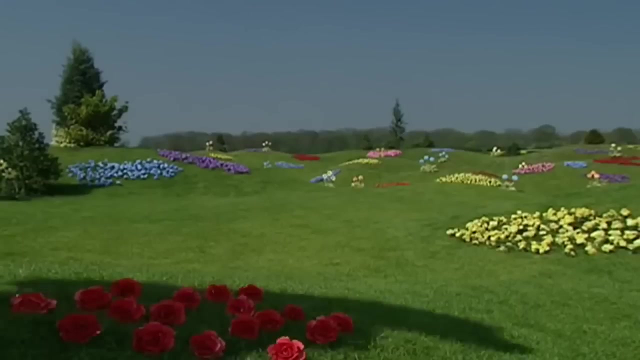 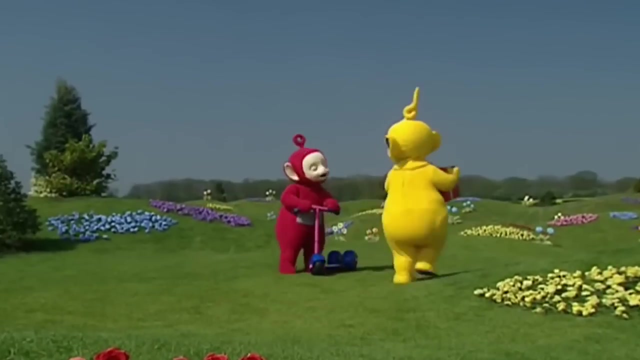 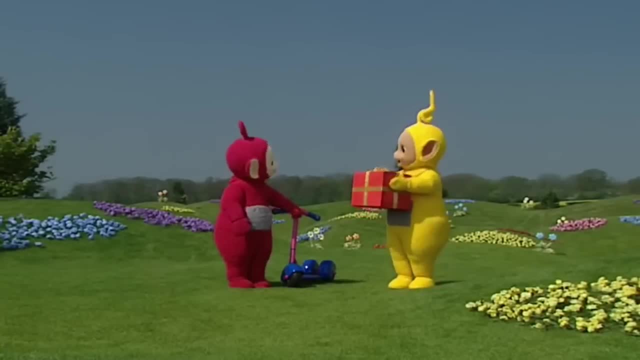 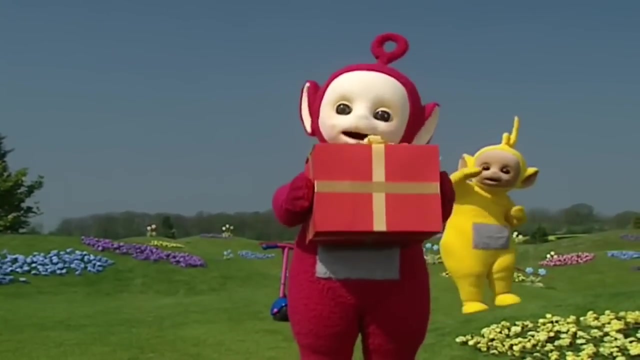 Po Po, Oh, Oh Po Oh La-Lo, Oh, Oh, Oh Po Oh La-Lo. Oh, Look, Happy present. Oh Oh-ooh Po was very happy to have her present back. 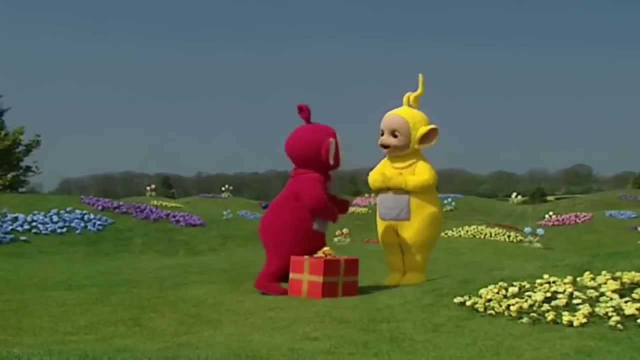 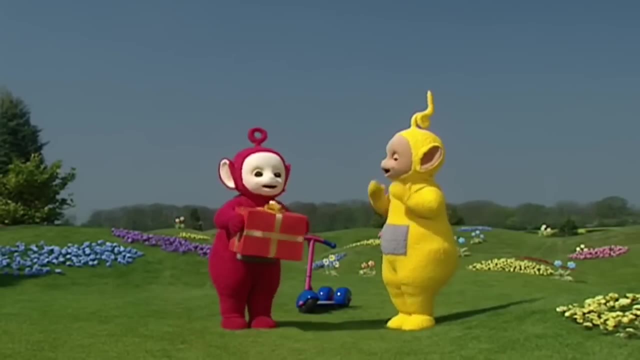 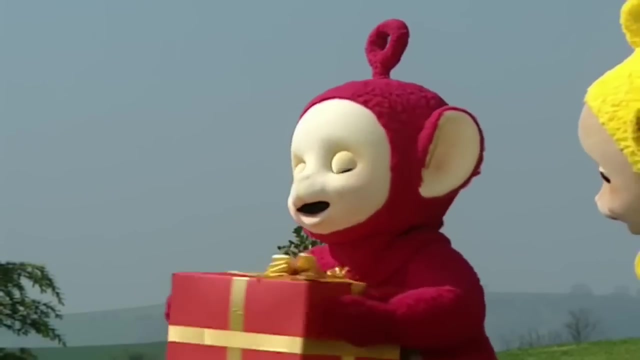 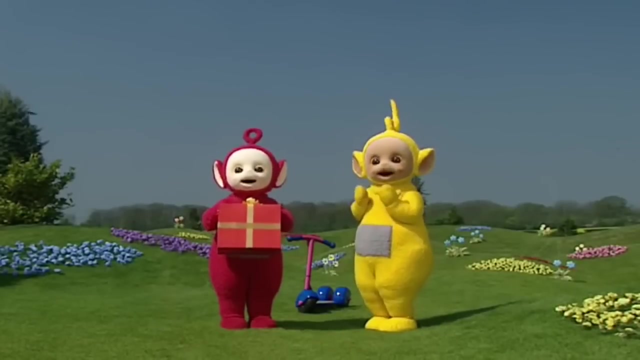 Aww, Peacock, Peacock, Ooh Present. Ooh, What's that? Ooh Poe decided to open the present Poe. up a present Poe. up a present Poe, up a present Ooh Ooh. 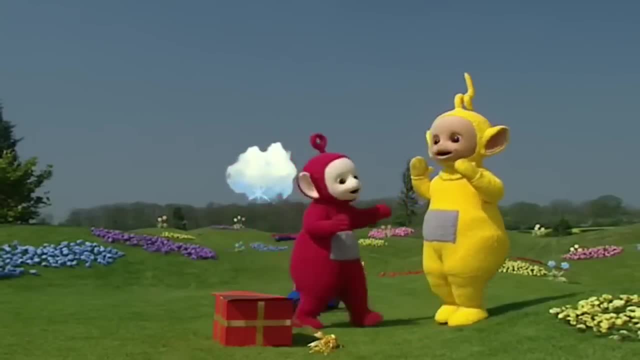 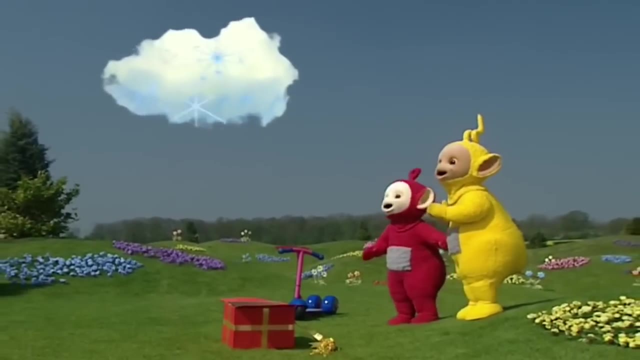 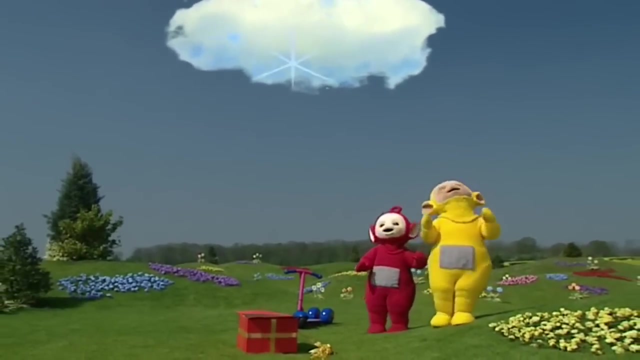 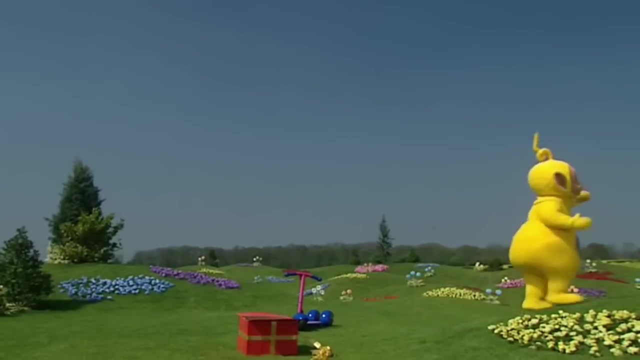 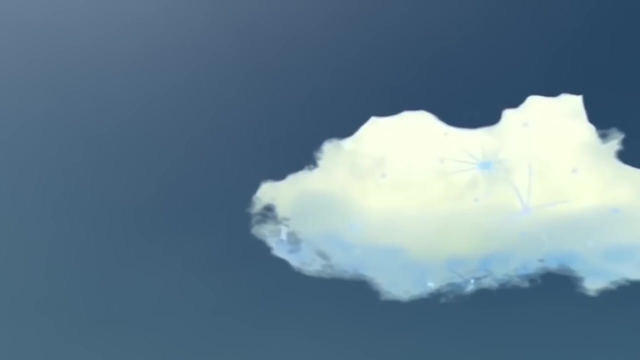 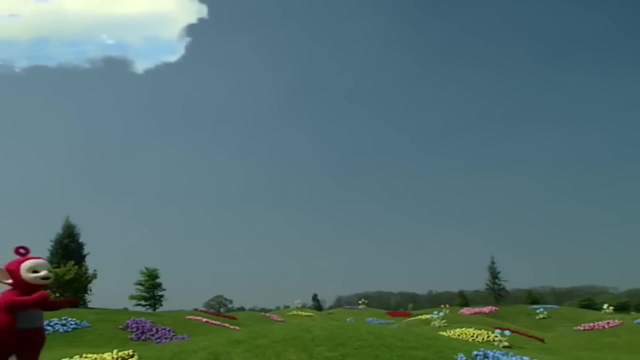 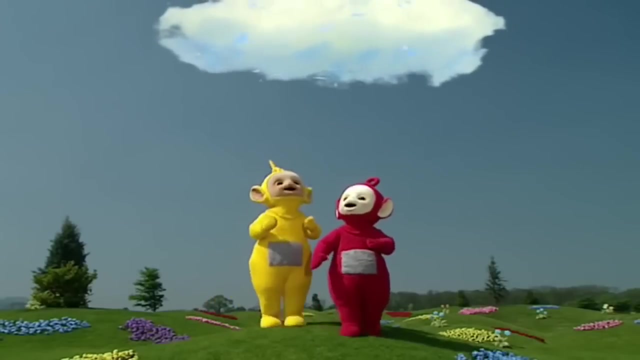 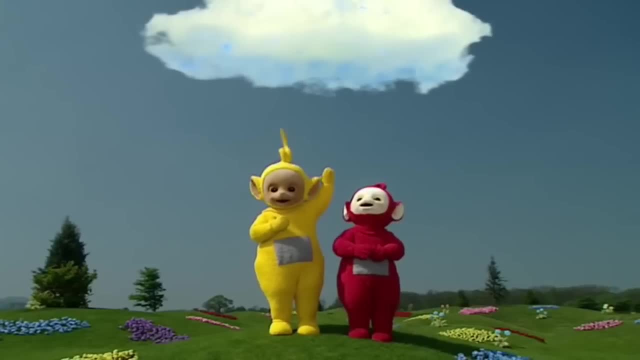 What's that? What's that? What's that? It was a little frosty cloud, Ooh, Ooh, Ooh, Little frosty cloud, And the little frosty cloud began to snow. Oh, Oh, But But. 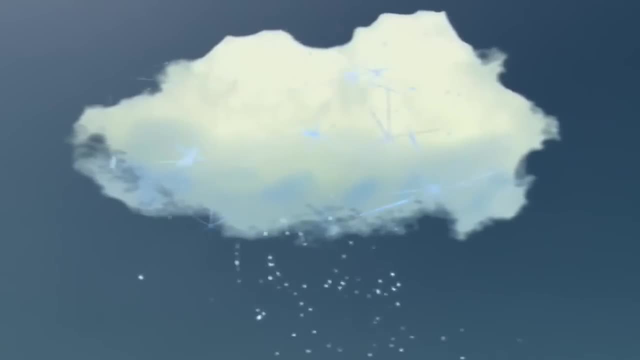 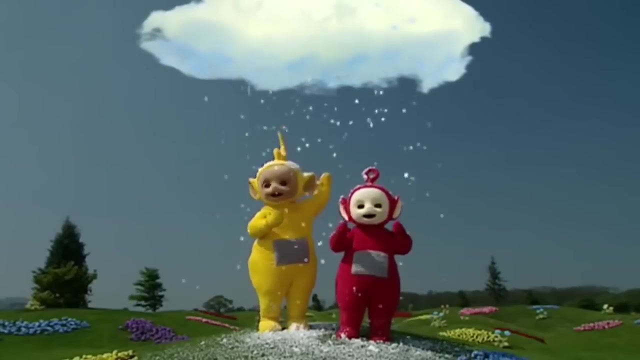 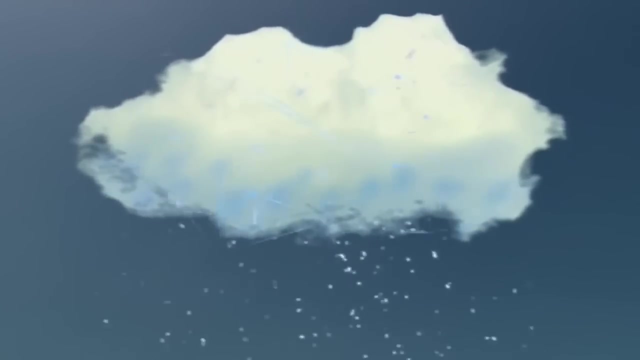 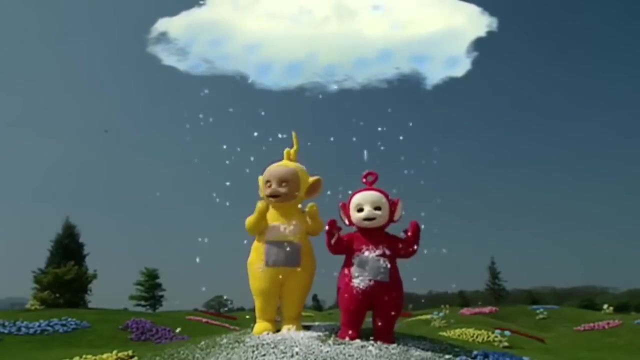 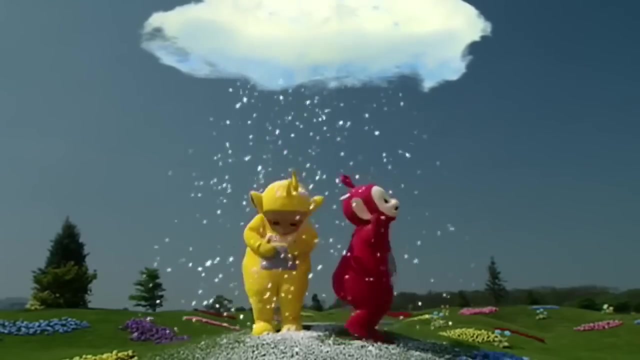 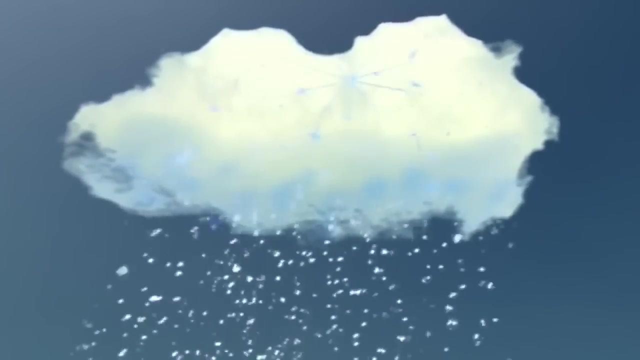 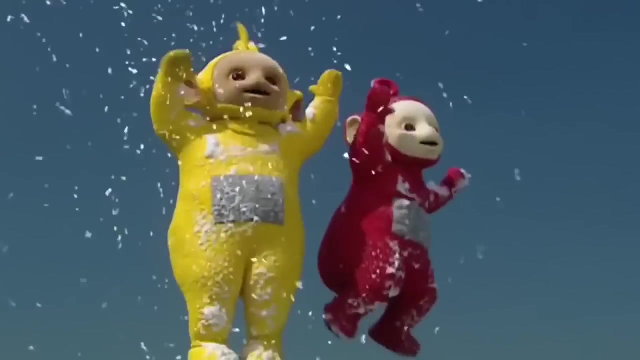 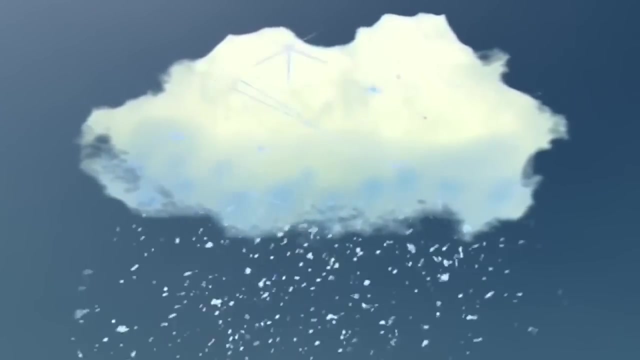 Ooh, Ooh, S'stop. What's that? It's all fuzzy candy. No, S'stop, No, S'stop, Oh, Stop, Hey, No, no, no, Stop. Tinky, Winky and Dipsy came to see the snow. 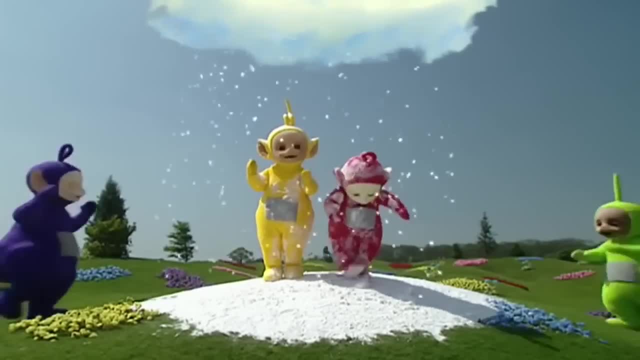 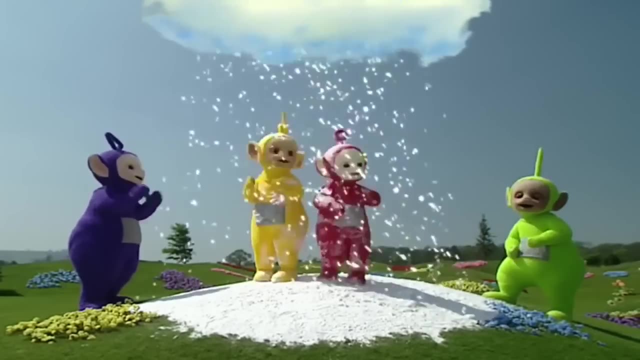 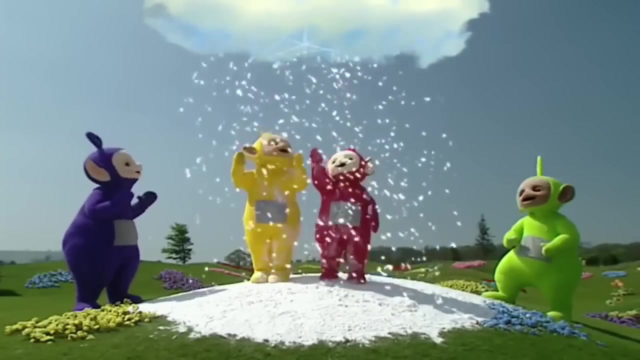 Oh, Oh, Oh, Oh, Oh Oh. Uh-oh Po, Uh-oh Nana, Uh-oh Tinky Winky, Uh-oh Dipsy, Look, Ooooh, What's that? 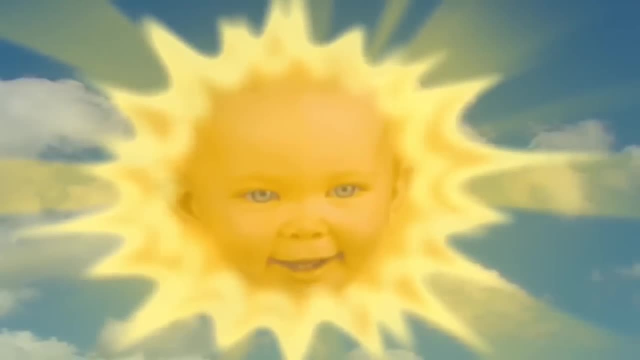 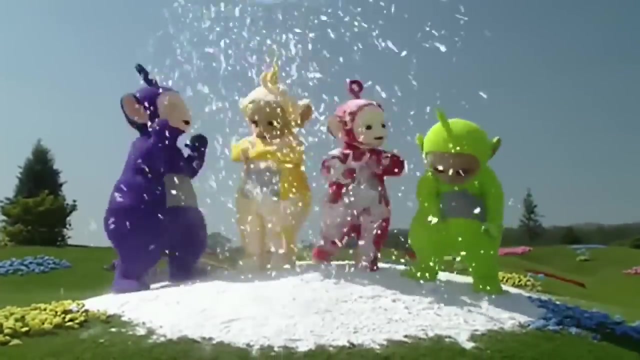 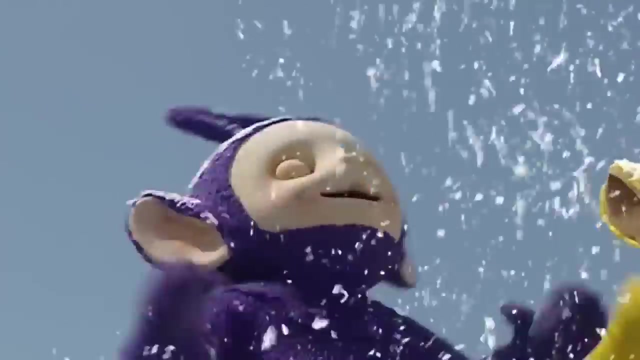 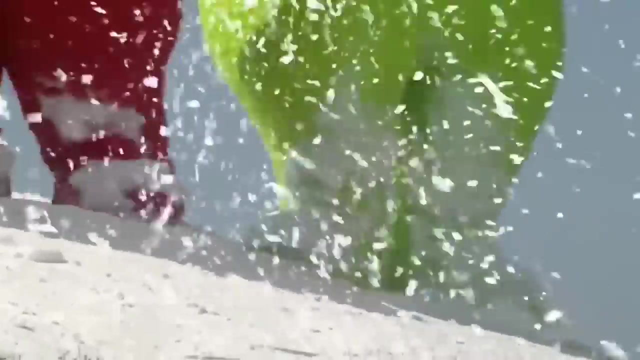 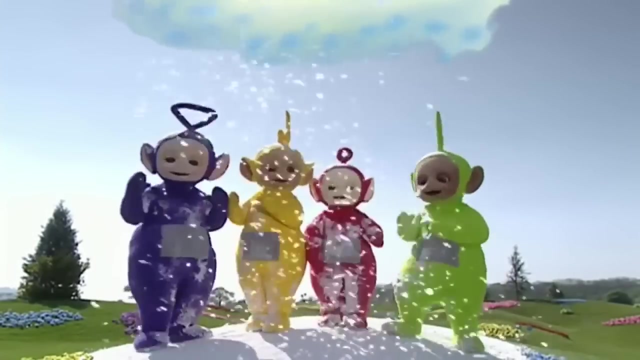 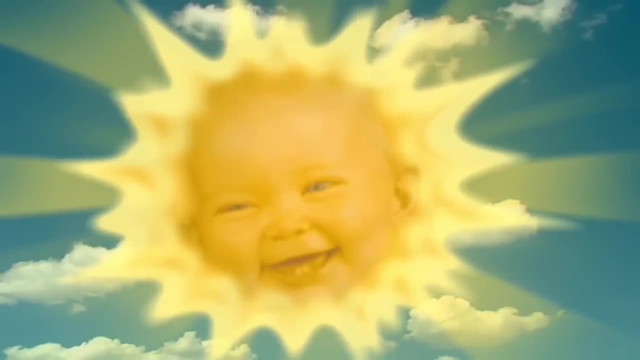 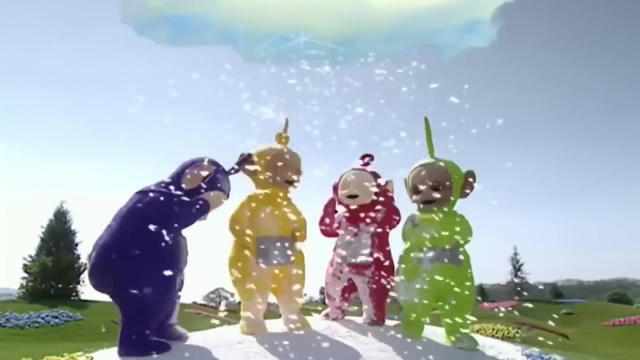 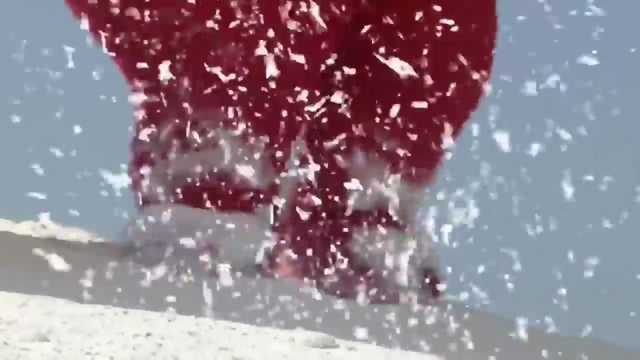 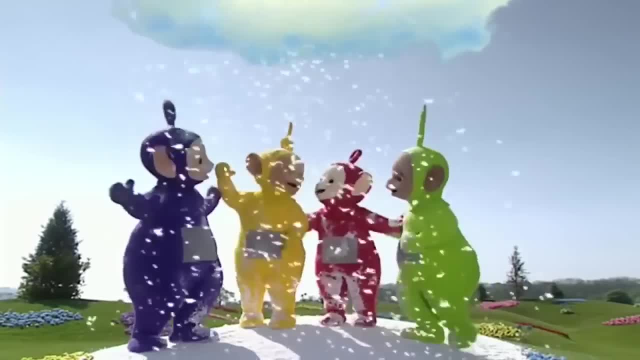 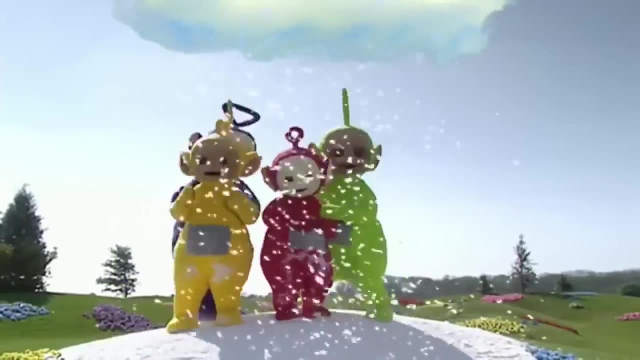 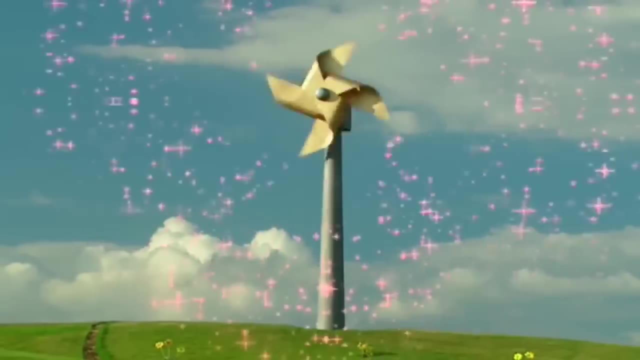 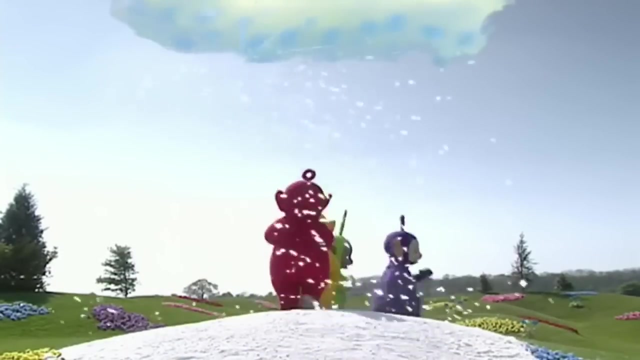 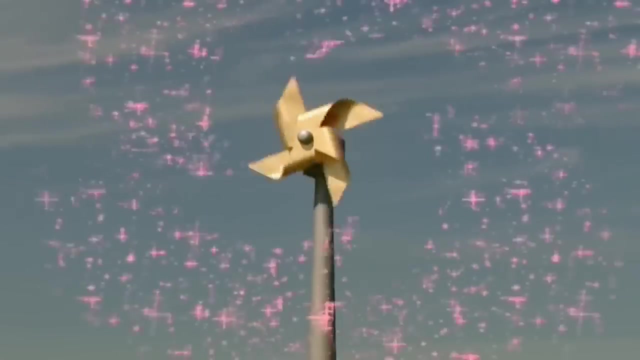 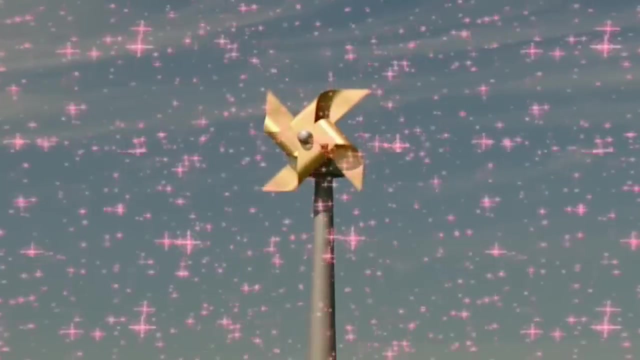 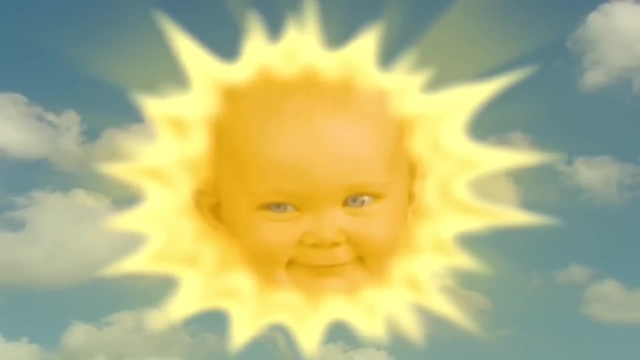 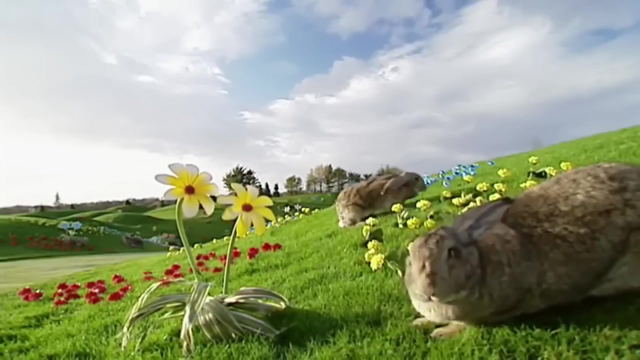 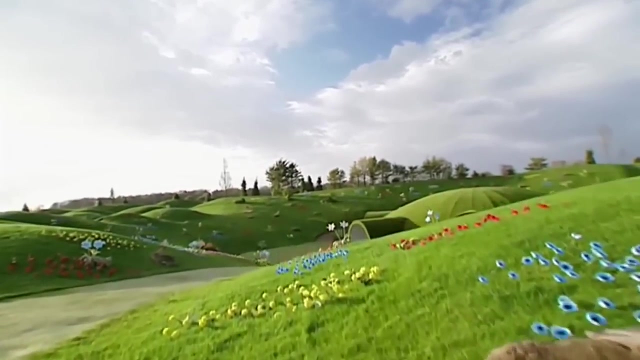 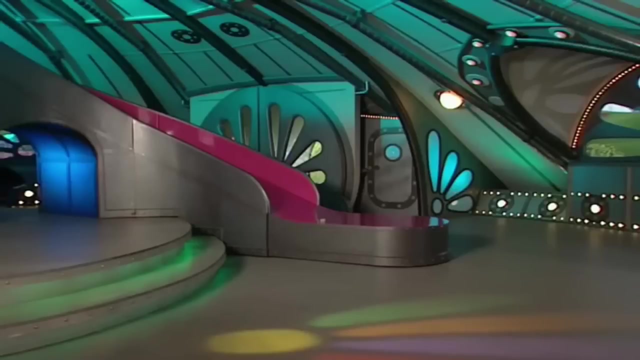 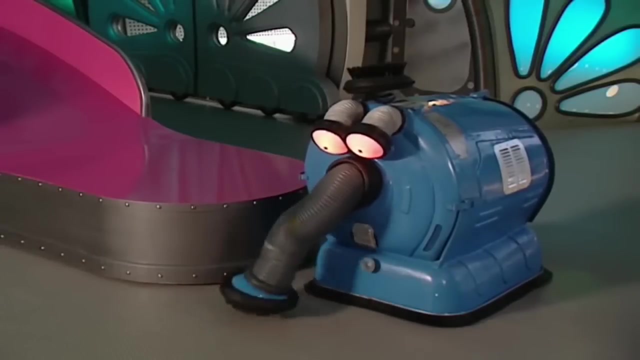 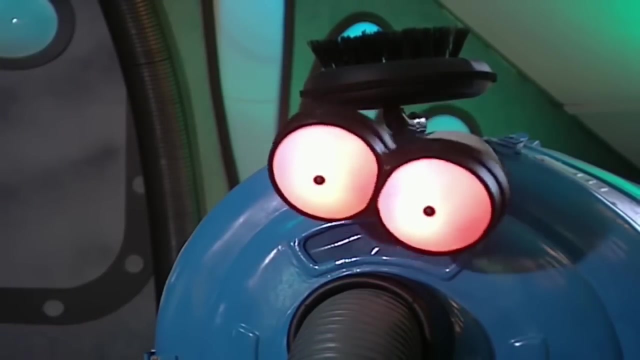 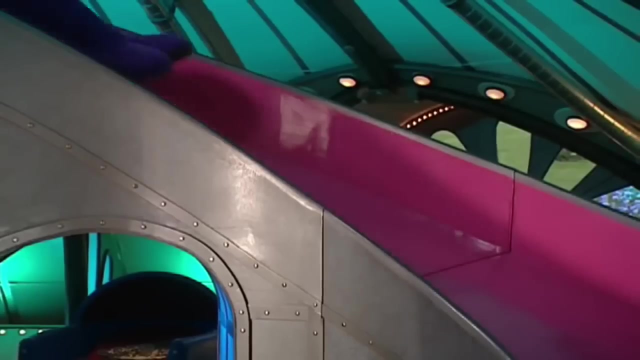 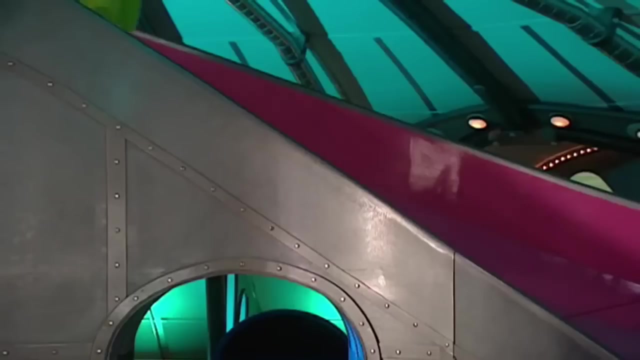 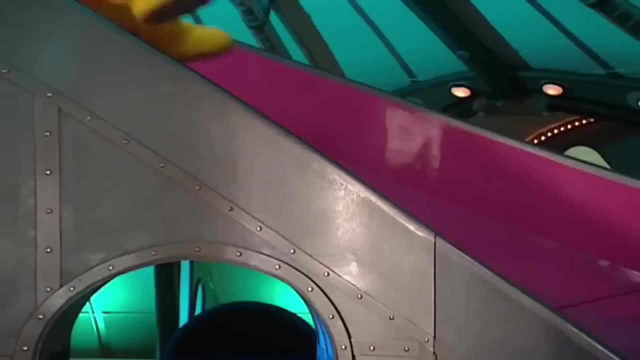 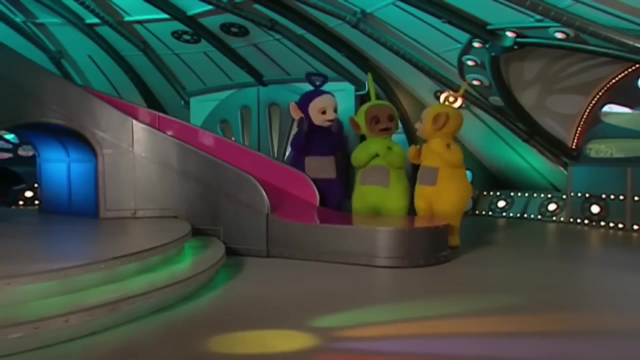 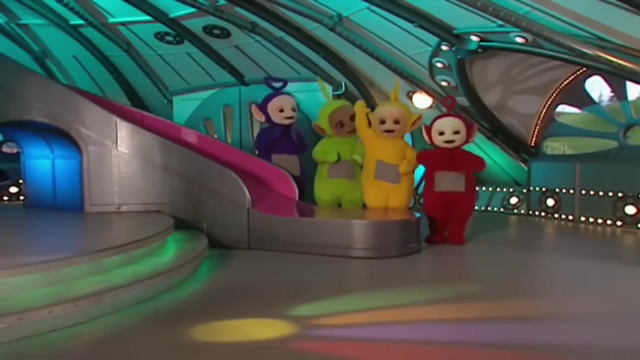 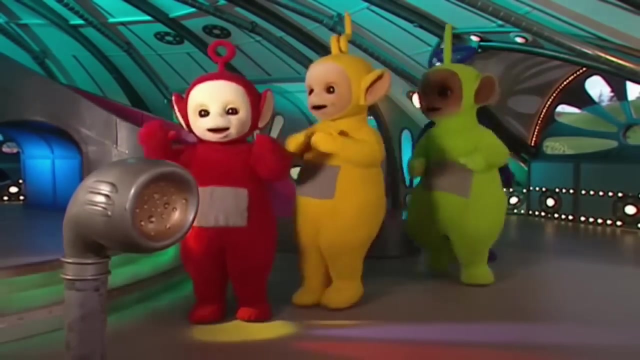 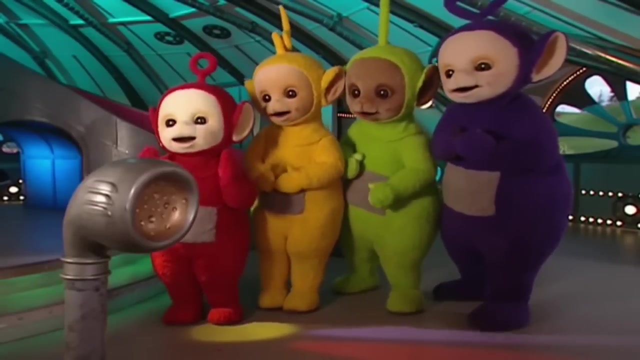 Because, Uh-oh, Uh-oh, Teletubbies love each other very much. Teletubbies love each other very much. Uh-oh, Christmases are coming and the goose is getting fat. Please put a penny in the old man's hat. 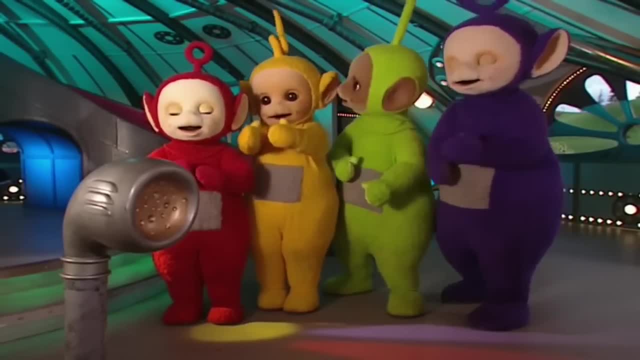 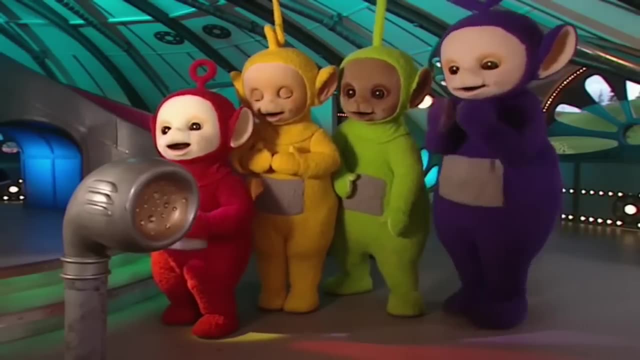 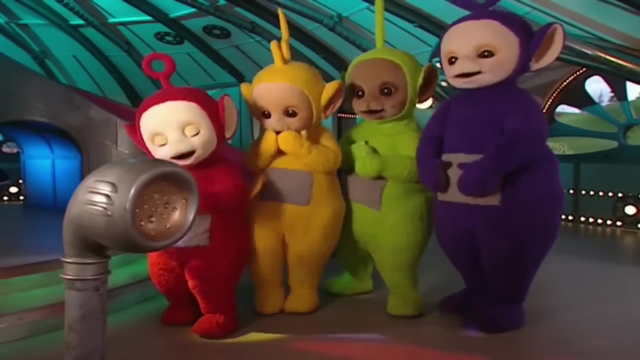 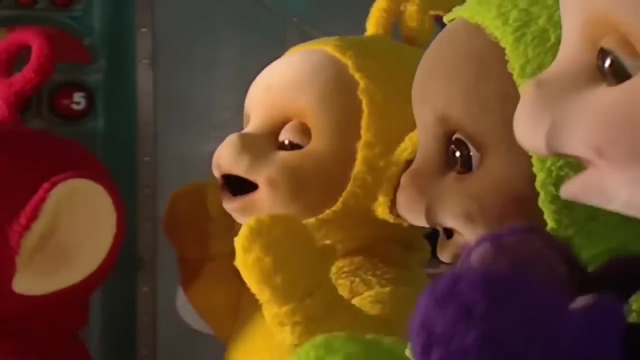 Ooh, Again, again, Again, again. Christmases are coming and the goose is getting fat. Please put a penny in the old man's hat. Uh-oh, Uh-oh, Christmases are coming and the goose is getting fat. 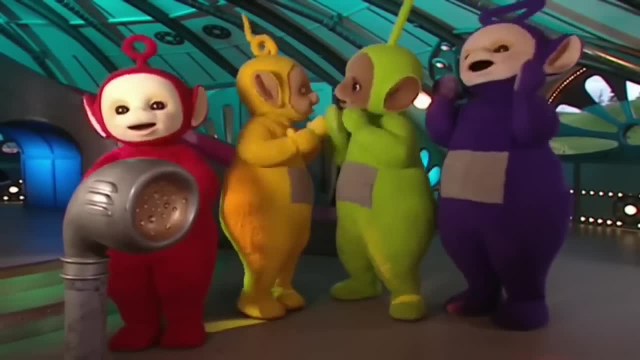 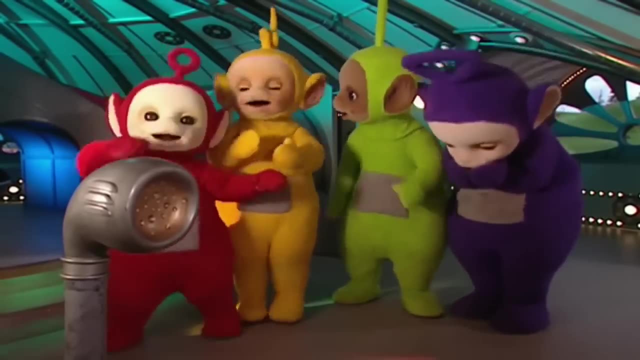 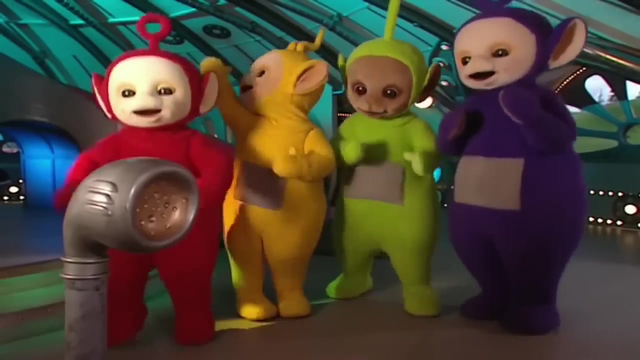 Please put a penny in the old man's hat. Remember the old man's hat. Christmas is coming. Christmas is coming. Christmases are coming. Christmases are coming. Come in, Christmases are coming, Come in, Christmas is coming. 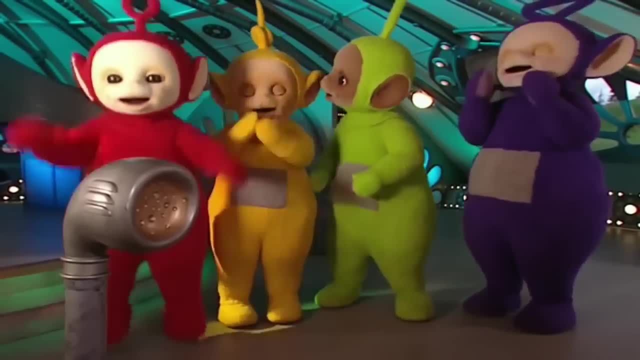 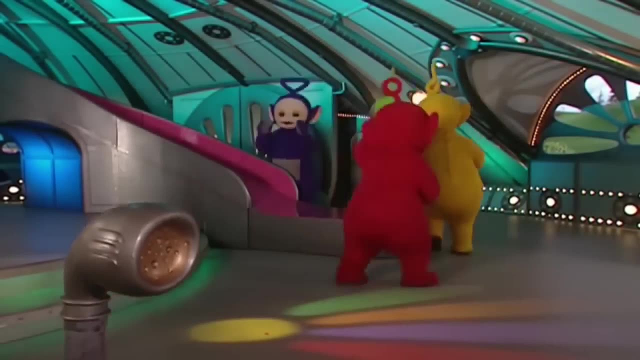 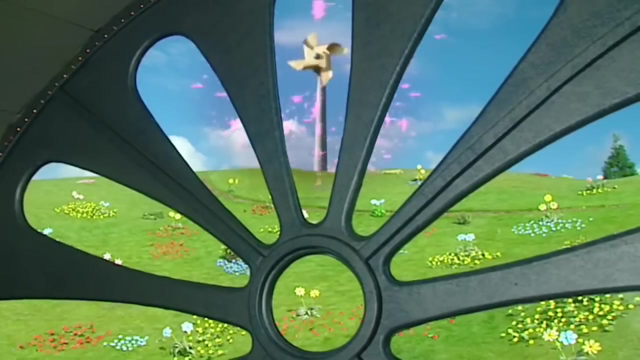 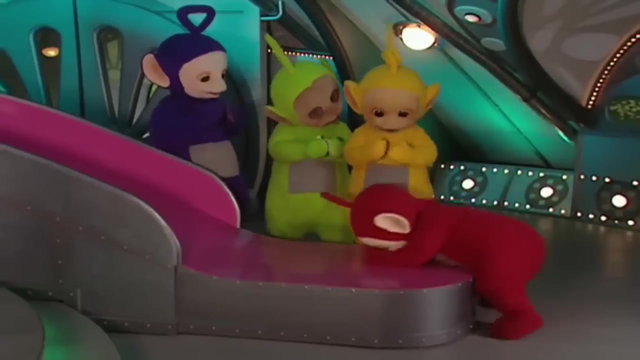 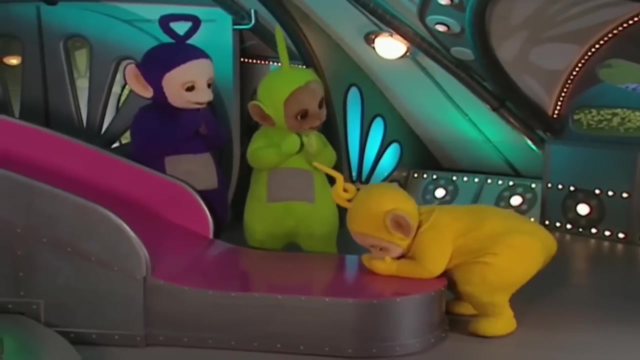 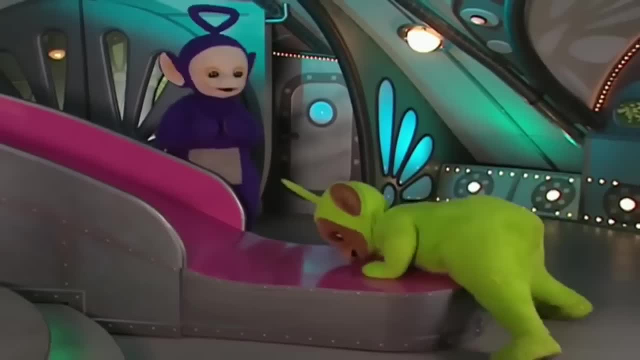 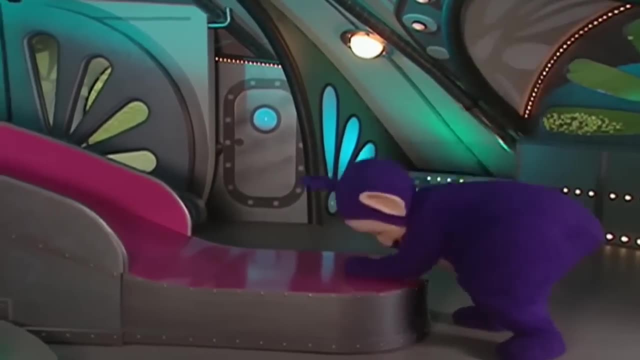 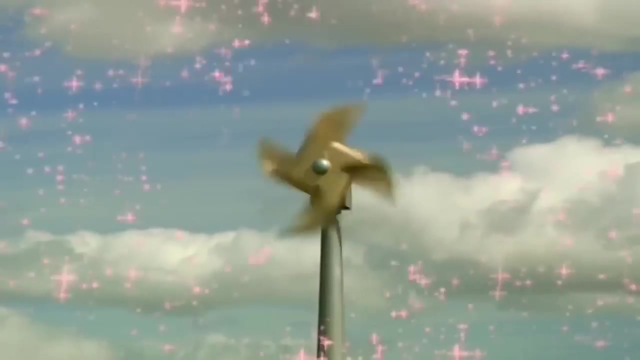 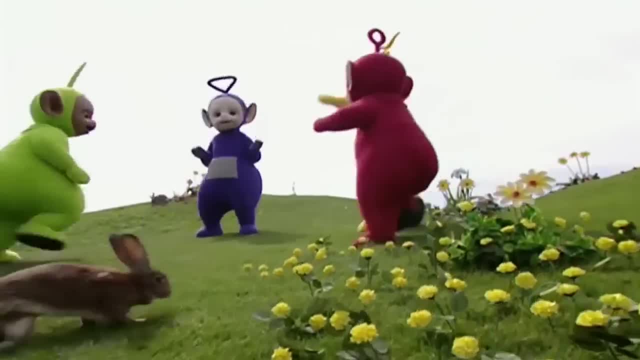 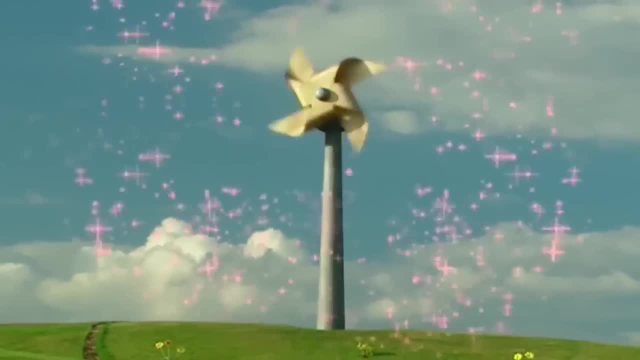 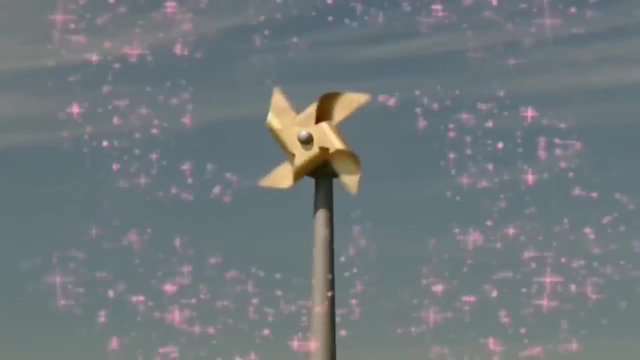 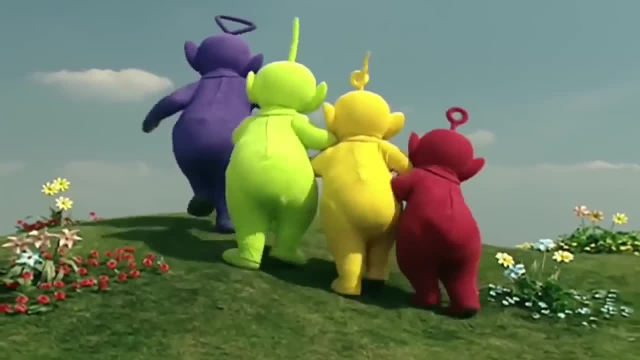 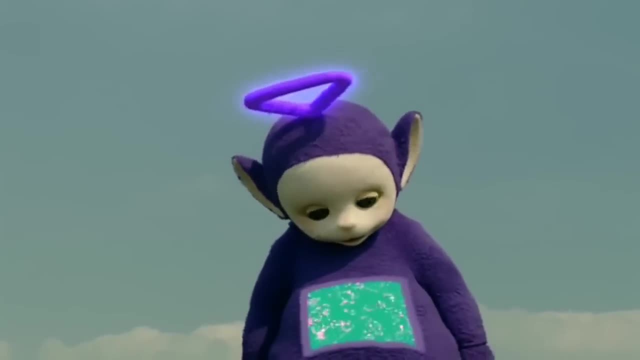 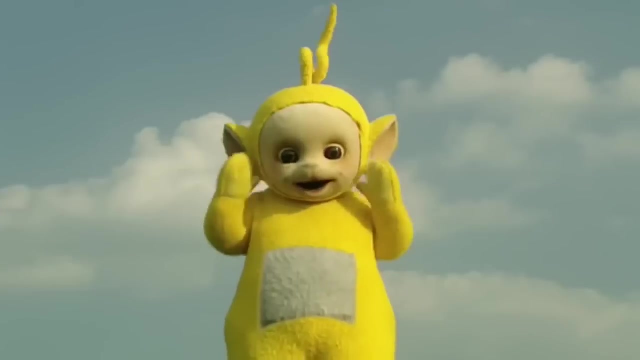 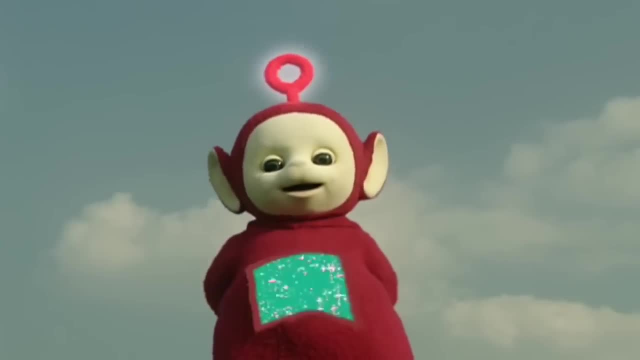 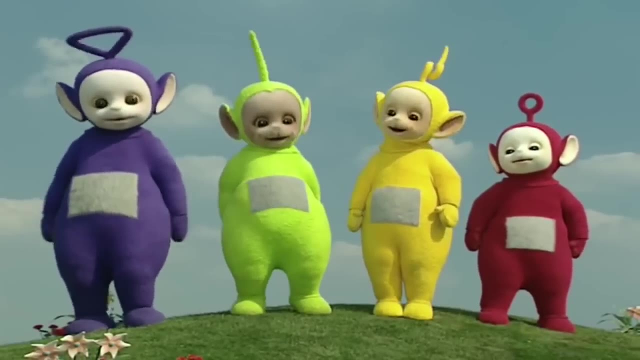 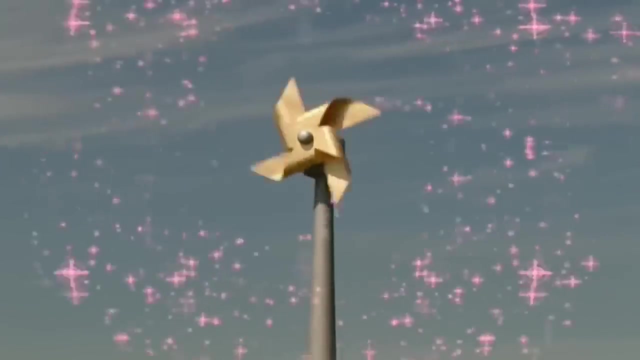 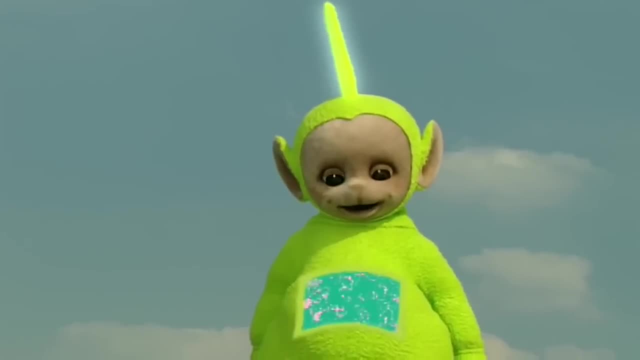 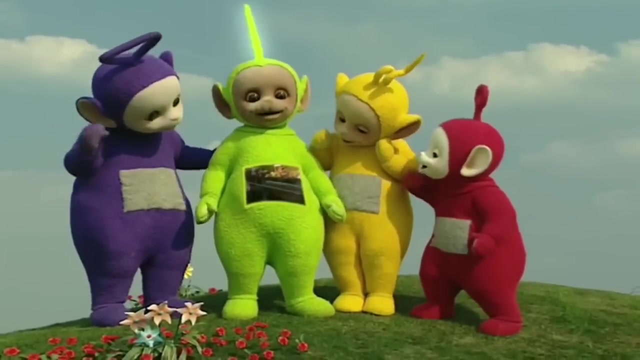 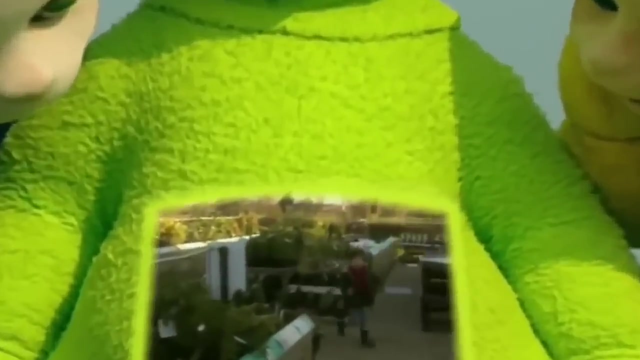 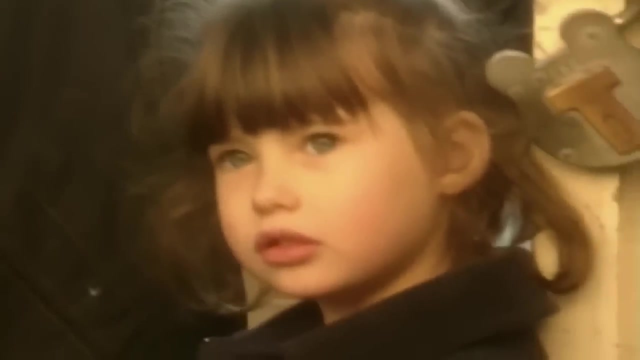 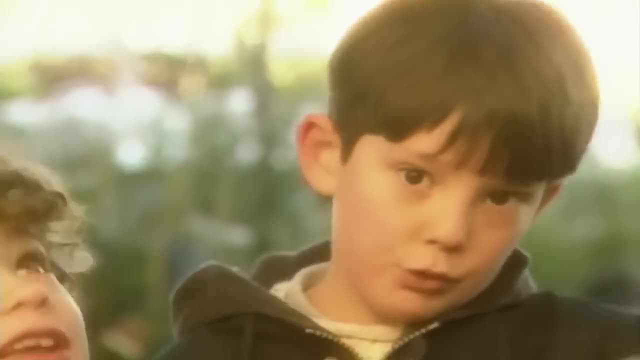 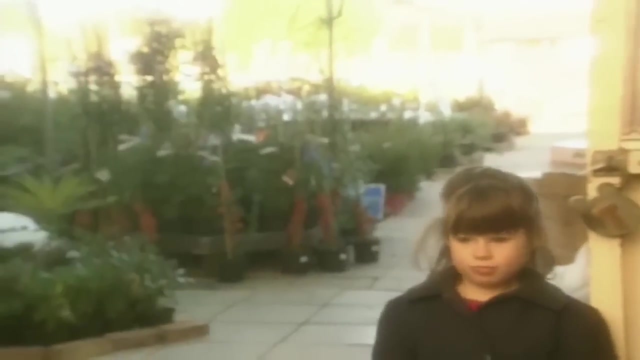 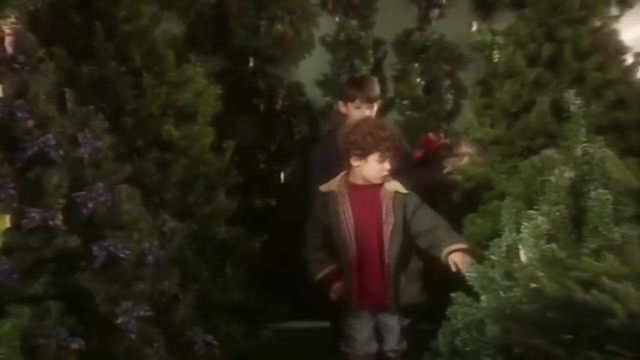 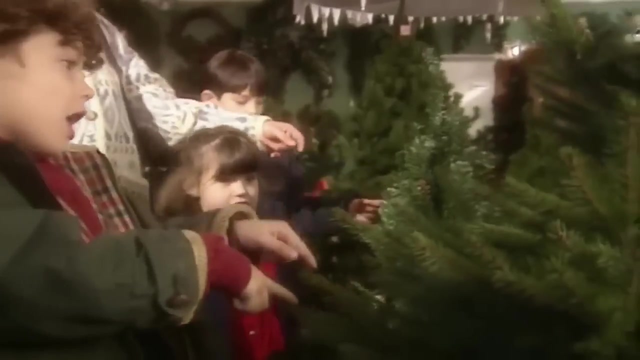 My name's Lewis. We're going to get a Christmas tree and then we're going to decorate it- Our Christmas tree. Mummy said we could have any tree we wanted. I like this one. Yay, This one. Yes, Yes, Yes. 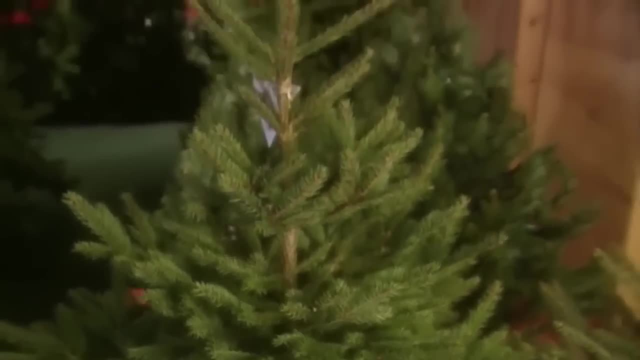 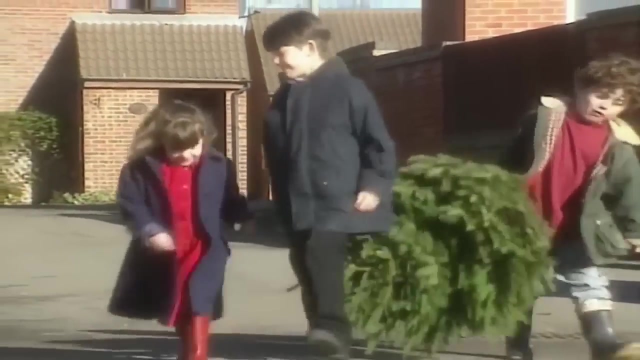 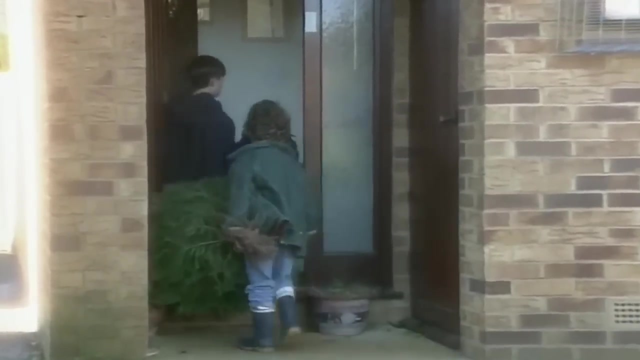 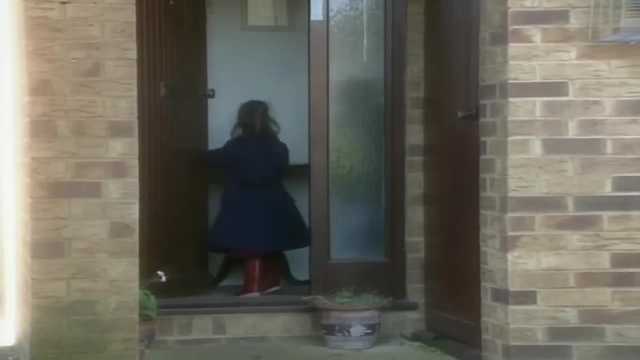 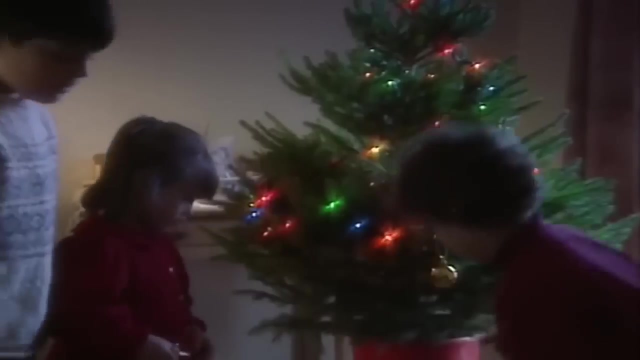 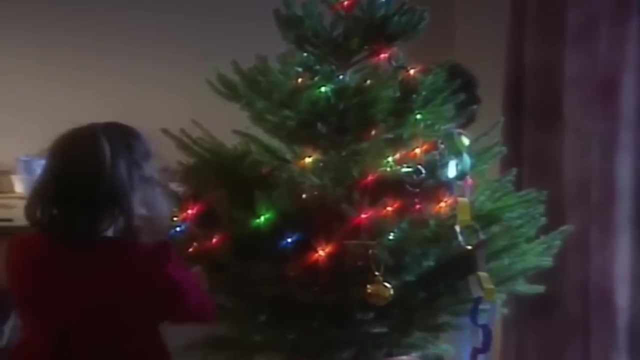 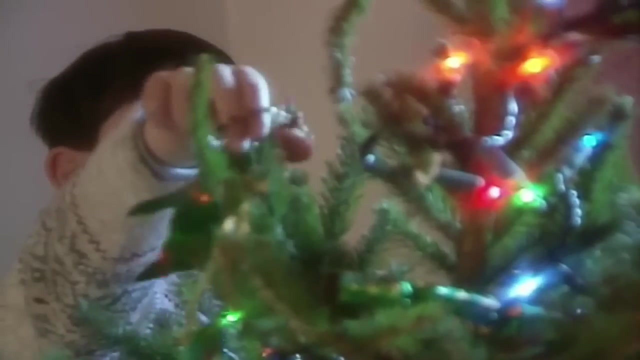 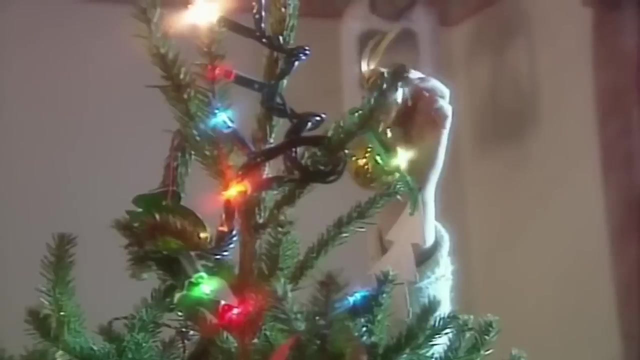 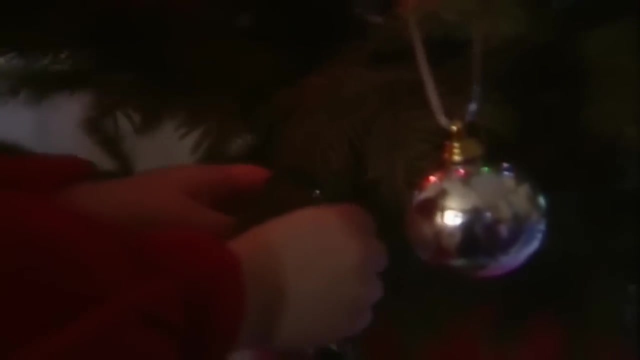 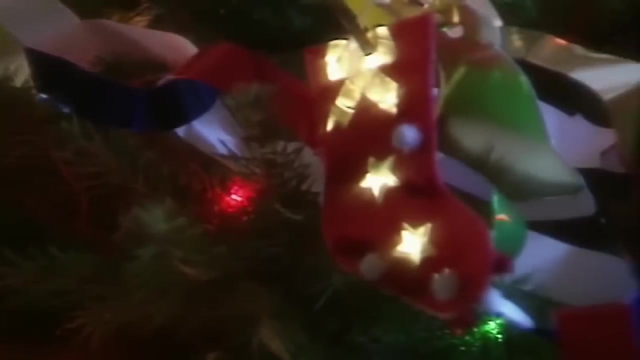 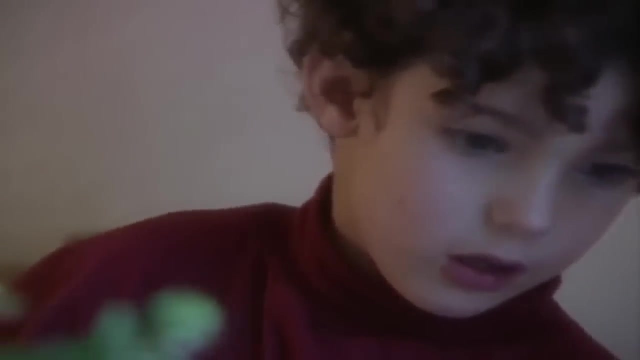 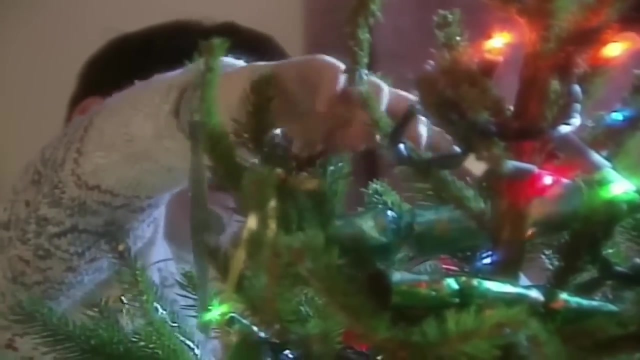 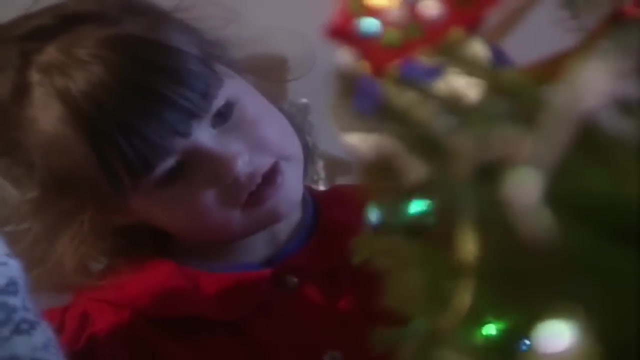 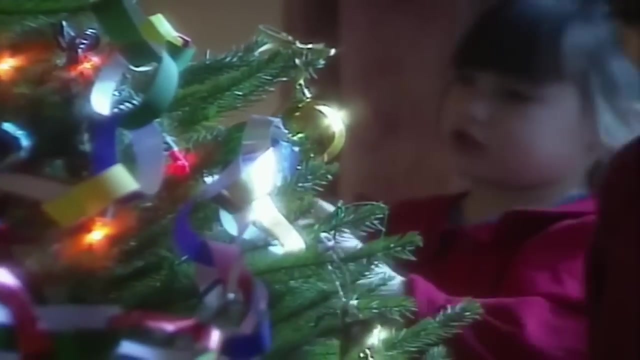 Oh, yes, we like this one. Come on, Come on, There it is. I like Christmas trees when they're decorated and sparkly like this Sparkly lights. I love decorated Christmas trees. I love decorated Christmas trees. Oh, I made this. oh, did I? 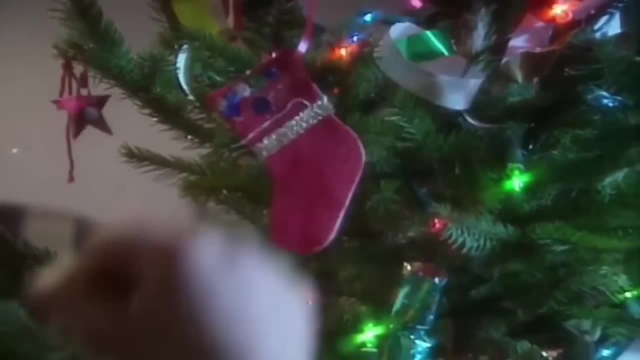 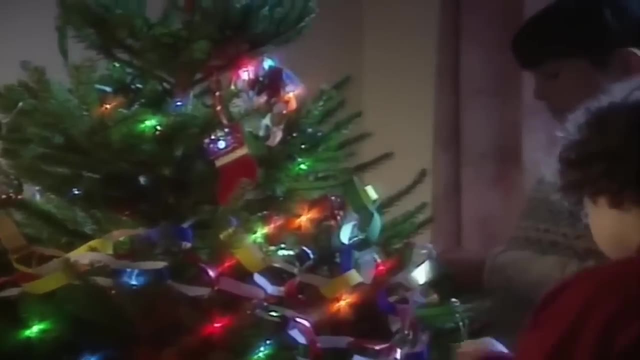 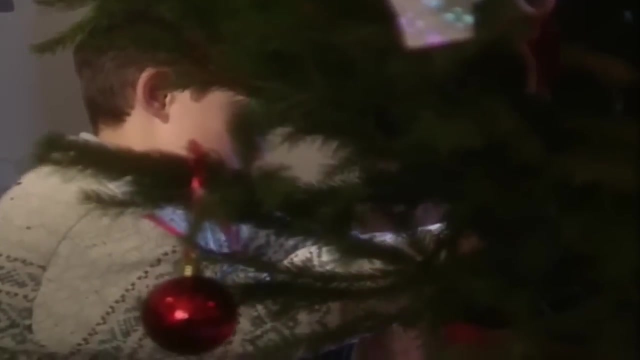 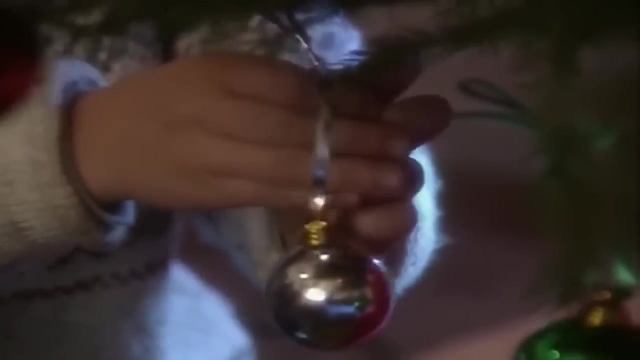 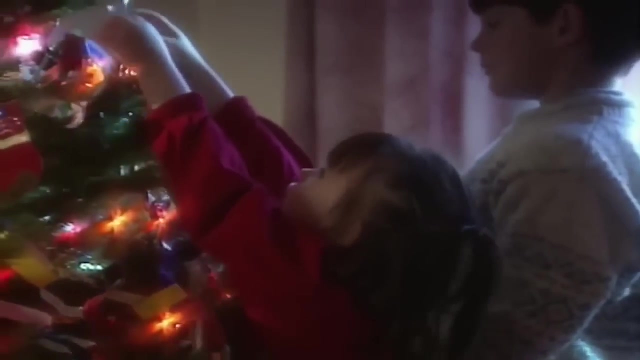 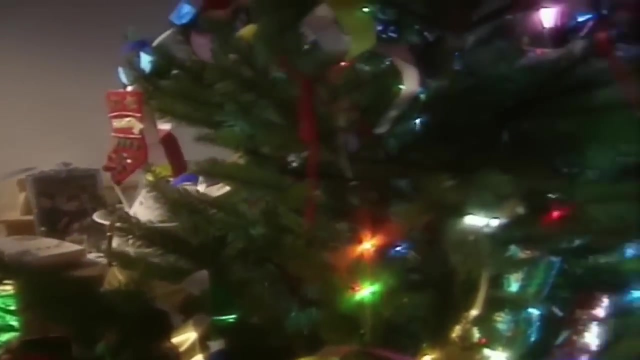 Oh, I made this. Oh, I made this. There's loads of them at the front. I'm putting some at the back now. I think I'll put that one back there. That's it. It's going to be the prettiest tree in the whole wide world. 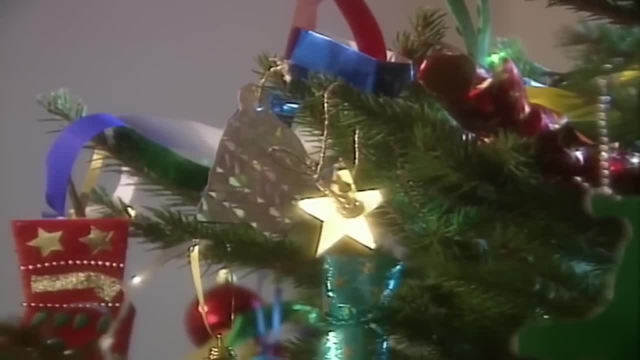 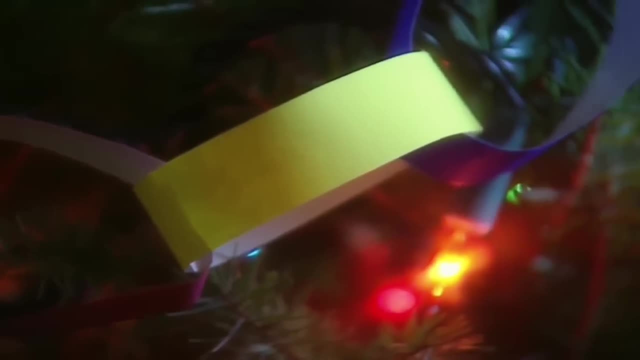 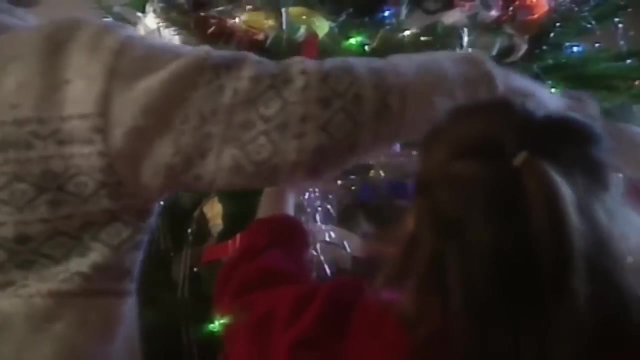 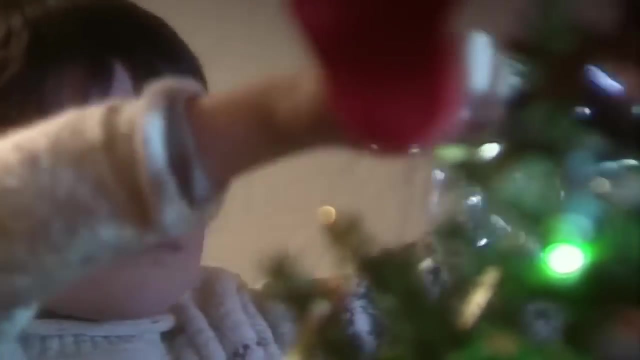 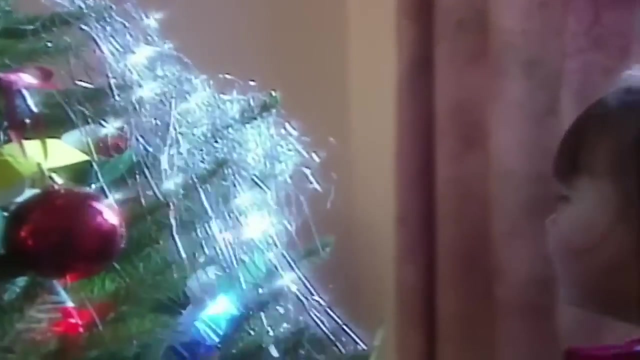 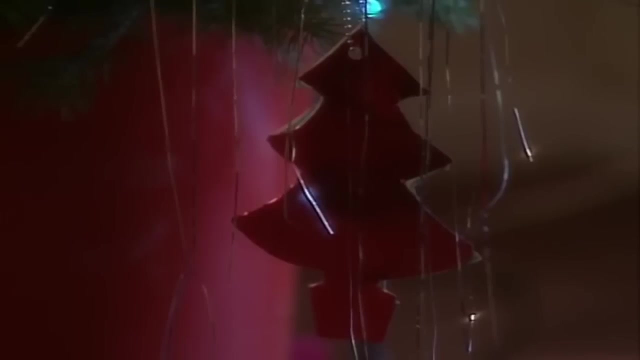 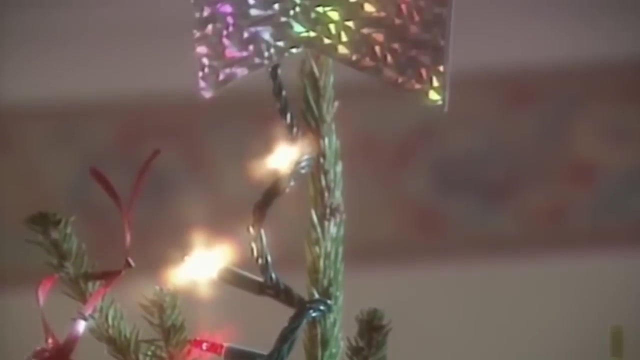 I like putting on the decorations I made. They look nice. I like these paper jets, what Lewis Jasmine and I made. It took us ages making this log. I love Christmas trees. I like that big star. I like that big star. 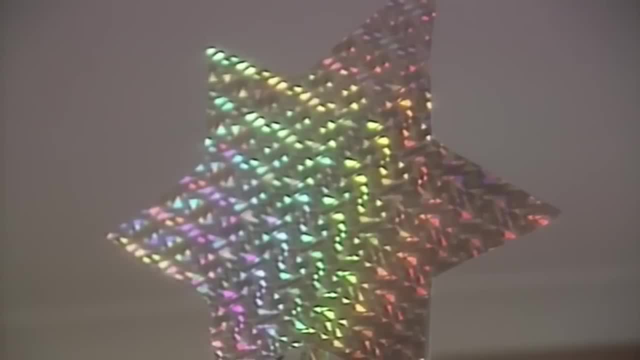 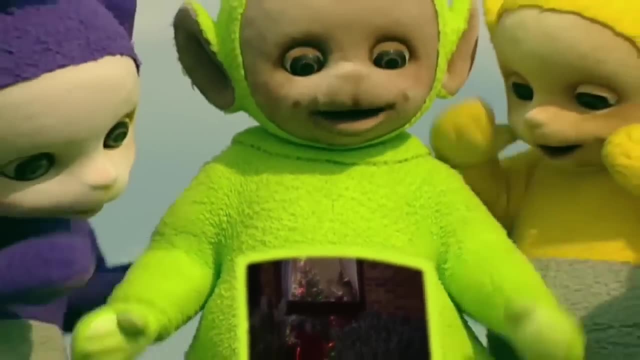 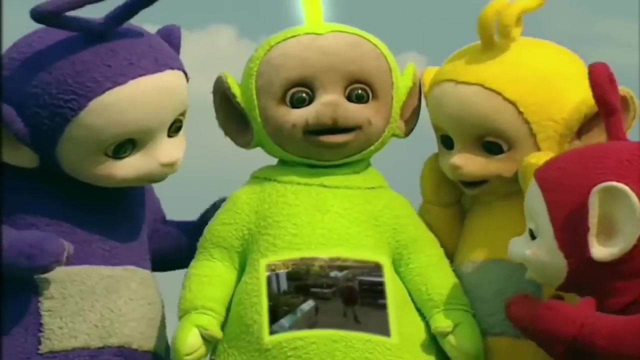 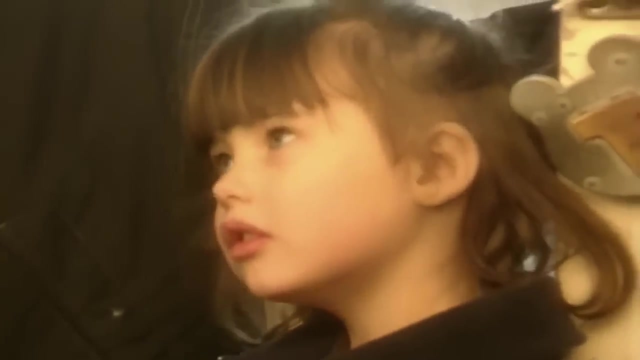 I like that big star on the top of the tree. Bye, Bye, Bye, Bye Again again, Again, again. Yay, Hello, Hello, Hello. My name's Elliot. This is my sister Jasmine. My name's Lewis. 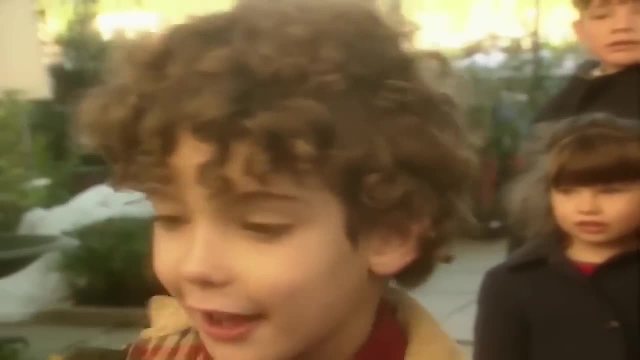 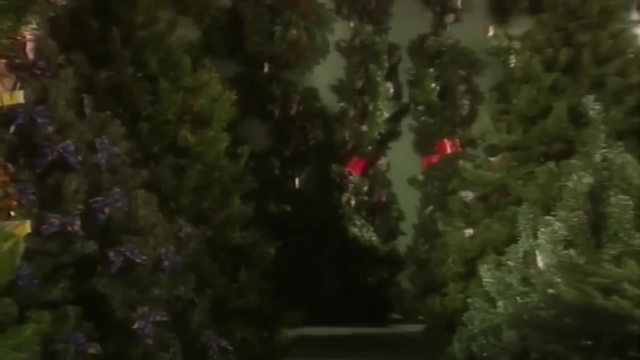 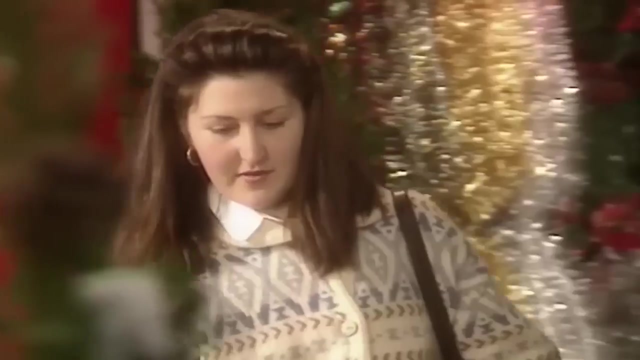 Welcome again. This is my sister, Jasmine. I'm going to decorate our Christmas tree. We're going to decorate our Christmas tree. Then we're going to decorate it, Our Christmas tree. Mummy said we could have any tree we wanted. I like this one. 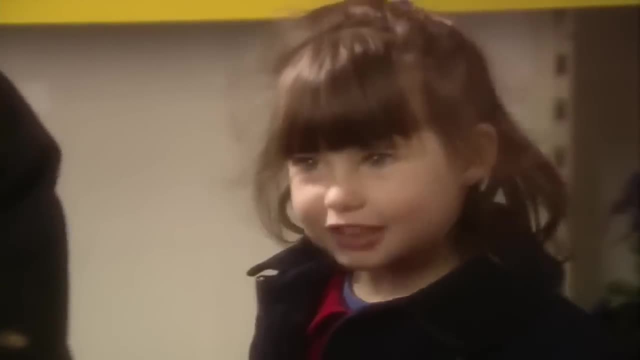 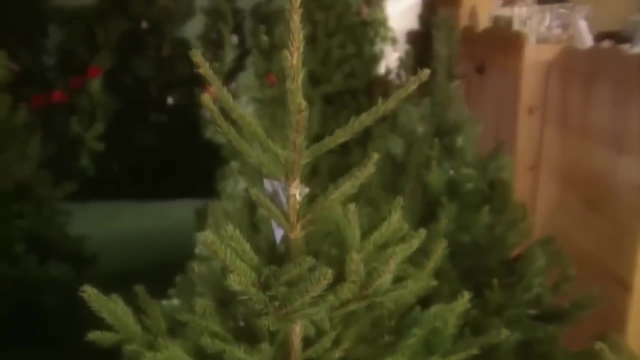 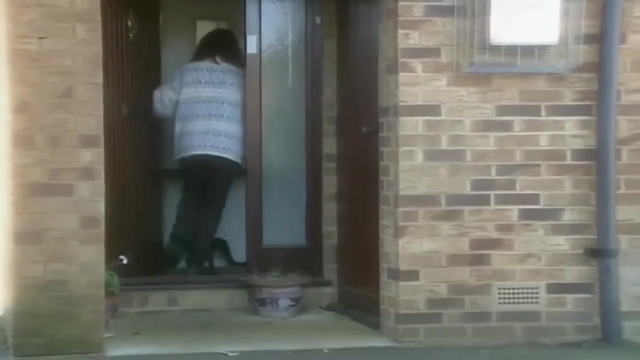 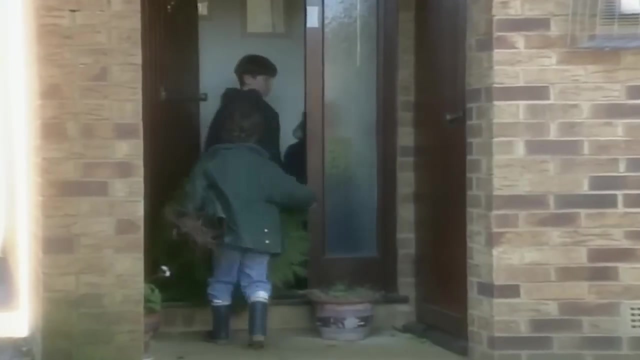 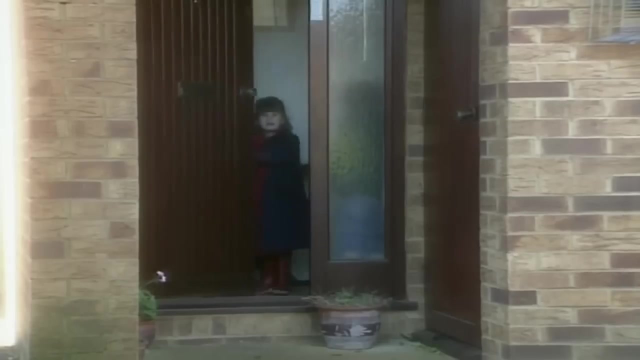 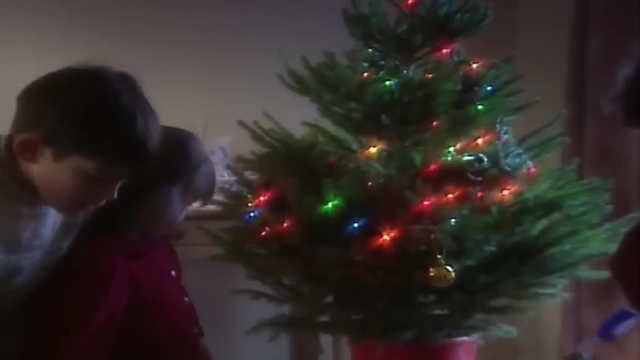 Yay, This one, Yes, Yes, Yes, Oh, yes, We like this one. This one, Yes, This one, Yes, Yes, This one, Yes, This is a Christmas tree for you. You can see this one. 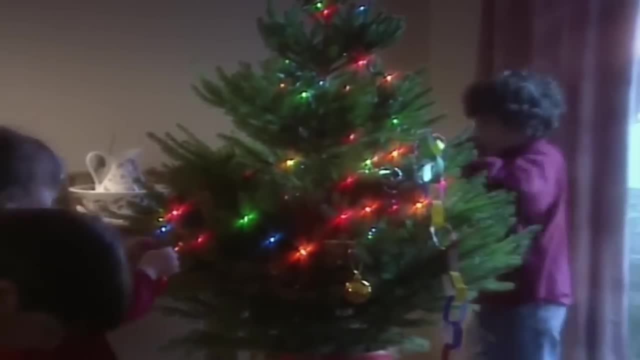 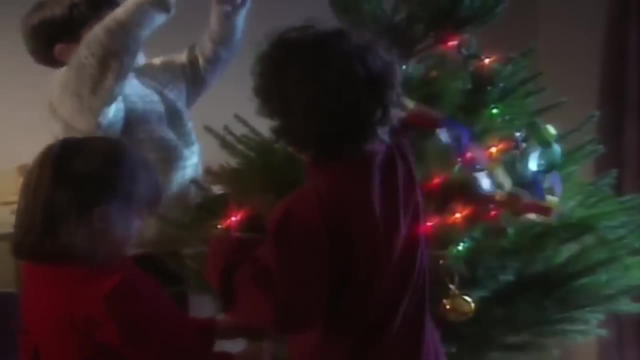 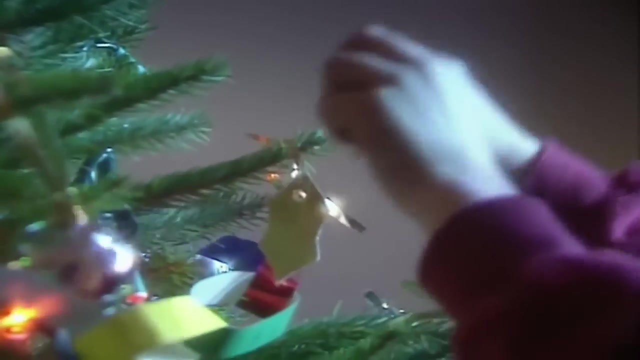 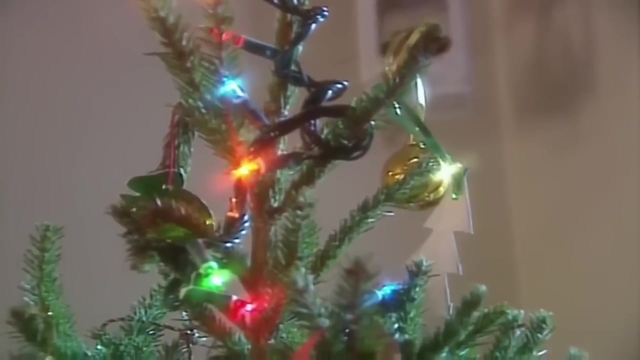 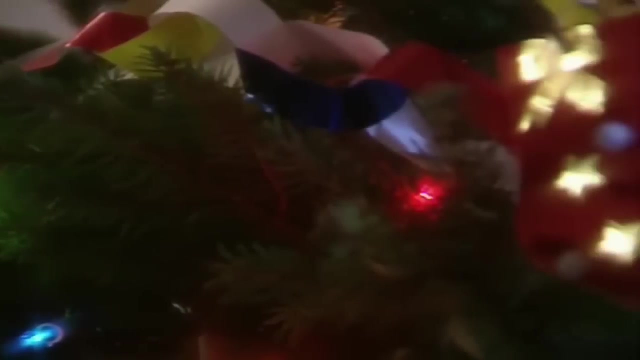 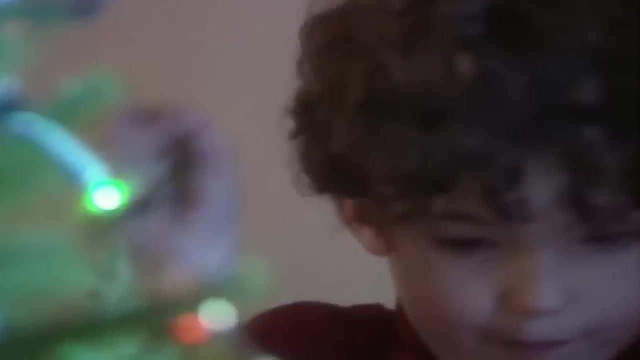 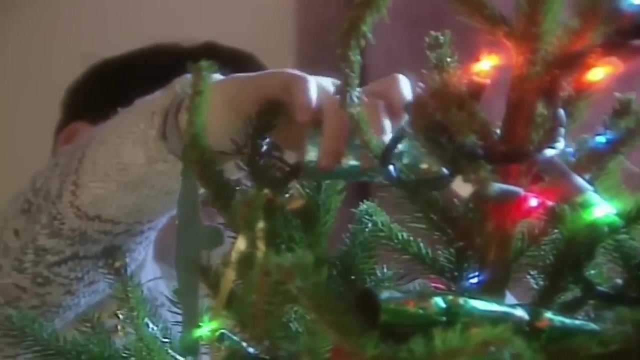 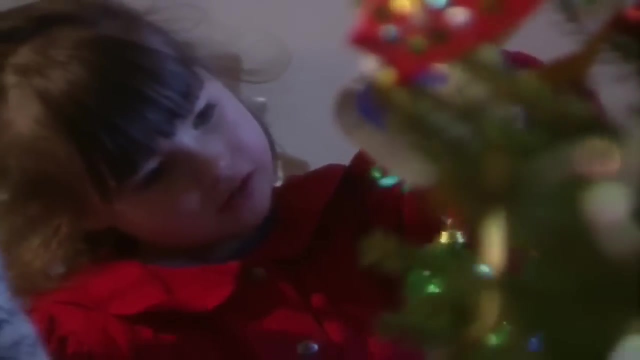 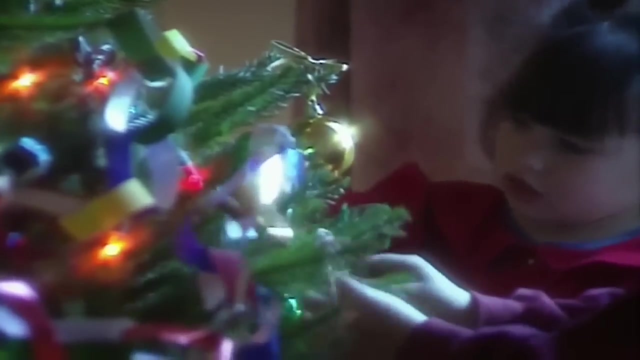 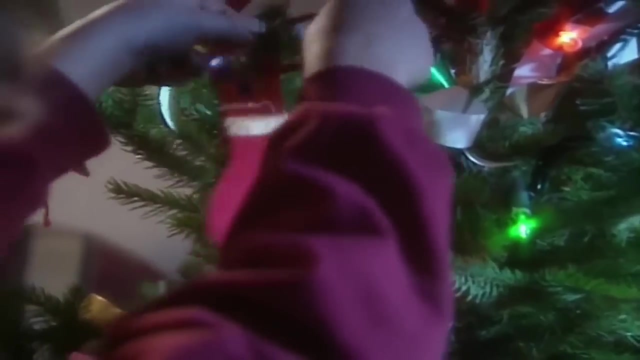 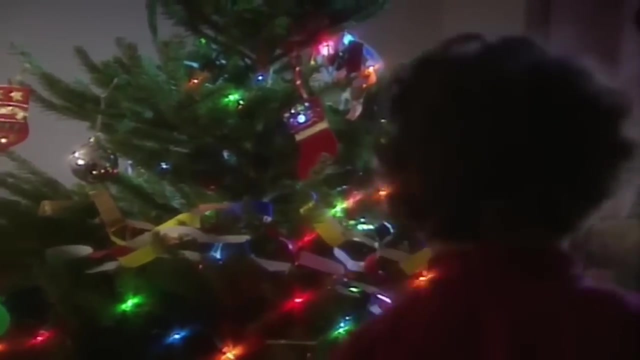 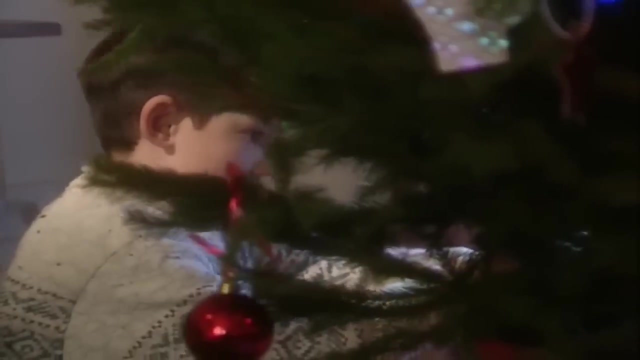 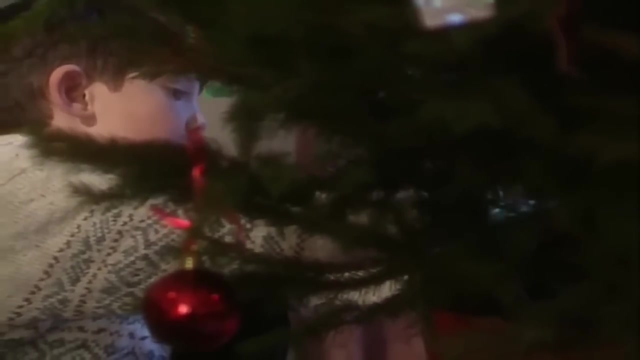 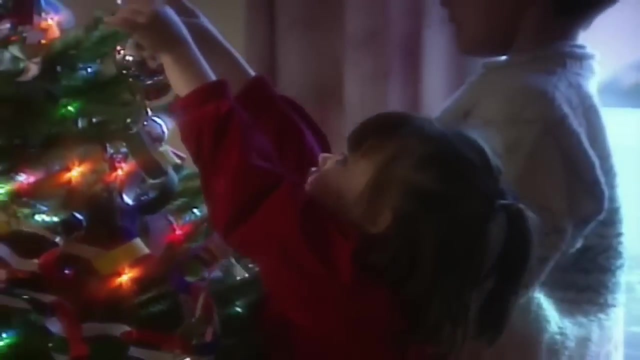 Come on. I like Christmas trees when they're decorated with sparkly lights. I love decorated Christmas trees. There's loads of them at the front. I'm putting some at the back now. I think I'll put that one back there. That's it. 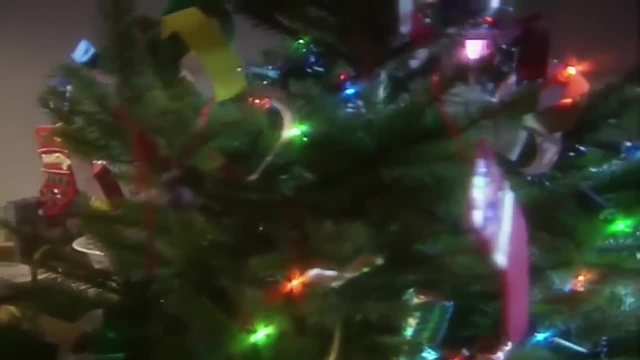 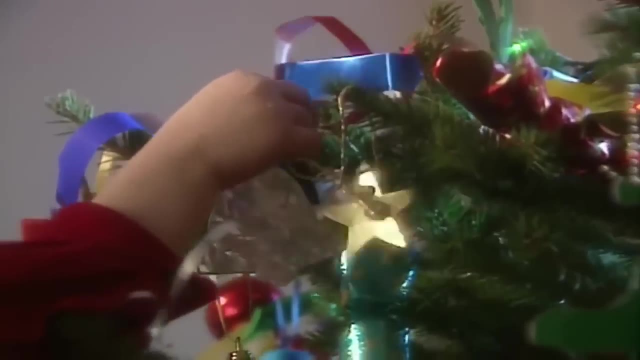 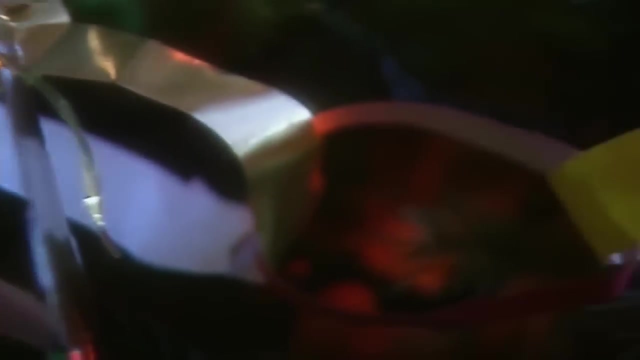 It's going to be the prettiest tree in the whole wide world. I like putting on the decorations I made. they look nice. I like these paper jets. what Lewis Jasper did, that I made. It took us a long time. Are you just making this log? 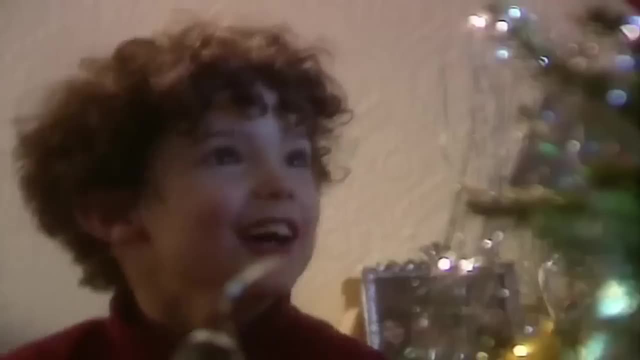 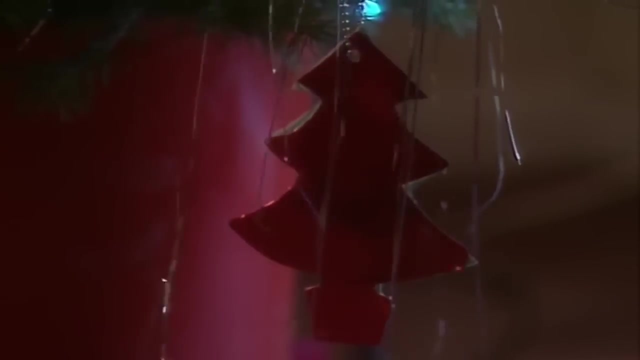 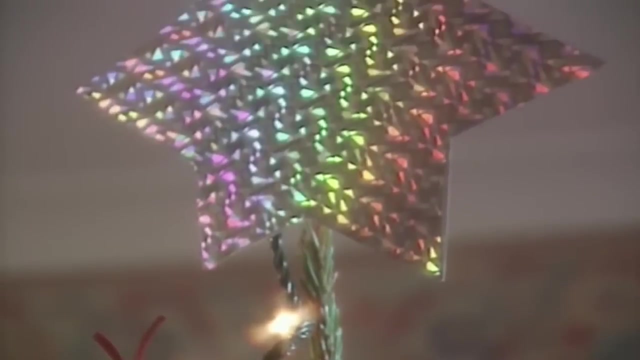 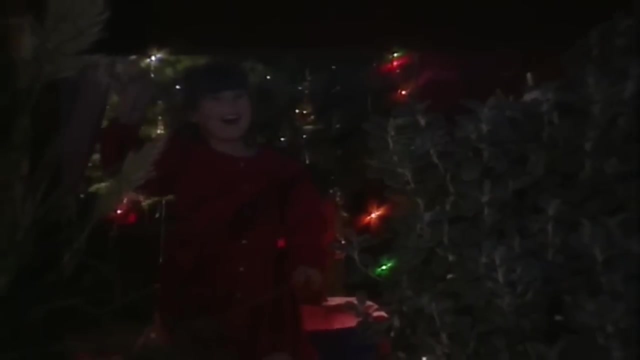 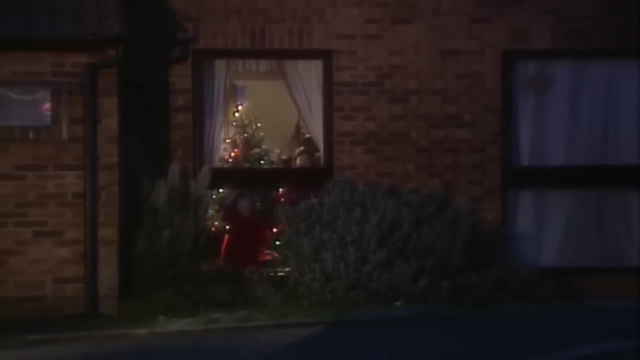 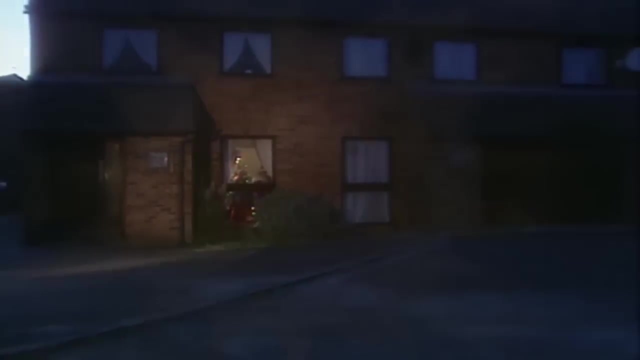 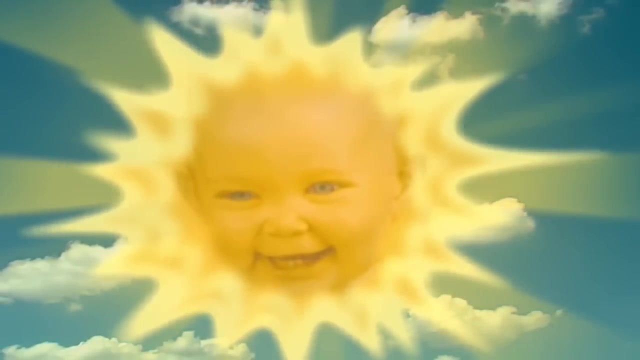 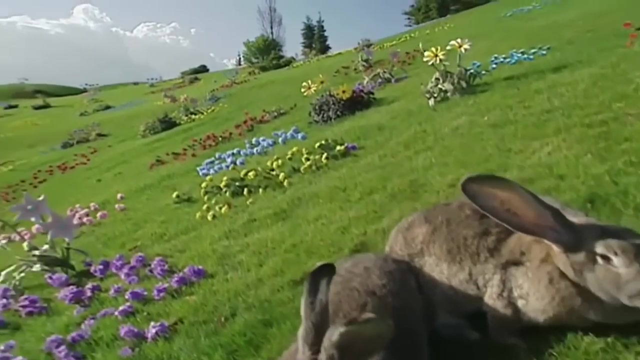 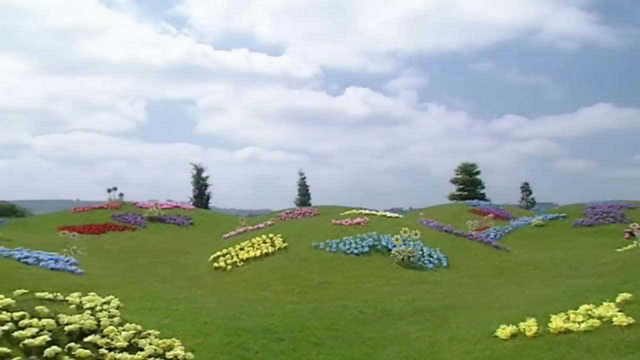 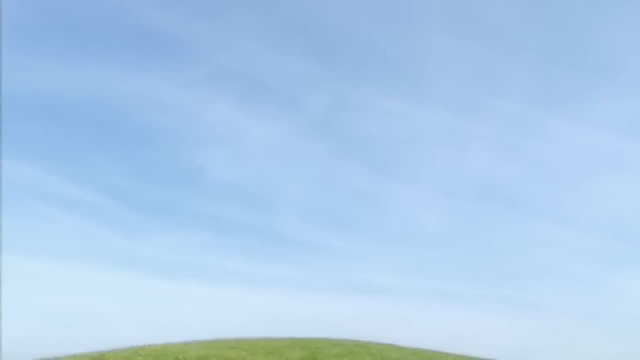 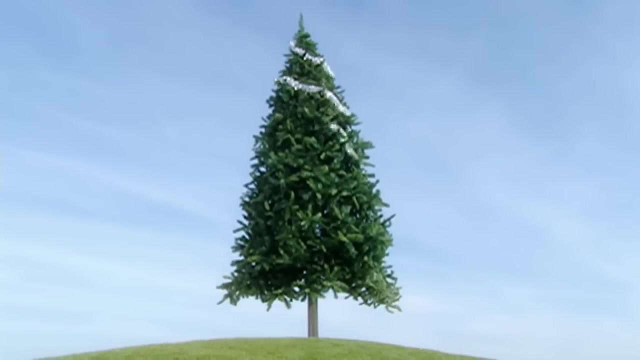 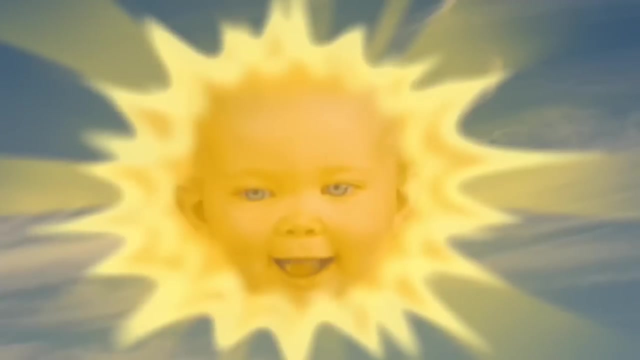 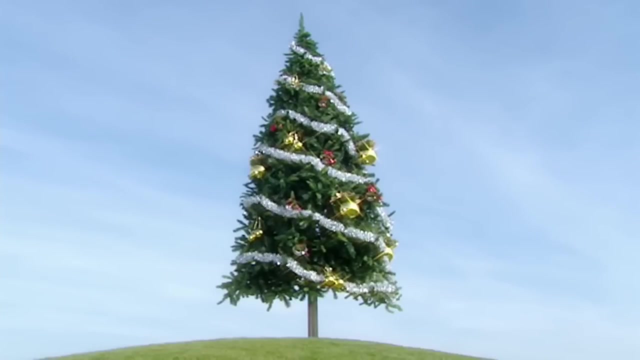 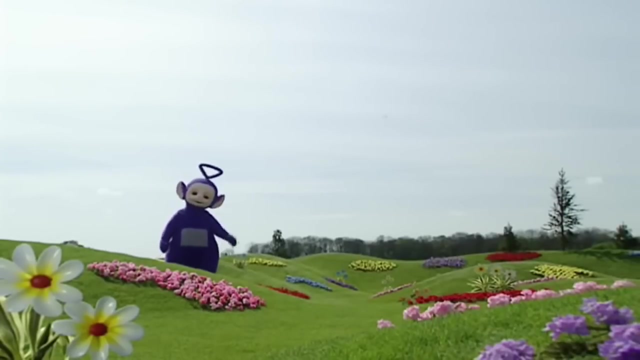 Bye, Bye, Bye. One day in Teletubbyland something appeared in the hills. I love you. Tinky. Winky thought he heard something: Oh, Must be a bird, Must be a bird. What's that? Dipsy heard it too. 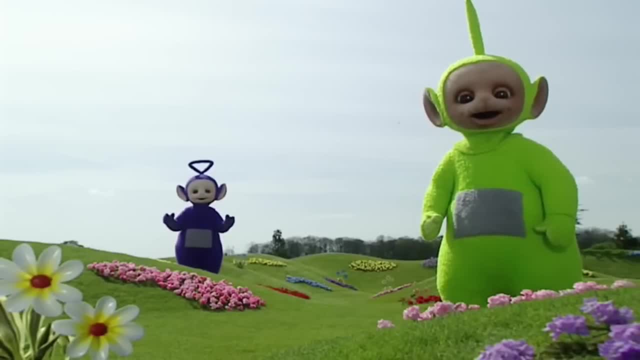 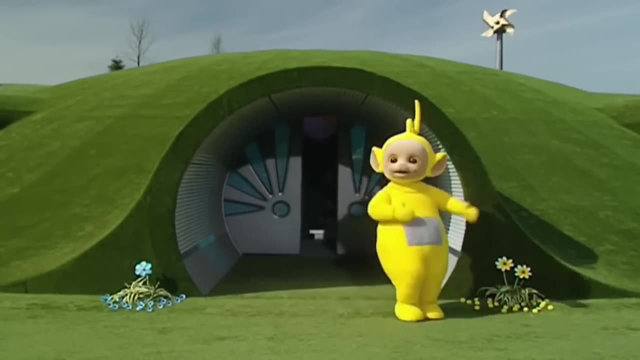 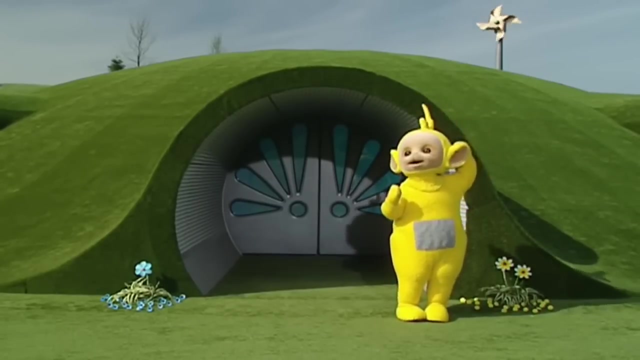 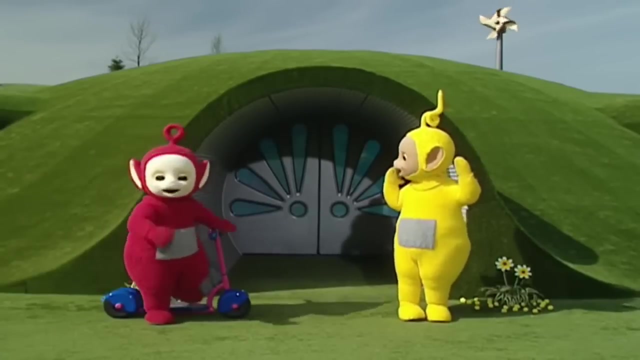 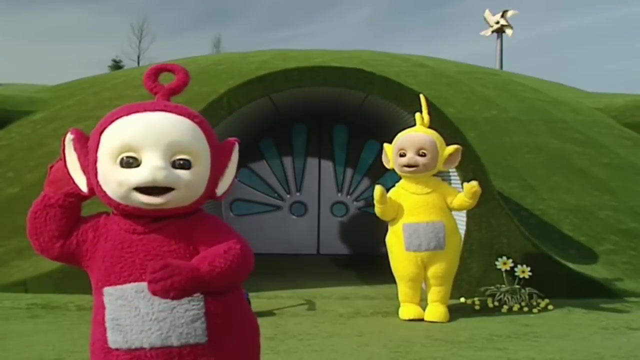 What's that? What's that? What's that? Lala heard it. What's that? What's that? Lala heard it too. What's that? What's that? Uh-oh, And Poe heard it. What's that? 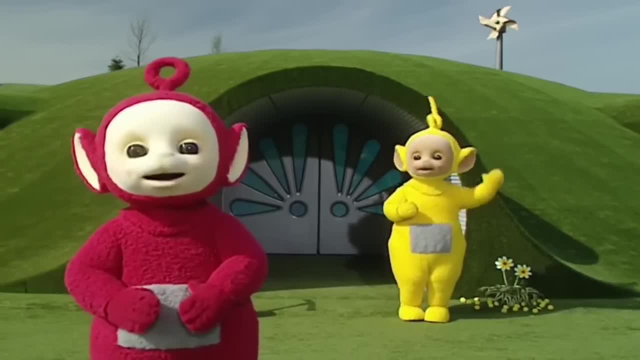 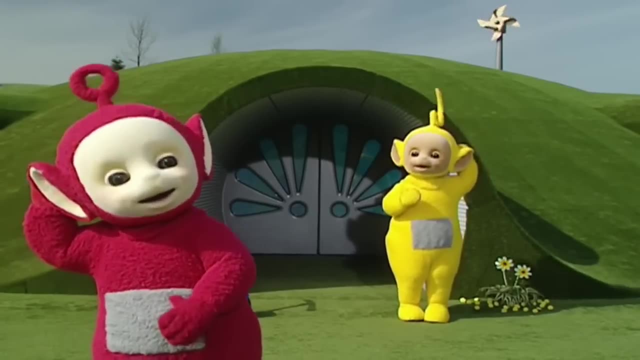 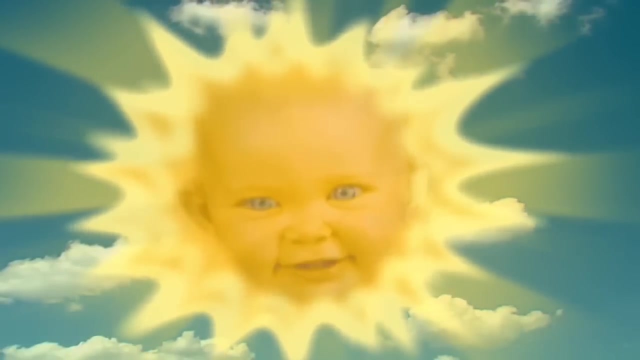 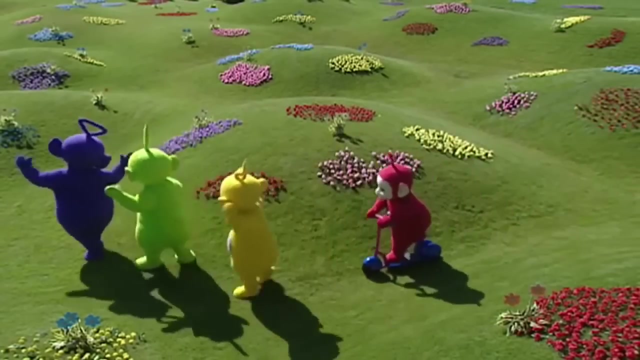 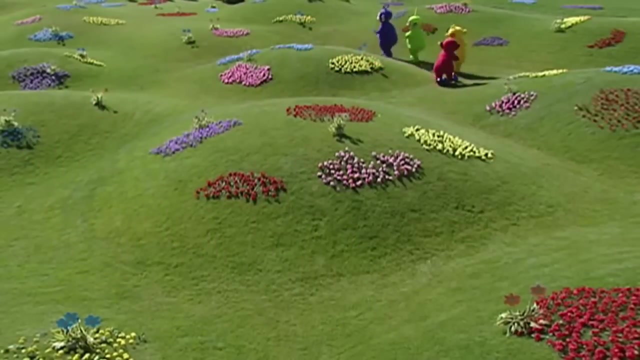 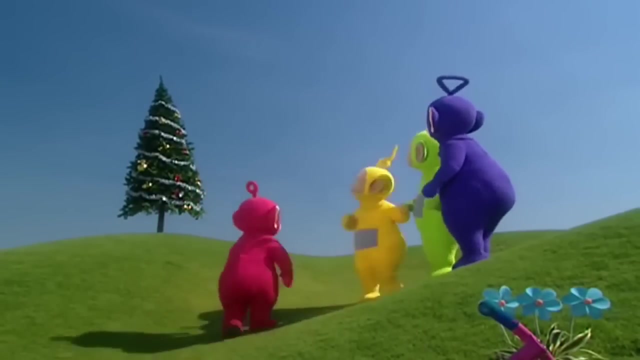 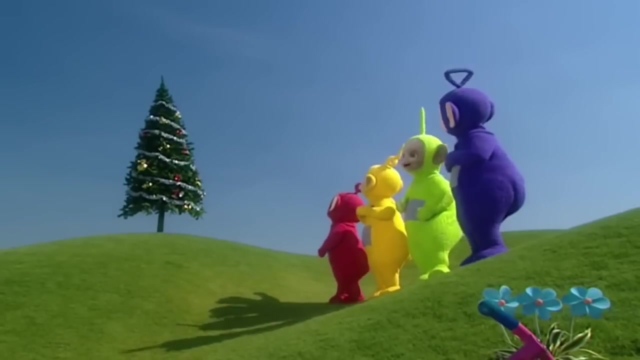 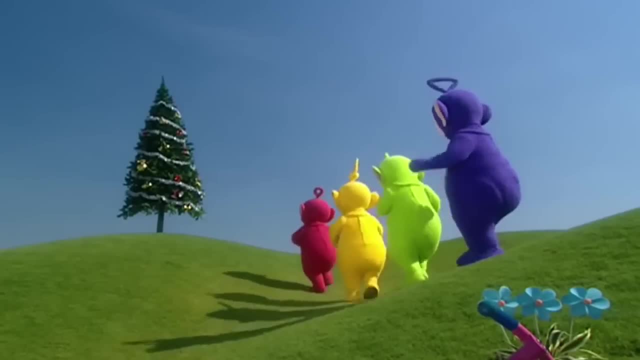 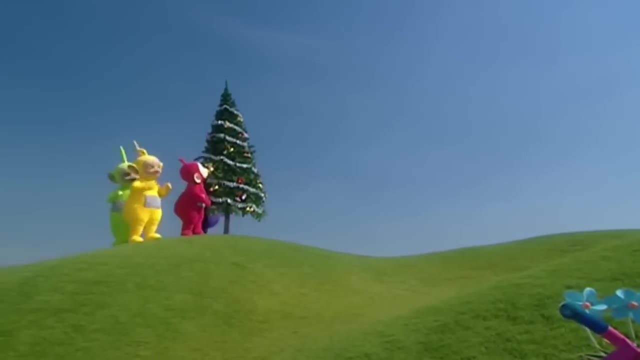 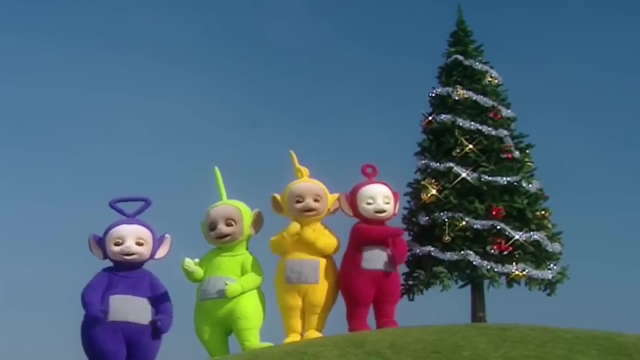 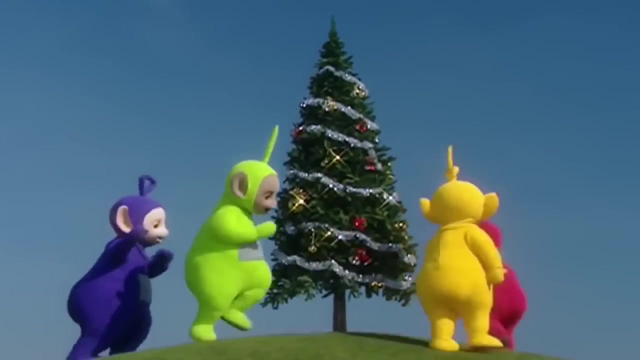 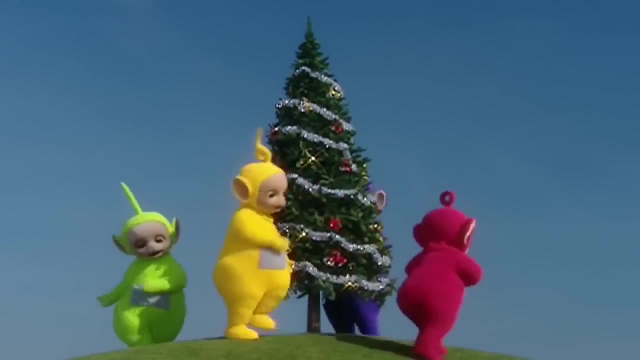 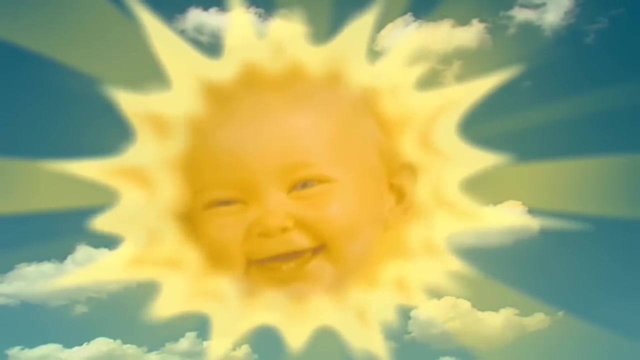 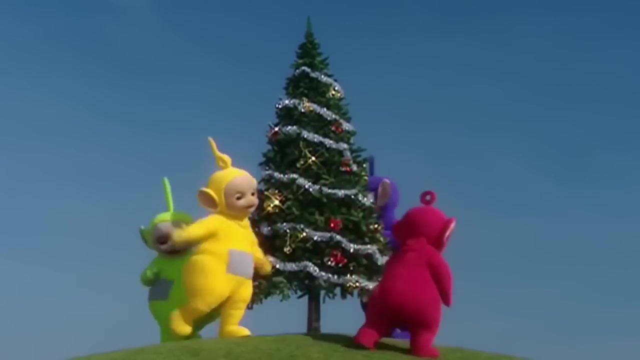 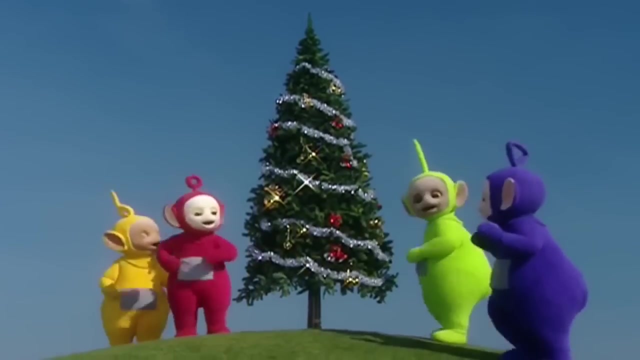 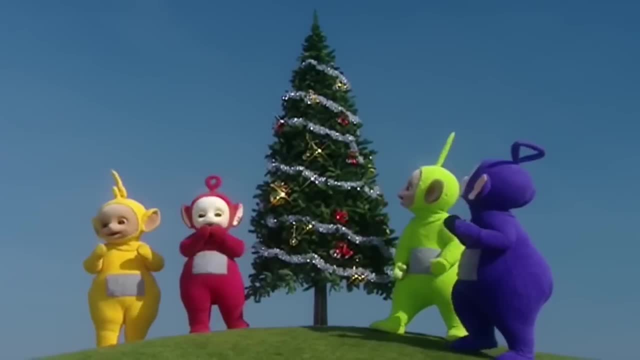 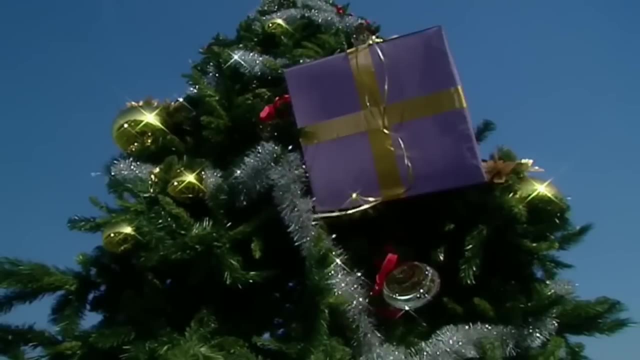 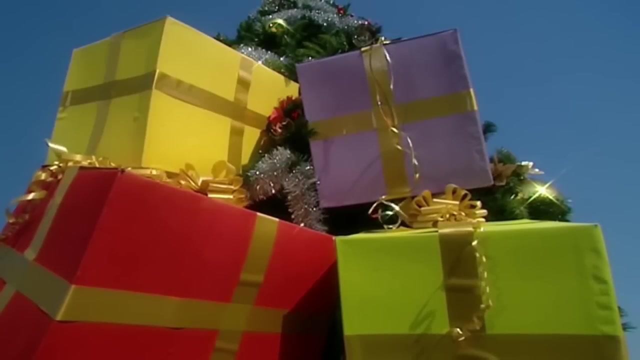 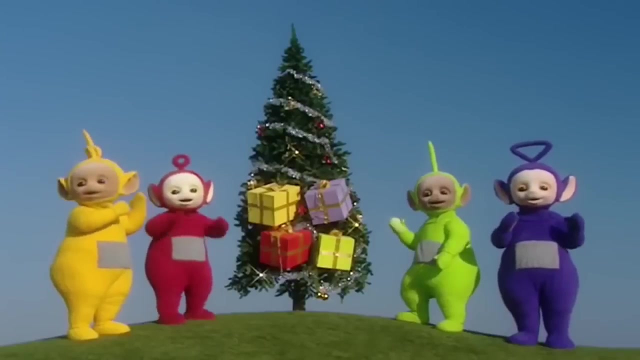 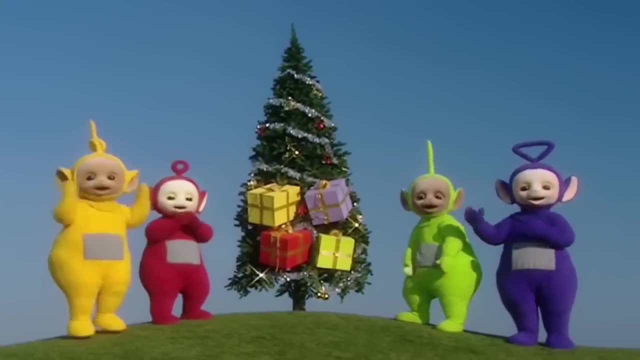 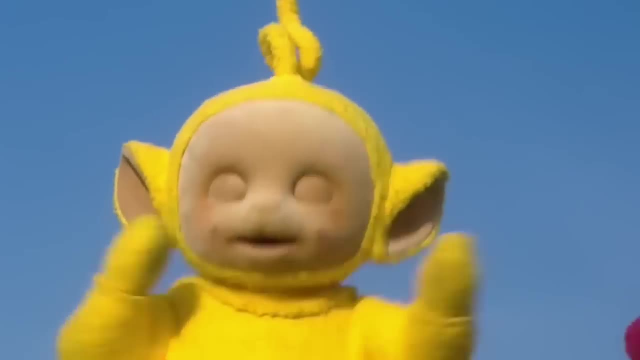 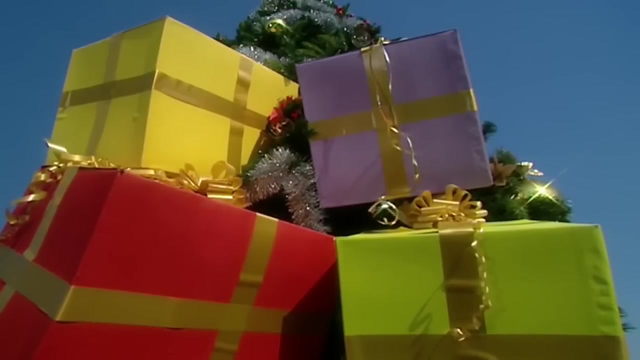 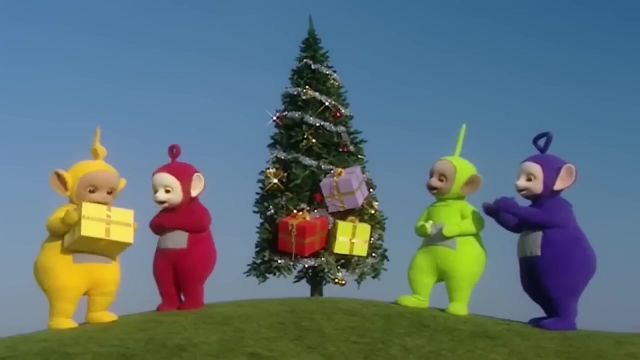 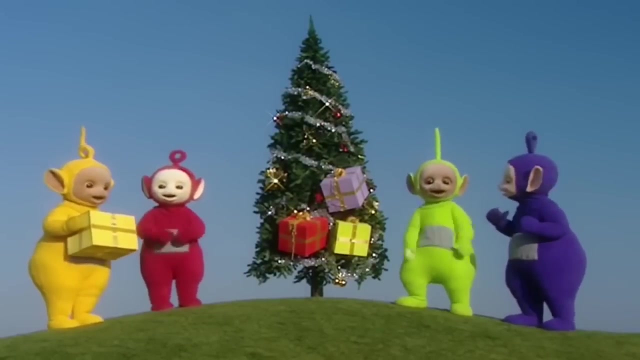 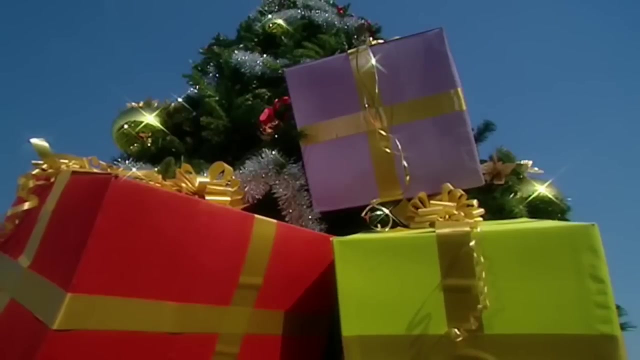 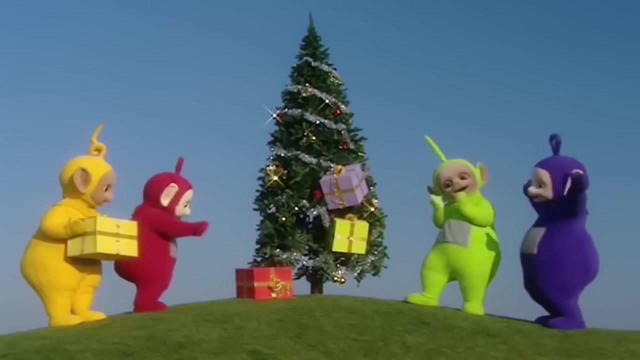 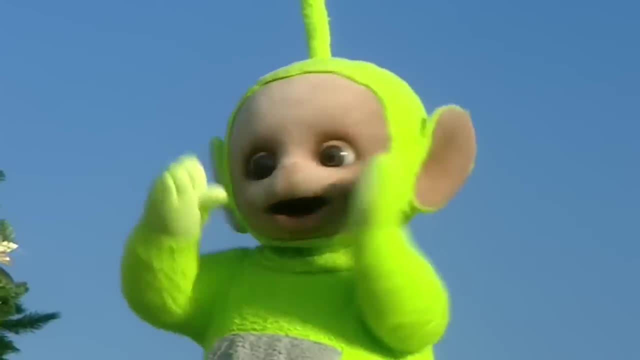 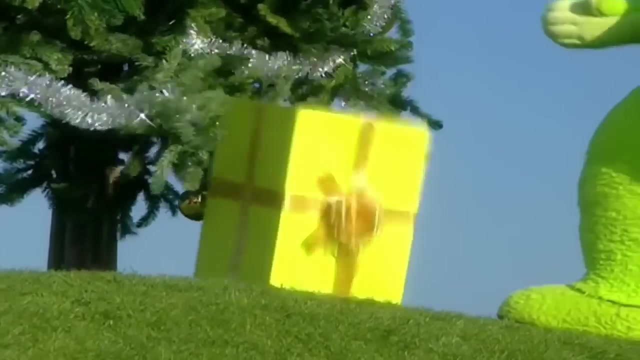 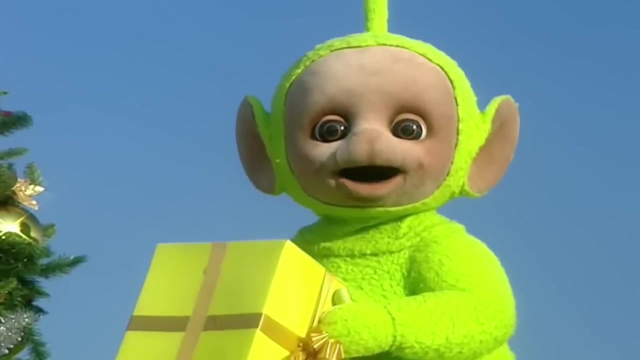 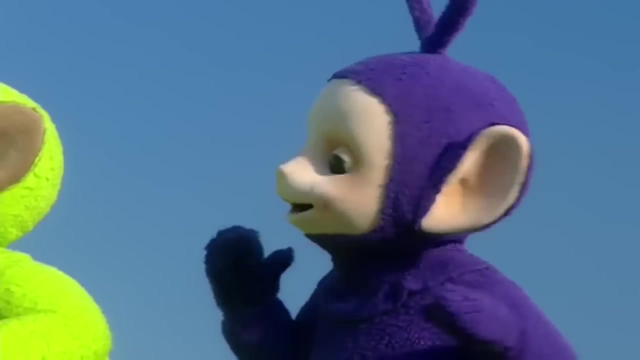 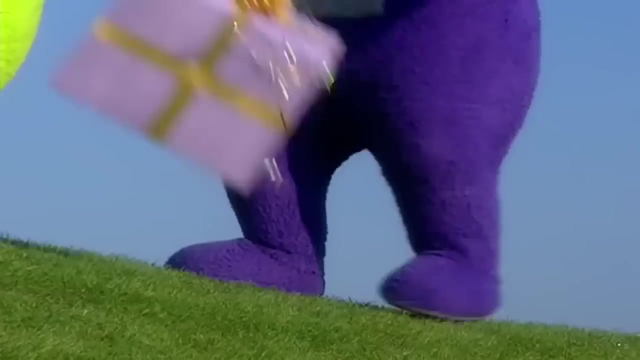 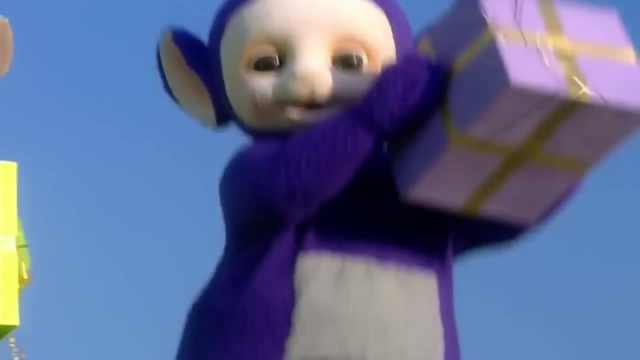 One present for Dipsy, Dipsy, One present for Dipsy And one present for Tinky Winky. Oh, Oh, present for Tinky Winky. The Teletubbies loved their presents very much. Present, Present, Present. 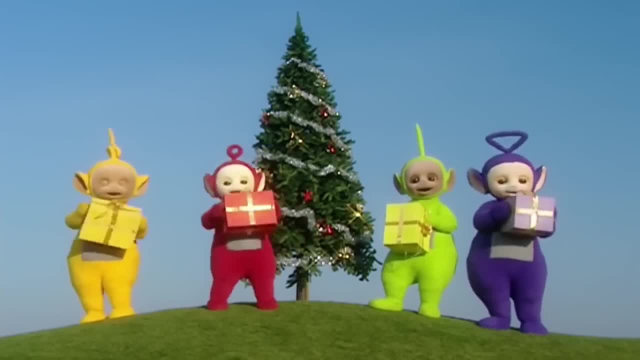 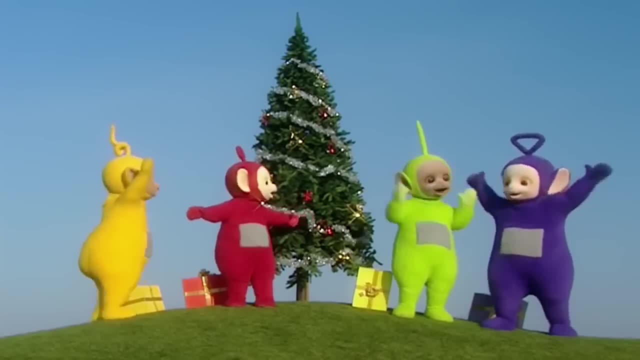 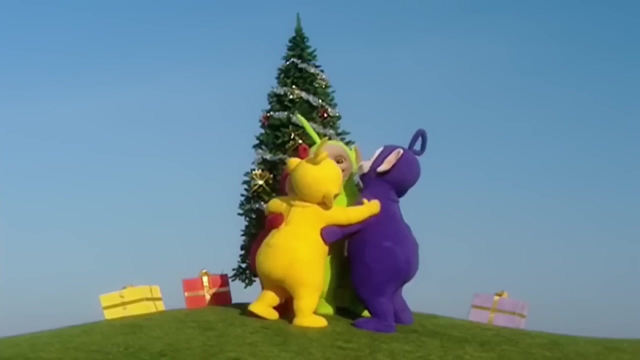 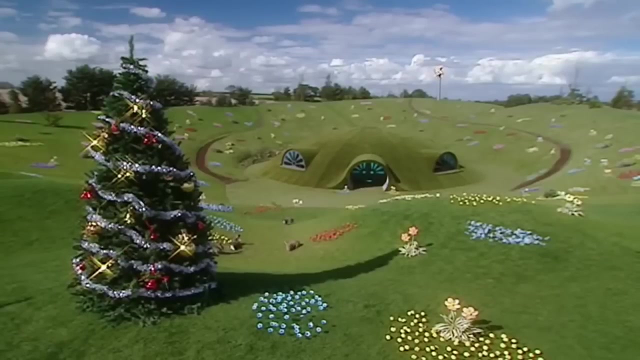 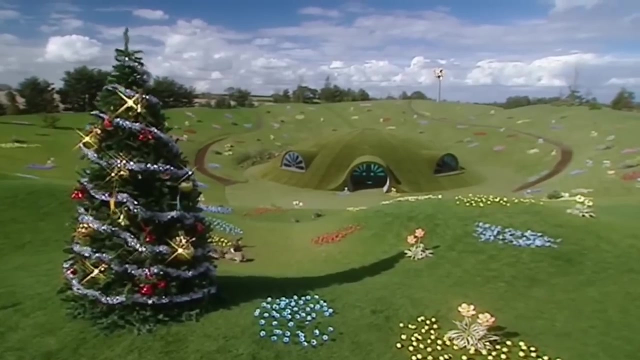 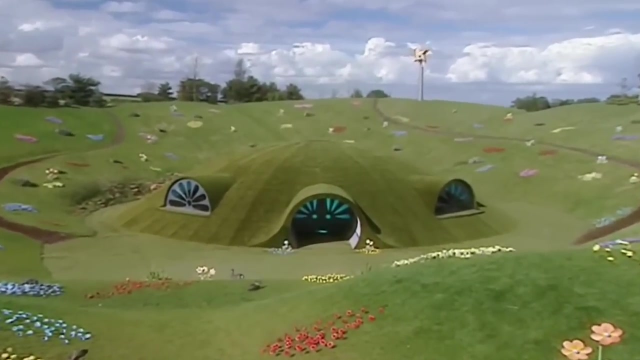 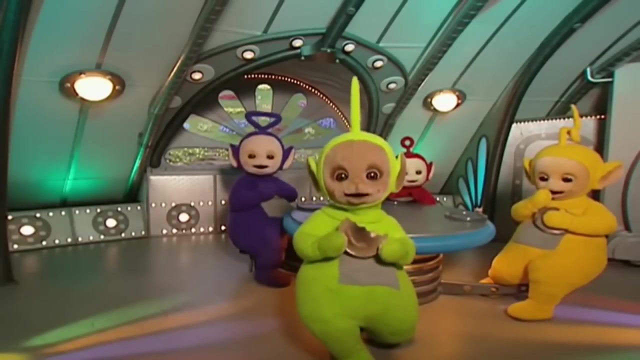 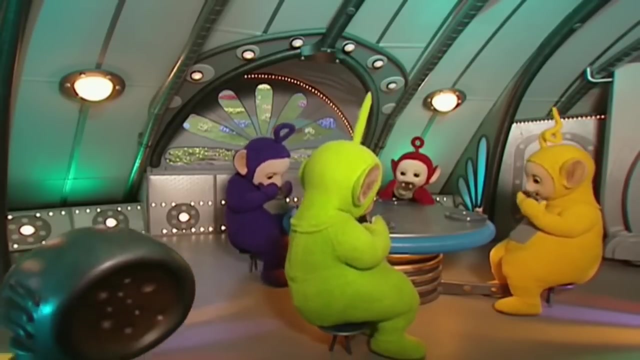 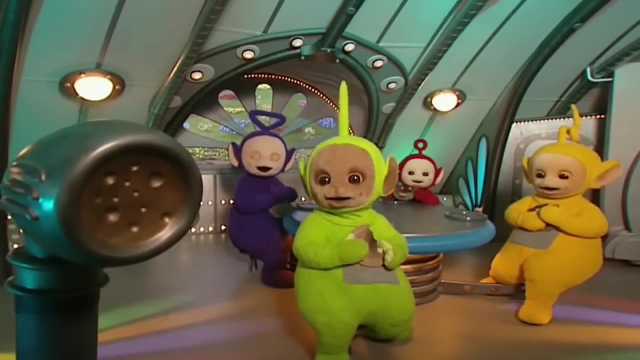 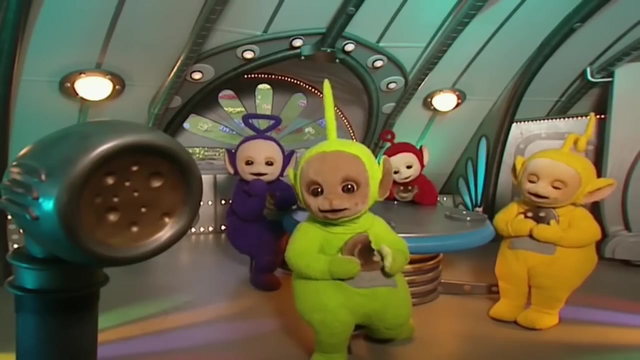 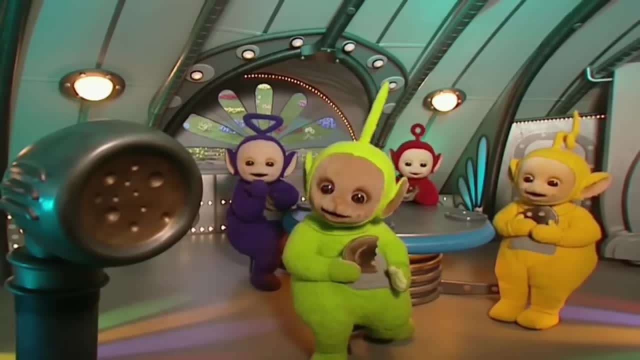 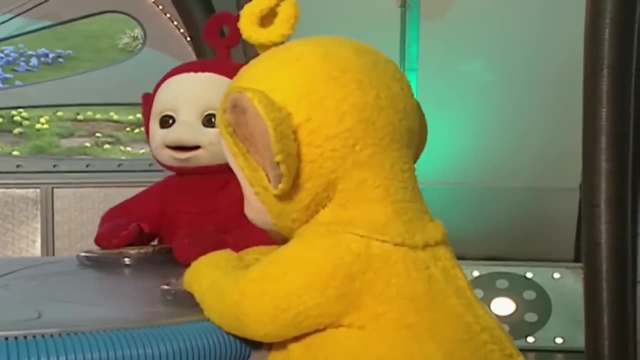 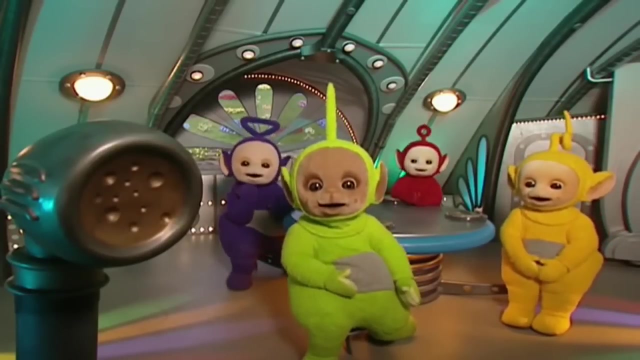 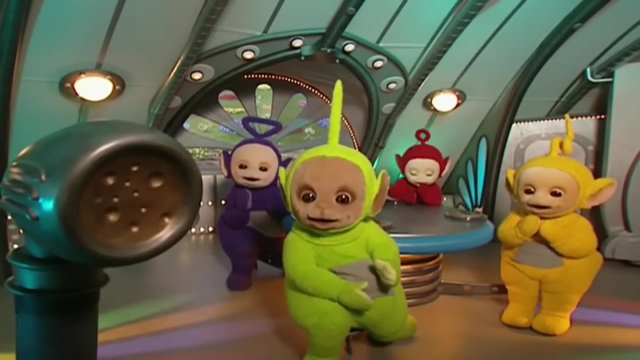 not a creature was stirring, not even a mouse. Ooh, Again, again, again, again, Shh. It was the night before Christmas and all through the house, not a creature was stirring, not even a mouse. Ooh. 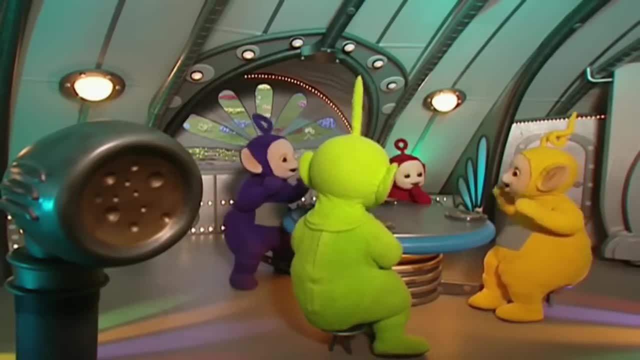 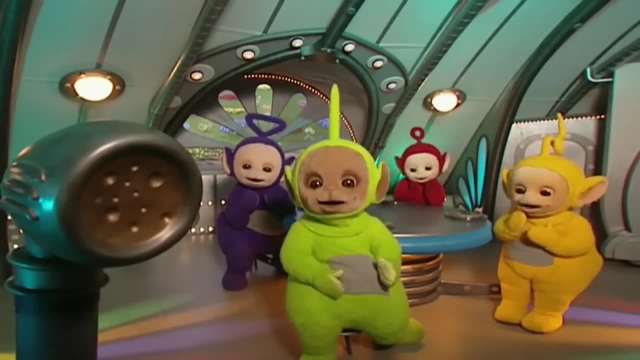 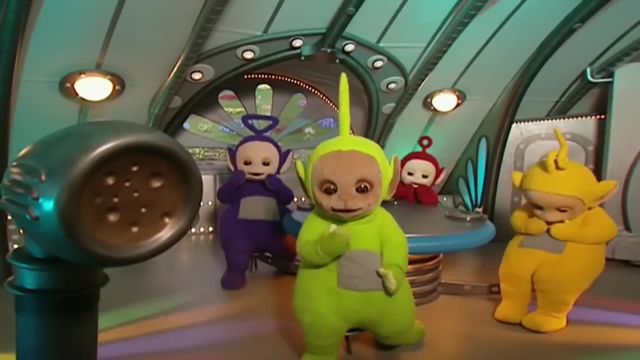 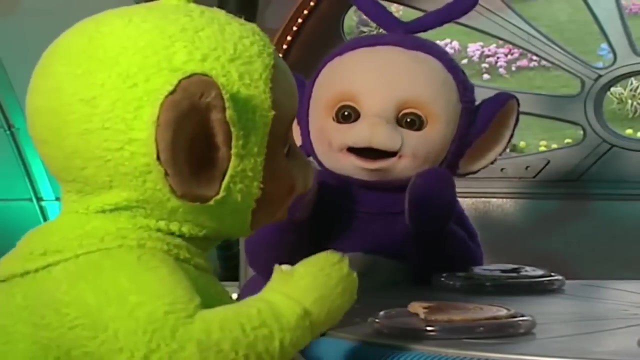 Shh, Again, again, again, again, Shh. It was the night before Christmas and all through the house, not a creature was stirring, not even a mouse. Shh, Shh, Shh, Not even a mouse. 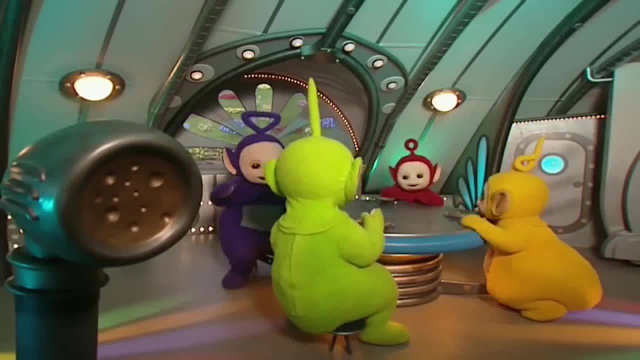 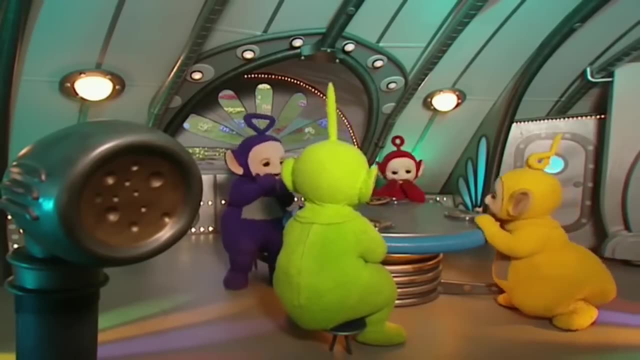 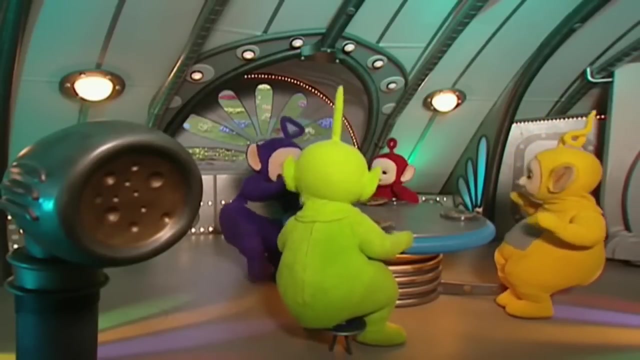 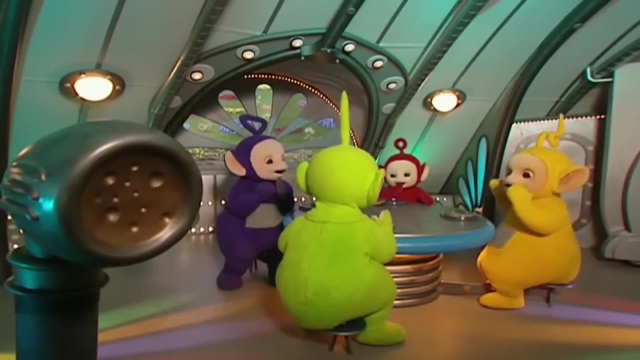 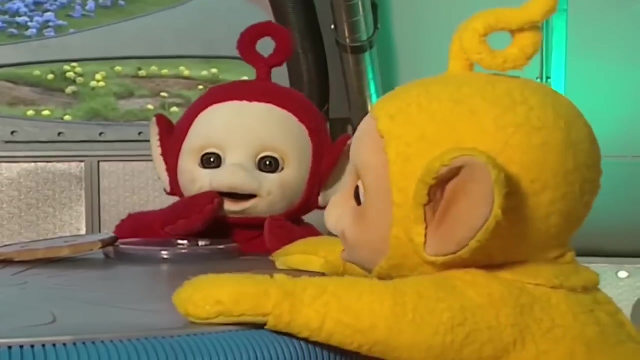 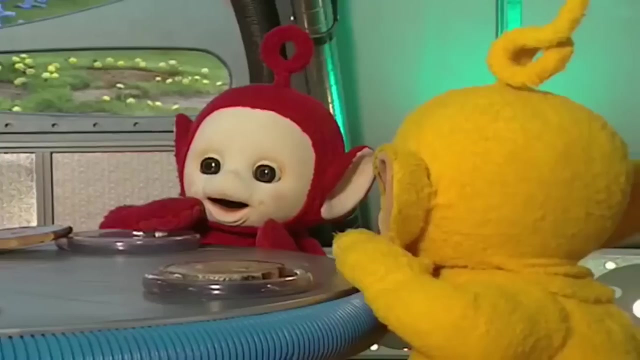 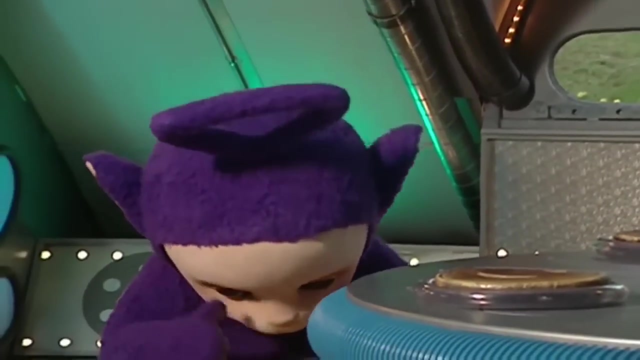 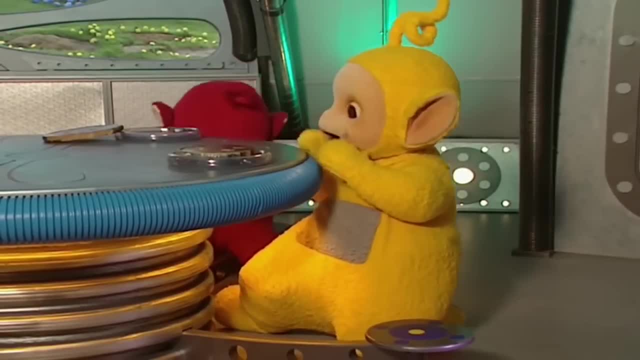 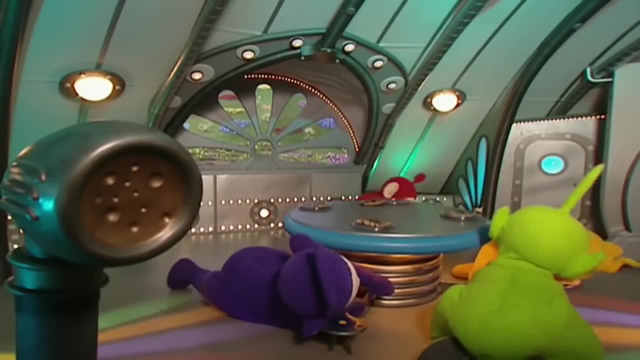 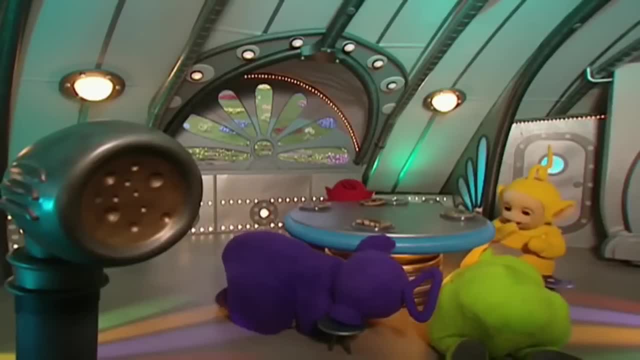 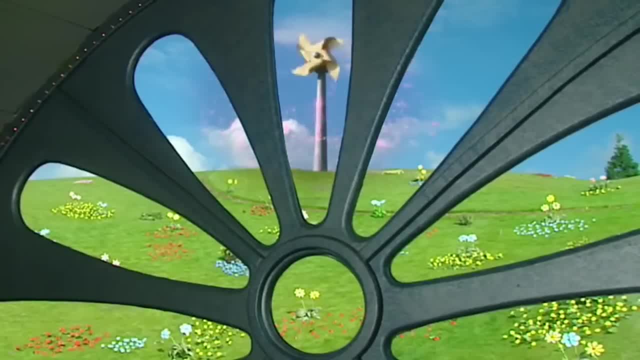 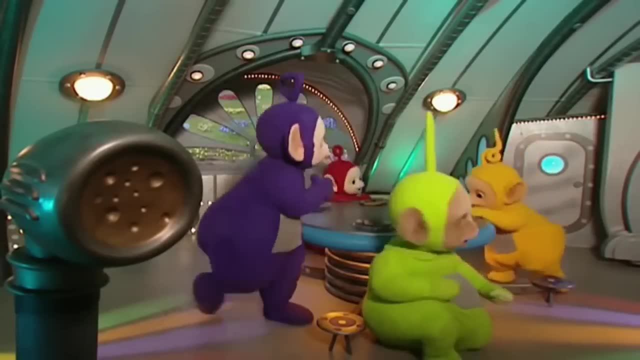 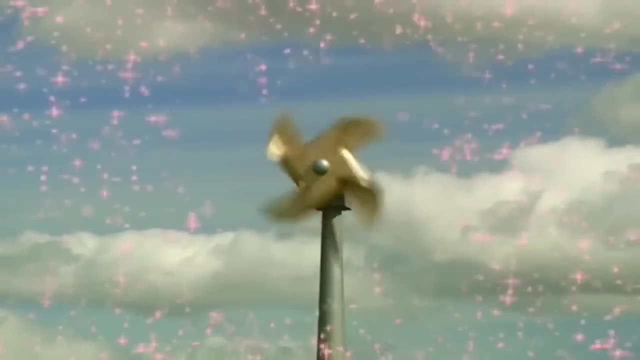 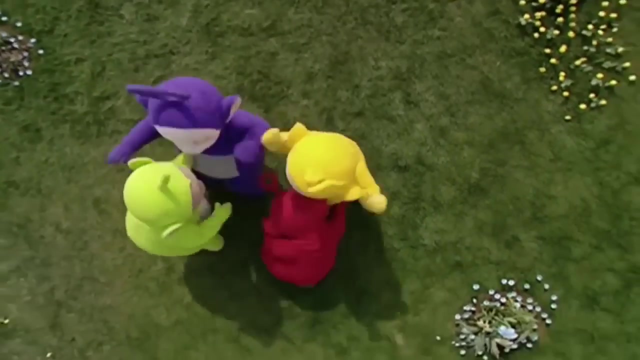 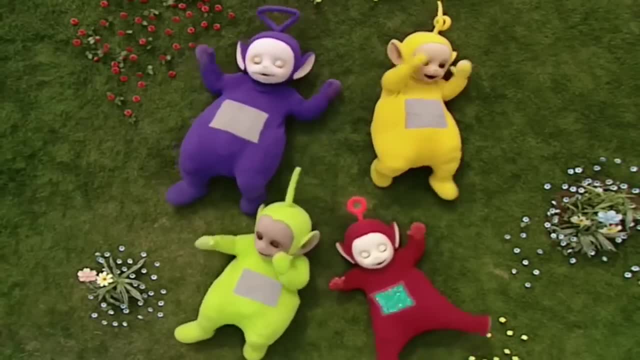 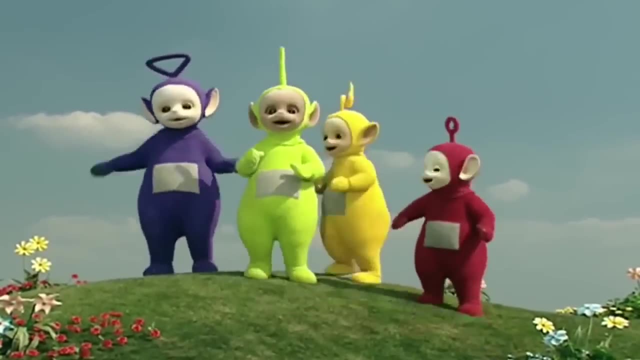 Shh Shh, Shh, Shh Shh. He did it. He naturalized to fifteen. You won three Bye. now Bye, Bye. That's great Good job. I appreciate it. See you guys. 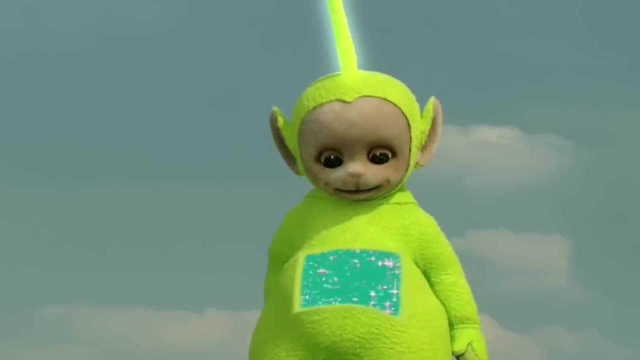 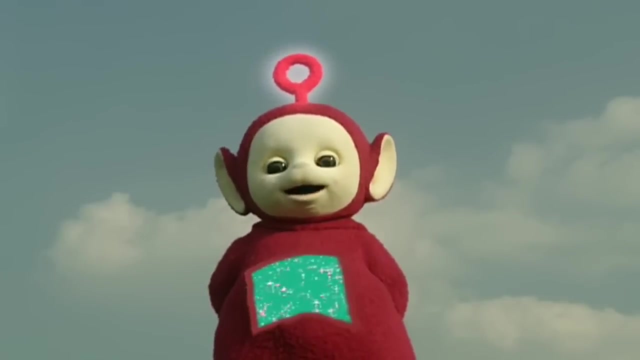 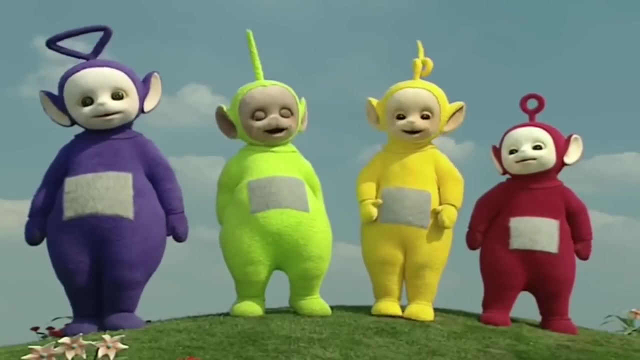 Have a wonderful day. Bye-bye, Bye-bye, Bye-bye. Singer's shh tool. I, going under the soarying, should return to the portrait as the current Tiki-wiki. Tipsy Lala Oh. 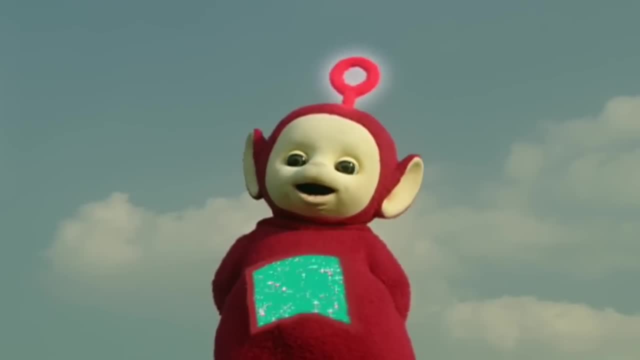 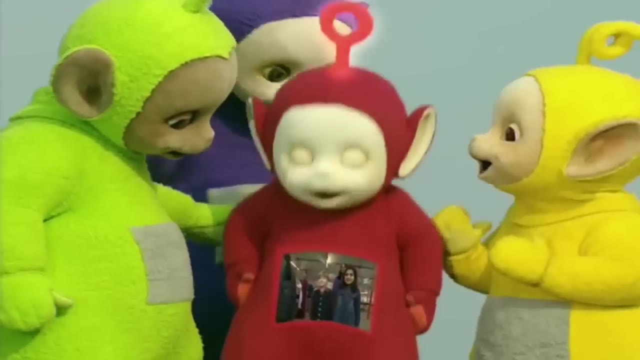 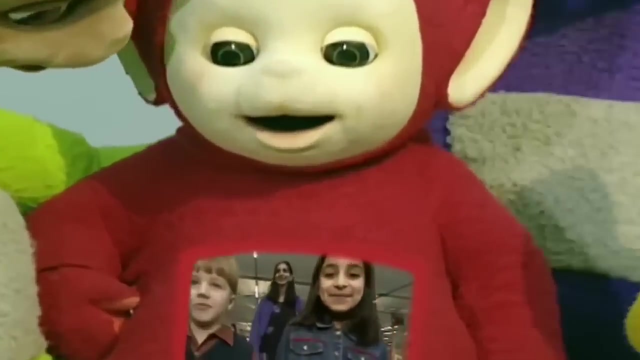 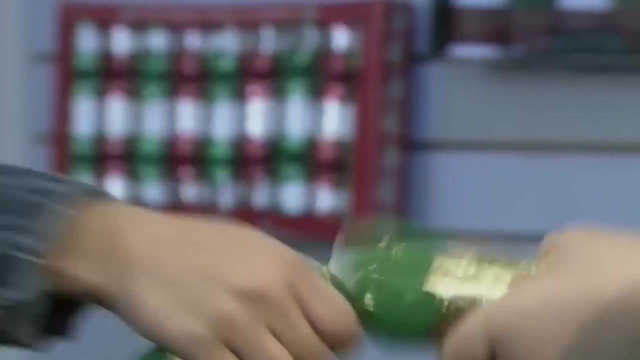 Oh Hook, Oh Hook, Oh, Hook, Hook, Oh Hook, Oh, Oh, Oh, Oh. Hello, Oh, Oh, Oh. Hello. my name is Sam. Hello. my name is Maddie Crackers. 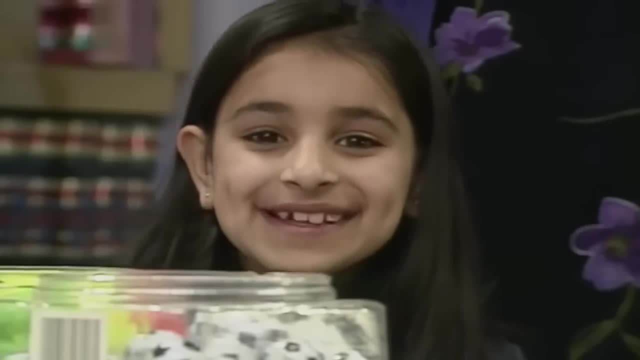 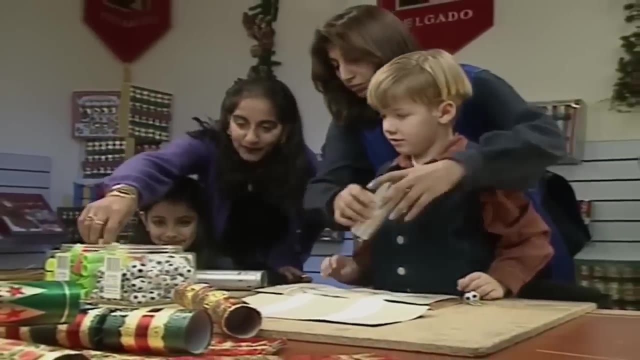 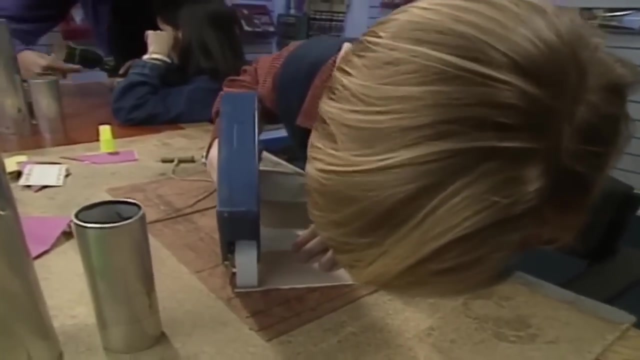 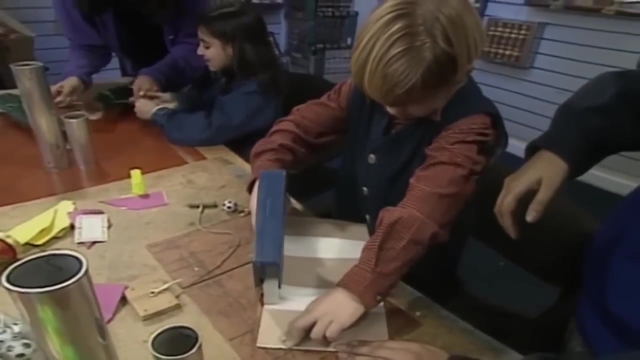 I know how to make crackers. My auntie makes crackers. Here she is, Hi, Am I helping? Yeah, I'm gluing this, I'm gluing it. I'm making the cracker for Nadia. Put the sticky bit on. 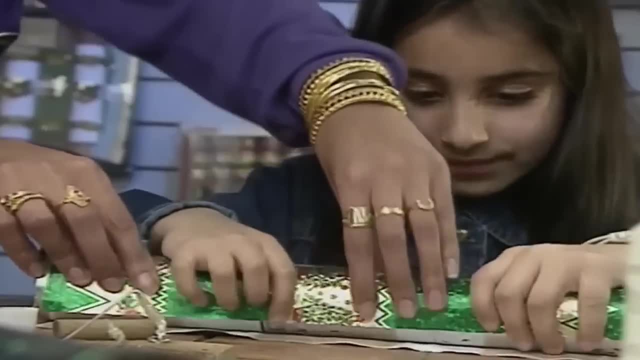 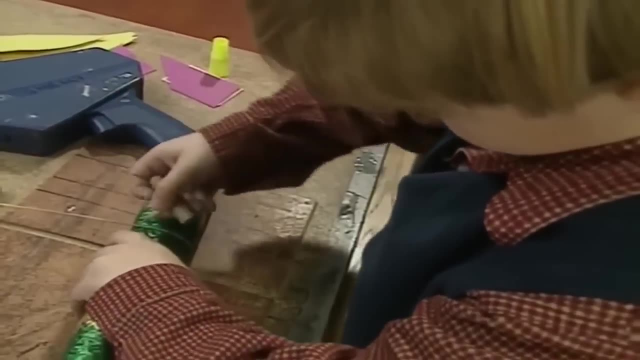 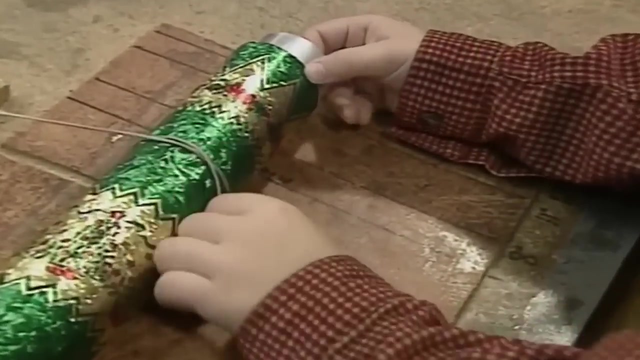 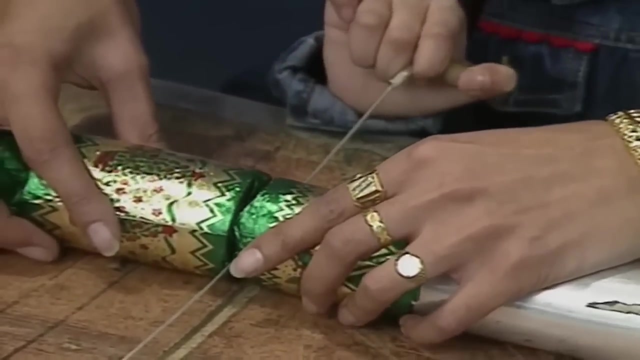 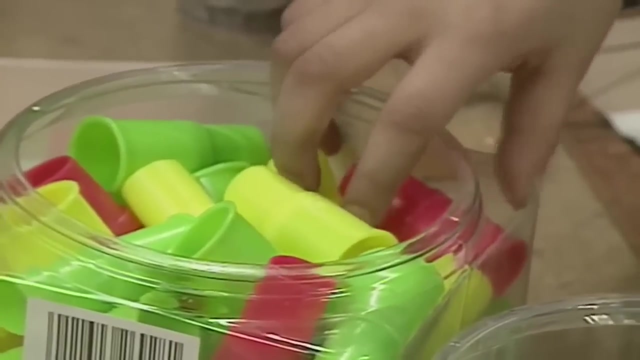 Hi, I'm going to roll the cracker. So it's tarred. Make sure it's tarred, Tarred. Put it in the string round. Go on, Crimp it a bit tighter. I've got a hat. Here is the blower. 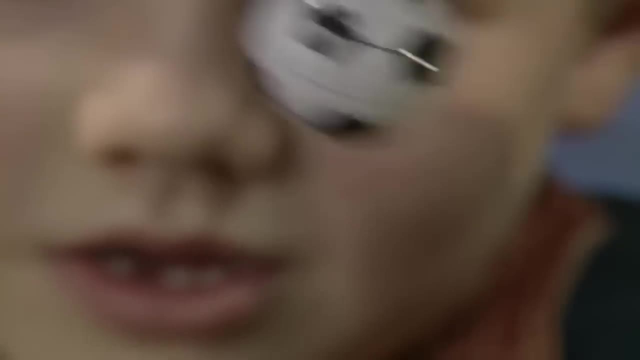 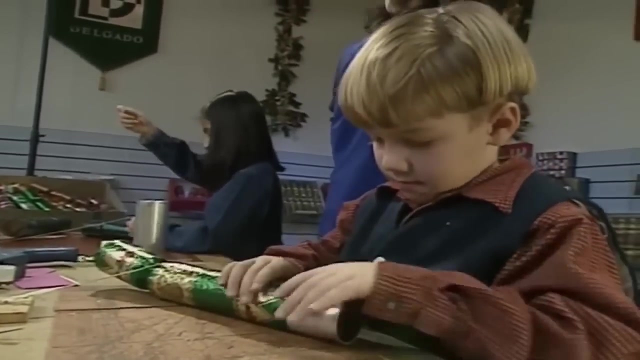 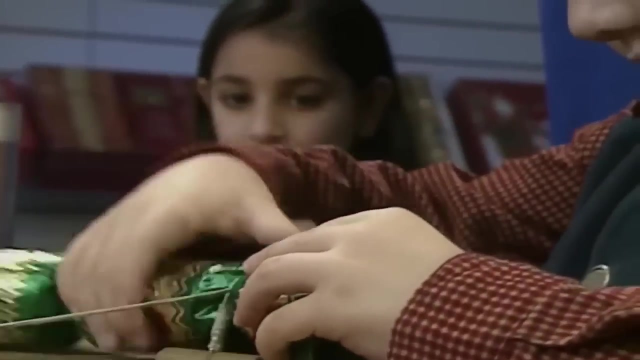 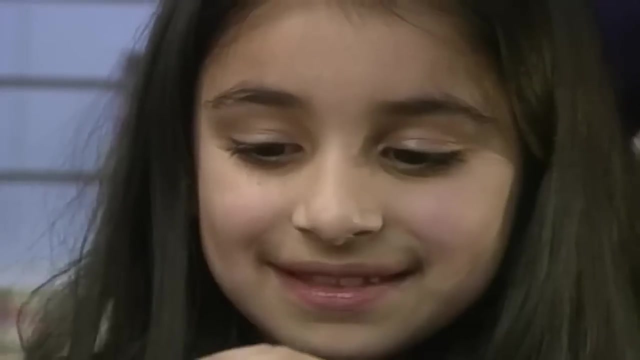 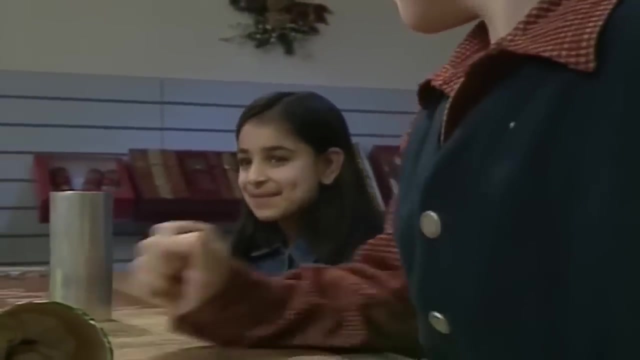 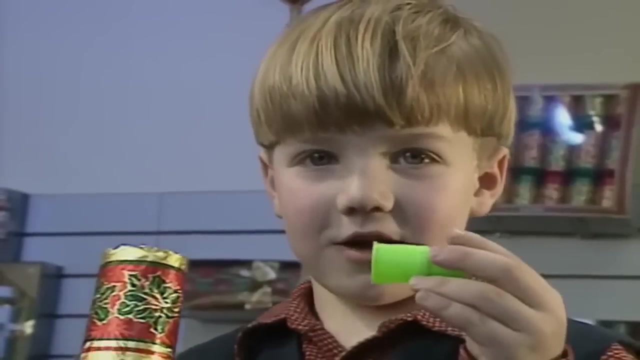 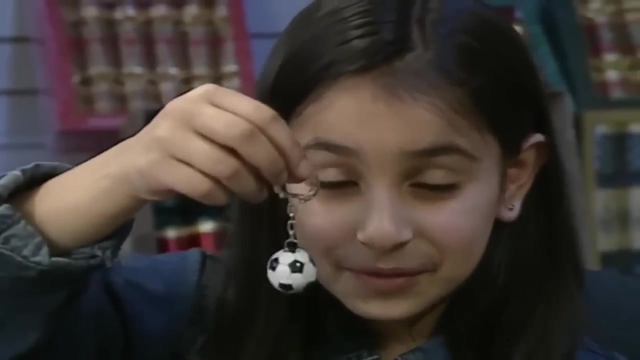 I'm putting a football in the cracker. It's a surprise. It is finished. There's my cracker for Nadia. Here's Sam's cracker. Look what I've got. There's my football. I've got a hat. 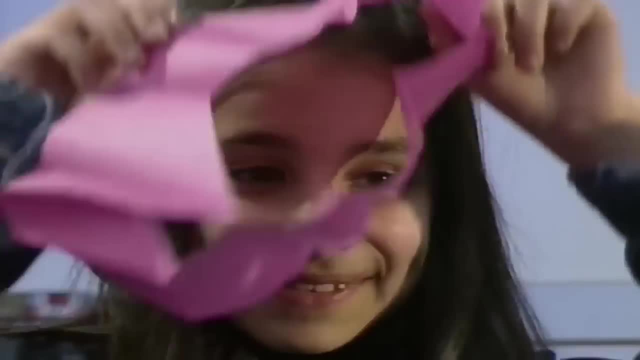 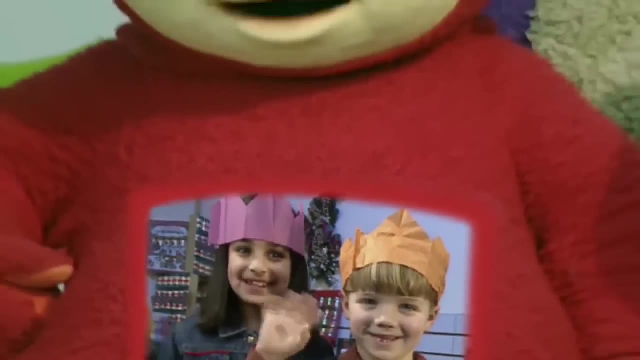 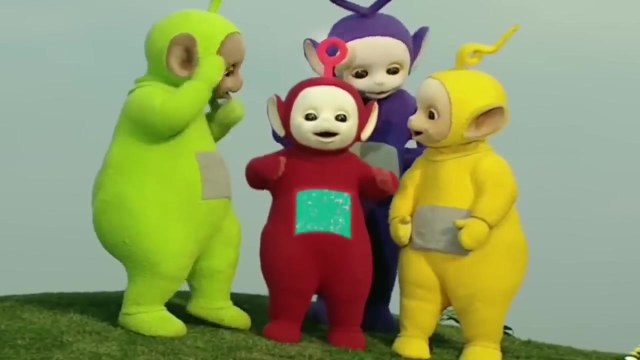 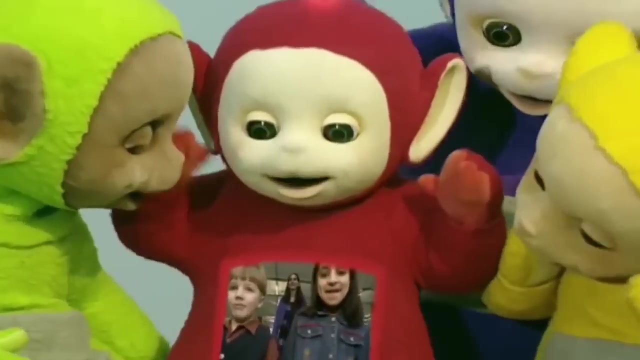 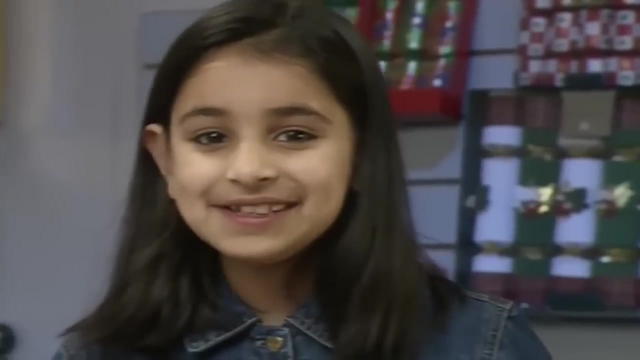 I've got one too. Okay, Congrats, Nadia Man. my arms Congratulations. I'mution. Goodbye, Goodbye, Goodbye, Goodbye. I know how to make crackers. My auntie makes crackers. here she is. 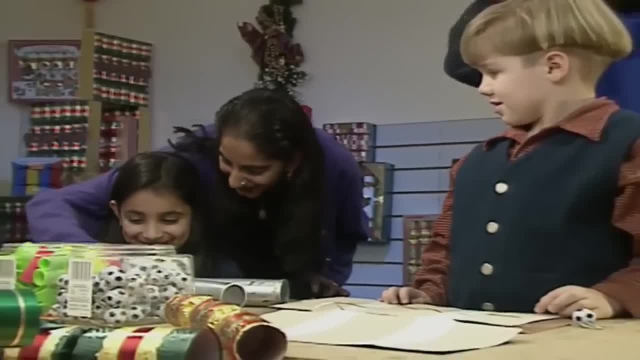 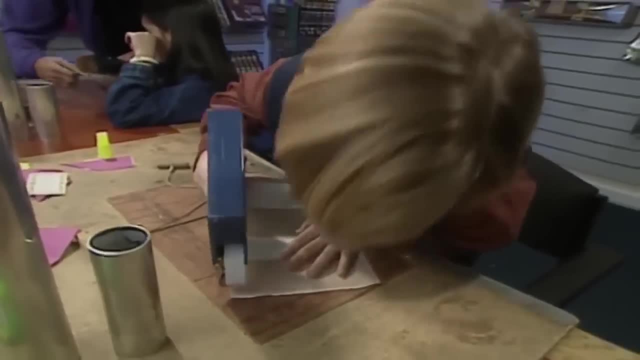 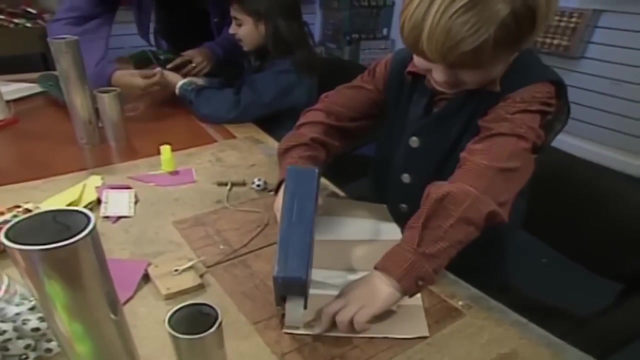 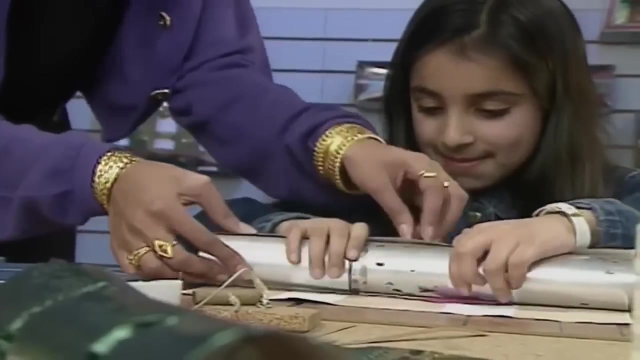 Hi, Am I helping? Yeah, I'm gluing this. I'm making the cracker for Nadia. Put the sticky bit on. Hi, I'm going to roll the cracker So it's tarred. Make sure it's tarred. 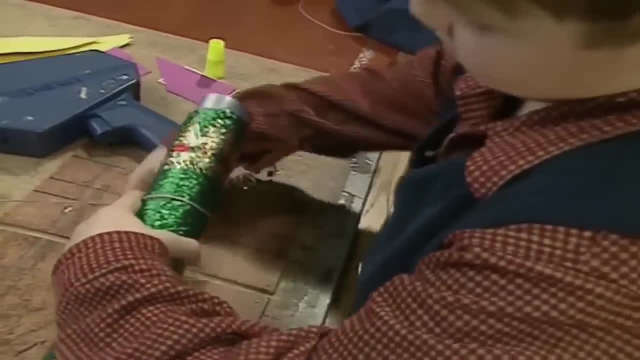 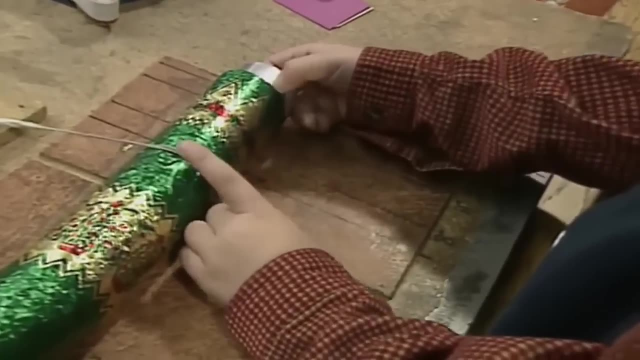 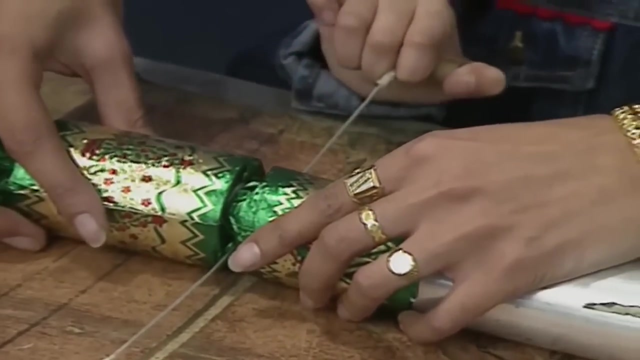 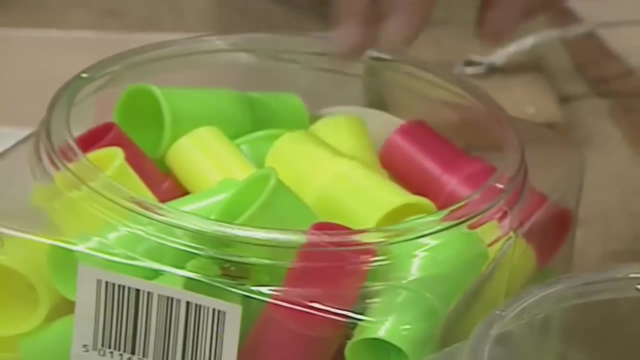 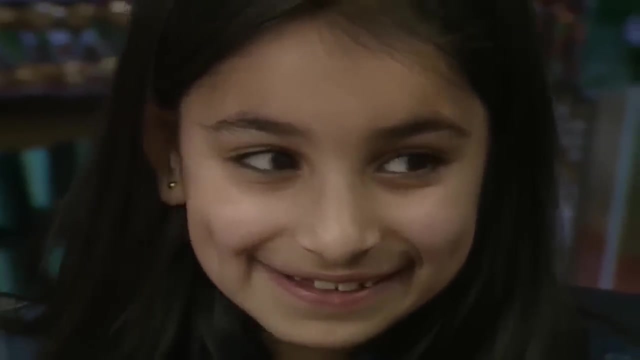 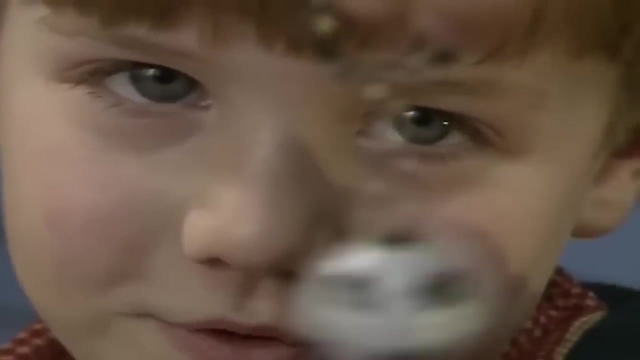 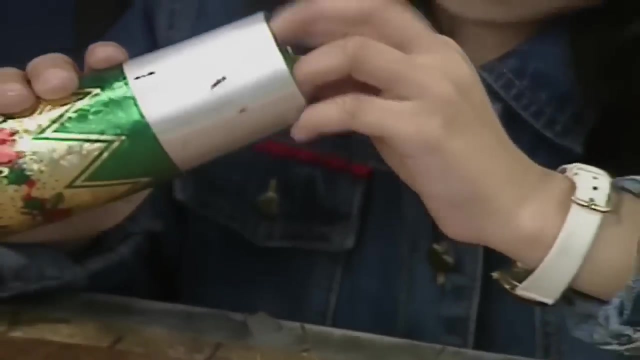 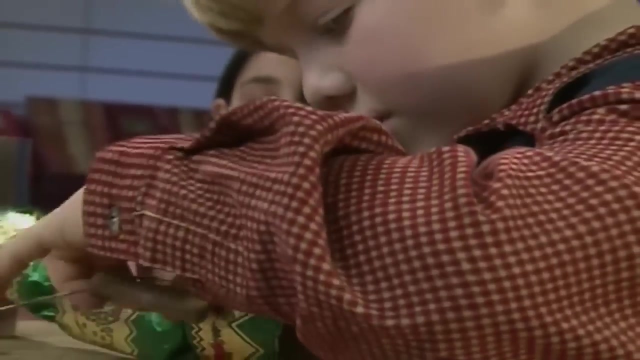 Tarred Pushing the string round. Go on, Crimp it a bit harder. Have a cracker. It's a hat. Here is the blower. I'm putting a football in the cracker. It's a surprise, Eek. 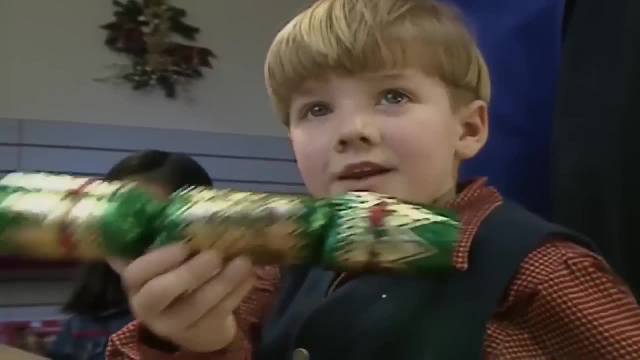 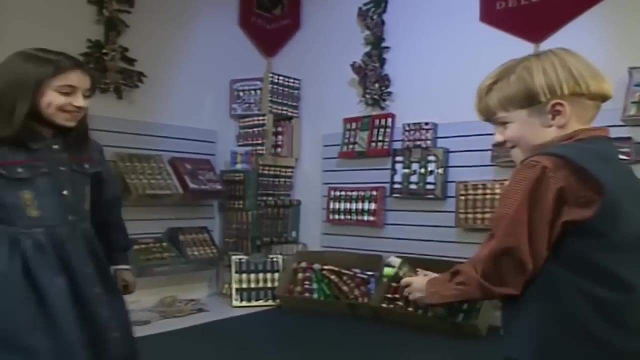 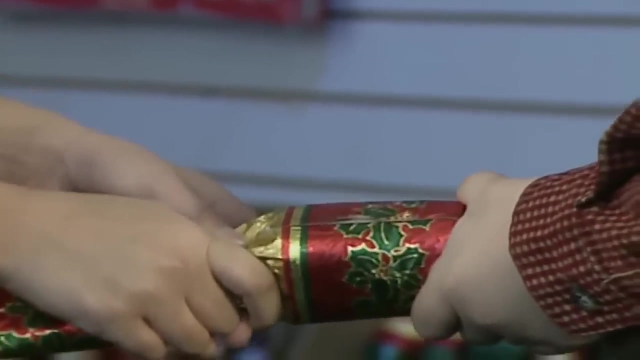 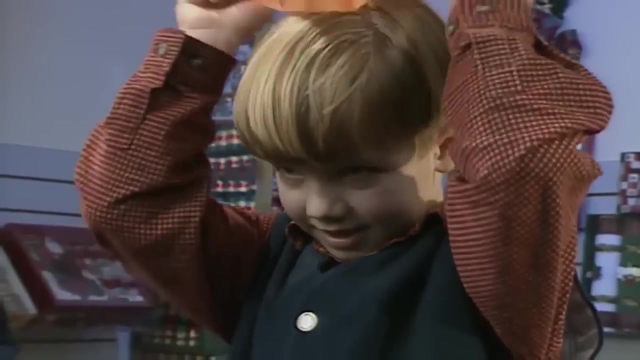 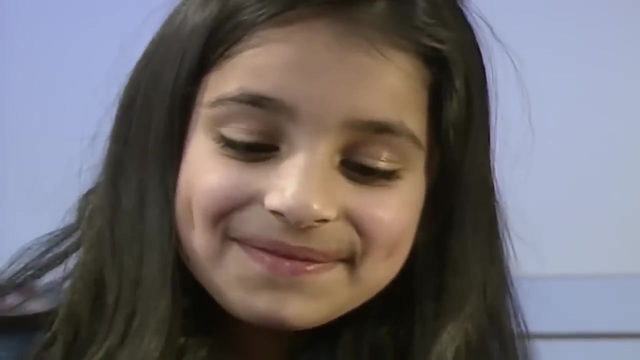 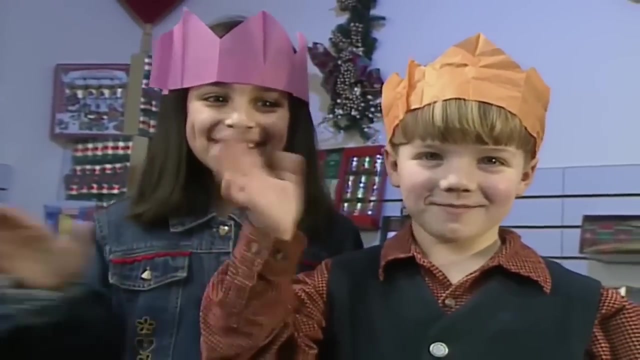 It's finished. There's my cracker for Nadia, Here's Sam's cracker. Look what I got. There's my football. I've got a hat. I've got one too. Goodbye, Goodbye, Goodbye. 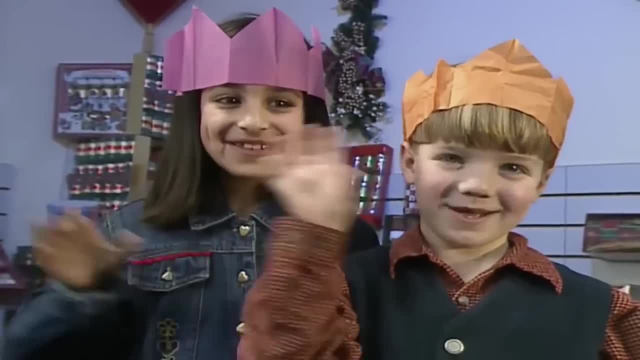 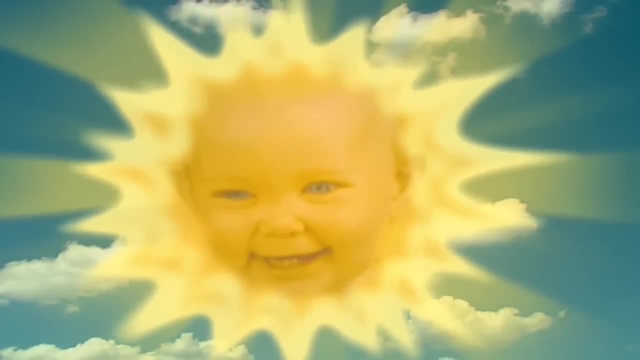 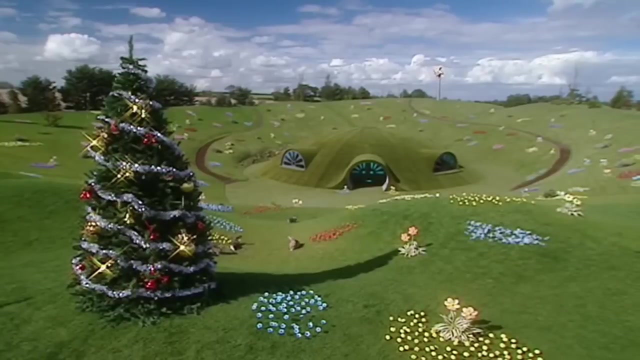 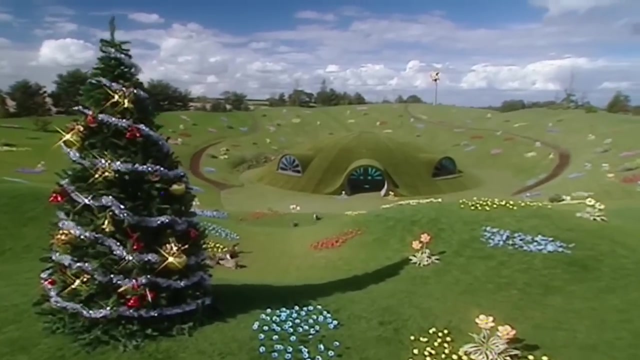 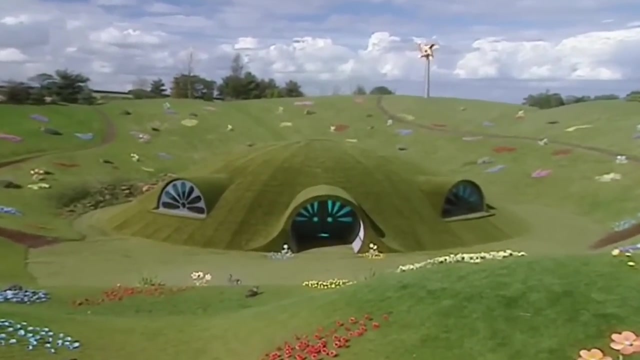 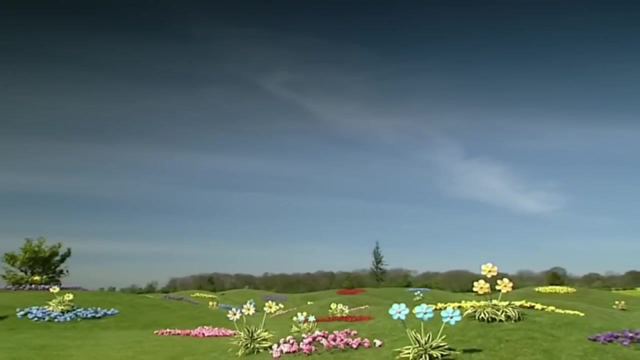 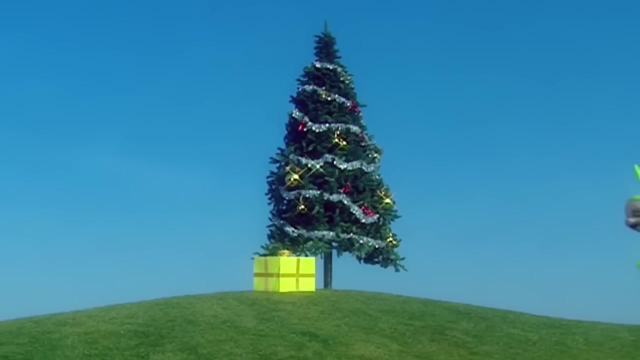 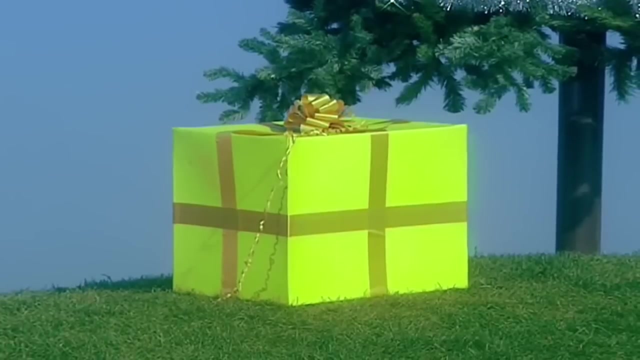 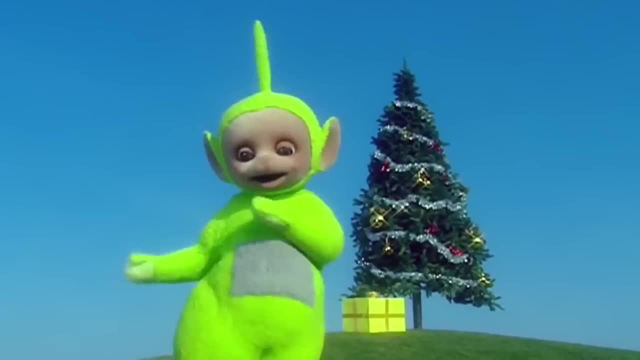 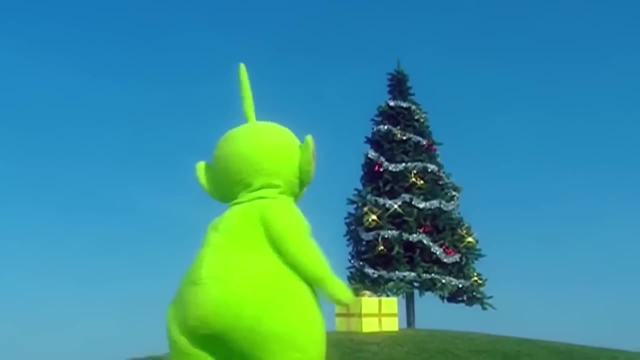 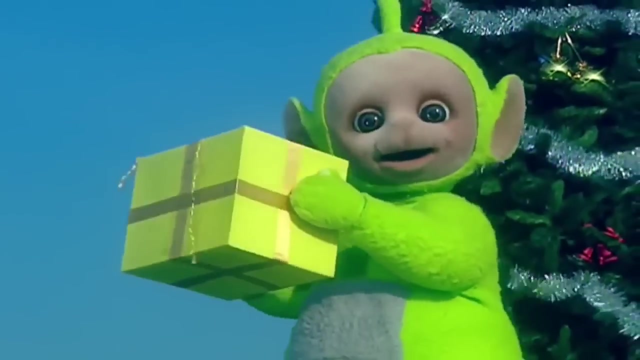 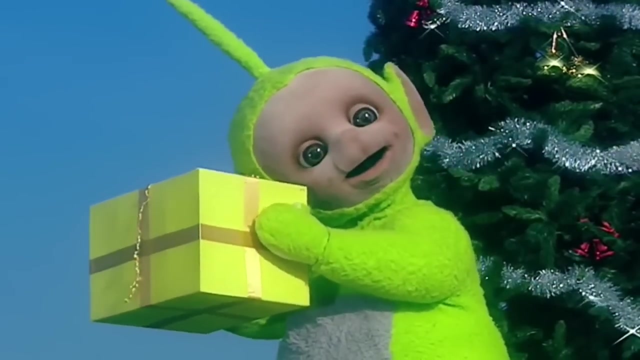 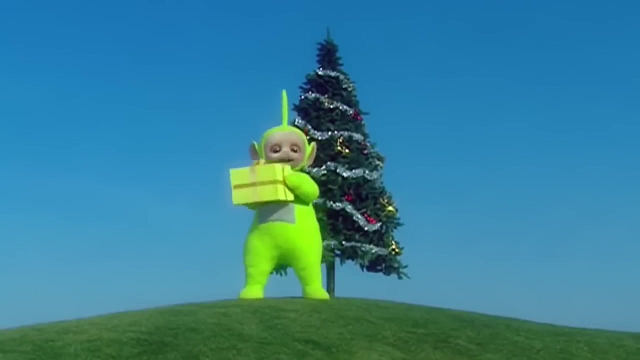 Dipsy brought a present. present. present. Dipsy brought a present. Dipsy brought a present. Dipsy brought a present Mm Present Hot, Ooh, Mm Hot, Present. present. Dipsy brought a present. 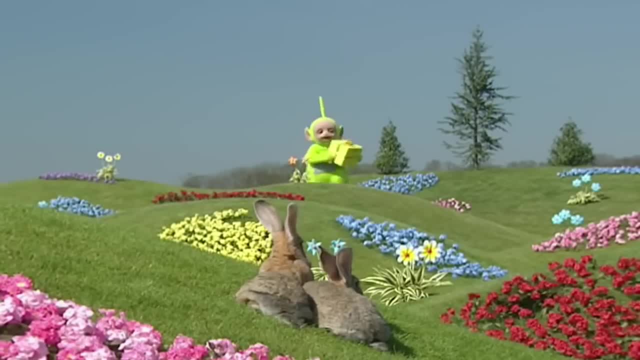 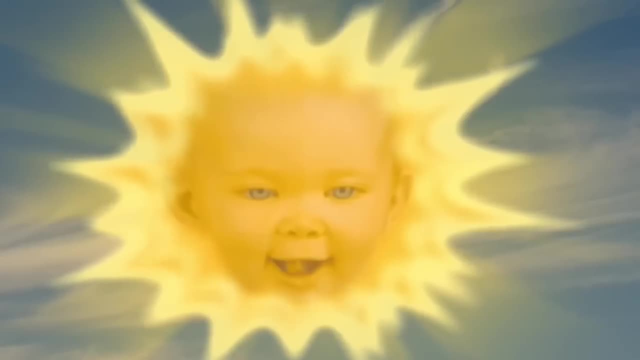 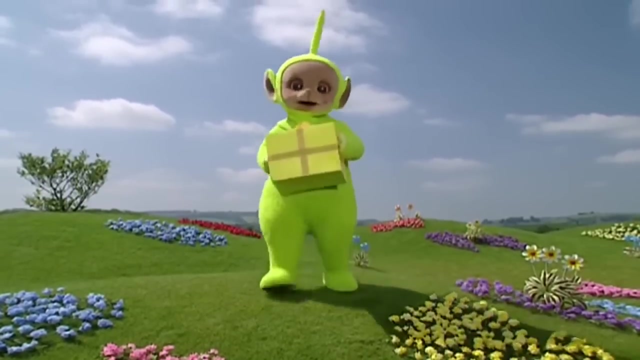 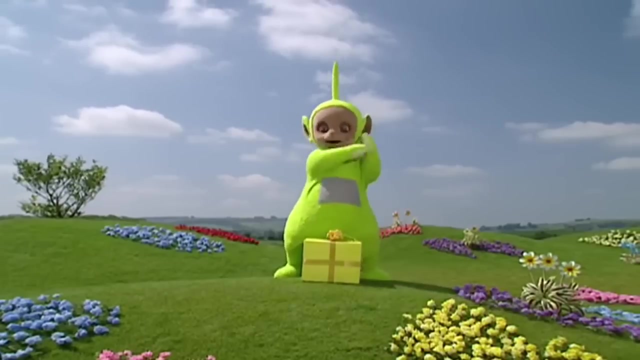 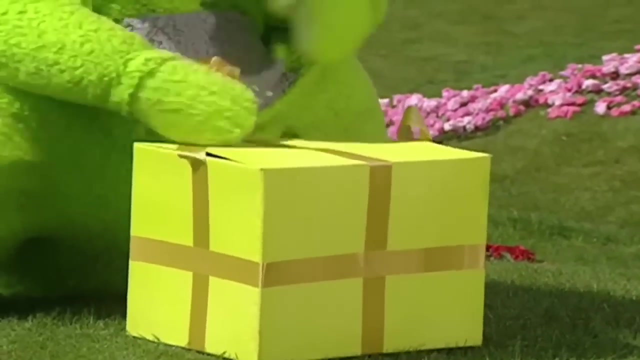 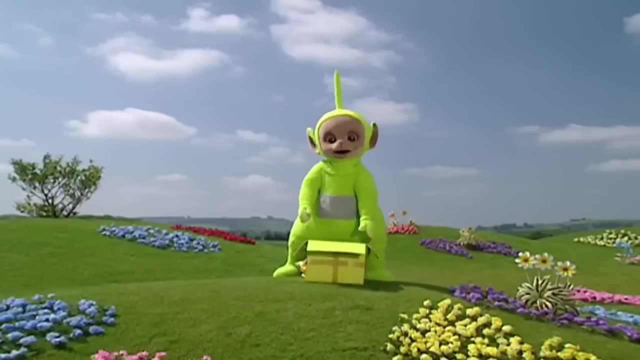 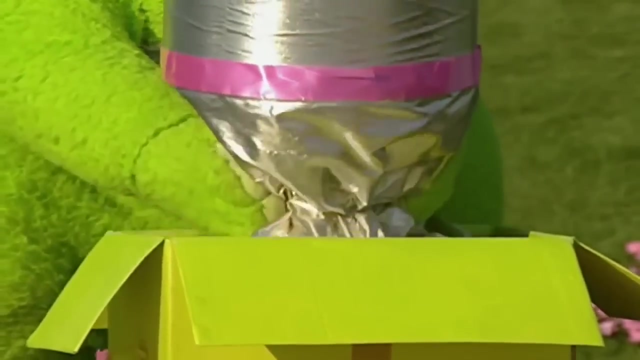 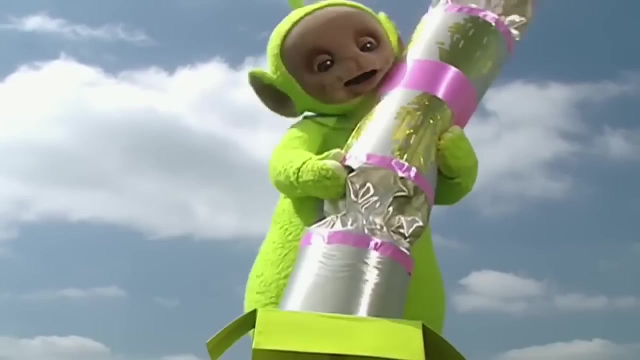 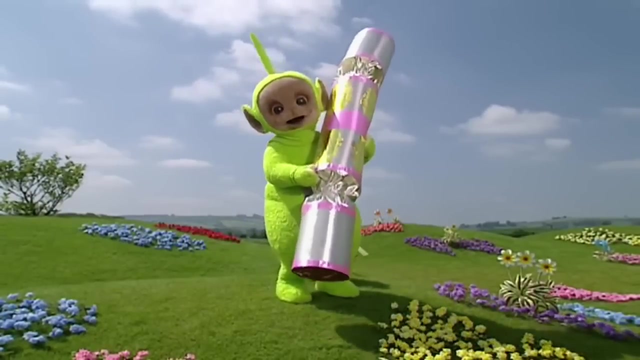 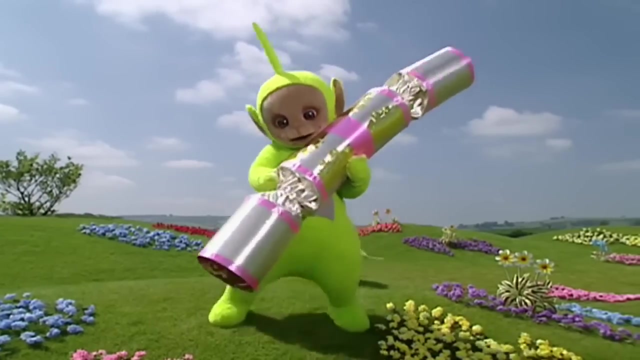 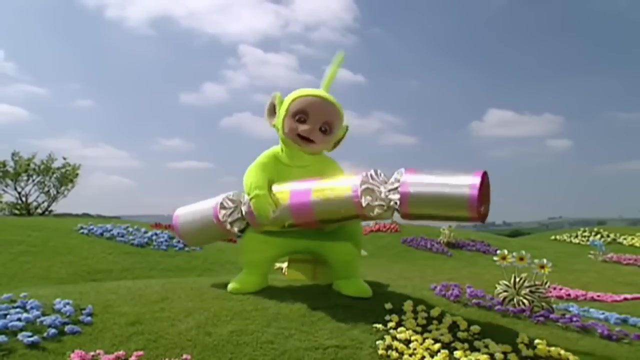 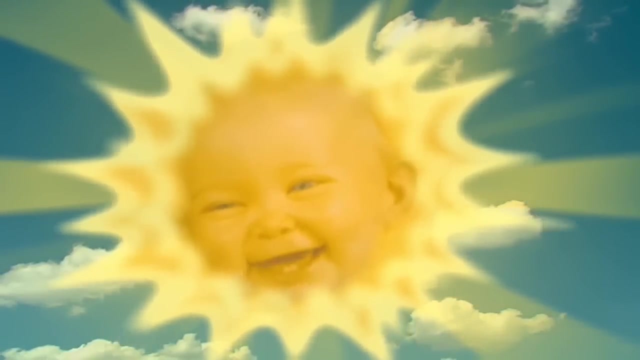 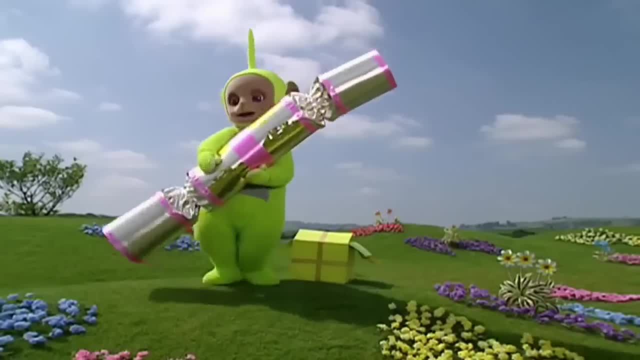 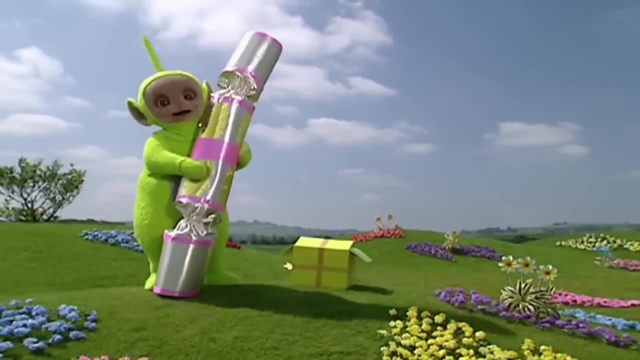 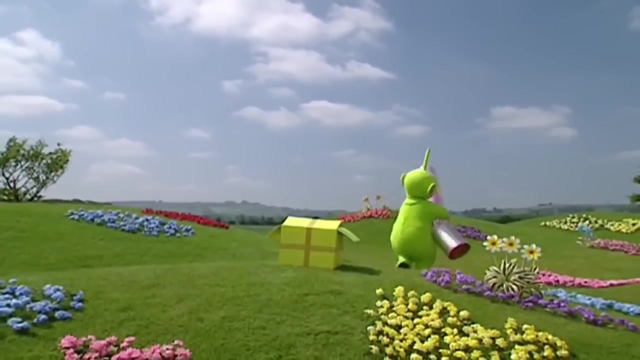 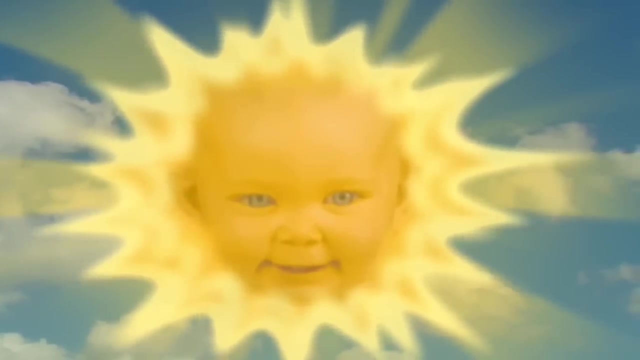 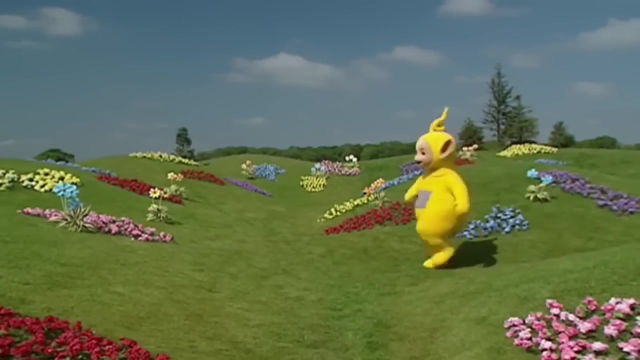 lollilalila, lollila, lollilala lollila La li, la li, la, La, la, li, la li, la. Uh-oh, Quack, quack, quack, quack. 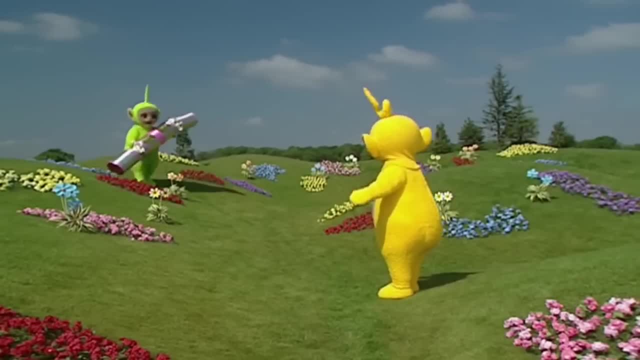 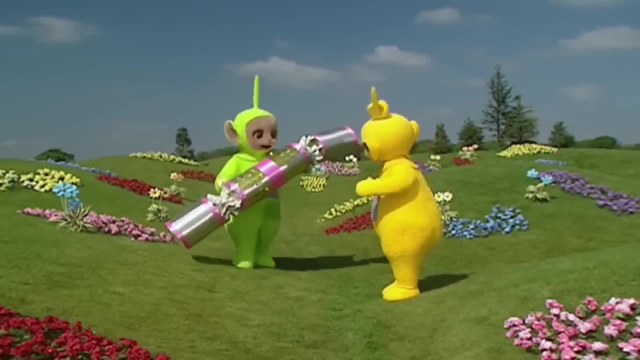 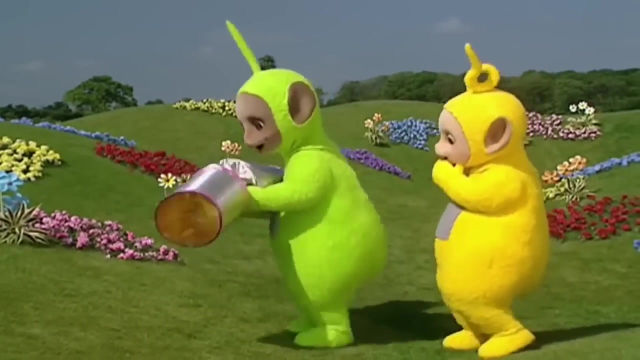 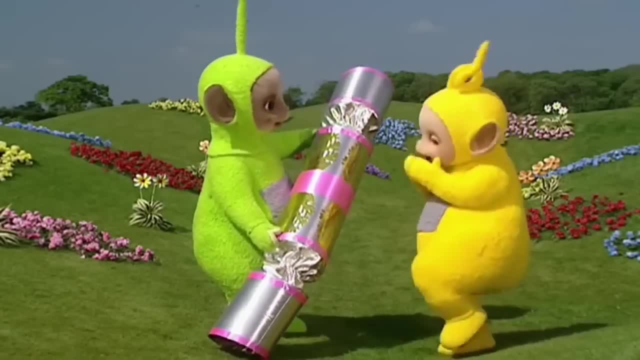 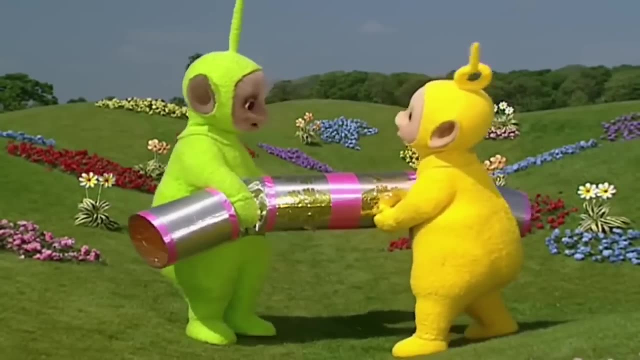 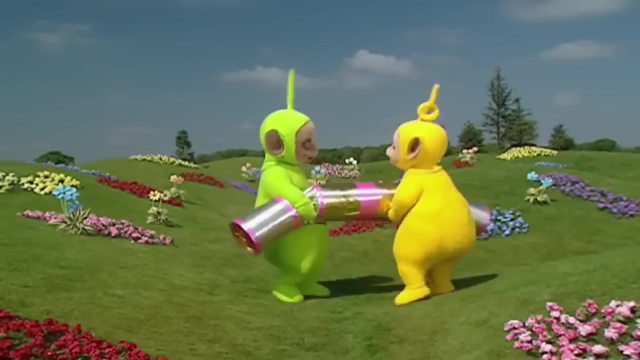 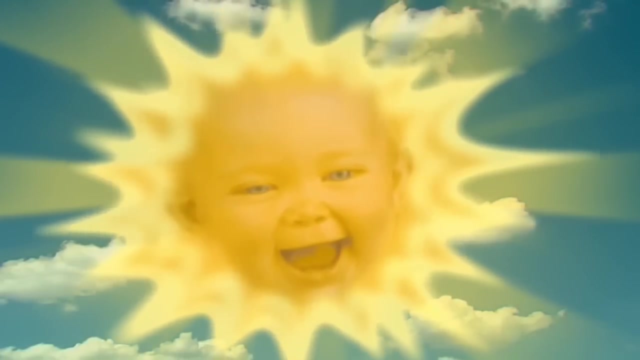 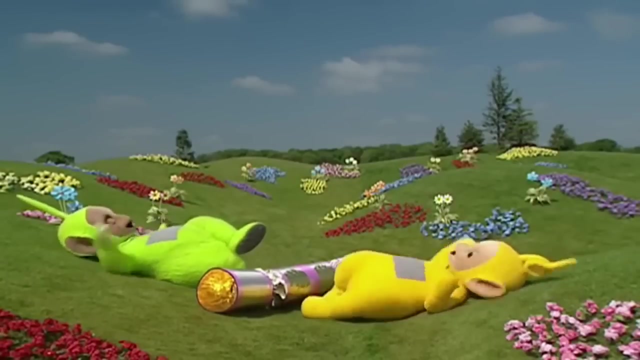 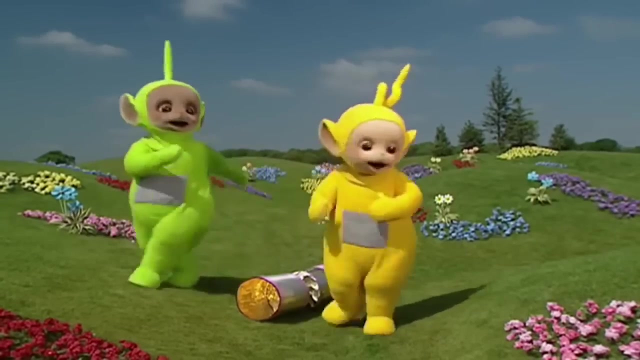 La-La help Dipsy. Yes, Dipsy and La-La pulled as hard as they could, Pull, Pull, Pull, Pull. But Dipsy and La-La weren't strong enough to pull the cracker. Dipsy and La-La are not strong enough. 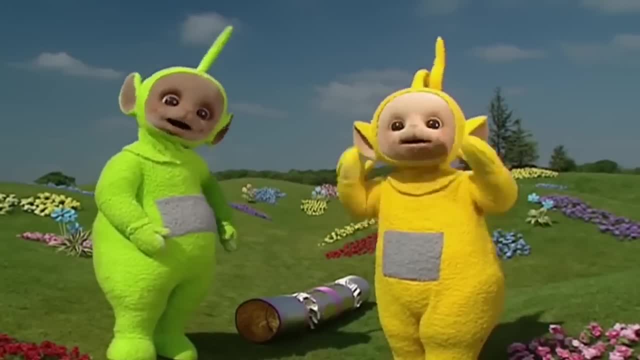 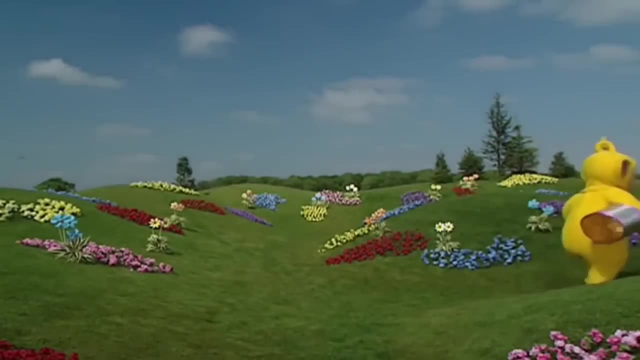 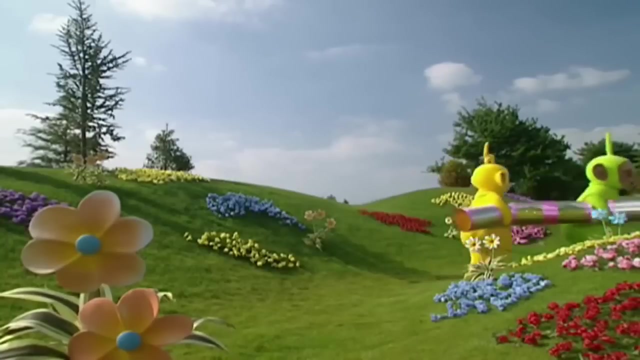 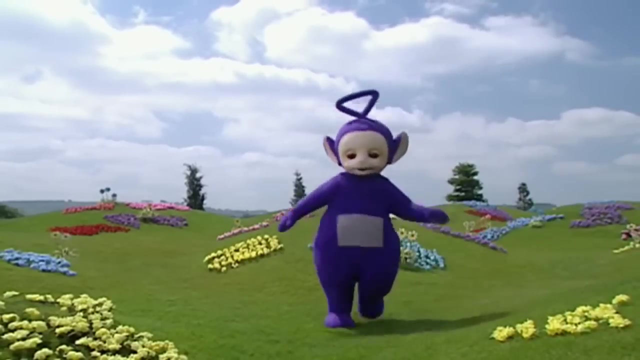 So they looked for someone else to help. Oh, Winkle winkle, tinky winky, pinky winkle. Uh-oh, Winkle, winkle, tinky, winky, pinky winkle. 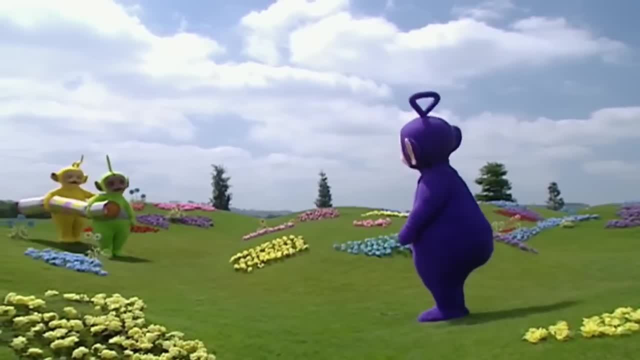 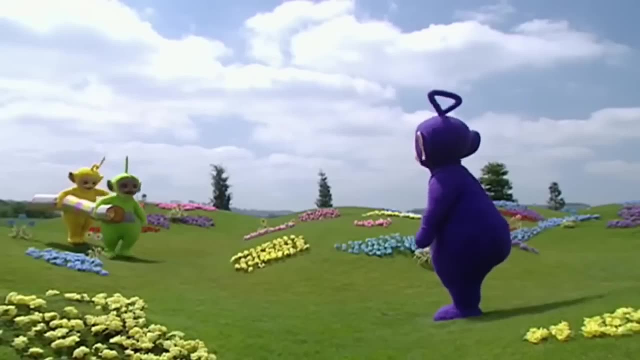 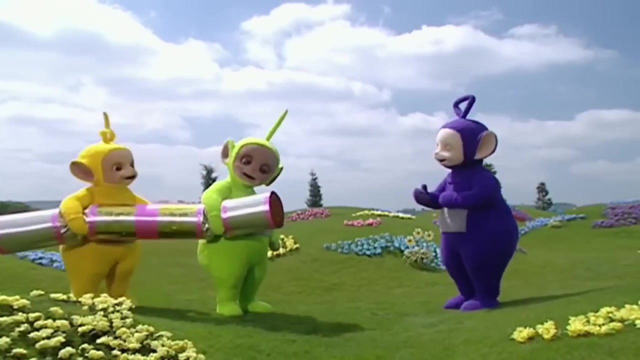 Winkle winkle tinky winky, pinky winkle. Oh, Tinky winky, Tinky winky, Winkle winky. Yes, Oh Oh. Dipsy and La-La asked Tinky Winky if he would help to pull the cracker. 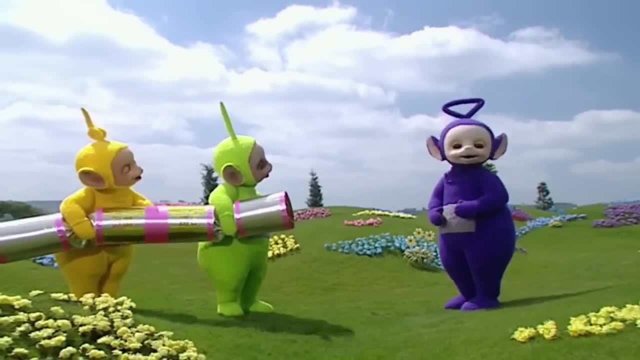 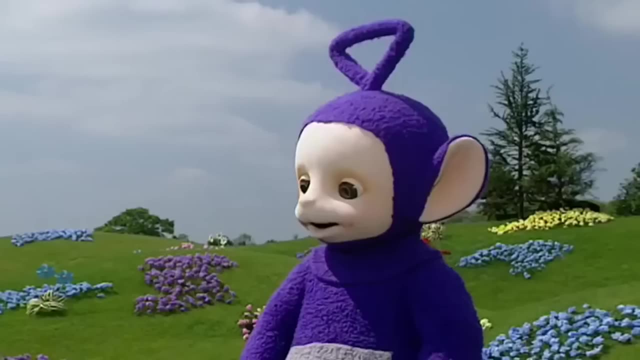 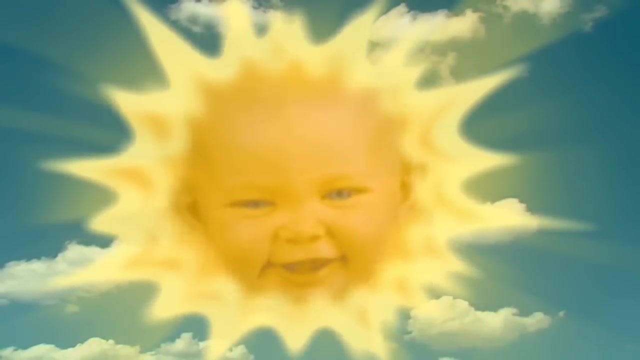 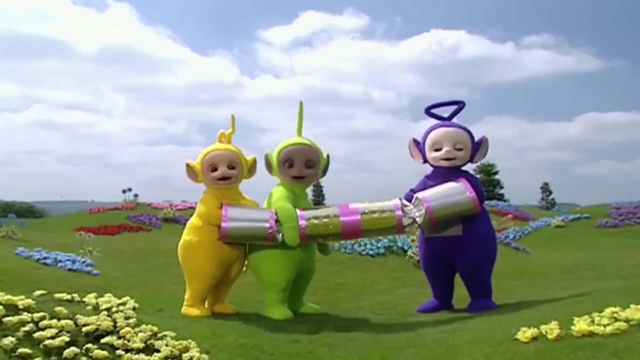 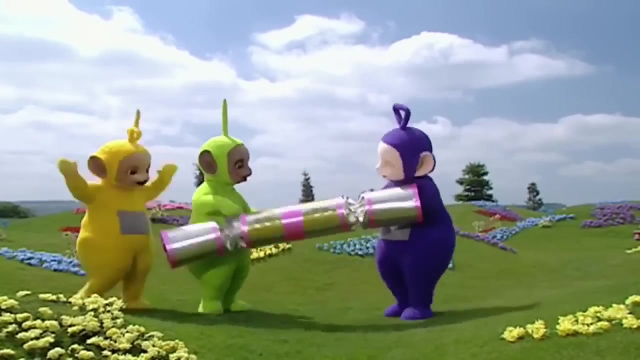 Tinky winky make a happy little cracker. Yes, Yes, Yes, Dipsy and La-La and Tinky Winky pulled as hard as they could Pull, Pull, Pull, Pull, Yeah, Go, go go. 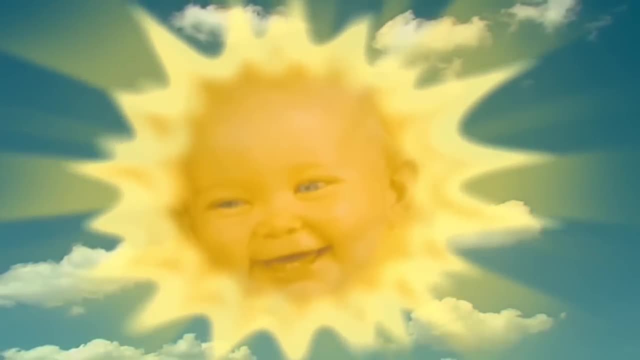 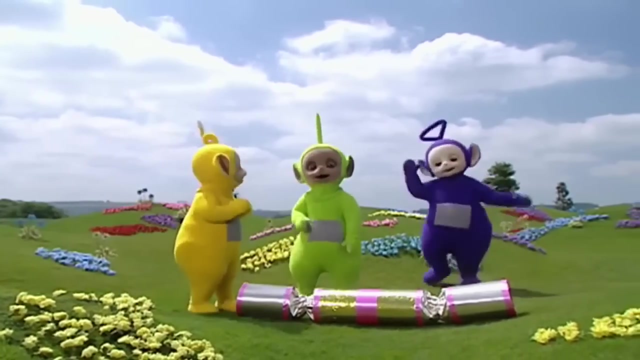 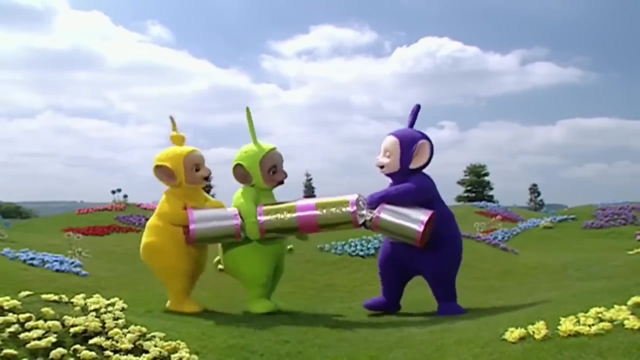 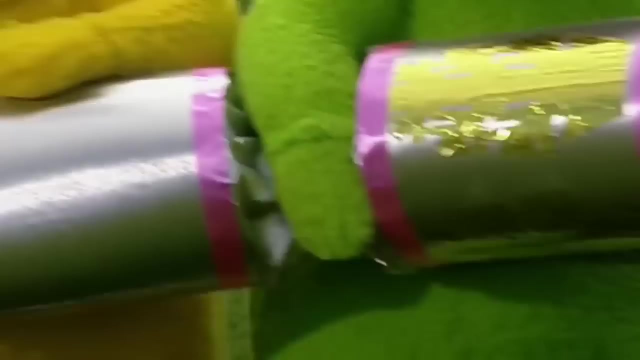 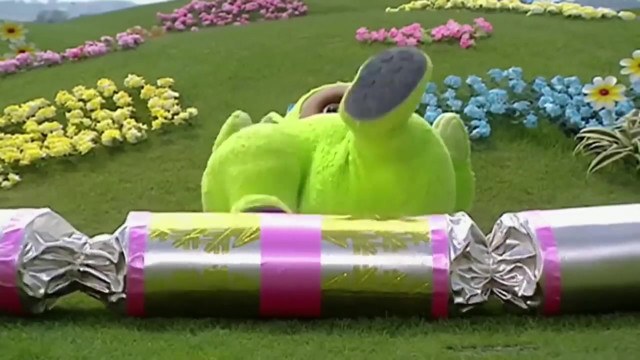 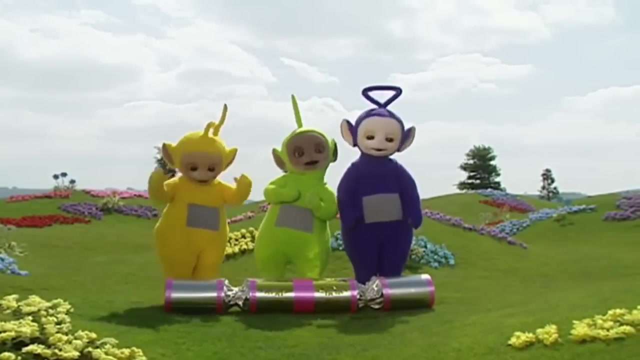 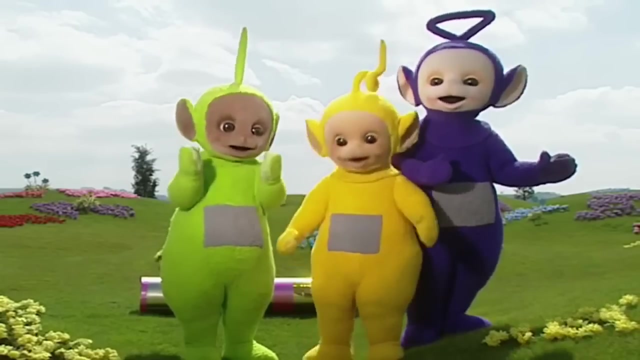 Don't, don't, Don't, don't, Pull Again, again, again, again. But Tinky, Winky, Dipsy and Laa Laa weren't strong enough to pull the cracker, So they looked for someone else to help. 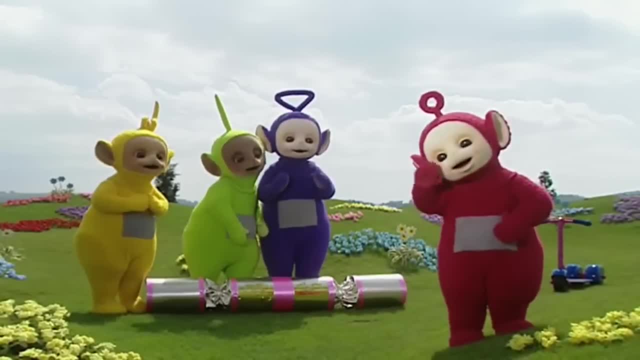 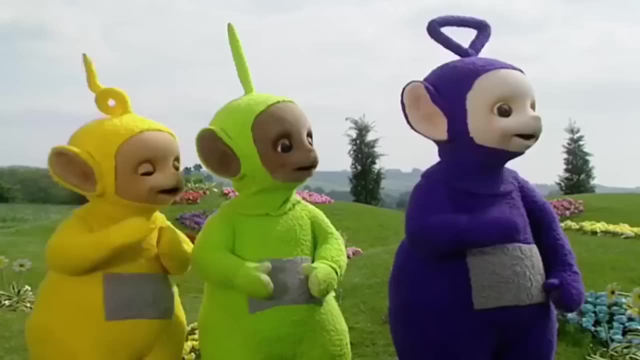 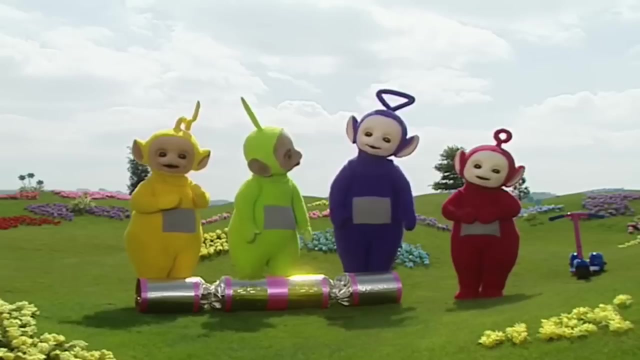 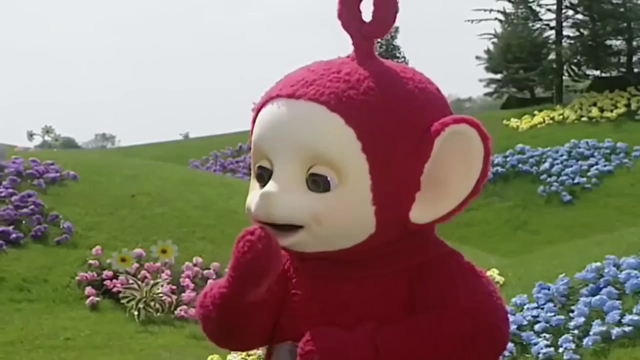 Tinky, Winky, Dipsy and Laa. Laa asked Poe if she would help to pull the cracker. Yes, Yay, Hooray, Hooray, Hooray, Hooray, Hooray, Hooray. 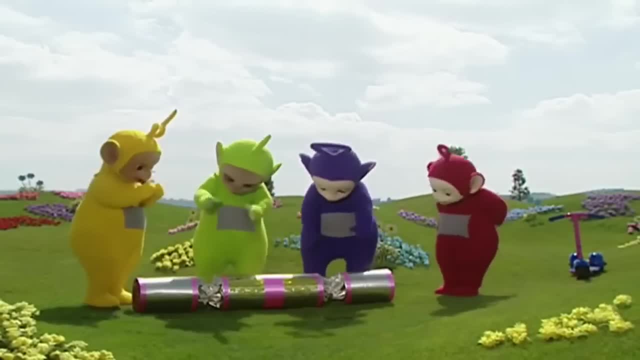 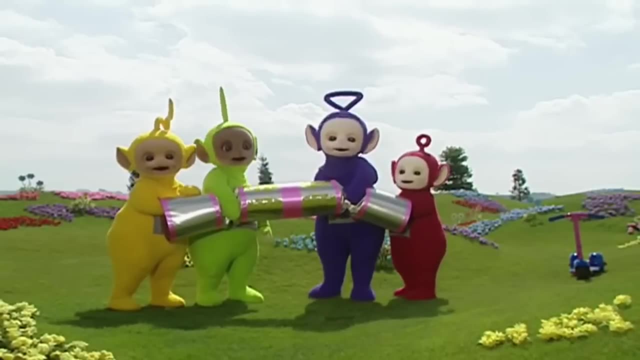 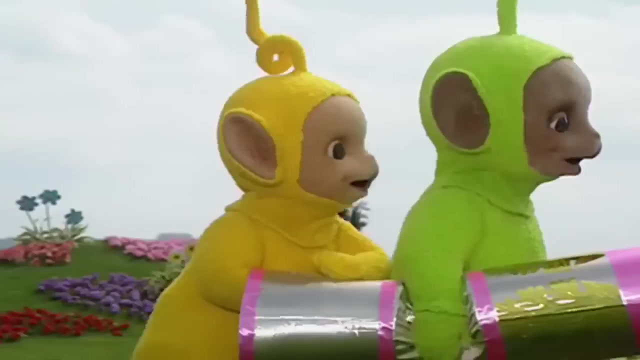 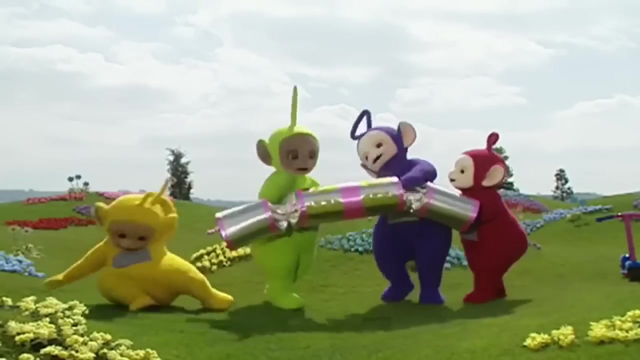 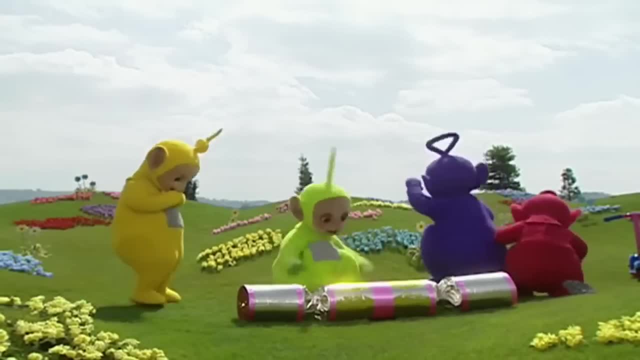 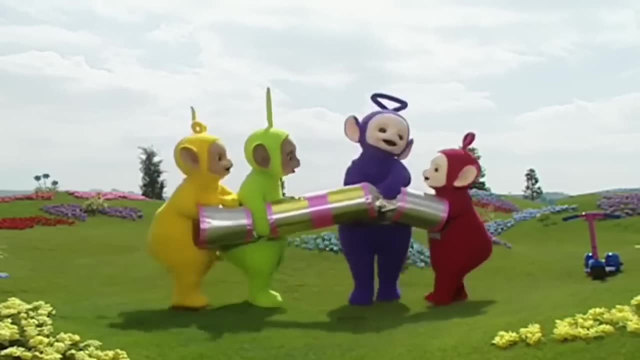 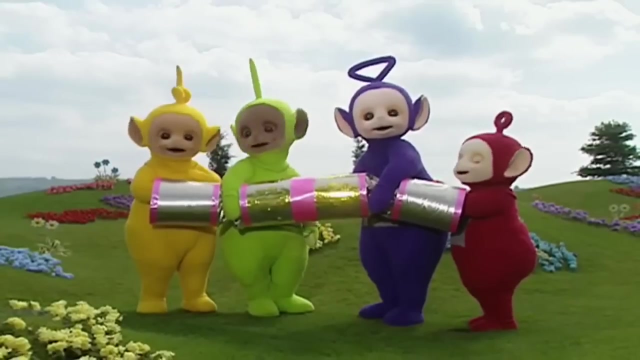 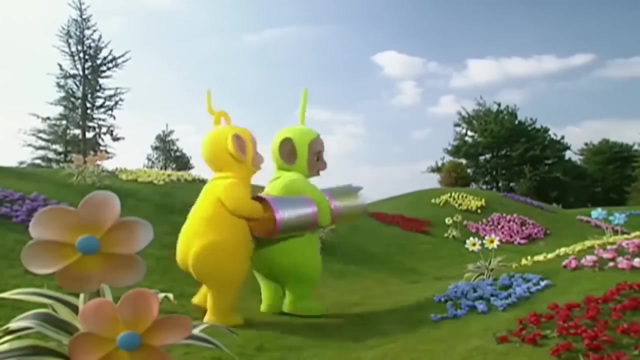 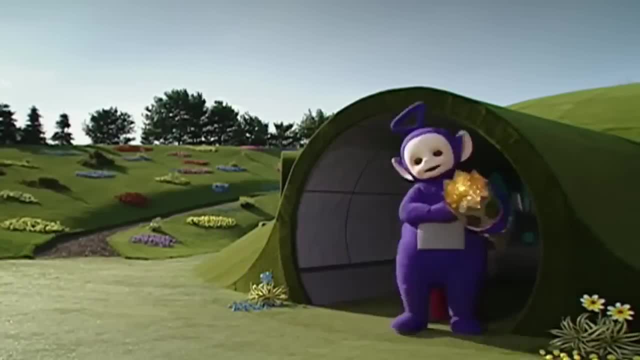 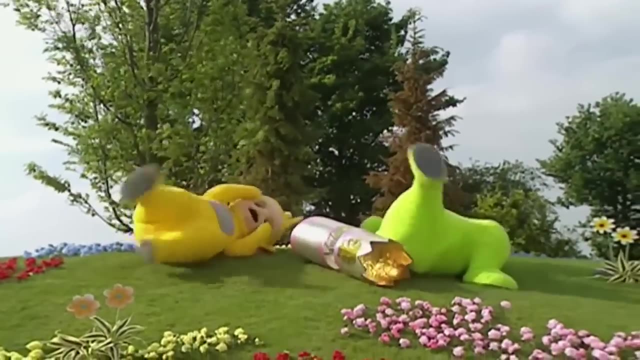 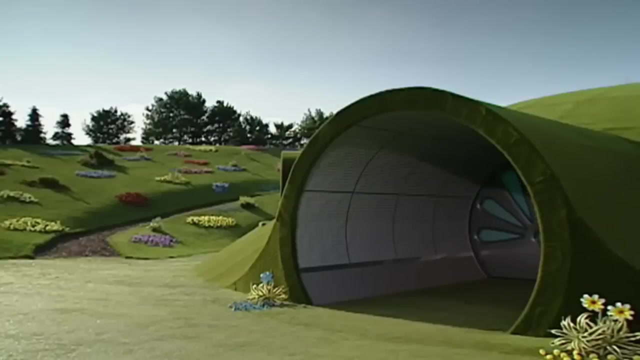 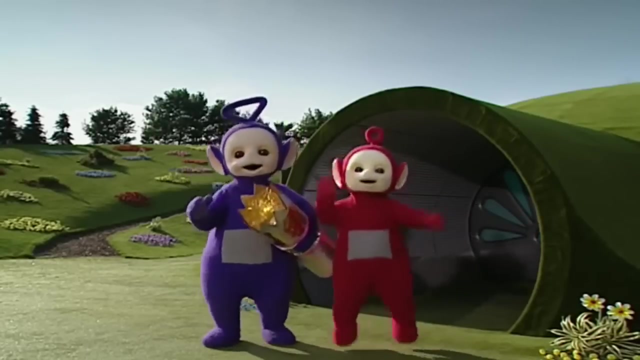 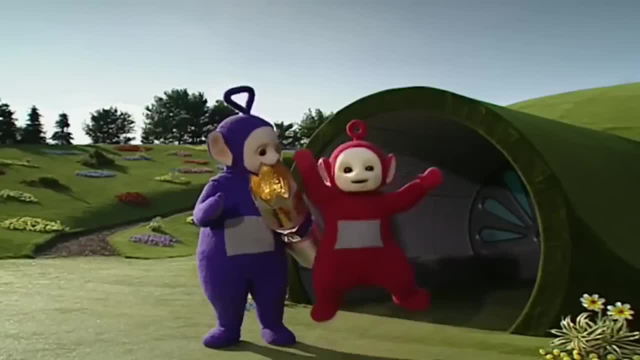 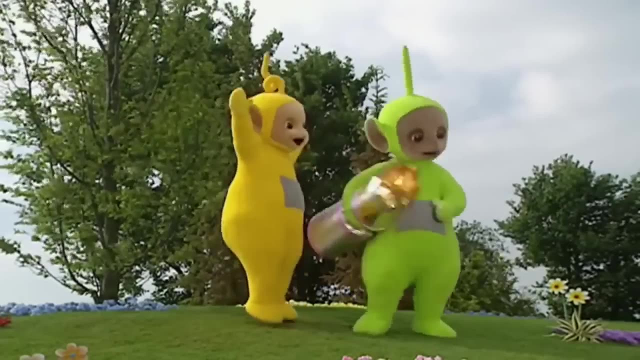 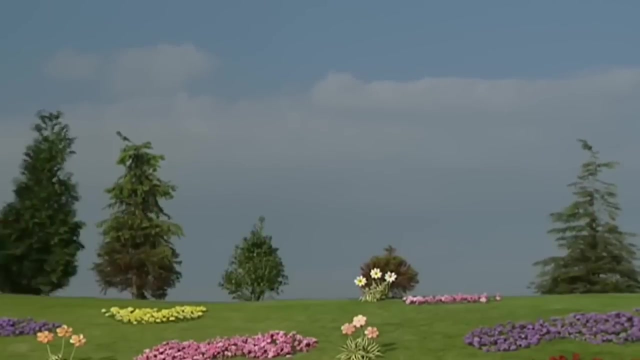 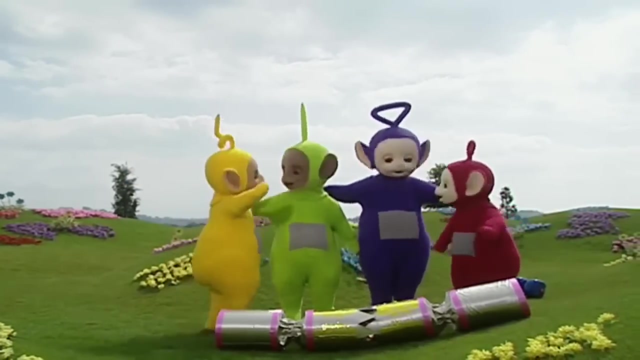 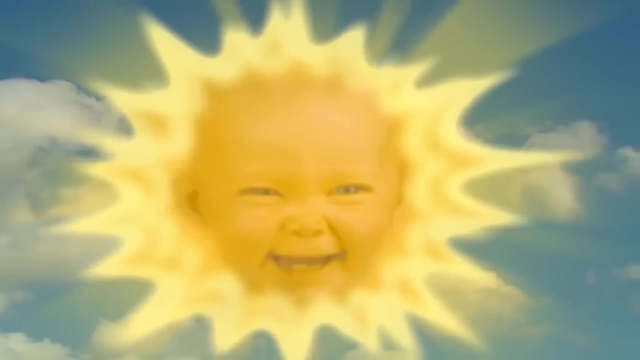 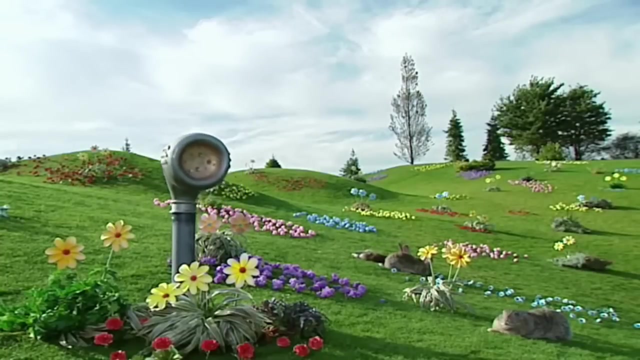 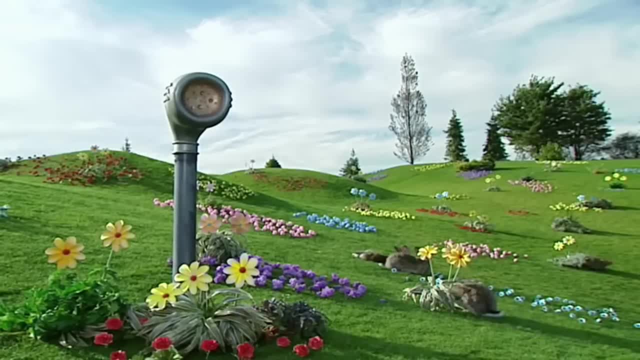 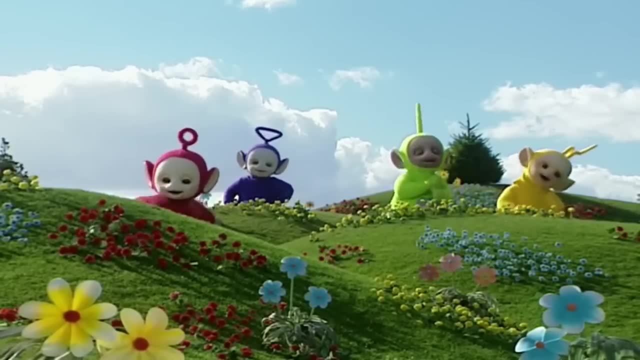 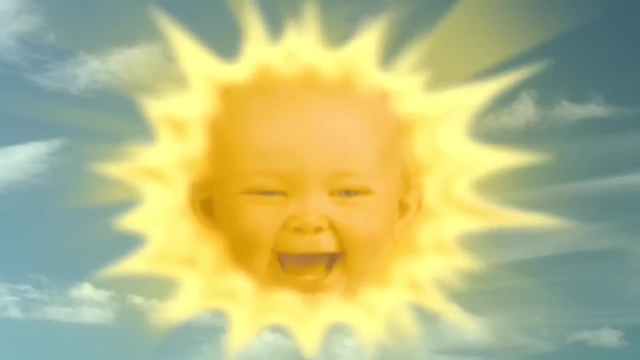 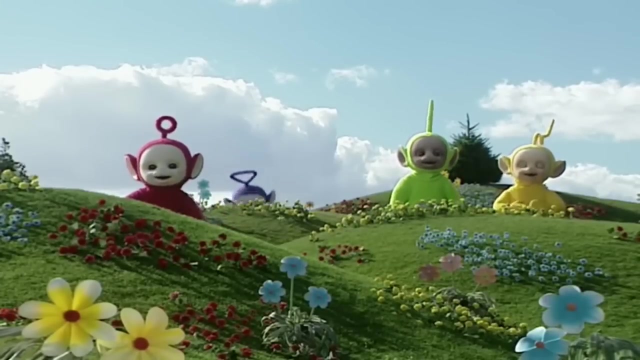 Time for tubby. bye-bye, No, No, No. Bye-bye Tinky Winky. Bye-bye, Bye-bye Dipsy. Bye-bye, Bye-bye Lala. Bye-bye, Bye-bye Poe. 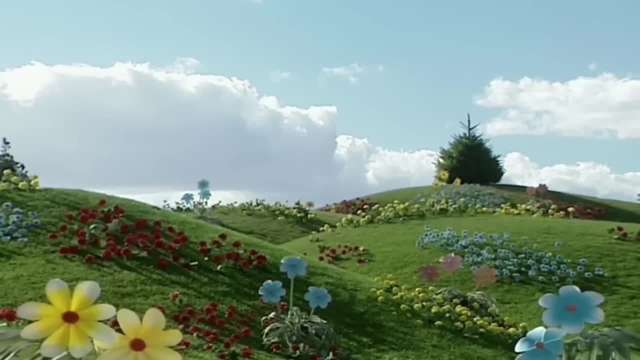 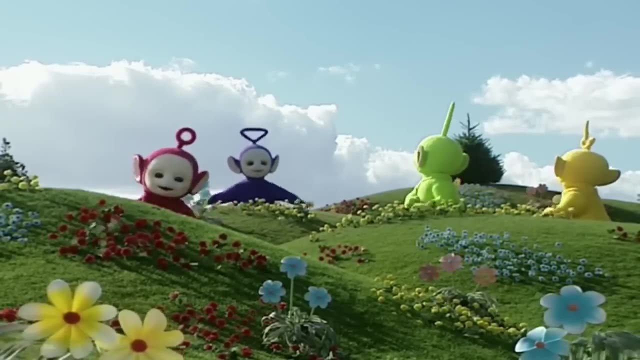 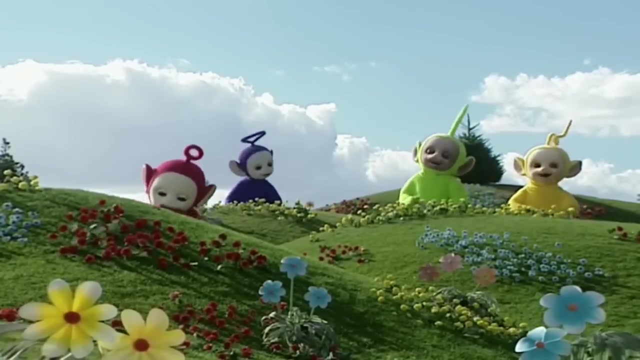 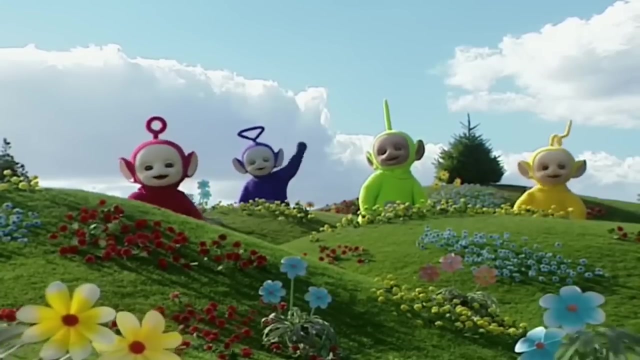 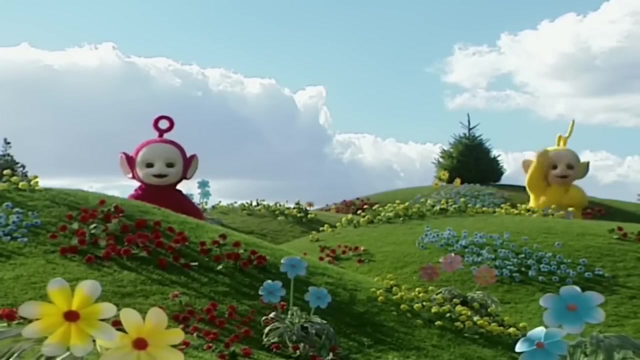 Bye-bye. Poe Poe, Poe, Poe, No, No, No. Bye-bye. Tinky Winky. Bye-bye, Bye-bye Dipsy Bye-bye, Bye-bye Lala Bye-bye. 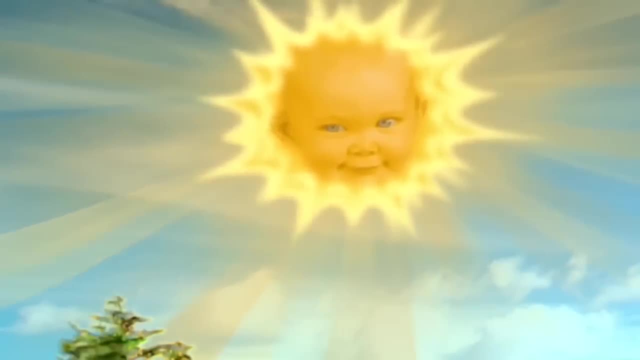 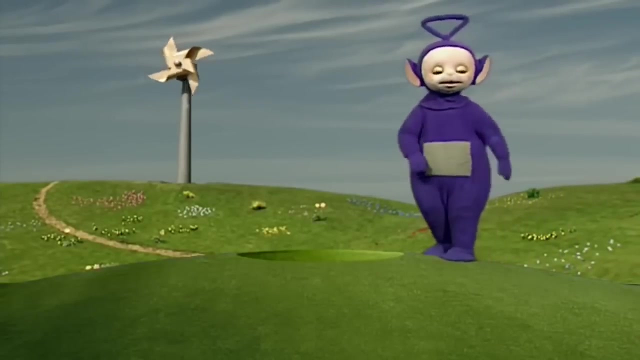 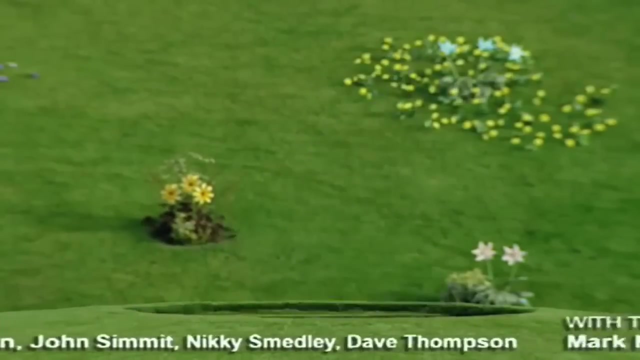 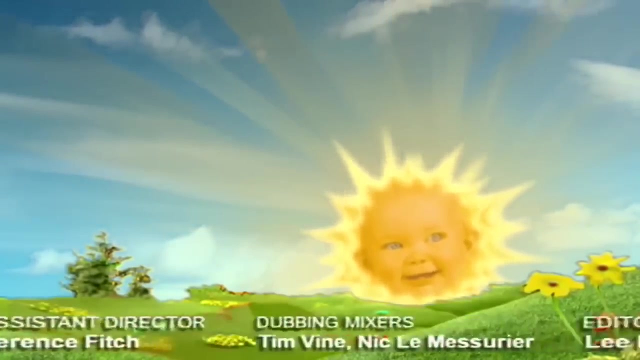 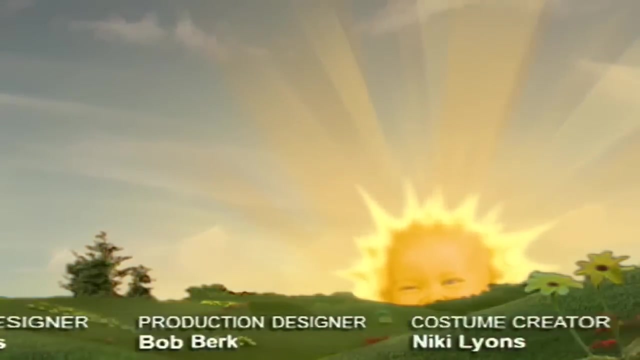 Bye-bye, Poe, Bye-bye. The sun is setting in the sky. Teletubbies say goodbye, Bye-bye, Bye-bye, Bye-bye, Bye-bye, Bye-bye, Bye-bye, Bye-bye.